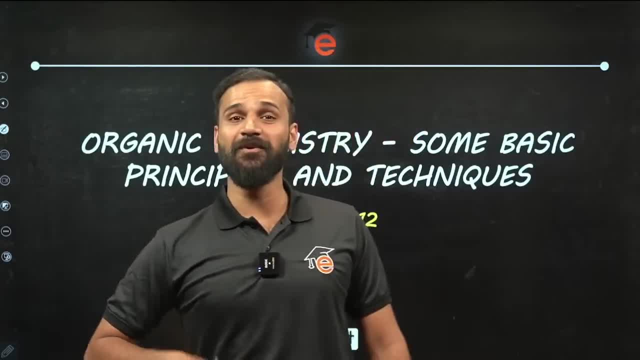 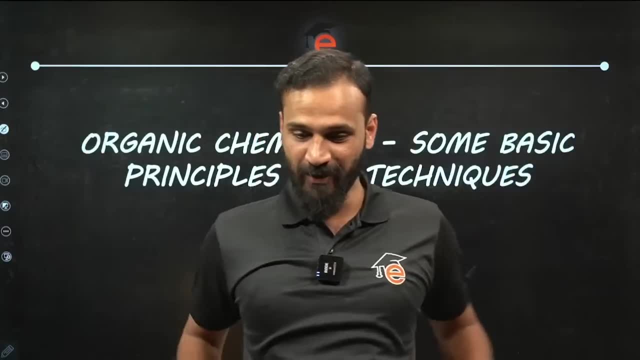 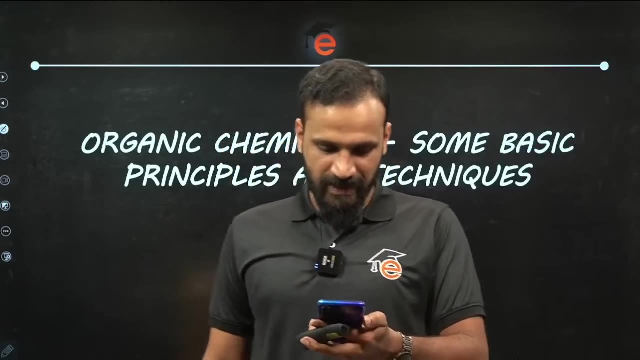 has some basic principles and techniques. There are also hydrocarbons, right In that, the first chapter to learn. is everyone ready, guys? Is everyone ready? If you are ready, please comment quickly. If everyone is ready, please comment quickly. Yes, everyone is ready, right. 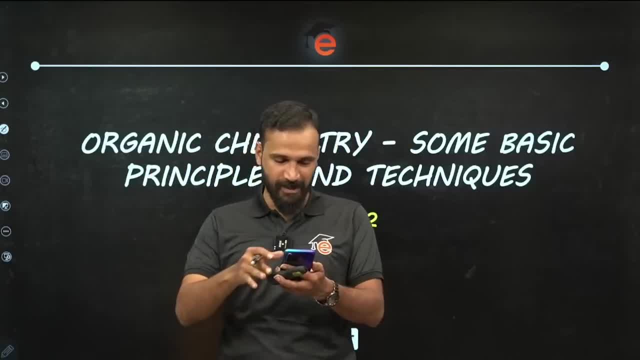 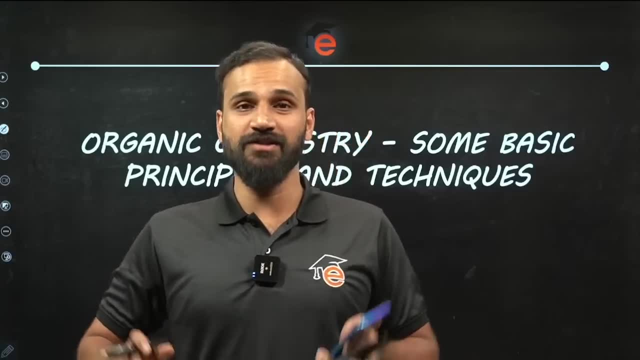 Please comment quickly, guys. Hi hi, hi, hi, hi. Yes, good evening, good evening, all of you, Good evening, good evening. Everyone has a glass of water, a note, a pen and a paper and is set up. We have to. 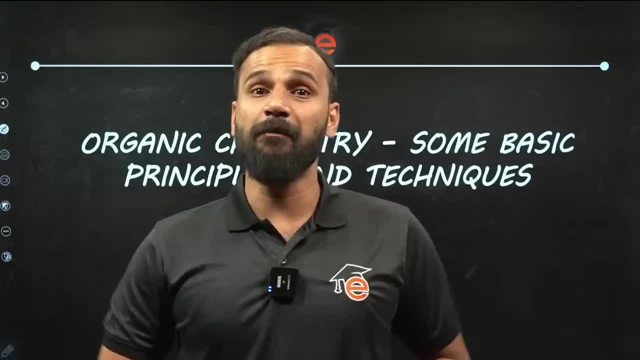 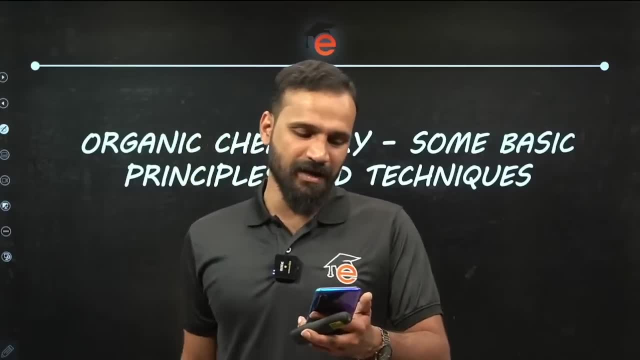 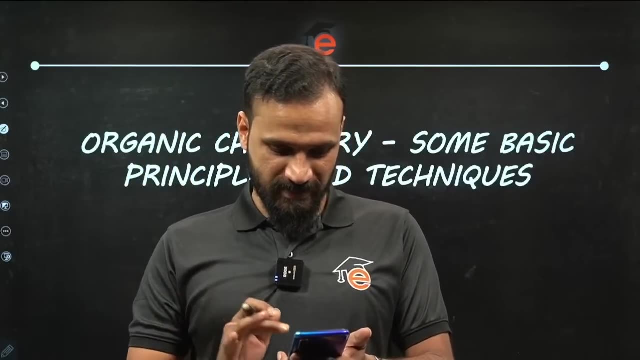 finish this chapter very quickly, very quickly. We have already studied this for the Christmas exam. Some people, some people have not studied. It's okay, We are going to study this thoroughly. We are going to study thoroughly, Yes, Yes, Tomorrow, this chapter exam. 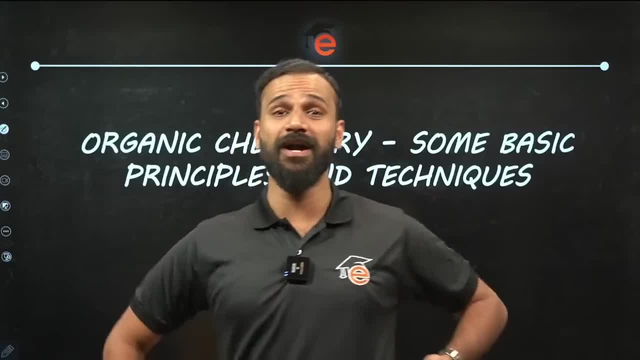 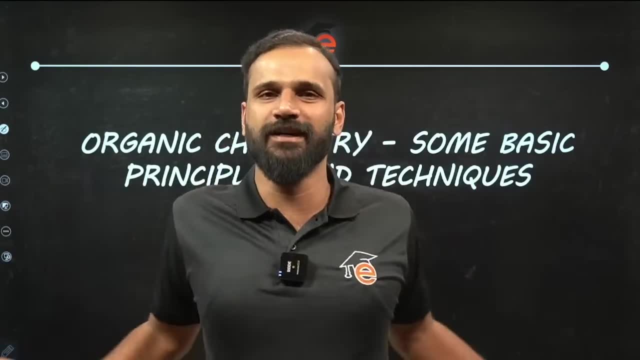 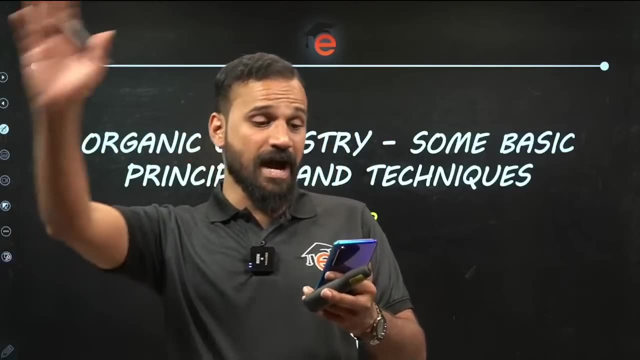 is live. Surely, you will find this very helpful, I am sure. Yes, it's a big chapter. It's a big chapter. We are going to discuss everything that is important in a very short time. Yes, Yes, Organic chemistry is set up, and 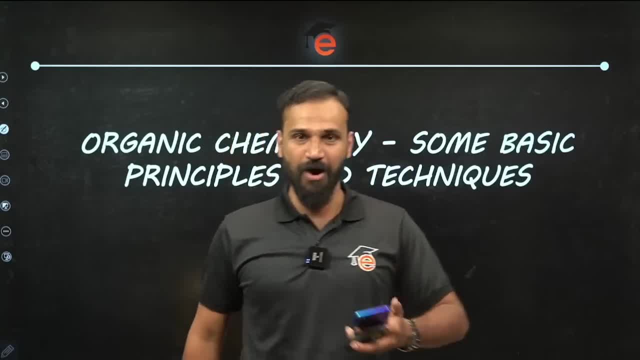 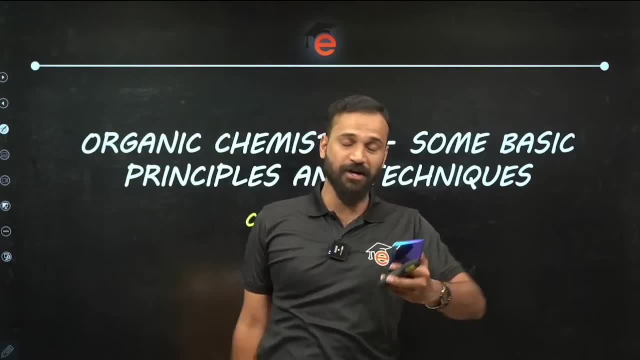 given to you. No one should be afraid of one. No one is afraid of one. No, We don't have to fear anything. Yes, So let's get started. Everyone, I hope everyone, is ready, Ready? If so, fire, fire, fire, fire. Let it come, Let's. 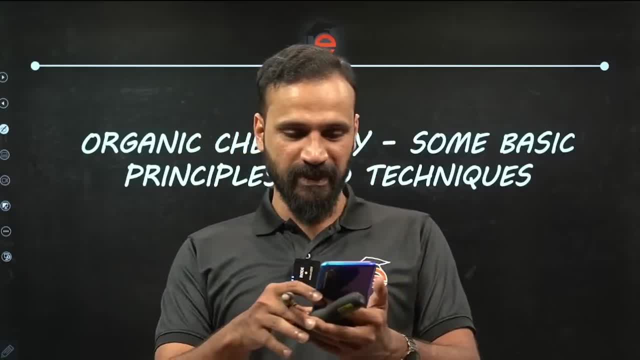 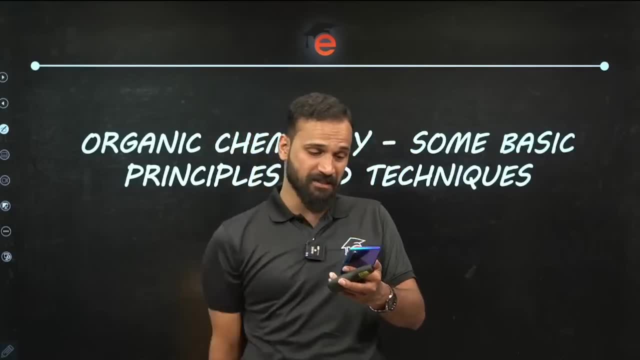 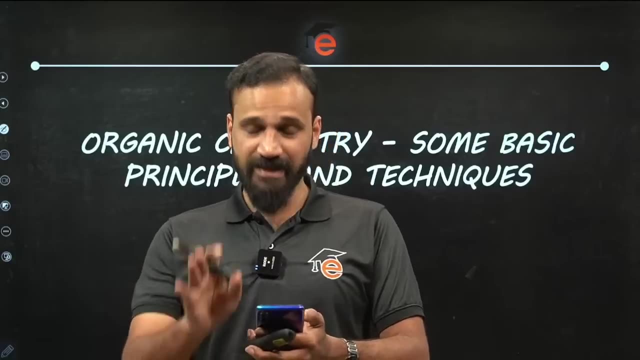 fill our chat box. Yes, Yes, Hello, Adityan Aditya, Hello, Yes, Yes, Yes, Yes, yes, yes, yes, The kids have taken over. the chat box is ready. You get in there. You want headshots? Yes, Yes, yes, yes, yes. 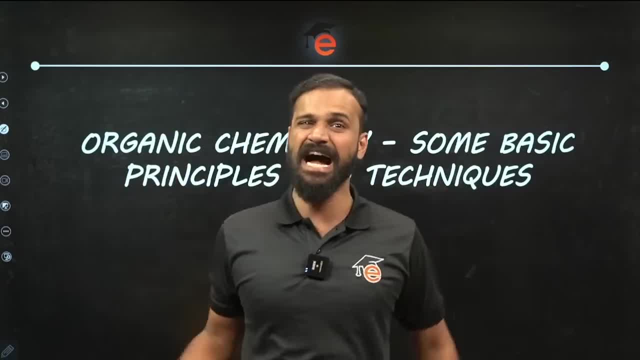 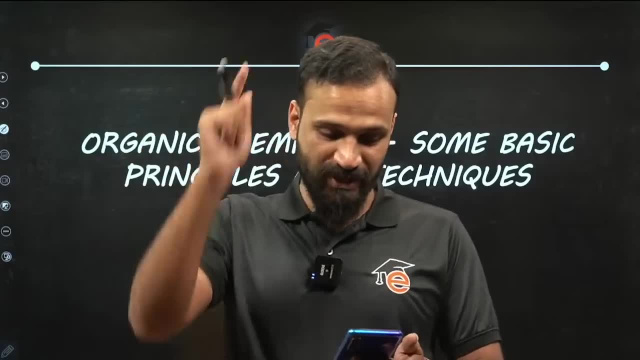 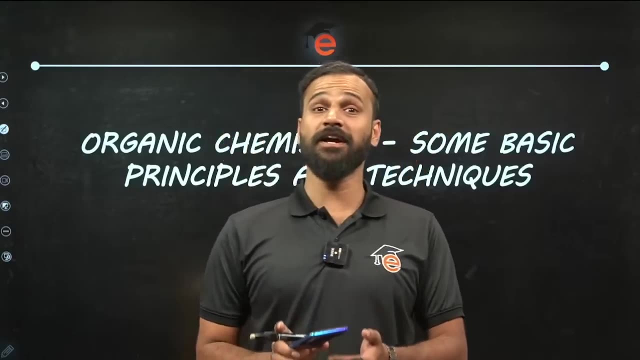 If you are ready to learn the first chapter of Organic, the chat box should be burning. Yes, Yes, Yes, Yes. Good, The chat box is burning Very good. The fires are burning Very good, Very good, Very good. 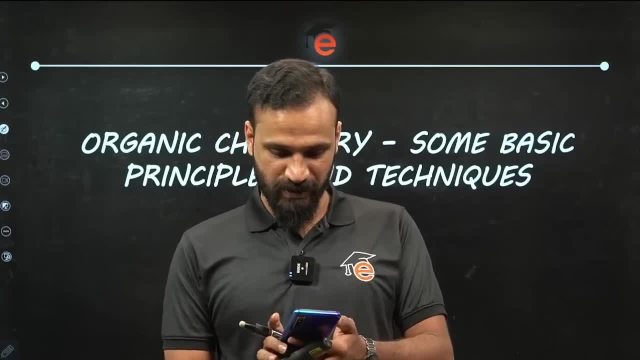 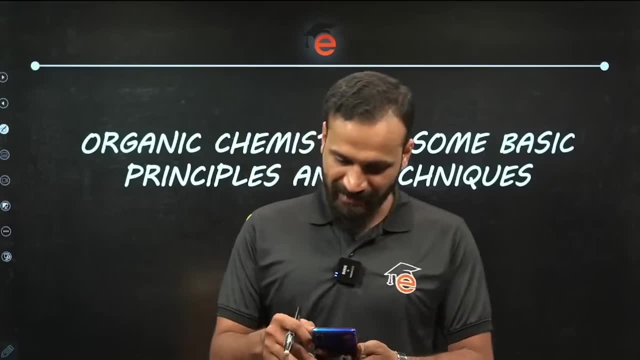 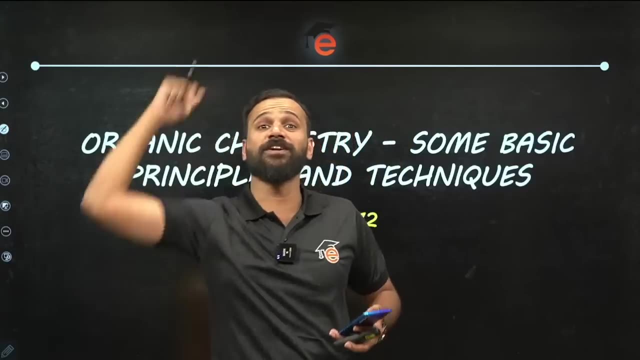 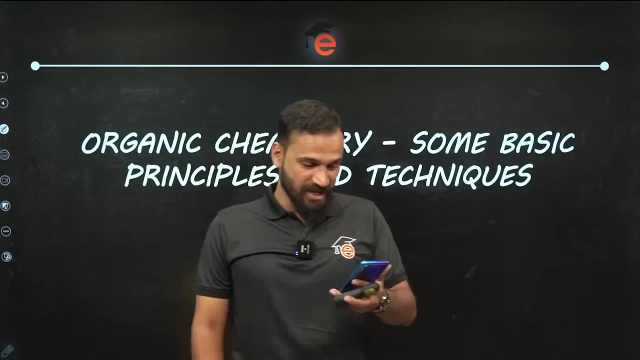 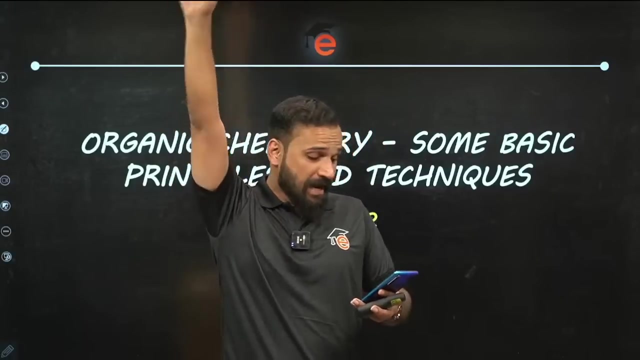 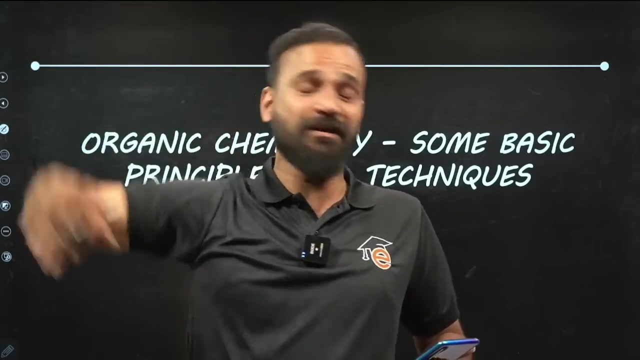 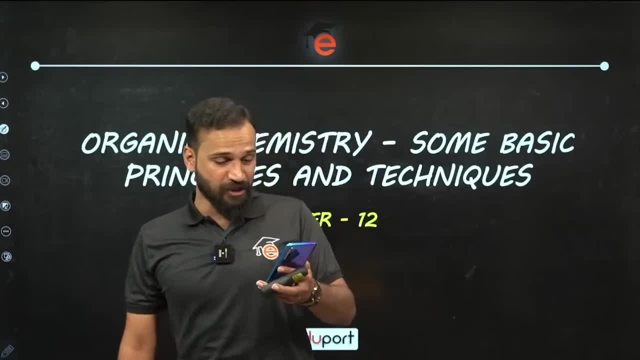 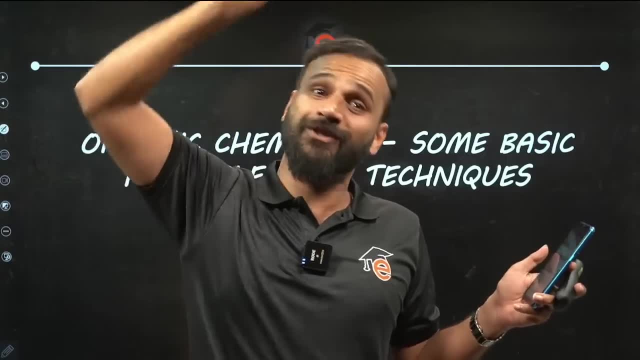 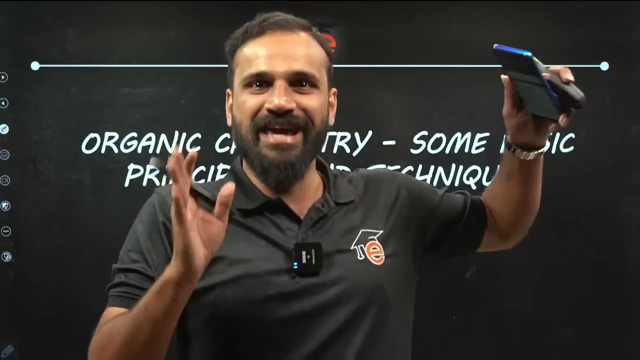 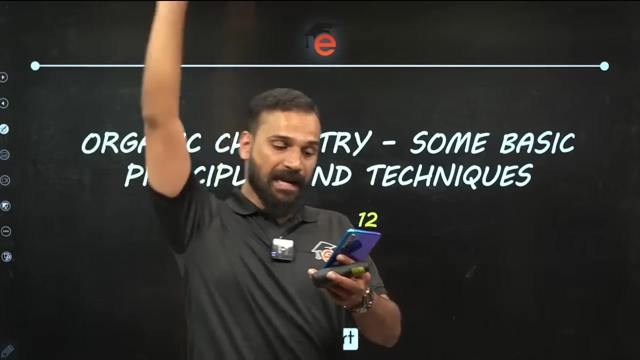 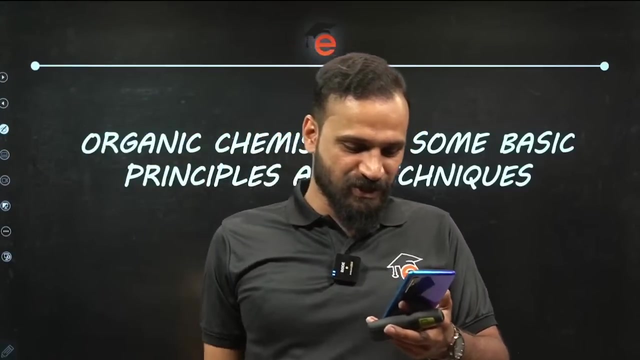 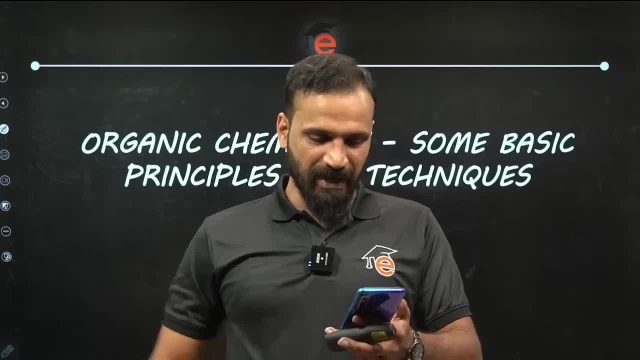 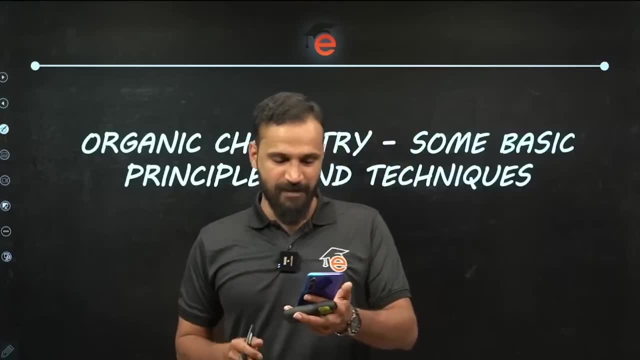 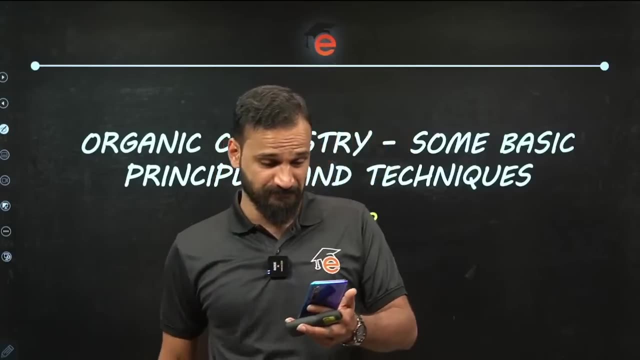 Yes, Children. did you share it to the group? Did you share it to your friends? If you gave, say you gave. If you gave, say you gave. Yes, Yes, Yes, Yes, Yes, Children, let it go completely. 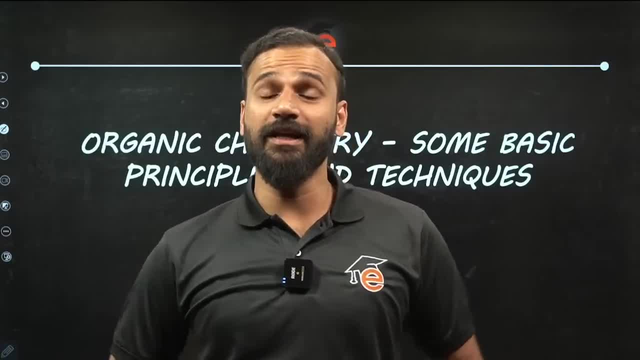 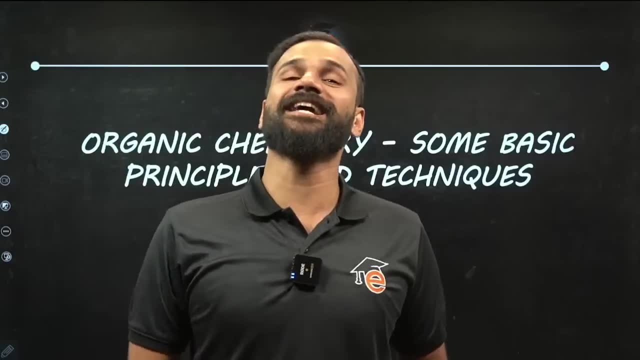 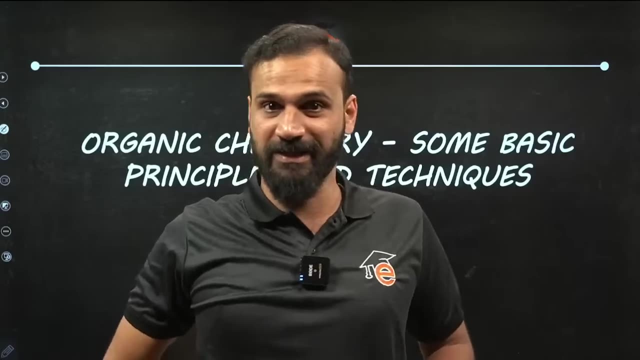 Please share it completely. Please share it completely. Today is Tuesday, children, After two days, there is a class of hydrocarbons. in the second chapter, after this, There is a class of hydrocarbons. You have to attend it thoroughly. 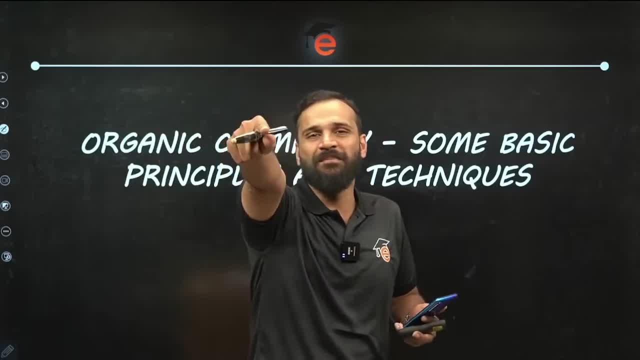 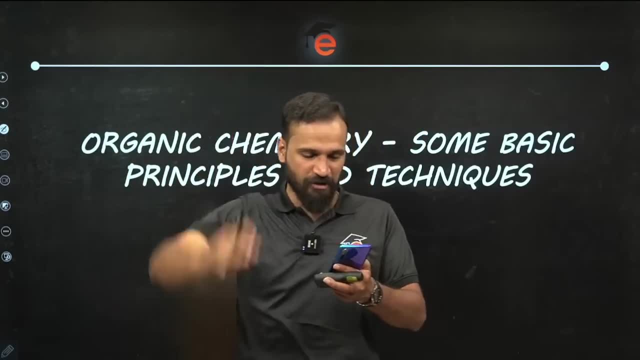 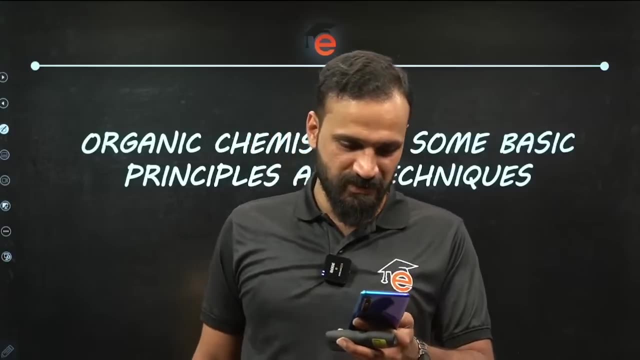 You have to be organic. You must be organic to be able to do this. You have to be able to come with confidence. Yes, You share it. Very good, Very good, Very good, Yes. Very good, Very good, Very good, Yes. 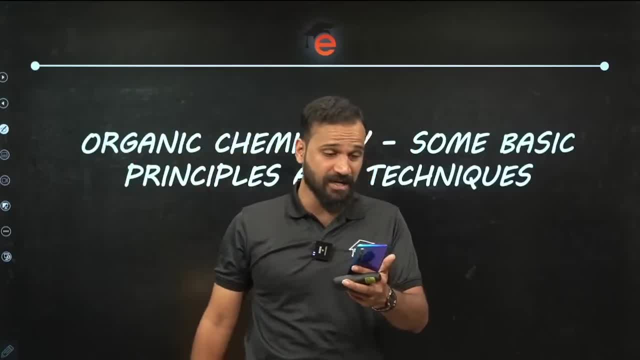 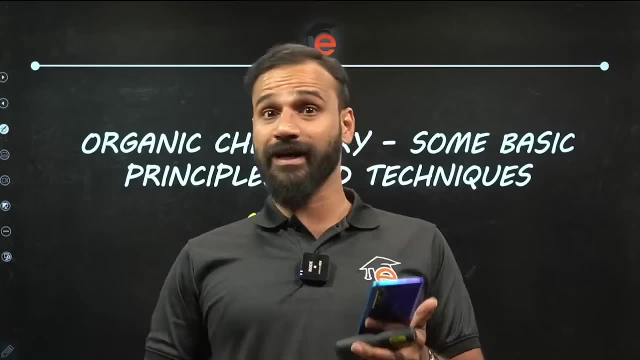 It has reached 900.. Children share 1k soon. 1k Yes. When will it be possible? I have to give you 2 to 2.5 hours is a big chapter. We can say it quickly. 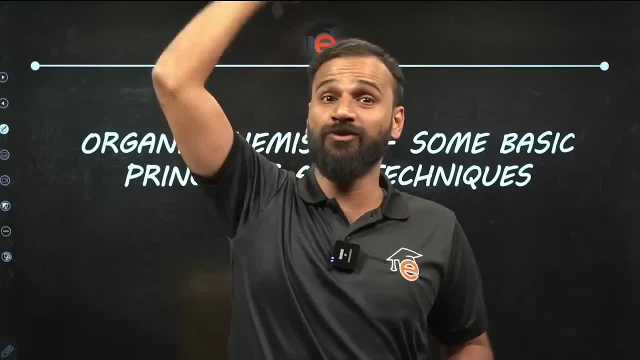 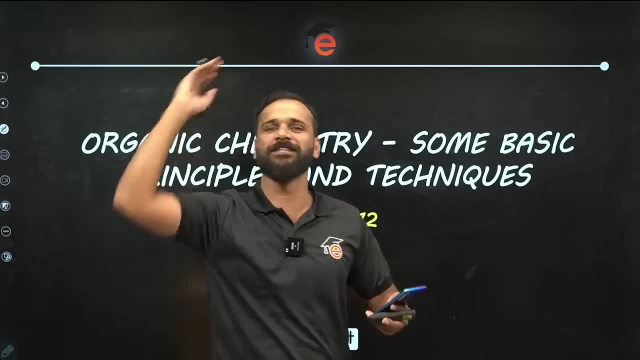 We can say it quickly. You have to be with me. Whatever I ask, you have to give a quick answer in the chat box. That's it? Yes, if that's the case, we can very quickly, very quickly, learn this chapter. 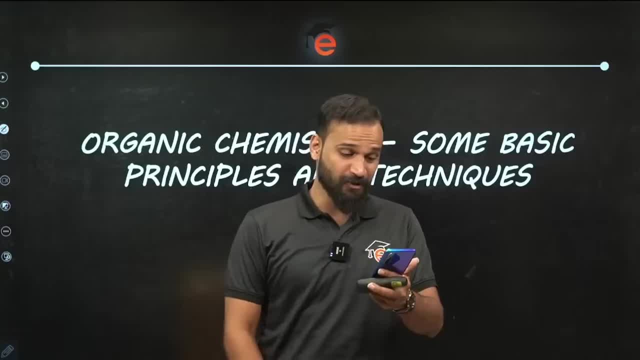 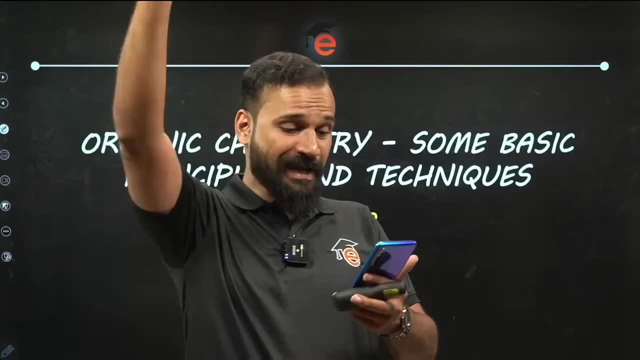 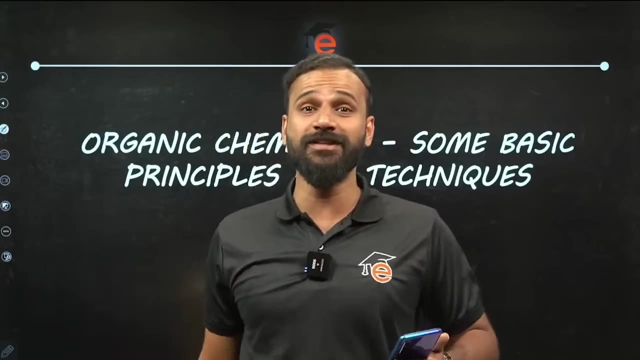 Yes, Yes, Gave. Many people shared it with friends. That's why our views are increasing. We are reaching 1k. Yes, Yes, Yes, New student Black says. a new student has joined in this, Black, you are welcome. You are welcome to Jupot. 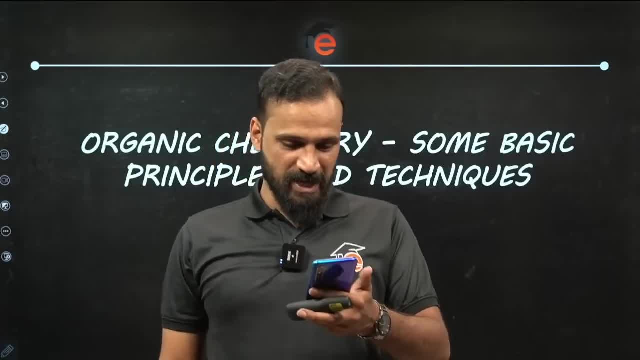 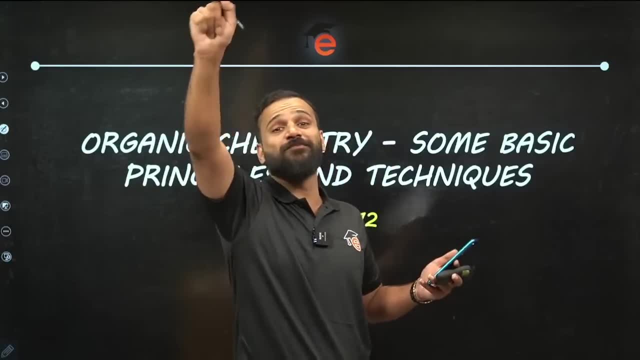 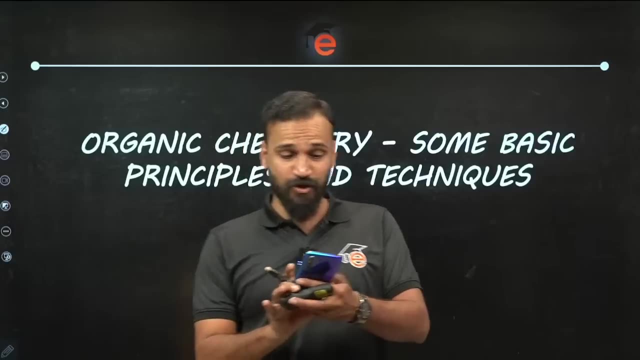 learning app. Yes, Yes, Yes, Yes, Yes, Yes, Not all. Yes, Children quickly see if anyone has left. you See if anyone has left. Someone has left To share, To send, To send a link. 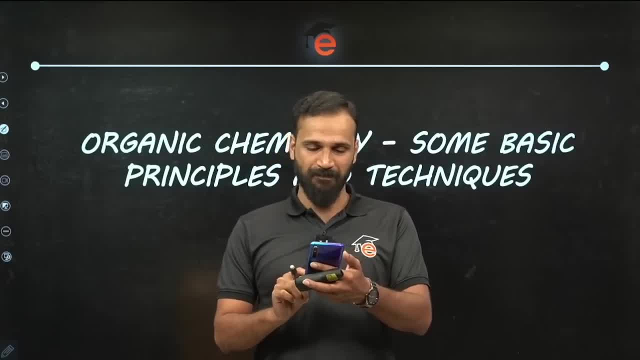 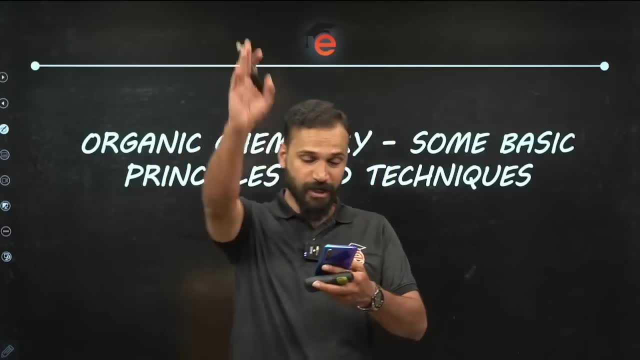 Has anyone left you? No? Yes, Do you get a note? Of course you do. If you join our community, you will get a note. There is no doubt You will get a note. Yes, Sana Fatima is asking to start. Yes, 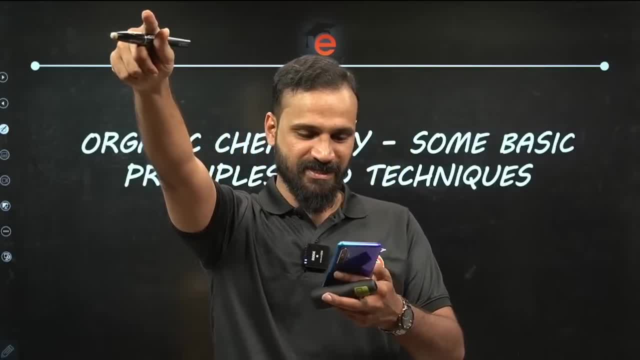 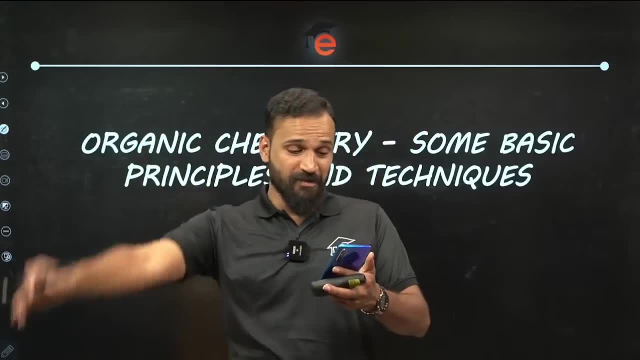 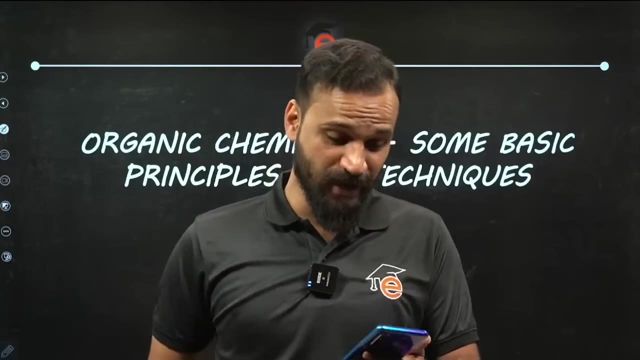 We are going to start. We are going to start. Yes, Yes, Devananda, Devananda, Like Black, another new student. Devananda, you are welcome. You are welcome to Jupot. Yes, New student. Creative vibes, Another new student. 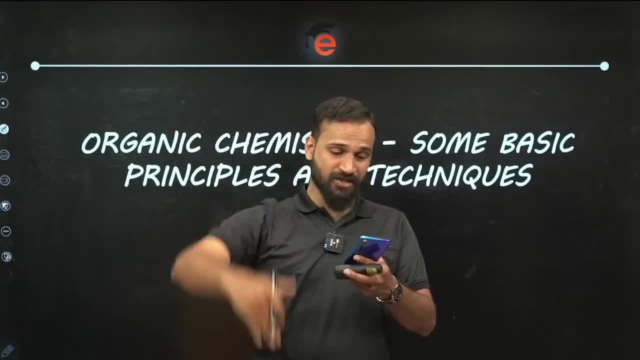 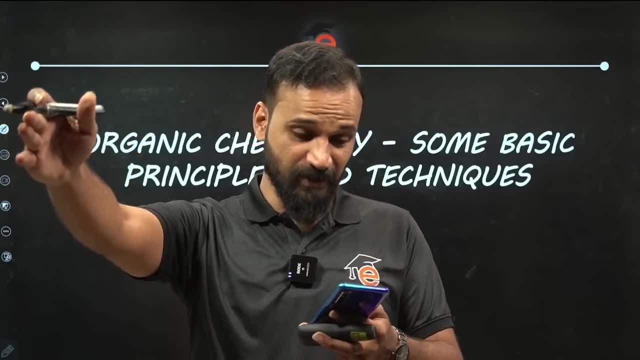 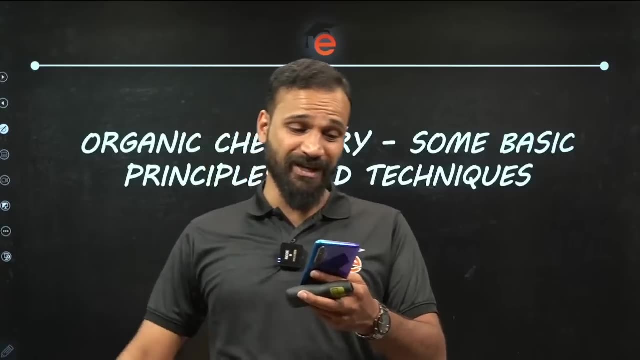 Very good, Very good. New people: They are joining our class. Very good, Very good, Very good. Yes, Rubanesh has shared. Very good. Yes, Everyone has gone to night class. Yes, Many people are going to night class. 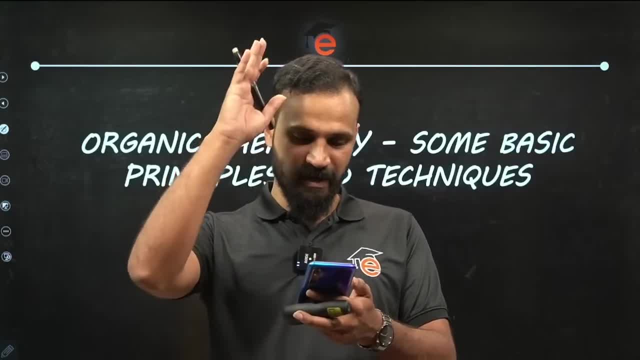 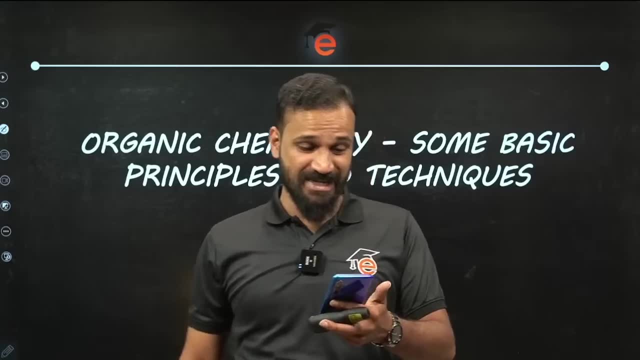 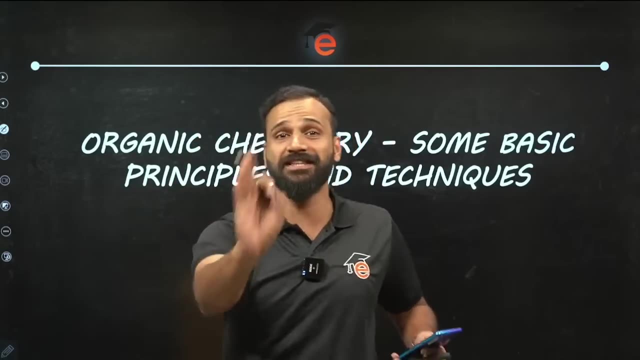 Okay, Fine, Yes, Everyone is here. Hi, Yes, Hi, Old student, Papa Isaac, old student. Good, Yes, Yes, It is one K, One K, One K views are there. I am not waiting even for a second. 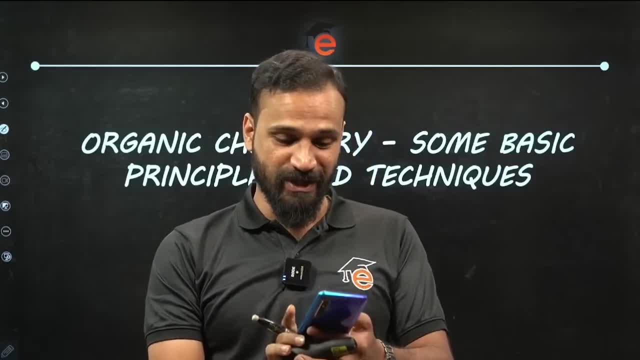 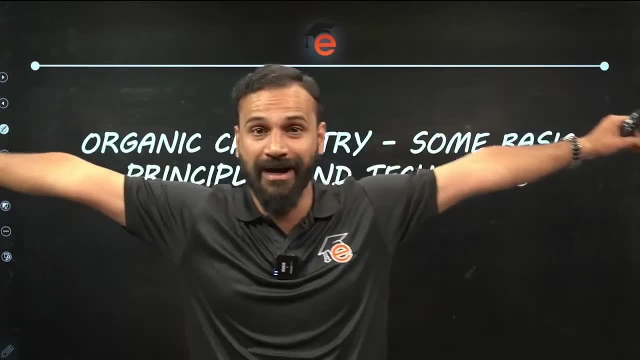 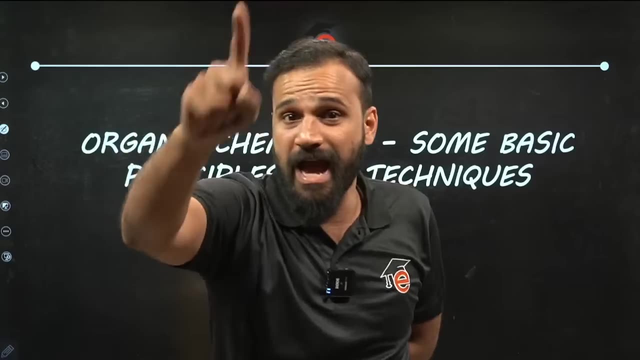 We are going to start. We are going to start, Yes, Yes, Yes, Children, our chapter is this. Now, your concentration should not go anywhere else. These two hours, or two and a half hours, we are dedicated to organic, The first chapter of organic. 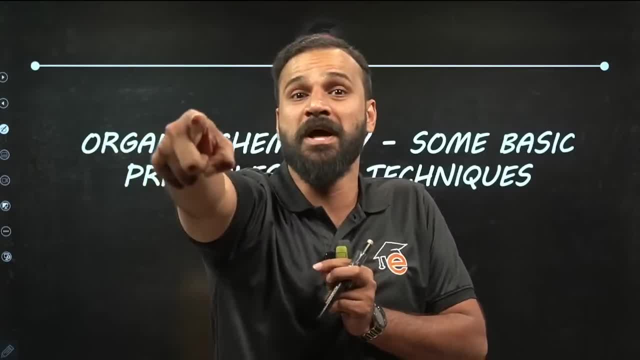 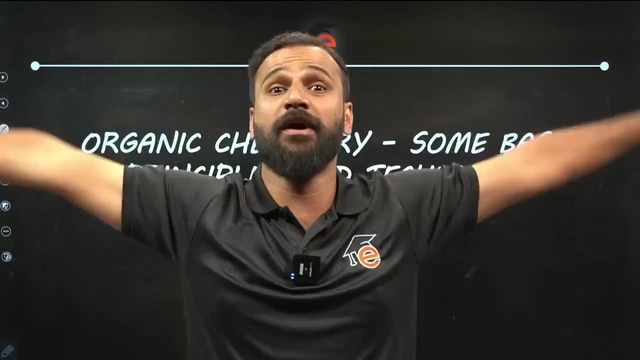 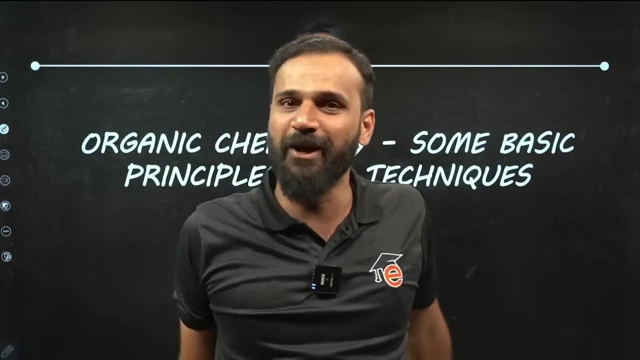 will be studied with this time. Children, that determination is in your mind. Yes, We should not go to these two hours for each other's activities. It should be fully focused on chemistry. It should be organic When I say the name of a compound here. 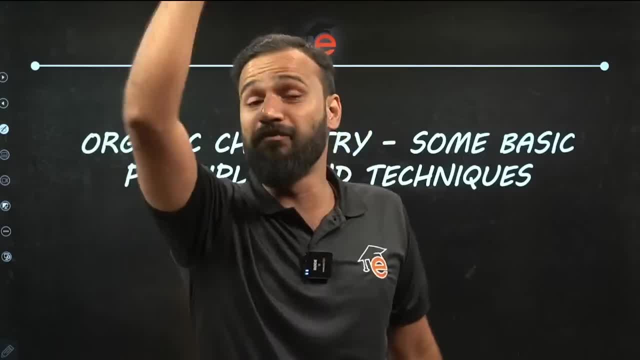 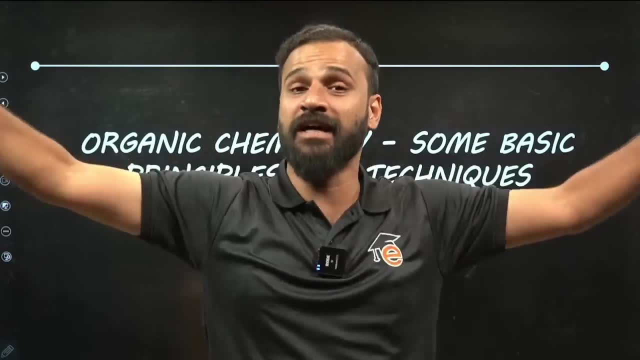 you can try it, You can say it, You can comment in the chat box. I welcome you to such a very active learning process. I welcome you to such a very active learning process. Not just to watch the video Not to be seen. 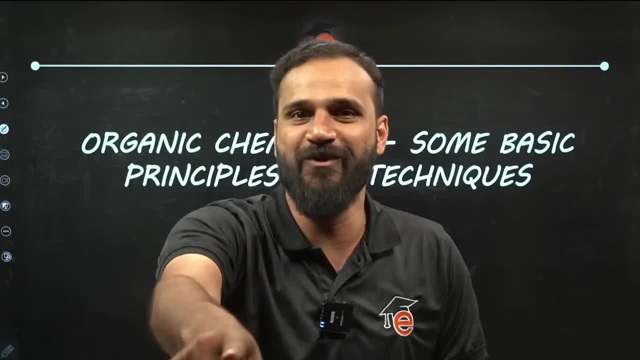 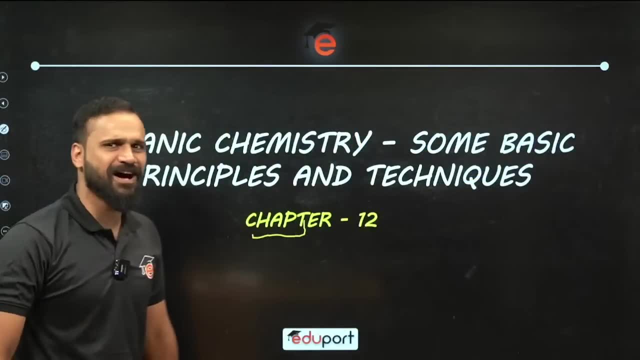 We have studied organically at this time. We are going to study organically at this time, Children, have you been well set up? Have you been well set up? Yes, our first point: What is the name of our chapter, Organic chemistry? Some basic principles and techniques. 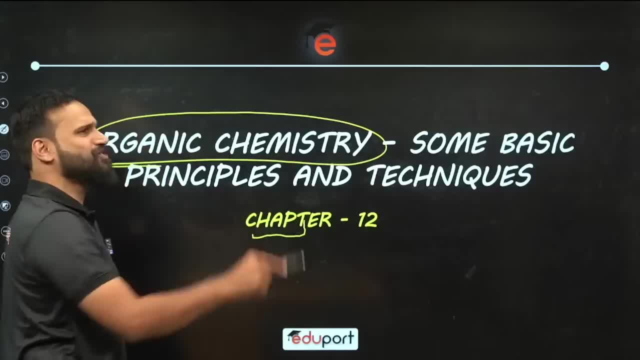 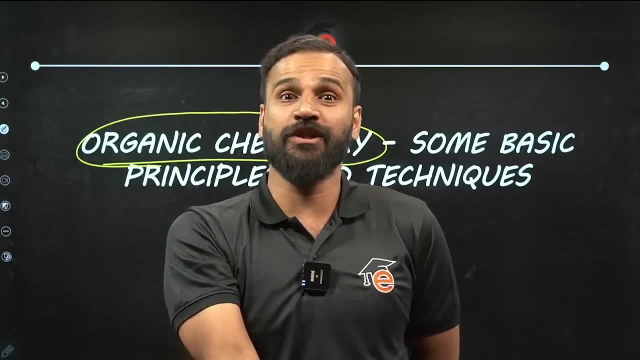 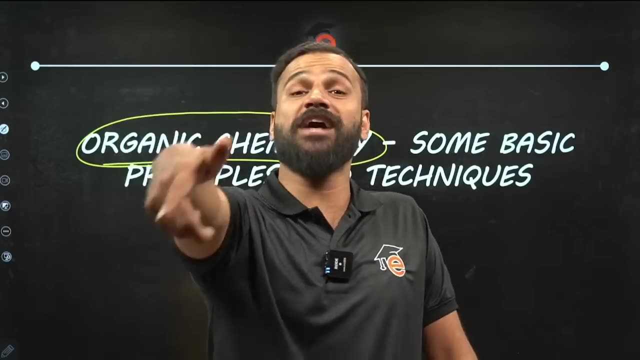 So what should be known first? What is organic chemistry? That is a question. What is organic chemistry? Let's say first What is organic chemistry. It is a branch of chemistry That is not known to anyone. Organic chemistry is a branch of chemistry. 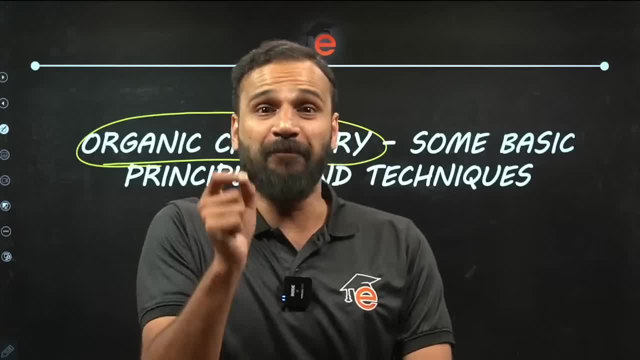 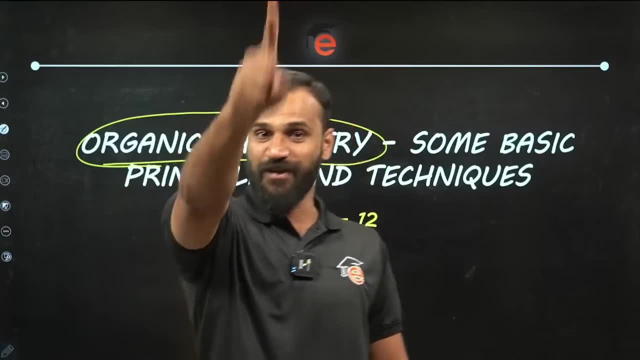 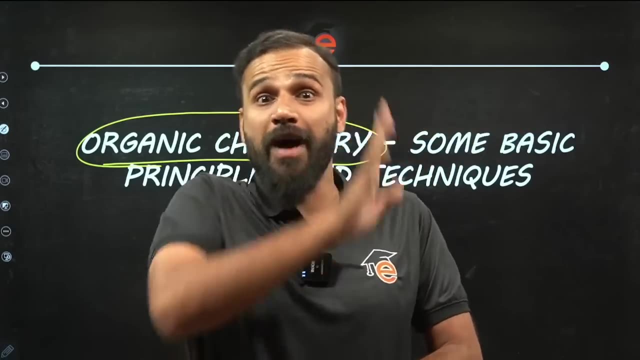 That is not known to anyone. Everyone knows that. Now, what do we study in that branch, Or what do we discuss in that branch? That is very, very important. What did I tell you, children? We study in organic chemistry. We have studied a lot of definitions in the past. 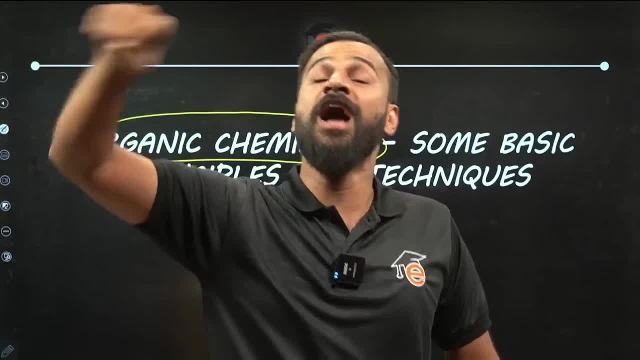 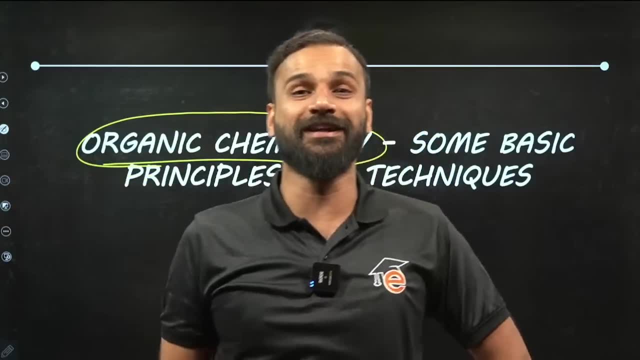 What did we study? Organic chemistry is a branch of chemistry that studies carbon-containing compounds. Similarly, organic chemistry is a branch of chemistry that studies hydrolysis. We have heard that it is a branch of chemistry that studies hydrocarbons. All of those are true, But what we are saying now is: 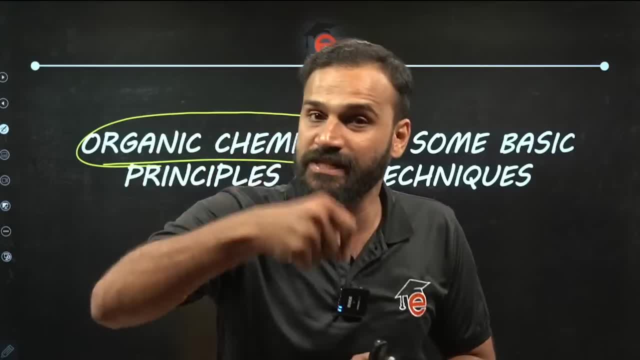 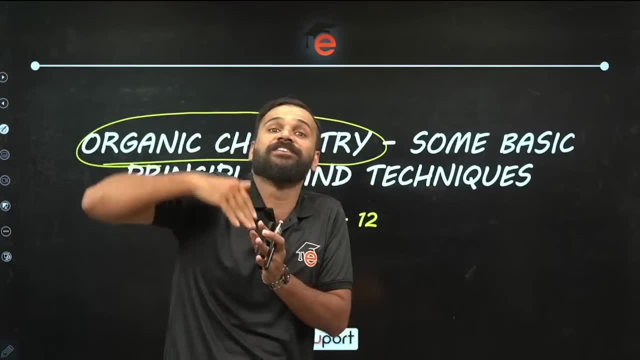 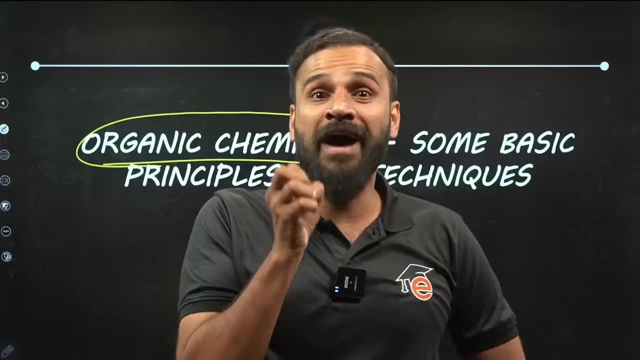 that organic chemistry is a branch of chemistry. It is a branch of chemistry which deals with the study of hydrocarbons and their derivatives. That is hydro. Who is hydrocarbon? Hydrocarbon is the compound that contains carbon and hydrogen. About hydrocarbons: what does it mean? 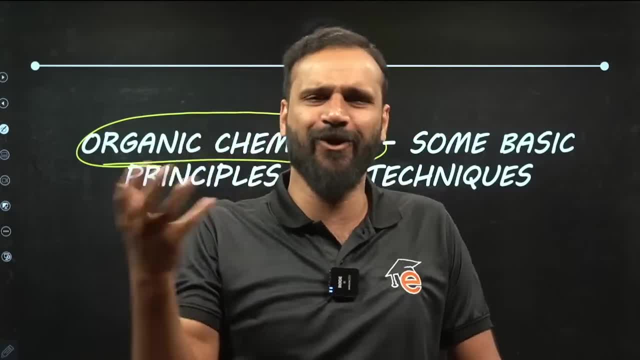 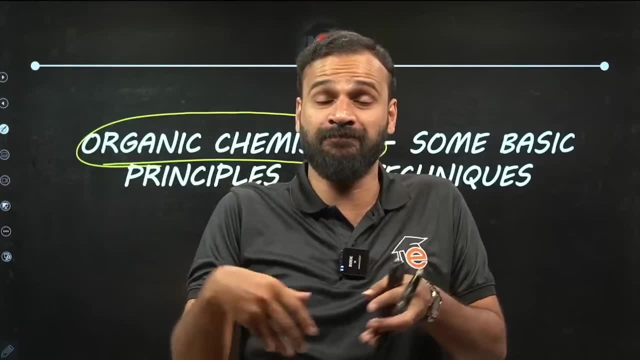 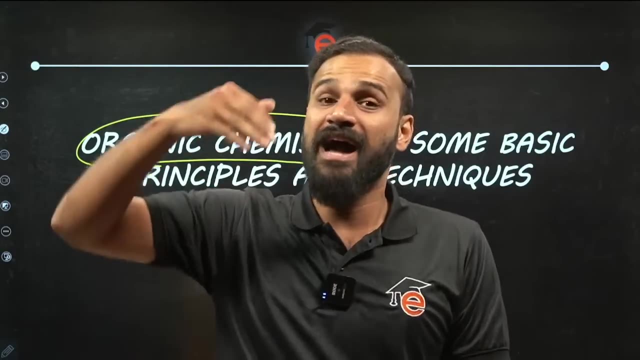 According to the derivatives of it. who is the derivative of this hydrocarbon? Hydrogen in hydrocarbon is replaced and sometimes other atoms and other groups come. They are called the derivatives of hydrocarbons. What are they called Derivatives? 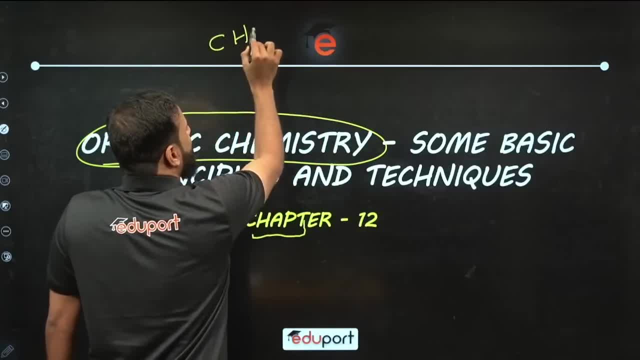 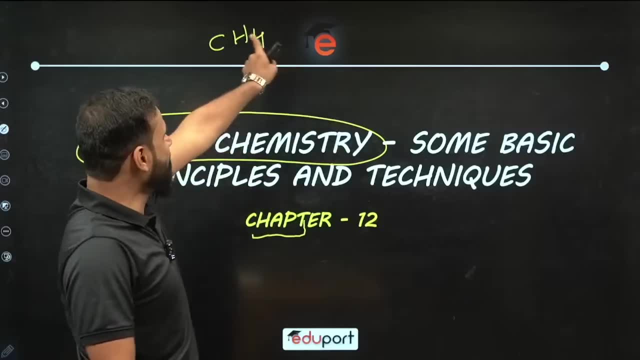 That is, if you look at this, CH4 is a hydrocarbon. Methane is a hydrocarbon Because there is only carbon and hydrogen in it After removing the hydrogen in it. for example, imagine that a chlorine came after removing a hydrogen. 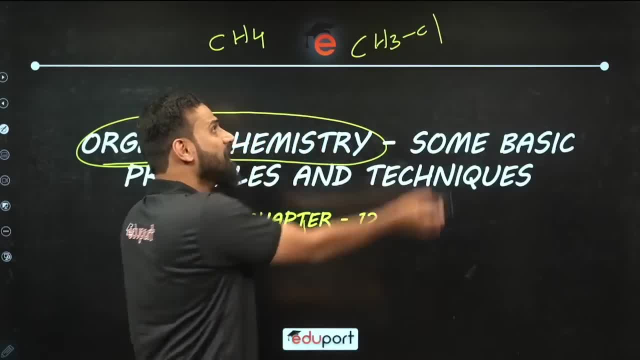 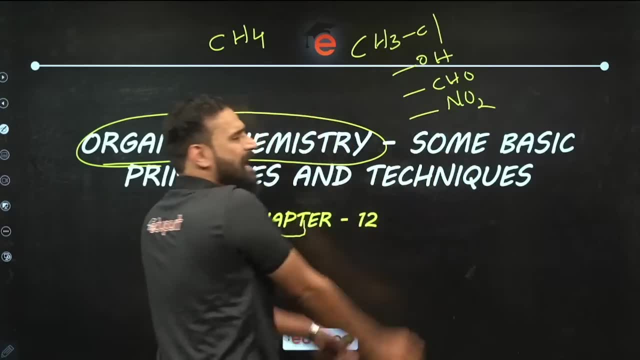 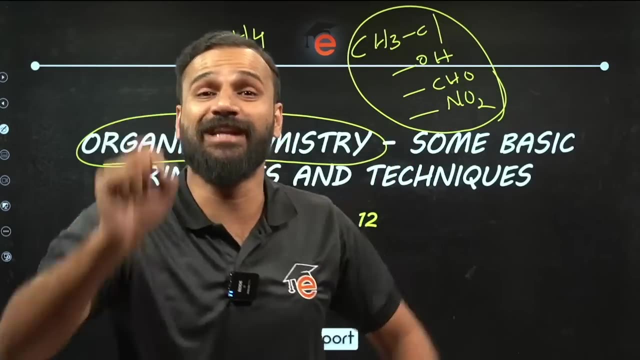 Then it will not be CH3Cl children, Whether OH comes there instead of chlorine, CHO comes there instead of that, NO2 comes there instead of that. whoever comes after replacing hydrogen. like that they are called the derivatives of hydrocarbons. 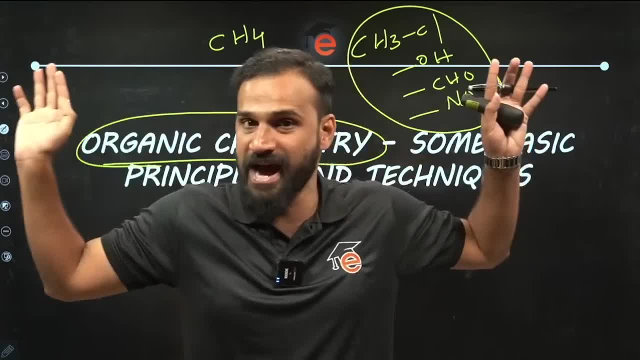 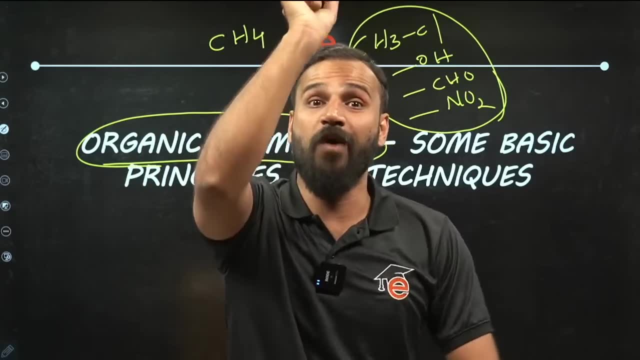 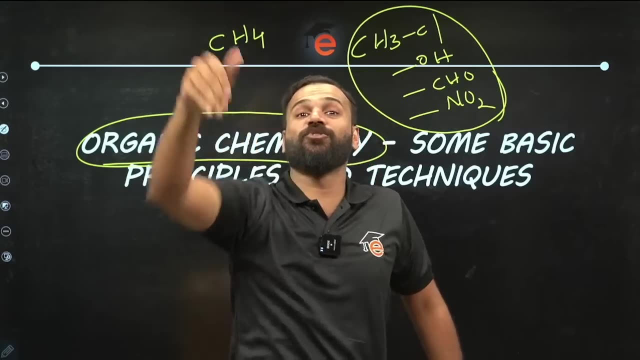 So, friends, The first point is clear to you. The first point is clear to you: What is organic chemistry? What we say, very simply, is that it is a branch of chemistry that learns about hydrocarbons and their derivatives. What did you tell the children? 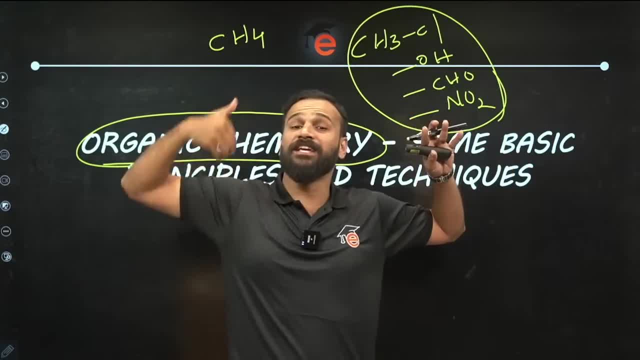 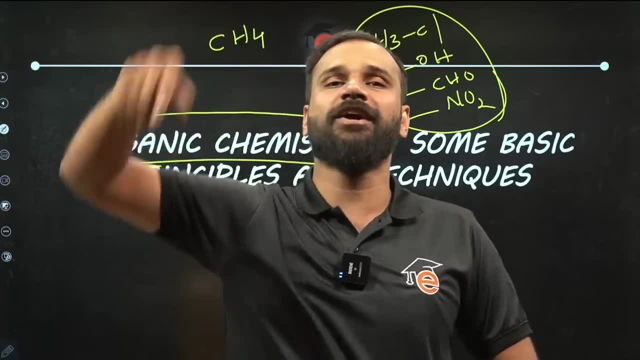 What did you tell the children About hydrocarbons and their derivatives? What to say Learning? The branch of chemistry that learns about hydrocarbons is called organic chemistry. Yes, you always have to keep this in mind. What is organic chemistry? 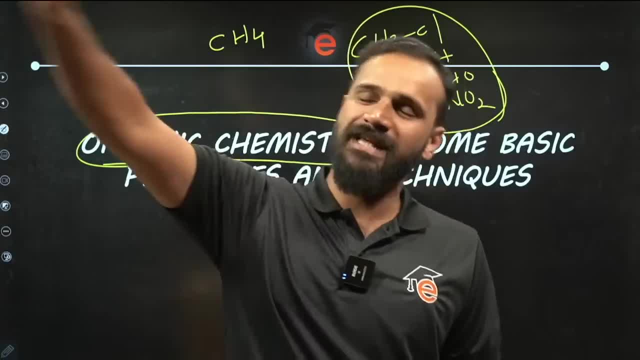 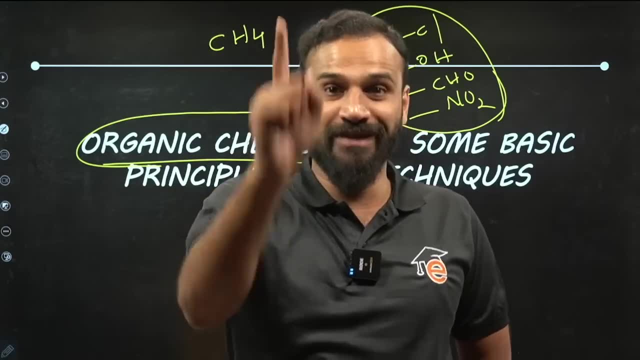 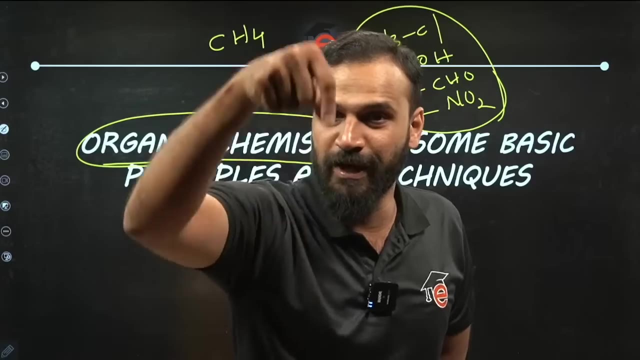 Ask us. No one is going to ask. No one is going to ask for an examination, But as far as we are concerned, we are going to learn a lot of organic chapters. What is organic chemistry? You should definitely know. That's why I said about hydrocarbons and their derivatives. 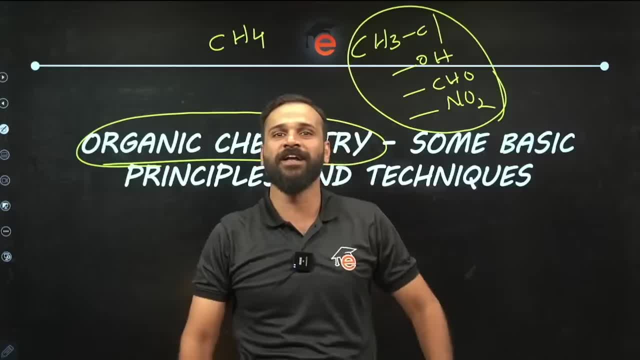 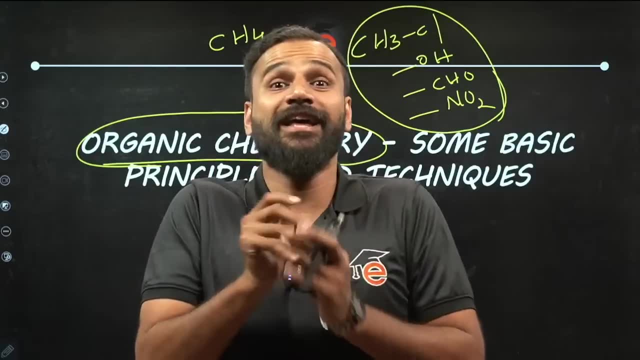 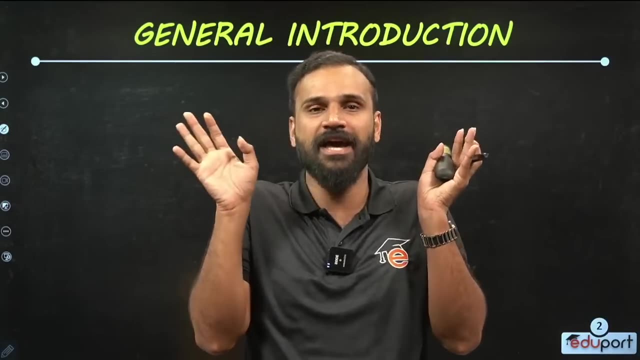 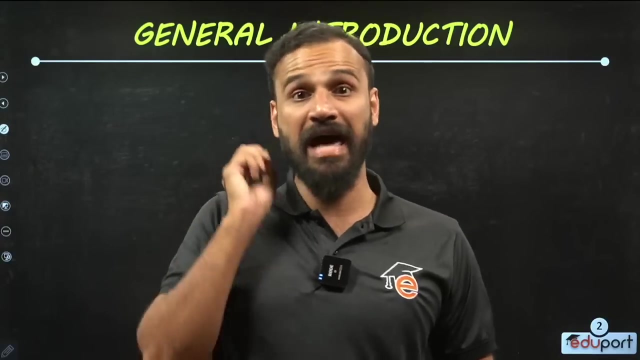 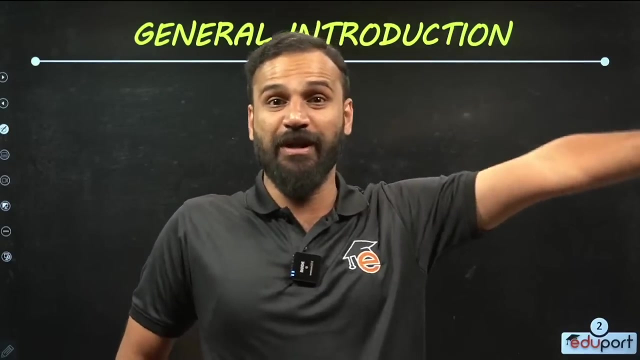 What is organic chemistry? We have to understand the first definition: All carbon-containing compounds are organic compounds. We never know. We should know that. Why did we say that first? It is said that organic chemistry is the branch of chemistry that studies carbon-containing compounds. 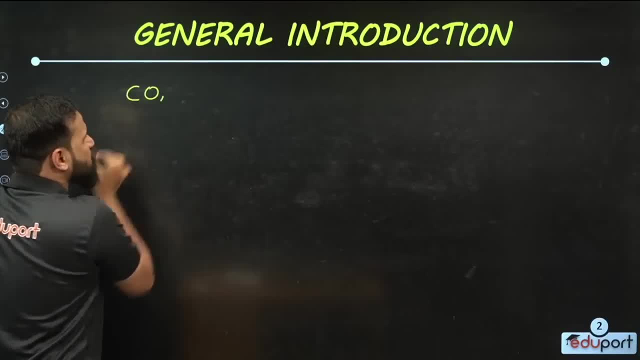 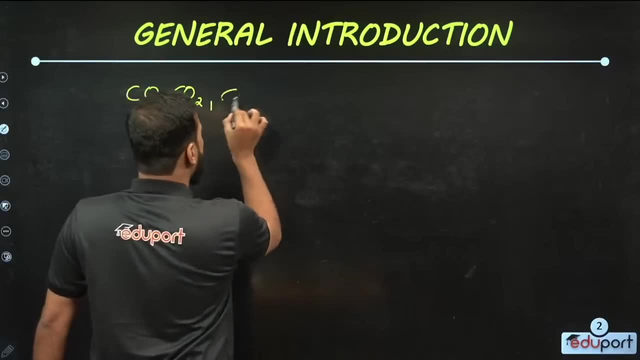 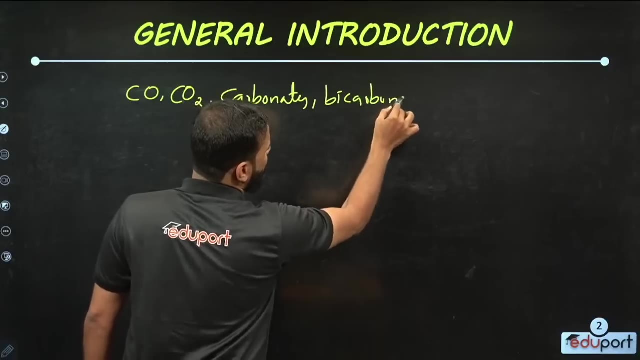 Yes, But look, you have carbon monoxide in it. there is no doubt Carbon dioxide. There is no doubt that there is carbon. Now you Take carbonates. What is it? Take carbonates. Or you Take bicarbonates. Take bicarbonates. There is all carbon in it. 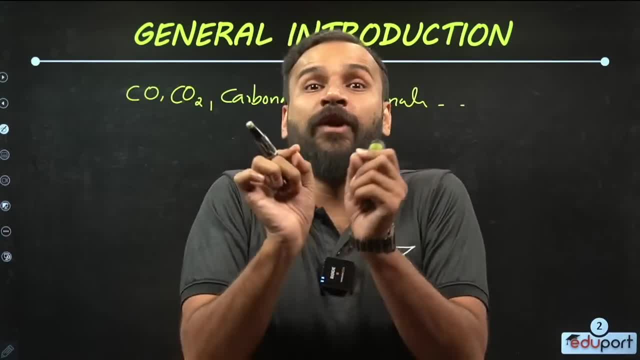 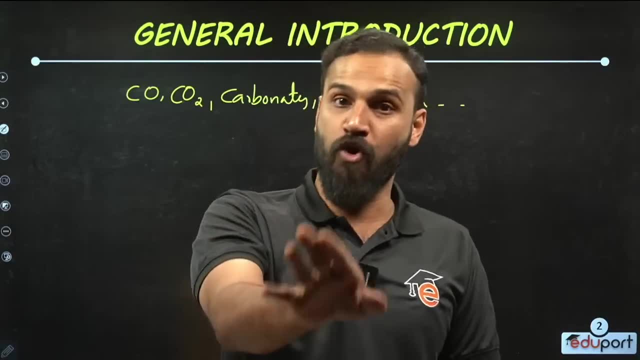 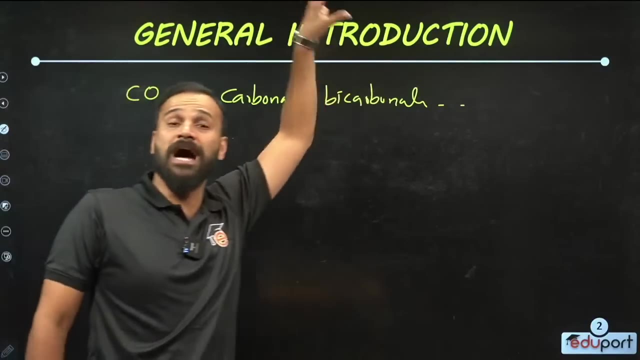 But they are nothing. You must understand that they are not organic compounds. That is, all carbon containing compounds are not organic. You must have in mind that they are not compounds. The example of that is carbon monoxide, carbon dioxide, carbonates. 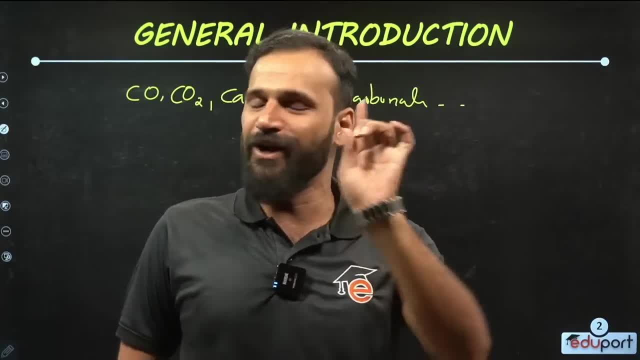 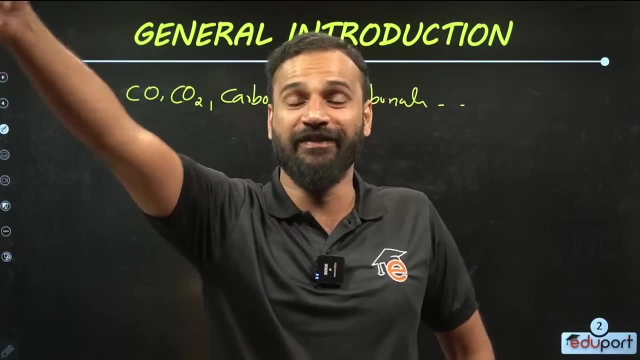 You must remember that there are bicarbonates. When we say this, we have studied another chapter. Do you know where I have studied in zoology, Which chapter? Carbon? It is the chapter called biomolecules. right There, you have studied a lot about biomolecules. 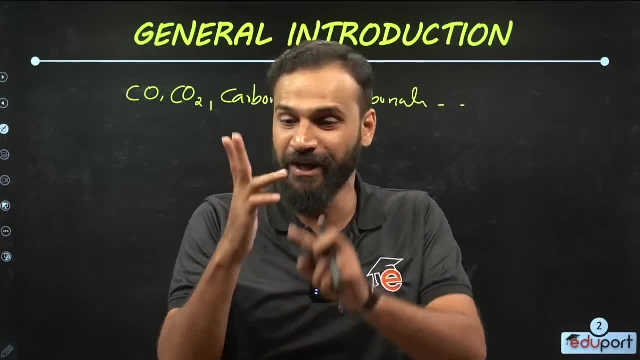 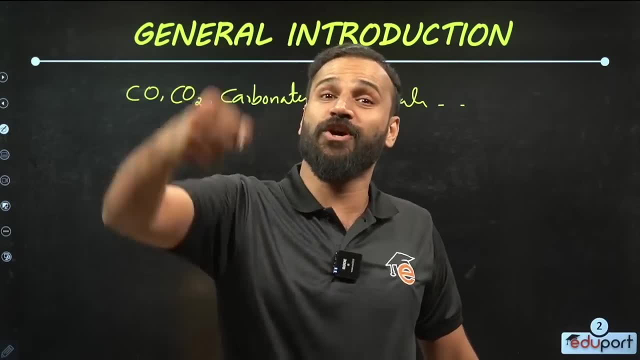 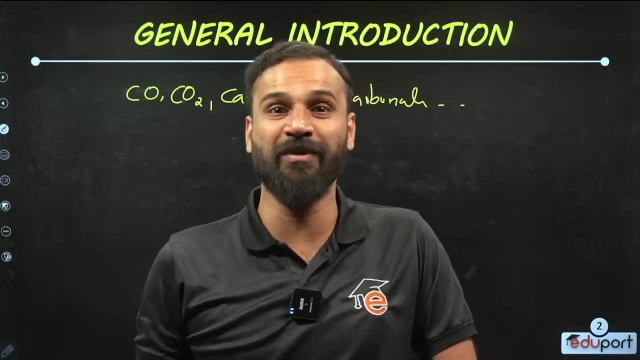 Have studied. Have studied carbohydrates, Have studied about proteins, Have studied about fat, Have studied about lipids, About vitamins, about enzymes, About nucleic acids. you have studied all about the biomolecules in zoology. Have studied in the chapter right. If so, one thing. 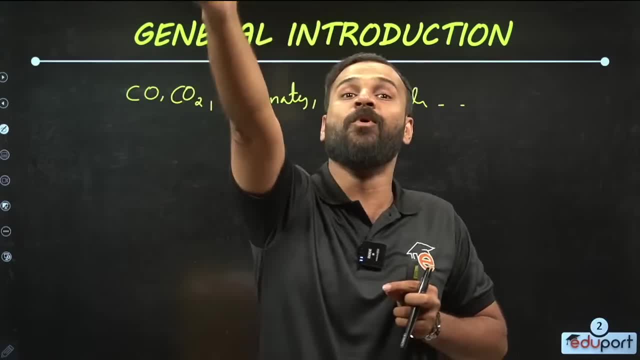 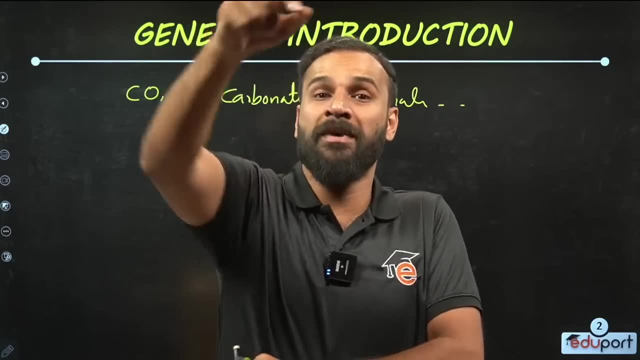 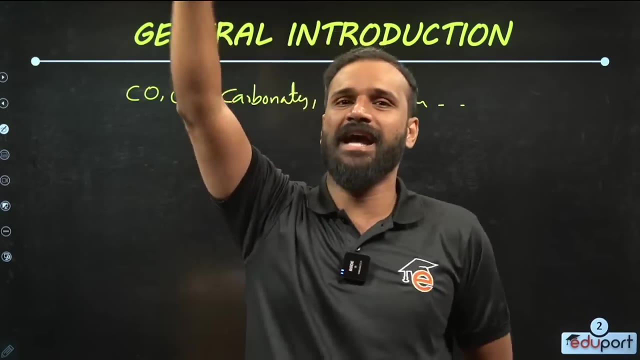 You must remember. Do you know what All biomolecules, What are the organic compounds and what are all biomolecules? carbohydrates, proteins, Enzymes, vitamins, nucleic acids are organic compounds In the mind. this is the first chapter of the organic chemistry. 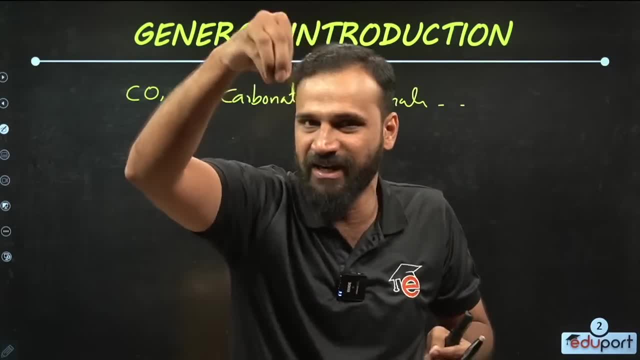 I'm presenting all the basic things in front of you for the sake of the importance in it. You must make note of it, inscrusted Precisely. you have to study it, okay, Isn't it, dear children? You must face it. salary pay: p 這個相当 nail嘲 cess г. 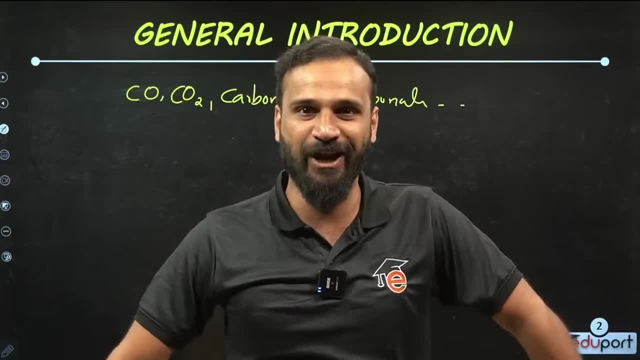 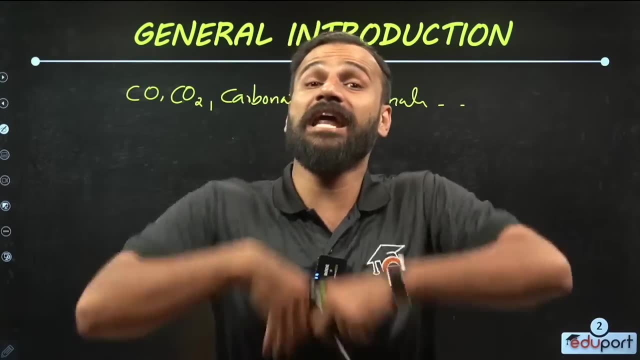 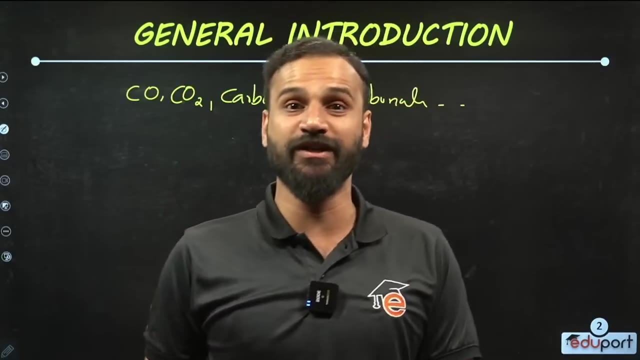 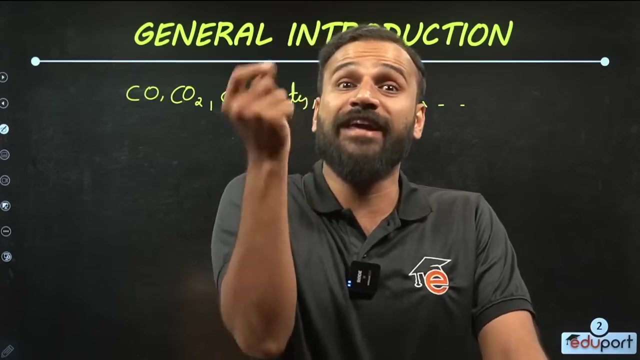 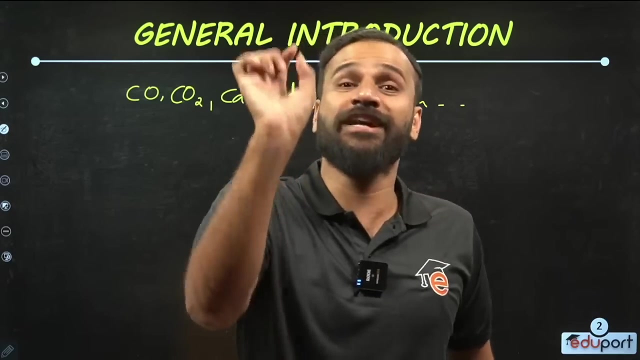 To study it. These things are the natural Icelandic, nämlich: Yes, let me ask you one more thing. let me ask you one more thing: where does an organic compound come from? or where does an organic compound exist? where does an organic compound exist? first of all, we are told by a scientist called Berzelius. he is putting a theory ahead. that theory is called the vital force theory. it is not to be studied. it is not to be studied, it is not to be asked. but it is just a thing mentioned in the NCRT, just a 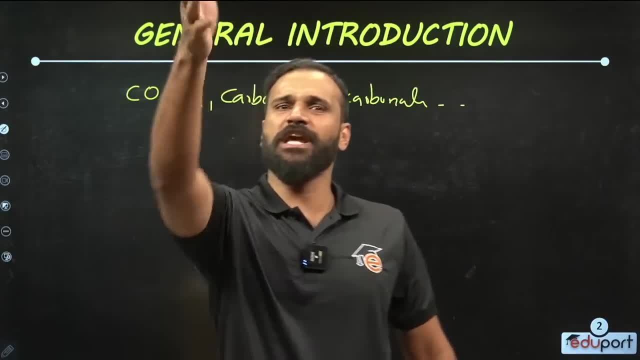 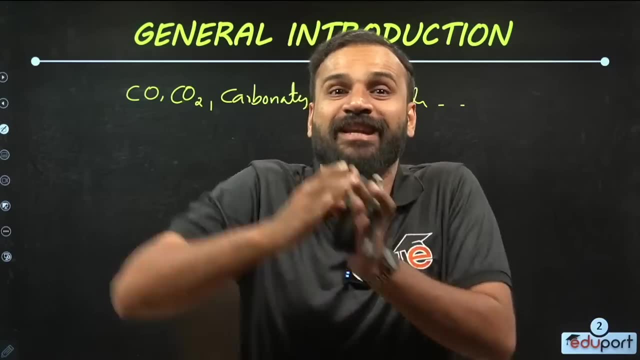 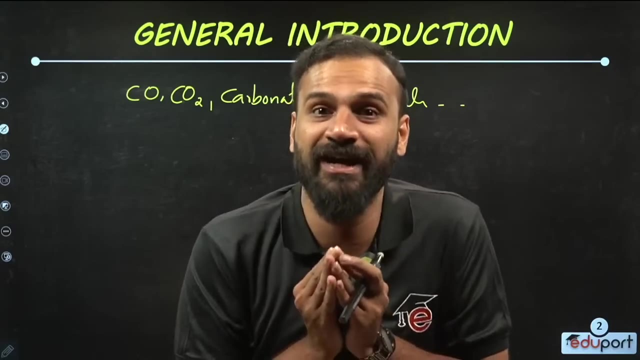 let me tell you. do you know what Berzelius is trying to say? in the vital force theory, there is an organic compound. where is it? it is inside the tissue of plants and animals. where does an organic compound exist? it is inside the tissue of plants and animals. that is very important. 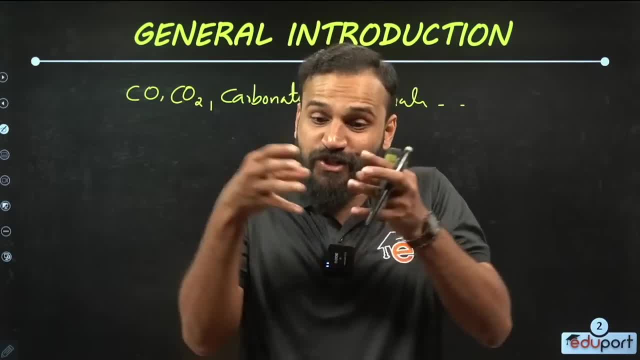 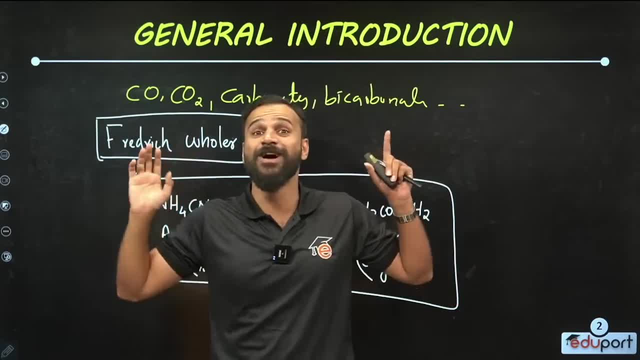 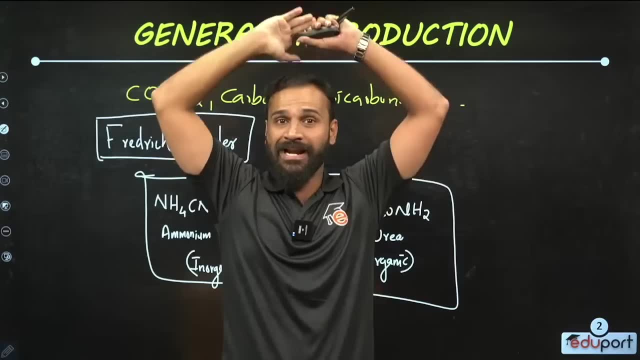 you have studied in biology. the tissues are made up of cells. you have studied in biology: the tissues are made up of cells. What we are going to learn is about a very simple chemistry branch. Are you all ready? Are you all very active? 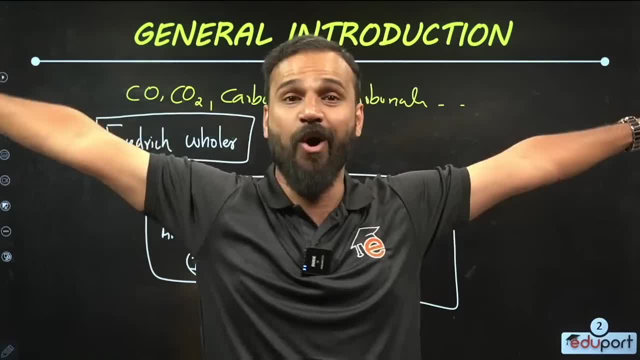 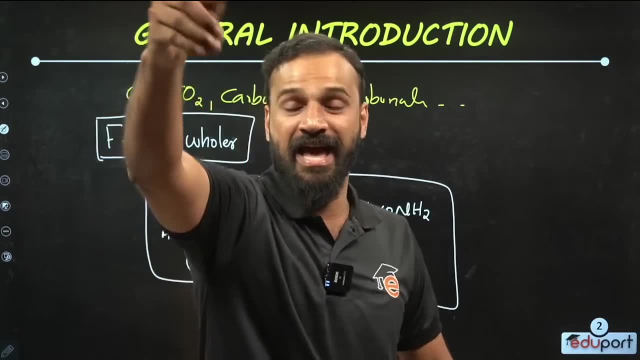 Let the fire come, children. Let the fire come. Let the fire come. If everyone is okay, let the chat box burn. Let the chat box burn. Yes, this is very important. We are getting into very serious matters. We are getting into the questions asked for the exam. 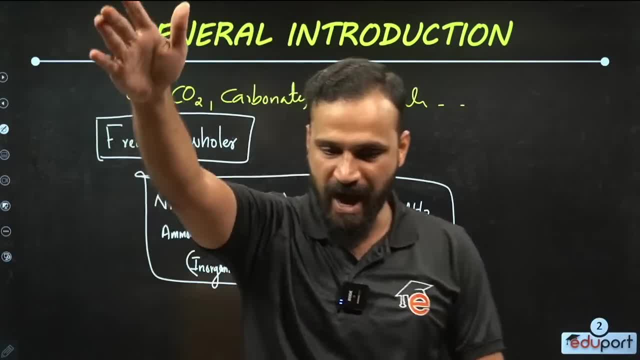 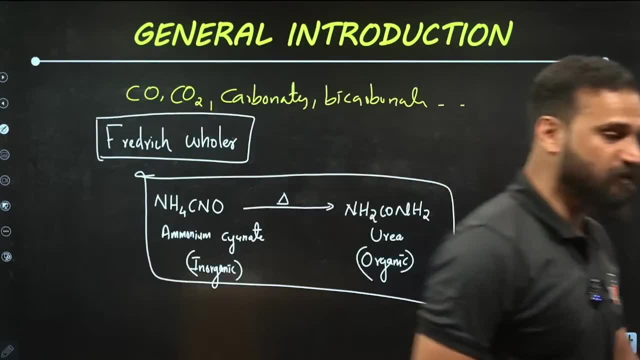 If you are ready, say it quickly. If you are okay, say it. Let the chat box burn. Let the chat box burn. Only then I can understand that you are active there. That's very important. Say it quickly. Say it quickly. 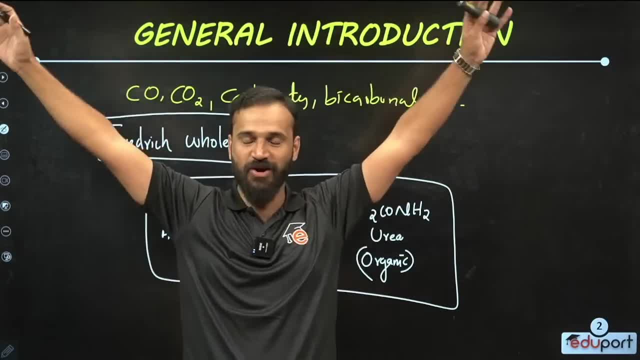 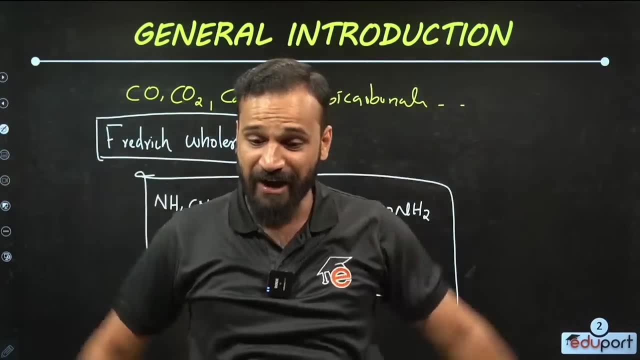 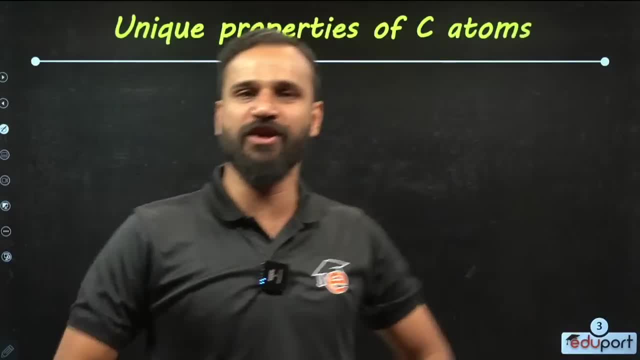 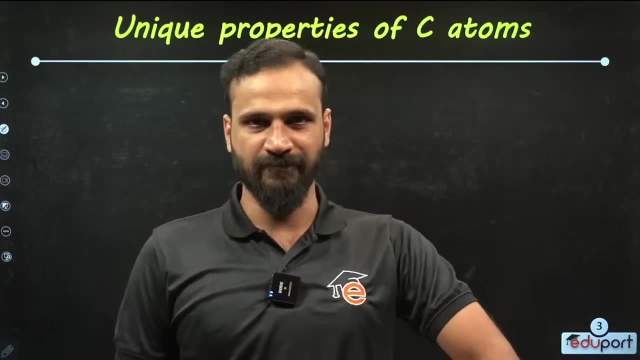 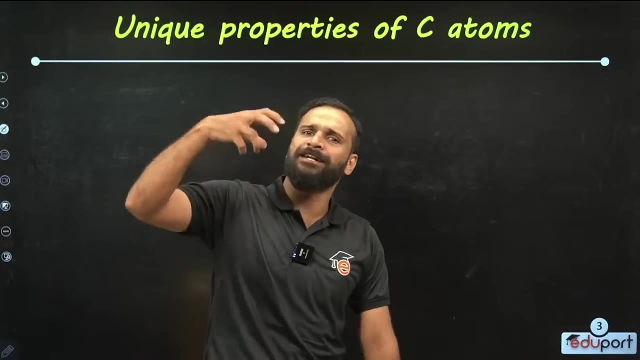 This is the first question you are facing from this chapter. What did I say? What did I say? Today, millions of organic compounds are available. Today, millions of organic compounds are available. Why are there so many compounds in carbonate? The answer to that question is a question that we can create. 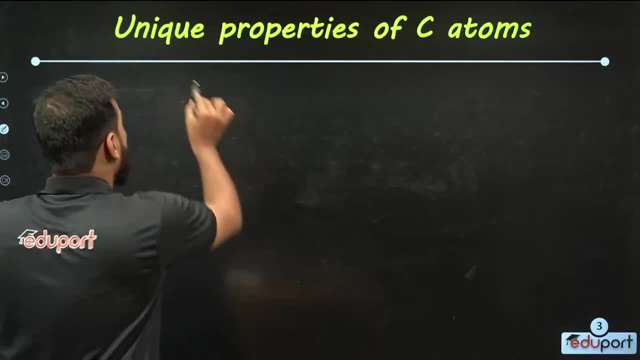 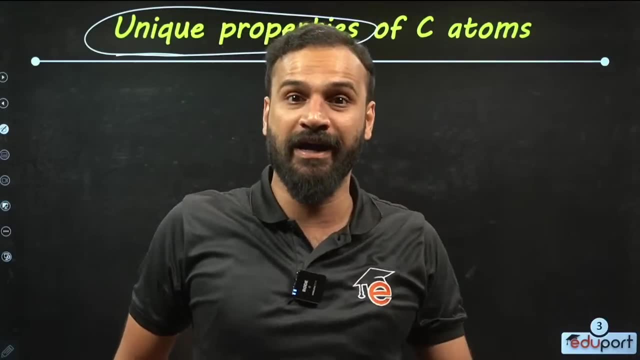 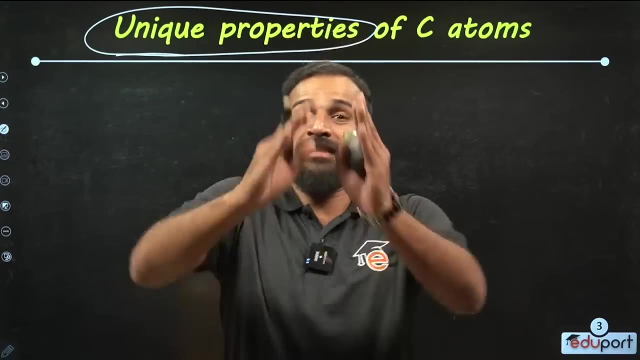 Do you know the answer to that question? Carbonate has some unique properties. Why can carbonate be made in large quantities of different types of compounds? When asked why another element is made of different compounds other than the amount of carbonate, we have an answer to that question. 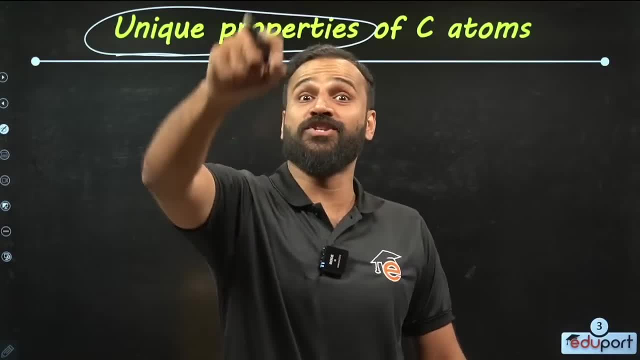 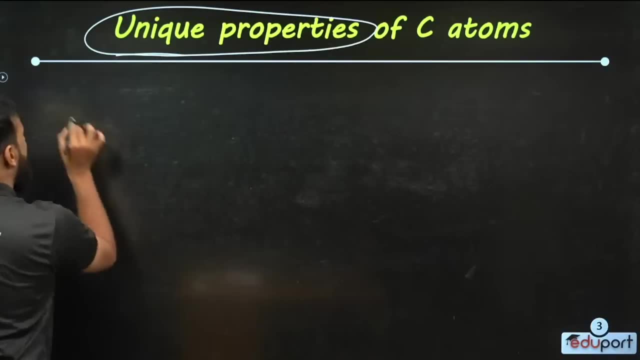 It is not because of carbon. Carbon has some peculiar characteristics properties. We are going to that. Look at the children. The first point in it is called tetravalency. What children Tetravalency? What is tetravalency? 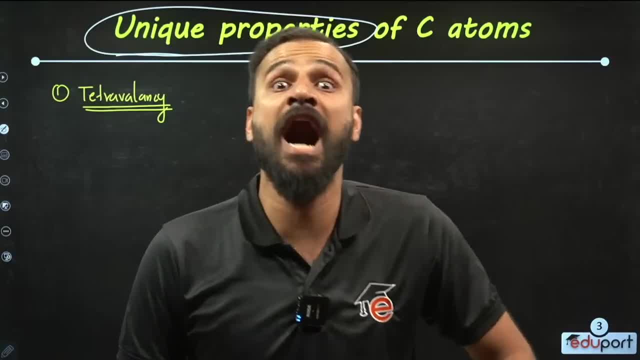 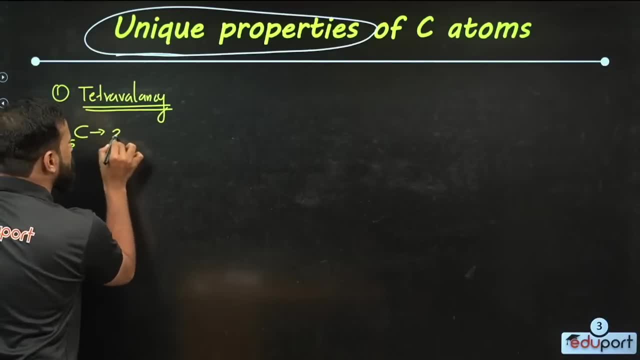 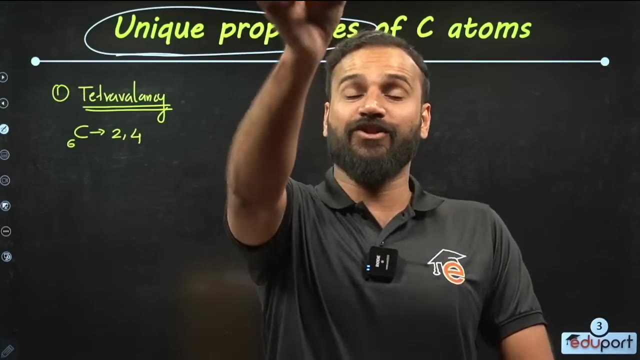 The valency of the carbon atom is four. It is very important. You know the atomic number of carbon is six: Two electrons in the first shell, eight in the second shell. With four electrons in the valency shell, a atom can be stable or can never be stable. 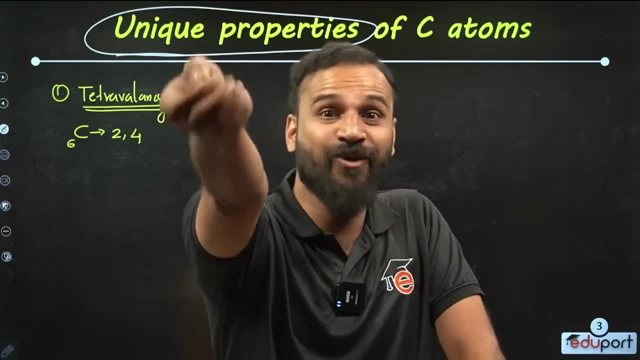 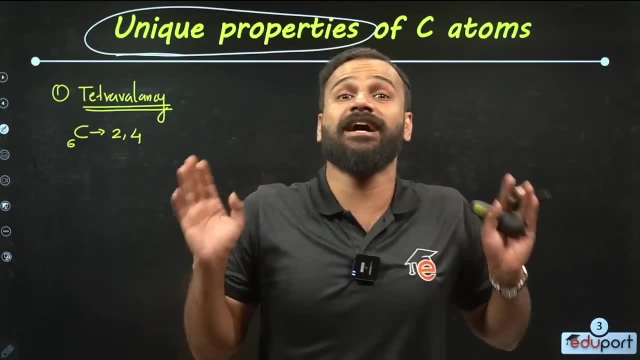 According to the octet rule, he needs four more. Four more. If there are eight, all the children will be stable, According to octet rule, So eight. what do you say? because there is a shortage of electrons. do you know what capacity he has? 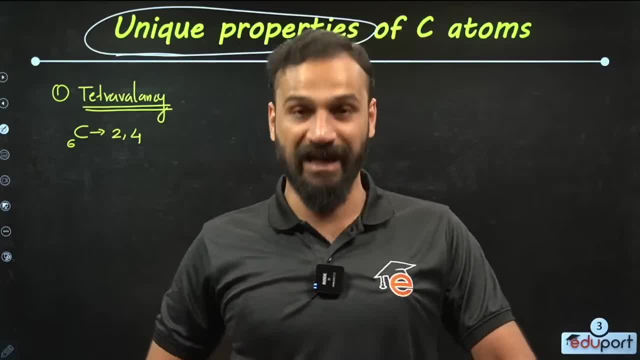 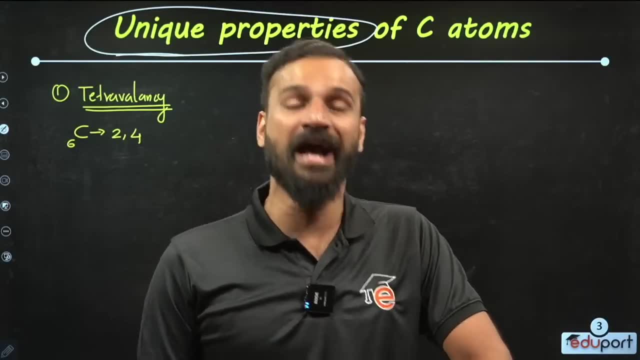 There is the capacity to make bonds with four atoms. That's why we are tetravalency. We define valency in the form of two in the third chapter right. What is valency To get stability? a Atom is the number of electrons that gain or lose. 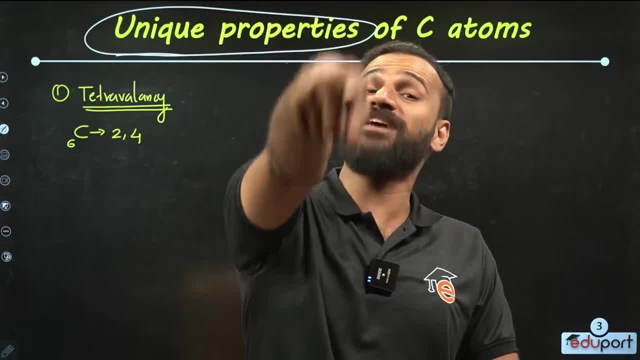 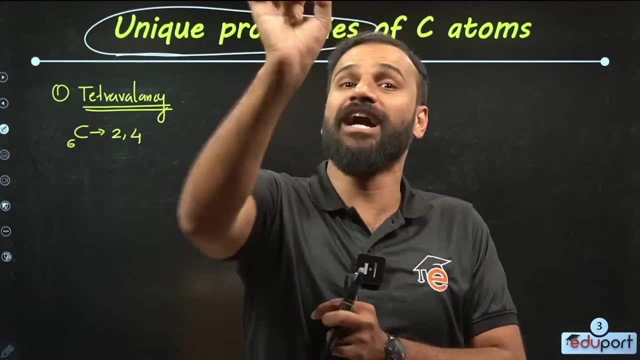 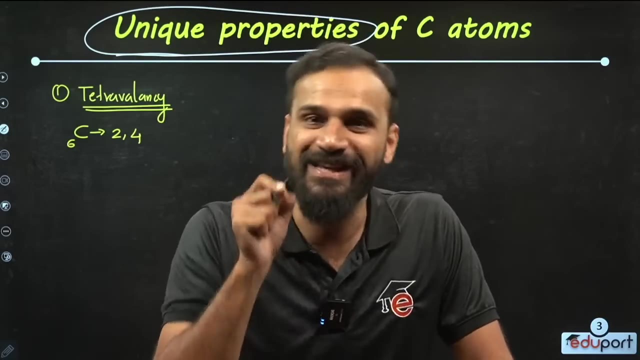 valency, Or the combining capacity of an element is valency. Haven't you learned that? So If the valency of the carbon atom is four, what does that mean? The carbon atom can make a bond with four atoms. Will those four atoms be the same? It can be the same, Or? 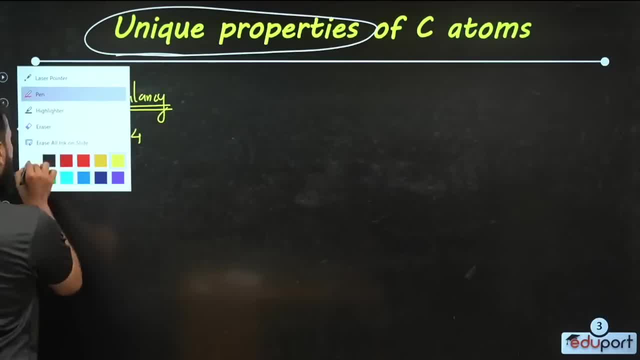 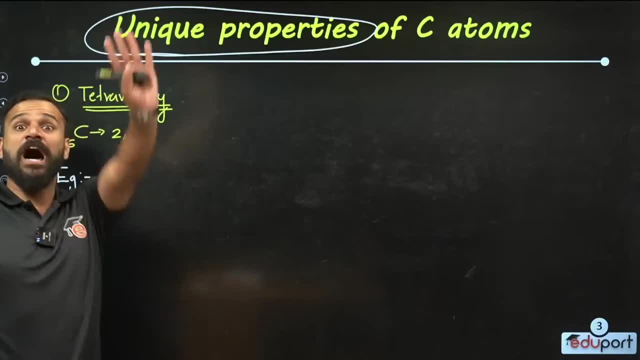 it can be different. Look you see. you see what is the example? You all know, isn't it Methane? What does carbon do in the methane? It was bonded with four hydrogen. You know right. Carbon tetrachloride: it was bonded with four chlorines. 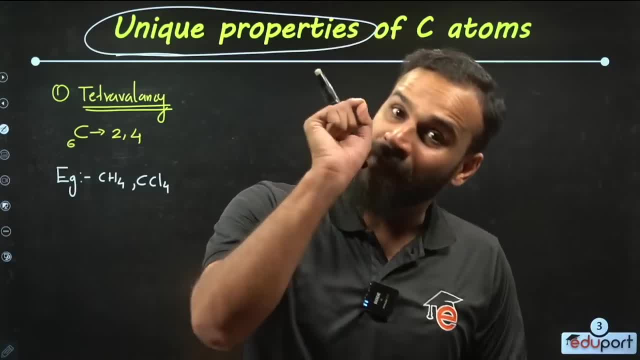 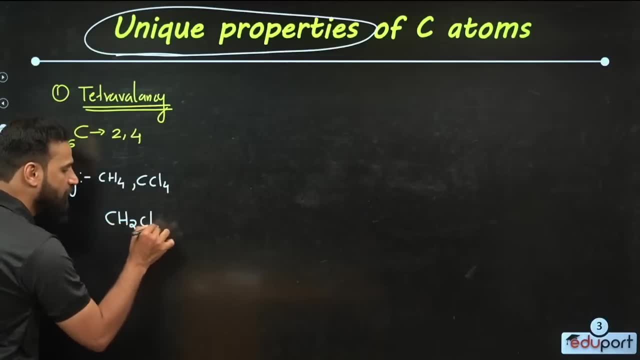 Then when you say to bond with four atoms, those four Atoms can be the same atoms. If you want another, it can be different. Look, with two hydrogen, two chlorines, they can do it. One percentage may do it. 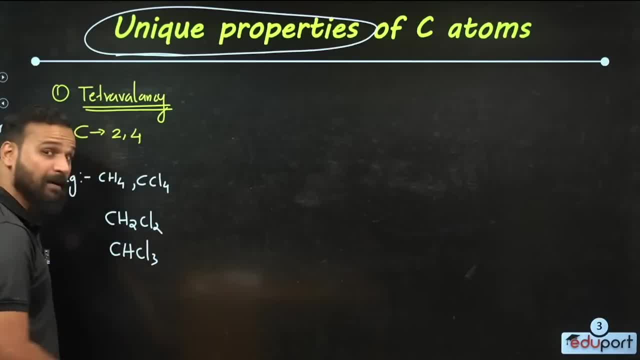 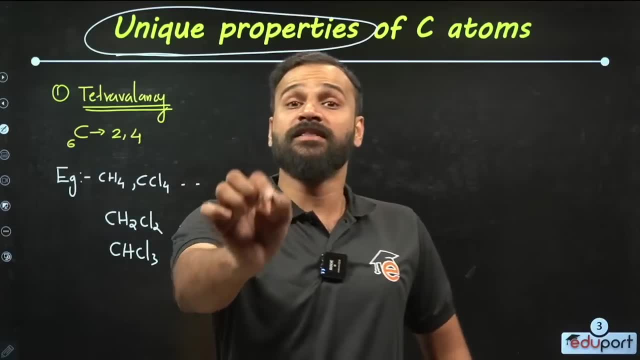 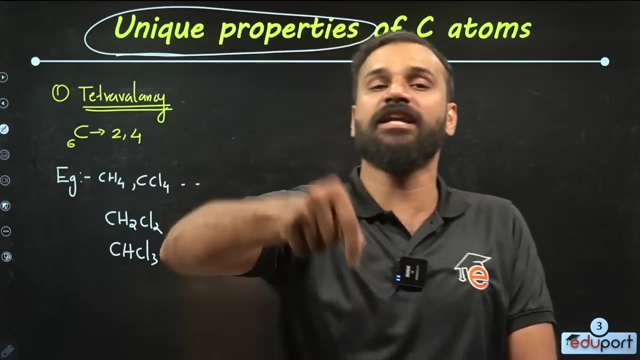 There is no problem. Now, one hydrogen must be combined with three chlorine. There is no problem to do it. So what is our point? my children? Our carbon atom can be combined with four atoms. That is its tetravalency valency. If it is four, it can make bond with four atoms. 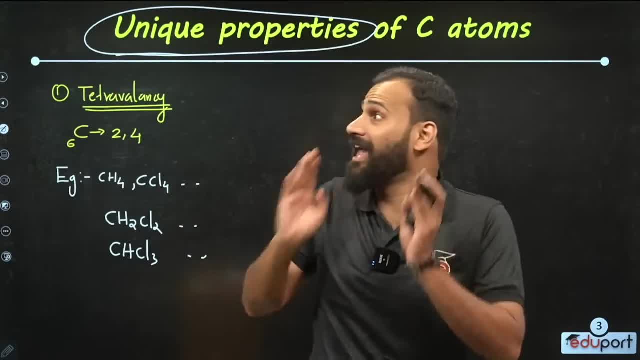 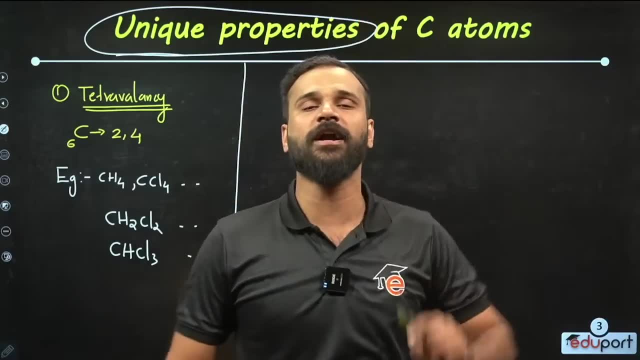 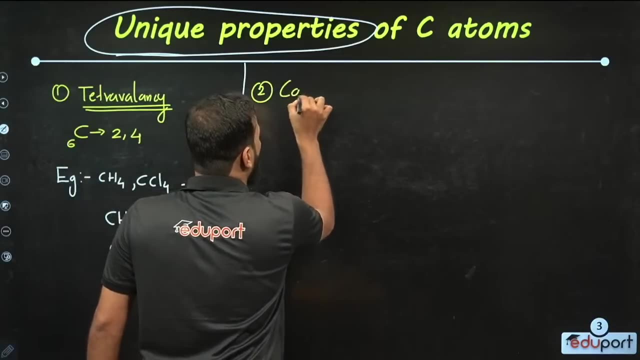 that may be same or different. Those four atoms may be the same or different. This is a unique property of carbon atoms. we must learn. Next, what is the second? What is the second? It is known to all to say the second point. 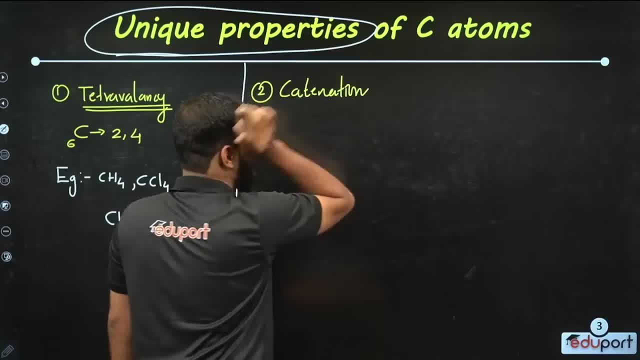 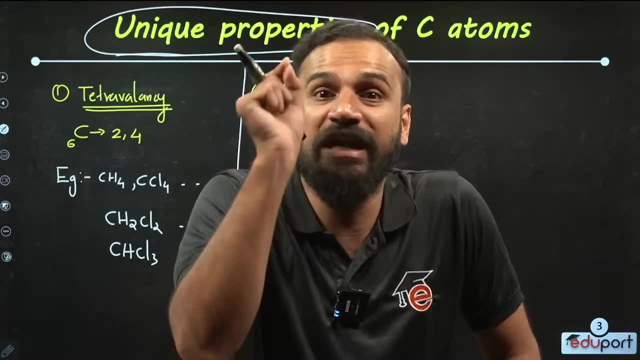 That is cationation. Right, children Cationation. they also say cationation. What is cationation? In one word, it is a self-linking property. What is cationation? What to say? my children Self-linking. 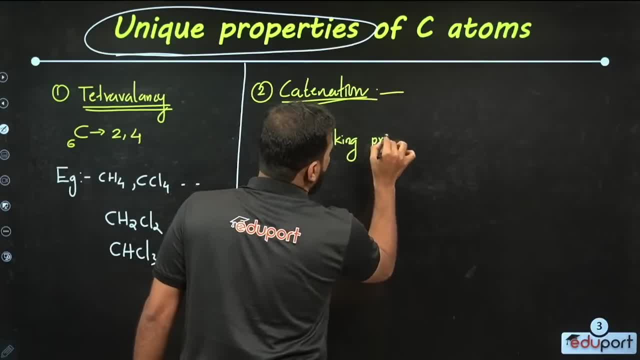 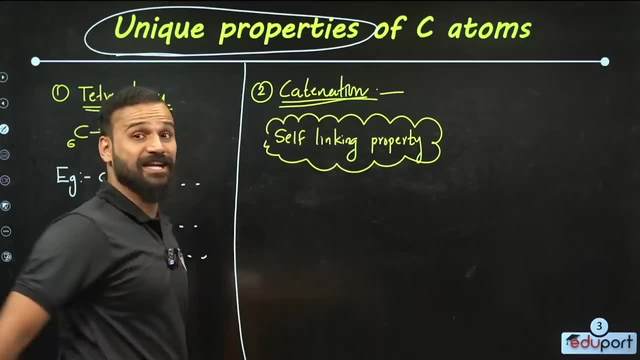 property. That is very important: Self-linking property, right? What do we call it? It is called catenation. What is the property of catenation? The name we call self-linking property is called catenation. What is? 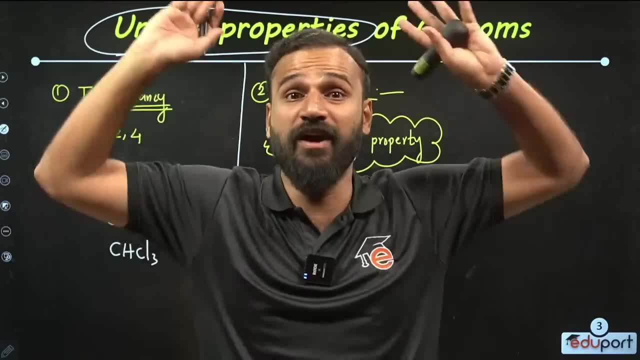 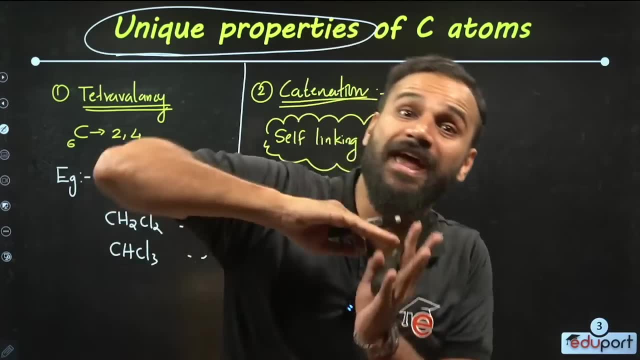 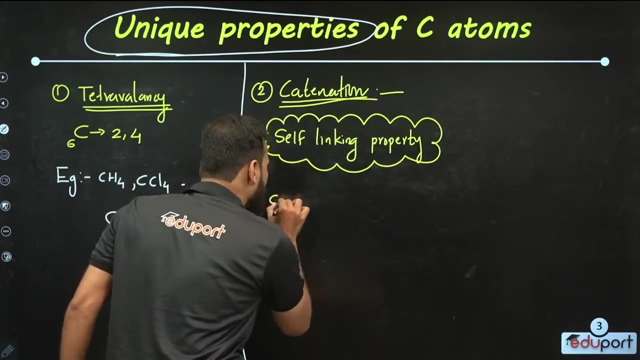 catenation. What is catenation? That's very, very, very important. Self-linking- What does it mean? One atom as its own atom, combined as the same atom, Big chains or big rings are made. Carbon is combined with carbon. 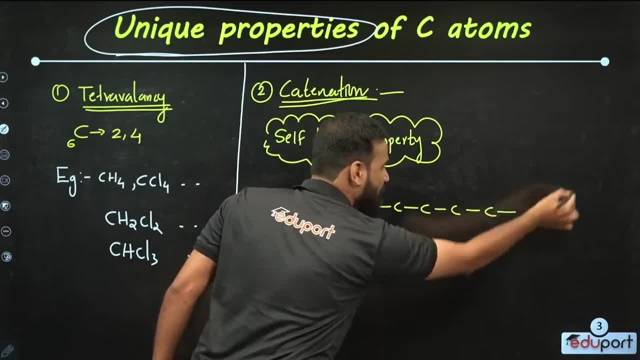 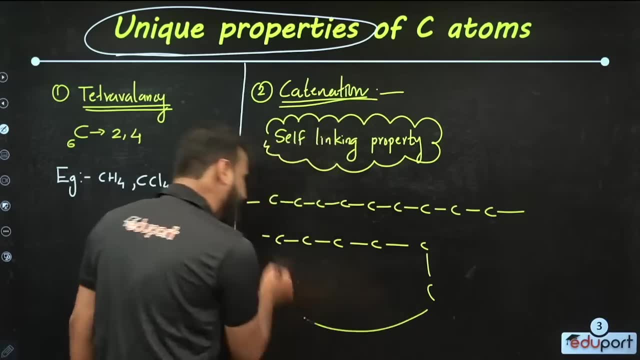 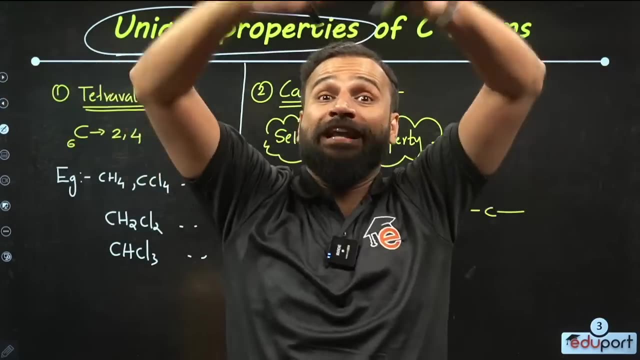 Just by combining carbon with carbon, Big chains are made. Or by combining carbon with carbon, Big rings are made. There is carbon here. Then Carbon is combined with carbon: big chains or big rings. The ability of carbonate to make all the rings, That's what we call it. That's the name of catenation. 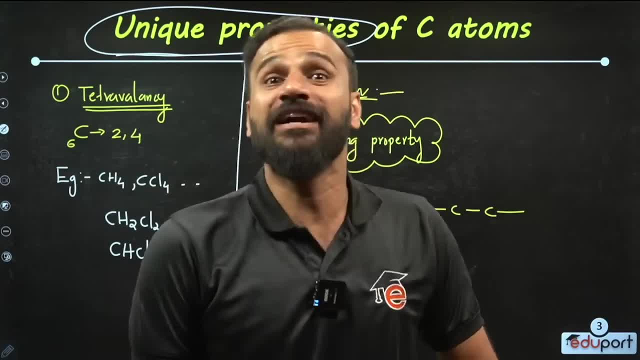 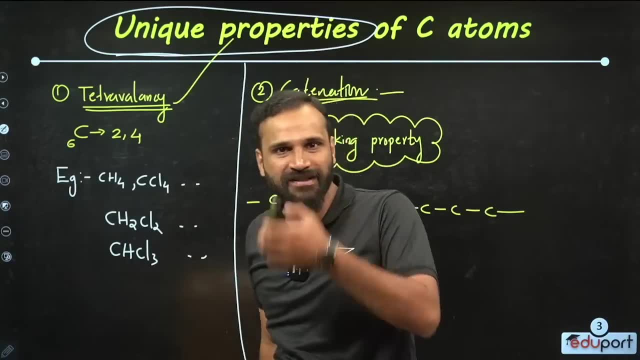 That's it. Catenation is a very important property of carbon. Two properties are mentioned. One is the tetravalence. What if I say that? What if I say that The valence of the carbon atom is four? Therefore, the capacity to combine with four atoms? 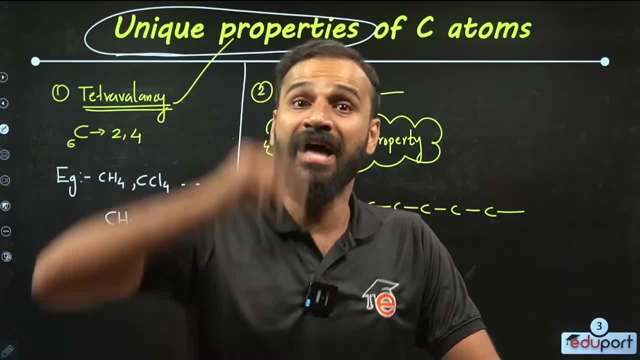 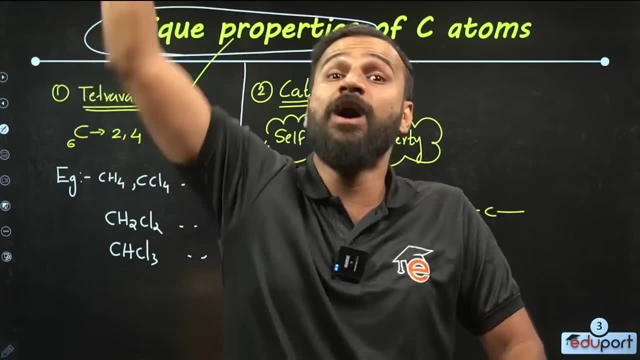 is there in the carbon atom. What is the second point? Catenation. What is catenation? Self-linking property? What if I say that, Combined with the same atom, Big chains or make big rings? Is the child okay? Is the child okay? 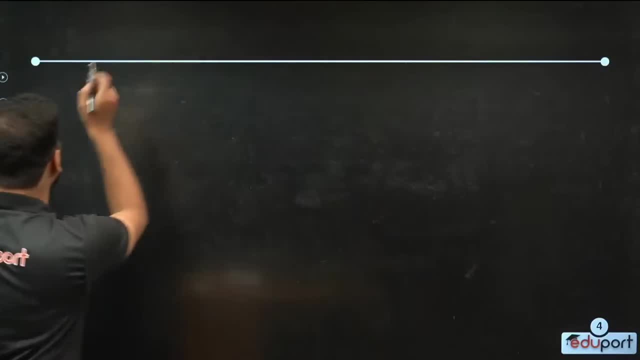 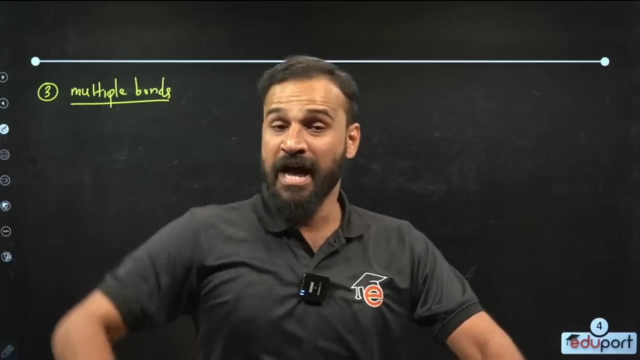 Concentration is not going. He is with him, Yes. third point: What is the third point? children- They have multiple bonds. What children They have multiple. The tendency to make multiple bonds is very high. Tendency for making multiple bonds is: 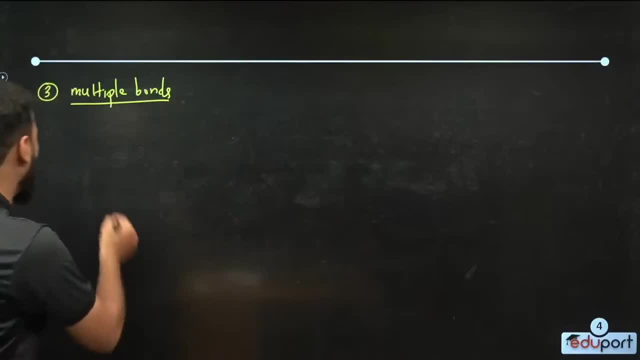 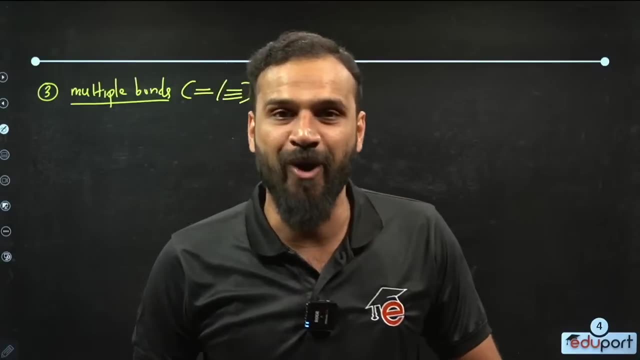 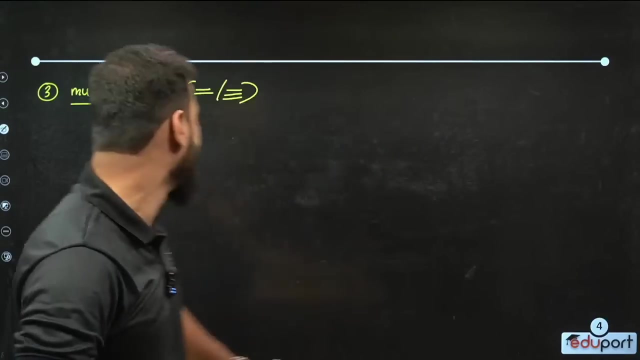 very high for the carbon atom. Who is the multiple bond? Children, do you know Double bond and triple bond? What is the name we call the double bond? Multiple bond? The ability of the carbon atom to make these multiple bonds is said to be very, very high. Children, look at you. 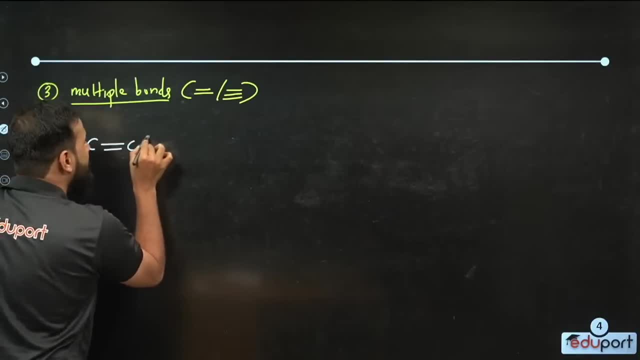 look at you. double bonds are made with carbon carbon. There is no doubt The triple bond is made with carbon carbon. We know. Is the double made only with carbon carbon Or is it made with triple? Not Carbon is made with other atoms. 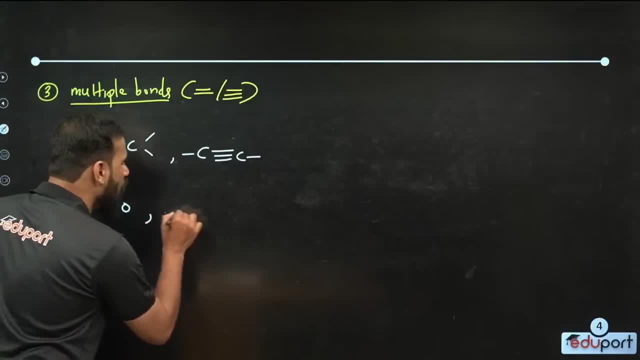 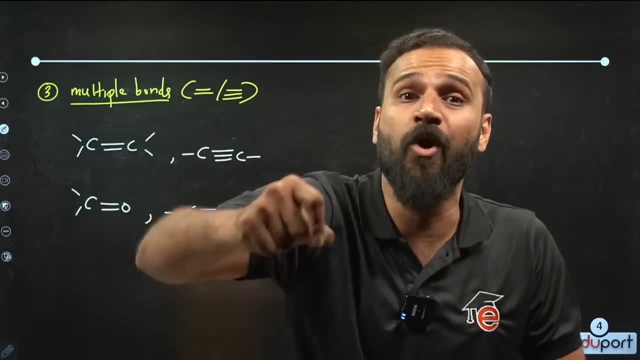 Double bonds, double bonds, Double bonus. See, Oxygen is made with double thee. only moment. Look, you are making a triple boron with triple boron. So carbon bonds for carbon atoms are the tendency to make double bonds and triple bonds say very high That is. 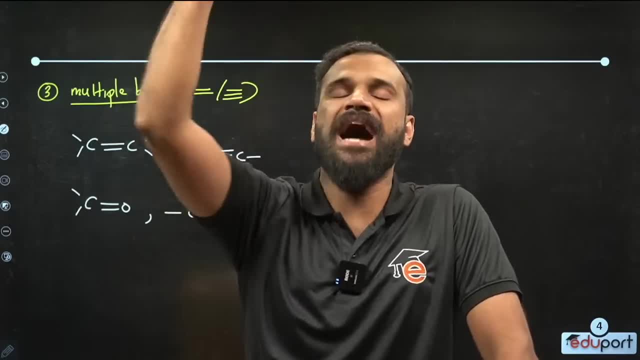 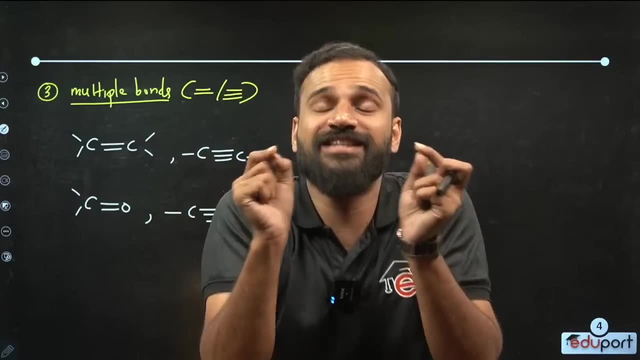 carbon is made with carbon and carbon is also made with other RX Show Tony Development. that is a very, very important thing. you have to be very careful. you have to be careful either. good to the brothers, make a good attention to the code, is it okay? Yes, now, children, people stating that this art is well taken care of, with a Bou pouvoir et Notier Wellnessкое Matter estar Çok Belo a A hiking positive. 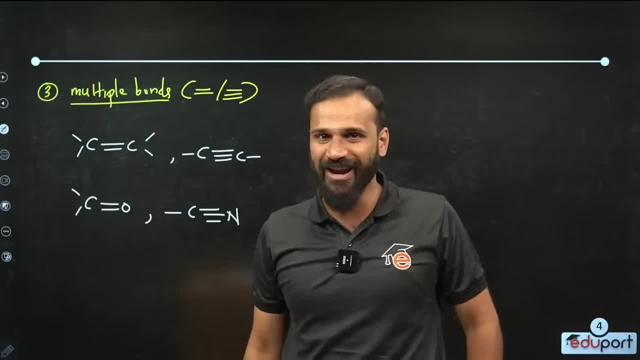 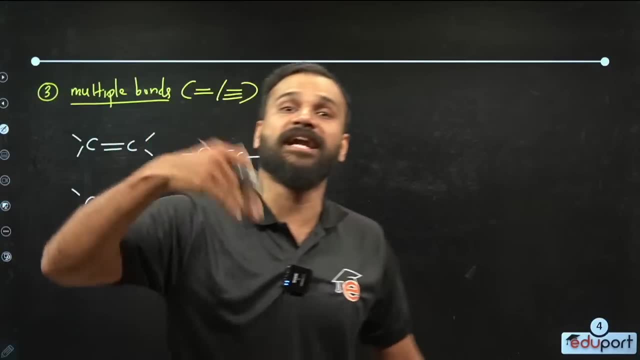 It is to be taken care of. It is to be taken care of well, Okay, Yes, now look at the children. There is also a fourth point. I don't have to say that In this chapter itself. It is a point that we can study in detail, That is. 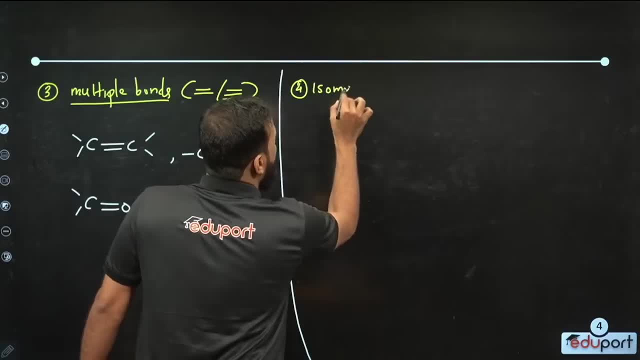 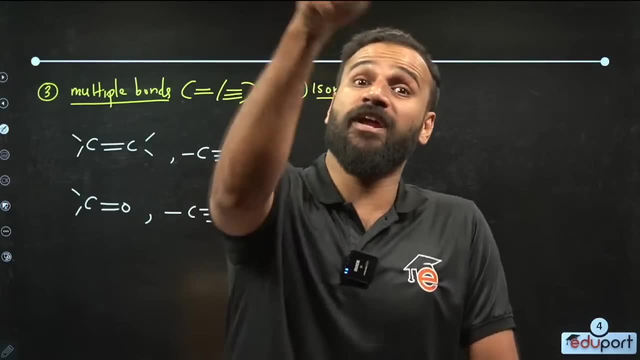 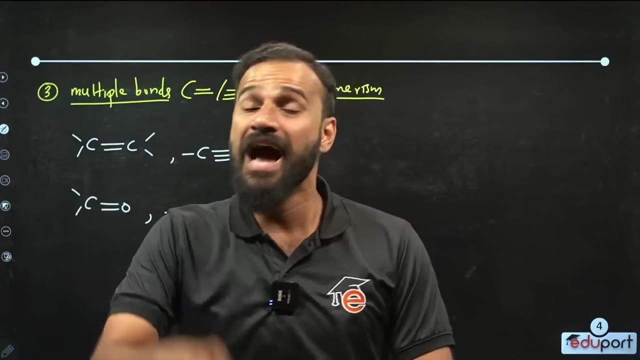 Isomerism. What is that, children, Isomerism? I am Not saying now. You all know Same molecular Formula and different structural formula. What do we call the molecules that show us? It is called isomers. That phenomenon is what we call. 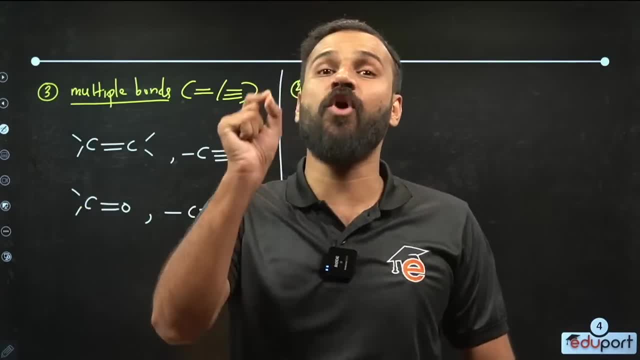 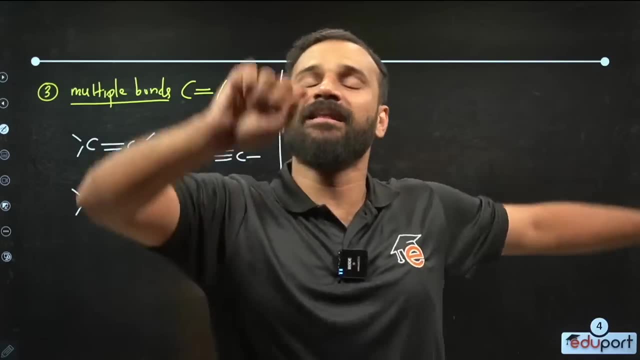 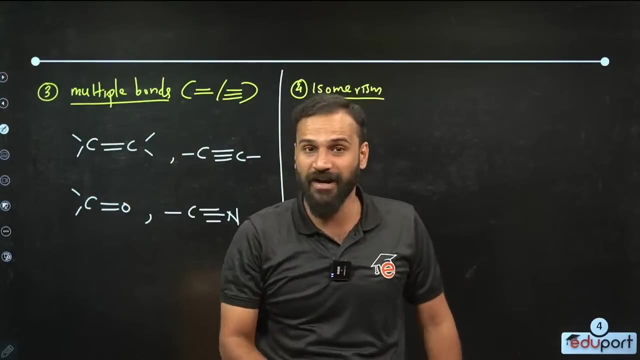 The name is isomerism- Carbon compounds. What does it show? well, It shows isomerism. I am not saying the example of it now, Because we have different types of isomerisms. What to do in detail After a while To say So, look at the children. What did I say? 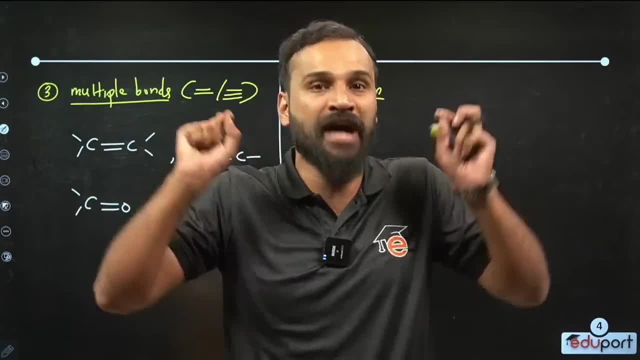 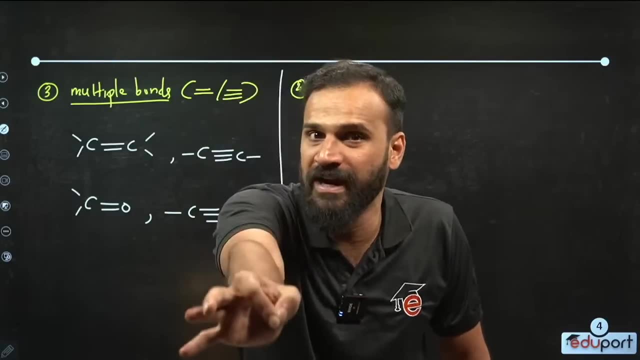 Today, millions of organic compounds. The reason for the existence of carbon atoms, At the end of the day, the reason for the existence of carbon atoms, Are four unique properties. What are the four unique properties? Now, you have to learn. You have to say it with me. 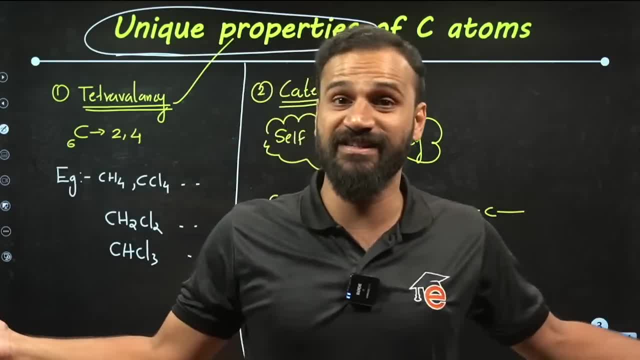 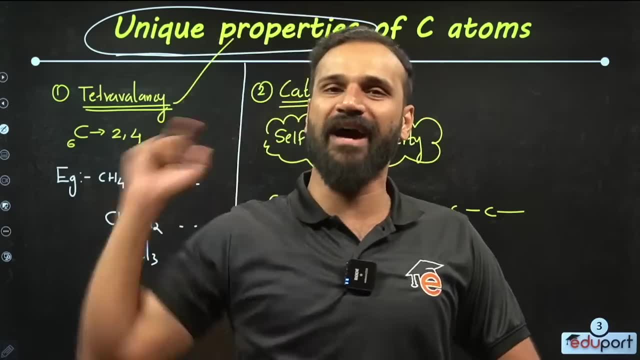 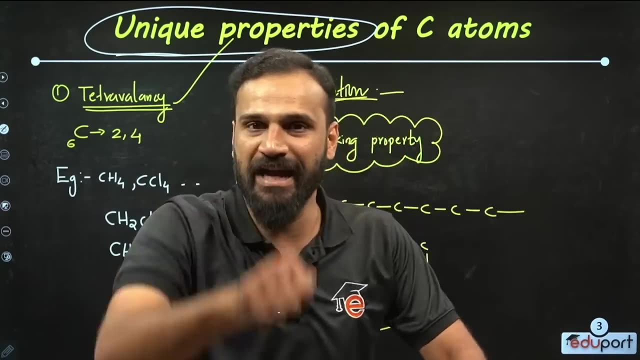 What is one? Tetravalency. What is tetravalency? There is a capacity to bond four atoms to a carbon atom. That is called tetravalency. Those four atoms Can be the same or different. The second is Catenation. What is catenation? Self-linking property. 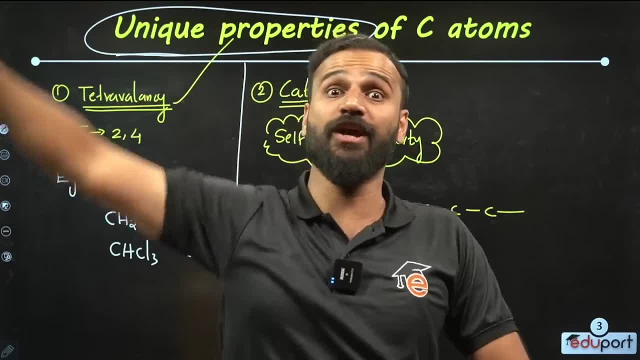 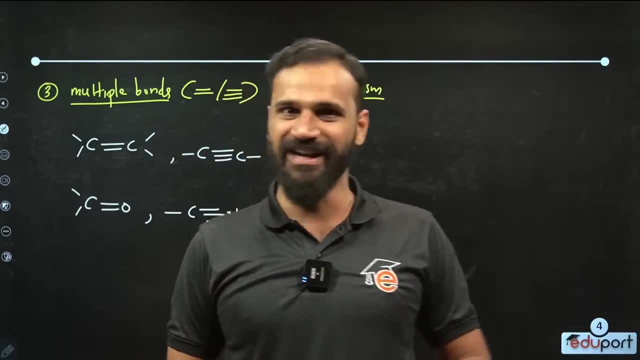 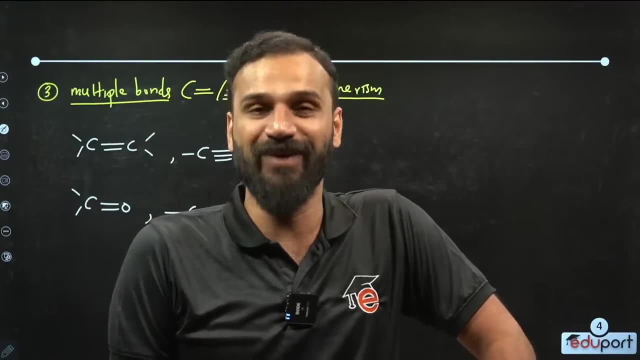 One atom is combined with the same atom: Big chain. The ability to make big rings is catenation. The third is the tendency to make multiple bonds, Tendency for making multiple bonds, Tendency to make double bonds and triple bonds. Carbon is very high. Finally, isomerism. 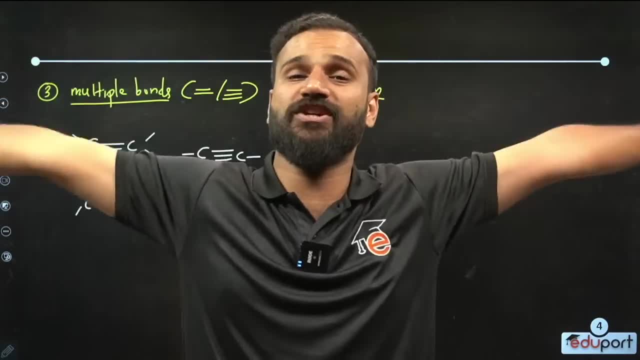 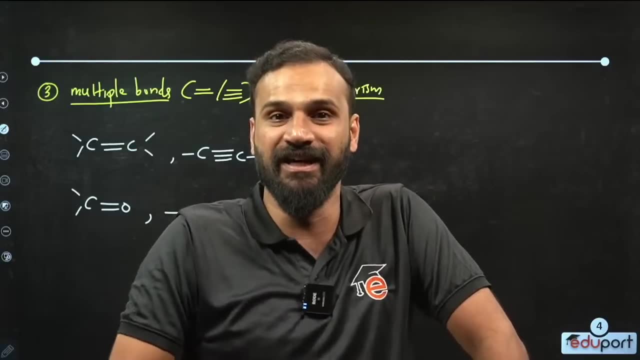 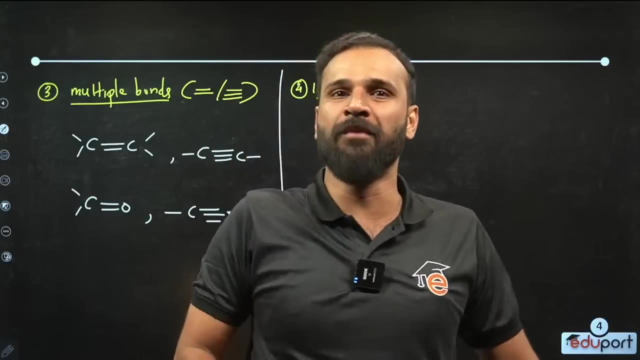 When there is the same molecular formula To show a different structural formula, The phenomenon called isomerism is called isomerism. What does carbon compounds show? well, Isomerism shows Children. what is it The first point or the first question I have for you? 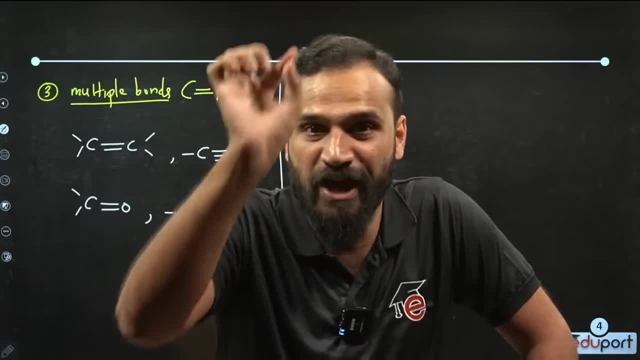 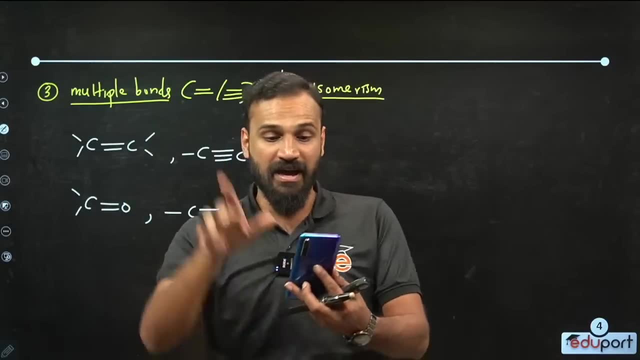 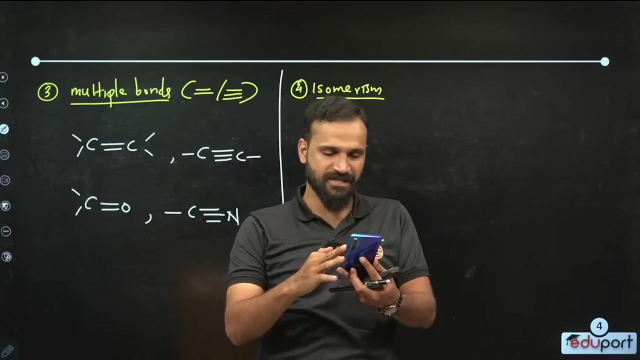 Are you okay with the four unique properties of the carbon atom? Are you okay with the four unique properties of the carbon atom? Children, say it quickly: The four unique properties of the carbon atom. If it is okay, say it quickly. Yes, Yes, Say it quickly. 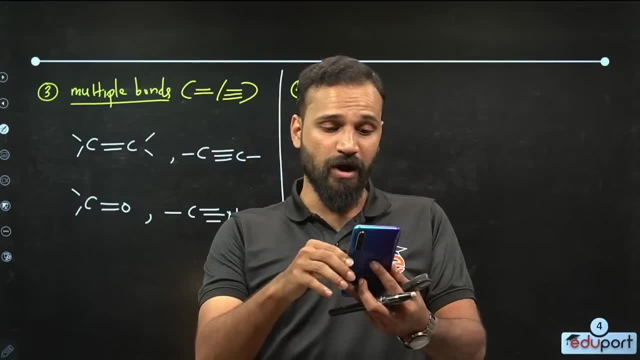 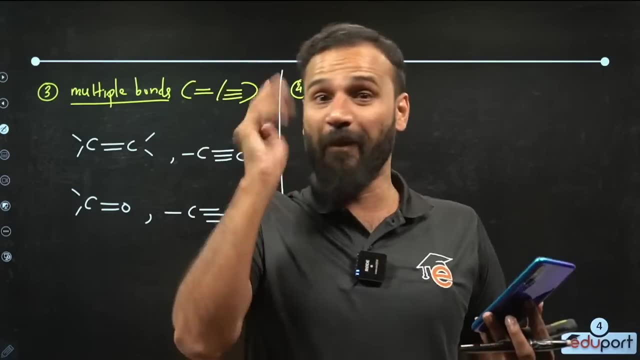 Say it quickly. We have just started gaming. We are somehow two hours away. Yes, Yes, Are you ready? That means quick. All are four unique properties. I have just started learning. If it is okay, then say it quickly. 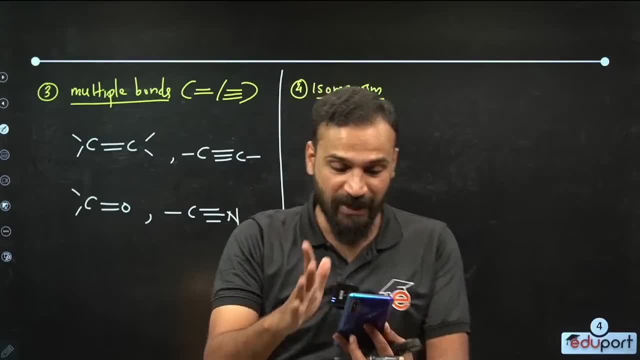 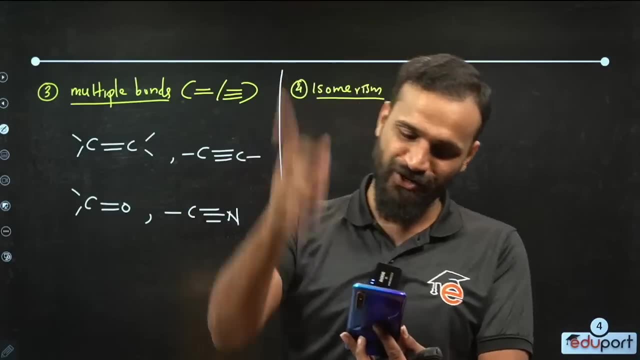 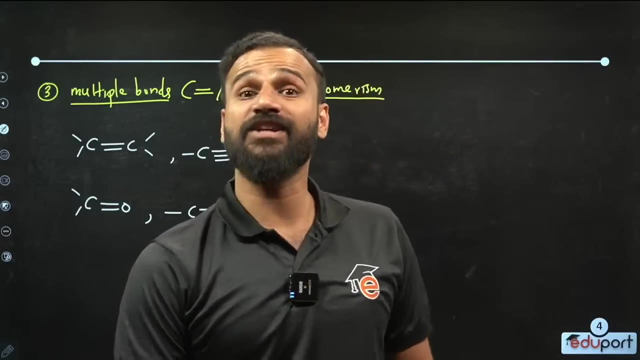 Let's not be late. Let's not be late. We have to reach the next point. Good, Very good, Good, Very good, Good leerr. Now, children, we're keeping on the exam. It's a topic that usually comes as quesion. 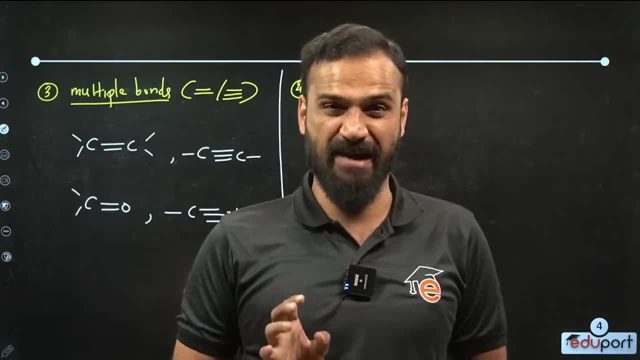 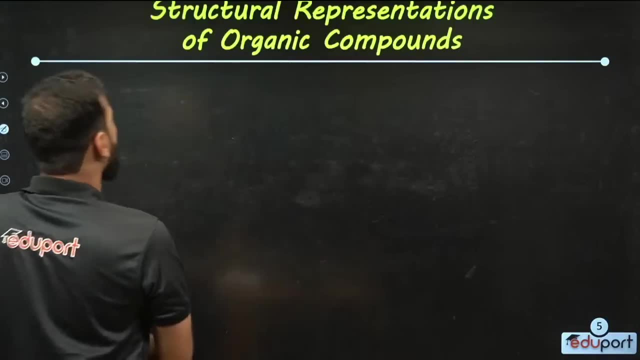 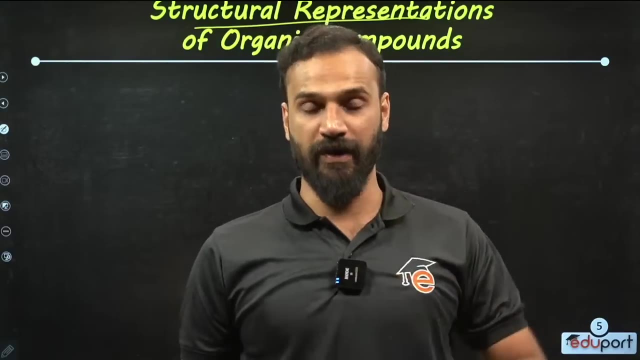 How can an organic compound be represented? How can an organic compound be represented? This is the main question. Look at the structural representation of organic compound. Look, an organic compound can be represented in four forms. You have to pay attention to this When I say to draw here. 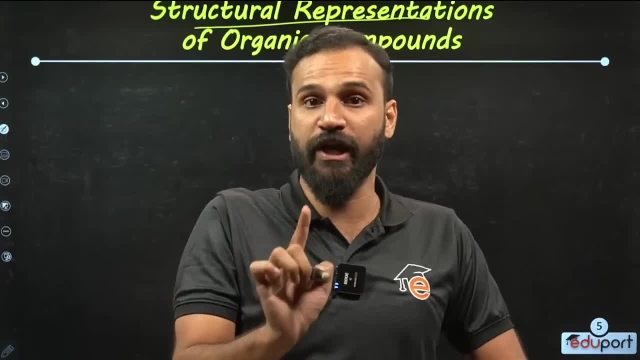 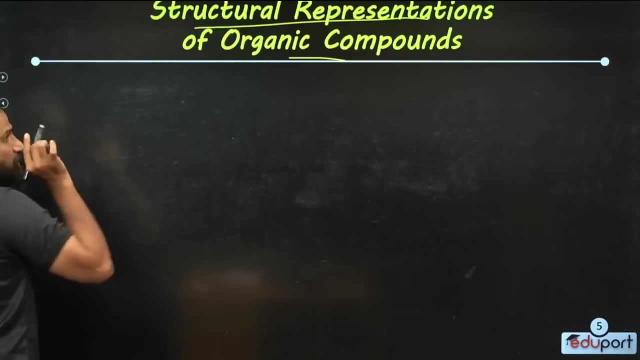 you have to draw it on the paper in front of you, Because this has to be drawn. the question is: to draw? Look, children, look. It was said that an organic component in four forms can be represented. The first representation of this is called: 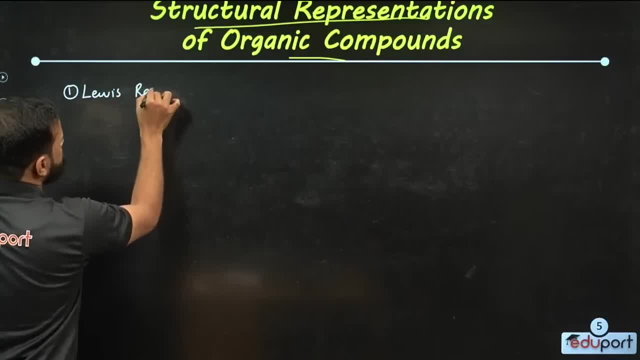 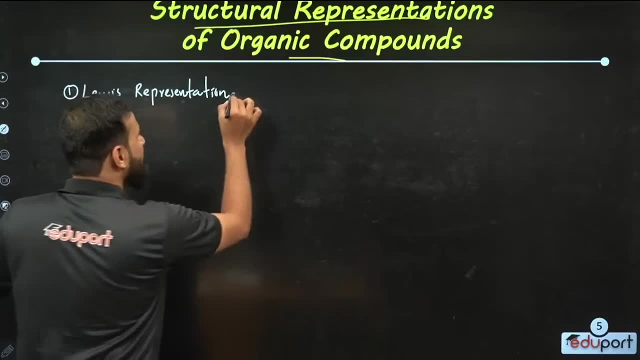 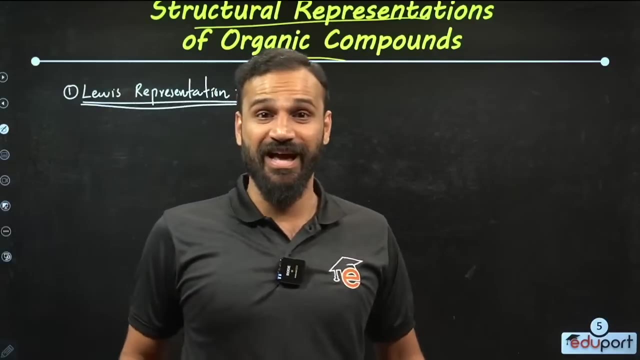 Lewis representation. What do you call that Lewis representation? This is very important. Which is the representation? Which is the representation, children? Which is the representation? Lewis representation? He says Lewis representation Or there is another name for it. That name is: 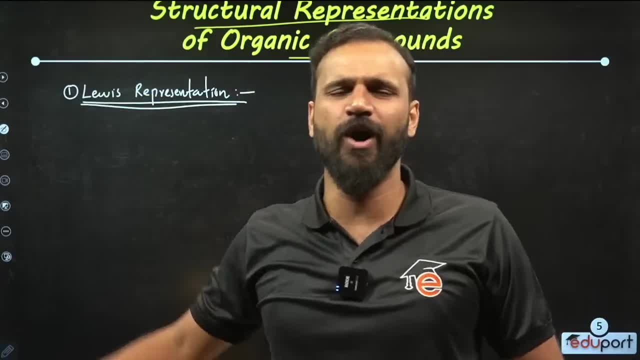 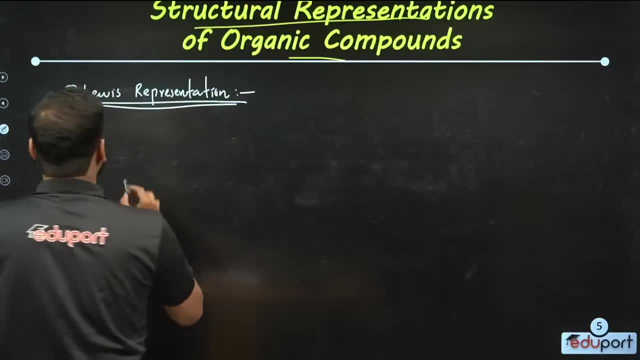 When you say it, it will run into your mind. Do you know why? This is a feature that we take and say: Not even Do you know what the reason is? Because We have learned it in chemical bonding. That's why, Look, look, we call this the electron dot formula. 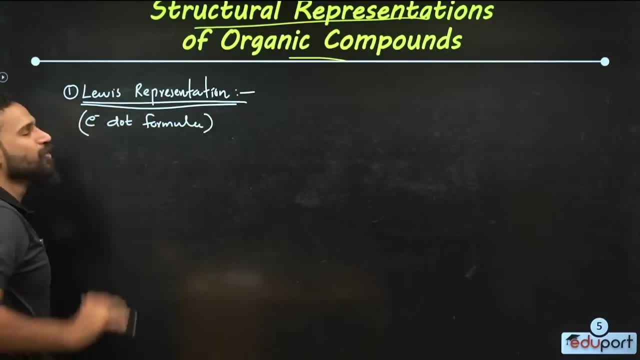 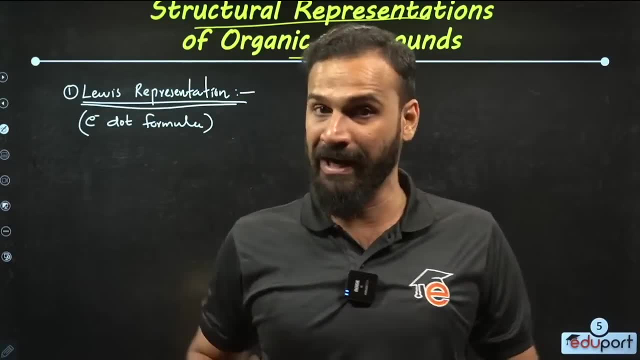 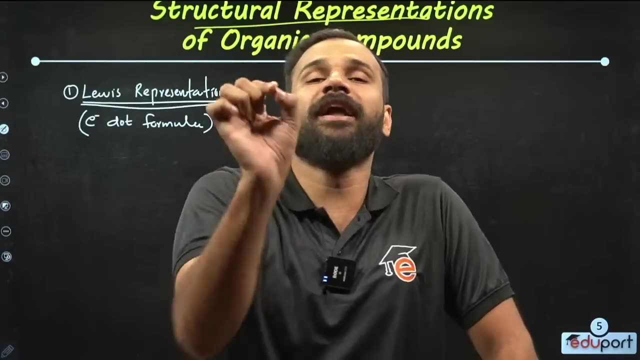 What to say to you? Electron dot formula. What is that? There is nothing to say. Where are the covalent bonds coming from? What are you guys? Where are the covalent bonds coming from? Change that covalent bond. What do we give in return? 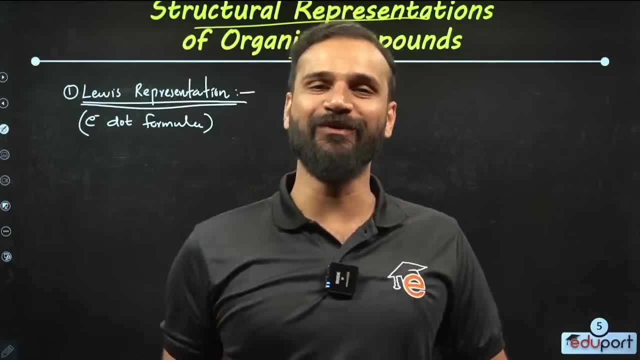 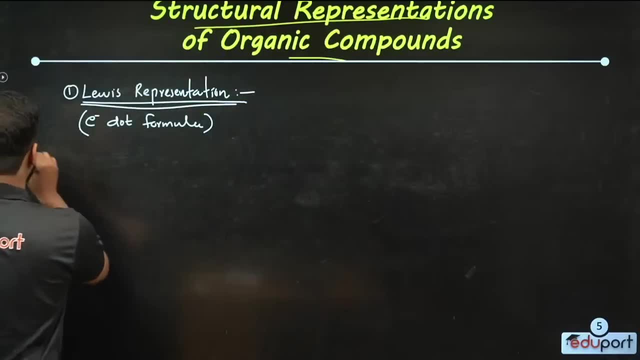 What do you give in return? Give a pair of electrodes. This is the Lewis representation or electron dot formula. I'll show you. I'll show you. Look, if you go to the example, If you go to the example, We take an ethane. 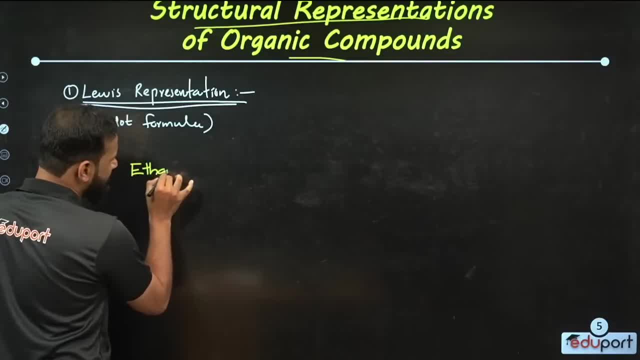 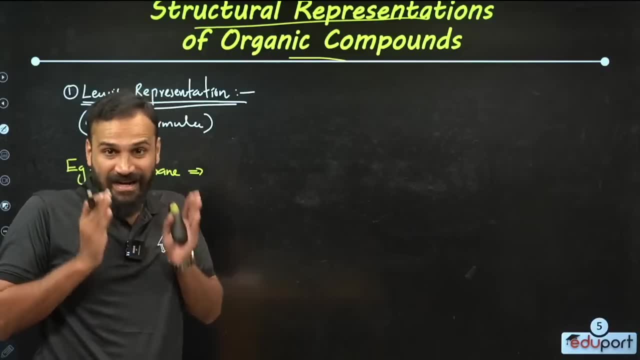 Think about it, guys. Which one do you take? Ethane, When you say ethane to your mind, CH3, single bond, CH3, single bond, CH3 will come When it comes. two carbons, If you say ANE. 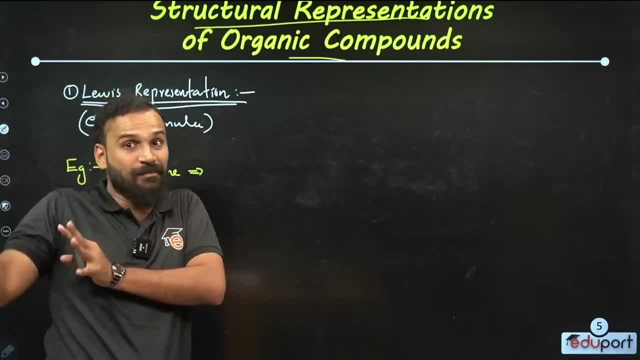 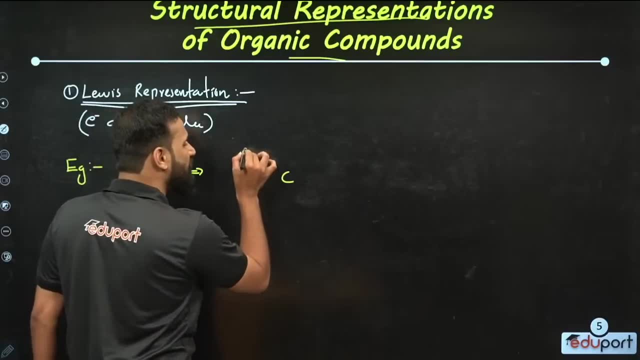 Single bond. That's it, This honey. Then CH3, single Bond, CH3 will come to your mind. But look, How do you know the Lewis representation of it? Look, Three hydrogen with one carbon, That's it. CH3, Single bond, CH3.. Three hydrogen with the next carbon. 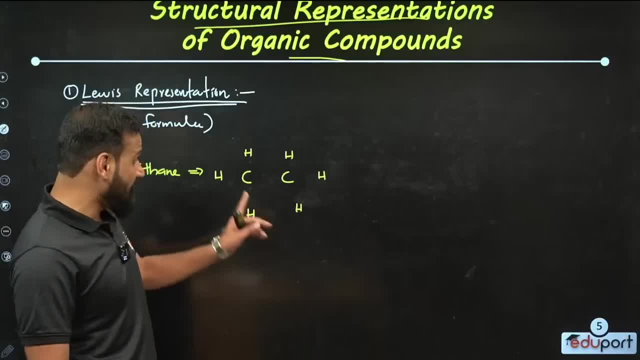 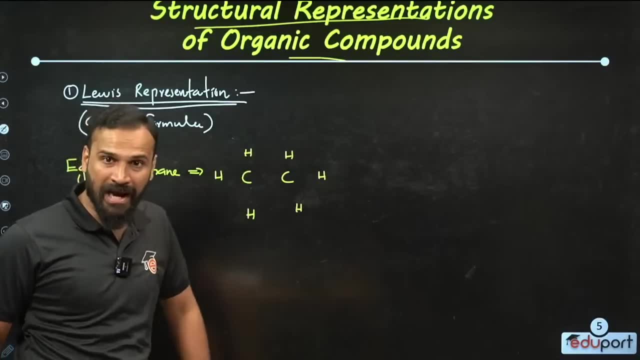 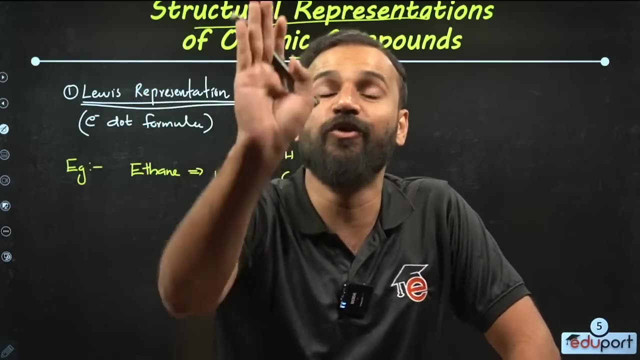 Isn't this guys? CH3, single bond, CH3.. Now, what is it here? One single bond. What is it here? Single bond Here, Single bond, Isn't it? I leftover the single bond that, If that one pair of electrodes is the Lewis representation, Look, guys. 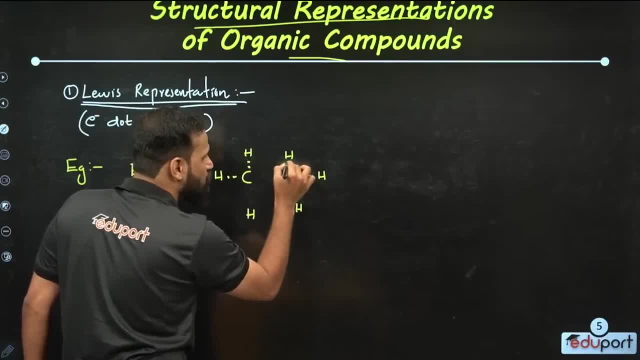 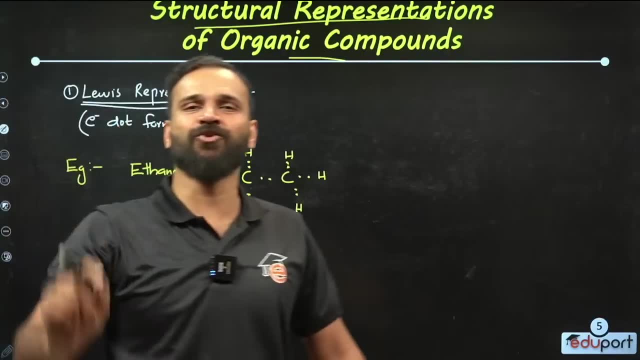 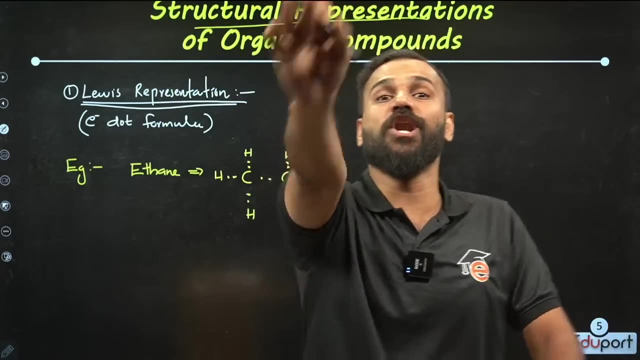 A pair of electrons. Here is a pair. Here is a pair Offered Here is offered. Here is offered Here is Okay, Brandy, change Bond changes. It is called electron Many. If so, that is called Louis representation. 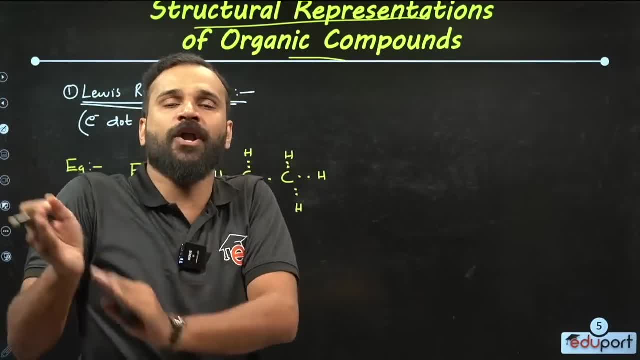 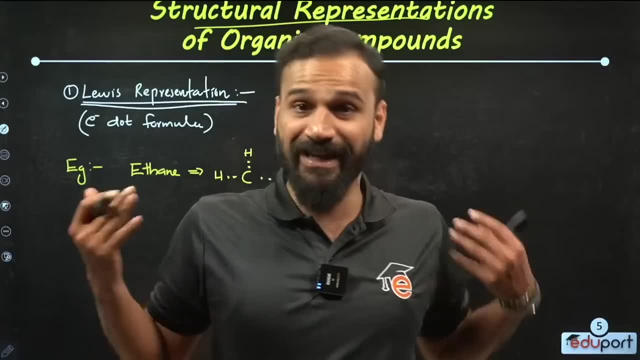 Uncle, it's okay, isn't it Nothing? Instead of one bond, Put it in one pair. So if there are two bonds, Two people should be put. If it is a triple bond, three people should be put. That's it. If so, children, look at it. 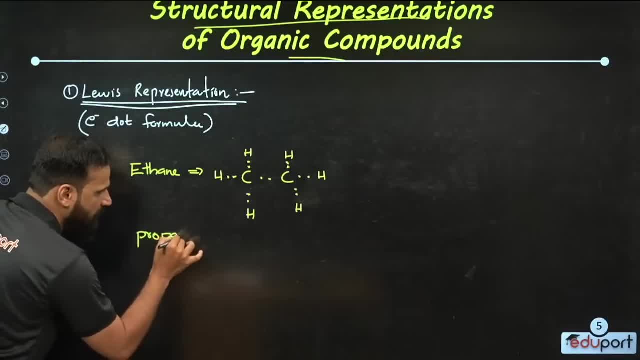 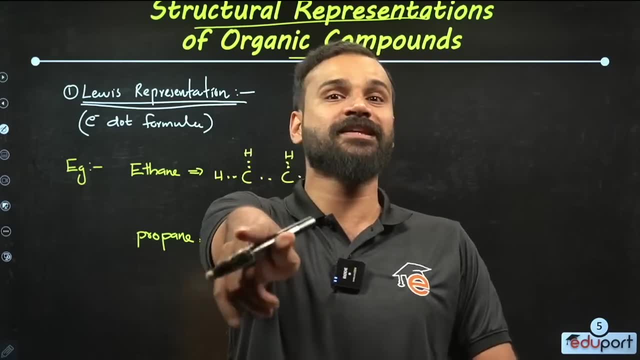 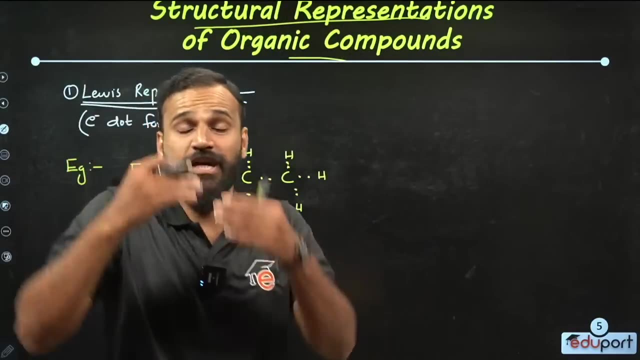 You try to draw propane. You try to draw propane, Propane in the paper in front of you. You have to draw, That's what I said earlier. You have to write it. You have to draw- That's very important- Propane. you draw What propane? CH3, CH2, CH3. 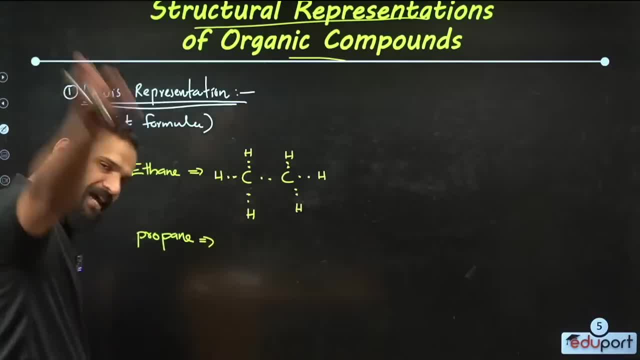 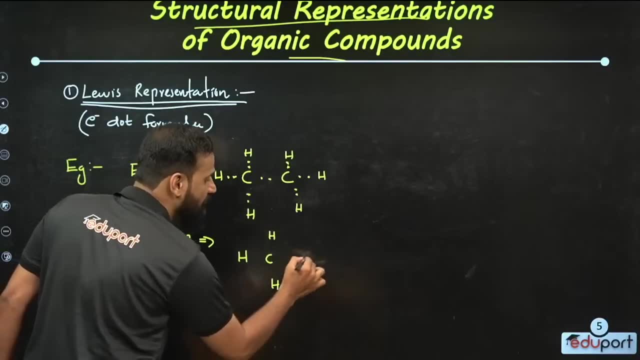 Call propane. Yes, yes, you try Here. Don't look, Don't look, Look at this, Look at this, Look at this. children, Just look at the drawing, Just look at the drawing, Just look at the drawing, Look at this, Look at this. Where is it? 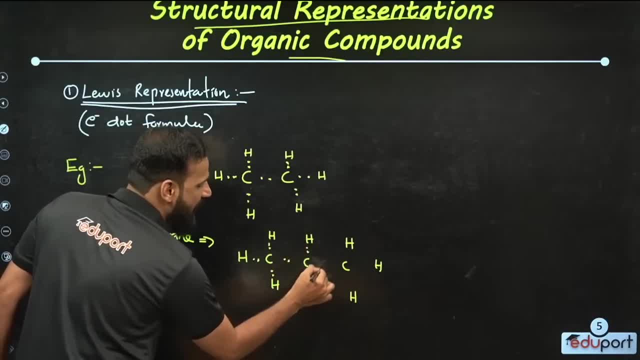 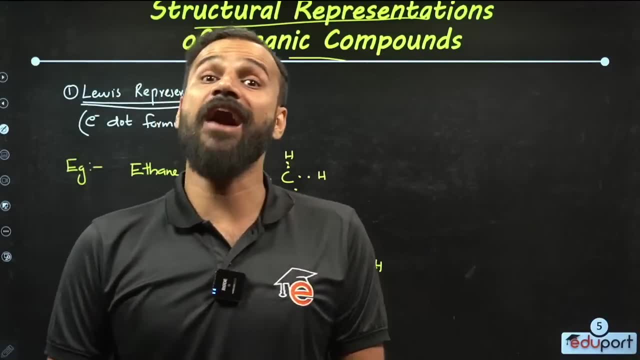 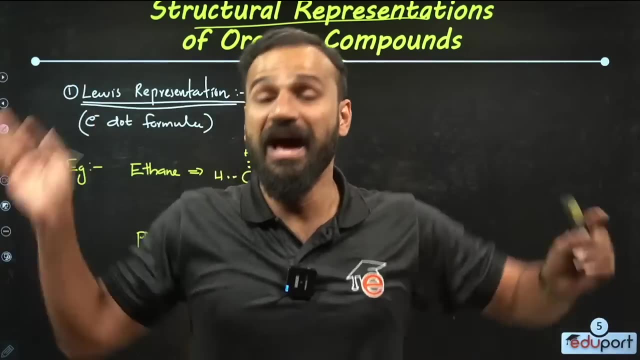 Single bond will come. Change that, After changing that, After changing that, If there is a pair of electrons there that is propane, What, children? That is propane, Isn't it? How simple is it? How simple is it If it is butane, you know? 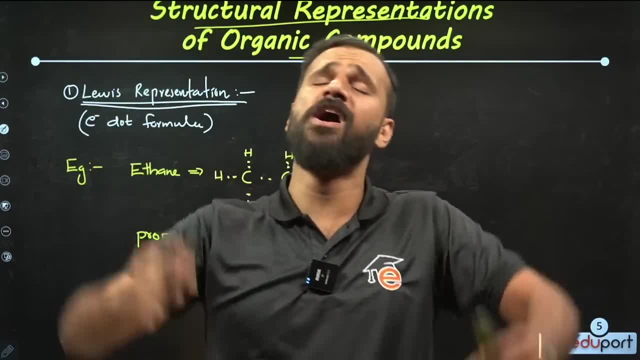 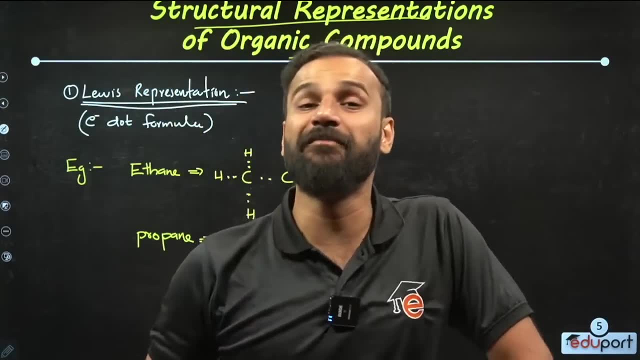 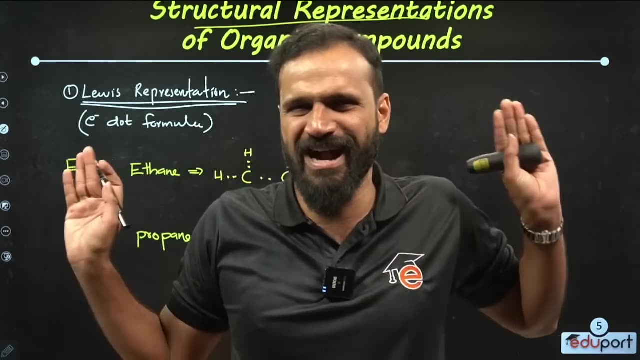 Whether it is pentane, hexane or heptane, We can draw anything Because of the name of the electron. Instead of a bond, an electron name. The name is in the Lewis representation or In the electron dot formula. everything is for everyone to know, for everyone to know. 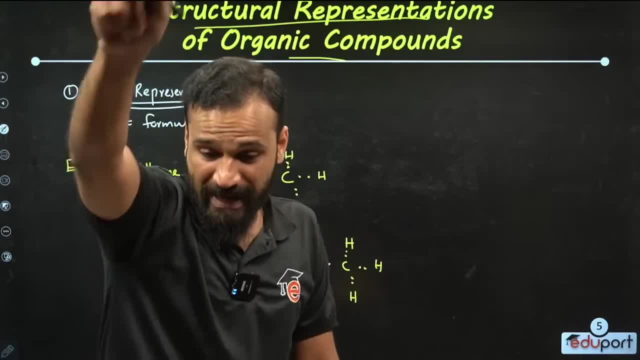 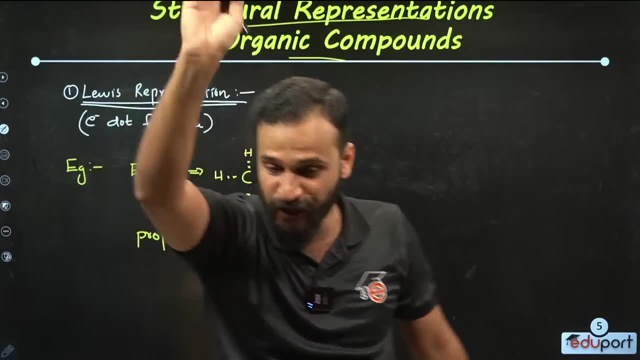 It's okay, right, It's not okay. If it's okay, If it's okay, don't stop talking like this, Sir, it's okay, It should be said. It's okay, It should be said that it can be done. 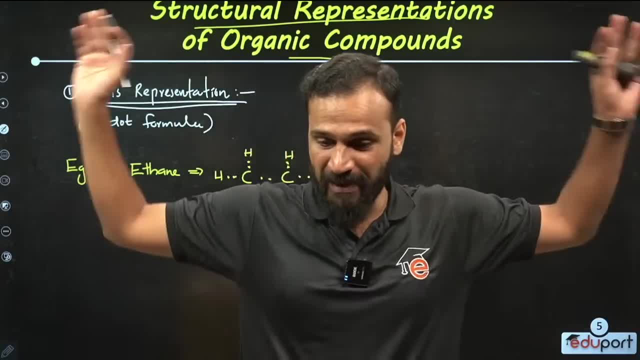 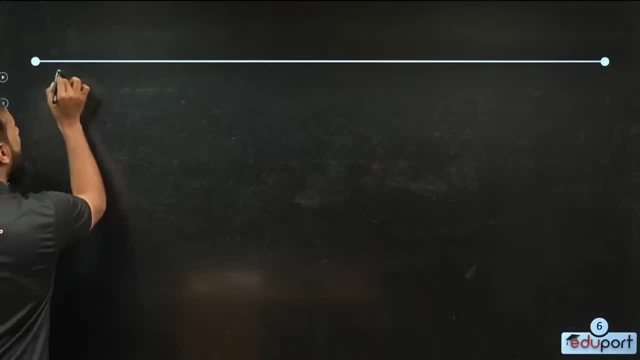 yes, yes, very good, very good. okay, not children Ready? not Is not ready. yes, very good, very good. Now look children. What do you know next? What is the next representation? Do you know what the next representation is? That is very important. For that we call for it. 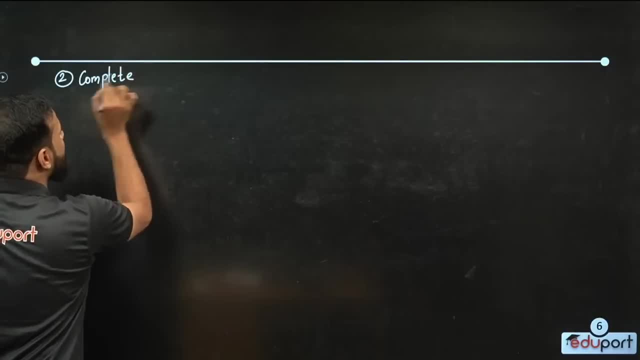 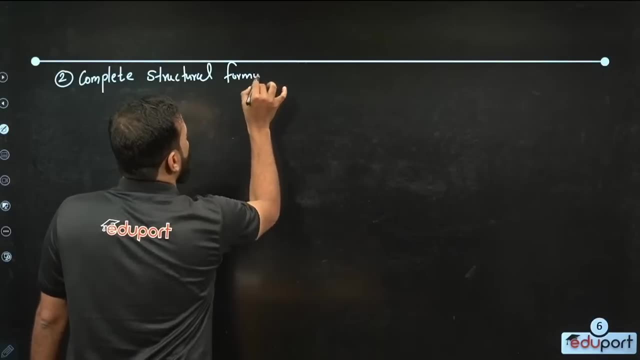 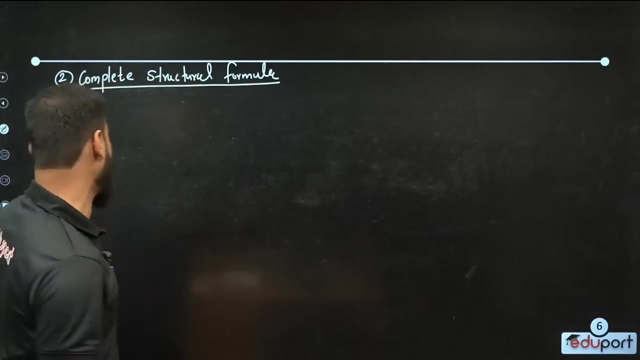 period in the tour bar total to each other in the complete structural formula and the monthly complete structural formula and the McLeod in the period complete structural formula in the world, the parent of an angle, para and the Mario. graphical representation in the representation on a graphical representation: graphical 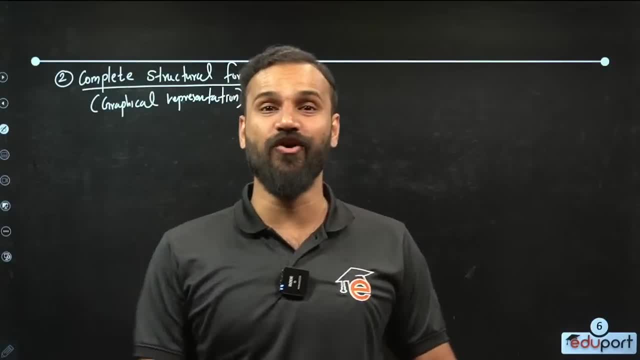 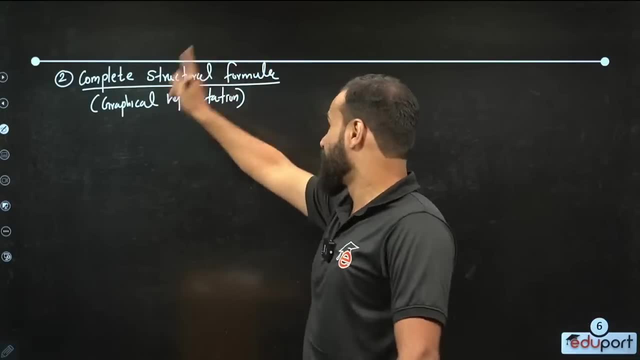 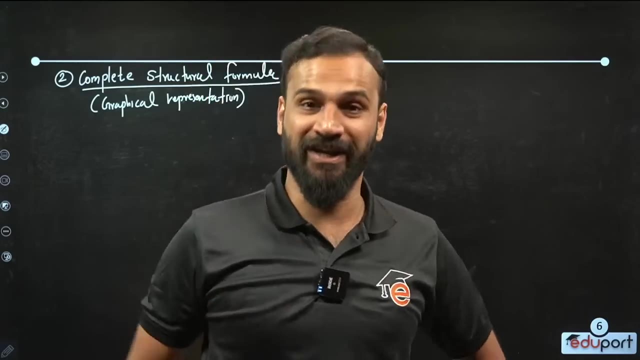 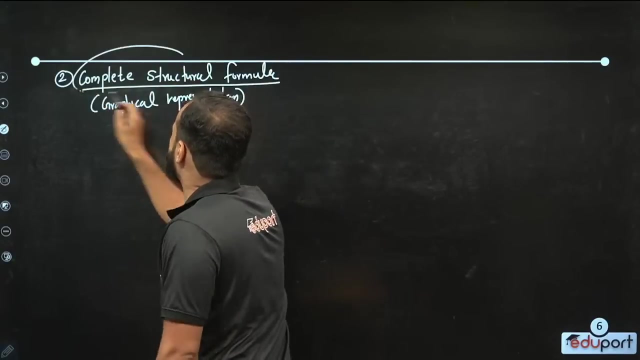 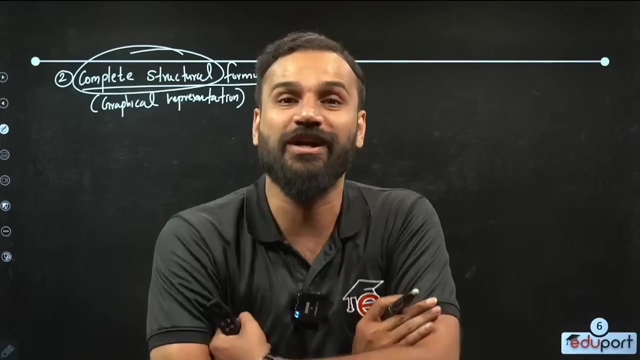 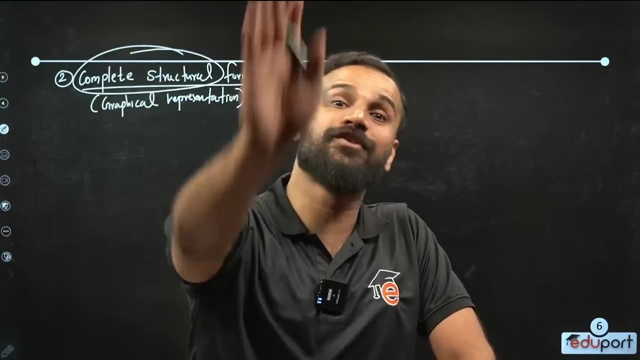 representation: complete structural formula in the graphical representation. complete structural formula in the graphical representation. This is very, very, very important. And the complete estructural formula I do the protecting of aiente and the complete title of person D over an ale at along in唔 ing настро present. 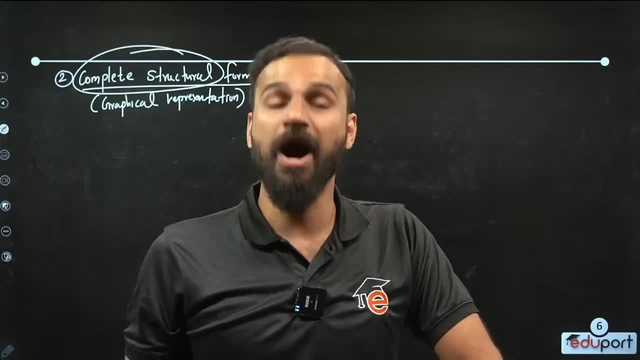 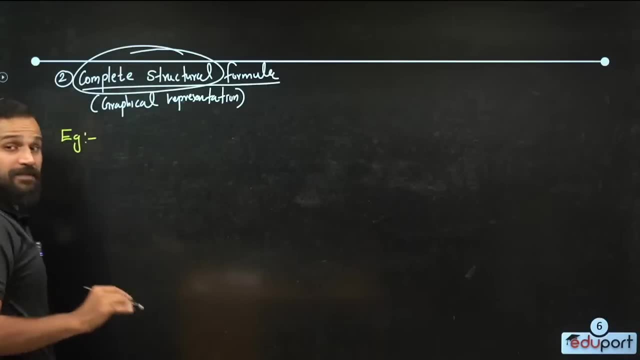 to You, puedes, you don't Ellabήσ on Children represent, Do you know? I put the company guy You know, number per annum approach, Oh, ok, Ok, Oh, first love, look my grey example: more Cup It the earth, Good. 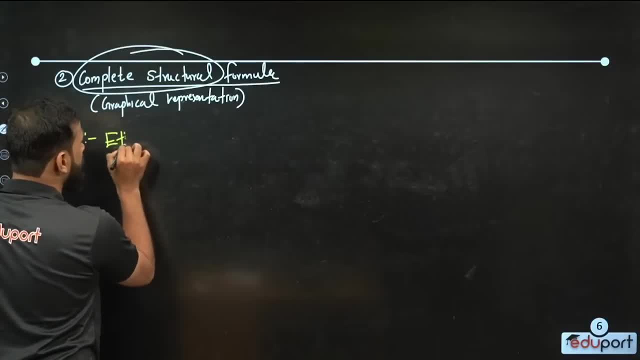 thought they eat the indigenous colour. They are thirty three of the. if they're into to eat a lot in themNOK a look today. ر Choi Sandi, I m a present here. No cook, No cook In, you know, and I make a. 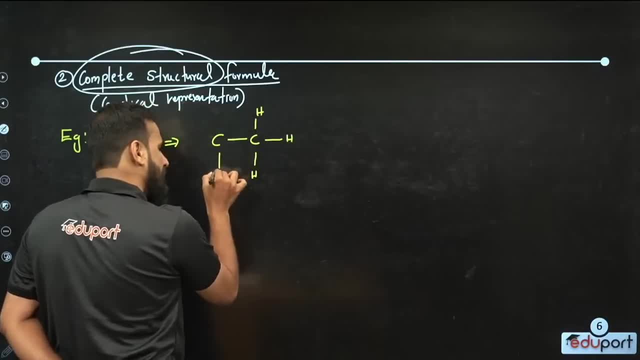 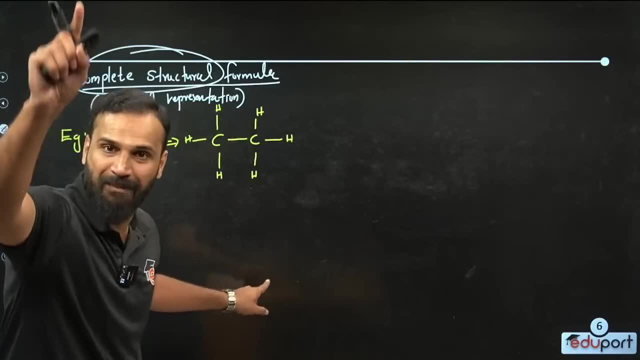 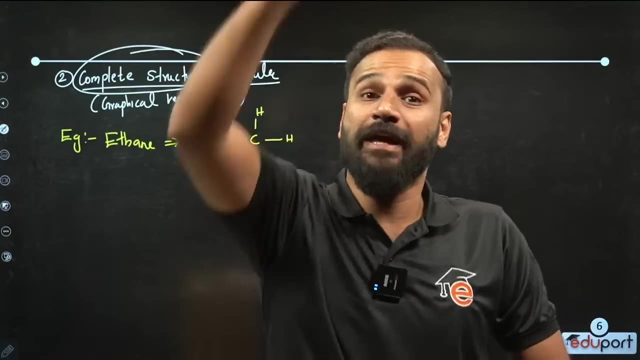 I represent you. Isn't it like this? children, I represent you. Isn't it like this? Represent? My question is any. Have I not represented any acts or not? Have I not represented any bonds or not? If all the acts and all the bonds are clearly represented, 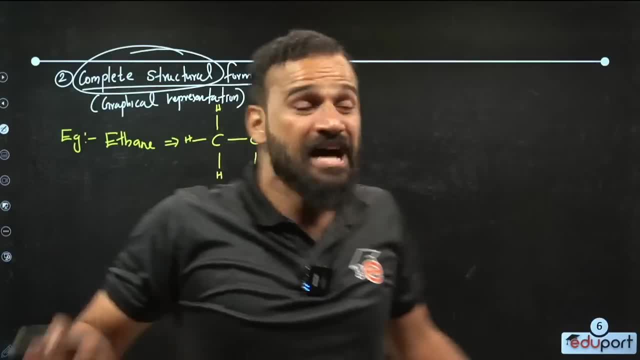 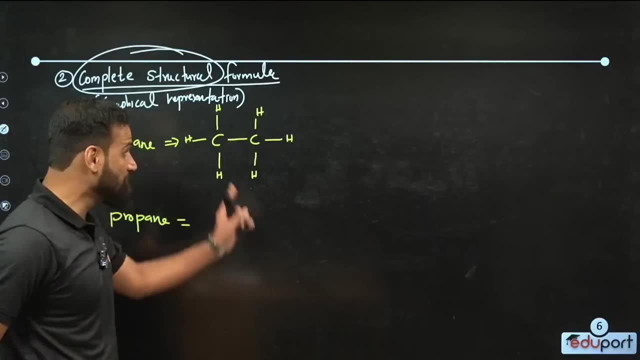 That's the complete structural formula: You try, you try, You try. children, How can we do propane, Propane? This is what I wrote, simply to make you understand. As soon as this is said, I will give you the question asked from here in the previous year. 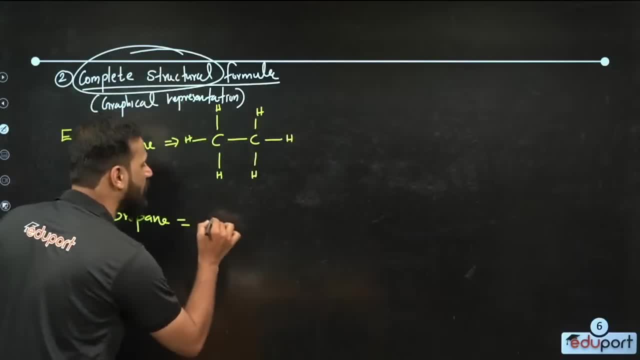 I will give you the question I asked you from here in the previous year. Don't worry about anyone. Look How is propane coming. children, If you want to come, you don't have to say it, You write in the paper in front of you. 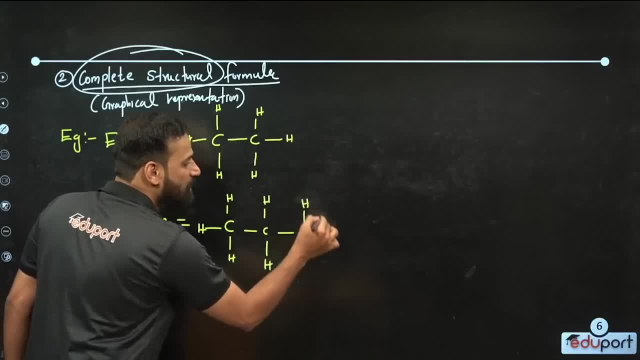 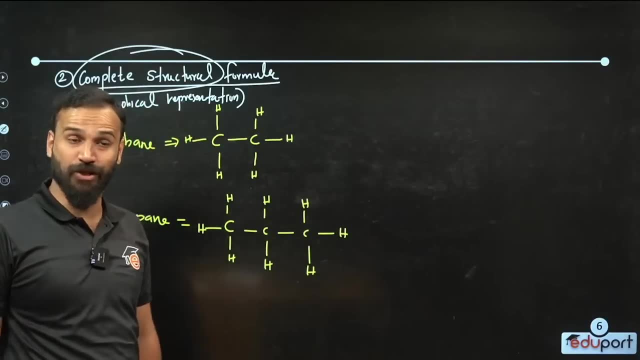 Write and see, Write and see. Children are like this. right, Propane is coming. What is the reason? What is the reason? All We represented, the acts, All the bonds Represented. If it is butane, it is the same. 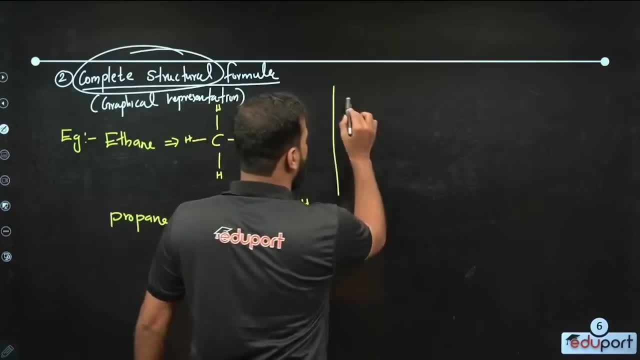 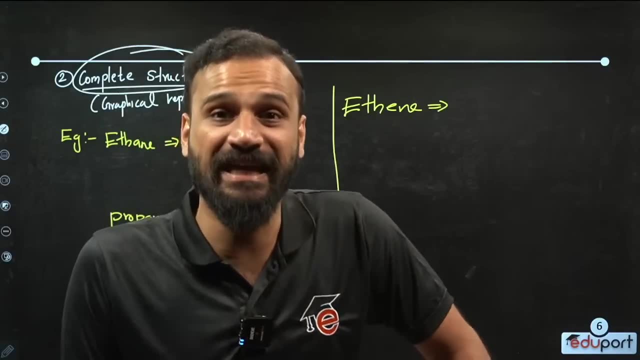 you Did you write the vaccine for women, Isn't it? Yes, children, Let me ask. I am asking you If it is ethylene. If you say ethylene, it is two carbons: E and E is a double bond. 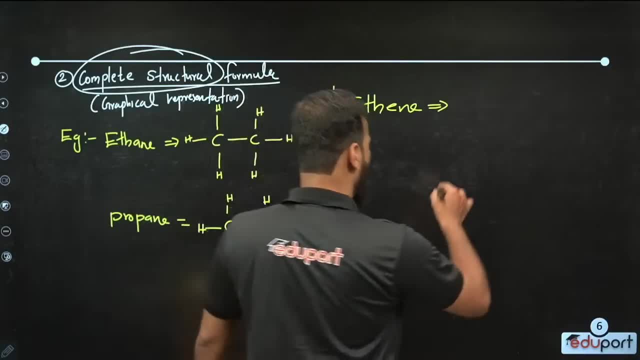 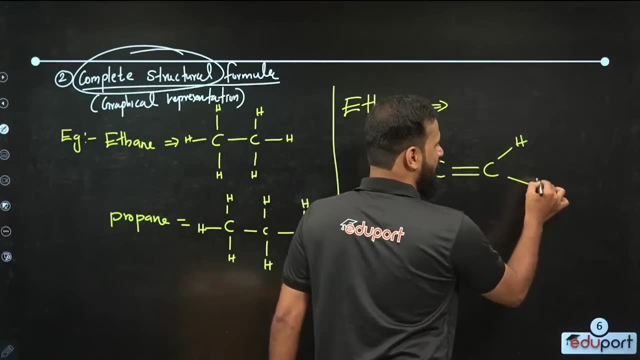 So if a double bond comes, we know it like this, isn't it? All the acts and all the bonds should be represented. Look at one: How much hydrogen is in the hand of the carbon Two hydrogen Children. how much hydrogen is in the hand of one carbon Two? 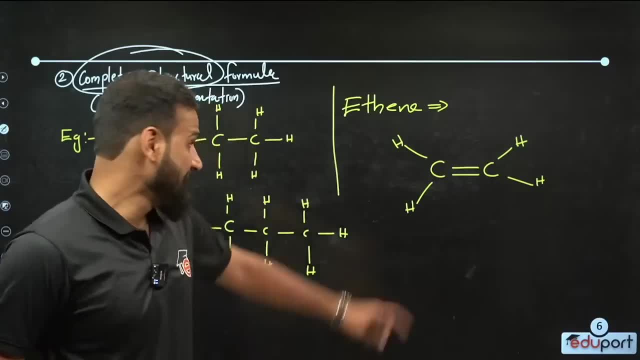 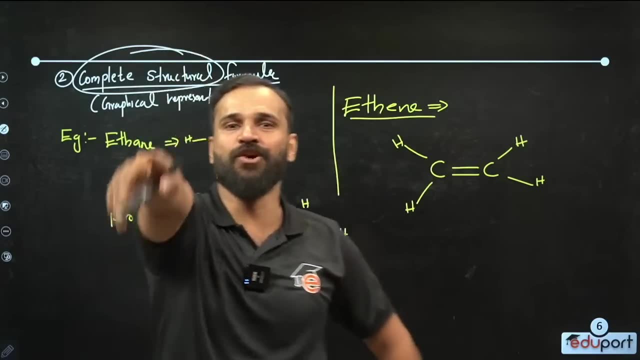 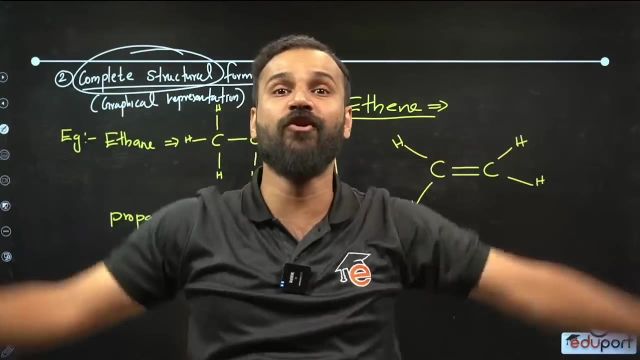 Hydrogen. This is what our ethylene says. This is not what ethylene says. Yes, we can tell you from ethylene. So all the pawns and all the bonds, If you can represent, that is the same: the complete structural formula or a graphical 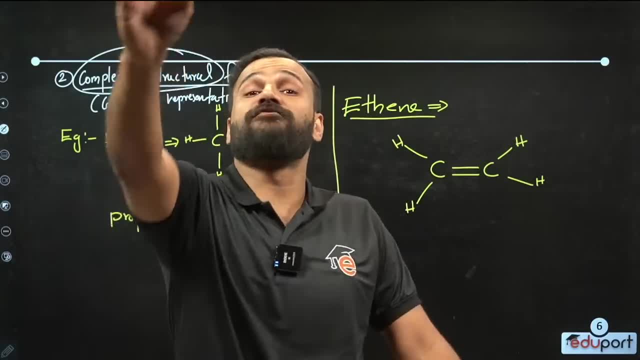 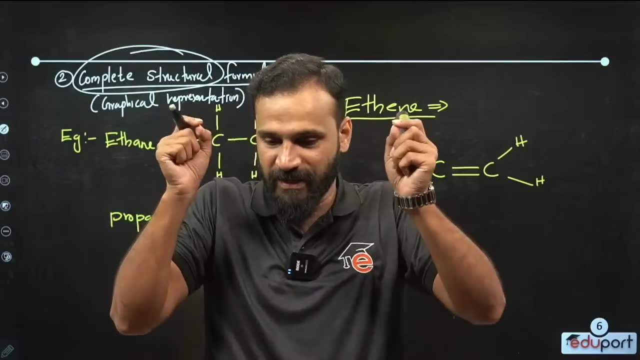 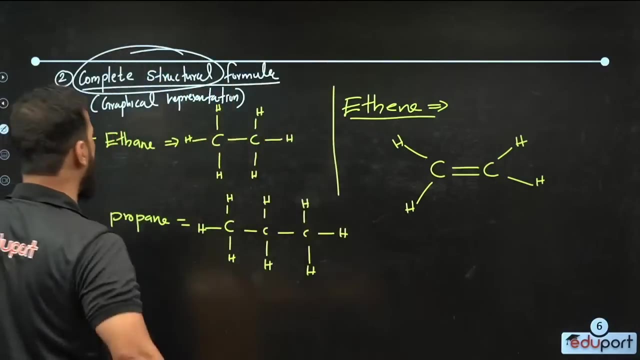 representation, graphical representation. If it is ok, children, very important, Say: this is what I ask. If that's okay, you Have to comment. If it's okay, you have to comment. Yes, this is very important, very important. 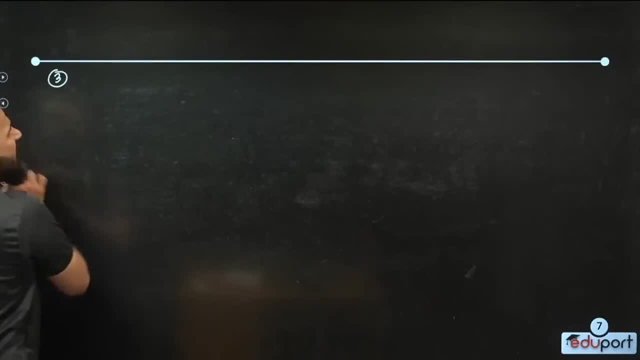 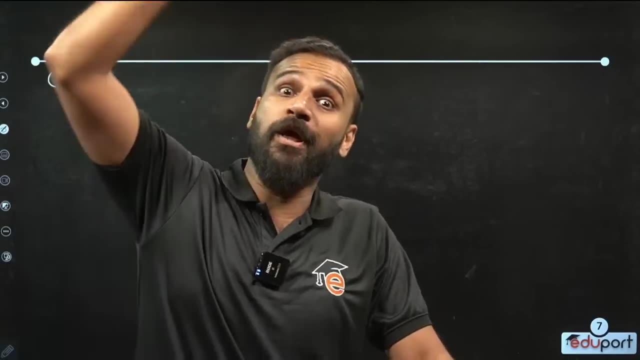 What is the next? What is the next? What is the third? To hear the name one is an electron dot. Represent as an electron dot. item Two: complete structural Structure is represented completely. All atoms, all bonds are represented. What is the third? 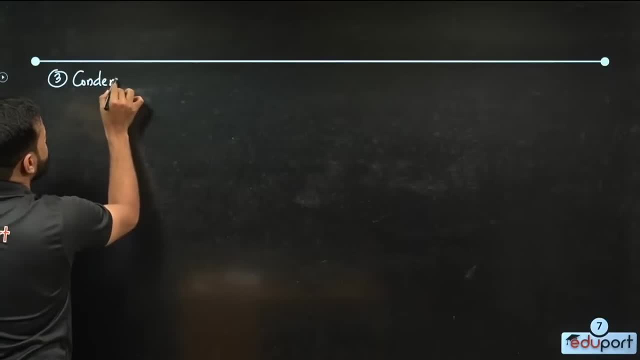 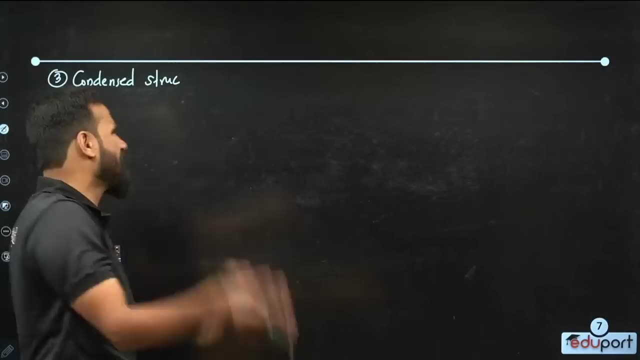 The third is condensed. What is it, children? Condensed structural formula. Now, without saying structural, you can say it is a condensed formula. There is no problem. Condensed structural formula. Condensed structural formula. What is it, children? 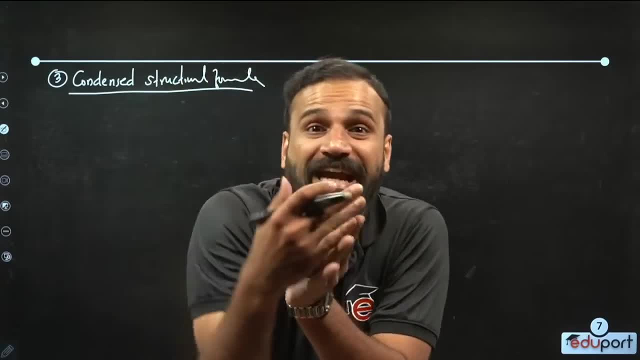 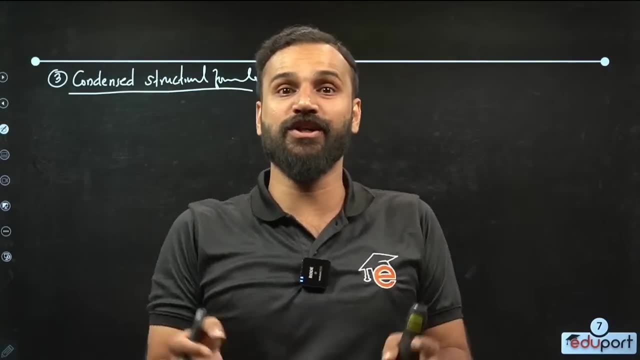 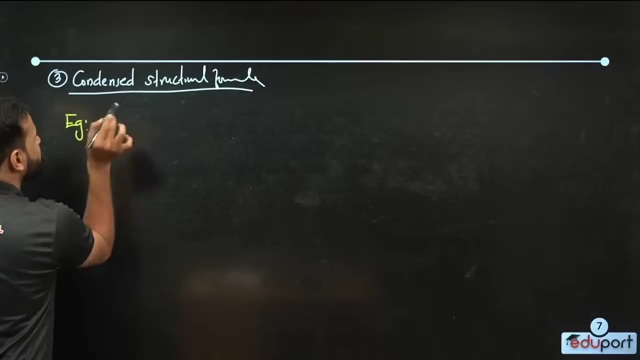 Condensed is not shortened. Condensed is not shortened, Isn't it? If you say complete, it is completely complete. If you say condensed, it is shortened. How simple it is. look, look, look, Look. we can take the same example we took earlier. 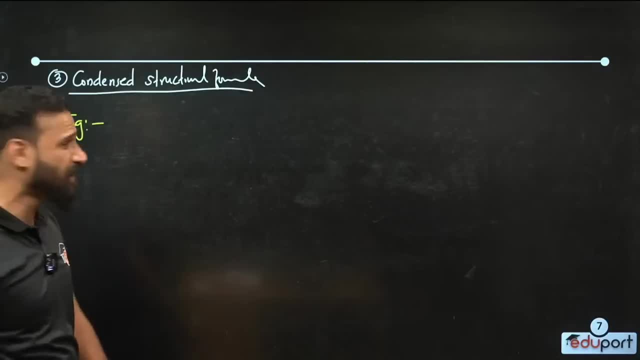 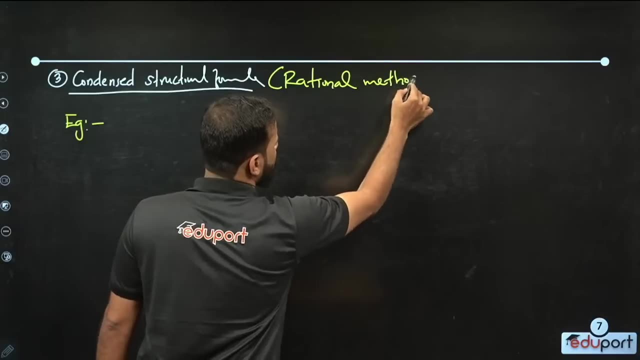 Then for complete- sorry, is there any other name for condensed? If you want, we can use the rational method. Then we can call it a rational method. What is it? children Rational method? What is the other name for condensed children? 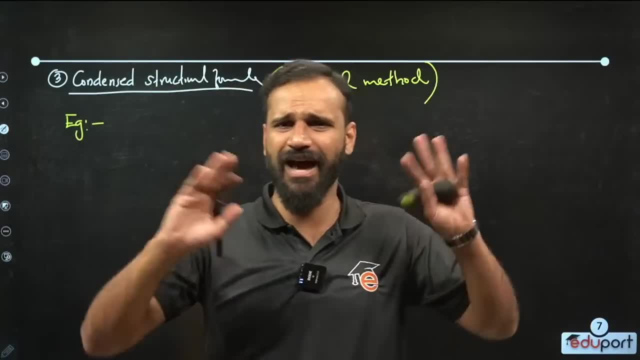 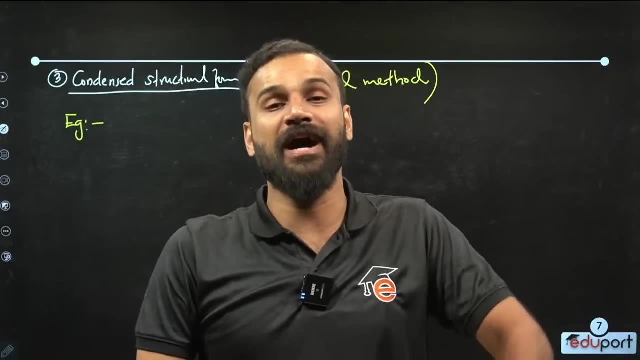 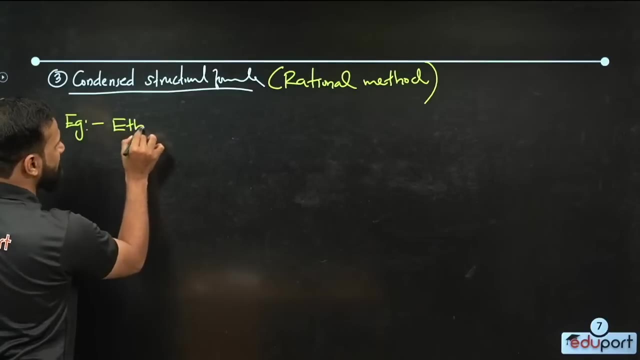 Rational method. What are they doing? Shortening is not such a big matter. Decoration is not needed. Shortening is the complete, sorry, condensed formula, or condensed structural formula. I'll show you what it is. Look. didn't we take Ethane earlier, children? 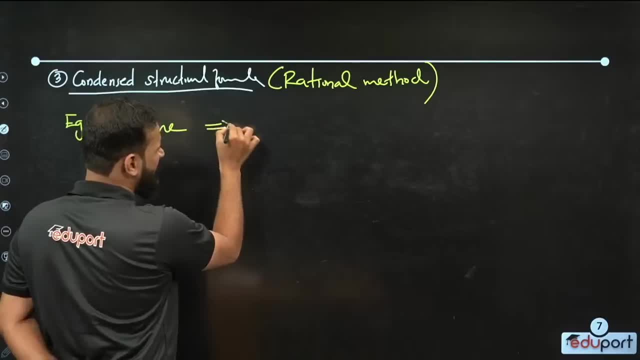 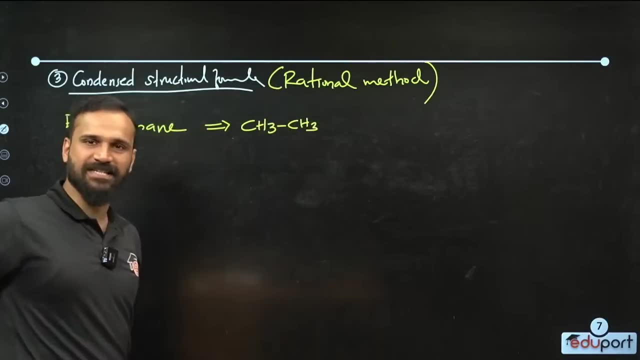 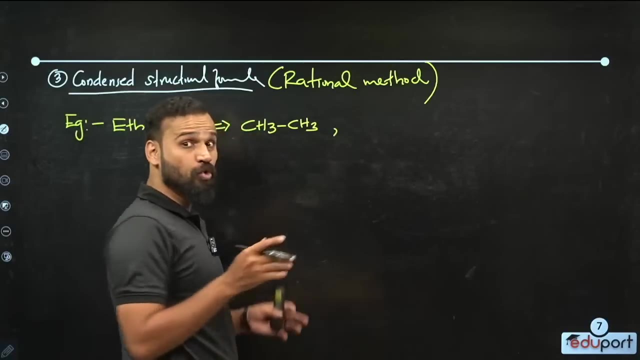 Isn't it, Ethane? Look at Ethane. how is it shortened? write it like this: We usually write this, honey as CH3, single bond, CH3, like this. Just write it like this. Ok, Now, if you want, you can write it one more time. How? 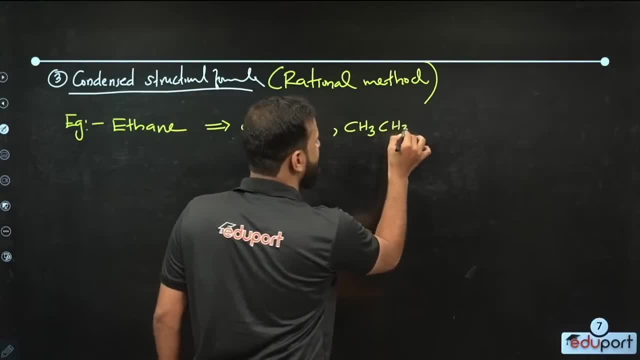 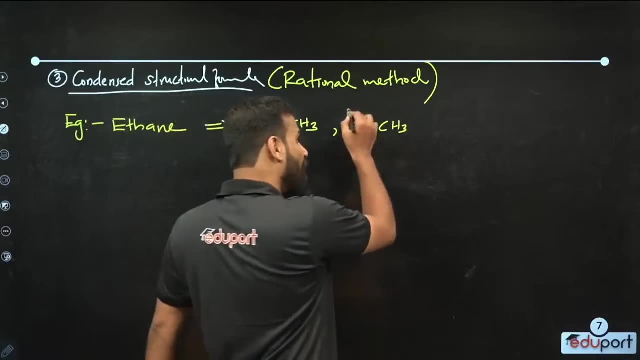 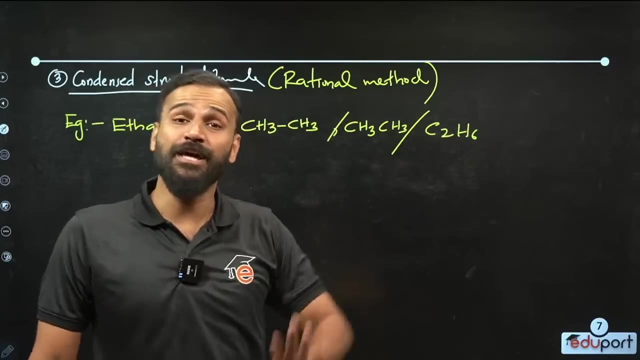 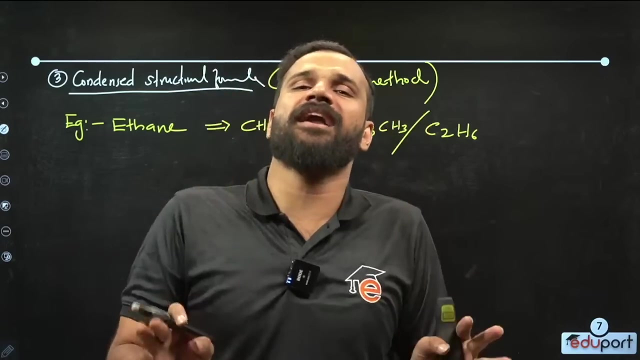 CH3CH, that is, avoid the bonds here and write CH3CH3.. Or you can write it as C2H6 one more time. What is all this? What is all this Condensed formula itself? It is a shortened representation itself. But what we usually write. 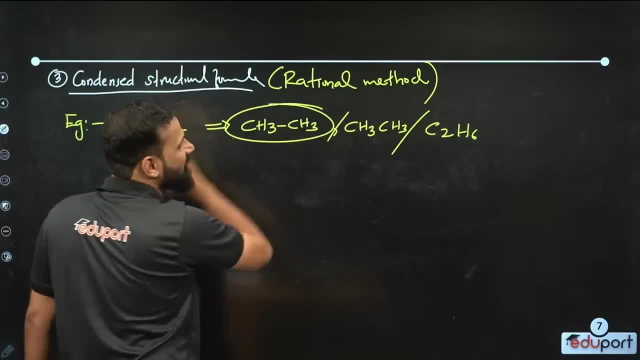 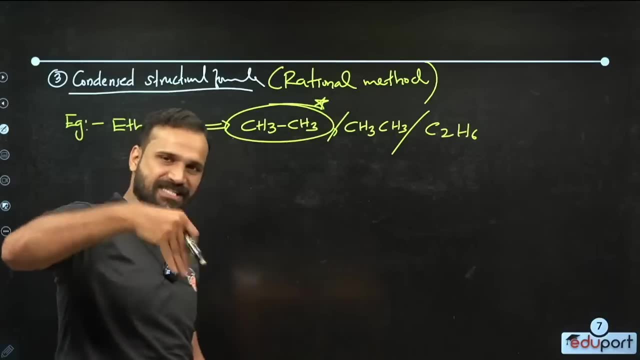 You also have to write it like this: So this is not condensed. This is not condensed, But this is what we usually follow: CH3CH2CH2.. So that's it. Ok, This is what we represent. That is what is meant by condensed. 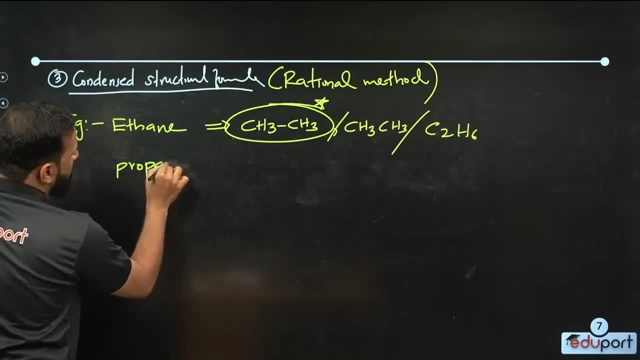 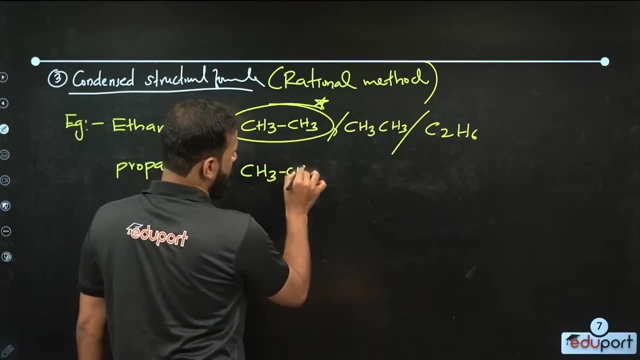 If so, children, tell me. If so, tell me. Propane: How do we represent propane? How do we represent propane? Propane: CH3CH2CH3.. This is condensed. You can condense more than this, but no. 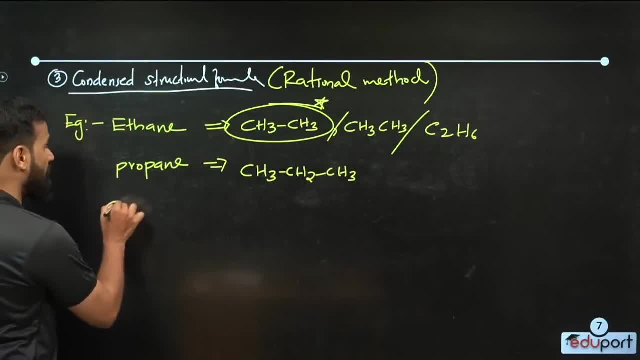 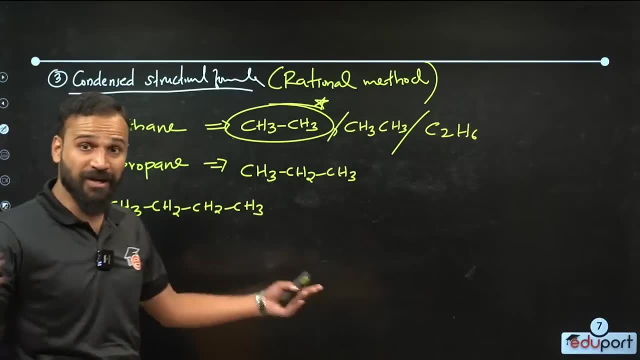 This is the usual condensed. How do we represent butane children? CH3CH2CH2CH3.. Similarly, pentane, hexane and heptane can be represented. Now, children, look, Look, A question is coming. 2-methyl 2-methyl propane. 2-methyl propane is represented like this: 2-methyl propane. What is propane? 3 carbon atoms: What is 2-methyl propane? There is a methyl loop in the second carbon. 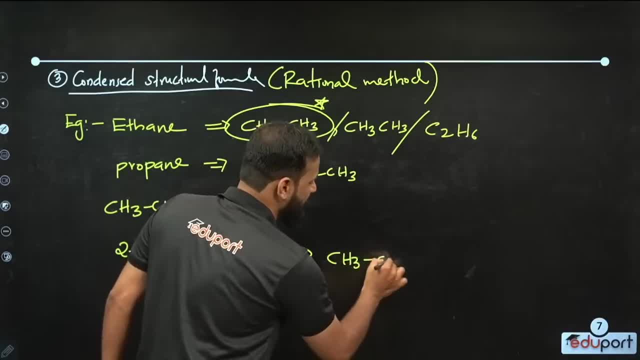 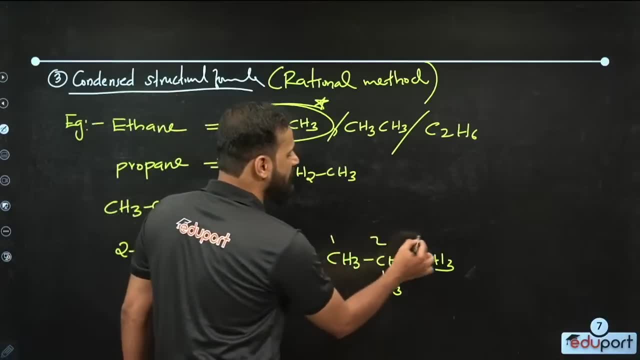 So how do we represent it? as condensed children? CH3CH, CH3CH3.. Isn't this the condensed formula? Look here: 1, 2, 3.. Methyl is in the second position. 3, carbon propane in the longest. 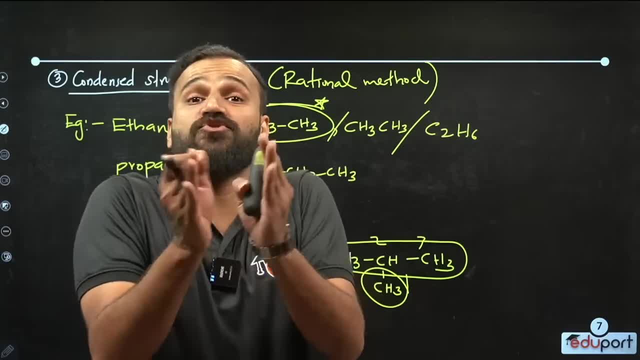 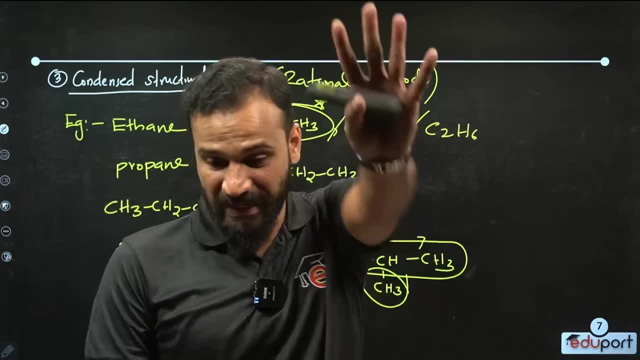 So 2-methyl propane. This is how it is written. It is called the condensed or rational method. Children, can't you write, Can't you write the condensed or rational method? You have to write, You have to write with me. 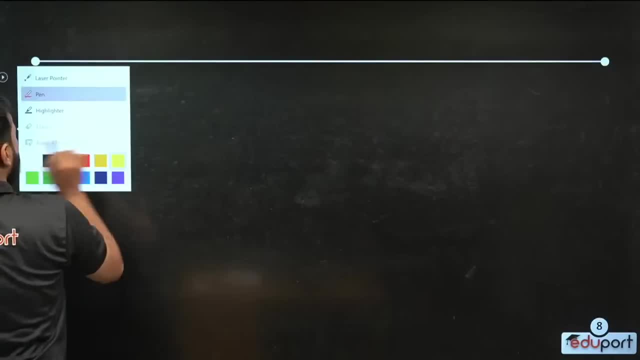 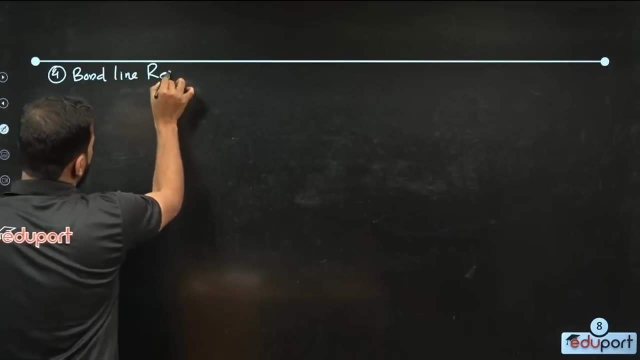 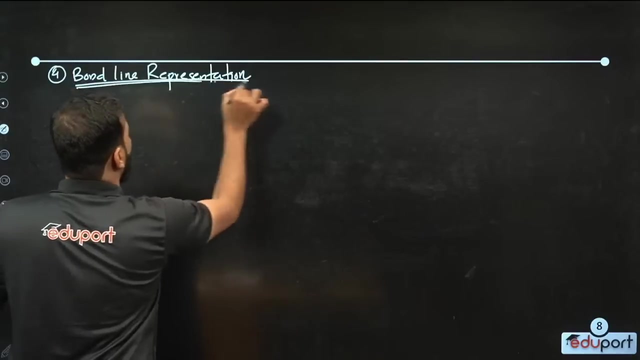 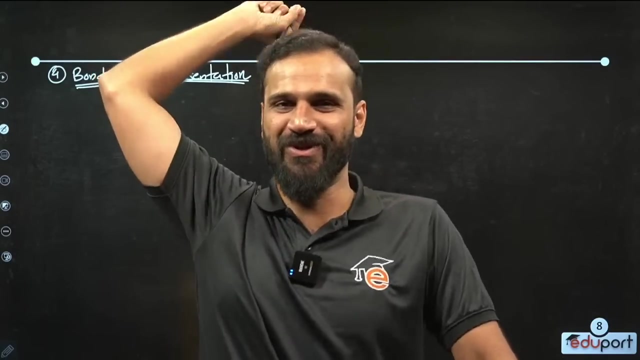 You have to write Yes. Now look children, Which is the fourth. The fourth is very important. That is bond line representation. Bond line representation, Children- it is a question asked many times. The specialty of bond line representation is the question asked many times. 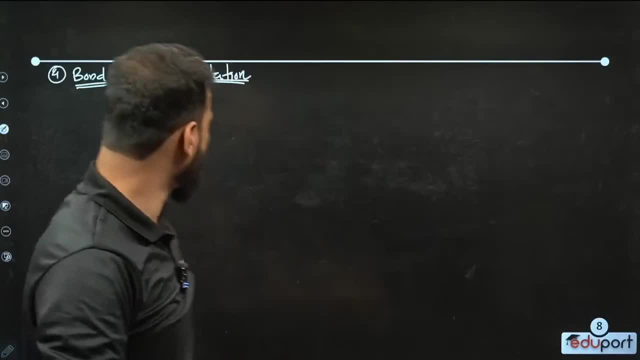 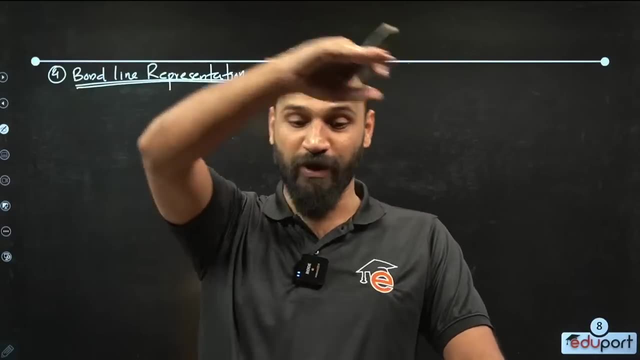 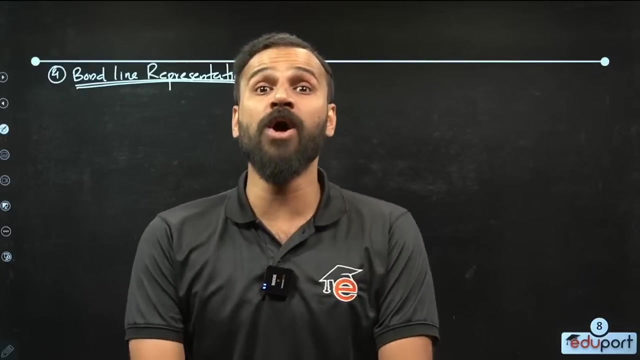 Don't miss it for any reason. Listen, study it. well, What is that bond line? Nothing In our carbon chain. which carbon chain? The carbon chain called CH3CH2CH2.. The bond line representation is represented by using a zigzag line for it. 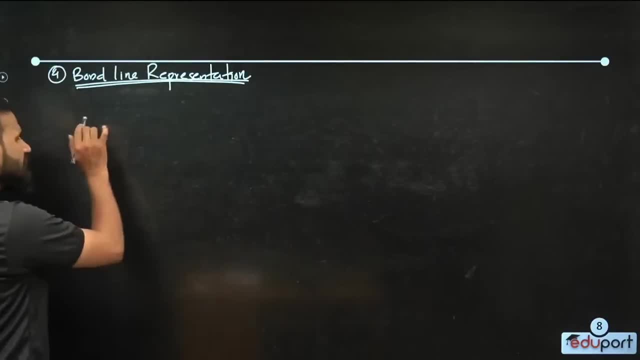 So, children, do you know what you have to understand? Do you know what you have to understand? We can start with ethyl. We can start with ethyl. What do you have to do with ethyl? Isn't there two carbonates in ethyl? 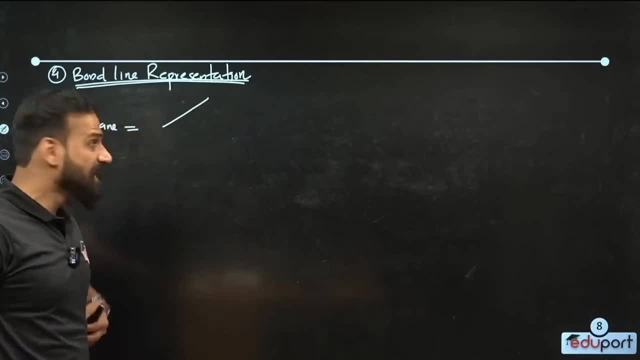 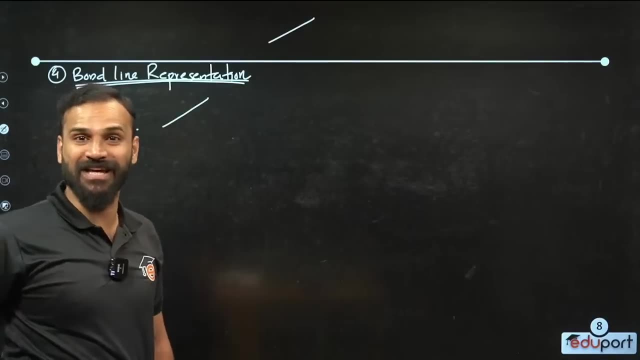 There, you just have to draw a line like this: This is ethyl. Do you know why? Because, according to the bond line representation, if you draw a line, do you know what it means? There is a carbon in those two ends. 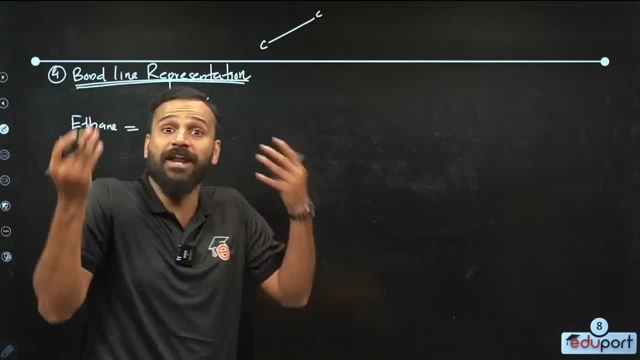 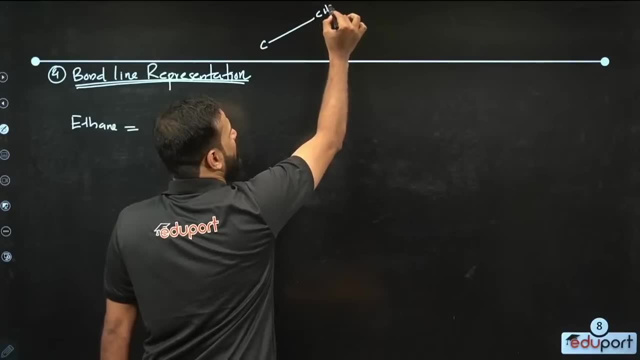 Not only carbon. How much hydrogen is required for them to become stable? That is also there. Look here Three: hydrogen is also needed. CH3. Here three are also needed: CH3.. So CH3 is single bond, CH3 is ethyl. 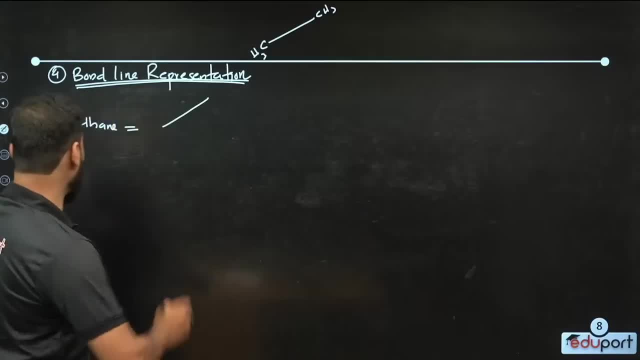 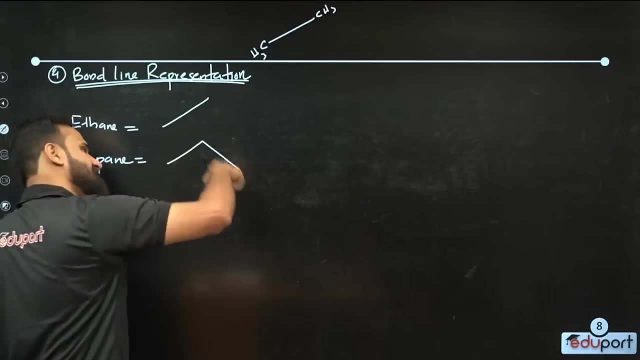 What is the purpose of this line? Now, children, do you need propane after ethane? If so, you draw a line down and draw it zigzag like that. Now do you need butane? Do you need butane? Draw a line again. 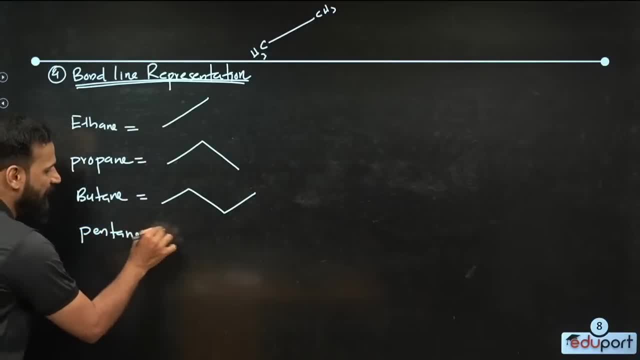 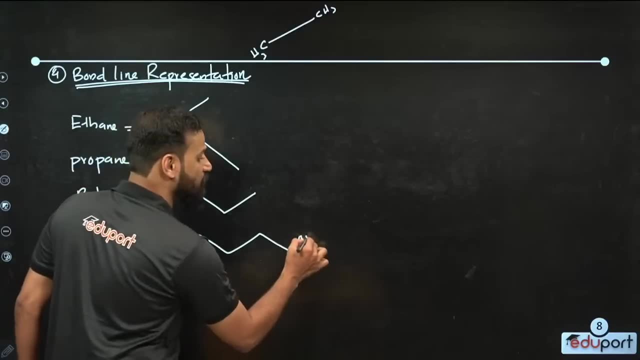 Now, do you need pentane? Do you need pentane? Draw a line again Down to the bottom. M is the pentane. Now one person has turned it. One person has turned it and put W. It is also the same. Usually we start the line from the bottom. 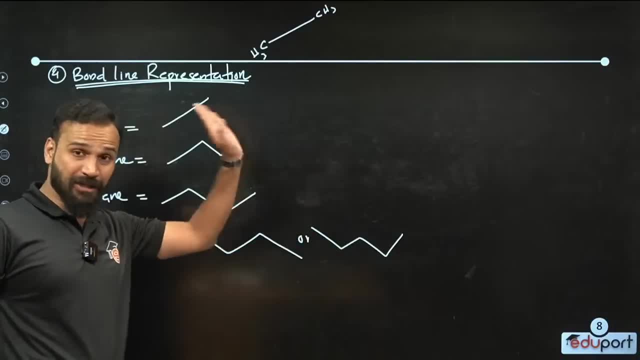 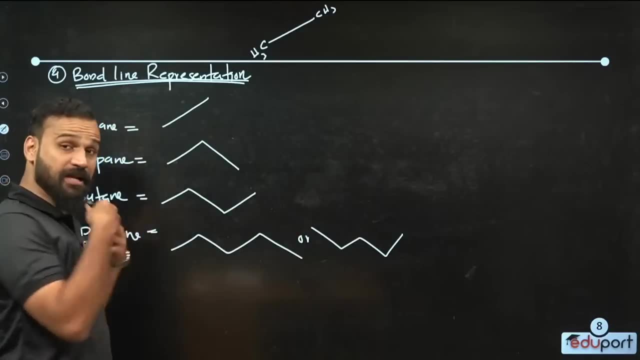 If a person starts from the top, it is not possible to say that it is not pentane, Because there are five or six, it is pentane itself. But when we draw, it is drawn like this: Yes, look, now you will draw pentane, hexane and heptane. 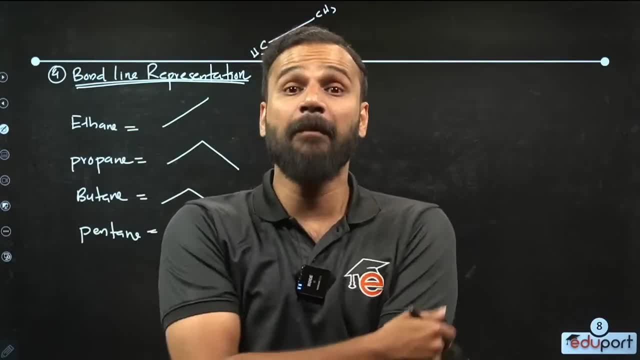 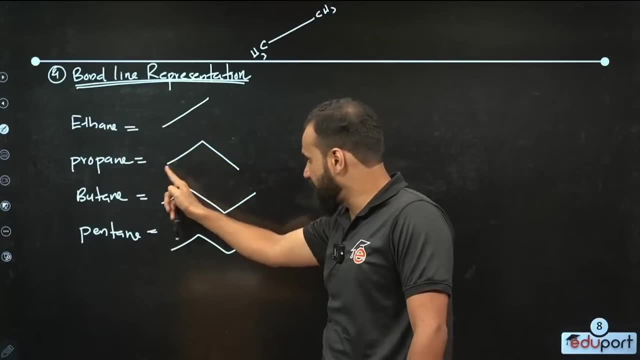 Just draw a zigzag line like this. But there is one thing, when children say this: Look, this CS3 single bond is not like this. It is drawn like this in CS3, CS2, CS3.. It is drawn like this in CS3, CS2, CS2, CS3.. 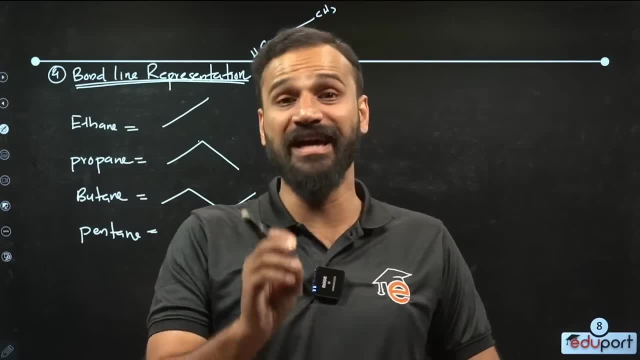 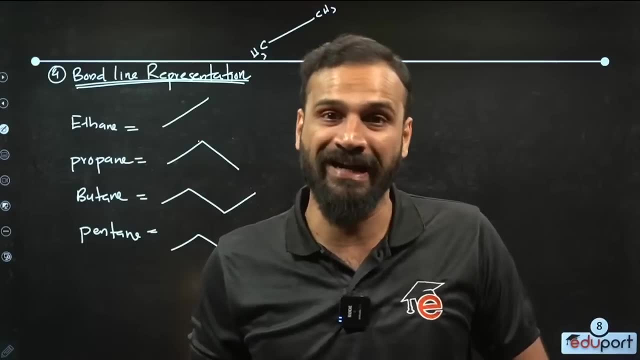 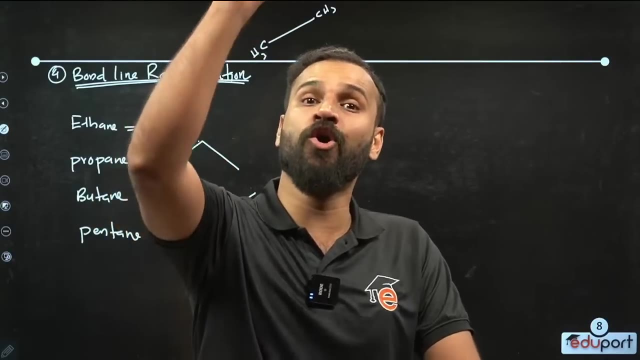 So we do not represent carbon and hydrogen there, Or we do not represent carbon and hydrogen in the parent chain. We have to understand that it is there Now if any functional group comes there or if double bond or triple bond comes there. 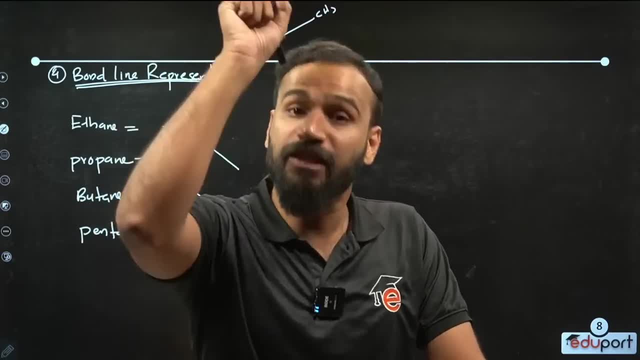 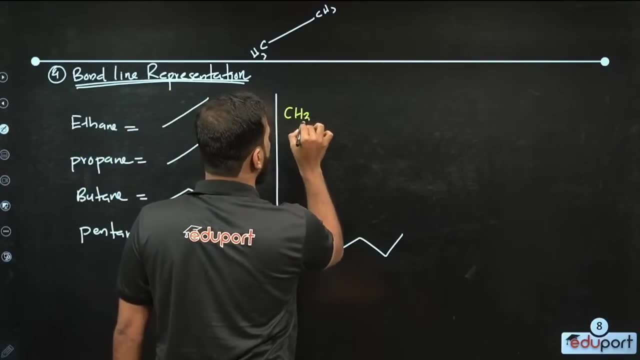 we have to represent it accurately. It is very important. Look when I say the example, you will understand. Look, children, when I say the example, you will understand. The compound given to you is CH3, CHOH CH3.. 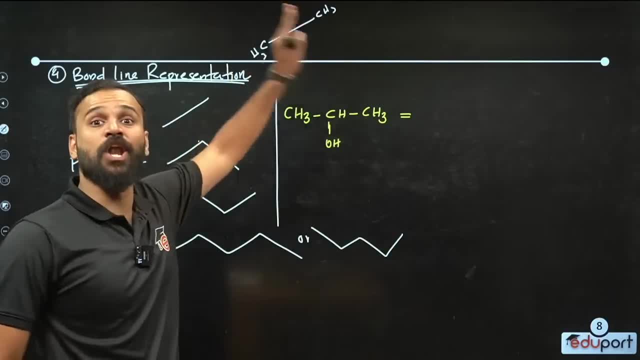 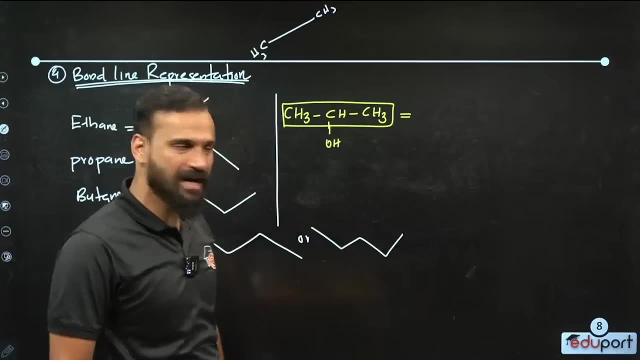 How to represent this, children. Look, first take the longest chain. Isn't this the longest chain, children, In that longest chain there are three carbons, right, It is propane, right? So how to draw propane? how to draw? 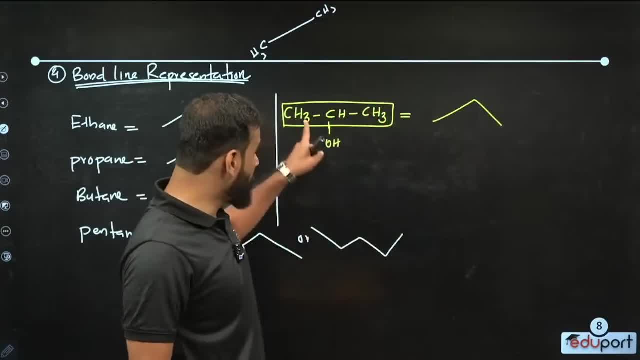 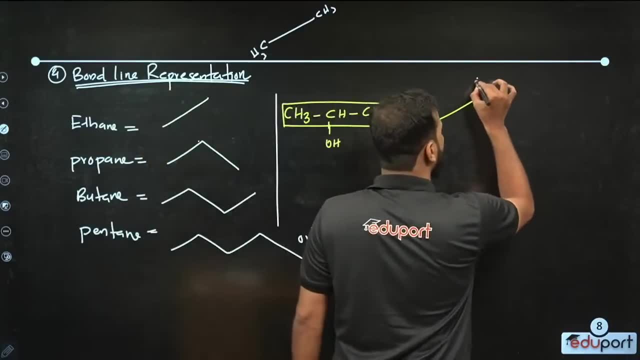 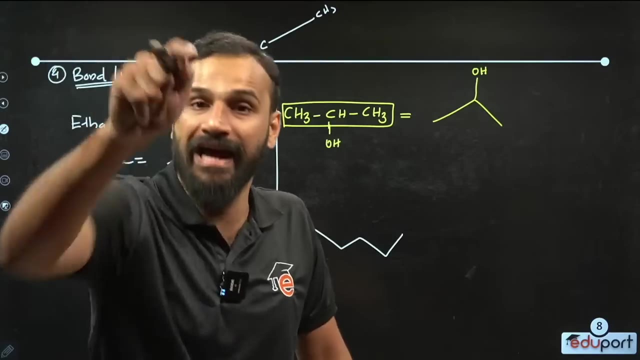 So you have to draw propane Now. the second in propane, in the second carbon atom hydrogen is replaced by OH. right, That OH is a functional group. It has to be written there as OH completely. That is the difference between bond line representation. 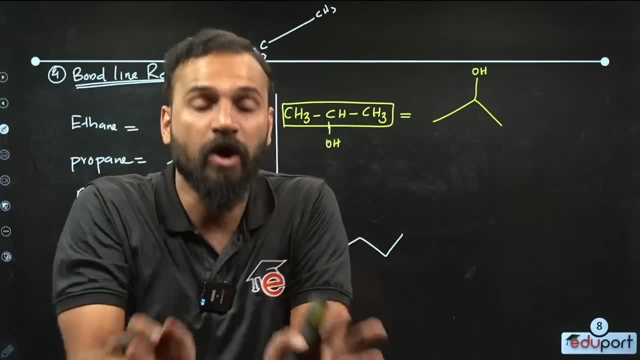 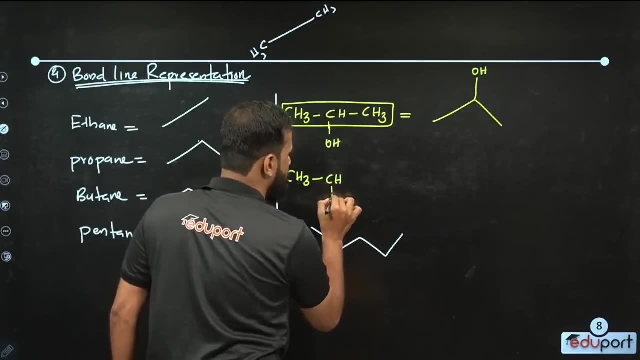 Functional group can only be represented completely. That is very important. Double bond has to be represented. Look, children. another example. Another example: CH3, CHCl, CH, double bond, CH2.. If given like this. if given like this: 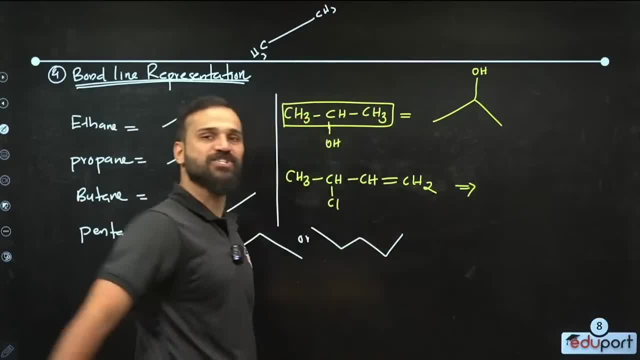 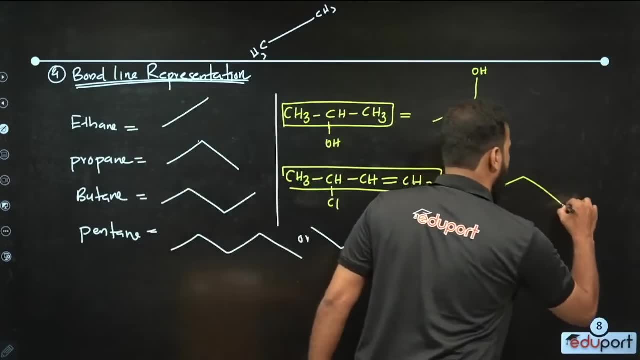 here also, you take the longest chain. Isn't this, children, the chain? How many carbons? One, two, three, four. If it is four, we can draw N like this: That's enough. In the second carbon atom, it is Cl. 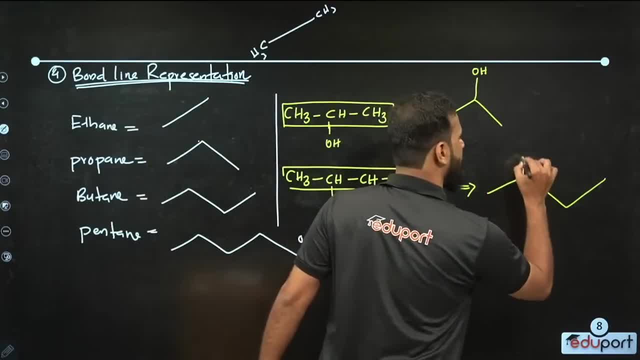 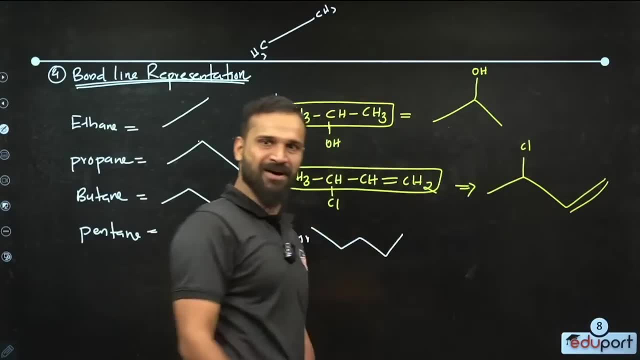 It is a functional group, It has to be represented like that. What is the difference between the three and the four? This is double bond. It is necessary to show there. If double or triple comes, it has to be shown there. Look, children, look. 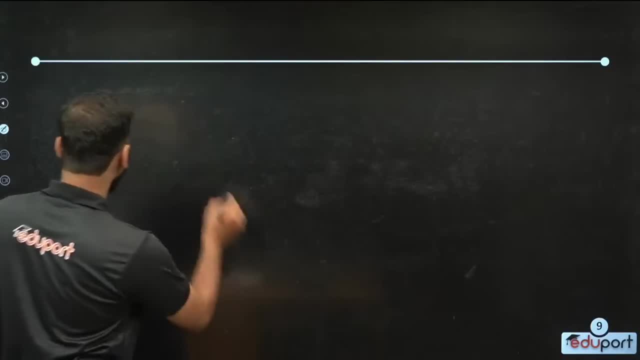 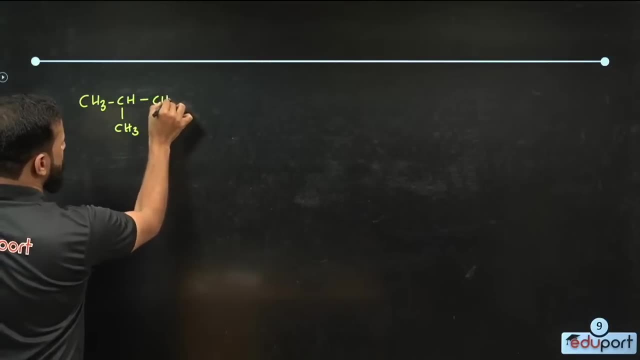 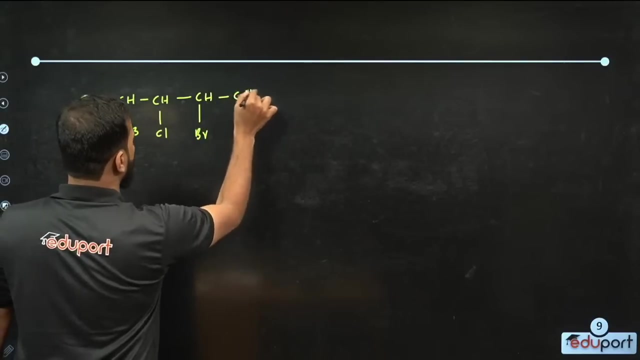 Look at the other question: CH3, CH, CH3, CH, Cl, CH. what is it? Br? CH3.. Think that it came like this: Look, this is the longest chain. How many carbons? Five. 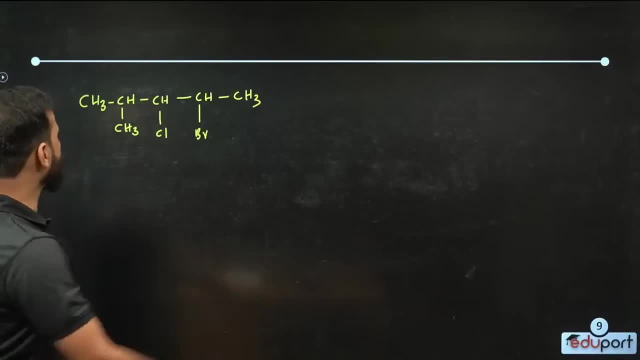 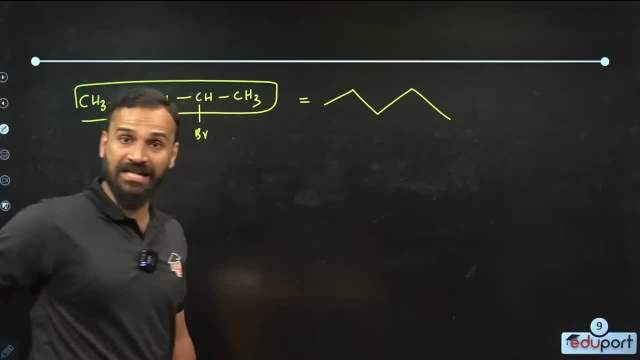 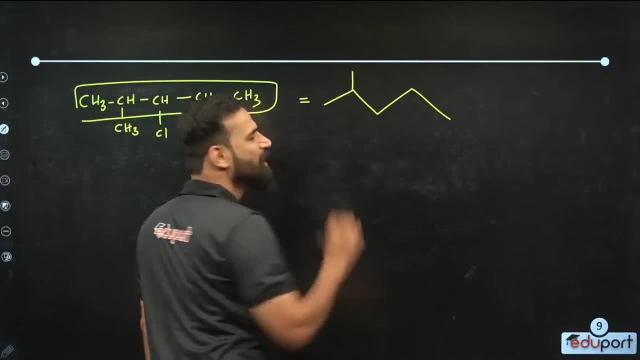 Yes, one, two, three, four, five. These are five. One, two, three, four, five. Look, it's CH3 in two right. See, CH3 is not a functional group, but it is a branch right. 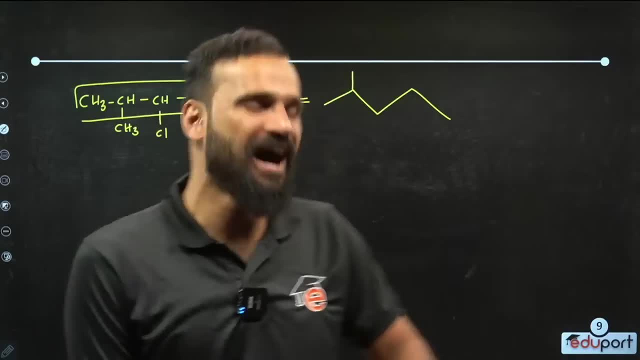 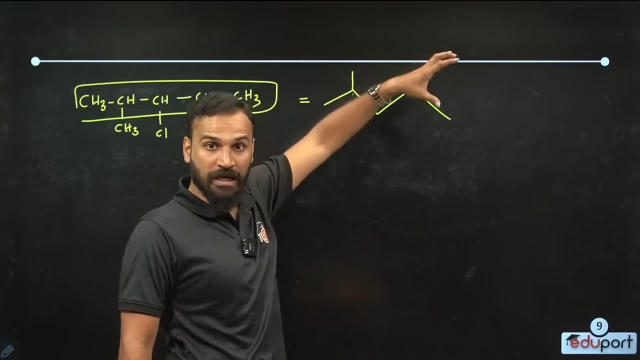 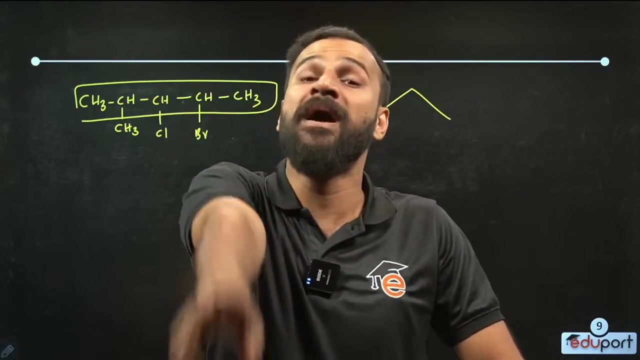 We don't represent either carbon nor hydrogen. No, So do you know what you should understand When you essentially, after deriving a line there, if there is carbon at that end and that carbon is necessary to be stable, means that there is three hydrogen there. There is CH3. 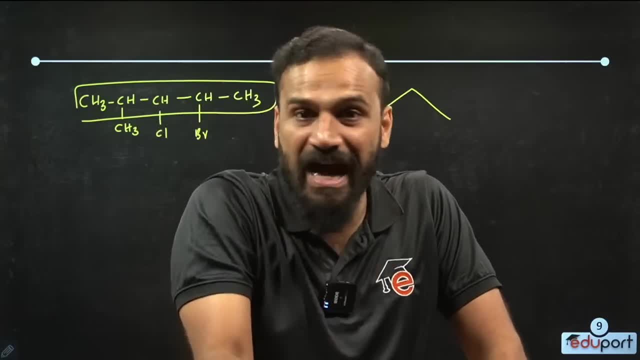 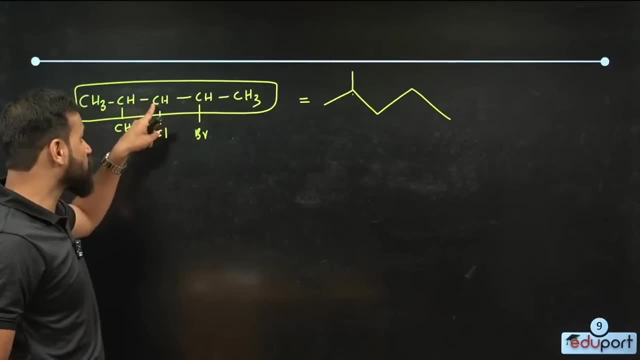 means It's not something you have to represent. It means that there is a methyl group there. if you draw a line Now, look at the second, sorry, the third carbon is Cl. right, It's not a branch, it's a functional group. 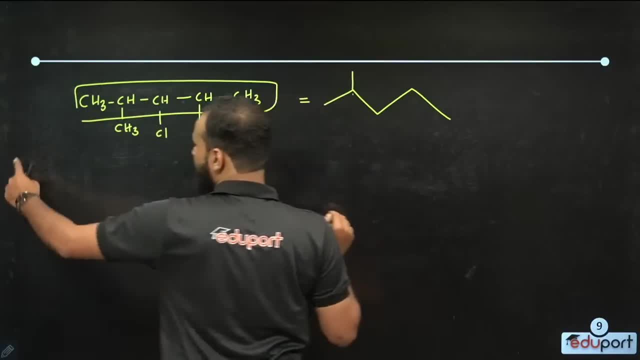 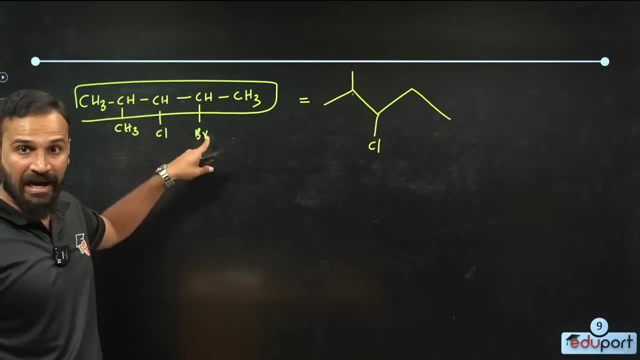 That's how it should be written there as Cl. That's how it should be written, guys. That's how it should be written there as Cl. See, in the fourth carbon BR. it's a functional group. it should be represented there. look, BR should. 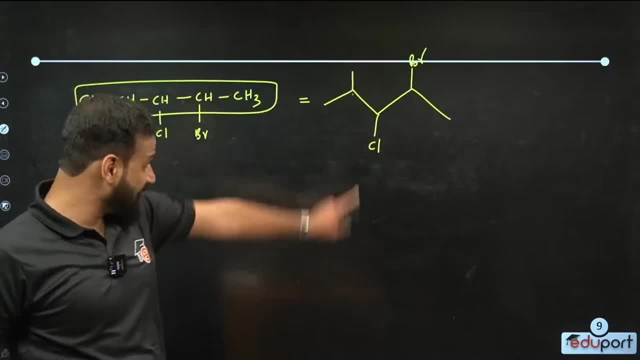 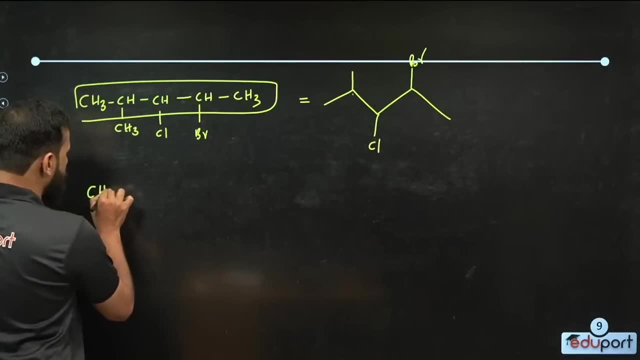 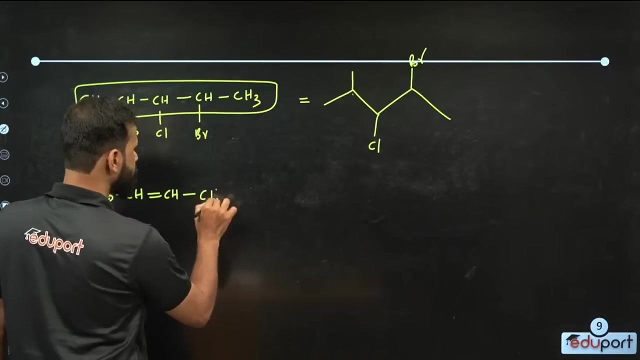 be represented. That's how it should be written. Do you understand this? This is very important, Very important. Look, here's the other question: CH3, CH double bond. CH single bond- CH2OOH- How does it look like? How does it come? How many? 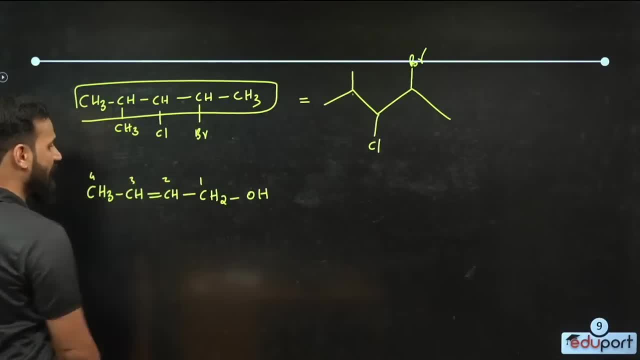 carbons: One, two, three, four, five, six, seven, two, three, four, Four carbons: right, If there are four carbons, we will draw like this right. children, We draw like this right. Yes, In that. 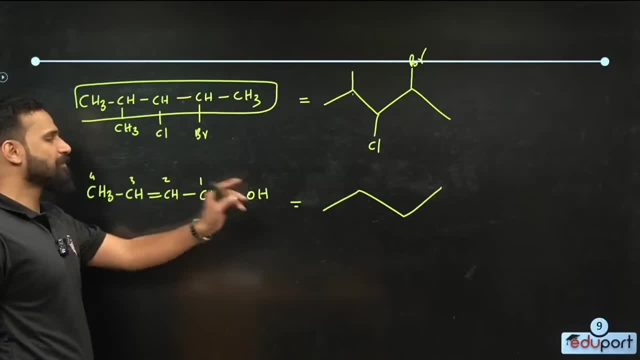 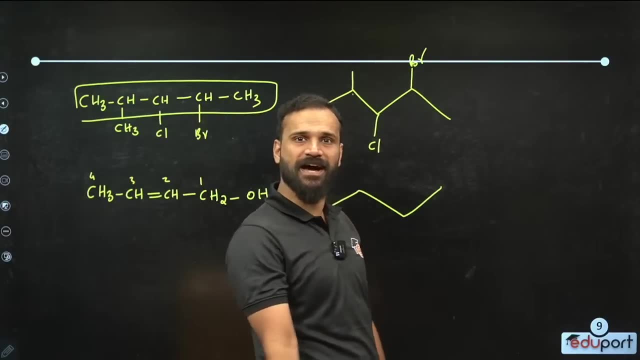 the first. if it is from there to there, there is OH in the first carbon. So here this is carbon, That is, this is the first carbon. OH is in that carbon. How do you represent it? You can write OH here. 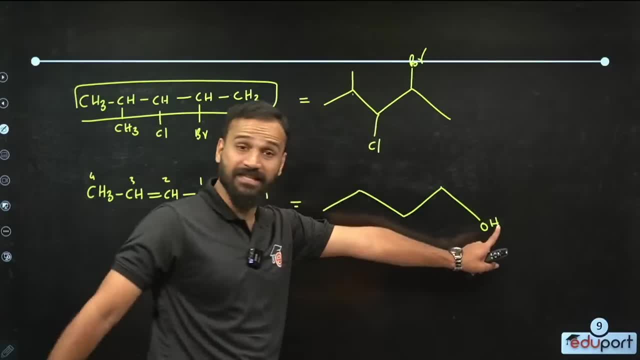 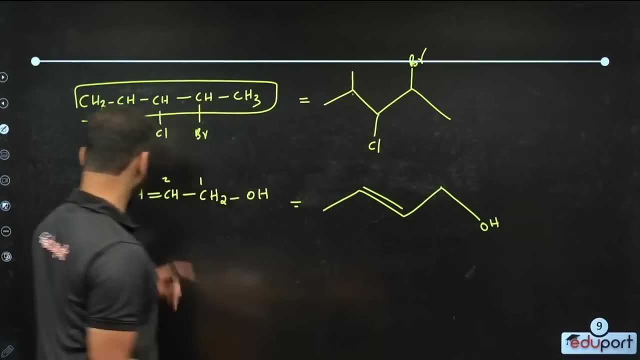 by putting a zigzag line. What can be written here? OH can be written After that, between two and three. what is there between two and three? There is a double bond. I showed it there. That's all, So how to represent it. 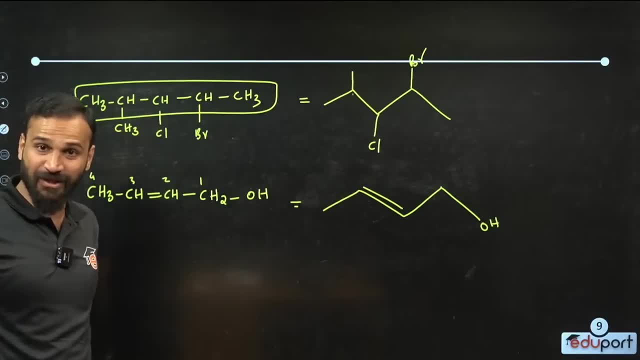 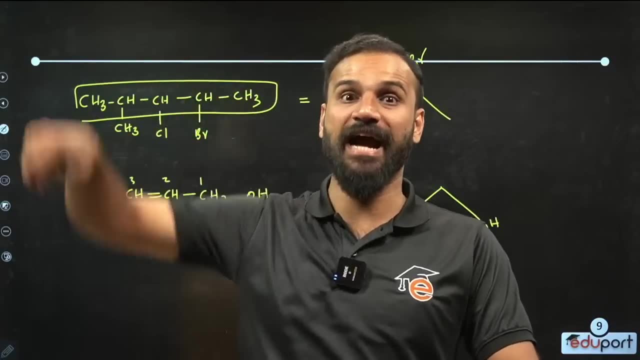 How to represent it. Do you understand what I am saying? Very simple. This is how the bond line representation is represented. The carbon chain is represented by zigzagging The carbon chain. Now let's look at another question. Let's look at another question. 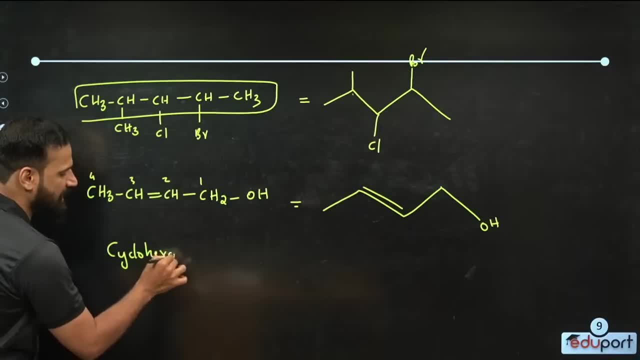 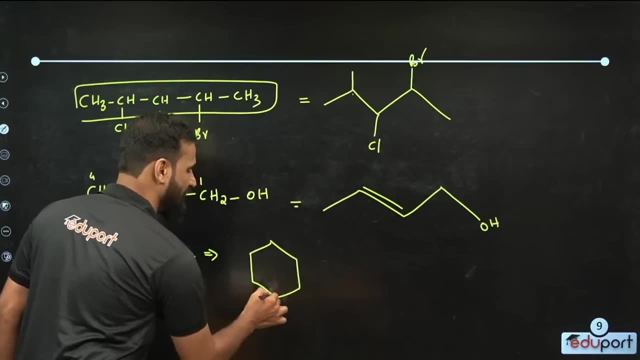 Cyclohexane, Let's Cyclohexane. How does Cyclohexane run the bond line representation Cyclohexane For whom? For those who don't know, this thing is also Cyclohexane, That is, CH2, CH2, CH2, CH2,. 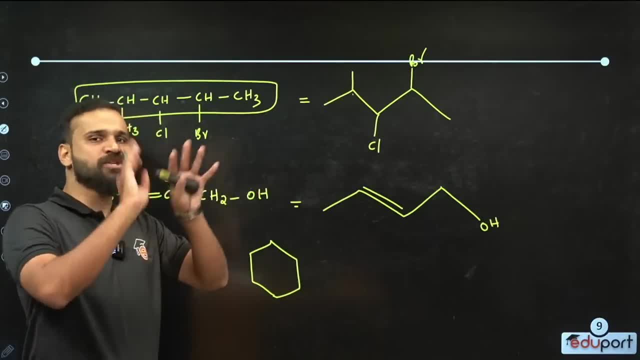 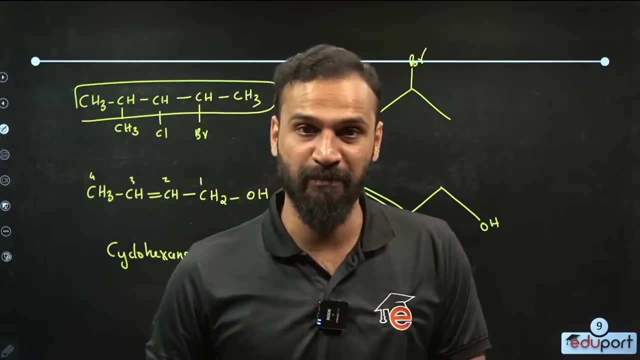 it comes cyclically, isn't it Cyclohexane? So carbon and iron should not be represented. So this is Cyclohexane. This is the bond line representation of Cyclohexane. You have to understand, Okay, children. 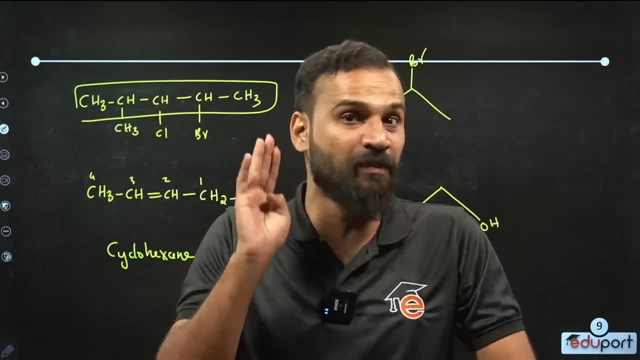 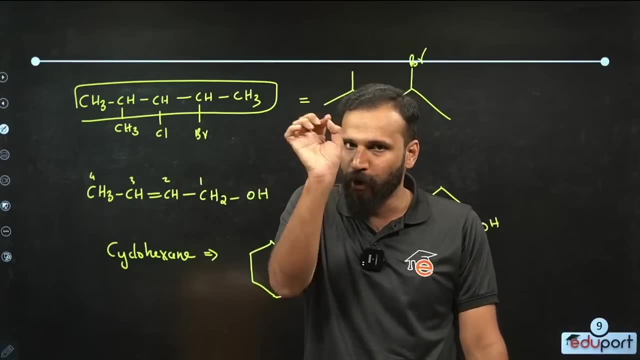 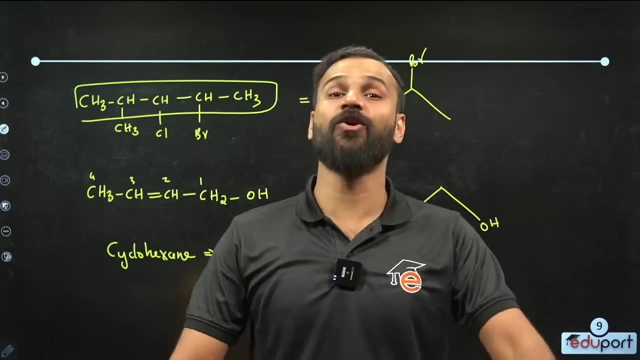 How is the bond line representation? We said four representations, What are all four? One is Lewis representation, Not one. But if one pair of electrons is given, it becomes a bond line or, sorry, Lewis representation or electron dot formula. Secondly, what is that? 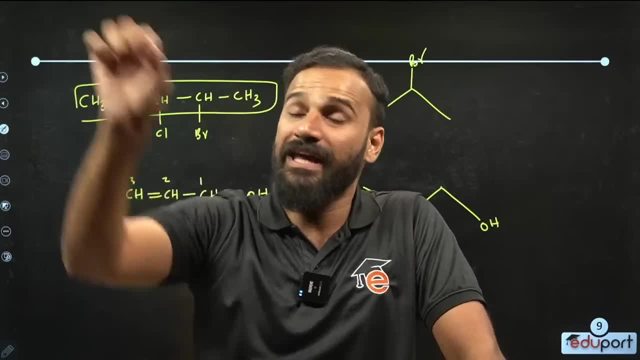 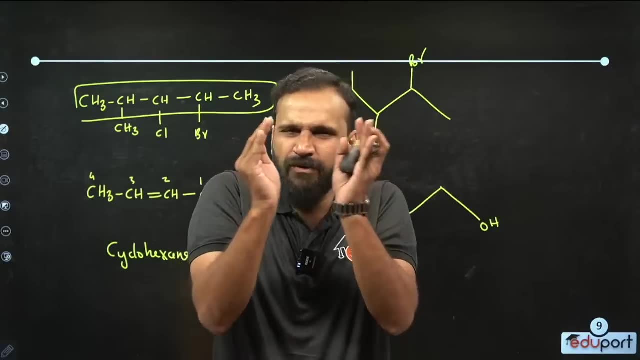 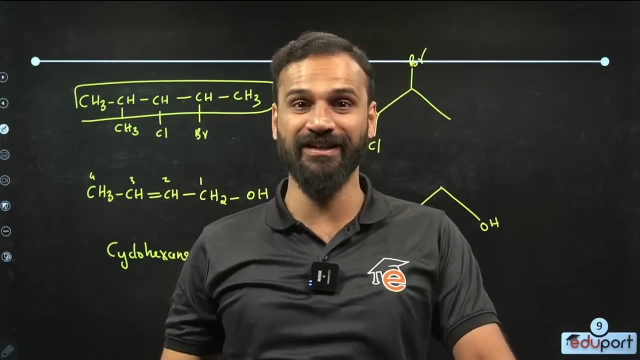 Complete structural formula or complete formula If all atoms and all bonds are represented. complete, What is condensed, or rational. At the very least, it should not be shortened. What is the bond line? The carbon chain that was discussed last, using a zigzag line to represent. 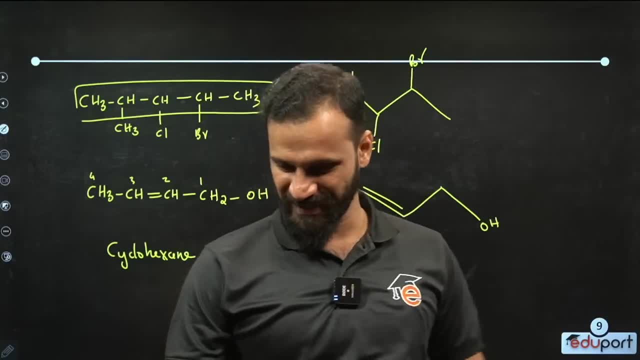 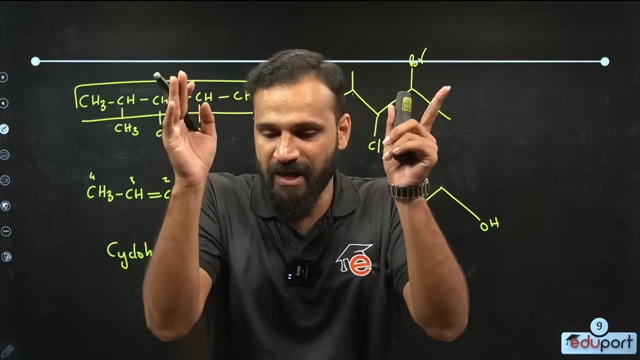 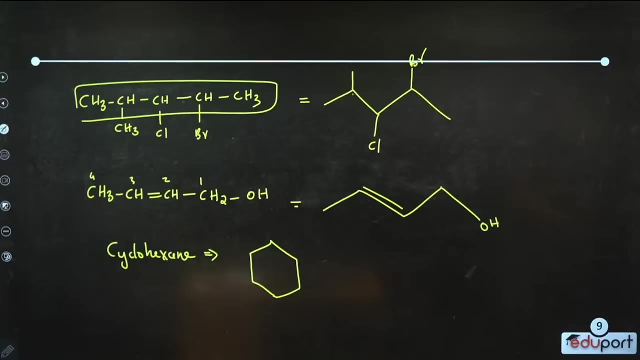 the bond line representation. Okay, it is very important, Very important. Okay, children, If all these four representations are okay, say it quickly. If all these four are okay, say it quickly, Because this is a very basic thing. Let me see the next one. 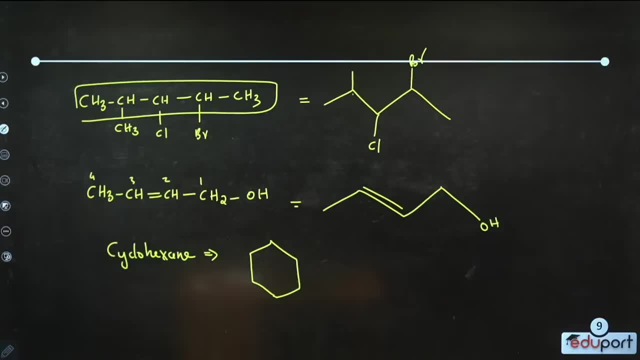 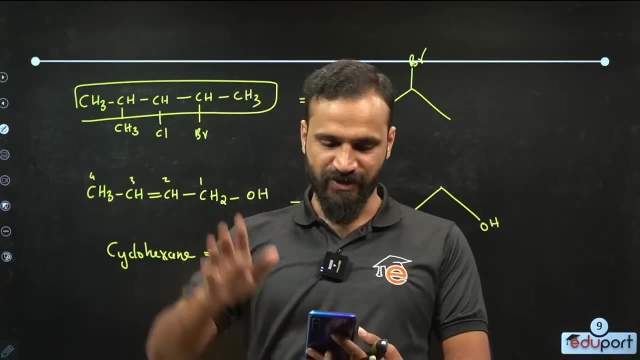 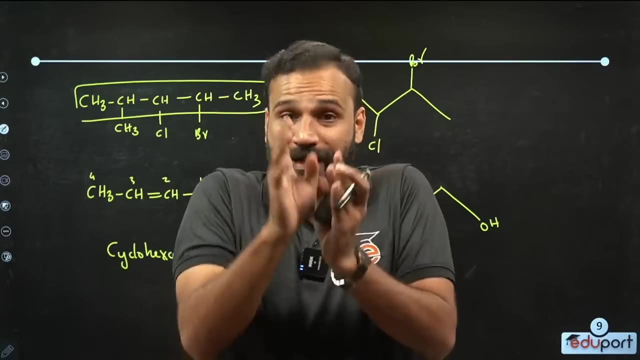 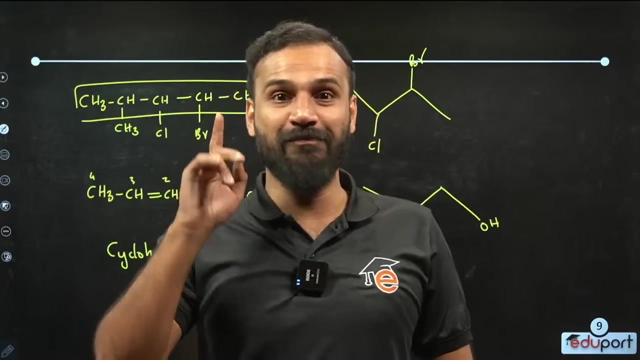 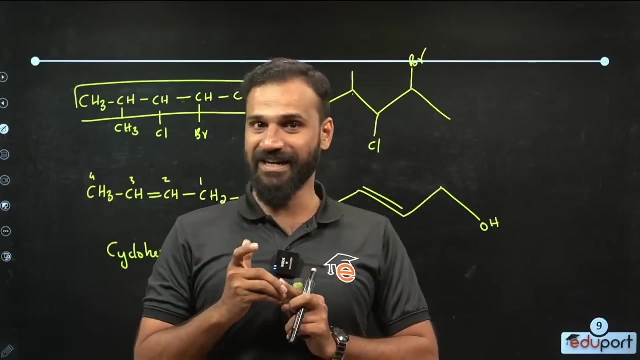 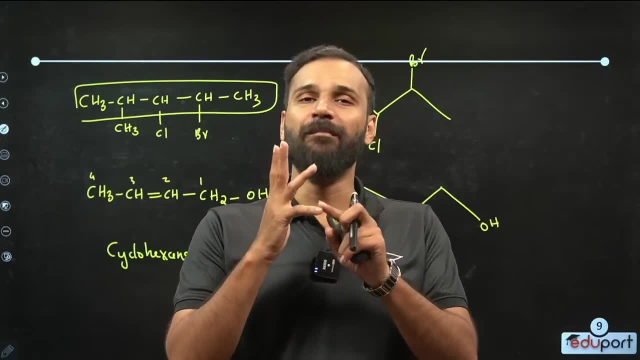 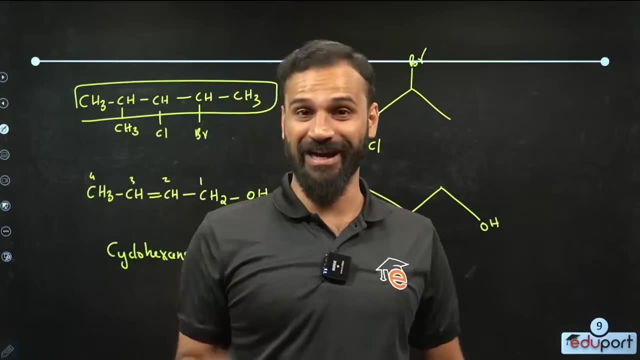 How can we represent them? There is Lewis representation, complete structural formula as well as condenser formula in the bond. Did you learn? well? Now there is one more method. There is no need to ask for an exam. but let me tell you. 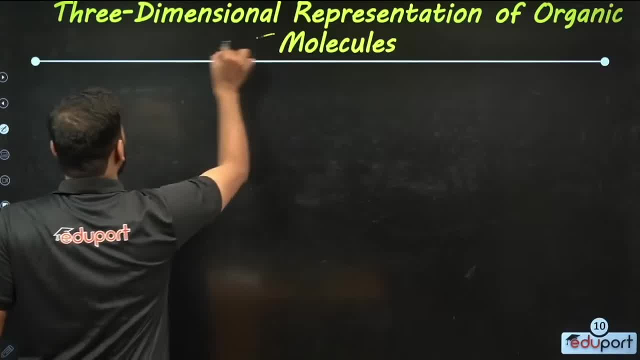 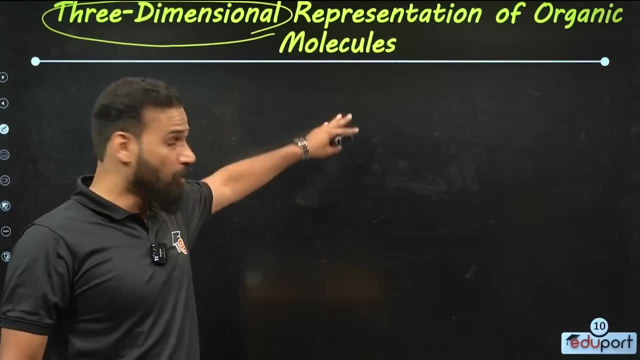 to know that it is a three-dimensional representation. What is it, children? Three-dimensional? Only one example is said. there is no need to ask. The question is: if we have already studied the four representations, will come to the question. Look, I have taken you as an example. 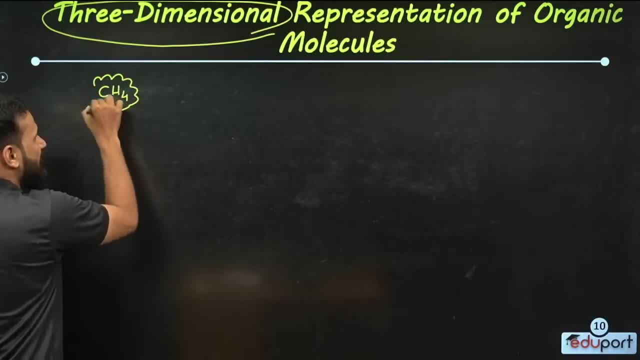 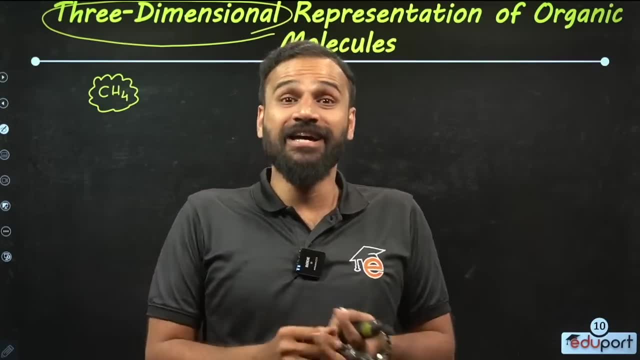 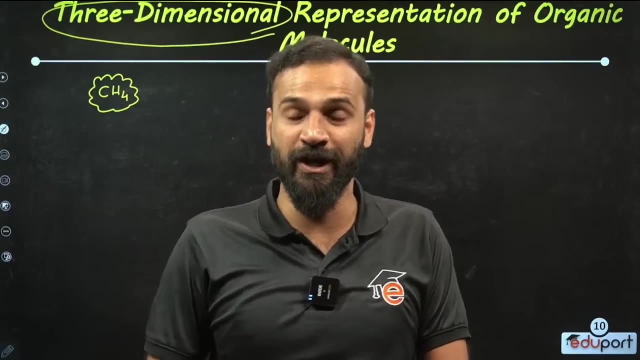 CH4.. What children have you taken as an example? CH4 methane taken as an example. Already chemical bonding has been done. If you have taken it as an example, you have learned that its hybridization is sp3.. The bond angle of this has been learned to be 109 degrees. 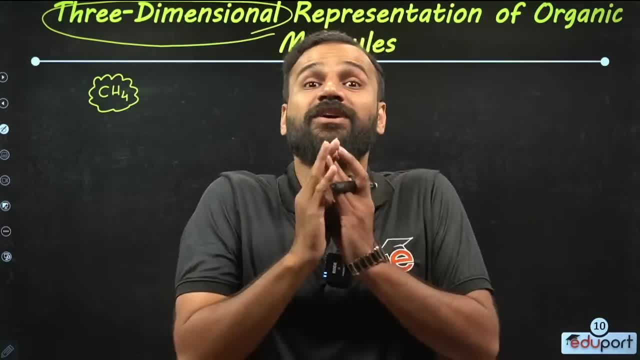 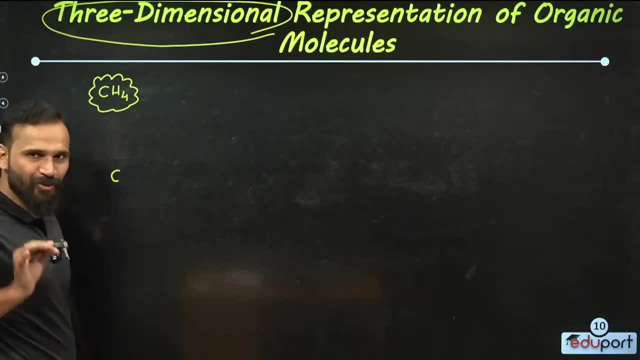 28 minutes. The geometry or shape of this has been learned to be tetrahedral. These are very basic things that you know. If so, look at the shape of it. One carbon is okay. There are four bonds around it. I drew two bonds in it. Look, how did I draw these two bonds. 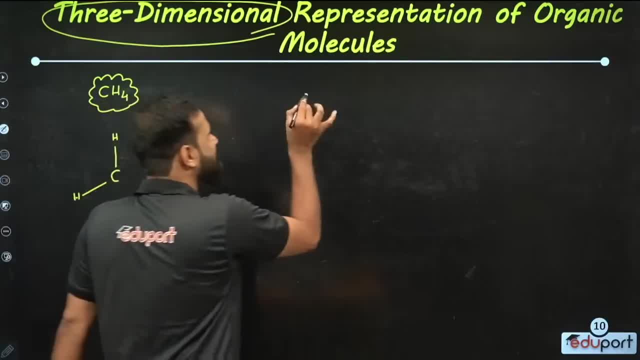 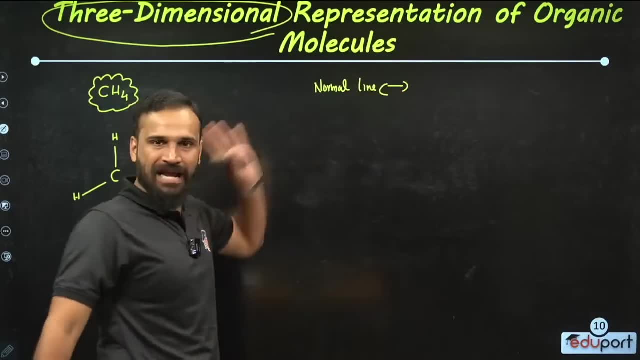 I drew it using a normal line. That's what you have to pay attention to. What did you use to draw A normal line? That's what this thing is. Didn't you use this to draw Children? do you know the meaning of that normal line? 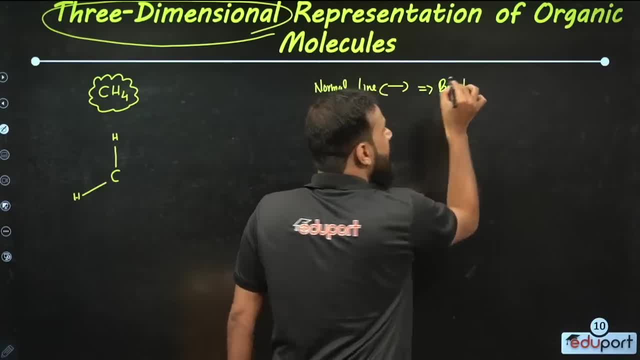 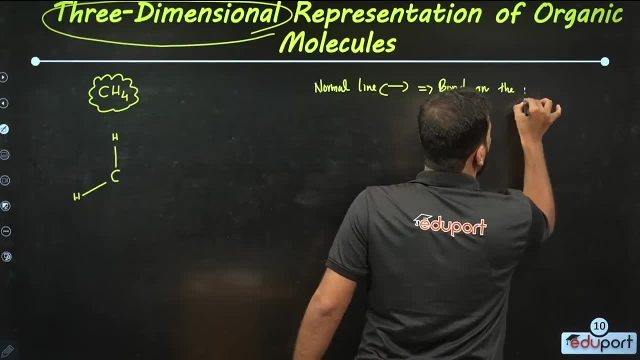 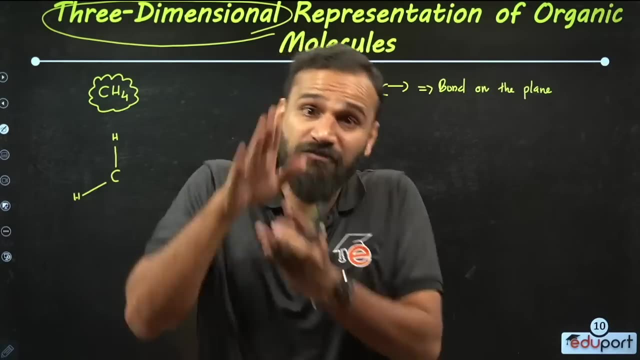 It is a bond. What is that? It is a bond. Where is that bond On the plane? The one with that bond is on the plane: Children. where is that bond? Where is that bond On the plane? What do you mean by plane? The surface? 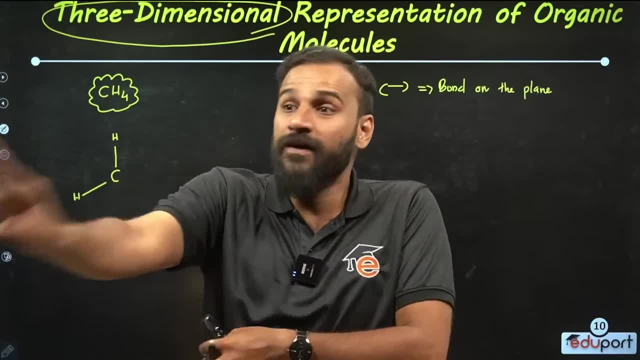 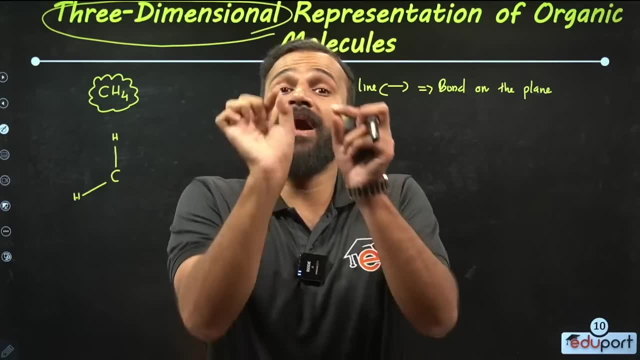 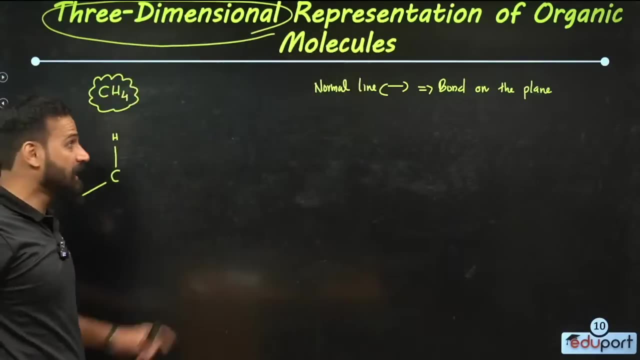 On which surface or on which plane do we represent that molecule? That bond is in that plane itself. That is the feature of representing a bond using a normal line. Now, children, only two of the four bonds are represented. How is the next bond? The next bond is represented. 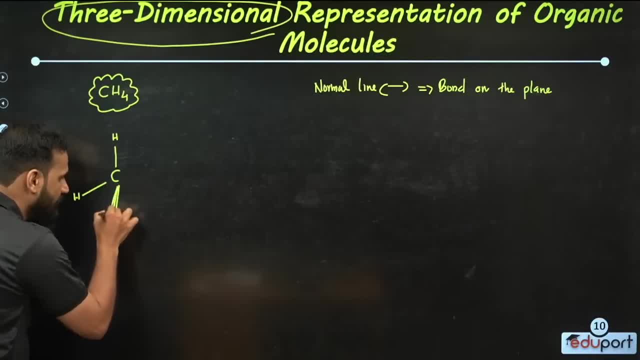 like this. Look at this. This is the next bond represented. What is this? This is a bond, Children. what is this? This is a bond. There is an edge here, Do you understand? So look, do you know what to say about that? 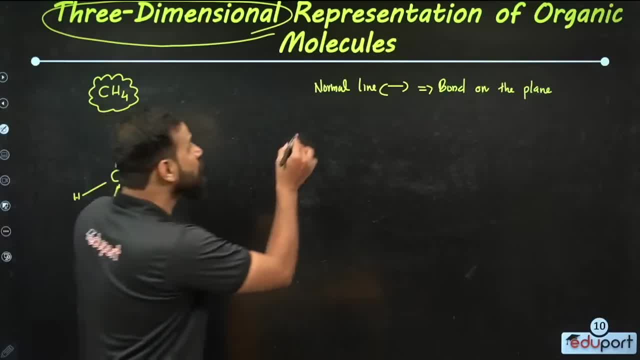 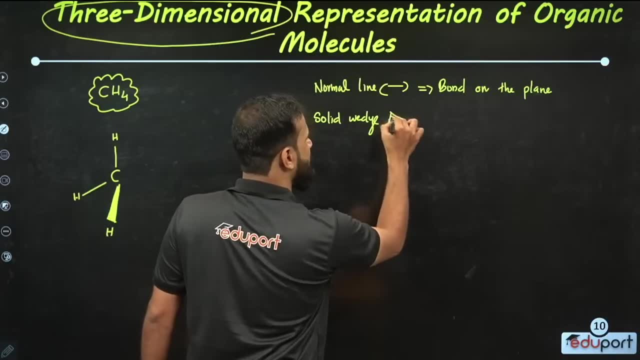 Do you know what to say about that? This is called a wedge. What is this wedge? This is a solid wedge. What is this, children? This is a solid wedge. How is this represented? This is how it is represented. Do you want to shade? 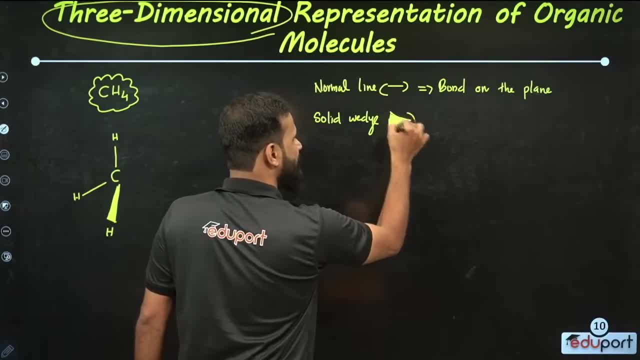 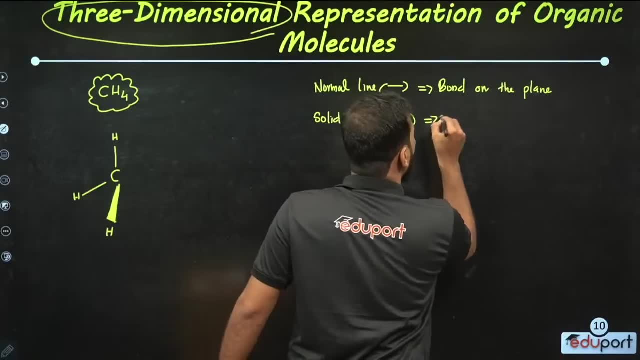 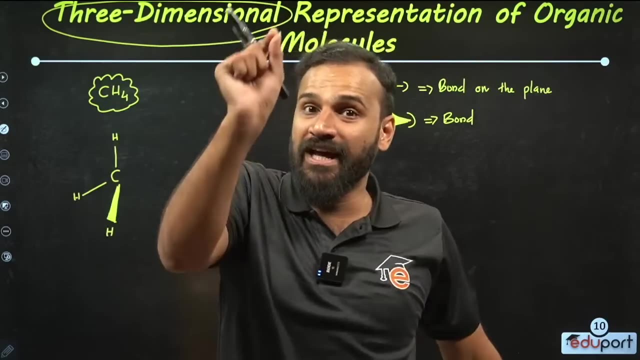 Do you want to shade? Shade in the form where the thickness is reduced. This is a solid wedge. What does that solid wedge mean? It also means a bond, But that bond is not in that plane. Where are you in this board that you drew CH4?? 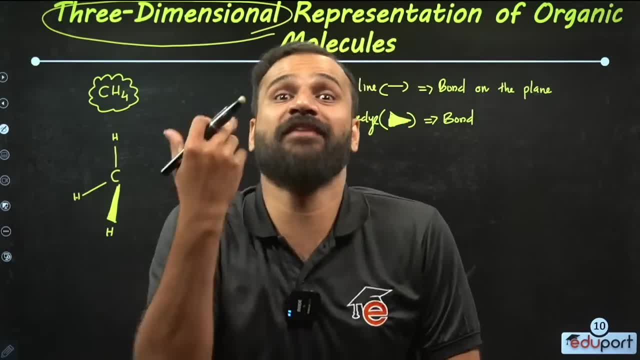 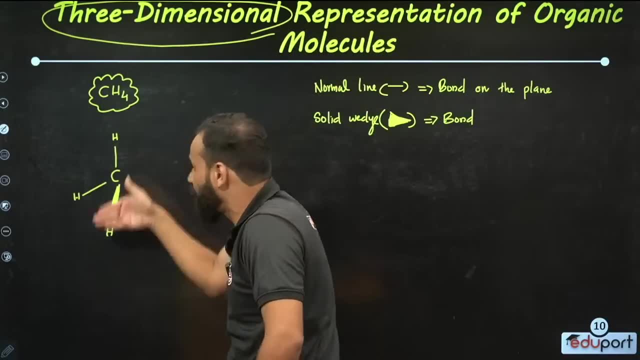 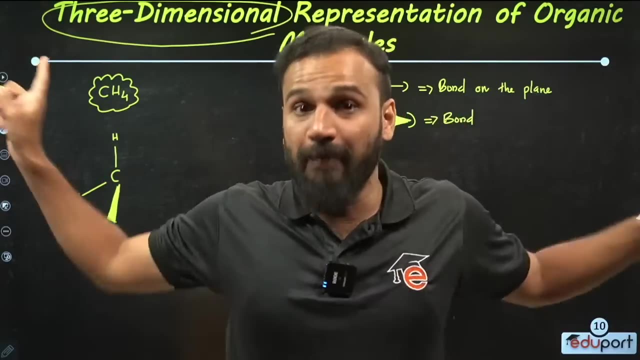 That bond is not in that board, Then where is that bond? That bond is towards the observer, When you look at this molecule from there. what are you doing next? directly, That bond is not in that board or plane. Children. where is that bond? 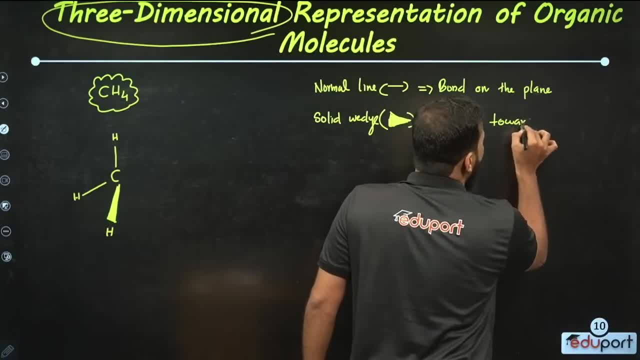 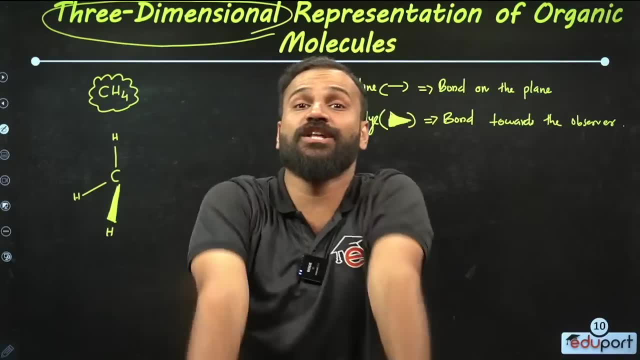 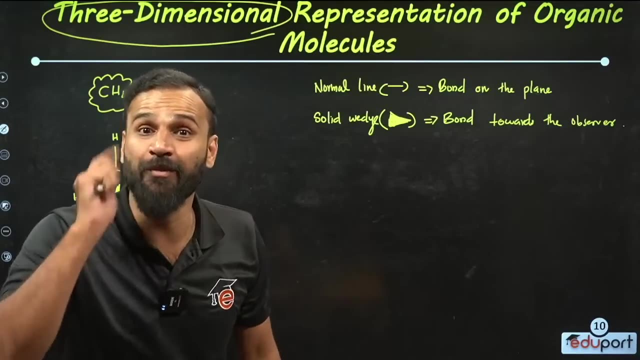 That bond is towards the observer. Who is looking? He is standing directly next to him. Understand that bond. Which bond? Solid wedge used to represent the bond. Isn't there another bond? Who is that? Look, look, look, look, look. 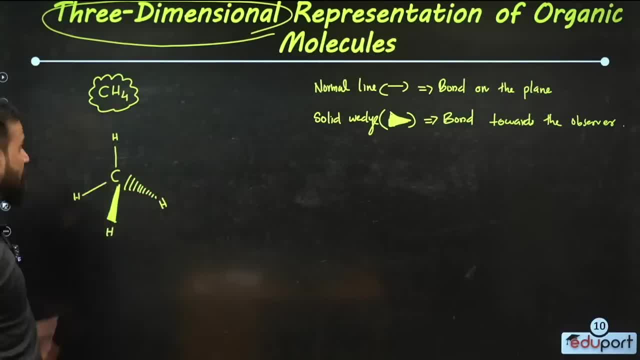 Look, this is the next bond. This is the next bond. Now there are four bonds. Look, what do you know about this bond? That is also a wedge. It is a wedge that decreases in thickness, But it is not a solid wedge. 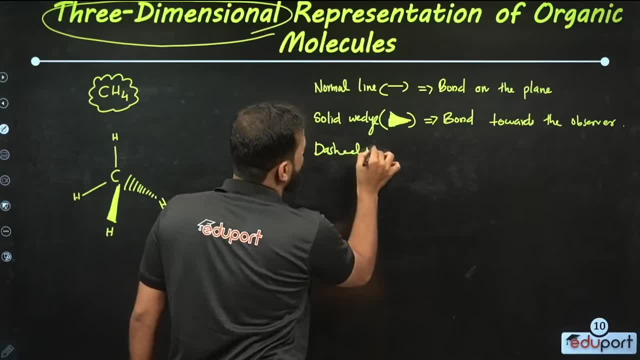 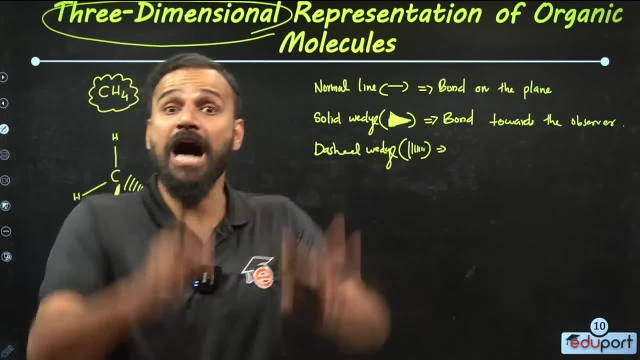 It is a dashed wedge. What is that, children? It is a dashed wedge. We represent the dashed wedge by using a line like this. Why does it indicate? It also indicates a bond. What is that, children? It also indicates a bond. 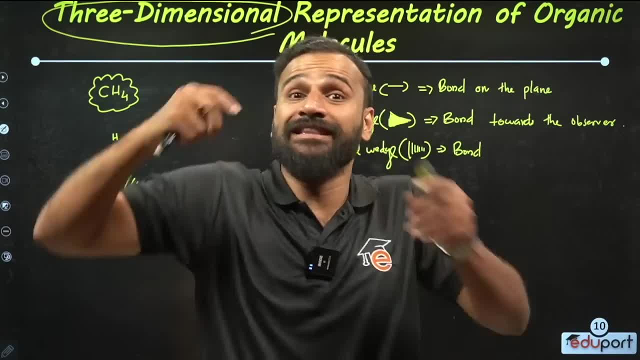 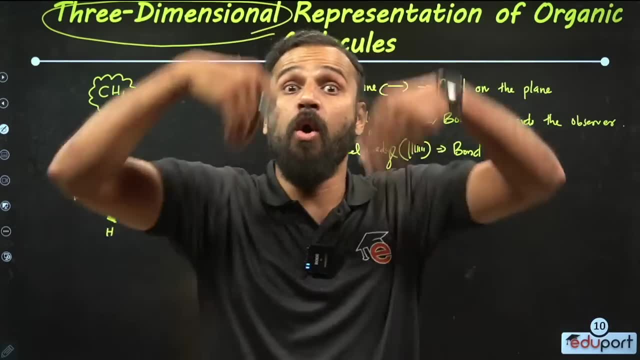 Which bond? It is not the bond next to you. It is the bond that directs you to the opposite side, to the back of this board. It is opposite to the observer Or it is away from the observer. So the bond is not towards. 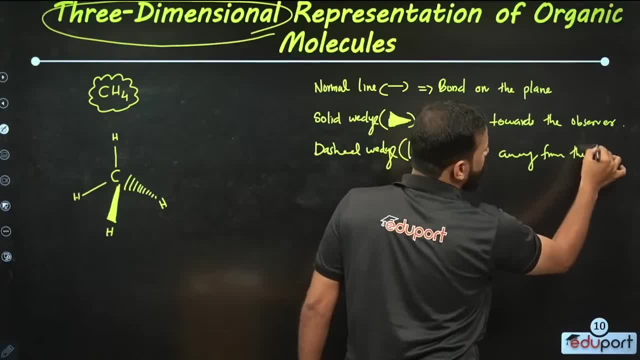 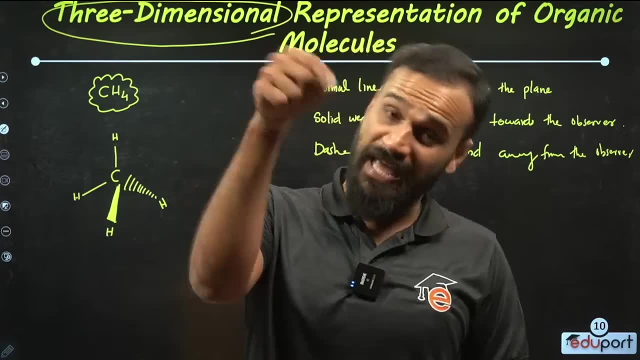 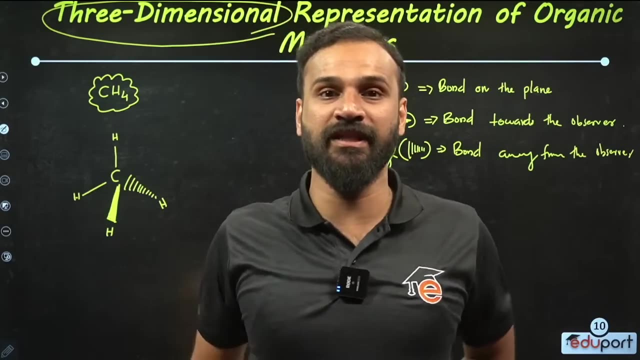 It is not towards, It is away from the observer. So, children, you have to understand. For one molecule, we can represent it in any way. It can be represented in three dimensions. If it is represented in three dimensions, we have to use three types of bonds. 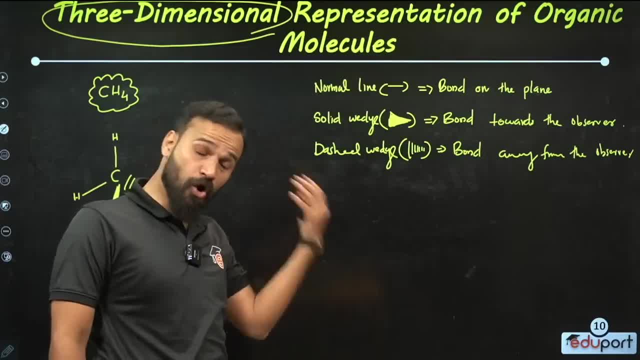 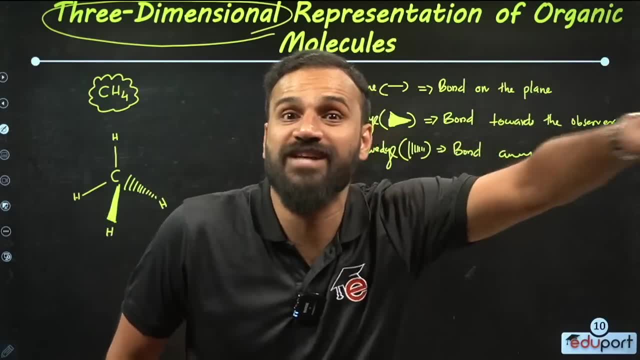 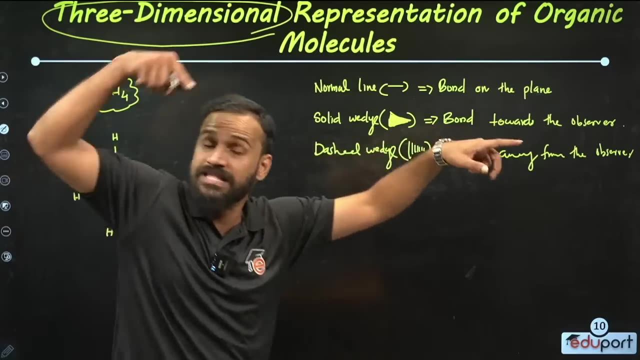 One is the bond that is represented by using a normal line. What is special about that bond? That bond is on the surface. It is on the plane, Children. where is the second bond? It is a solid wedge. That bond is towards the observer. 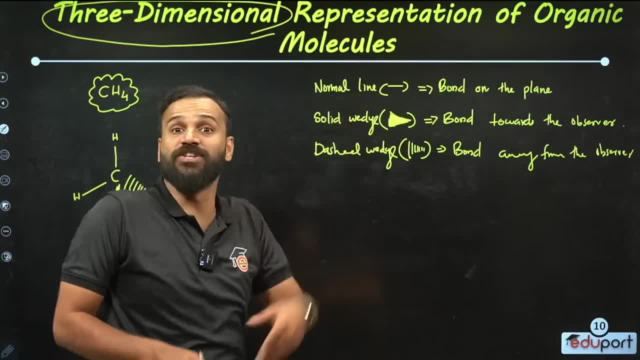 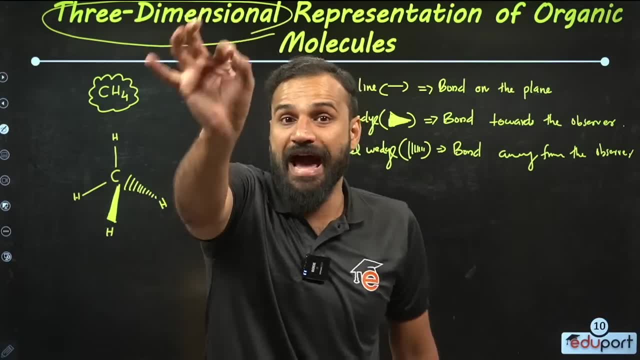 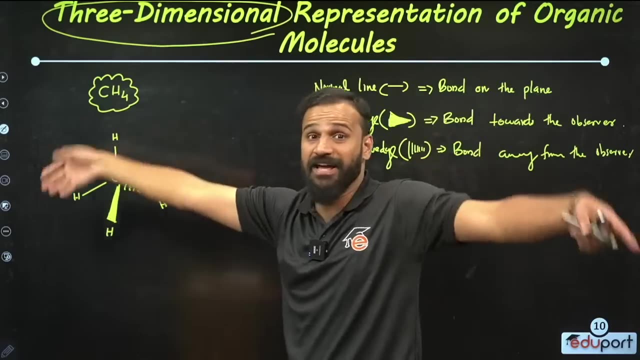 Children, what is the third bond? It is a dashed wedge. It is directed in the opposite direction of the observer. Children, did you understand how methane is represented in three dimensions? That is, where are these three or four bonds? Did you understand where it is directed? 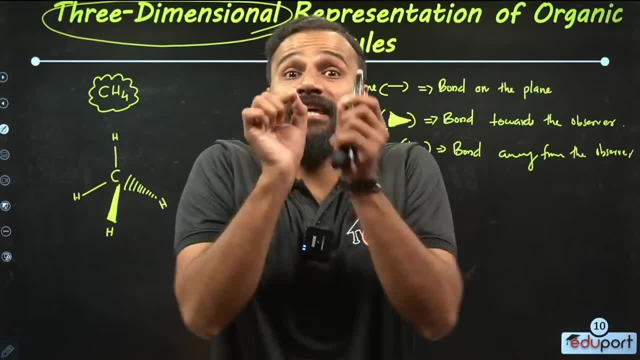 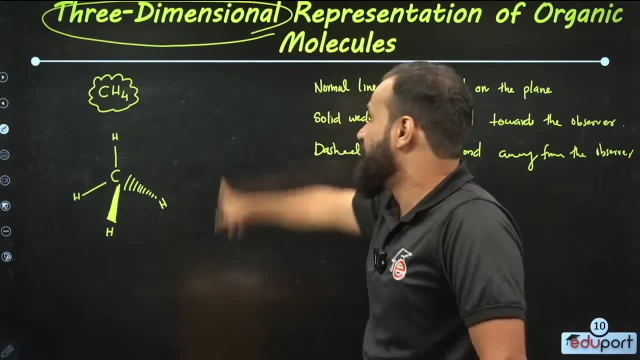 If it is okay, you have to comment, Because the question asked based on this. We are going to say it, We are not putting it to the last, We are not putting it to the last The question asked from here. The question asked is going to be studied right now. 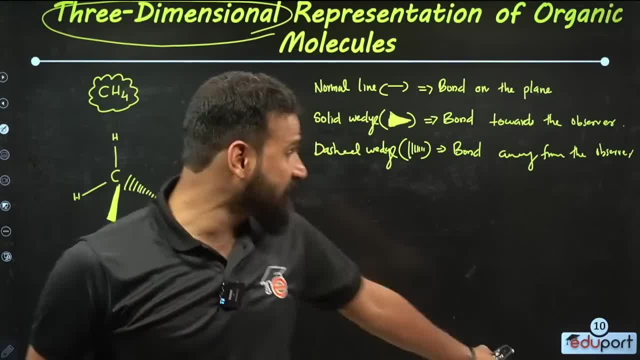 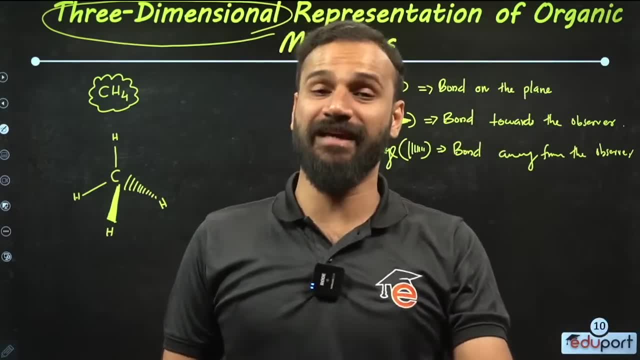 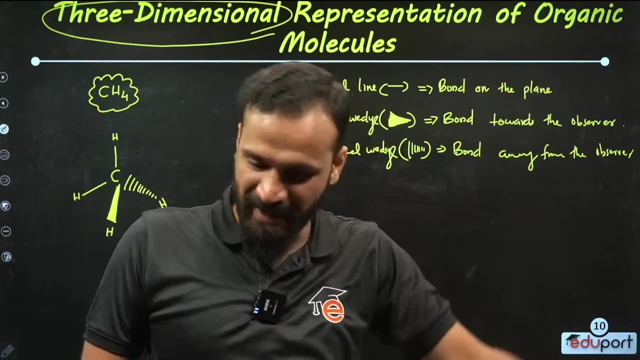 If it is okay, children, say it quickly, Say it quickly. Say it quickly Because we studied four representations. There will be a question from there. There is also a new representation from the fifth or fifth. It is three-dimensional. We clearly said how to do it. 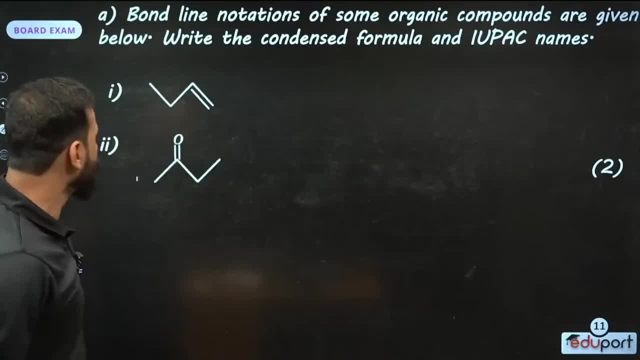 It is okay. It is okay, Very good. Then let's come to the question. Look, children, One question. Bond line notation of some organic compounds Are given. below Bond line notation has been given. Write the condensed formula And the UPSC name. 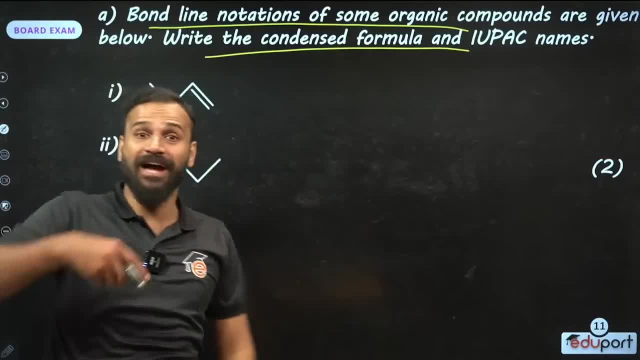 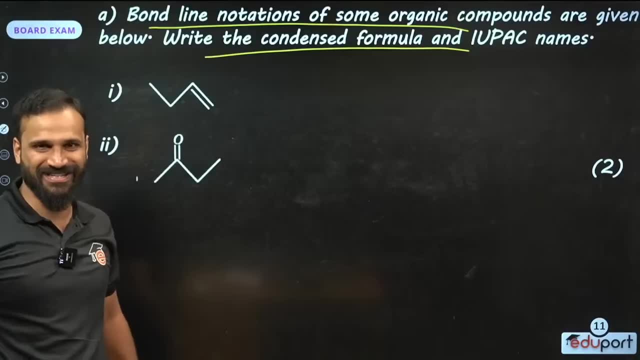 You don't have to say the UPSC name now, Because we are going to study naming. What is the question asked before that? The one who asked to write the condensed formula of this Short? This is the bond line. Write it short for this. 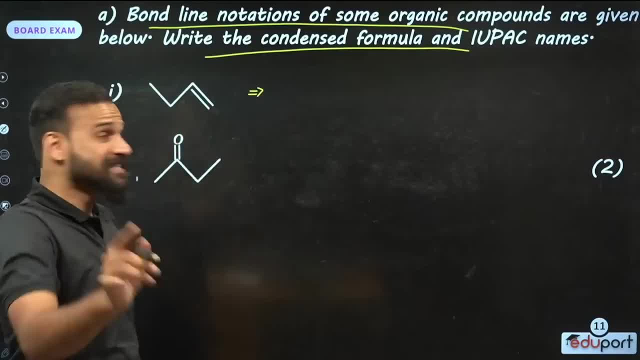 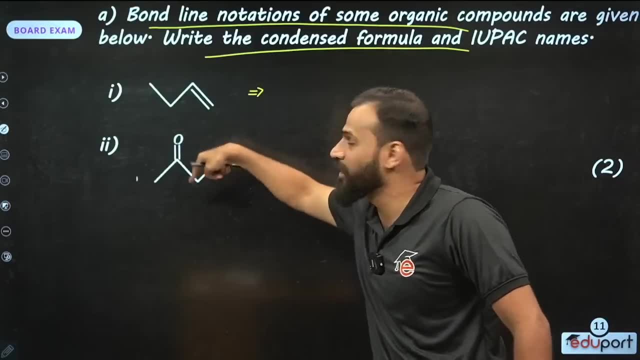 How do you write children? You have to write it. Don't you look at what I write? Don't I look at it? You write it. Write it in the paper. Write it The condensed formula of these two. Try to represent it in the paper in front of you. 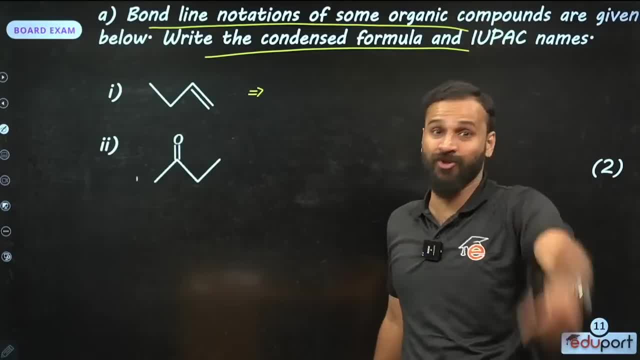 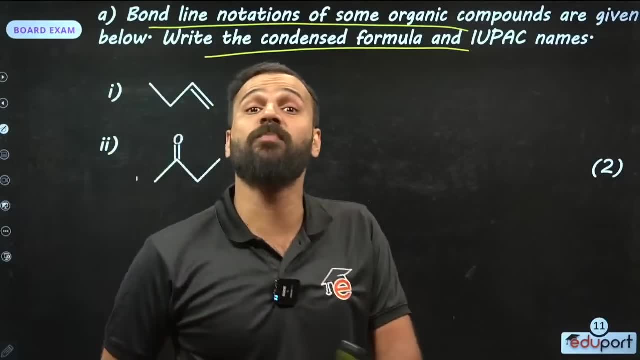 I will say it anyway. You can see whether it is right. You can see whether it is written correctly. This is very important. You have to do it with me, Then it can be studied from here. This is very important. Look, children. 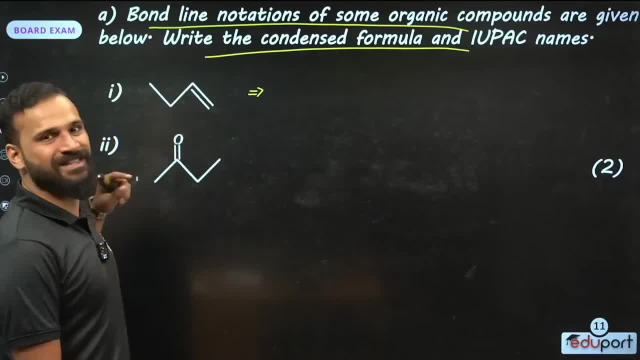 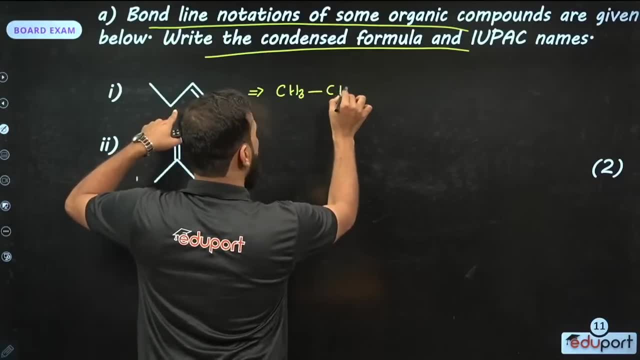 It is very important. Be careful. Yes, What? Who is here? Here is CH3.. Then write it. Write from CH3.. Who is here? CH2.. Write it like that. What do you have to look at? You have to get four carbon bonds. 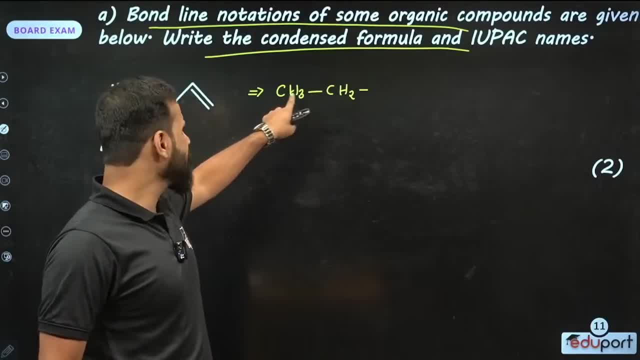 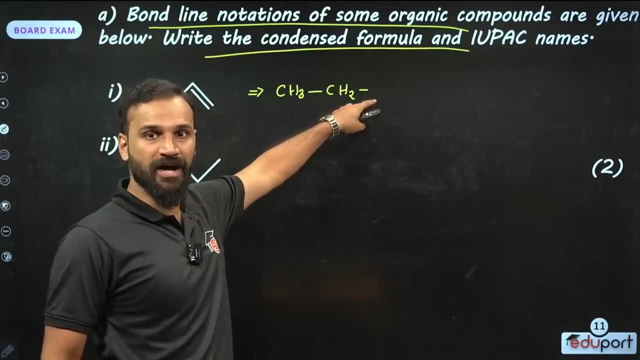 That's all. How many bonds are there? There is only one here. There is only one carbon here. Then there is a deficiency of three. Then put three hydrogen- There are bonds on both sides of this carbon. Then there is a deficiency of two. 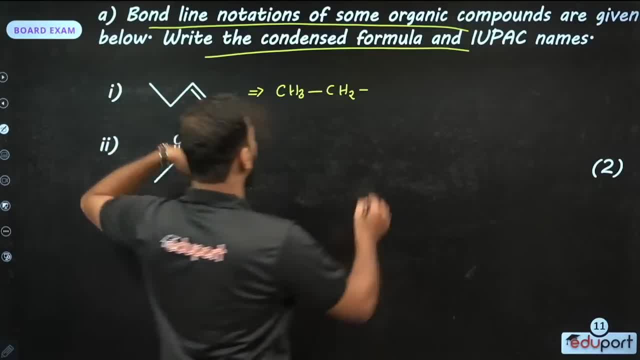 Then put two hydrogen. You have to look at it like that: Now, what is here, children? Third, carbon CH2 is not needed. CH is enough, Because there is double bond, Double bond. Then look One, two, three, four. 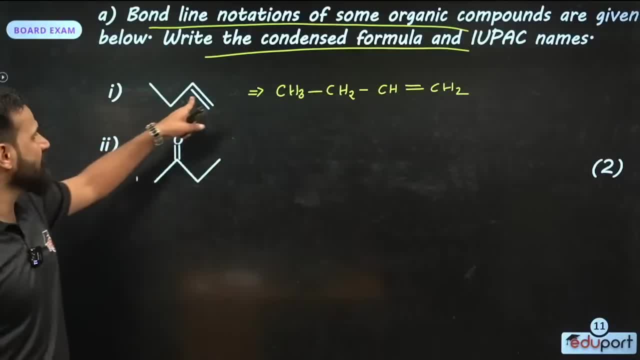 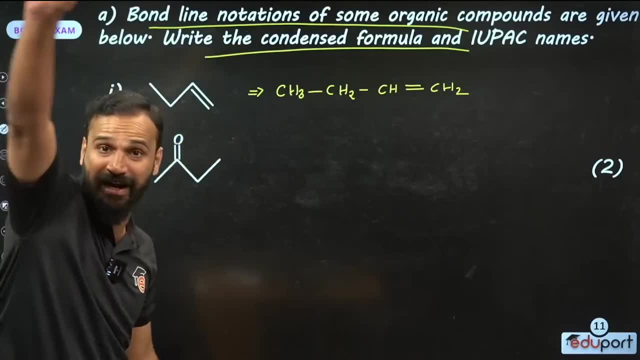 What will happen here? CH2.. Then this is its condensed formula. Very simple. If you have got a condensed formula like this, Then comment that someone got one. Yes, look What is coming from here. What is coming from here? CH3 is coming from here. 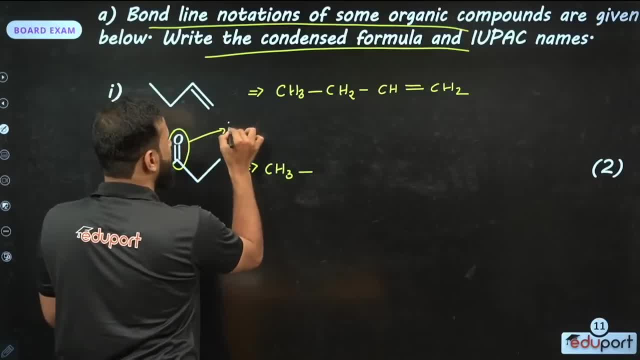 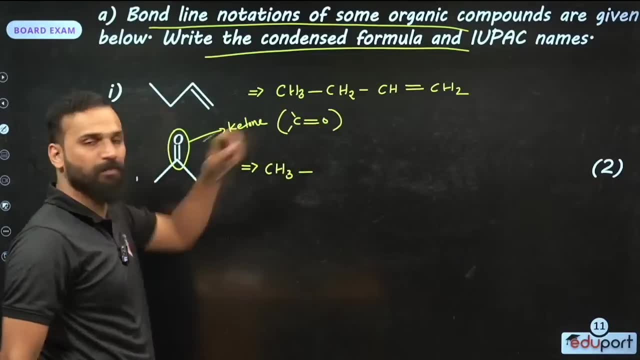 Who is here? Who is this? You should know. This is a ketone functional group. It says formula CO, It says ketone group. So he is simply showed to us what to do. That double bond has to be shown there. 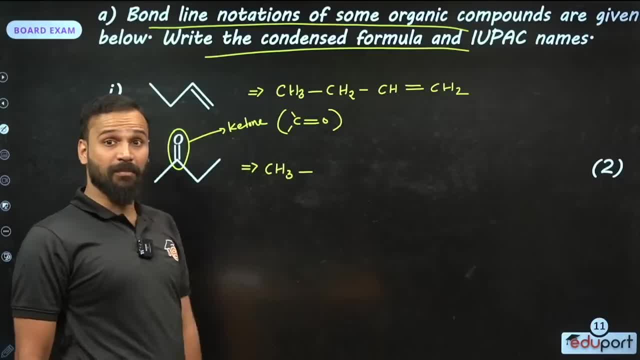 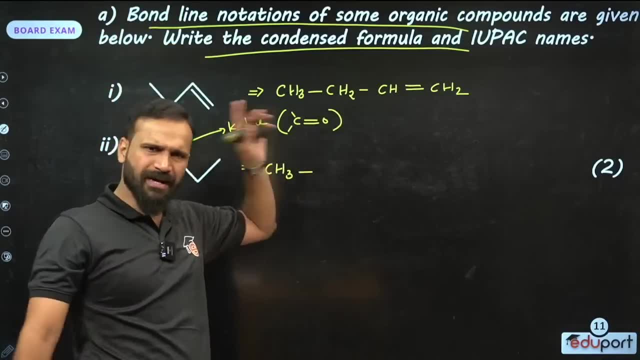 C1 has to be written. Then you will ask: the double bond has to be shown as condensed. That is, the CO is a functional group, The double bond that comes inside it. this double bond has to be shown there. Just write it as a function group: CO. 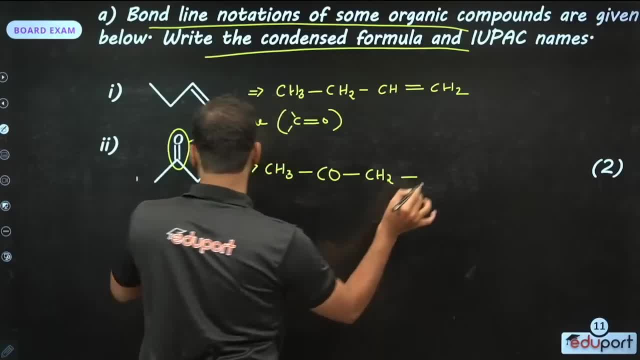 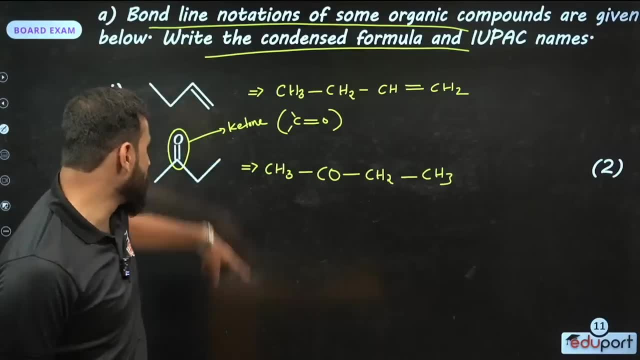 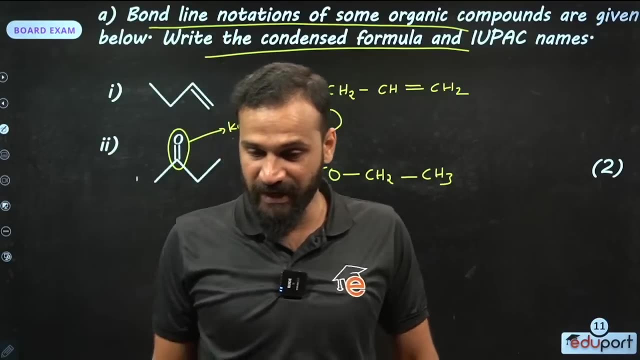 What is CH2 here? What is CH3 here? This is how we write the condensed formula. The condensed formula of these two molecules is written like this: You must have got it correctly. Very good, you have got it in Nauffal. 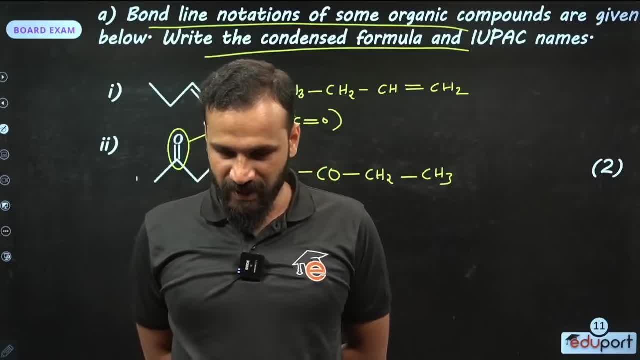 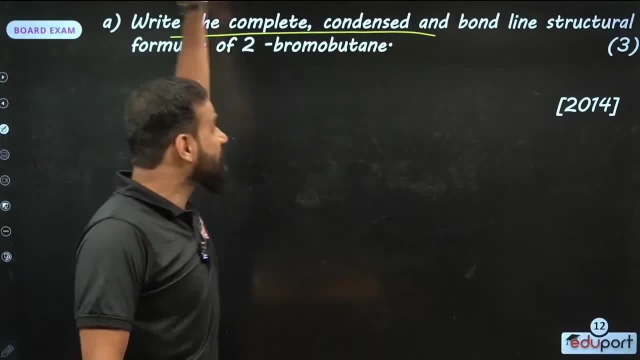 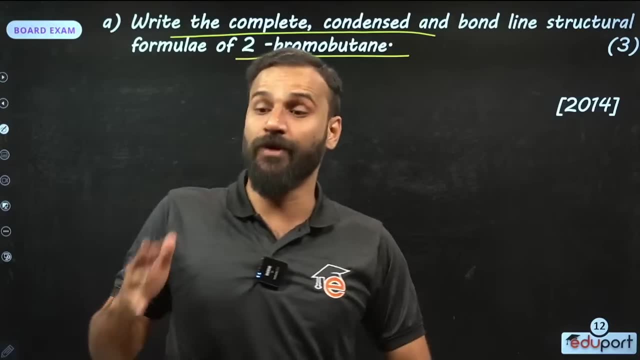 Write the complete, not just the complete condensed and bond line structure of 2-bromobutane. The complete, the condensed, the bond line of 2-bromobutane should be written First. I will write it as condensed. 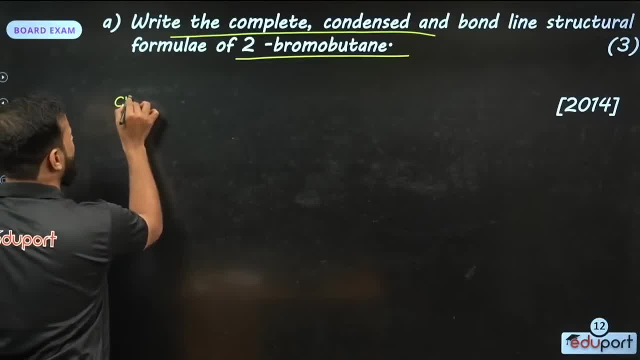 Isn't it 2-bromobutane? Isn't it 2-bromobutane? How does condensed come children? How does condensed come? 2-bromo means the second carbon is bromine. Isn't it 2-bromobutane? 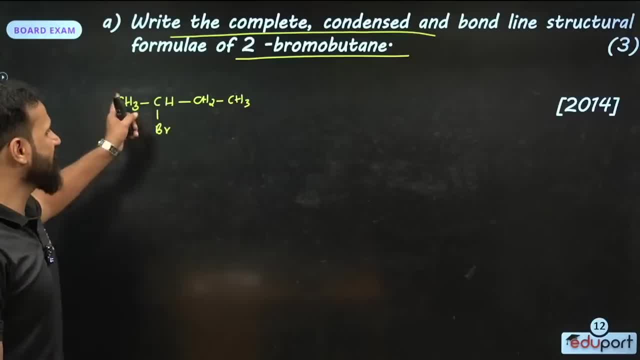 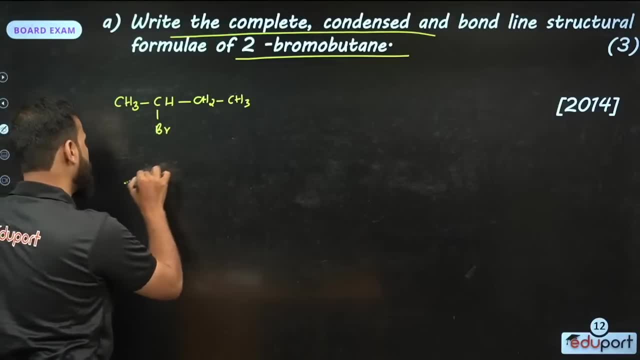 So 4 carbons, Isn't it like this, children? CH3, CHBr, CH2C. This is condensed. Now, children, how does the bond line come, Isn't it? 4 carbons, 1,, 2,, 3,, 4.. 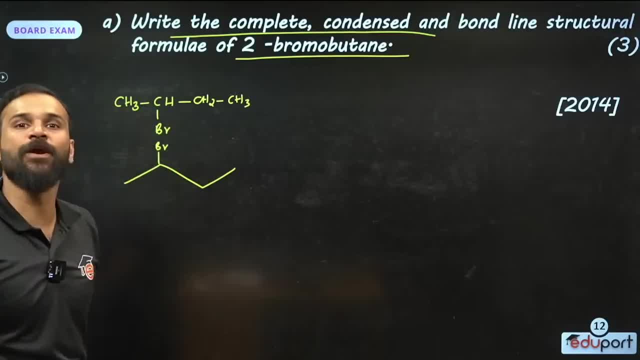 Who is in 2? Bromine? This is the bond line of this. This is the bond line: representation. Now, children, how to complete it? How to complete it? Look, Isn't it? 4 carbons: 1,, 2,, 3, 4.. 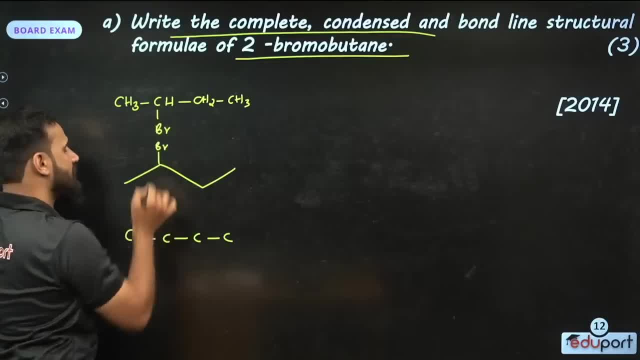 It can come like this, Isn't it, children? Look The second, that is, there is a bromine in the second carbon. This is the same thing. Now, all the rest can be filled with hydrogen. There are three here. 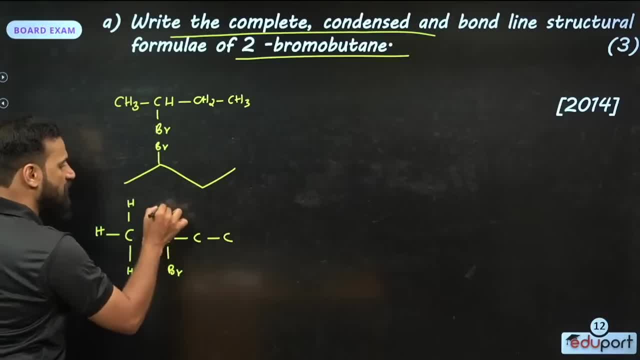 So did you show those three completely? Here is an H. Did you show it completely? There are two Hs here. Did you show it completely? There are three Hs here. Did you show it completely? Children- it is very important. 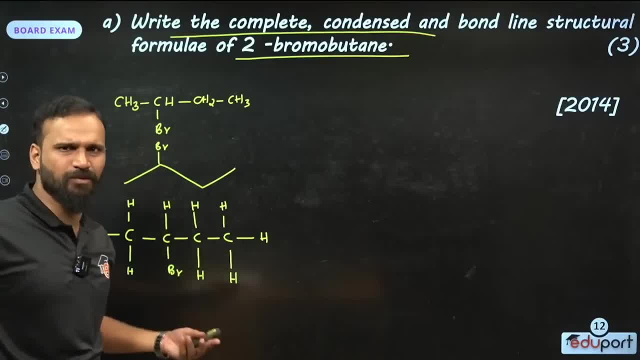 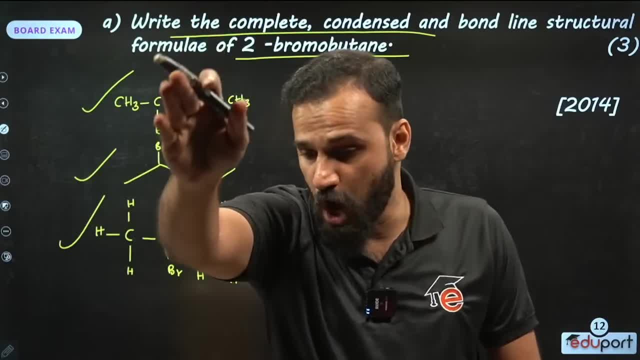 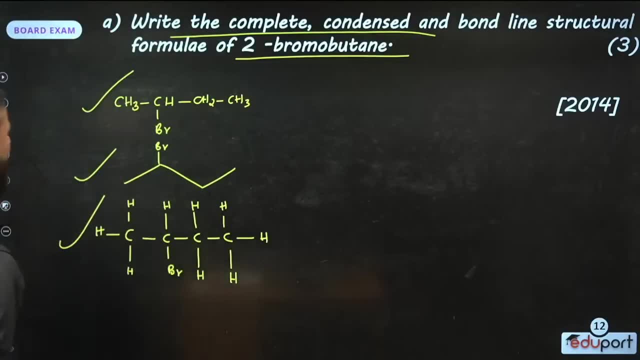 Can you write? That is very important. Yes, Very good, A lot of people can do it. Yes, Children, look, Look. Look at the next question. What is the question? If you change this question, it is the name of the UPSC. 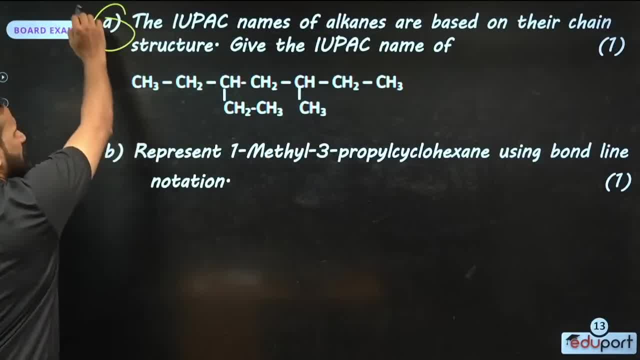 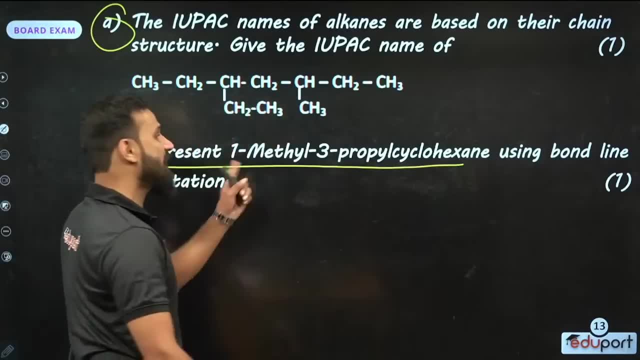 We will discuss it after we have said it. Yes, Very good, A lot of people can do it. Yes, We will discuss it after we have said it. There is a question here In the B part. represent one methyl three propyl cyclohexane using bond line notation. 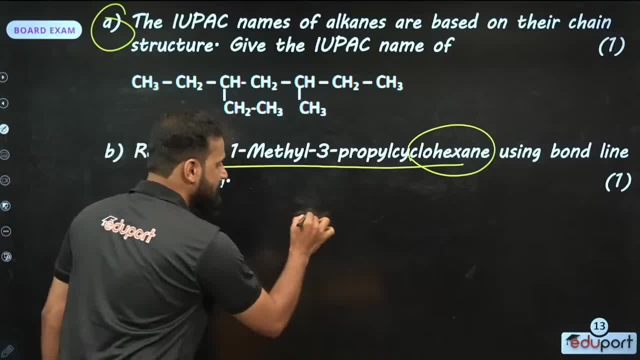 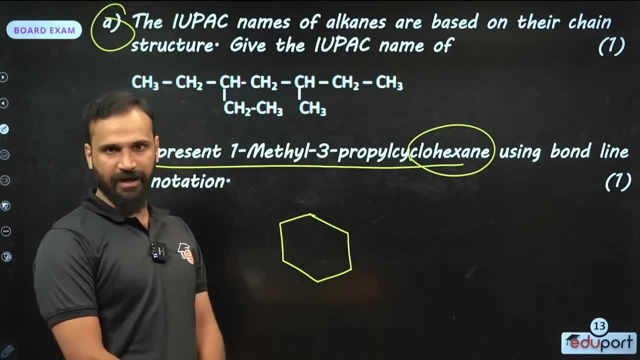 So first say cyclohexane. If you say cyclohexane, you can say that cyclohexane is the bond line representation of cyclohexane. Ok, Now, in the first position, methyl, In the third, propyl. 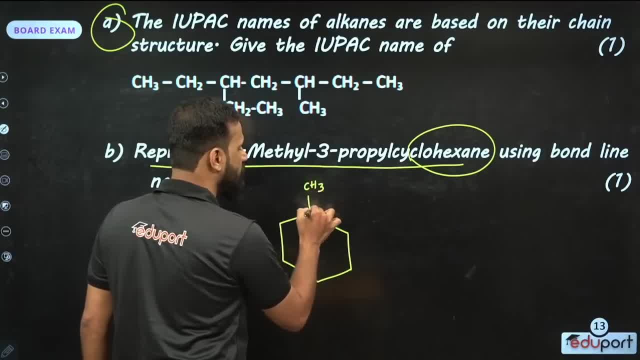 It is simple. You can say: methyl, CH3. Methyl, Then this is the bond line, right? Since it is a bond line, CH3 should not be given there. If a line is drawn, it means that CH3 is there, right. 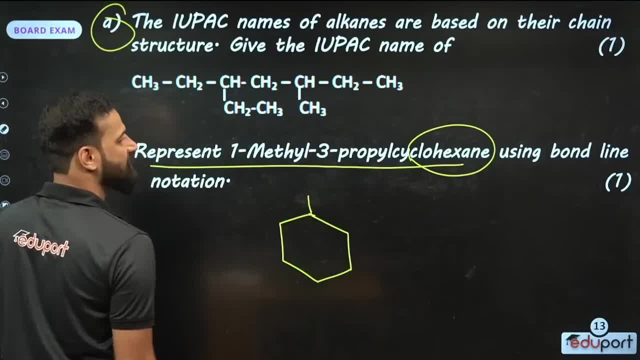 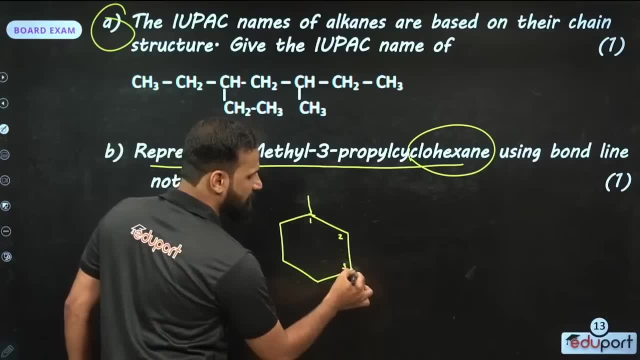 So it should not be given Now who is in the third position, That propyl. In the third position it is propyl. So if this is one, if this is two, this is not three, How to represent propyl children. 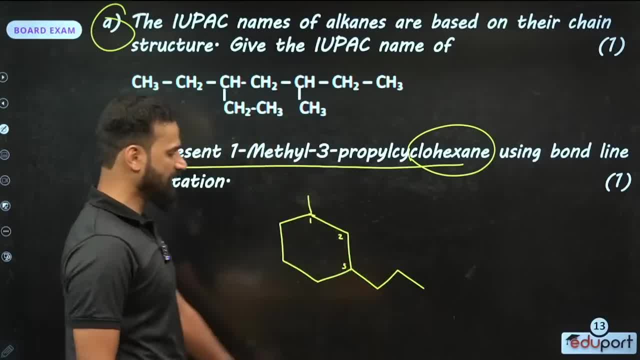 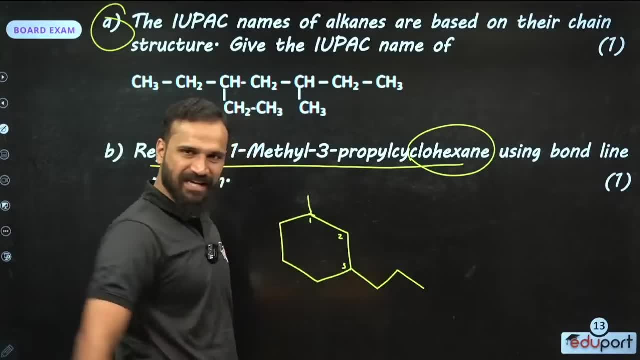 One, two, three. This is propyl. That is from here to here. one carbon, two, three. So propyl is in three. One has propyl, one has methyl. This is how their bond line representation comes. 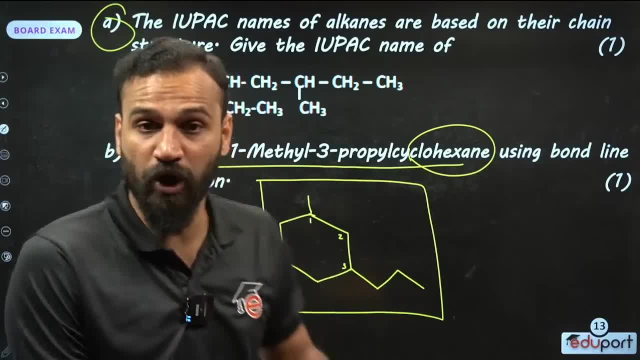 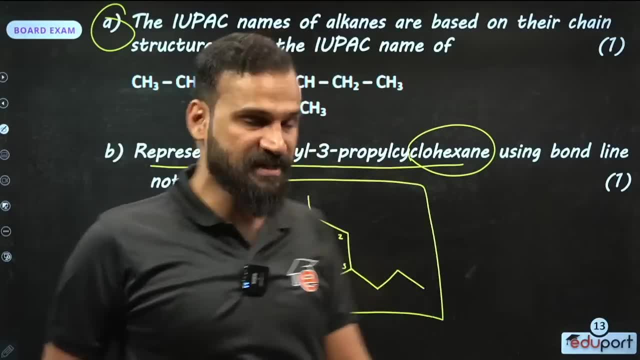 The question of one mark is: children, do you want to practice? Look, I have asked many times Kostya. So this is to be practiced and studied, Because if this is not practiced, it cannot be written right. 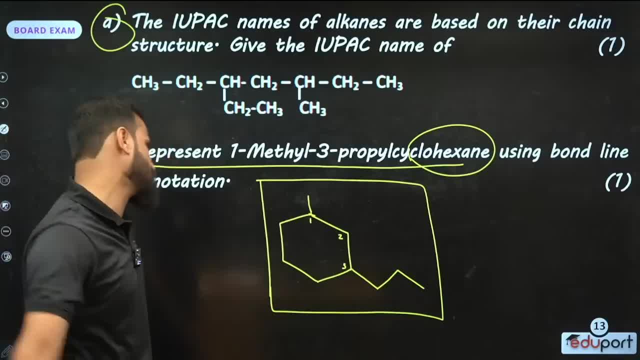 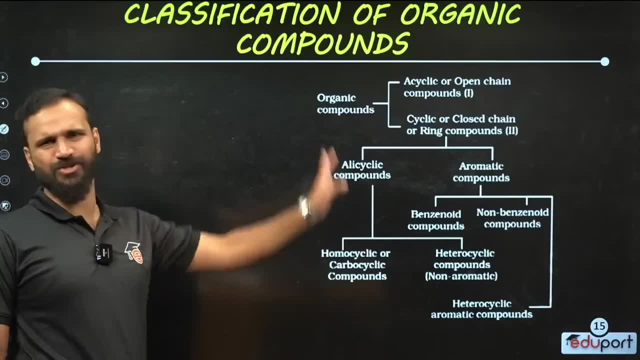 Yes, it is very important. Ok, children, what I said? Yes. Next look, Classification: How to classify organic compounds. This does not come as a question, Just know. Look, there are two categories of organic compounds. One is acyclic. there are two cyclic. 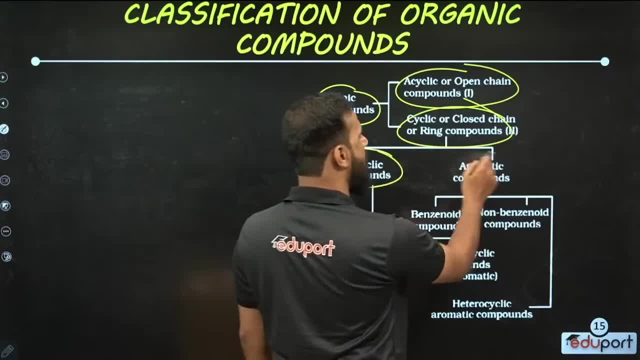 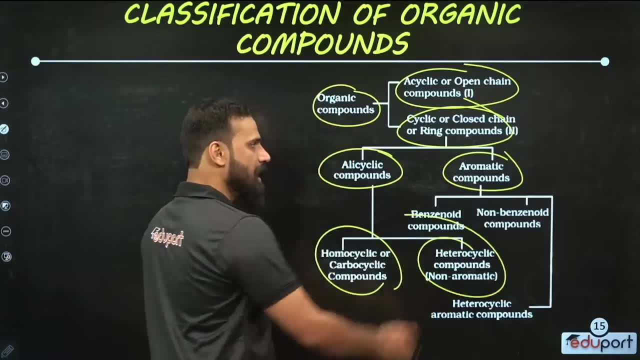 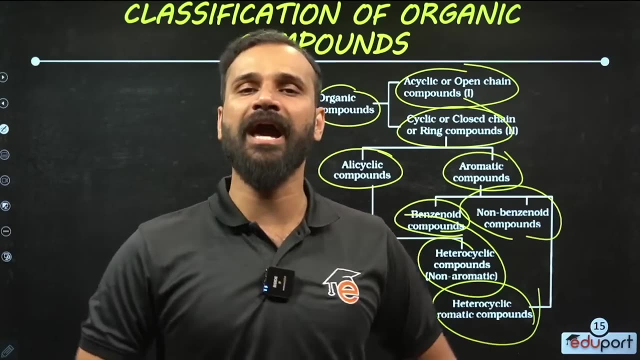 For cyclic. we classify it as allocyclic aromatic. Allocyclic has homocyclic and heterocyclic Aromatic has benzynoid, non-benzynoid and heterocyclic aromatic. That's just how organic compounds are classified. You will have an idea in your mind. 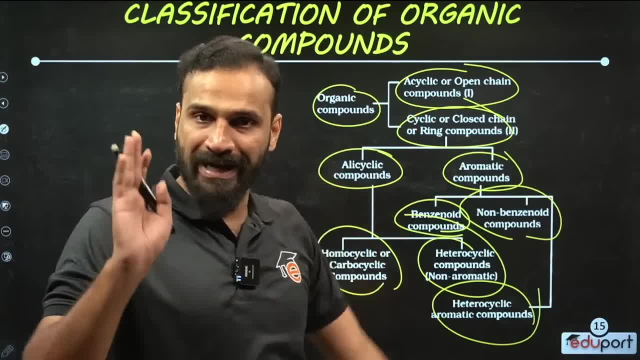 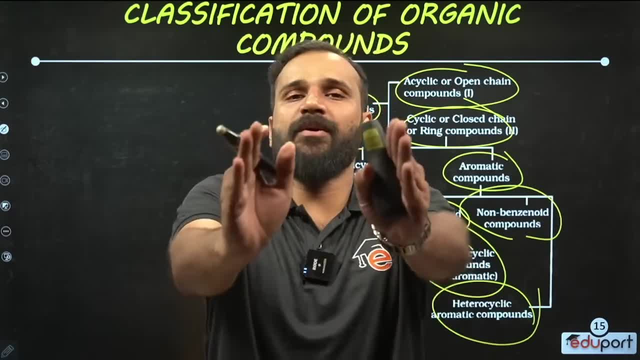 That's all there is. This is how organic compounds are classified. I am focusing more on where the exam question will come. My goal is only one This time the public exam The model before that. Everyone needs a plus, Not enough. 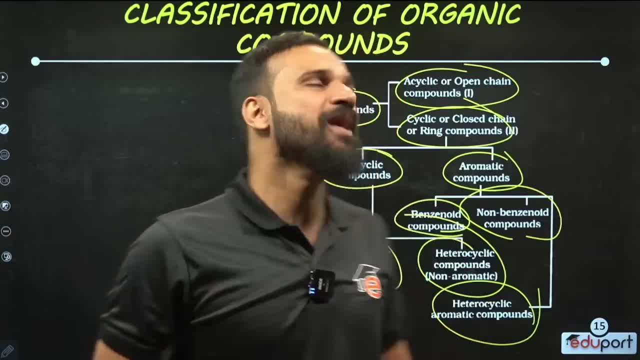 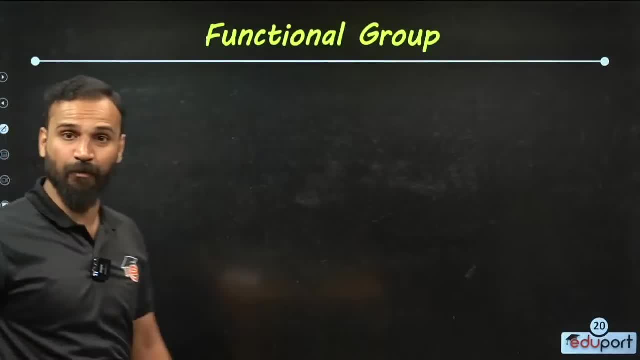 Everyone needs a full mark. I am saying without asking where that question comes from, So you just know this. There is no need to classify organic compounds like this. Now look, children. Functional group. The question asked for a mark is: what is a functional group? 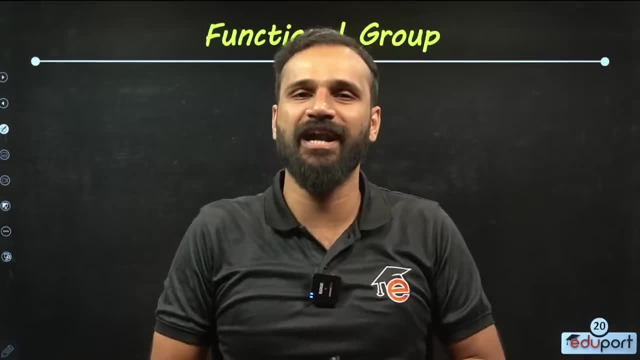 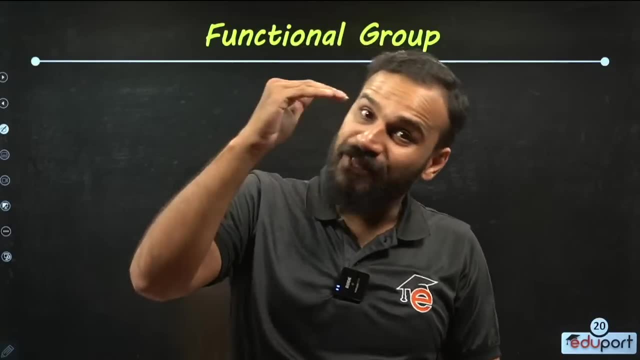 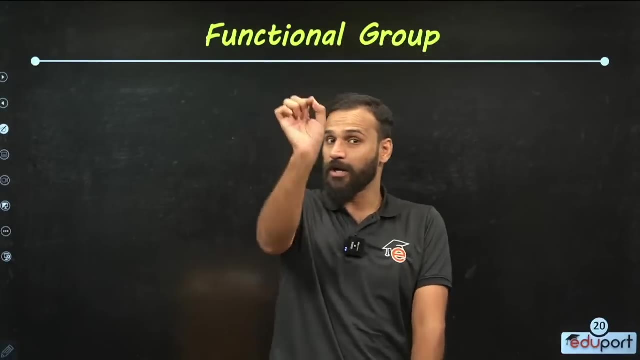 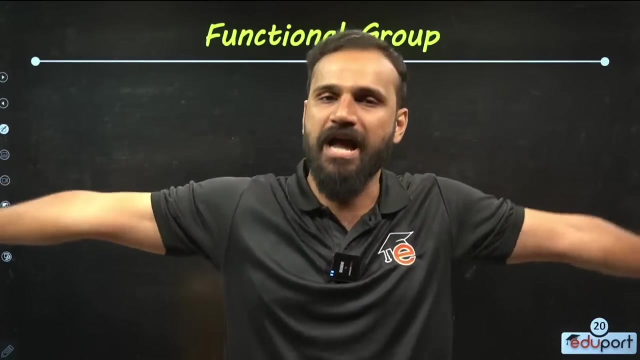 Children. this is all there is. Functional group is an atom or a group. What does that atom or that group do? It is bonded to a carbon atom within an organic compound. So what does that mean? You can call any atom or any group that is bonded to a carbon atom within an organic compound as a functional group. 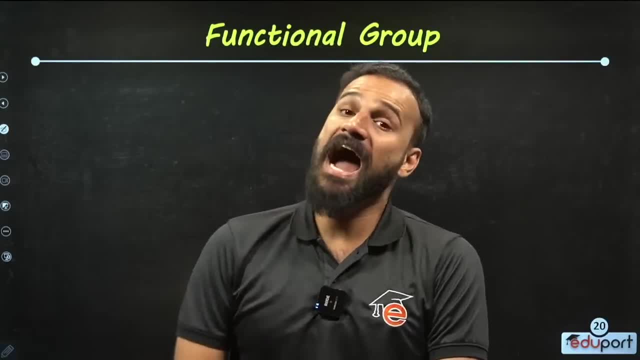 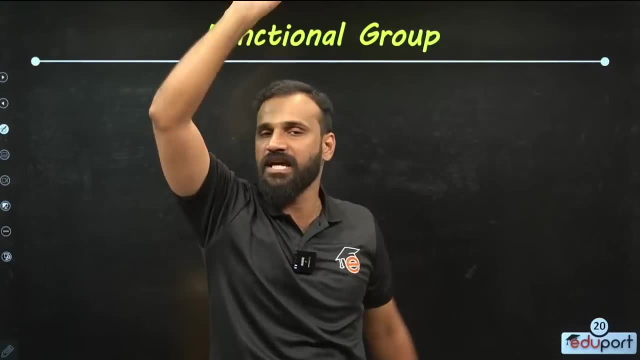 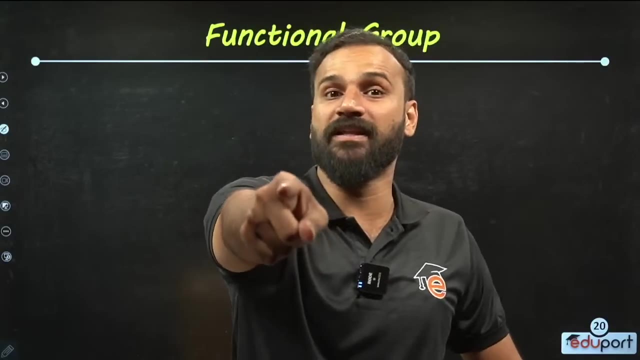 Except hydrogen. Not hydrogen, That is any atom or any group that is not hydrogen bonded to an organic compound is a functional group. This is very important. You have to study it well, You have to know it well. Okay, Let me ask you one more thing. 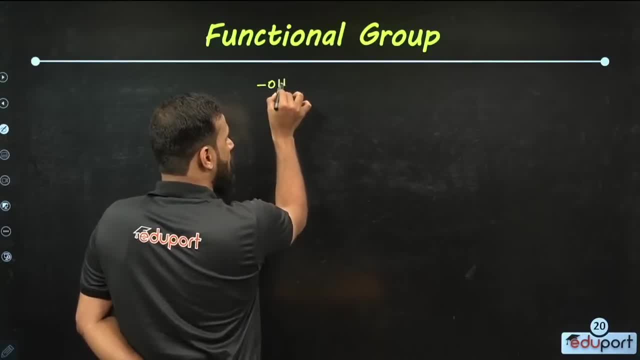 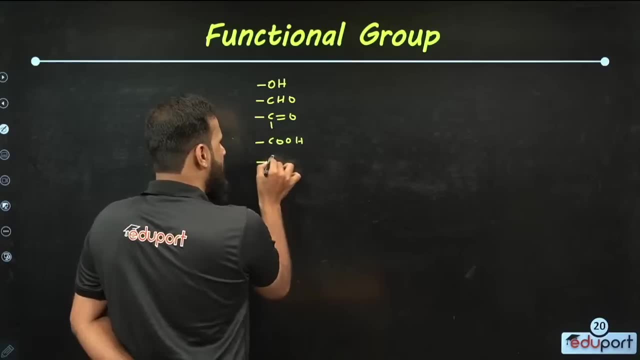 If so, there are many functional groups. Alcohol is a functional group. Aldehyde is a functional group. Ketones are functional groups. Acid is also a functional group. Amino group is also a functional group. Nitro group is also a functional group. 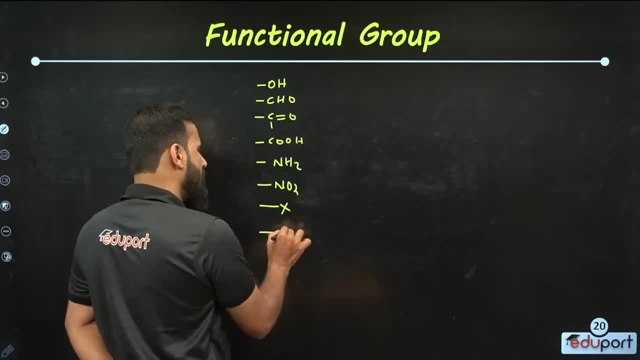 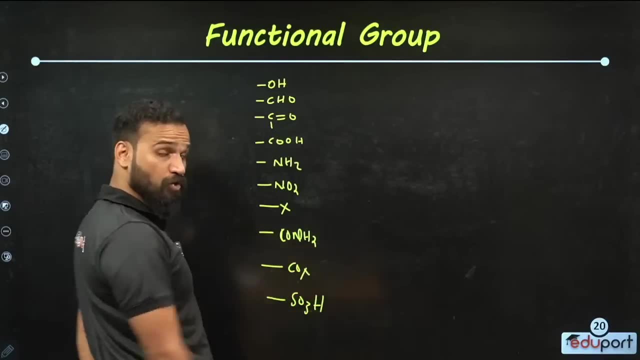 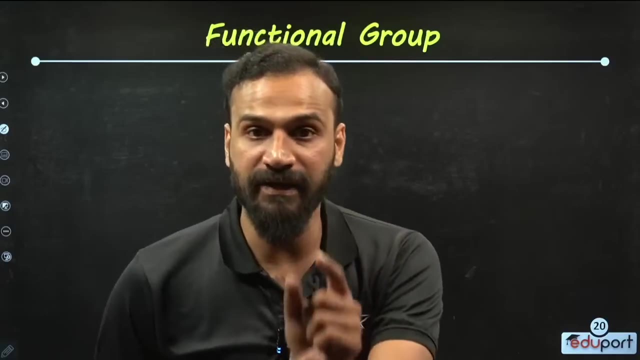 Halogen is also a functional group. Likewise, Amide is a functional group. It is also an acid halide functional group. SO 3-H, sulfonic acid is a functional group. There are a lot of functional groups, meaning that An Omega Darb which belongs to the ban 마스�io. 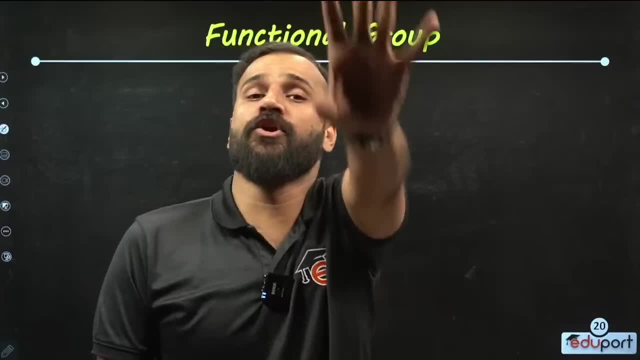 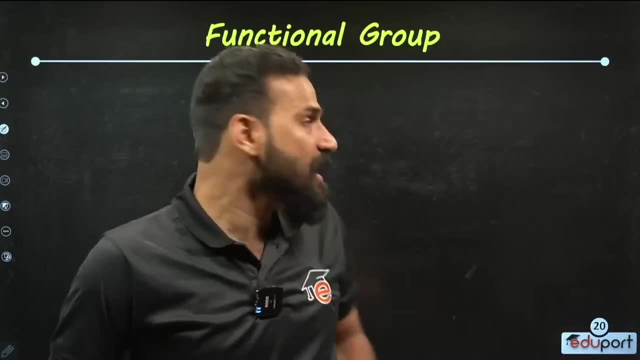 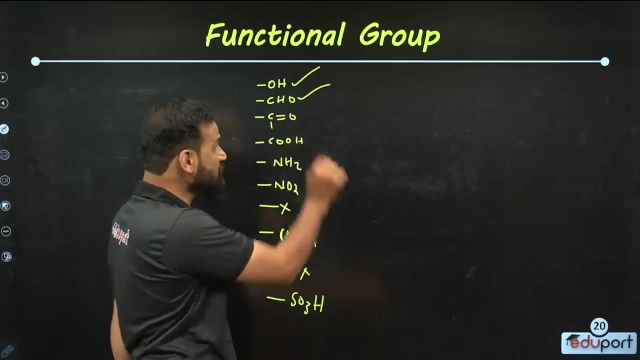 functional group is a name that you can call any act without hydrogen. It's okay, isn't it? kids, Let me ask you one thing: Is it the nature of alcohol that aldehyde will have? No, Is that the nature? Will there be ketones? No, 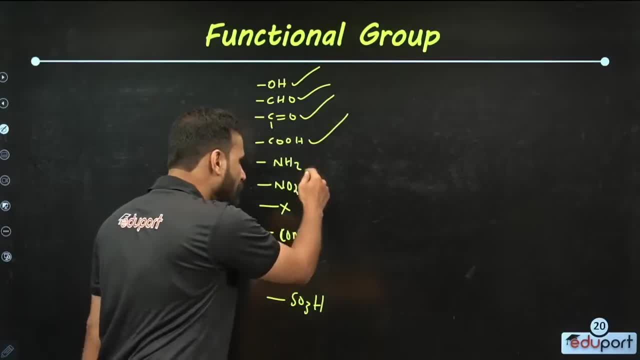 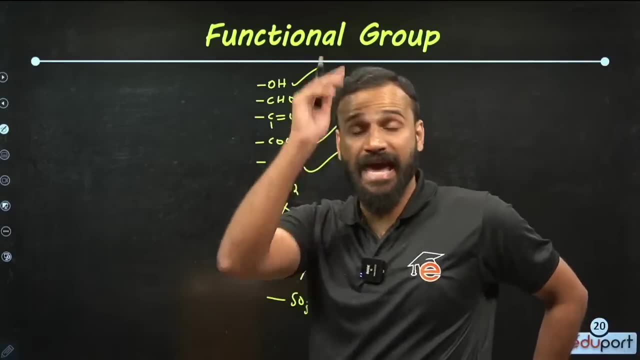 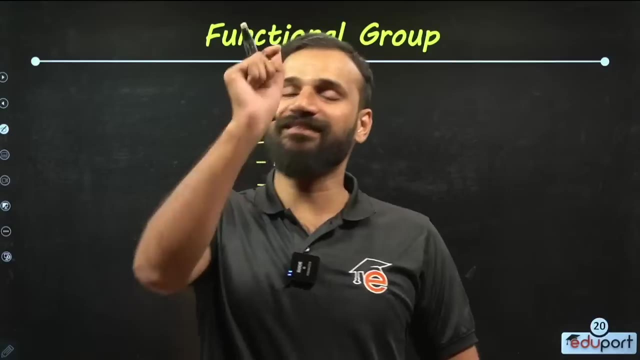 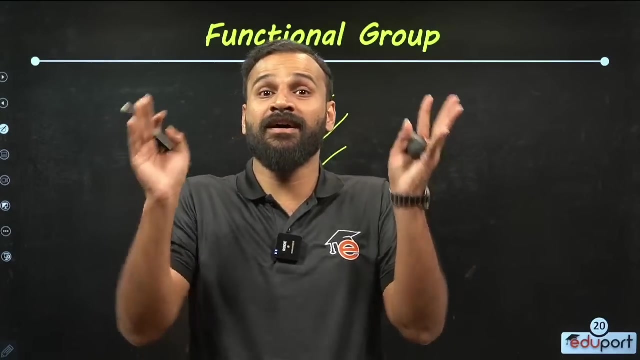 Is that it Not to show acid? Is that it Not to show amines? So you need to understand the character or chemical property of an organic compound. Who decides it is sect gal are very important that it's a functional group inside it. It must be remembered and learned. 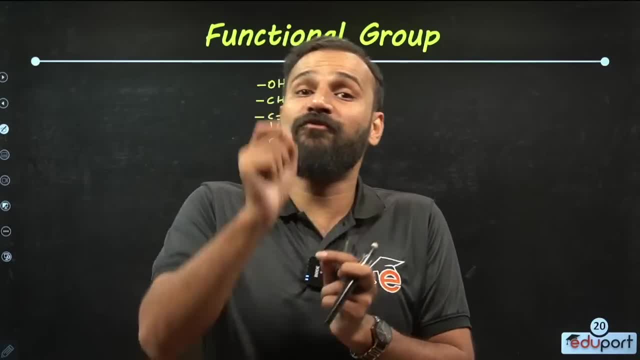 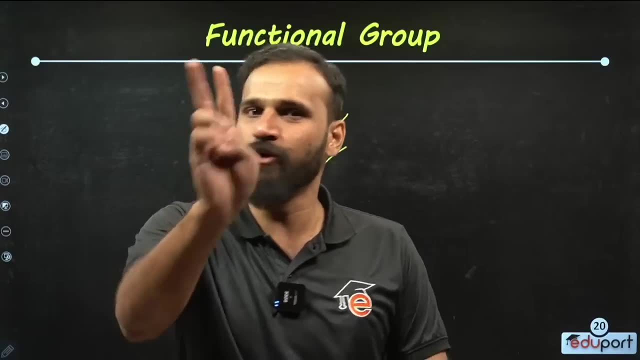 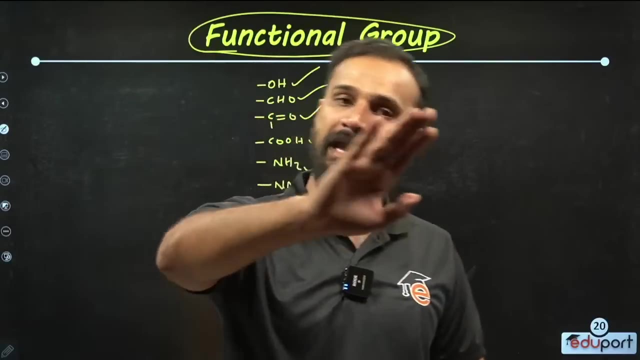 It is that functional group in an organic compound that оз. What does the compound decide? It decides the properties. These two things should be known. So the functional group is all atoms, and all groups that are bonded to the carbon atom are functional groups. 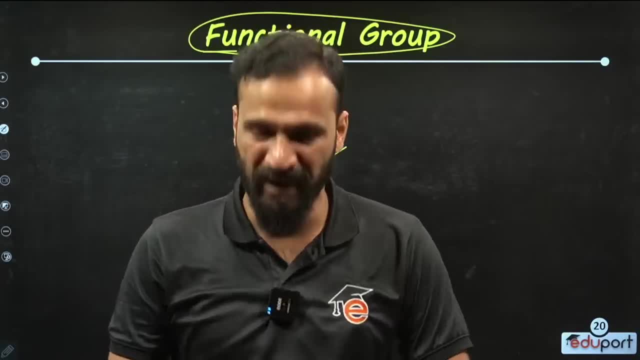 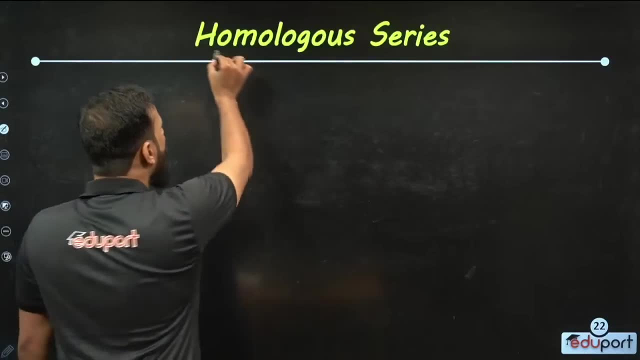 The chemical property of that compound is determined by that functional group. These are all examples of it. It is a question for everyone. Study it Now. look at the homologous series. What is the homologous series? Homologous series. 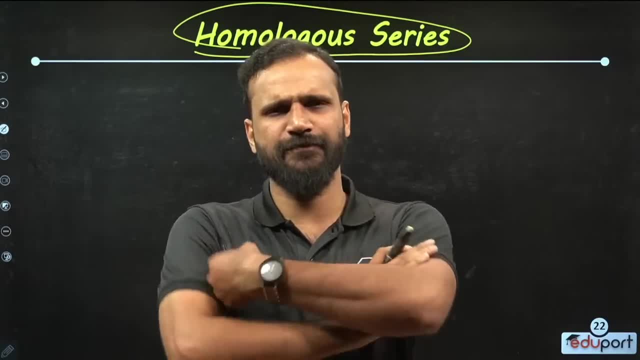 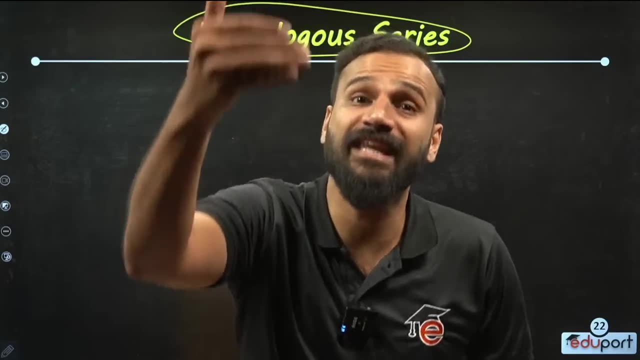 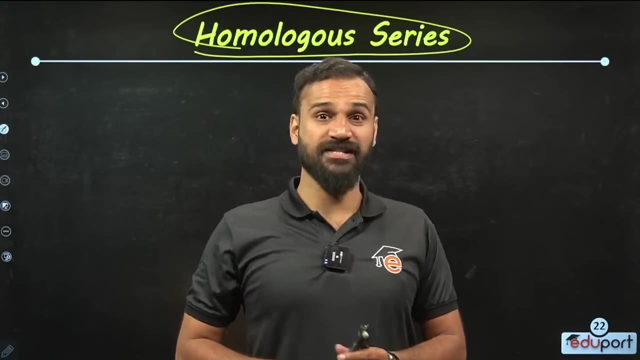 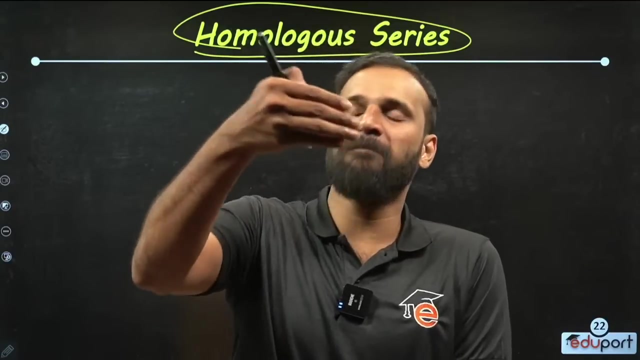 It is important to know what is the homologous series. What is the homologous series? What is the homologous series? It is the series of organic compounds having the difference, having the difference: difference between the adjacent members, difference between the adjacent members. 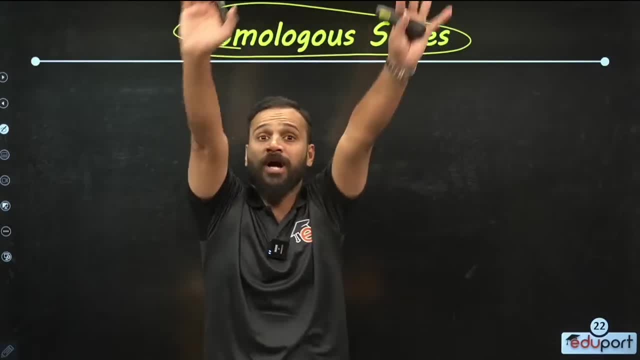 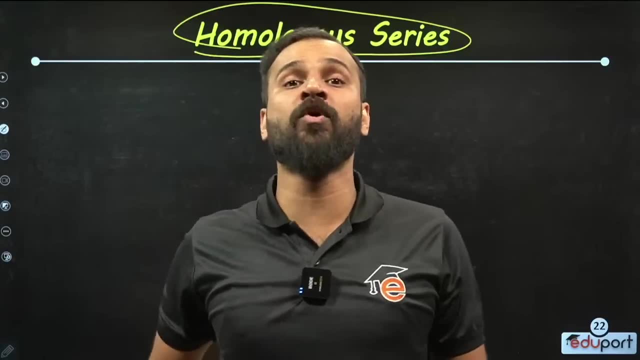 What is the difference? It is a CH2 group. If you ask the homologous series, what is the homologous series? It is a series of organic compounds. The homologous series is called a series of organic compounds. What is the specialty of that series? 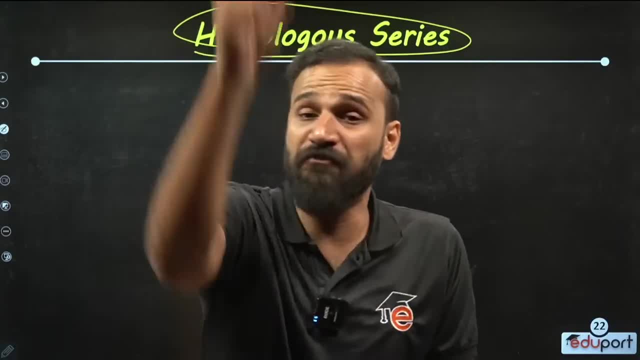 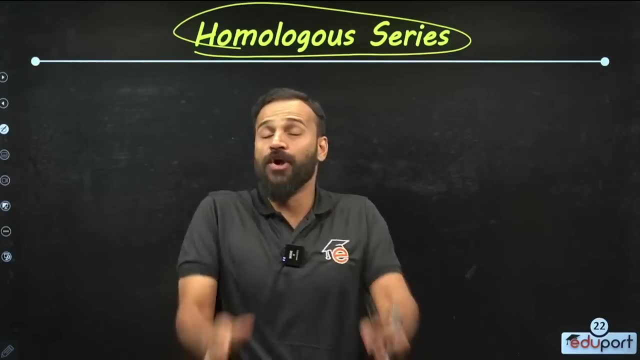 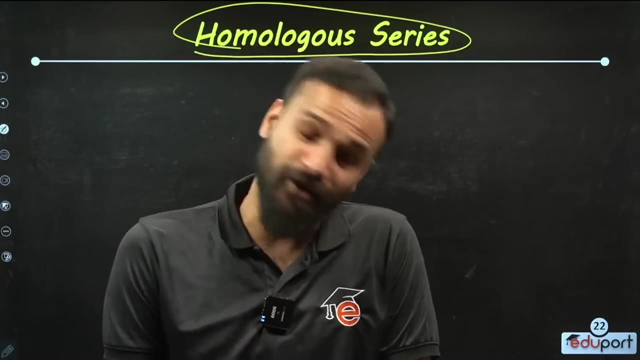 The difference between the adjacent members of that series is a CH2 group. What is it, dear friends? It is a CH2 group. The difference between the adjacent, The group of elements with differences, adjacent members, sorry, the group of compounds or series of compounds. we can call it homologous series. 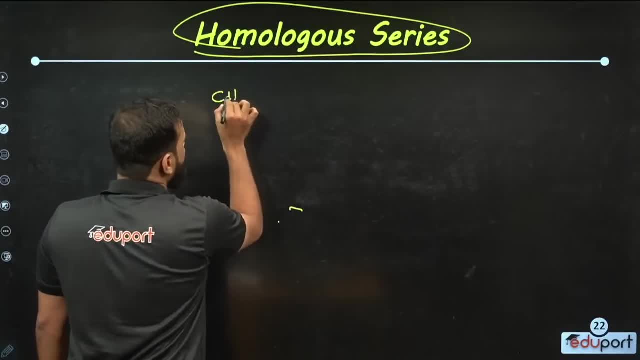 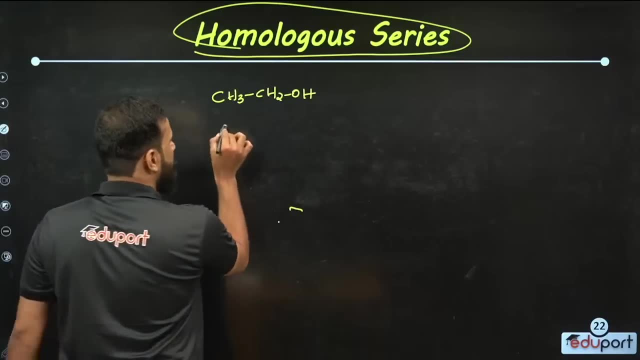 When we say example, it becomes clear: See CH3CH2OH. This is the first member of a homologous series. Do you know who is the second member? CH3CH2CH2OH? Do you know who is the fourth member? CH3CH2CH2CH2OH. 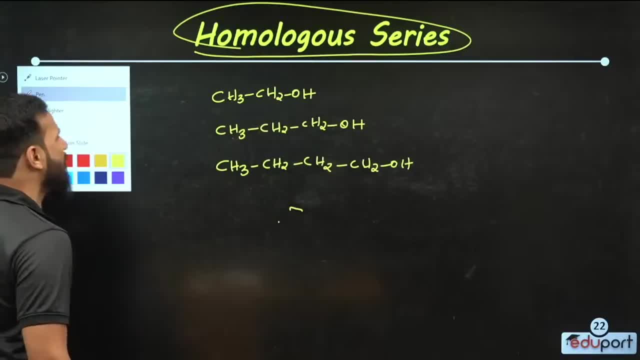 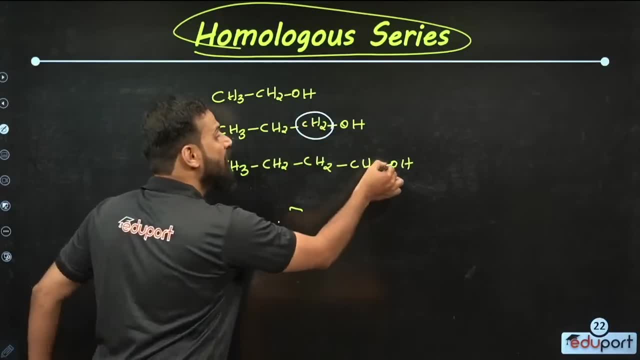 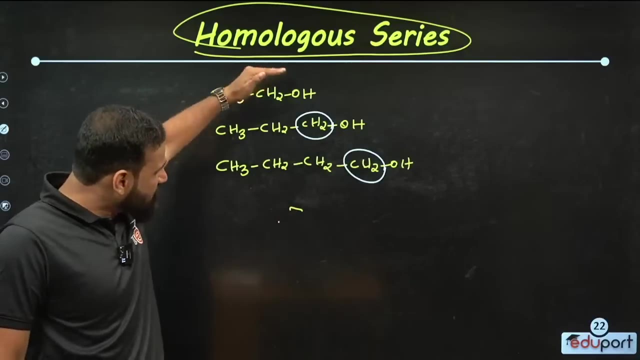 The reason is that the difference between the first and second members is that one CH2 is more here. When it comes to the third member, again one CH2 is more. Okay, Again one CH2 is more. So the difference between the adjacent members is the difference between a CH2 group. 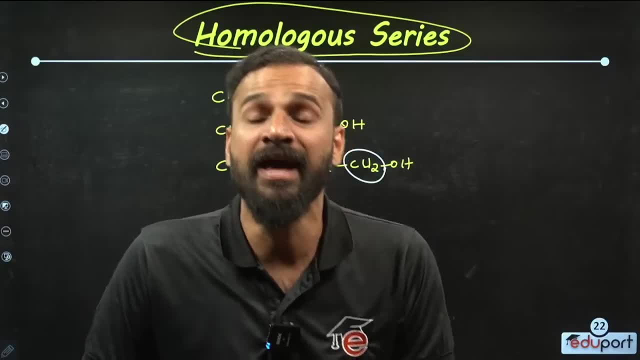 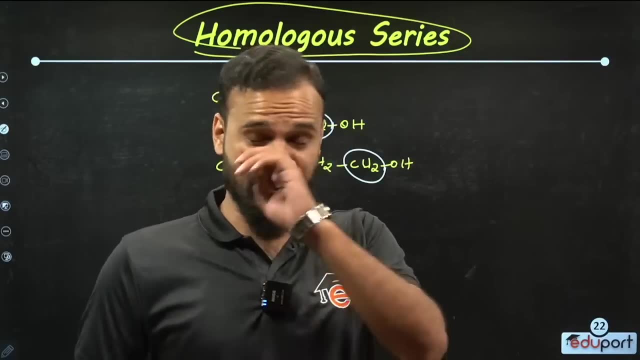 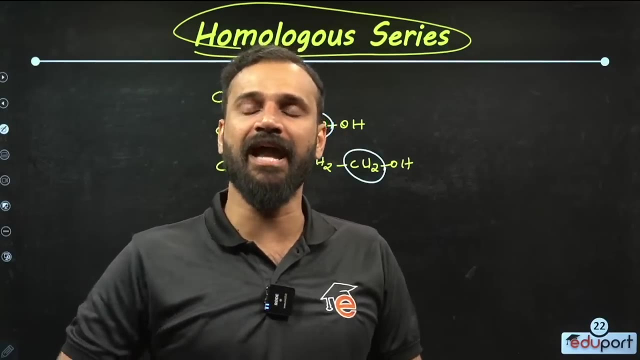 For such series of organic compounds, you can call it homologous series For one person. what is homologous series? Okay, series of organic compounds in which the adjacent members are differed by a CH2 group that is called homologous series. 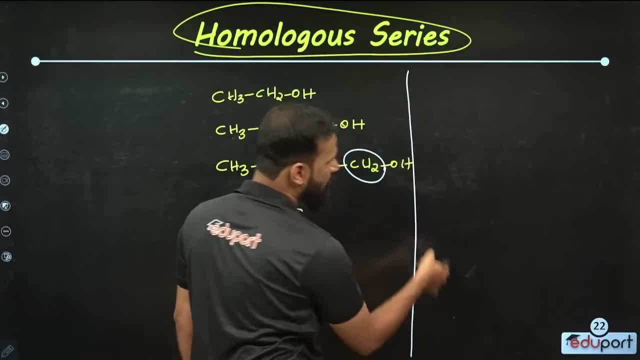 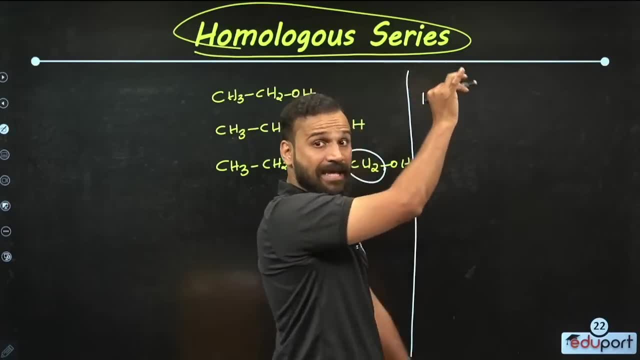 If you want, you can add one more thing to it. There are some features of homologous series. Do you know one thing? What will happen to all the members in that homologous series? It will be the same functional group. 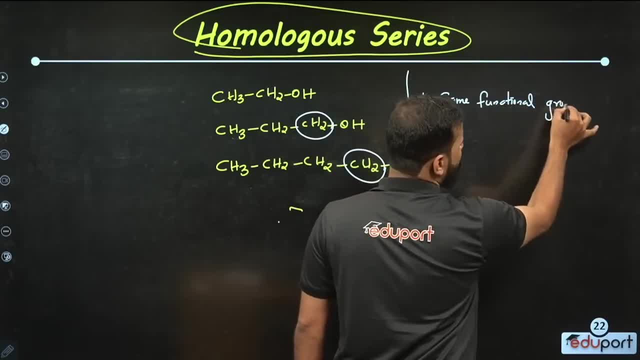 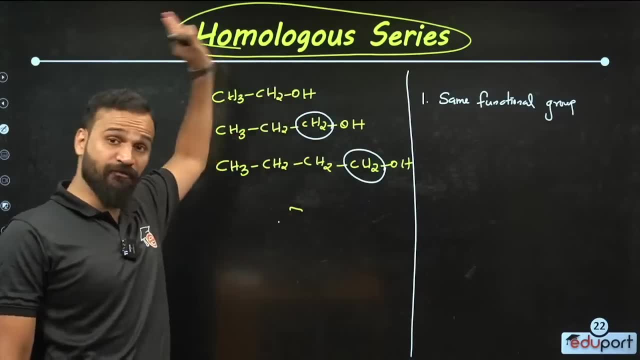 What will happen to the children? It will be the same functional group. See, here OH is not present. If so, then OH will be present in all. First there is no functional group, Then it will not exist in anyone. So if there is a functional group, it will be the same. 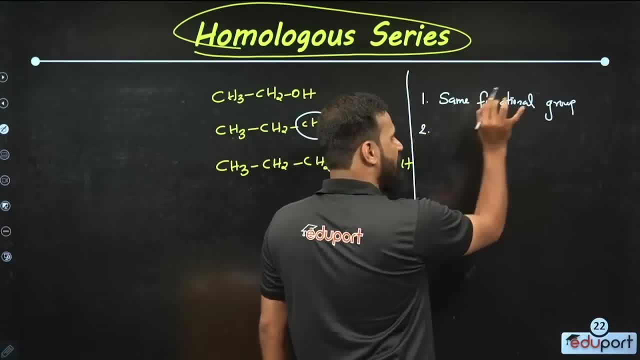 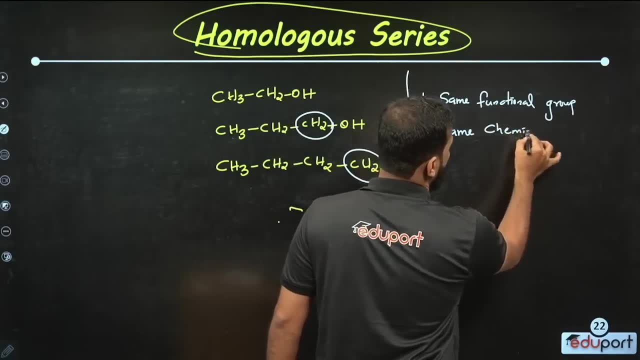 That is a special thing. Second thing, since the functional group is the same, what is the chemical property they show? It is the same. It is the same chemical property. What is it? It is the same chemical property that he shows. 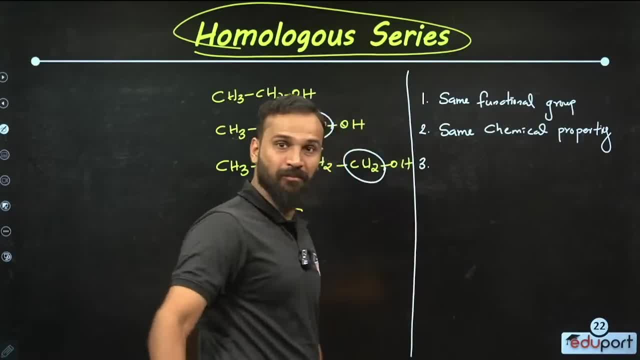 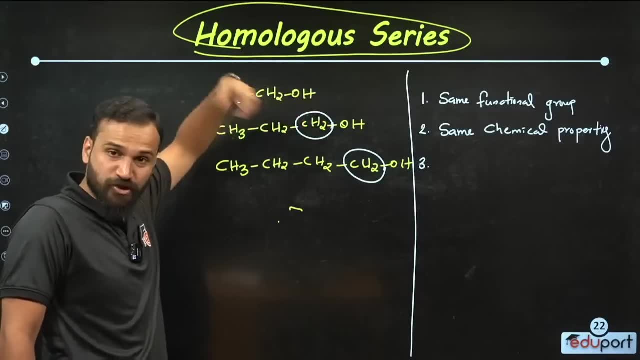 Likewise. do you know what is the third point? The third point is the physical property of regular change, Because when the CH2 is added from the first member to the second member, the CH2 increases right. So there will be a slight change in the physical property. 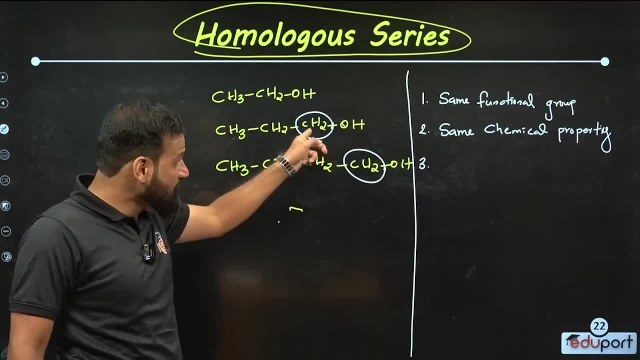 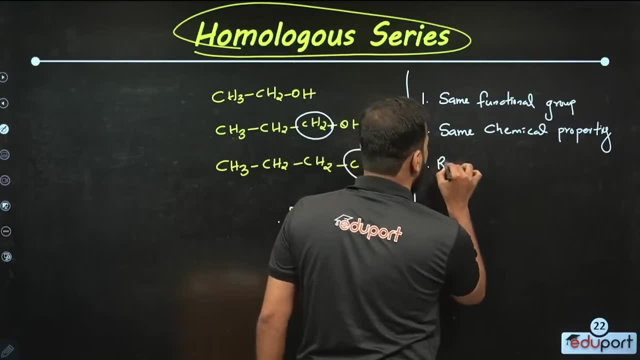 like physical belt and point, Then look after that. when it reaches the next member, another CH2 increases. So there will be a regular change again. So what is regular change? What is it, children? It is a regular change. 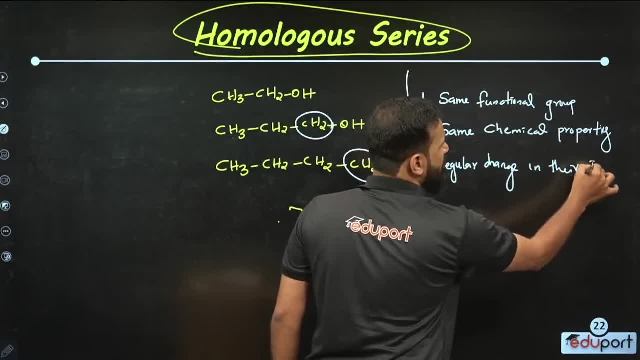 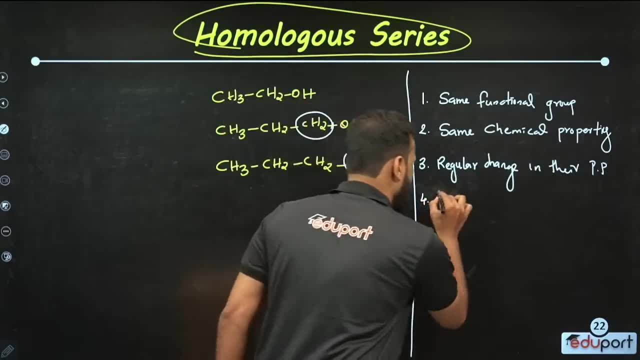 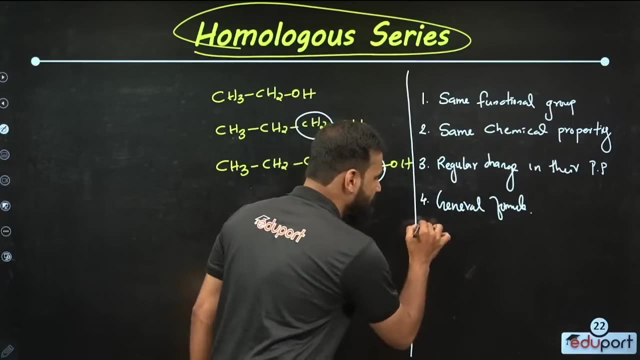 Regular change in their physical properties. Remember that. What is the fourth point? children. They will have a general formula. What will happen to them? They will have a general formula. They will have a general formula. Do you know what is the fifth point? 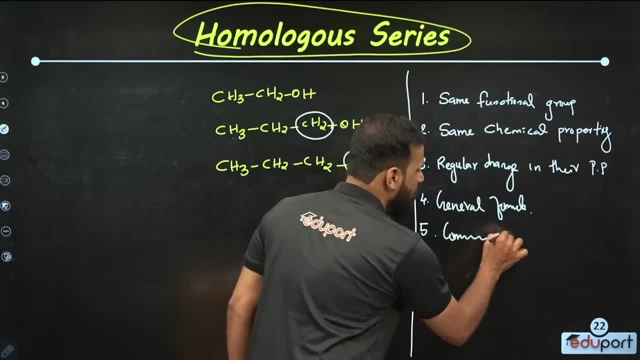 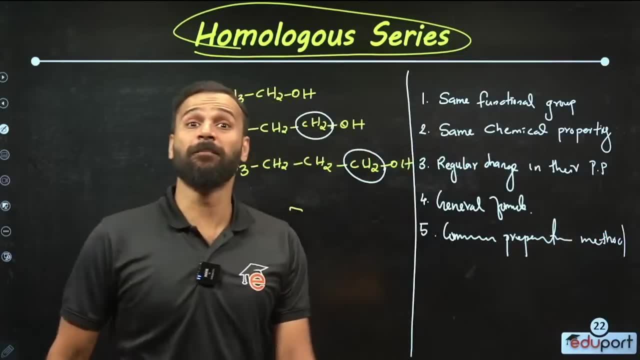 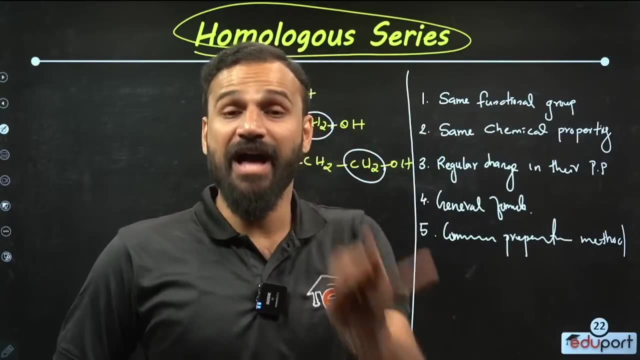 They will have a common preparation method. They will have a common preparation method. They will have a common preparation method. So what is the point of the homologous series? It is the same functional group. Everyone will have it. What is the second point? 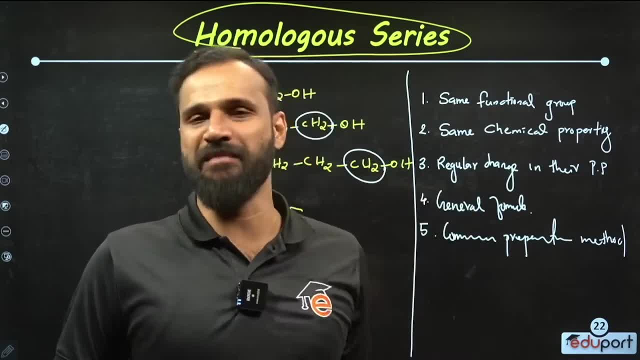 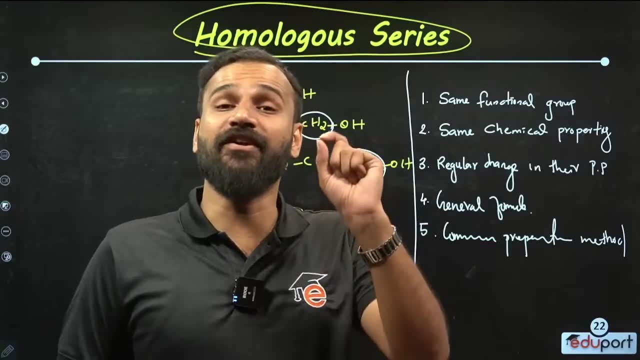 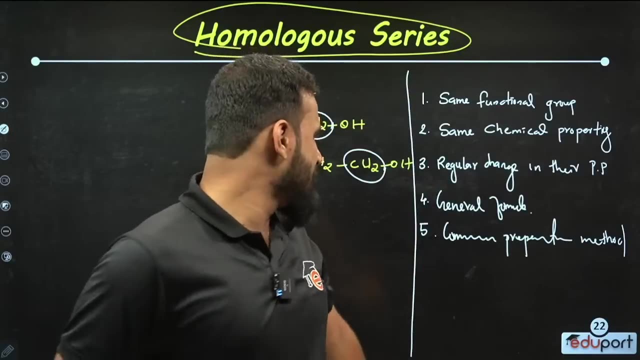 The second point is that their chemical property is the same. What is the third point? There is a regular change in physical property. What is the fourth point? They will have a general formula. What is the fifth point? There is a common preparation method. 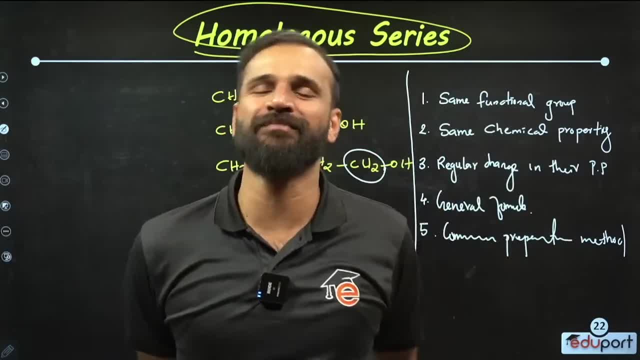 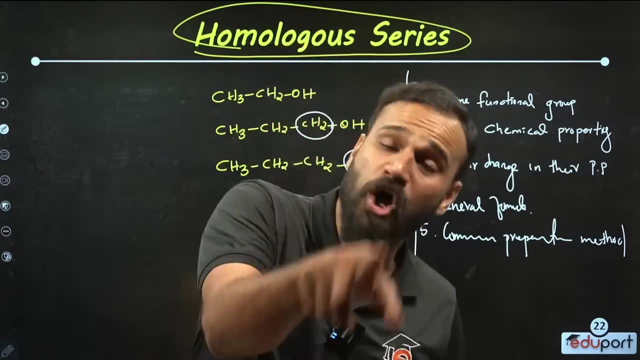 What is there? There is a common preparation method. You have to remember and learn. So what is the functional group? What is the homologous series? We often ask this question to someone. That is what we have learnt at the end. 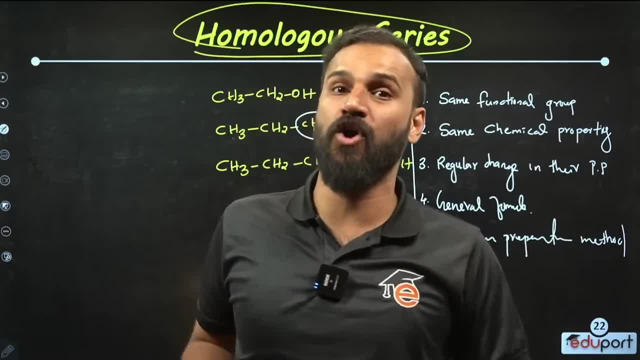 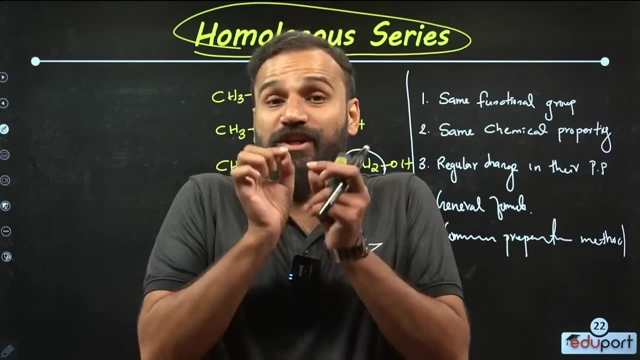 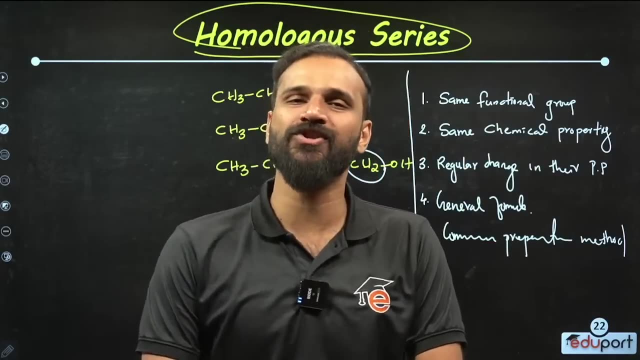 What is the homologous series? It is a series of organic compounds in which the adjacent members are different by a CH2 group. What is the difference of a CH2 group? There are adjacent members. Such series of organic compounds can be called homologous series. 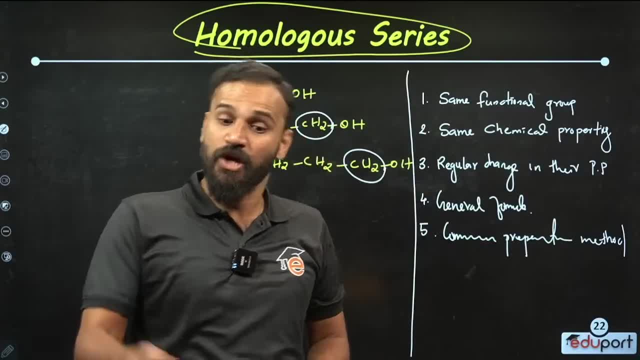 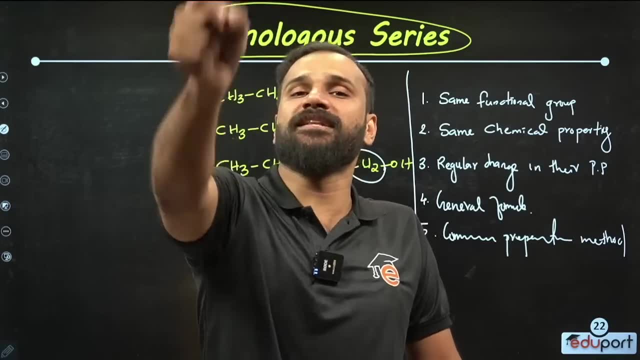 We have discussed the characters of it. What did we say before? What is the functional group? It is a group of atoms that are bonded to the carbon atom of an organic compound that is not hydrogen. All atoms and all groups are functional groups. 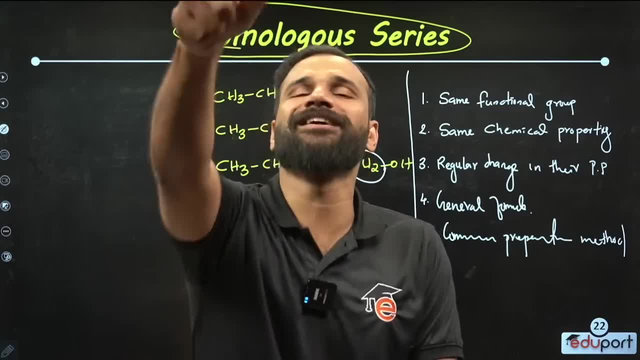 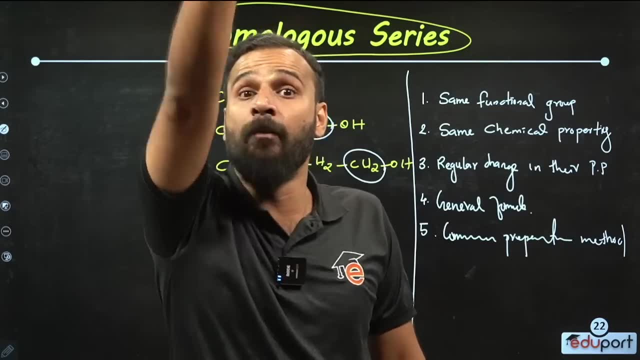 That functional group determines the chemical property of that compound. Children. is it okay? The last two points of the first mark: What is the functional group? What is the homologous series? Is it okay? If it is okay, say it quickly. 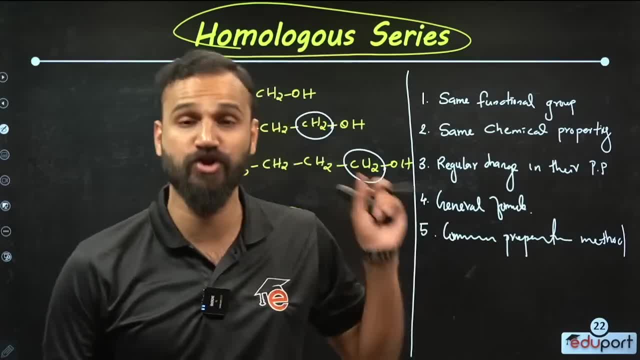 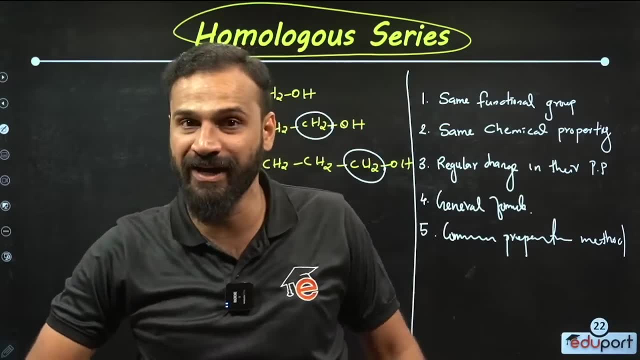 Children. if it is okay, say it quickly, Because each one should be studied and studied. We have studied the unique properties of carbon. We have studied how to represent organic compounds. We have studied the functional group. We have studied the homologous series. 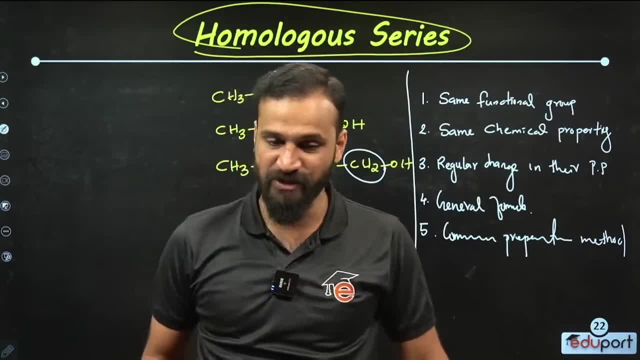 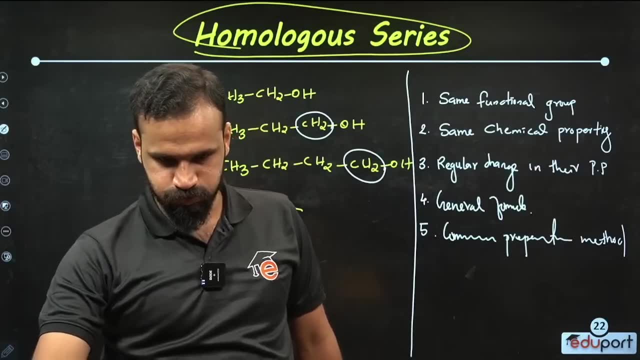 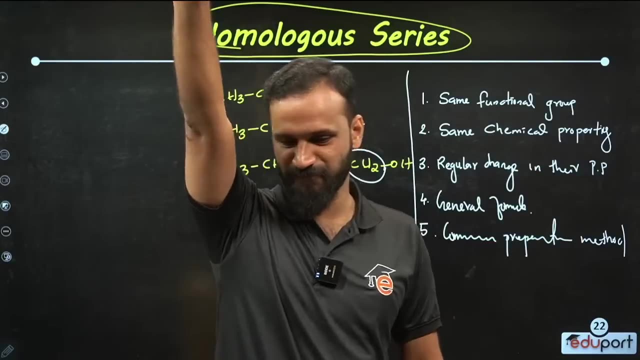 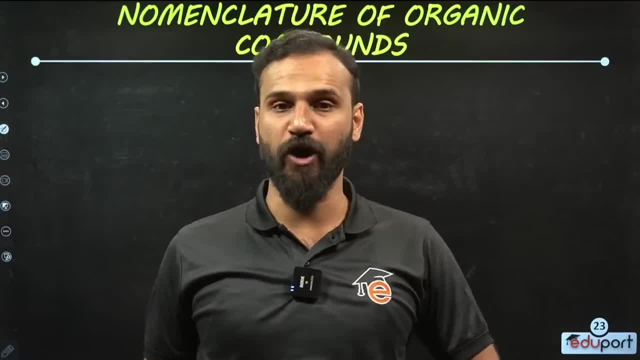 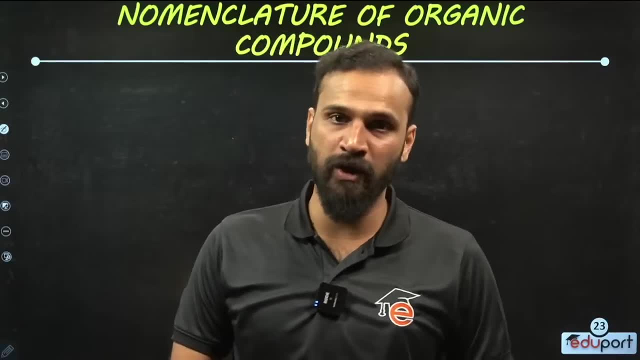 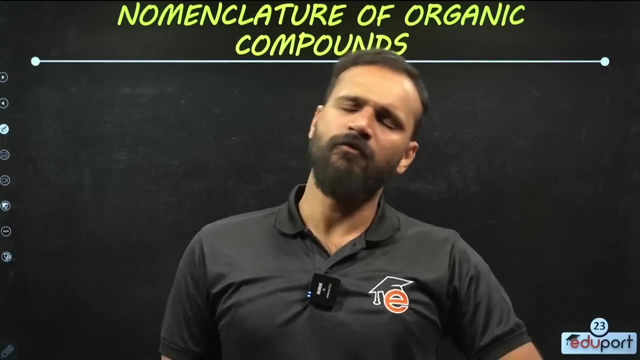 Children. the most important topic in this chapter is nomenclature: How to name an organic compound. This is our question: How to name an organic compound. This is a very important thing. It is very important. There are many rules for this. 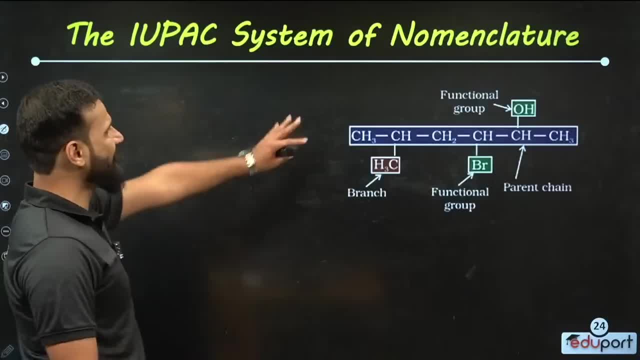 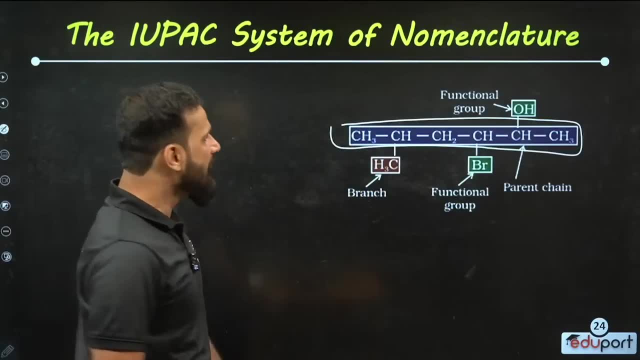 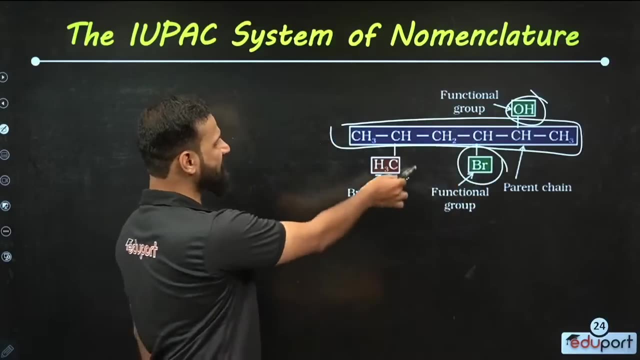 You know that there are rules. Look, if you take an organic compound, there will be a longest chain. No one has any doubt Longest chain. There may be functional groups in it, Functional groups like OHO and BRU. There may be branches like methyl, ethyl and propyl. 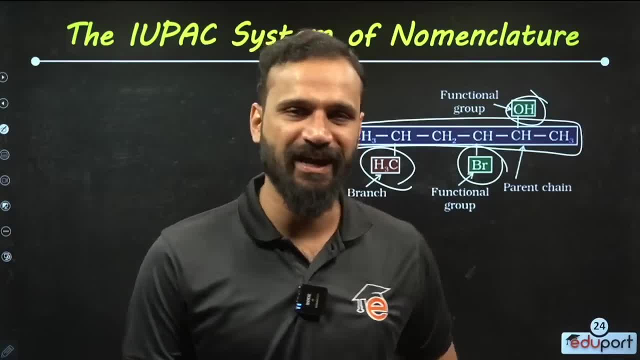 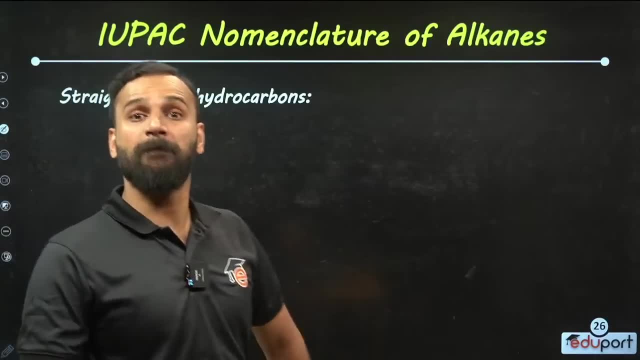 You know that this is nothing new. You know that. Look, children, How to give the name of an alkane. How to give the name of an alkane. That is what we are going to discuss first. Okay, children, How to give the name of an alkane. 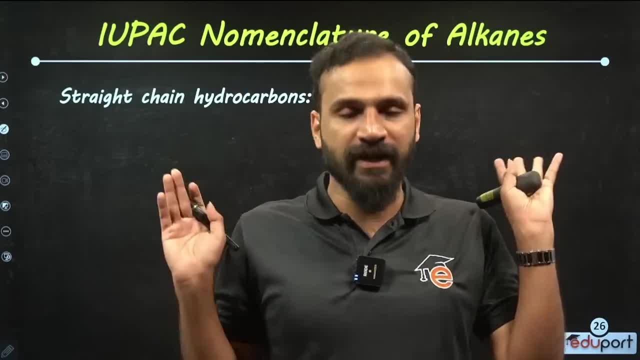 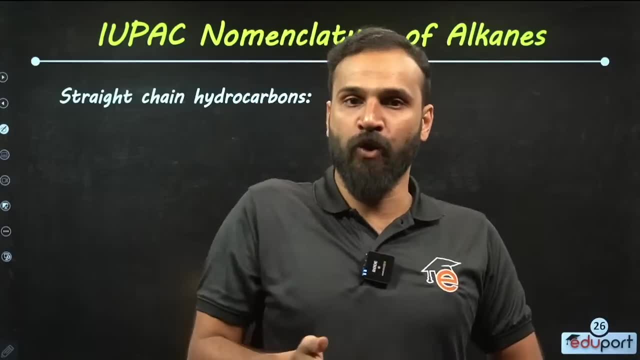 So I'm not just saying that there are some rules like this. I'm giving you a question, You have to try it. Through such an example, we can write and learn together. Look children, Look children. Do you all know? 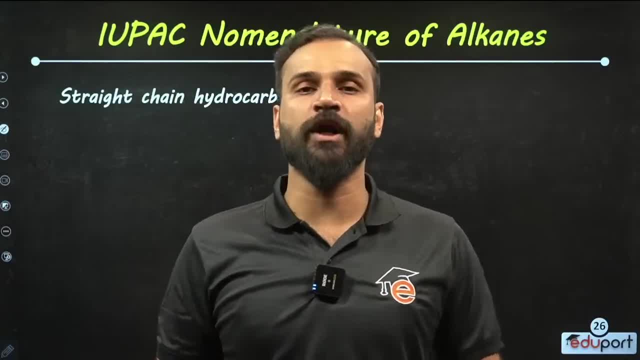 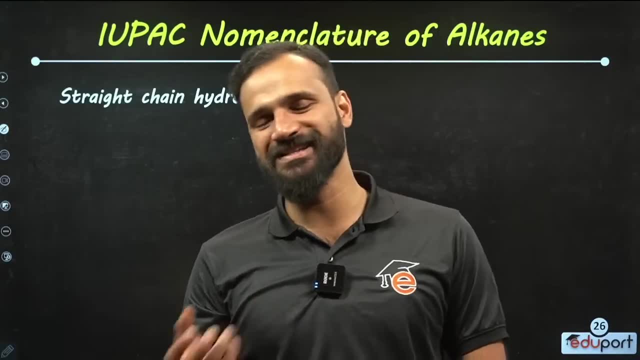 Before naming this alkane, the most basic thing to know is: what is it? Everyone knows this. We have learned this in SLC. We have learned this in Tenth. What is it? It is the root word, If there is one carbon. 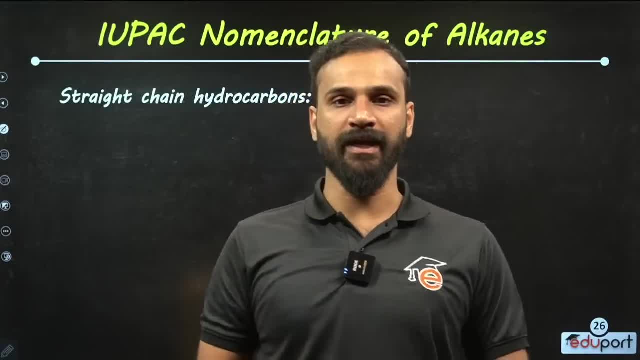 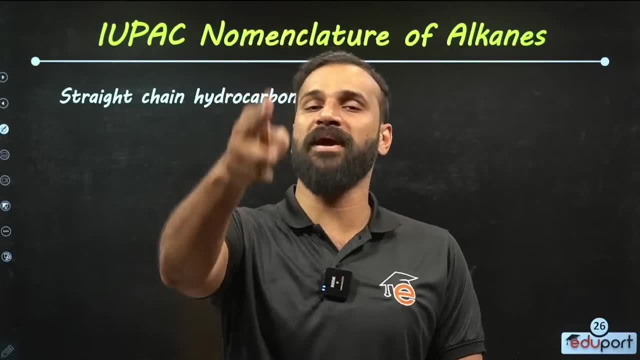 its root word is methyl. If there are two, it is ethyl. If there are three it is propyl Butyl, Pent, Hex, Hept, Oct, Nan, Dec. There are names after dec, But you are only asked up to ten. 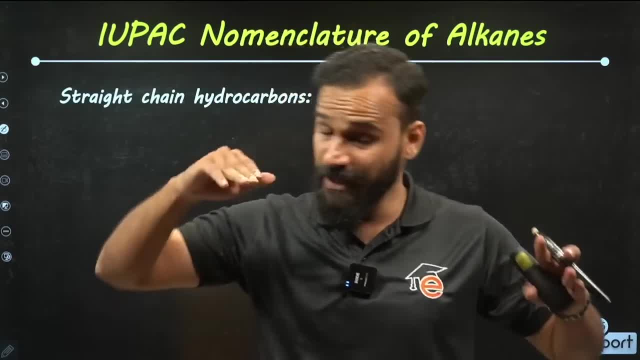 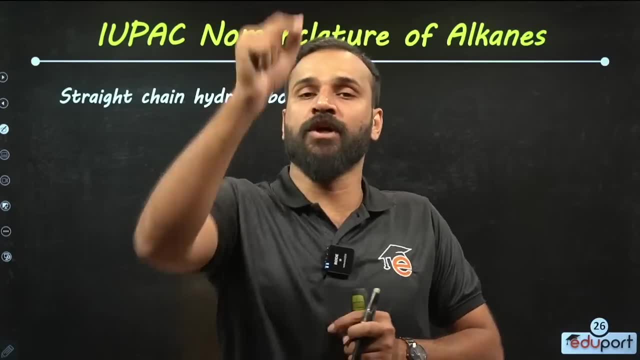 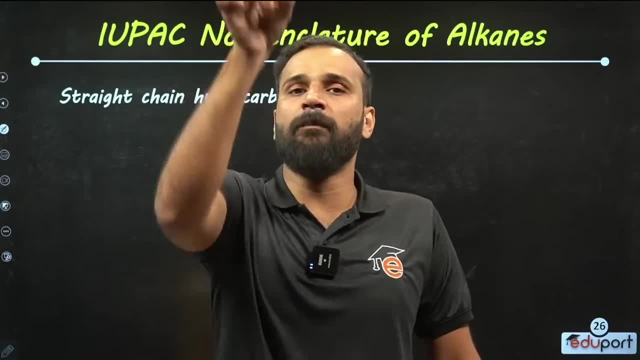 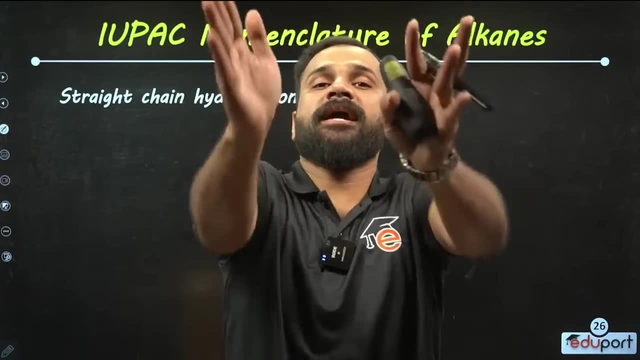 You have to comment here and say it. What do you know? I know from one to ten: Meth Eth, Prop, Butyl, Pent, Hex, Hept Oct, Nan, Dec. You have to comment that you know up to dec. 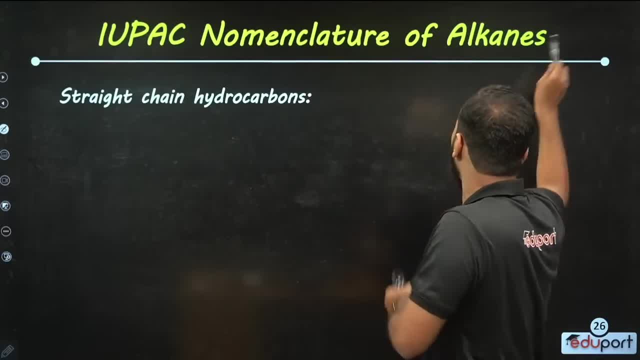 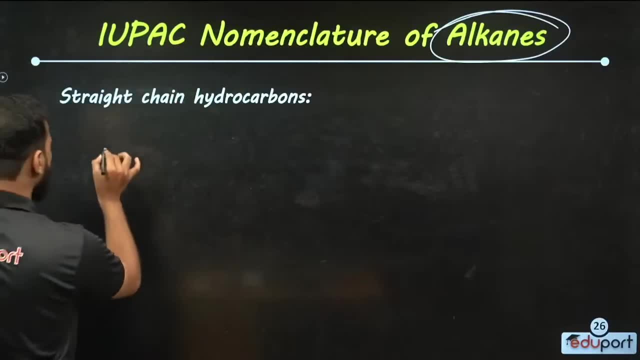 Because if you don't know that, it is a problem. If you know that you can name anyone with alkane, I am sure that everyone knows that We will come to the name. Look, children, Let one car go, Methane. 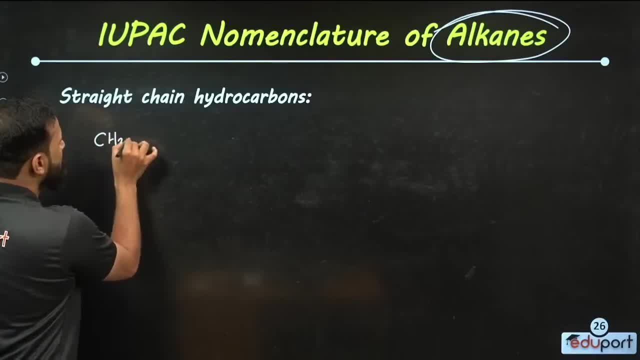 Let it go: Two cars, Two cars And one carbon, Two carbon, Two carbon From CH3 to CH3.. What is this? Do you know just what this means? There are three carbon. There are three carbon And CH3,. 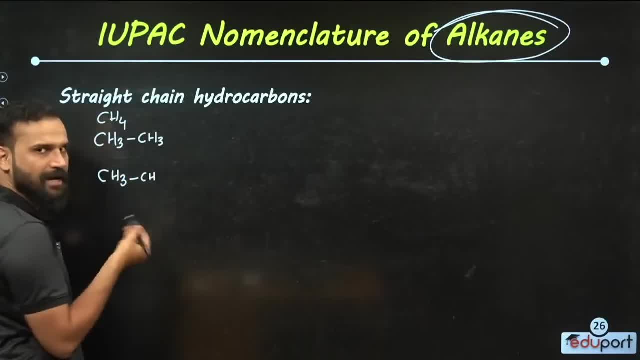 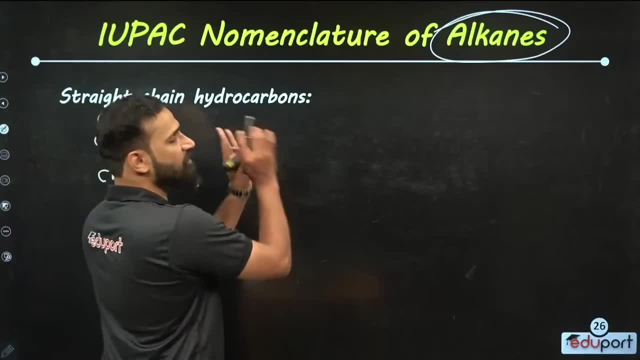 one carbon says CH4.. One carbon says CH5.. And know that this also, Even if it is three: CH3, CH2, CH3,. What is it? Propane. That is the root word. we wrote For the root word. 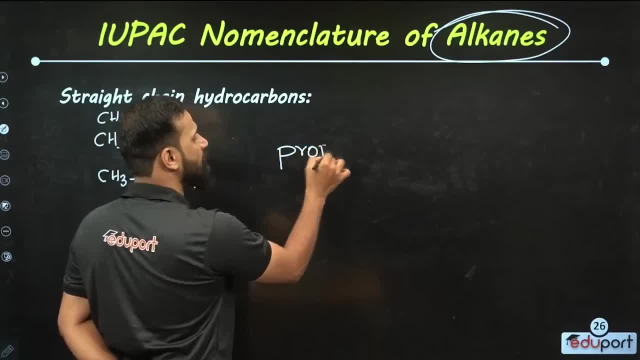 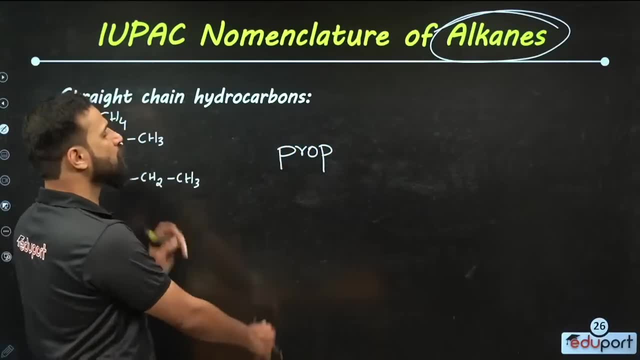 if it is a prop, it will be prop. If it is only three, it is prop. All are single bonds. We are ig47, kar, we are. We don't have to say exactly because we take alkane. If everything is a single bond, add A-N-E. 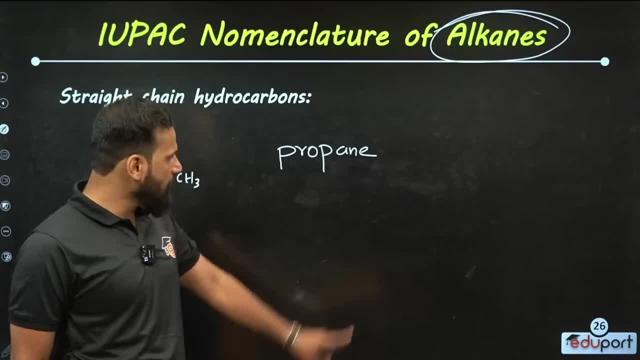 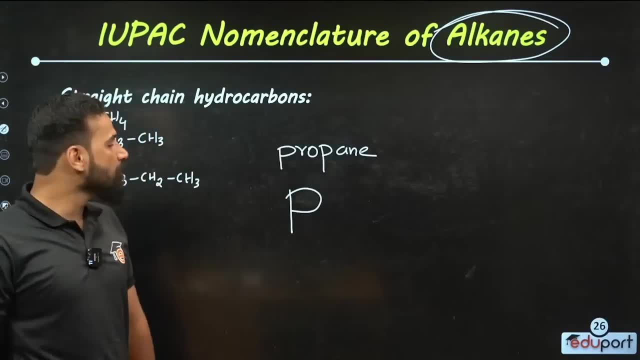 Isn't it? So the name of it is propane, Isn't it? When you write, you have to pay attention. If you want, Only the first letter can be written in the capital letter. The rest of the letters should not be capitalized. Then 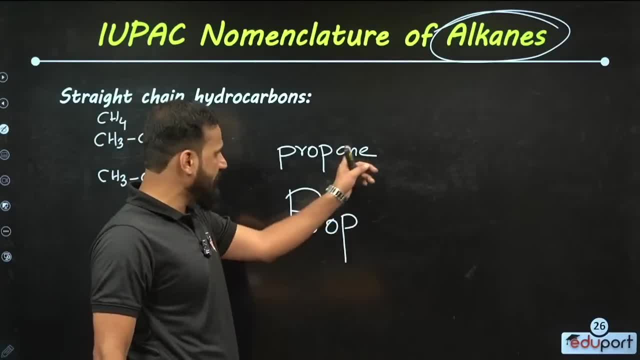 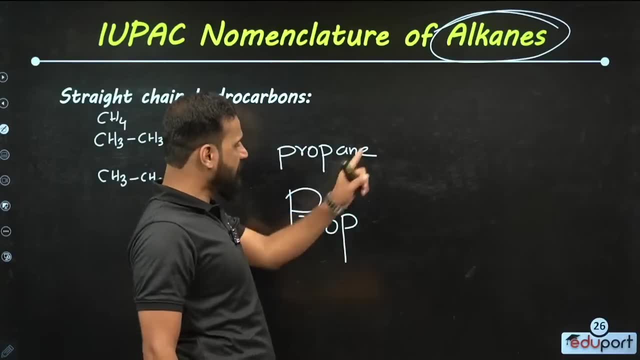 Wrote prop After the prop. when you write A-N-E, Isn't the first letter of it A? It should not be capitalized. It should be a small letter. Now there is no space between the prop and A-N. Is there a part? Then it is propane. This is how it is said. 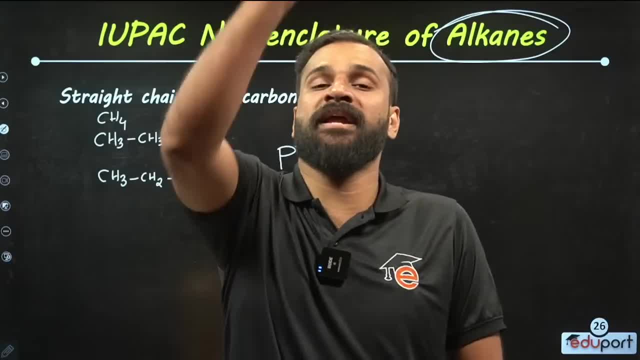 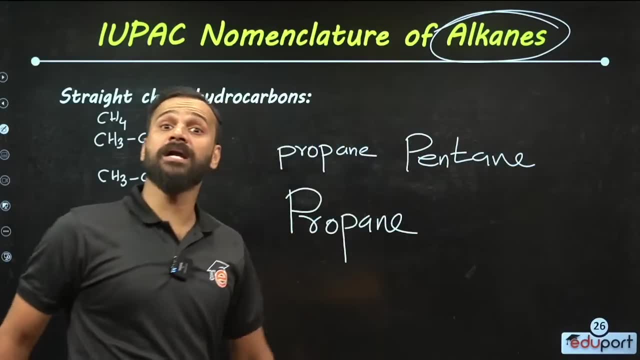 This is how the name is said. Now, if there is five carbons, PEND. If there are five carbons, the root word is PEND. If everything is a single bond, PENDANE If it is six. HEXANE. 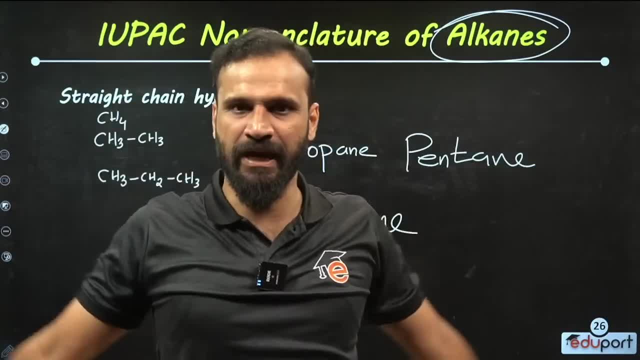 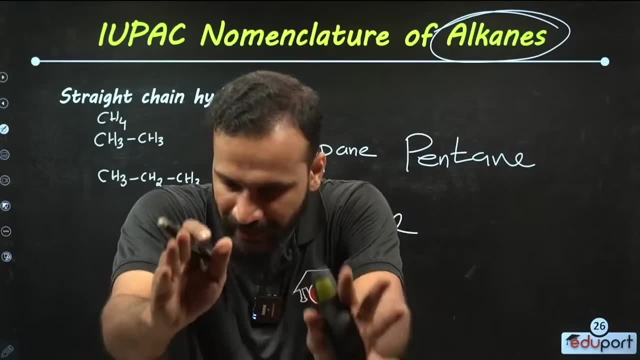 If it is seven HEPTANE, If it is eight OCTANE, If it is nine, NONANE, Isn't it? If it is ten DECANE? We know This is not a new thing. I know that everyone knows. What do you know now? 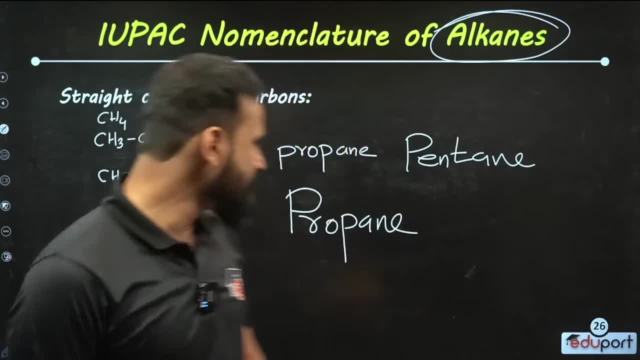 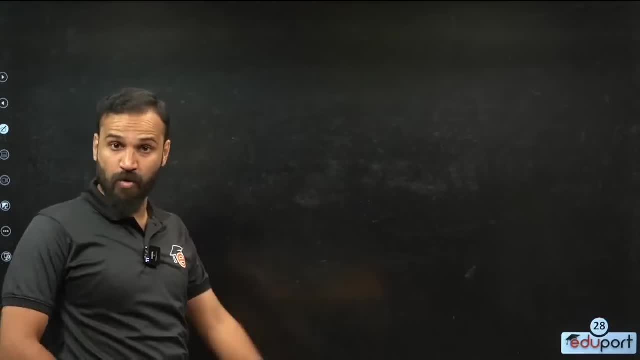 When the branch comes, our game will change. Let's go to that. Look, we don't have to say meth, meth, prop butane, PEND here. We know everything. Now, look, children, I'm going to the branch. 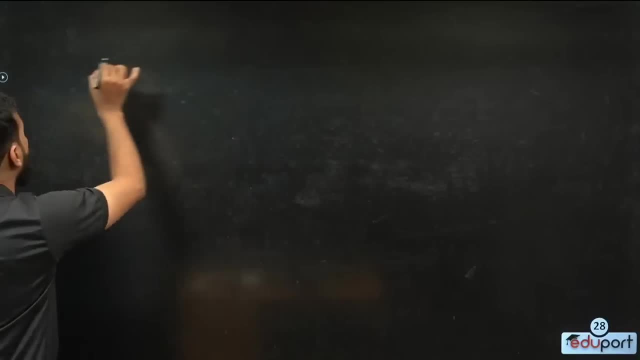 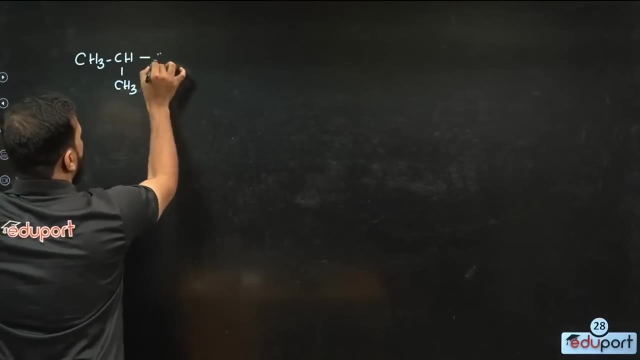 Let's go to the branch. Look, you have to tell me, Look, let's do it. CH3, CH, CH3. Children, this is a compound. What is it? Aren't you going to tell me that you know nothing? But some things are virtual, some things are real. 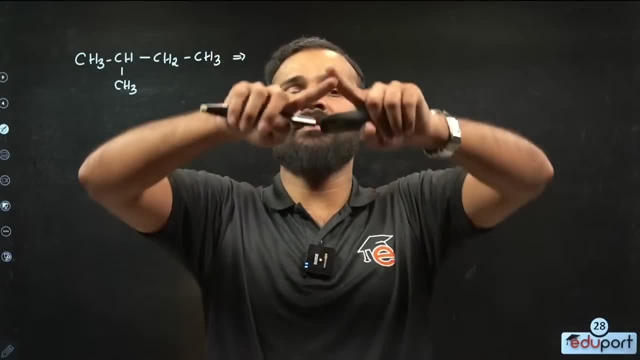 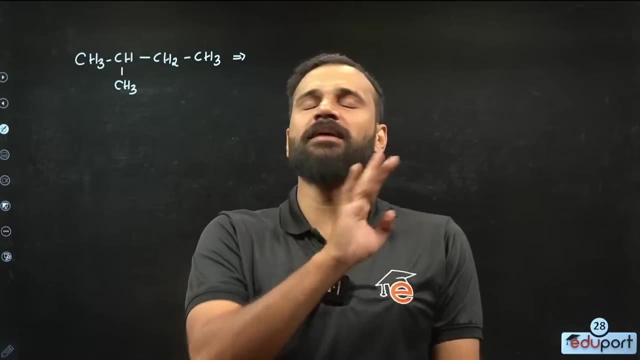 y'all. we have nothing bad in the world right now. Why do we have the thing? The thing you are vulnerable to is material, material with little further limitations. It's nothing like a hand. It's something strong enough. Give me, give me, Never say what I'm saying. 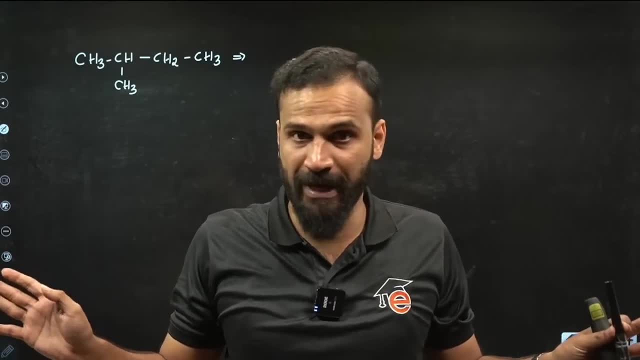 For a long time in a world where you don't have a dealer. It's meant to come in front of you. No abrasive, You bought a reward. in These days where you can come in front of creativemoney? Yes, of course. 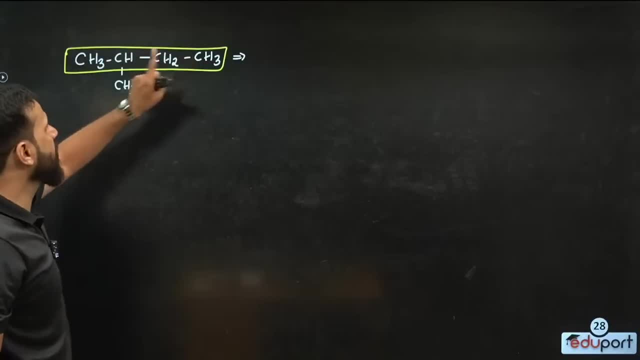 Then you can look for it everywhere. If you see these songs, you must take them. no one cares. One, two, three, four carbon, Isn't it? Now, if one, two, three come down here, is four carbon, isn't it? So, no matter how you look at it, 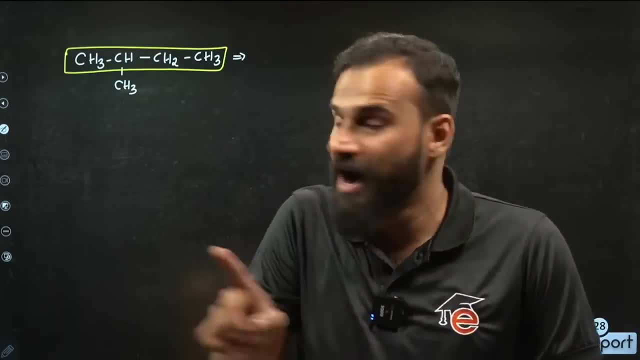 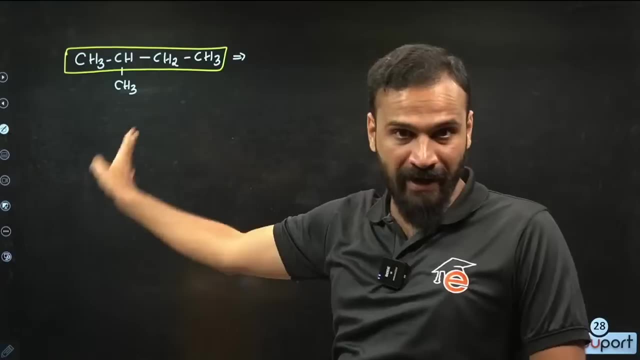 a chain with four more. carbon is not obtained from this, So the longest chain is the same. Now, even if you take it down, it is four. OK, Now look, you can do left to right number, you can turn it over and number. 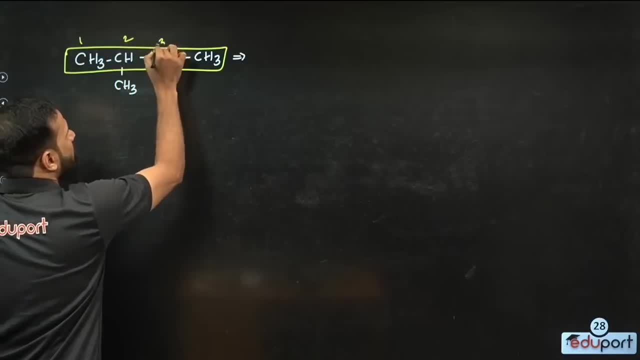 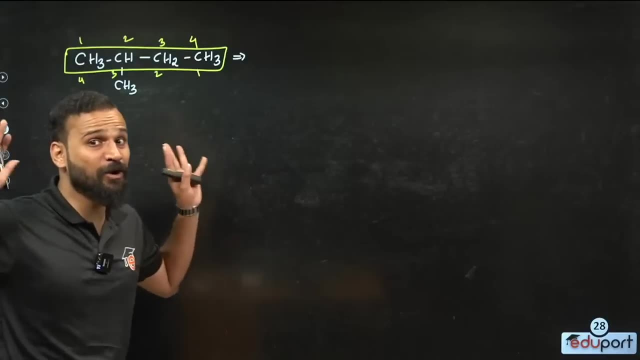 OK, isn't it? Look at the number One, two, three, four. Turn it over. and number One, two, three, four. This is said to get something that no one knows. I know that you have always told me the name. 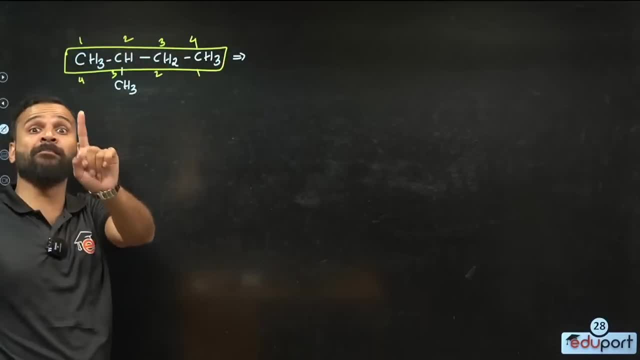 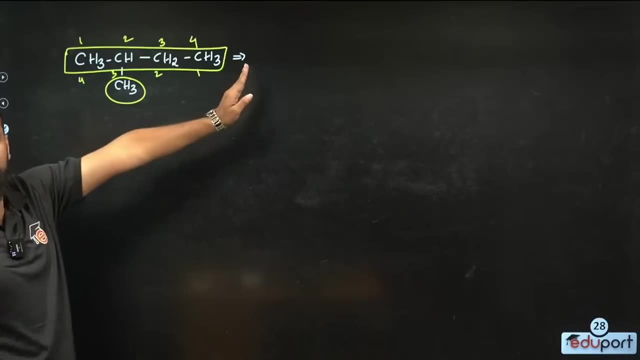 Look when you number, from where to where the least number of this branch here is obtained: Left to right number. So the branch is in the second position in the meta. This is a different number. The number is in three. So which one do you have to? 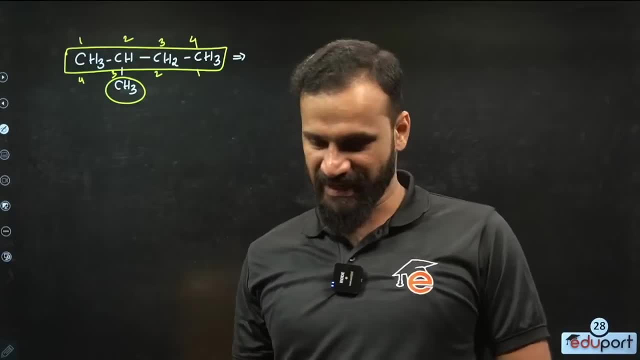 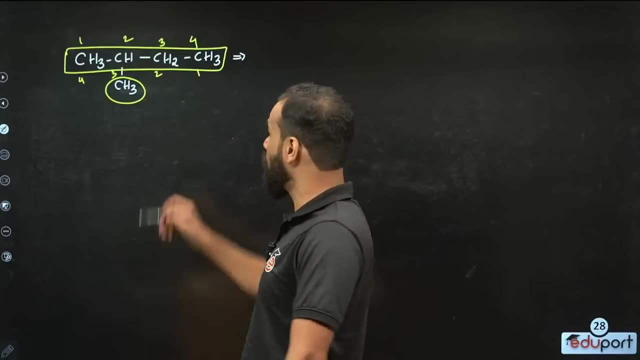 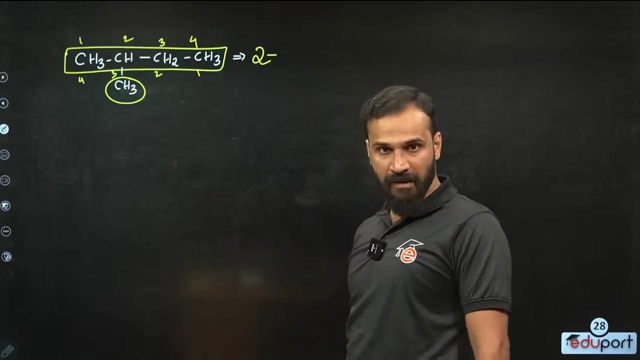 select The least number to be selected. Even the branch should get the least. So left to right select. So ask the children. first branch is to be said In the second position in the meta. So put two. If you put a number, hyphen is mandatory. OK If the name is in between. 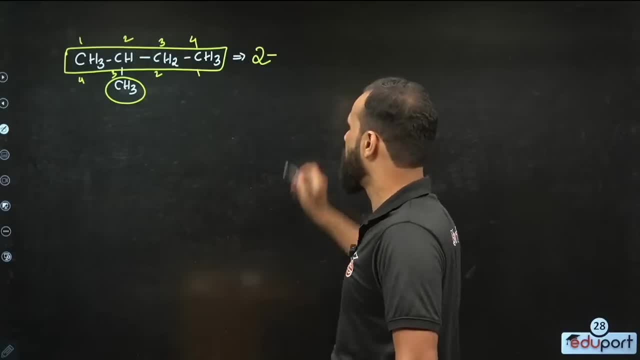 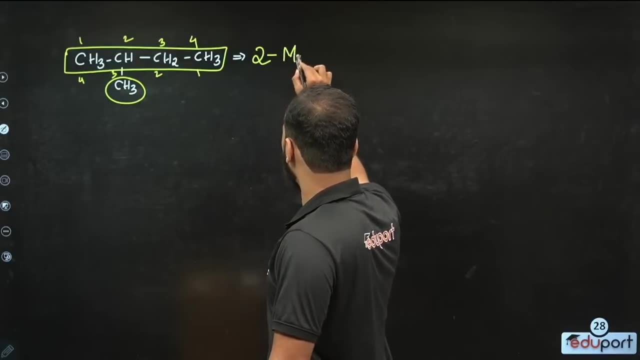 the number should be hyphen before putting it. Let's do an example, So two. In the second position, which branch is meth? There is only one carbon, One card, first letter capitalized. What is meth? Meth is not a root word, It is not the longest chain. 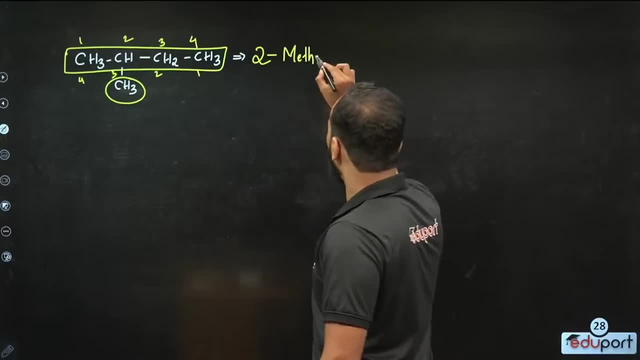 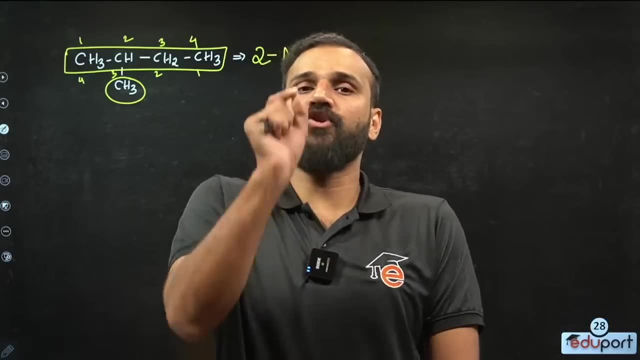 Then where is the branch? Since it is a branch, it should be added to a Y. So his name is methyl. What is it, children? Methyl? So two methyl. What is it, children? Two methyl. Now, take the longest. 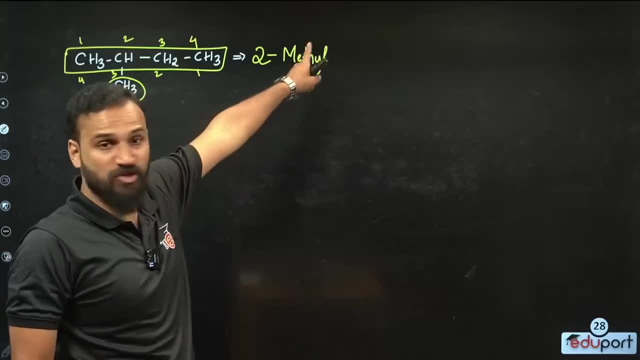 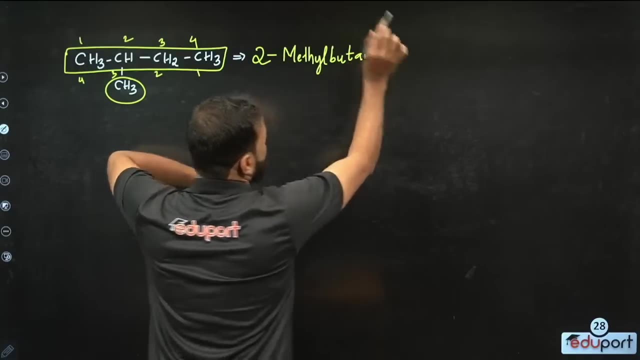 chain. The longest chain is four carbon right. So is there a space bar in butyl? No, This is called butyl in small letters, Butyl, OK, All of you. thereu is no single bond, So write it as any. So what is the name? 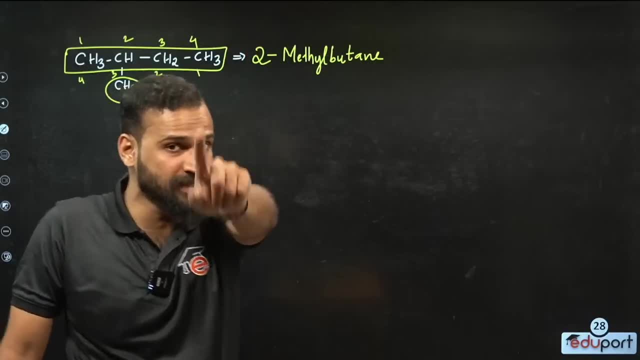 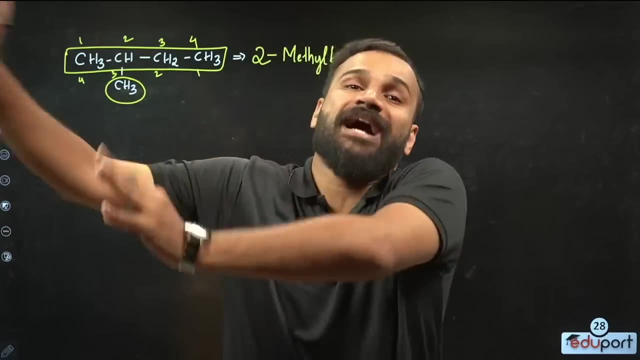 Two methyl. Now, sooner or later, I'll tell you the compound. You have to tell me this way and come. Yes, two beutäin. What is the name of the compound? children, Bethyl betane, Say the name. Say them Two methyl butane diye. 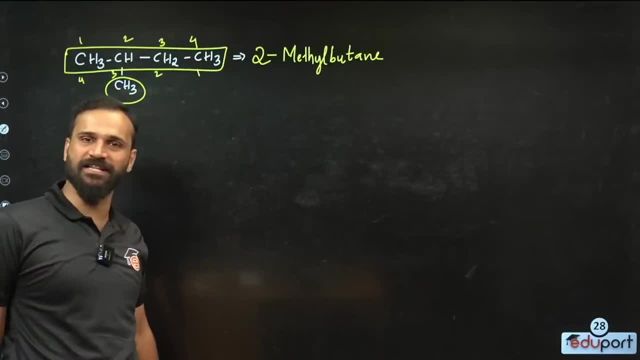 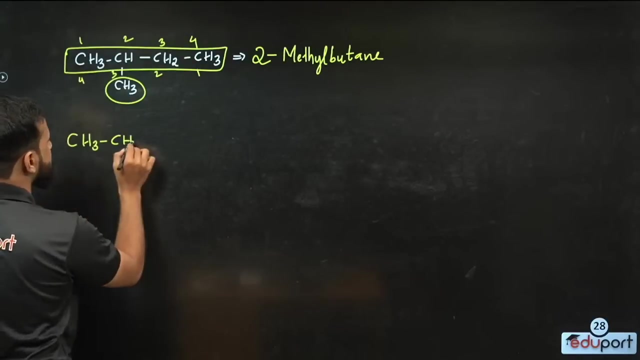 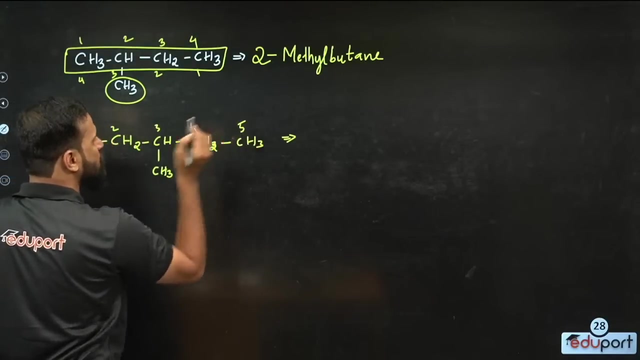 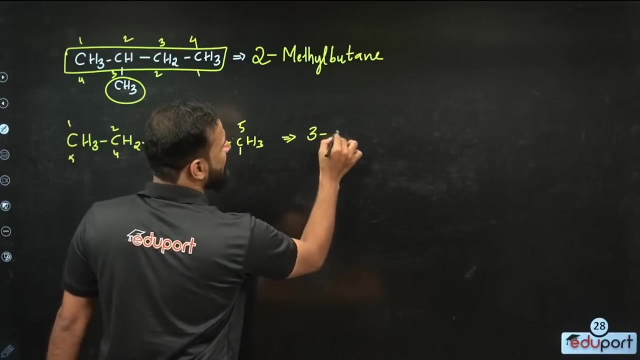 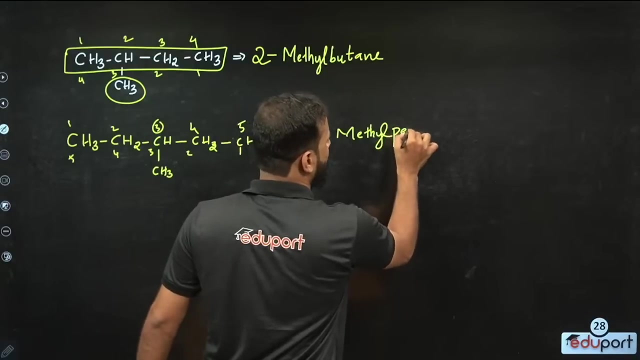 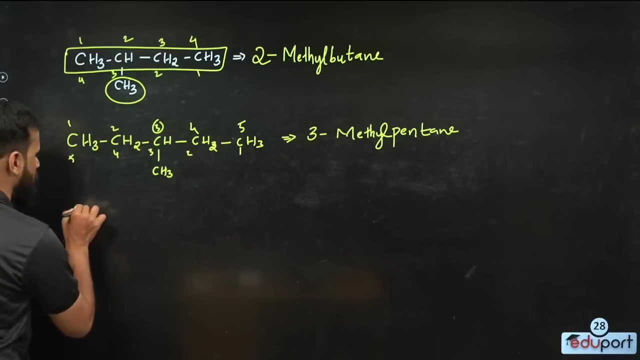 Jean. yesss, phidife, Let's see the next one: CH3CH2CH3CH3, CH2CH3, CH3CH3CH3. If everything is a single bond, it is PENDEIN. Do the next one yourself. 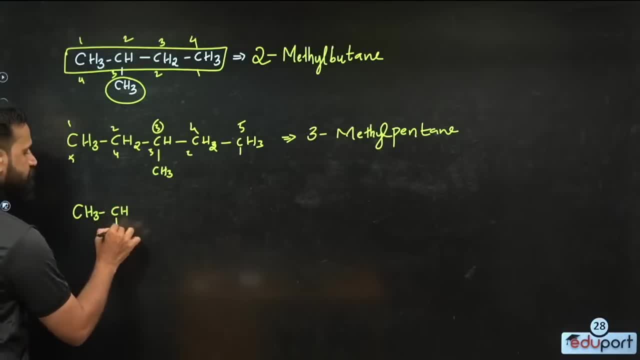 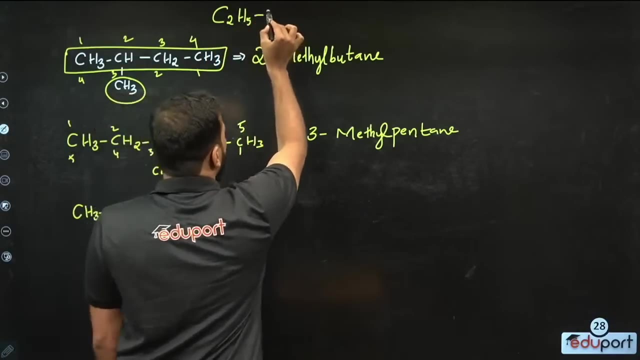 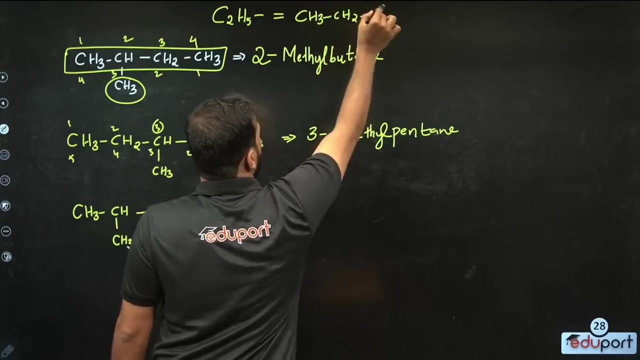 CH3, CH2, CH3, CH2, CH5. Who CH2? You have to learn it. Who is CH2, CH5? Note it down: CH2, CH5. In other words, CH3, single bond, CH2 group is written in short: 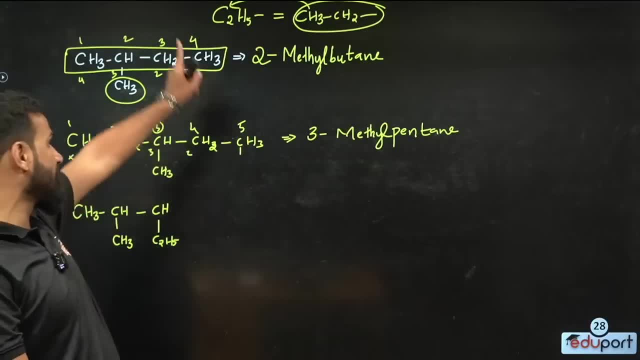 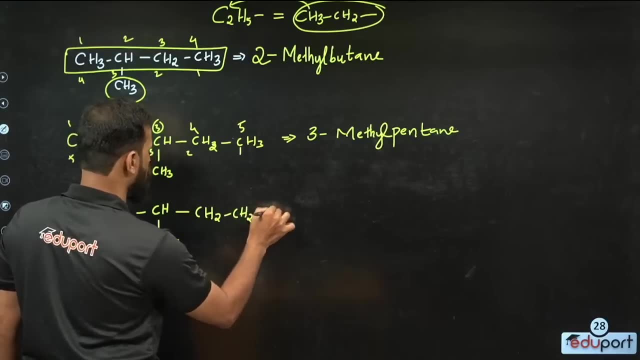 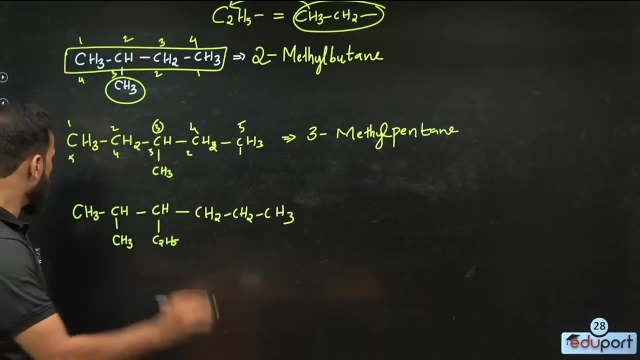 CH2- CH5. It is written in short: Do you remember CH2- CH5? Yes, CH2, CH2- CH3. Is it ok? The first step is to find the longest chain. There is no doubt, Here we are. The longest chain is in this box. 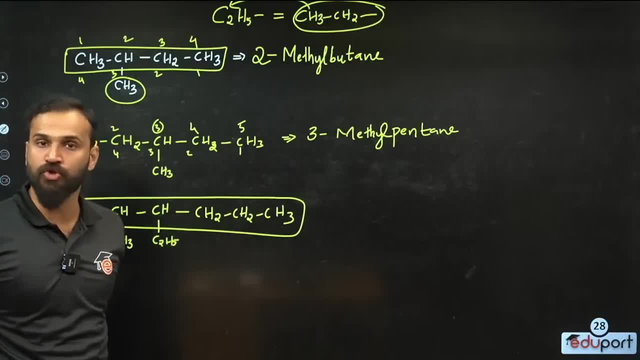 Now there is a question of where to do the number. You can do the number on both sides, But when you do the number from left to right you get the least number for both the branches. Those who are doubtful should do it. 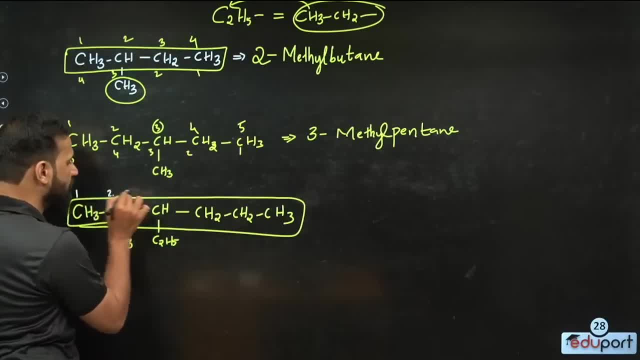 Those who are doubtful should do it. So you have to do the number: 1, 2, 3, 4, 5, 6. It is like this: It is from here to there. When you do the number like that, you will get the least number. 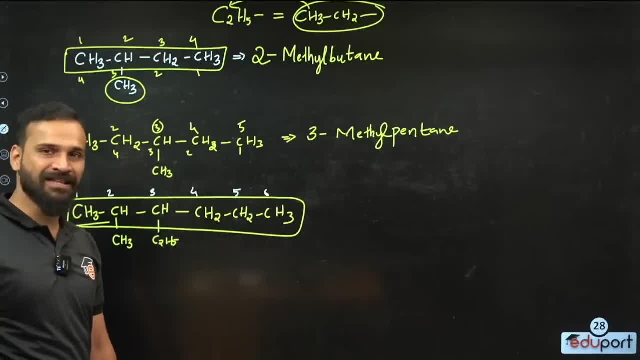 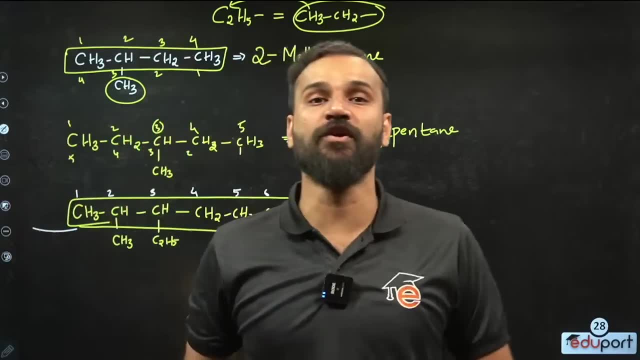 You will get the least number. There is no doubt There is another problem. Do you know what it is? These two different branches have come here. When such different branches come, which branch do we have to calculate? We have to look at the alphabetic order there. 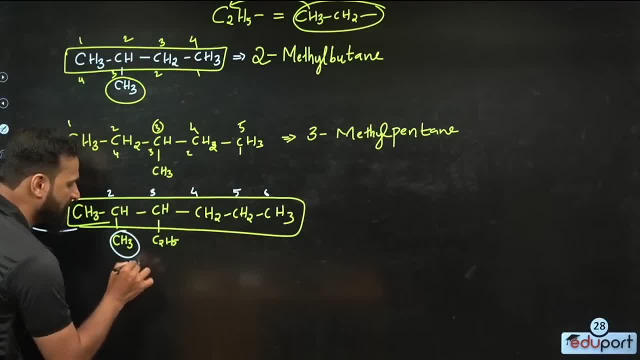 Look, Who is this? Who is this, children? This is a methane right. There is only one carbon right. Then we can call it a methyl group. Here, children, there are two carbonato oils. We can call this ethyl. 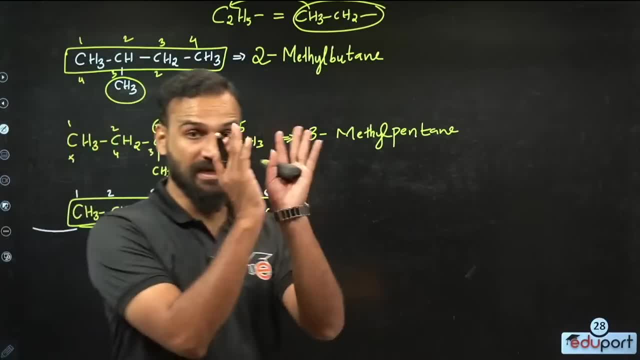 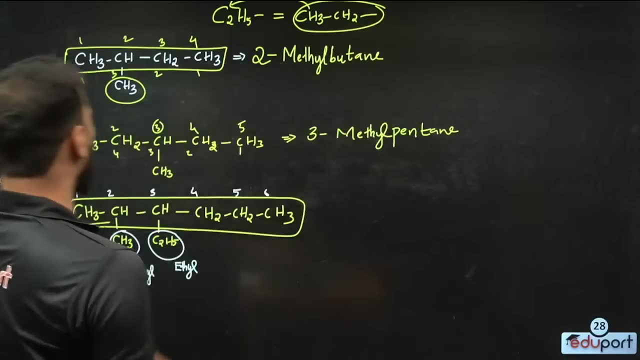 What can we call it, children? Ethyl. So there is methyl. What is it? Methyl is there. Ethyl is there. Methyl is there, Ethyl is there. So you say, Is M the first in the alphabetic order. 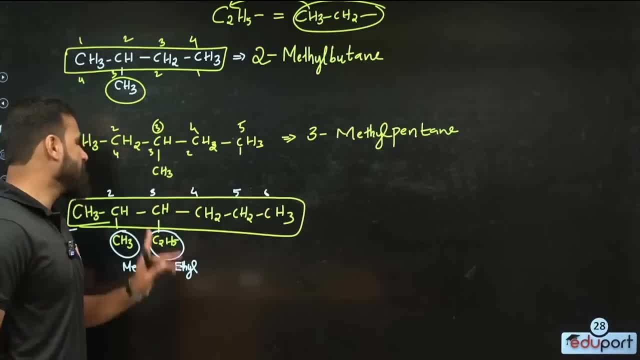 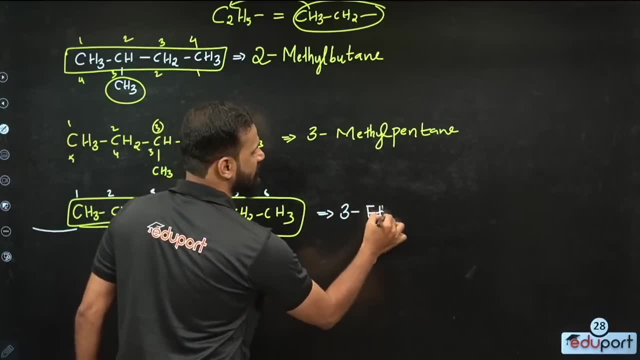 Is it E? There is no doubt E. So E has to be said first. So you say: Where is E In three? So three ethyl, Three ethyl. Put a line, Put an iPhone, And then, And then. 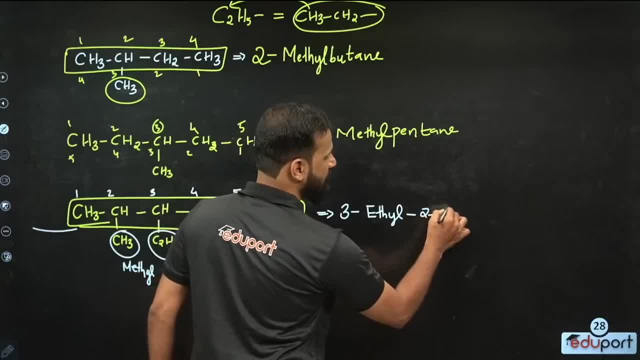 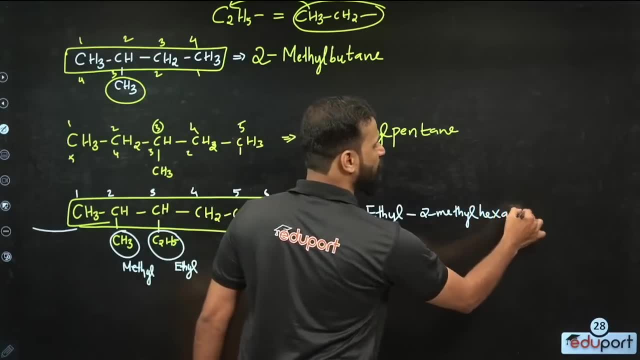 And then In two methyl Methyl in two Methyl in two Methyl in two Methyl, 6 carbon atoms in the longest chain. The root word is hex. Because everything is single-bond, they are called any. 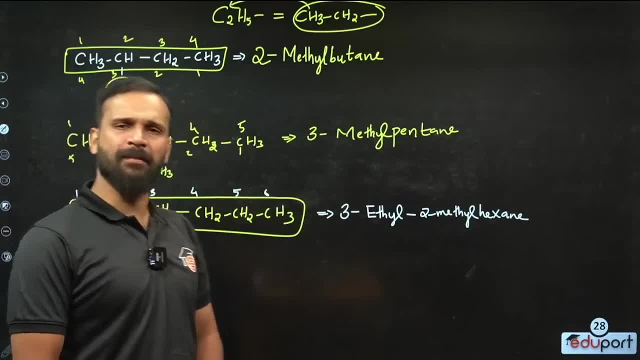 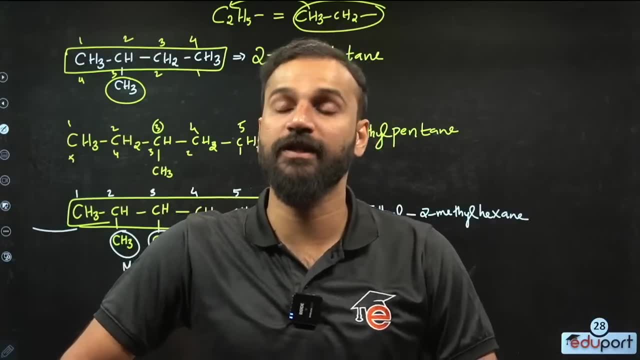 Isn't it children? Isn't it people? So what do you understand? You have to consider the longest chain, That is the parent chain. Right, That's what the parent chain says. Now, if there is a branch in the form of the least number of that branch, 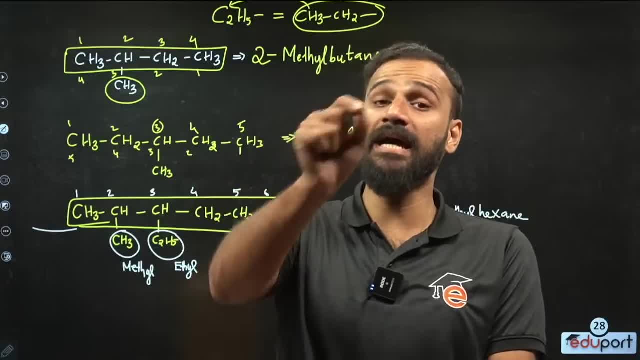 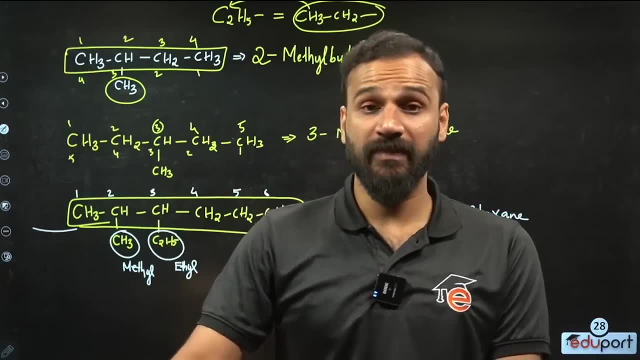 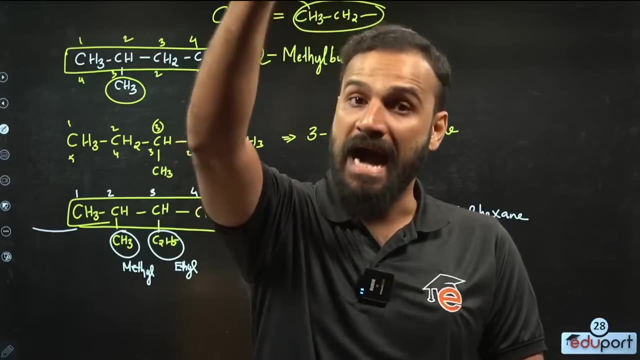 give the name, name it. That branch should be named in the form of the least number. Okay, Then what did we say? If there are two different branches, which branch is the first in the alphabet? He is the first to say. 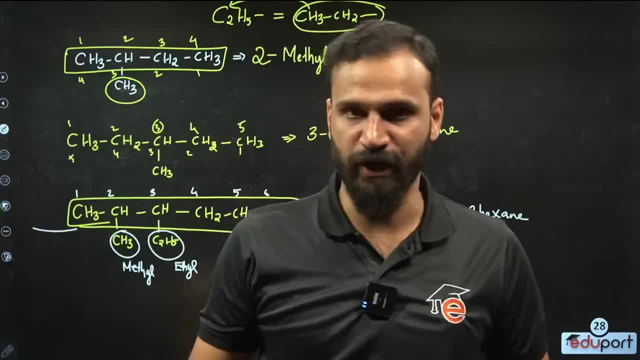 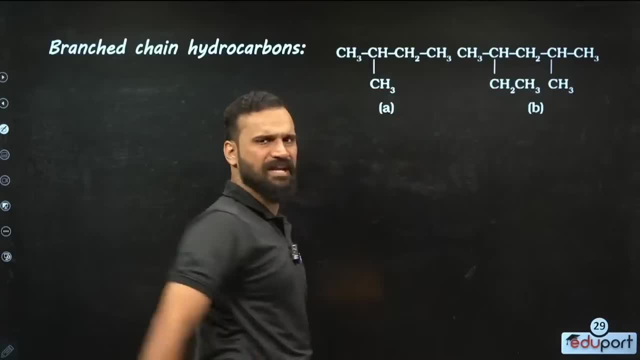 Then the next person has to say: Pay attention, See Now, look at the children. What is said here? Nothing. The number is said. I will give another question. I will give another question. Try to do it now. CH3. 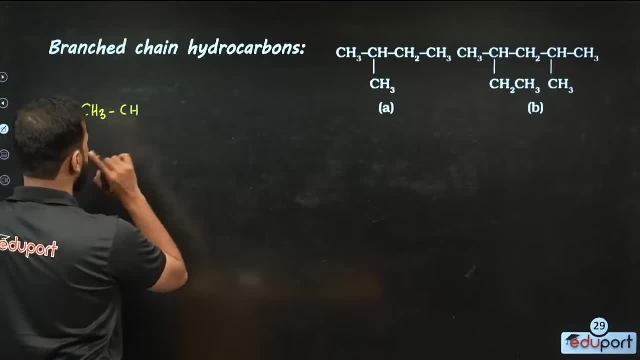 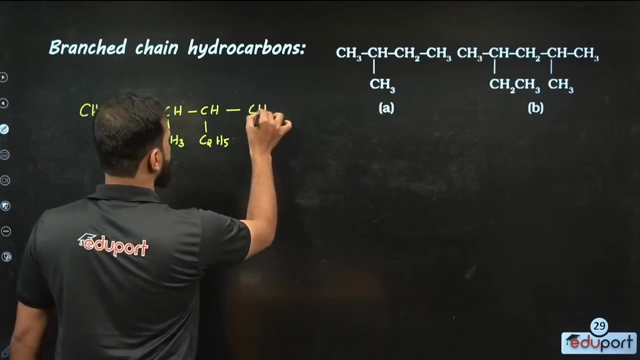 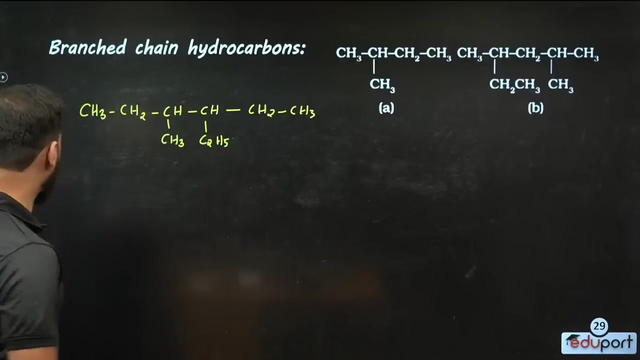 What is it, children? CH3, CH2, CH, CH3, CH, C2, H5, C2, H5. I have to remember this, children, What is next? CH2, CH3- This is how it is given. So, everyone, If you say to take the longest chain, there is no doubt this is the longest chain. 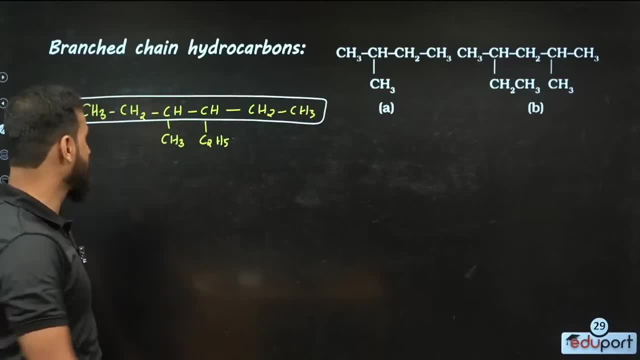 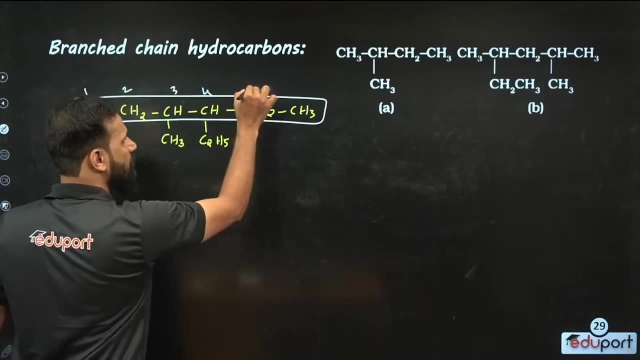 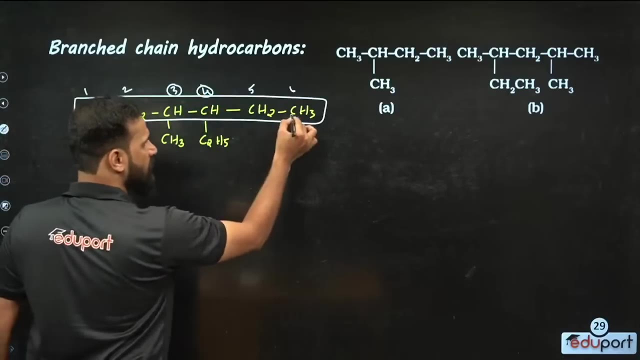 Let's see how to get the least number of these two branches: One, two, three, four, five, six. When you do this, there are branches in three and four If you number it: one, two, three, four, five, six. 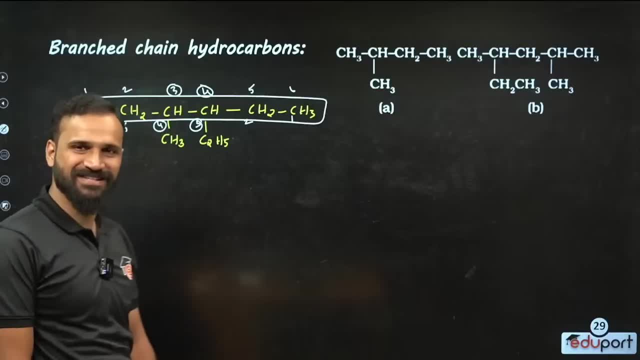 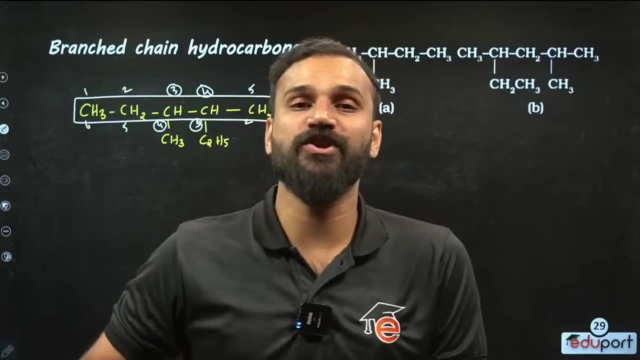 Still in three and four. There are branches in three and four. Even if you number left to right, even if you number right to left, the branches come in the same position, Isn't that so? If that's the case, which one do you have to select? 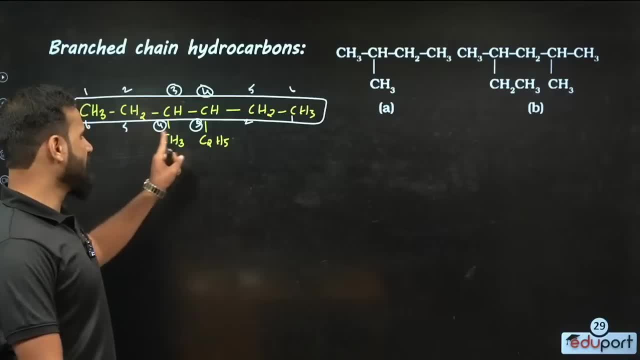 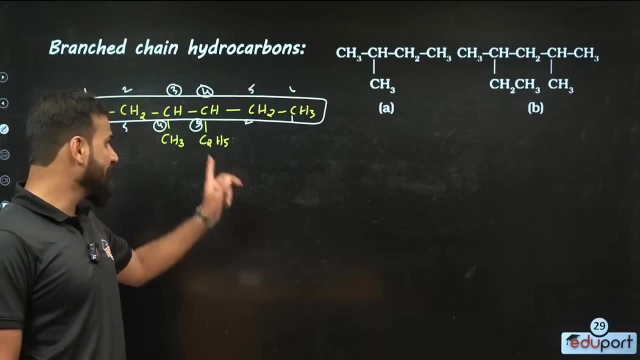 So you have to look at one more thing. What Are those two branches the same? Is it the same? No, If that's the case, which branch is the first in the alphabet? It is in this, If you get the least number in this. 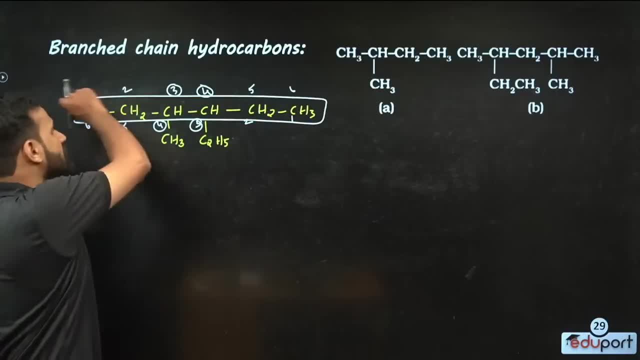 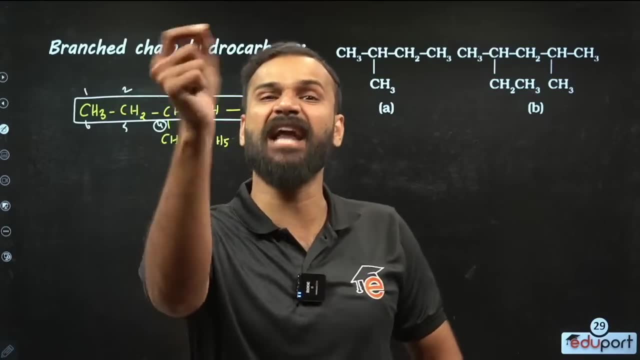 when you number from here to there or when you number back. when you number from here to there, Ethyl is in the fourth position. When you number back, Ethyl is in the third position. If that's the case, who should be given the least number? 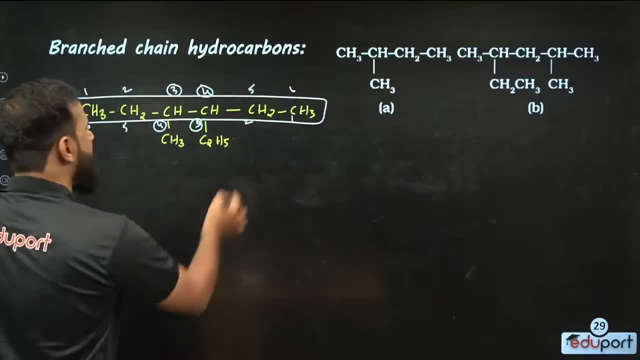 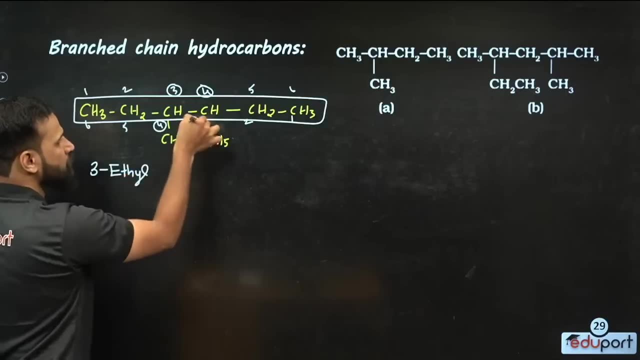 It should be given to the person who comes first in the alphabetic order, So we have to select the number from there to here. What should the name be? Three Ethyl, Three Ethyl. There is Ethyl in three. Then what girls? Four Methyl. 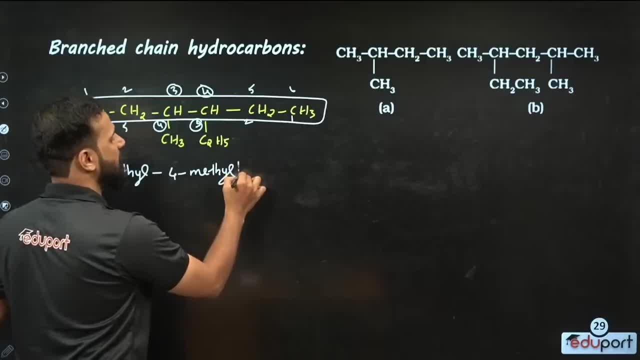 Four Methyl, Now girls, since the longest chain is six carbonates. if it is six, it is Hex, right, If it is six, it is Hex. If it is six, what should we say? Hex, Since everything in the longest chain is single bond. 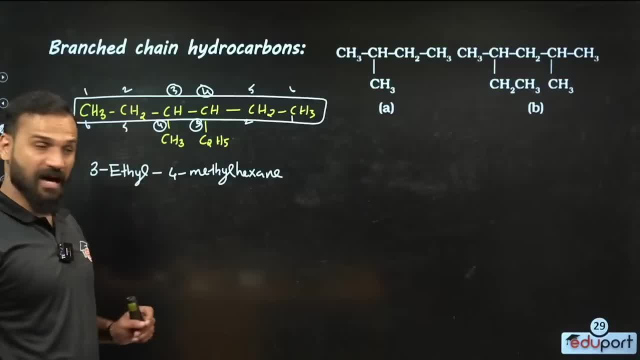 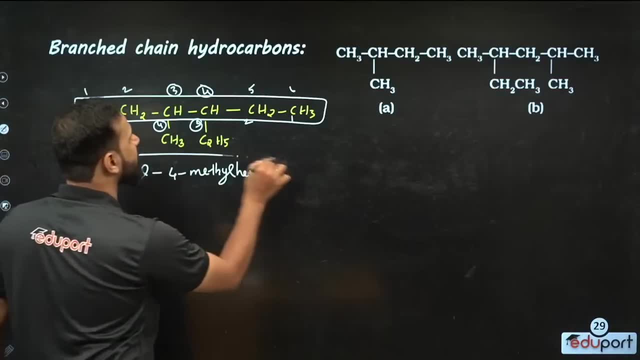 Any. So what girls? Three Ethyl, Four Methyl Hexene. I am teaching you each thing through each example, So you have to understand it properly. So you have to look at the least sum. You have to look at the alphabetic order. 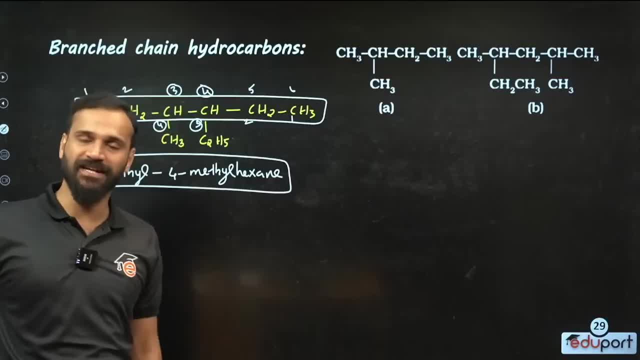 Both sides are in the same position. If you get the position in the alkyl loop, if you get the position in the alkyl branches, you have to select it in the form of the first person to get the least, in the alphabetic order. 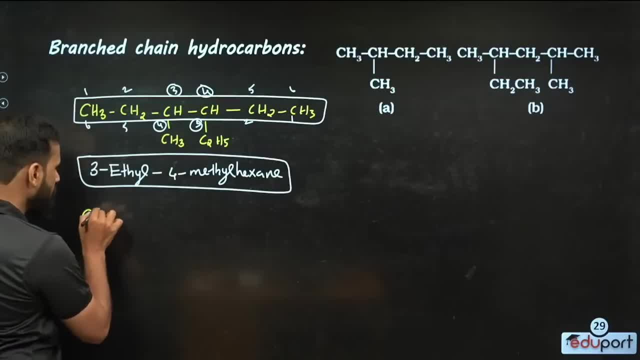 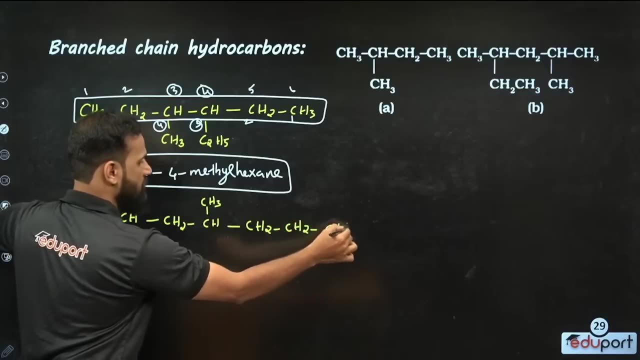 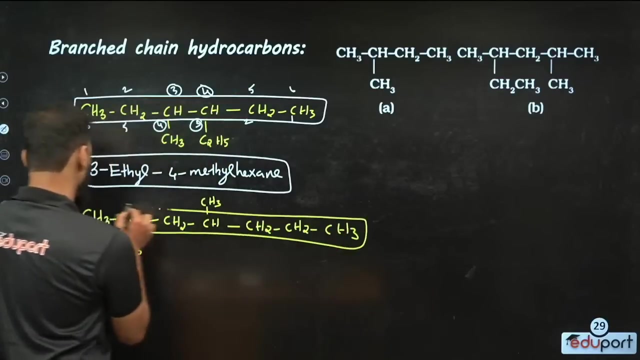 Now, girls, let me tell you another point. Look, CH3, CH, CH3, CH2, CH, CH3. Single bond, CH2, CH2, CH3. Okay right, First of all, we have to do the longest chain. No doubt This is the longest chain. 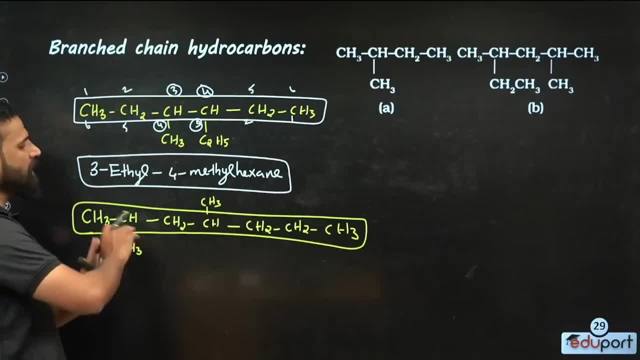 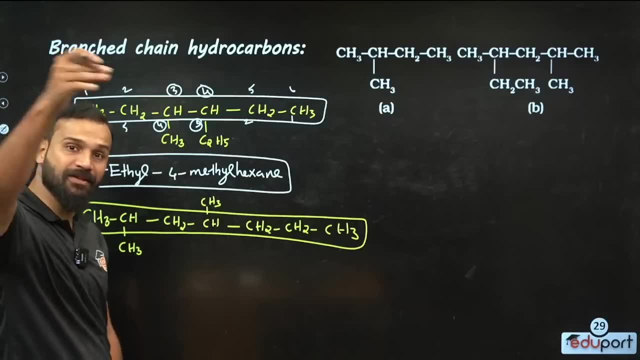 This is called the longest chain From where to where these branches get a small number. There is no doubt. You can see it yourself. If you don't know, after seeing it, you can do it and see it When you do the left to right number. 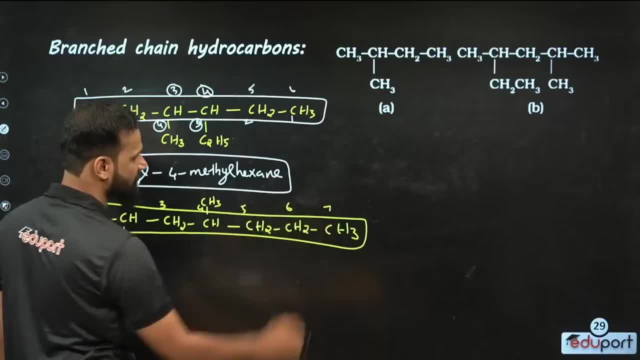 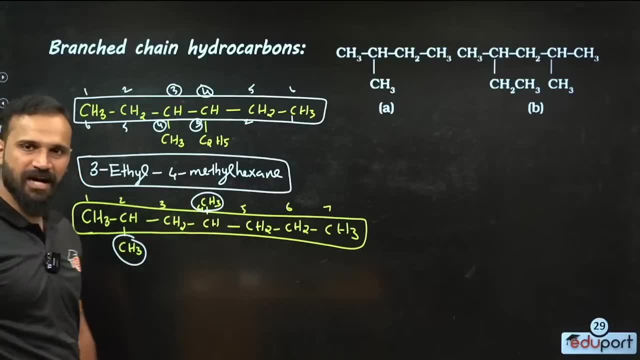 you get the least number: Three, four, five, six, seven. It comes like this, right. But I understand that you will have noticed one thing here: What are these two branches? They are the same branches. What are these two branches? 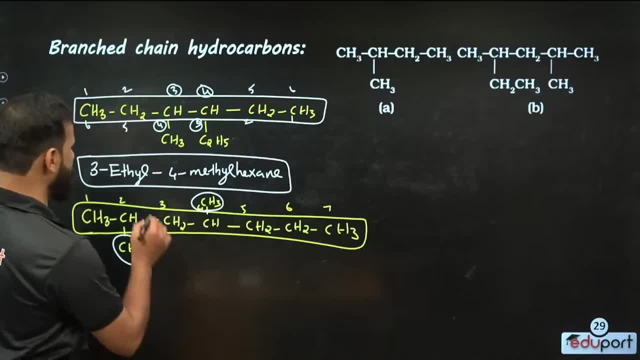 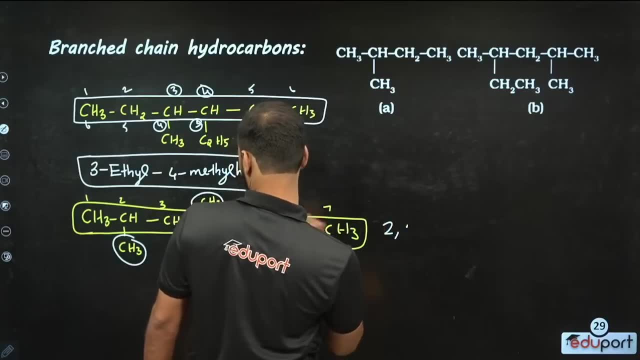 They are the same branches. So what do we do? Look, There are four branches in both. So two comma four. No, not four in both. Yes, two comma four. Two and four are the same. Who is four in both? 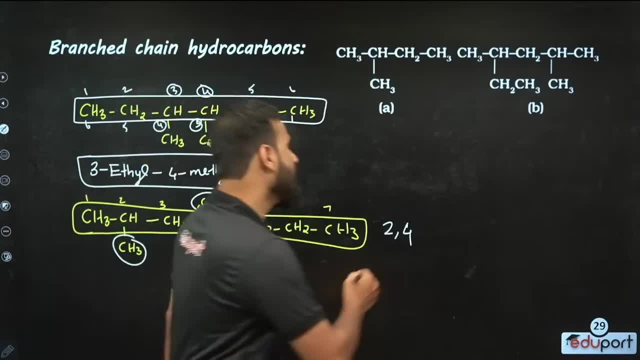 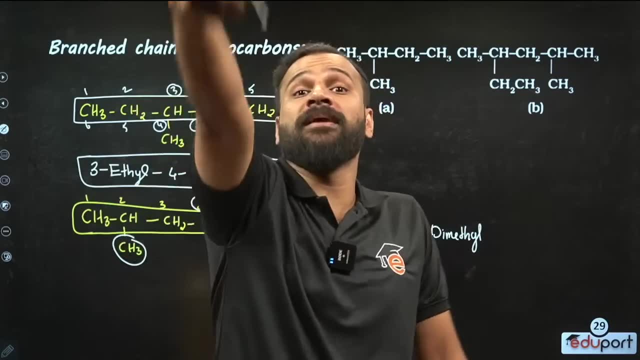 Methyl, How much methyl is there? Two methyl, So we have to write dimethyl. Dimethyl, Is it three or three? Ten, Trimethyl, If it is four, tetramethyl, If it is five, pentamethyl. 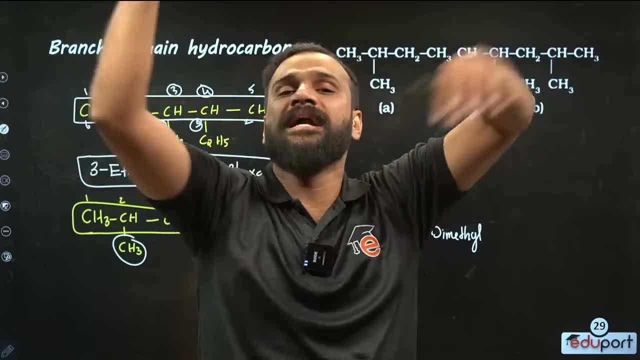 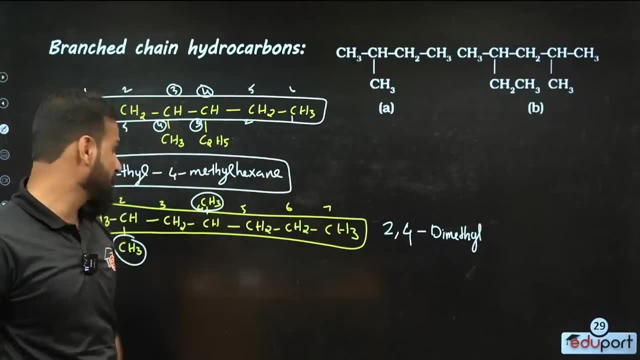 We have to write like that. If the branches are all the same, we can represent it by using di, tri, tetra. Look, So there is methyl in both and four. So two comma four dimethyl. The longest chain is seven carbon. 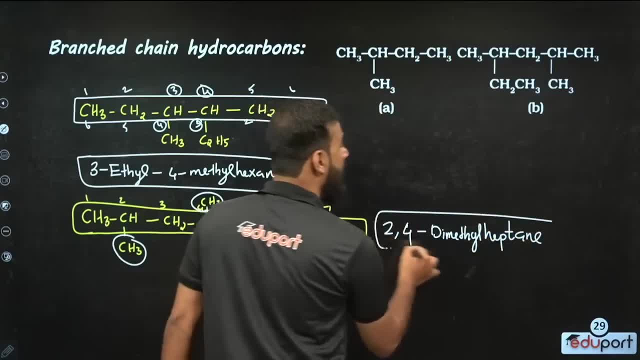 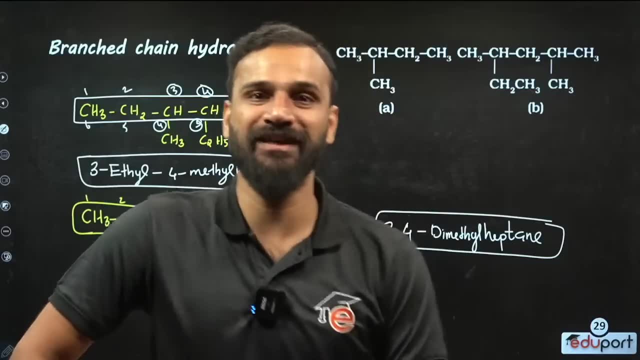 so it is hept. Since everything is single bond, it is any. So children say the name: Two comma four dimethyl heptane, Two comma four dimethyl heptane. Is it okay? Is it okay? It is very important. 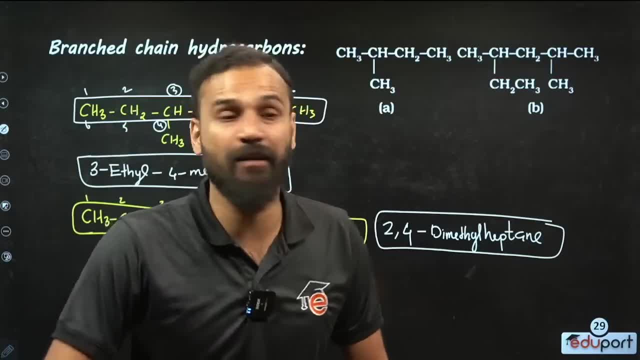 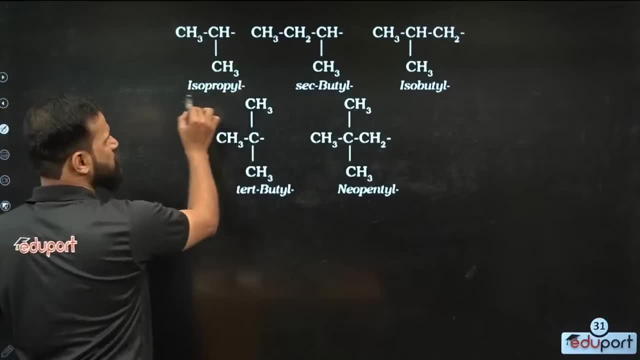 It is very important. I am going to give you a question. You have to answer it quickly now. Look, Then. this is about the branches Methyl, ethyl, propyl butyl, etc. This branch is called isopropyl. 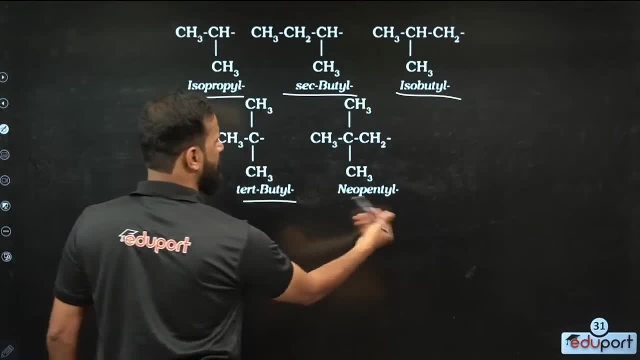 This is secondary butyl. This is isobutyl. This is tertiary butyl. This is neopentyl. Know everything. The names of the branches are given. I will give you a question. You have to give the answer quickly, children. 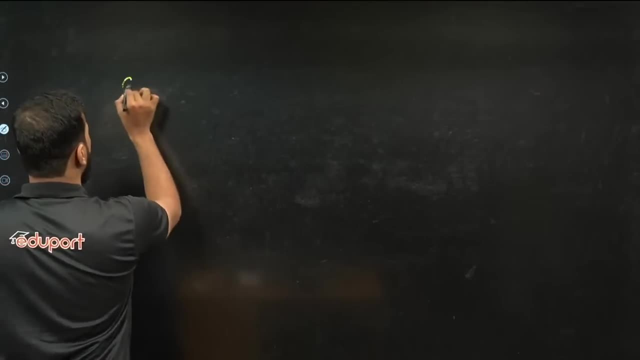 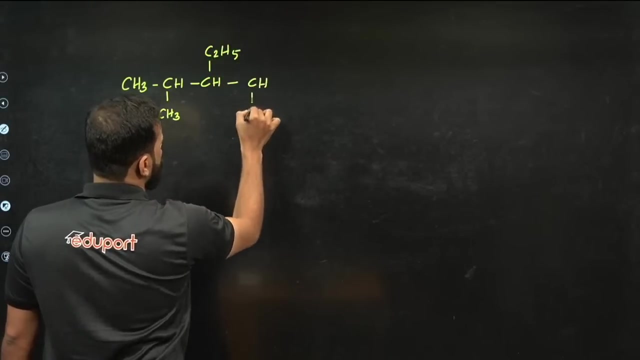 Look, My question says CH3. CH3. CH3. CH3. CH3. CH3. CH. CH3. CH2. CH5. CH. CH3. CH2. CH3. CH2. CH3.. 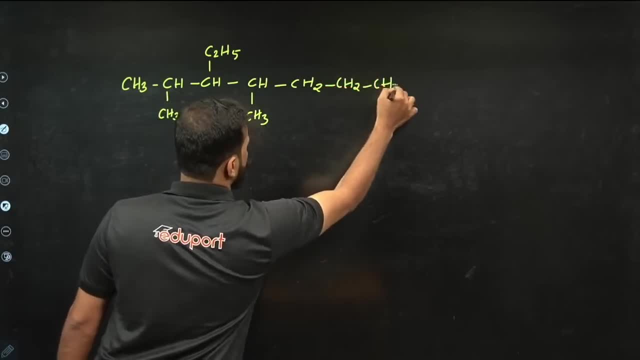 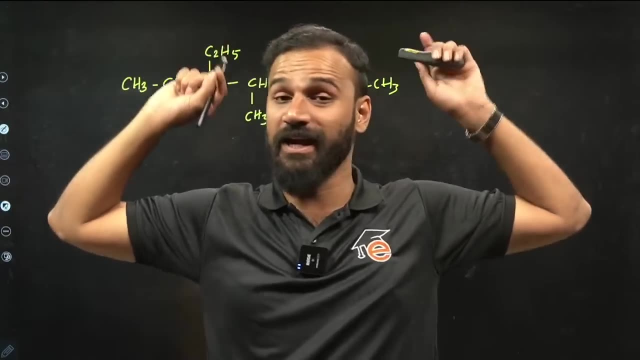 CH3.. CH1. CH2, CH3. CH3. CH2.. CH3. CH3. CH1. Thenнить also CH3.. CH3 is CH3.. dashicamente CH3.. If you can say the name of this. 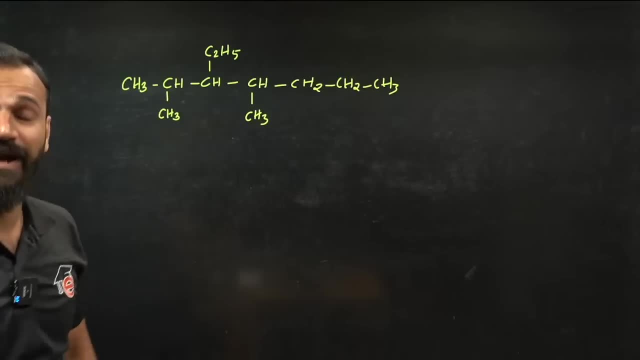 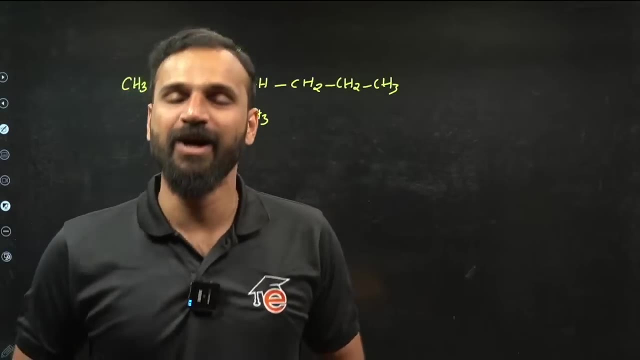 you can say the name of this quickly. You can try to guess it. You can try to do the number. I want to get the name of this Because naming is always the area where the question is asked. Say it quickly. What is the name of this? 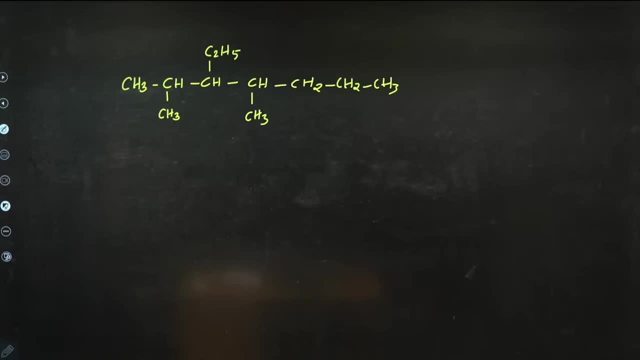 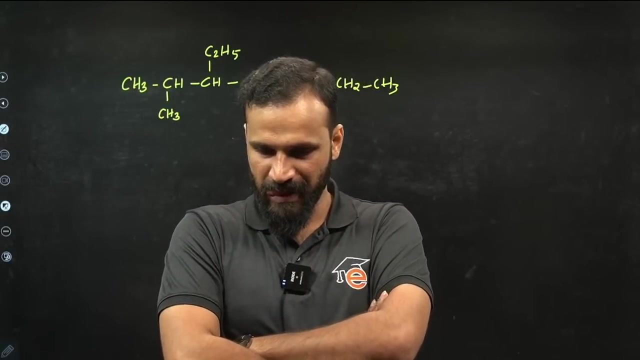 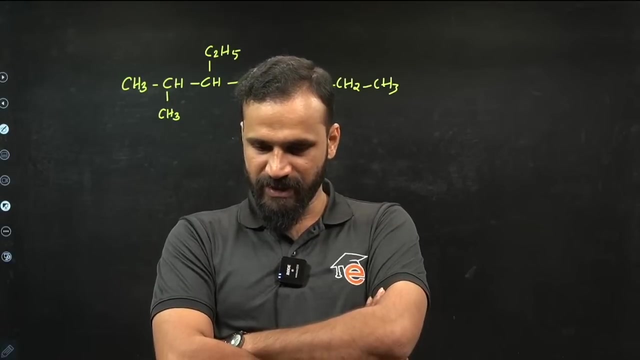 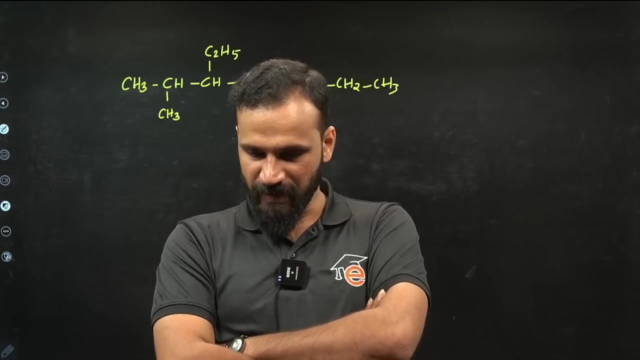 Say it quickly, Yes, Say it quickly, Yes. Kirtan has commented. Peter has commented. Very good, Jessie has commented. Absam has commented. Anna Amna has commented. Feba has commented. Kuttan has commented. 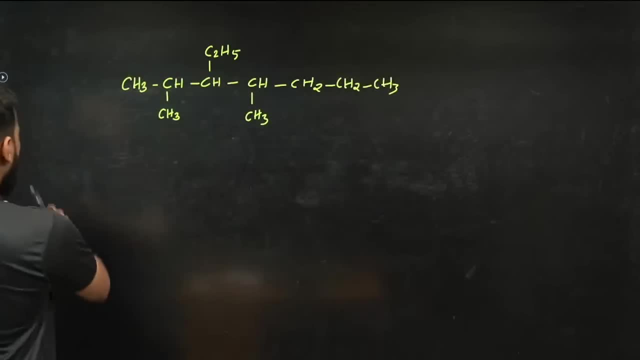 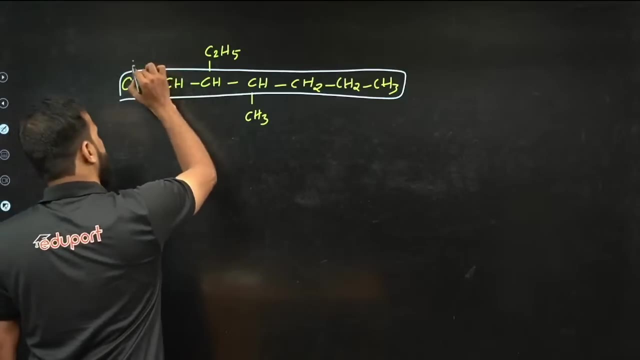 Ayesha- Yes, a lot of people. Very good, So children see if this is how you got it. This is the longest chain, No doubt about it. The number has to be left to right: 1, 2,, 3,, 4,, 5,, 6,, 7.. 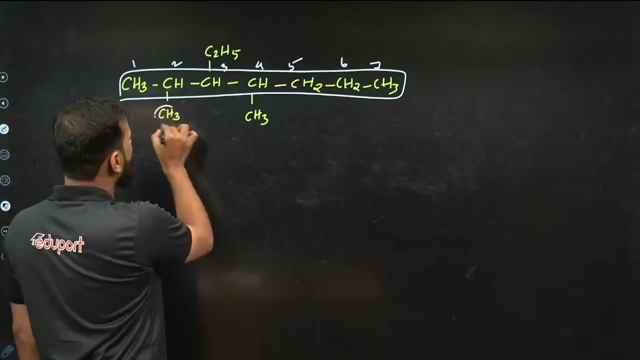 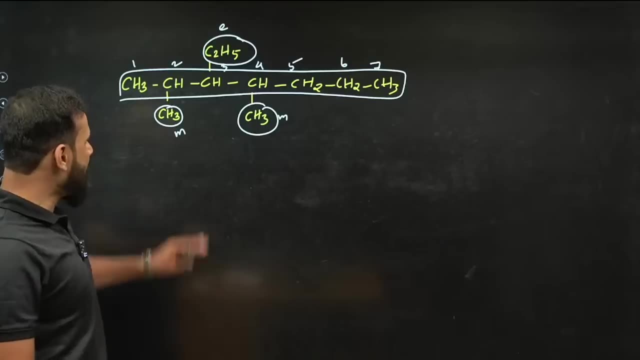 Right, This is a methyl group. This is an ethyl group. This is a methyl group, Right? So the first one in the alphabetic order is E, So he has to say it first. So let's say 3-ethyl. 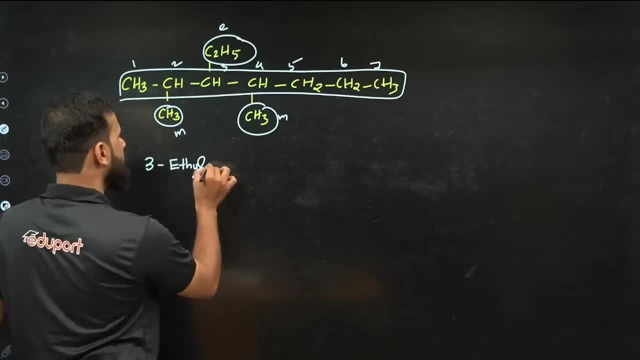 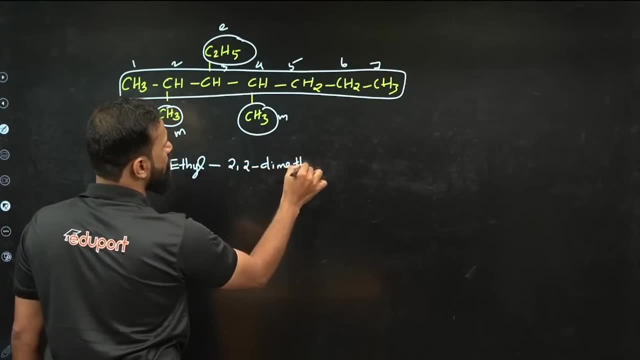 So children 3-ethyl. Now both 2 and 4 have methyl, So 2, 2, dimethyl 2, 2- Sorry, not 2, 2 but 2, 4.. Because both have 4.. 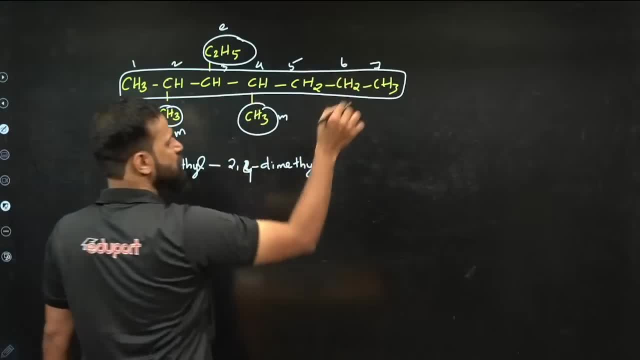 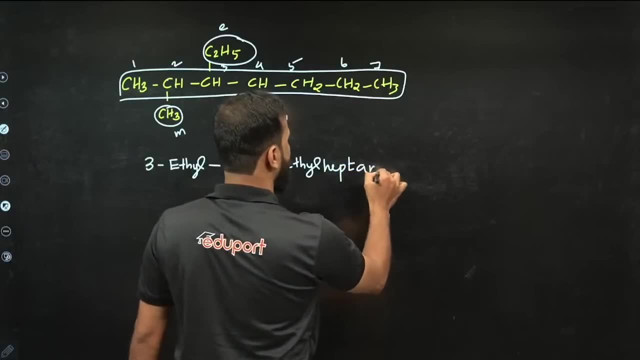 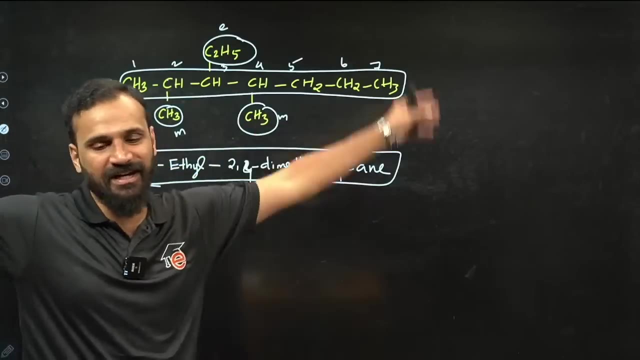 2, 4 dimethyl. Longest chain is 7 carbon atoms, So that is hept, Hept. All are single bonds, so any So 3-ethyl, 2,, 4 dimethyl heptane. 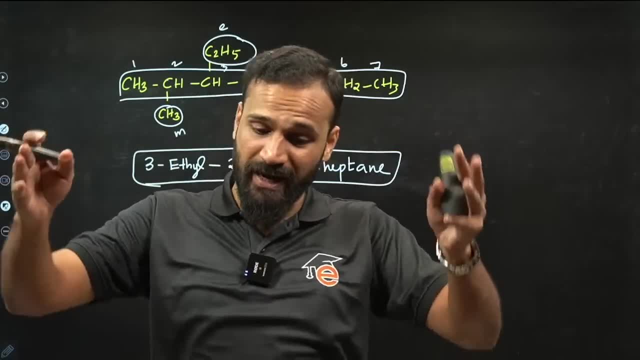 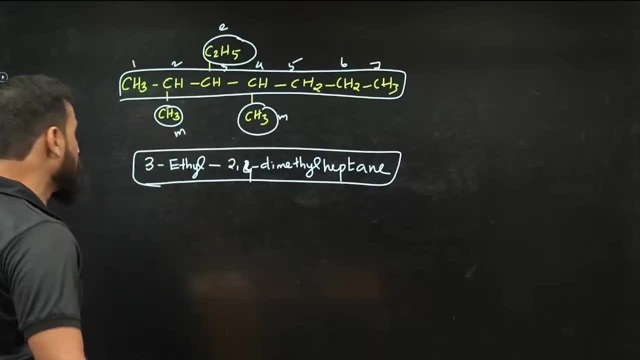 Have you got it today, children? Have you got it today? Don't ask if you got it today. Everyone got it today, right? Very good? Everything you see is the correct answer. Everything you see is the correct answer, Very good. 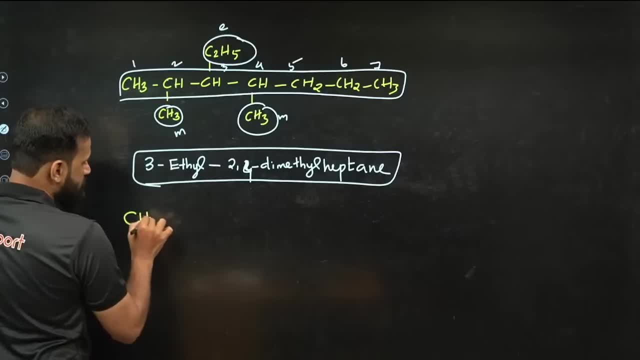 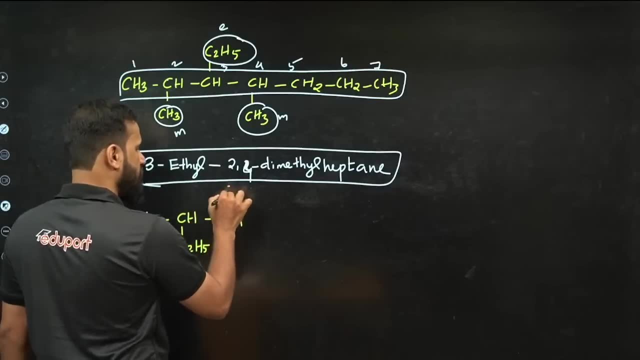 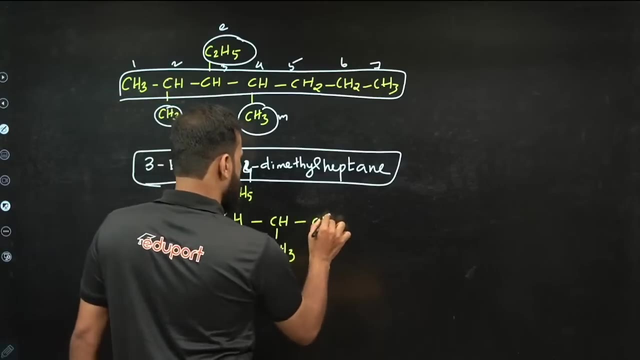 So I will give you one more question. I will give you one more question: CH3CH, CH2H5, CH2H5, CH2H5, CH2H5, CH2H5, CH3CH, CH2, CH2H5, CH2H5. 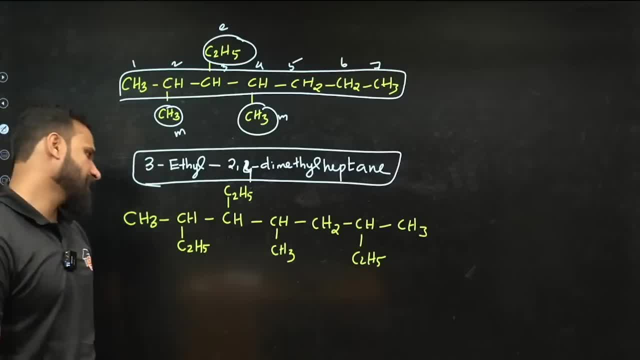 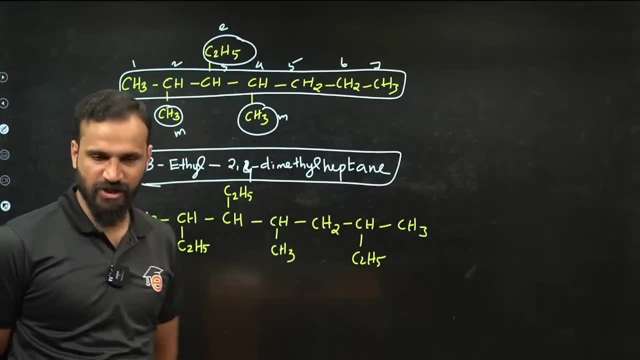 CH3- Children, say it fast. What is the UPSC name of this? What is the UPSC name of this? What is the UPSC name of this? Children, say it fast. What is the UPSC name of this? Many people are getting it. 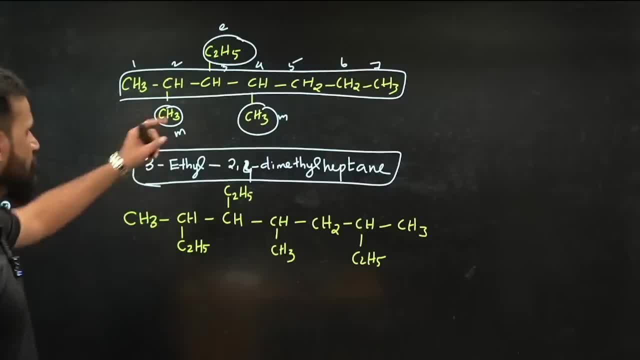 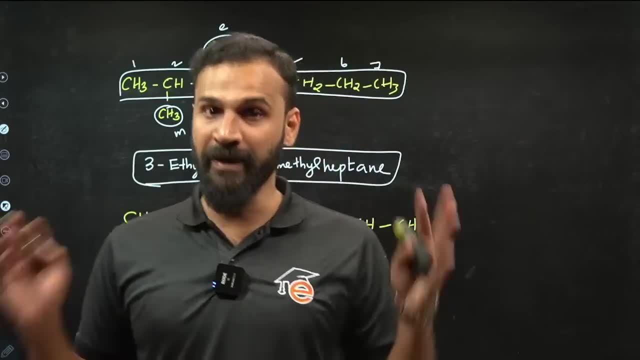 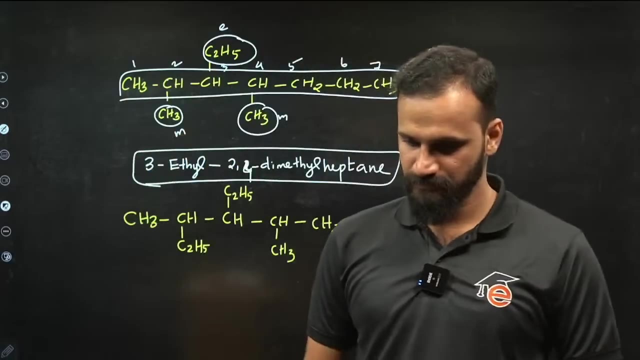 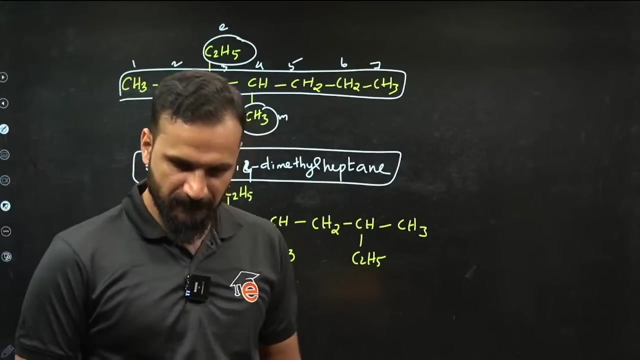 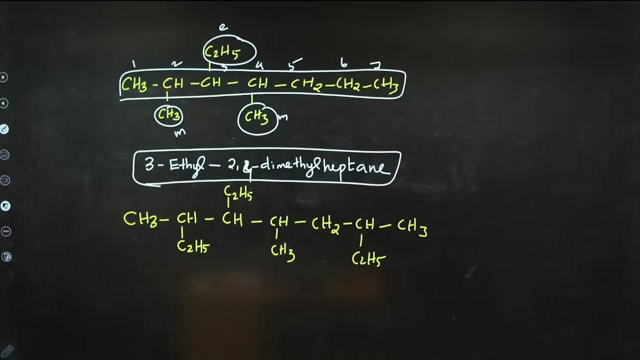 Very good, Very good. What is the UPSC name of this? What is the UPSC name of this? Yes, Yes, Yes, Yes. Look fast, Look fast, See if you can say it, See if you can say it. 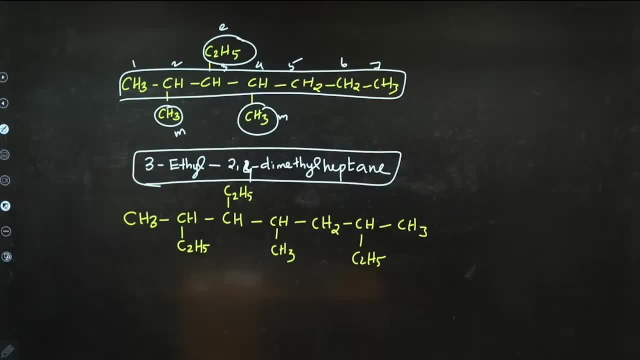 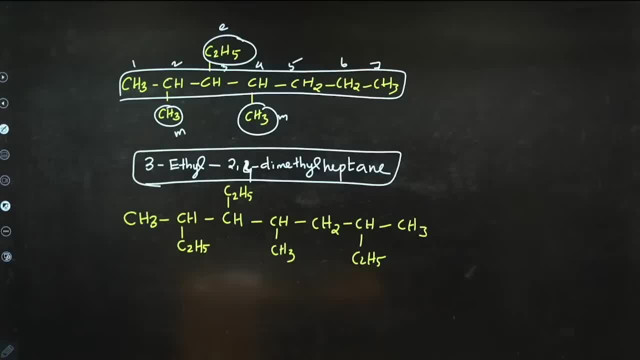 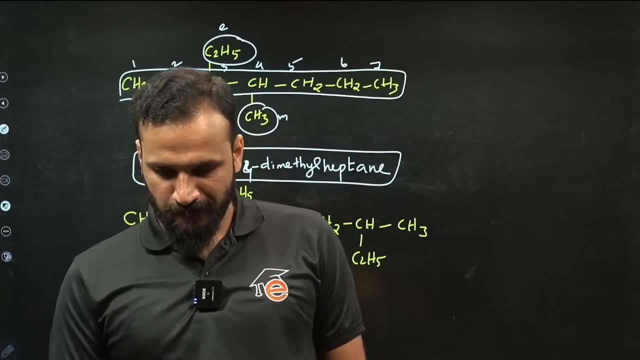 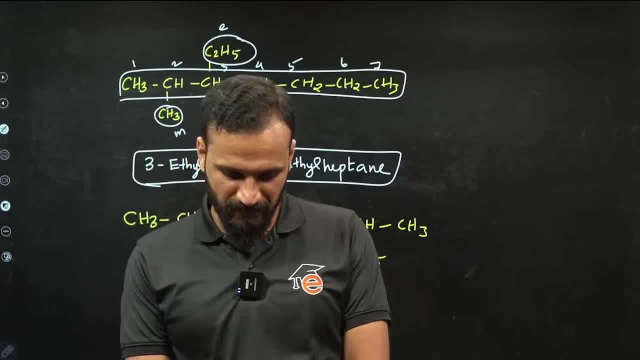 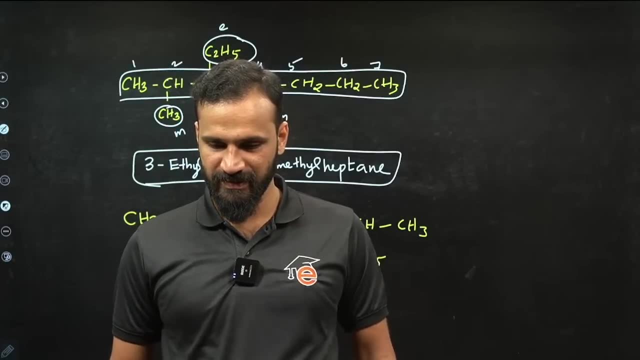 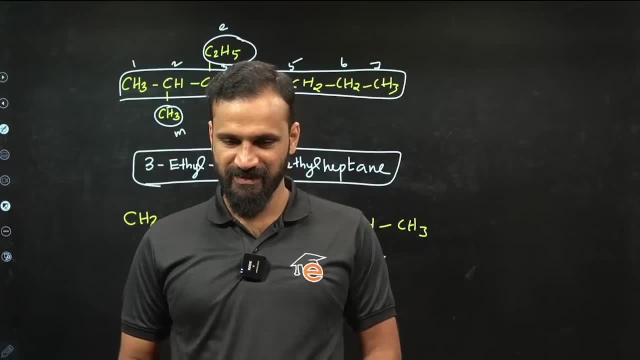 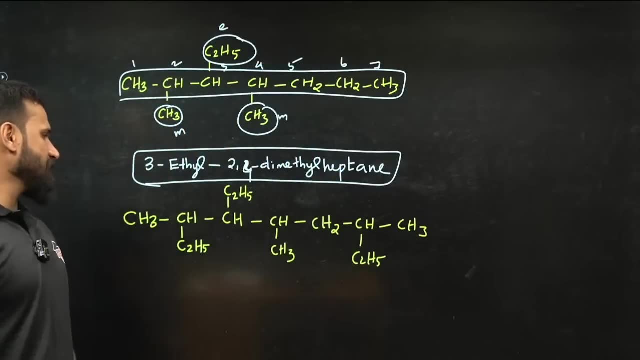 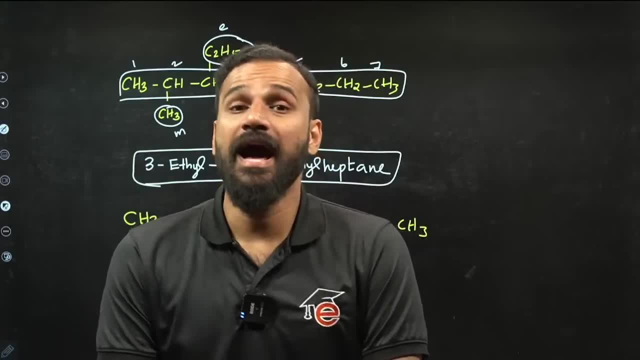 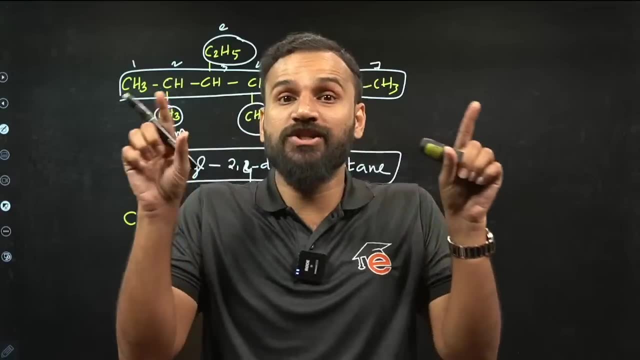 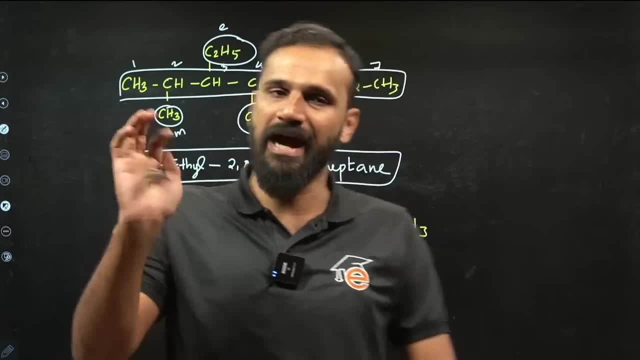 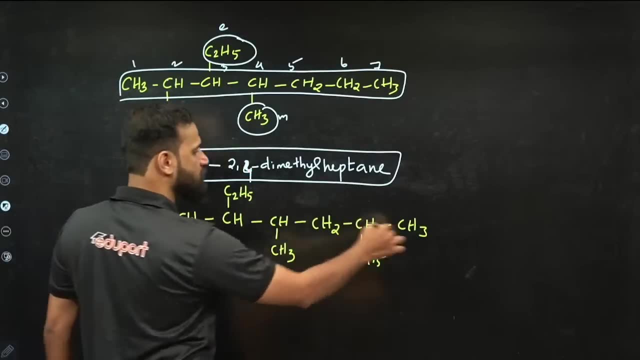 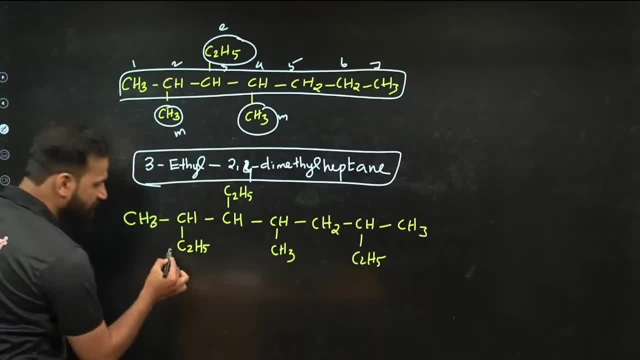 Longest chain is said to start from here. Here is not CH3.. Here is CH2CH3 or CH2H5.. There are two carbon atoms here, Isn't it? I said earlier? I said earlier, CH3CH2 is written like this: 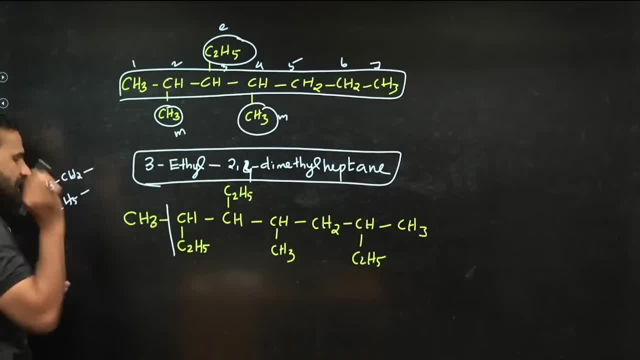 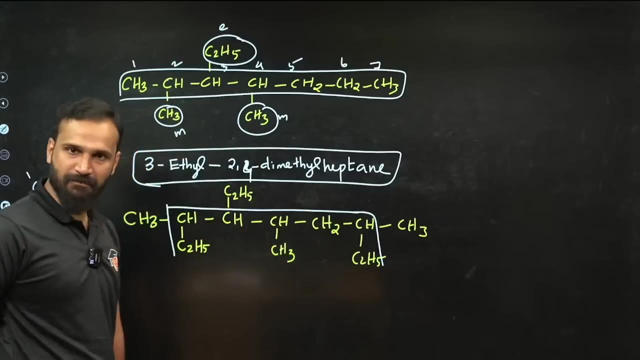 It is written as CH2H5 in short. So If you see CH2H5, there are two carbon atoms there, Understand. So here are two, three like this. All of that has to come down Because there are two carbon atoms here as well. 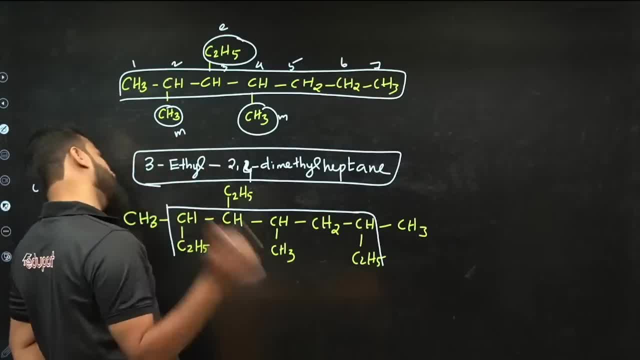 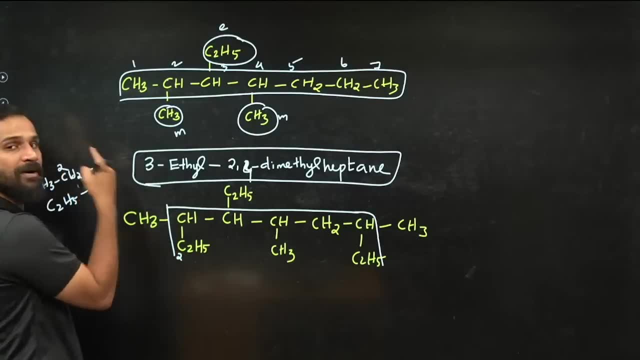 So how do you have to number it? So, children, how do you have to number it? Pay attention, Ah, how many are there here? One, two, So two Give it. How did I give two? Because there are two There is. That's why Here is the third. 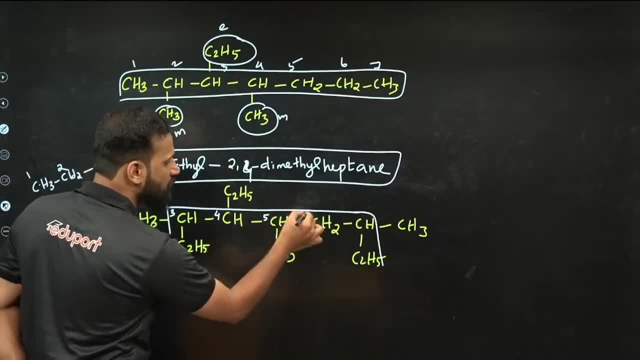 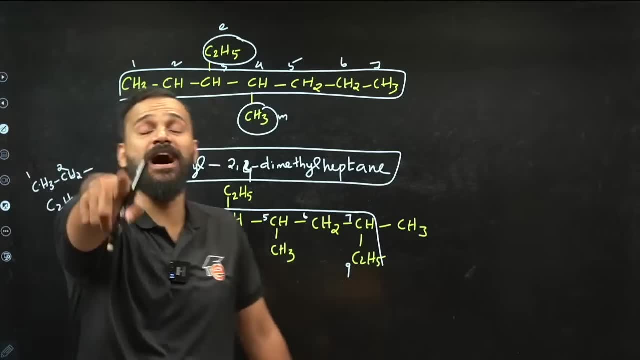 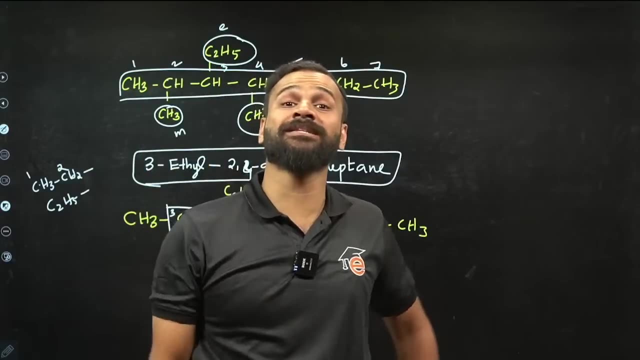 What is it? Three, four, five, six, seven. Then what is it down there? There are two, Eight, nine, Nine carbon atoms. There is the longest Chain. I know many of you will have missed it. Many will have missed it Because what is it? 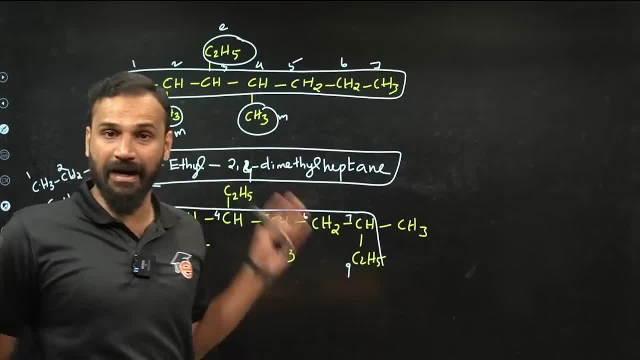 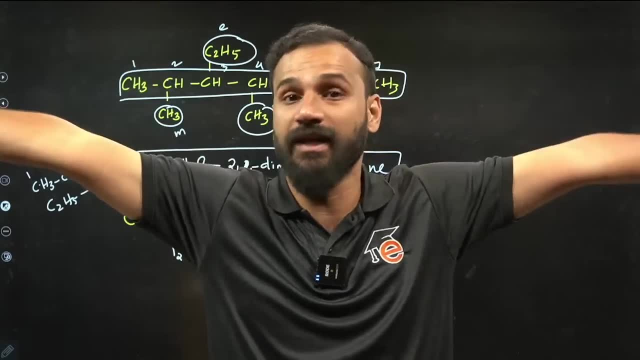 There is no need to run and waste time by suddenly drawing a line. What I am saying is that the question comes to two marks or three marks. Just don't miss it by mistake. Ah, longest You have to mark the chain and look into it again. 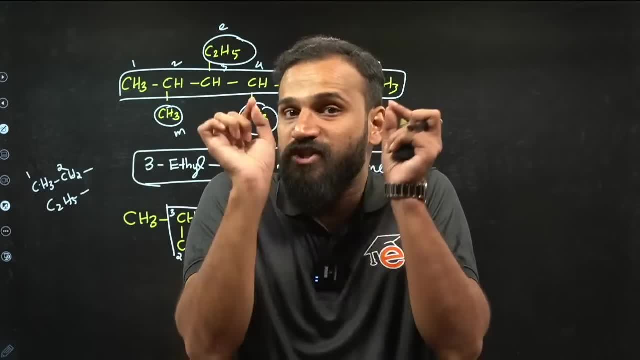 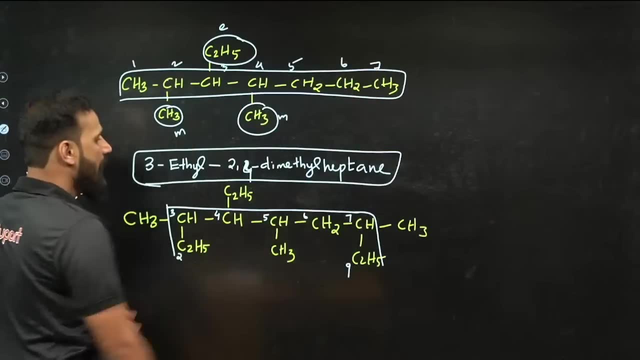 Whether there is any other chain there, because that first step, If wrong, then everything went wrong. then there was no sudden thing. Yes, So this is the longest. So if you do this number, look You, There is a branch in the third, carbon methyl. 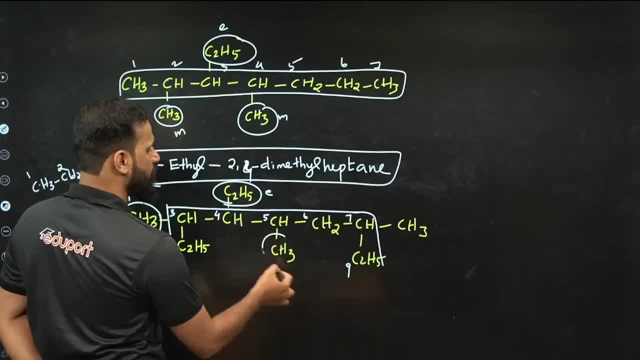 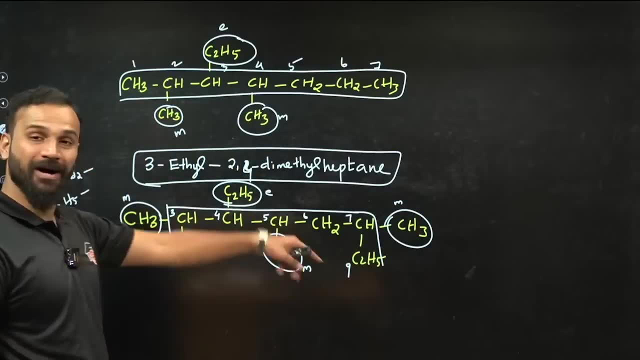 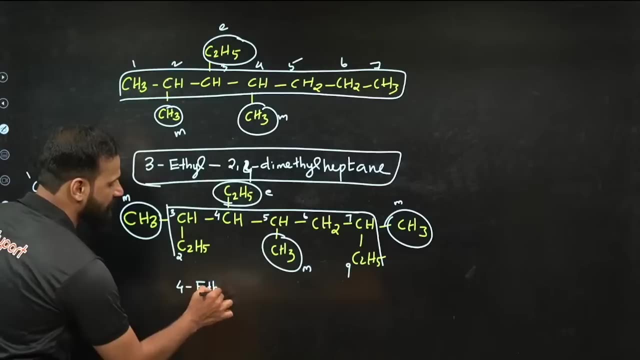 There is a branch in the fourth ethyl, There is a branch in the fifth methyl, There is a branch in the seventh ethyl methyl, So the longest chain is nine carbonate Three. there is ethyl in four, So the name of it is four, ethyl Four. 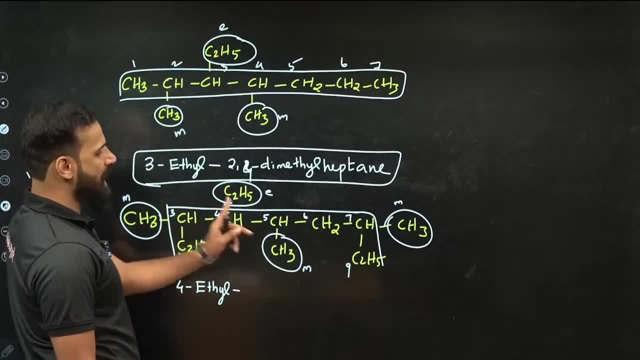 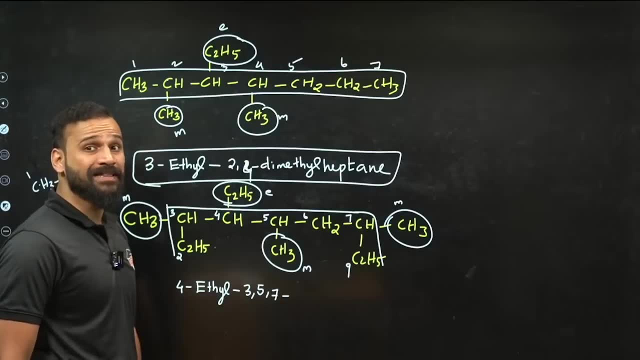 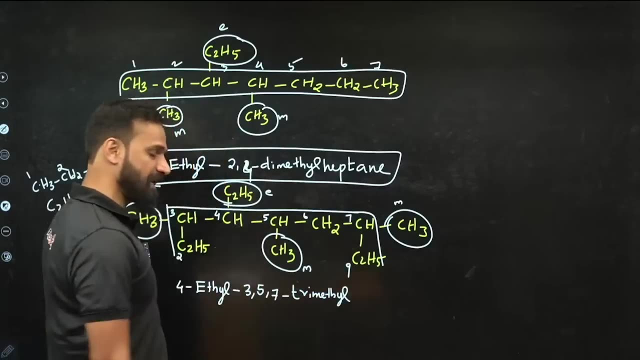 ethyl In three in five in seven, In three in five in seven. Who is it? Methyl? So how much methyl is three methyl Tri-methyl? Our name is tri-methyl Tri-methyl. 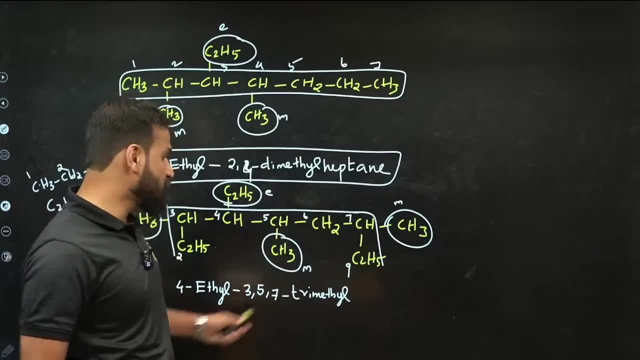 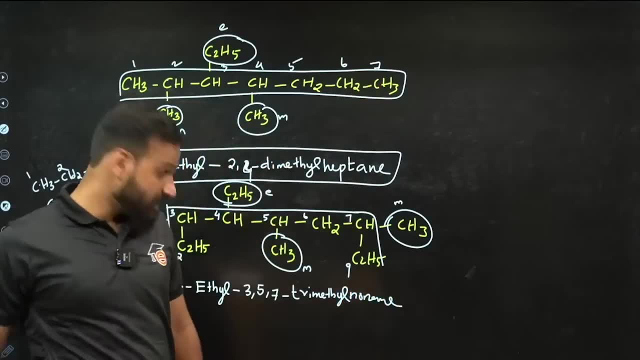 Longest chain. how much carbonate Nine, All single bond, Any So non-ane is good guys, Non-ane is good. Non-ane is good. Yes, This is the name: Four ethyl, four ethyl three. 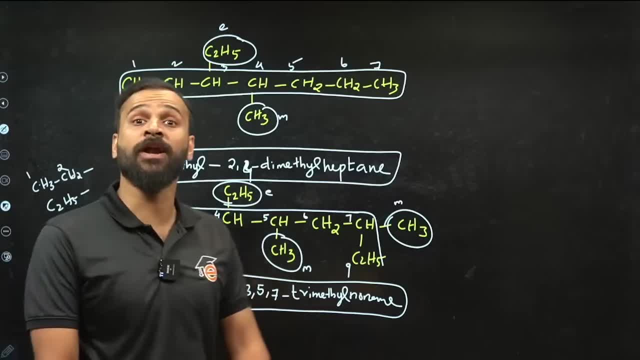 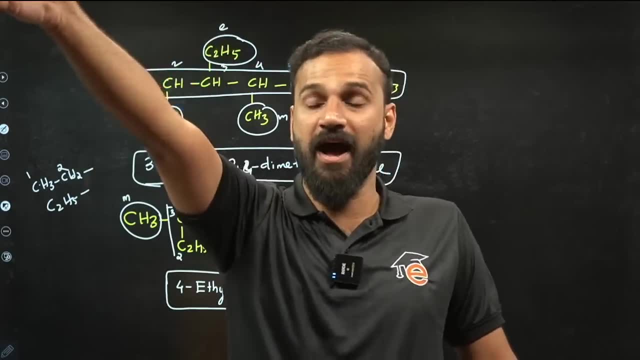 comma five, comma seven: tri-methyl non-ane. So saying wrong is not a matter of one thing. Make it right by making it wrong, like this. At the very least you practice. That's what I just said about the rules without telling you. You are taught through questions. 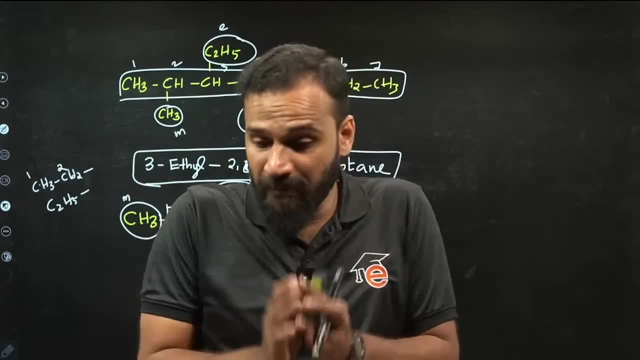 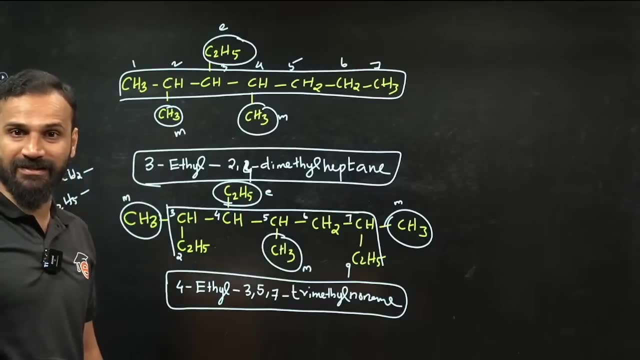 There is only one thing to do and practice like that, Because when such questions come, we must be able to write it correctly. That's where the point lies. That's where the point lies. Okay, guys, Okay right. Yes, there is still to be done. 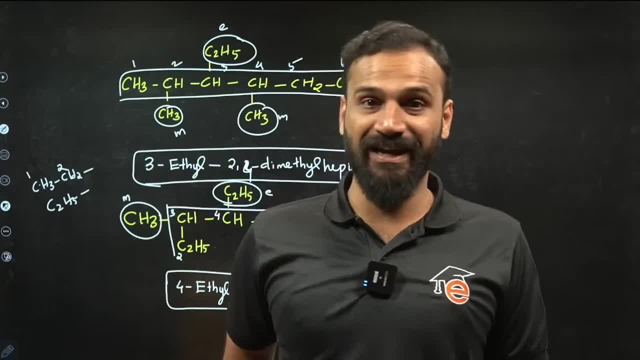 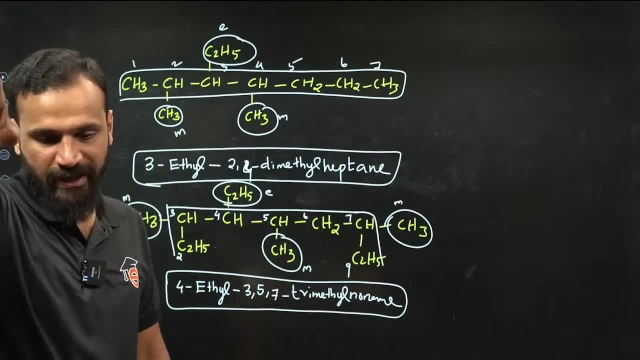 We have only reached hydrocarbons here. We have only reached alkane. We have not reached functional double bond or cyclical. We can go to that. Guys, take good care of yourself. The longest chain is taken by anyone. If that is so, you must be very careful. Don't miss it. 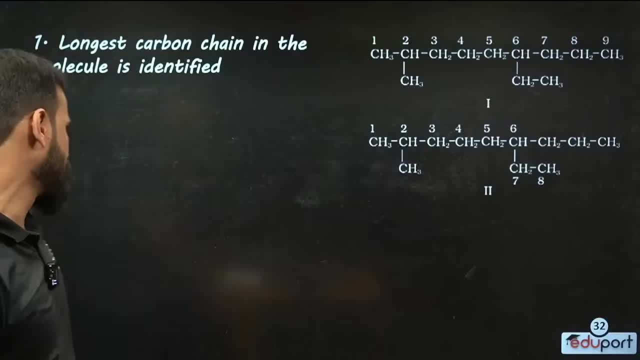 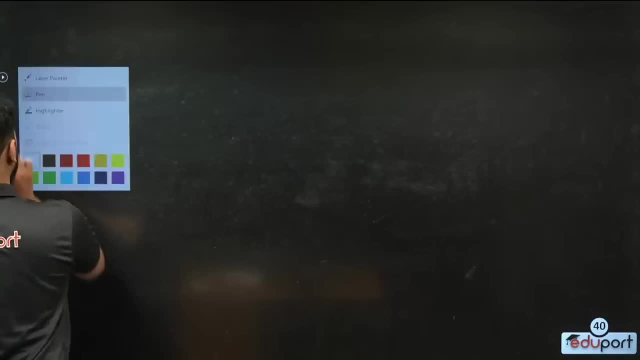 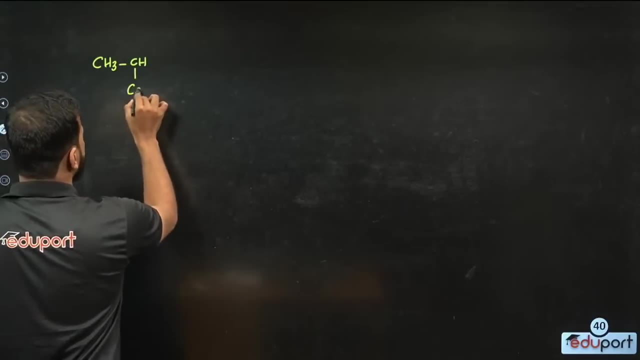 There are a lot of people who have made mistakes. It is okay, But I have to pay attention to this next time. if I made it, I should pay attention. Look, we can tell the rules all. Let's go Before that. look, kids, I will give one question. 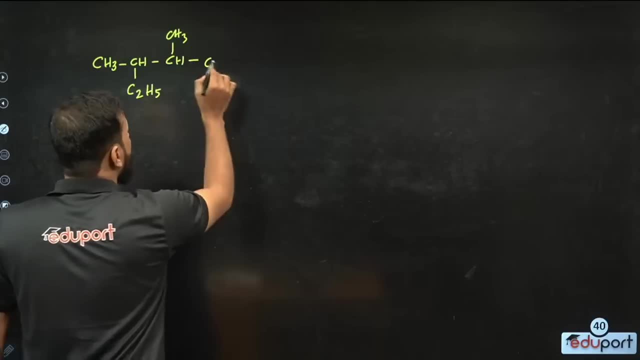 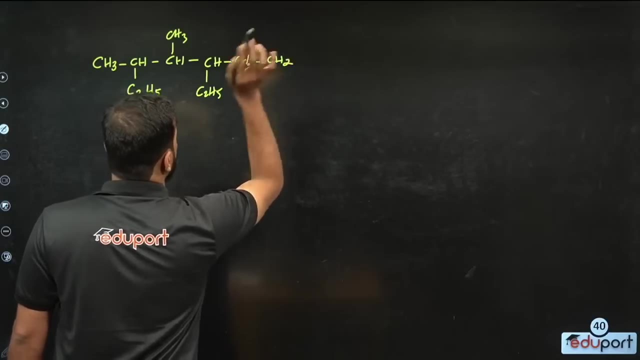 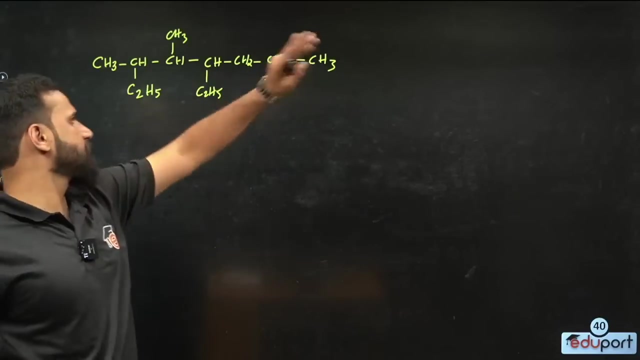 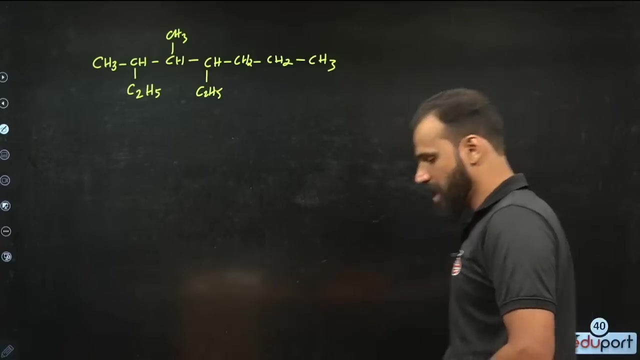 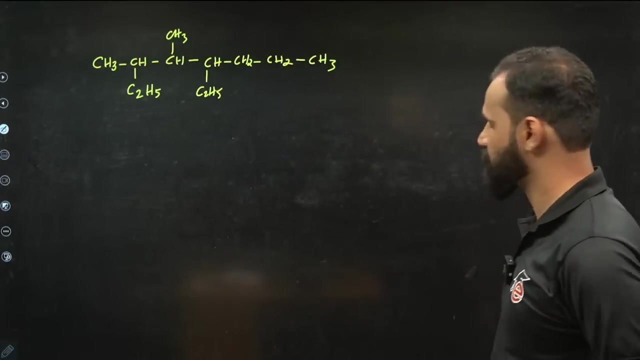 I will give a question. Do it quickly. C H three. C H, C two H five. C H three. What is this? C two H five. What is C2H5, CH, CH2, CH2, CH3.. Children, if you say that the name of this is wrong, if you say that the name of this is wrong, don't mistake that you are taking the longest chain. If you make a mistake, it's all gone. Okay, do it carefully. Do it carefully. do it carefully. It's very important. It's very important. That's why I'm saying that Yes, 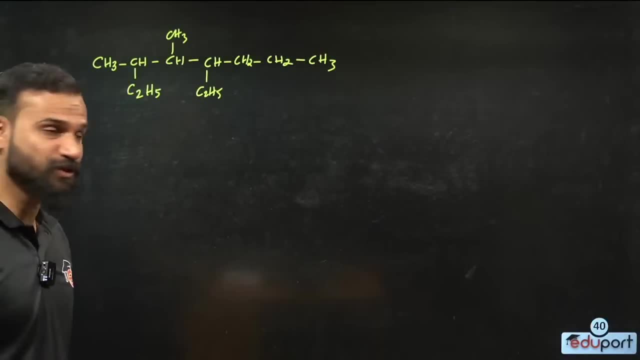 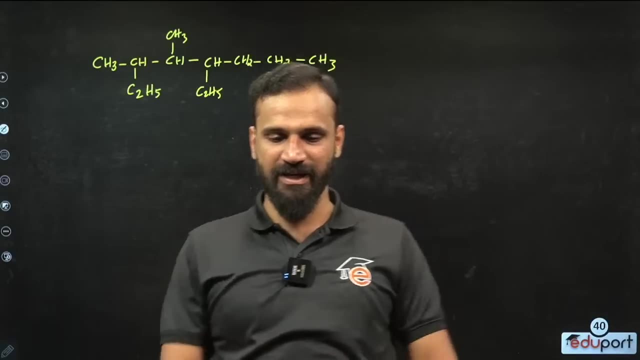 Okay, it's very important, Take good care of it. Take good care of it If you write it immediately, immediately in the chat box, immediately in the chat box, you can comment on it. Immediately in the chat box, you can comment on it. It's important, It's important. 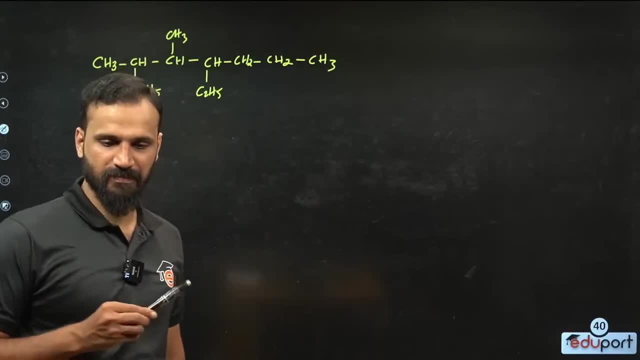 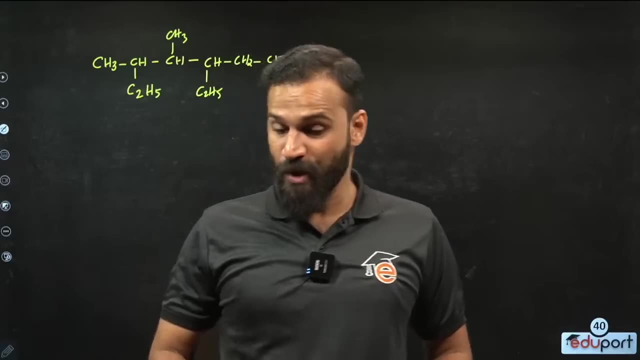 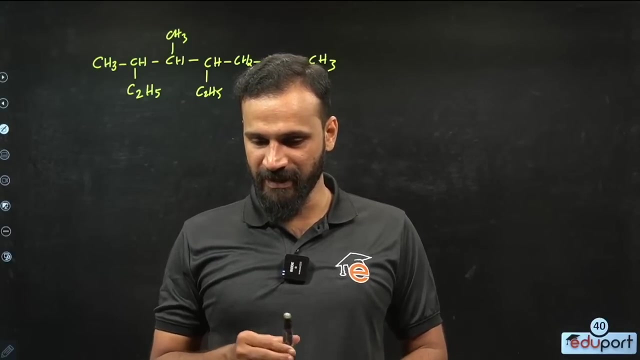 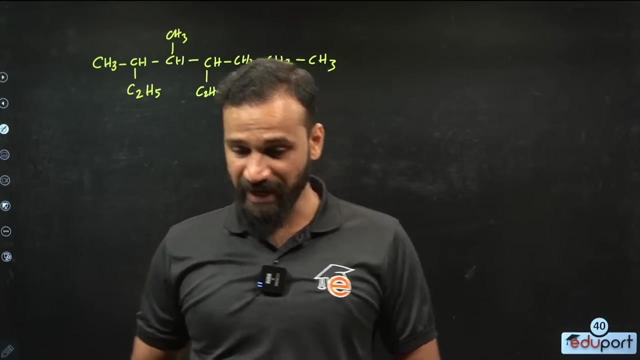 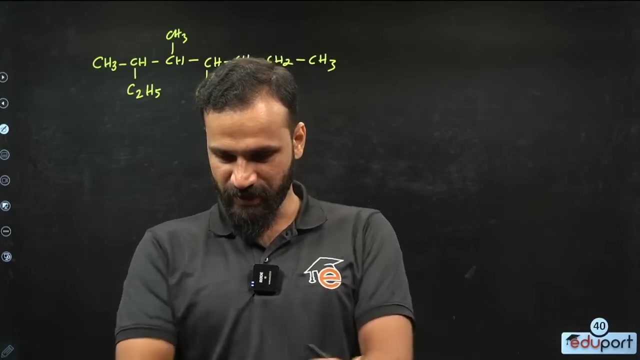 It's important. Let me see who comments first. Let me see who comments the name of IUPAC first. It's a very important thing. Yes, Who comments first? Yes, Basel, Basel, Skaria, Basel, Skaria comments first. Very good, Amina Nazar comments first. Very good, Very good. 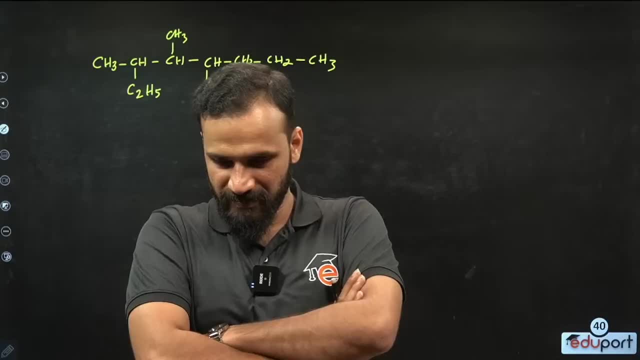 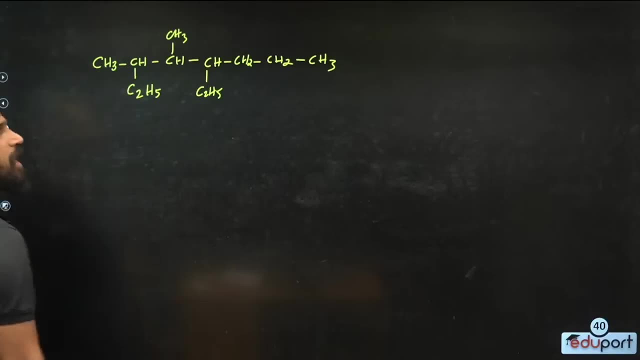 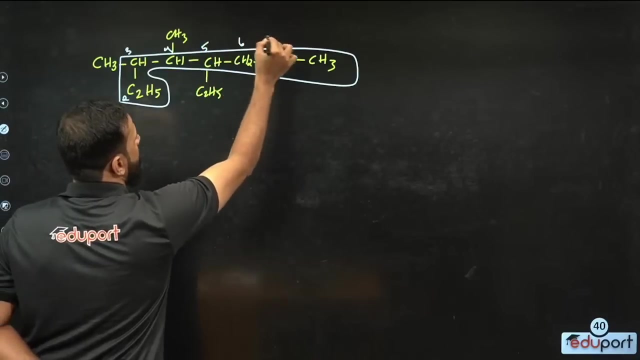 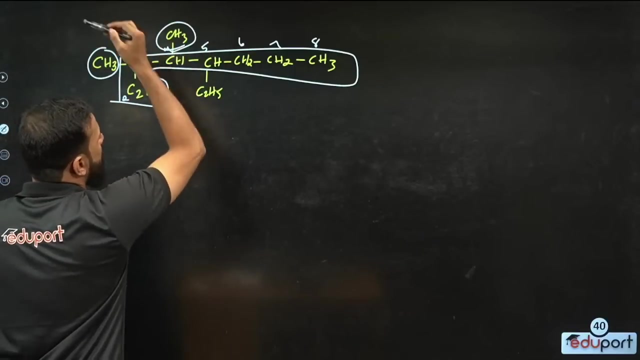 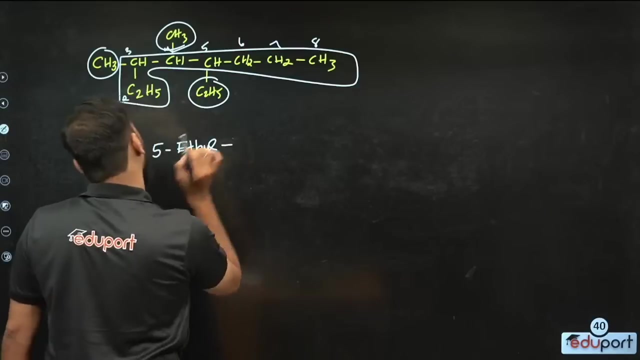 Yes, This is not the longest chain. Yes, this is the longest chain. How do you count? One, two, three, four, five, six, seven, eight, Like this right? Yes, Three is ethyl, Four is ethyl, Five is ethyl, Then five is ethyl. Let's say, five is ethyl, Five is ethyl. Three comma four. Three comma four. 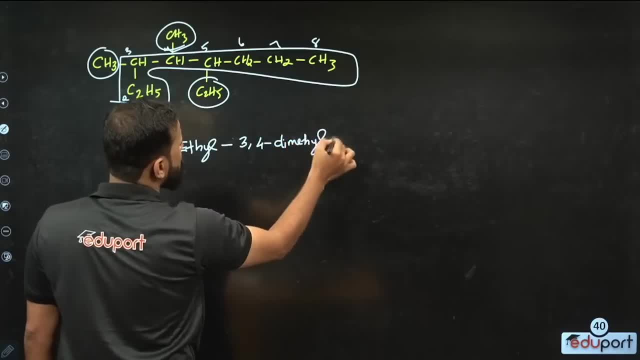 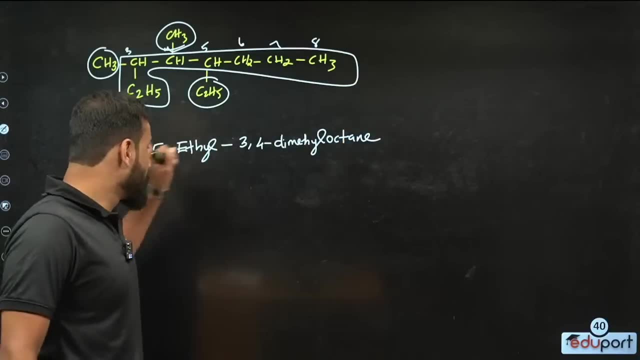 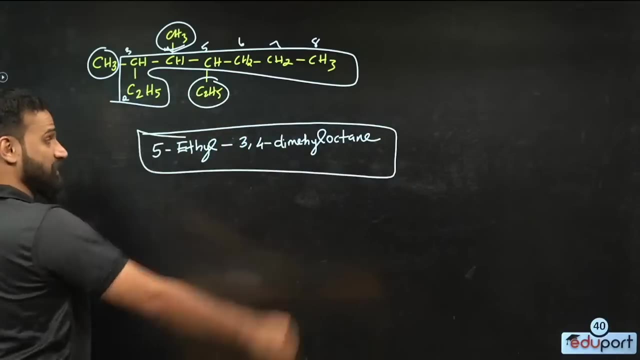 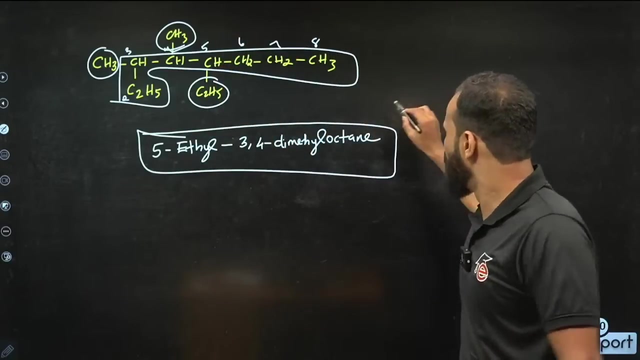 Dimethyl Longest chain, eight carbon oct Single bond. I don't A N E Five ethyl, Five ethyl. Three comma four dimethyl octane, Five comma, sorry, three comma four dimethyl octane, Dimethyl octane. So very simple idea, Very simple idea, Very simple idea. 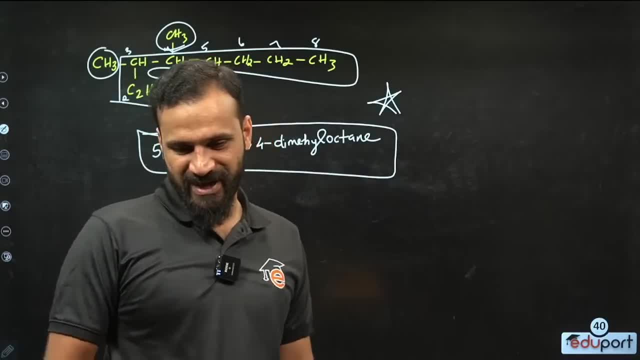 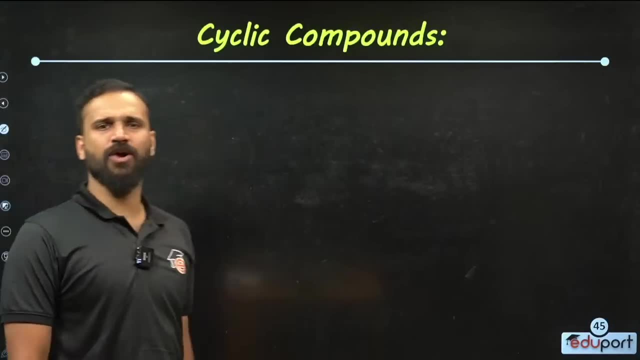 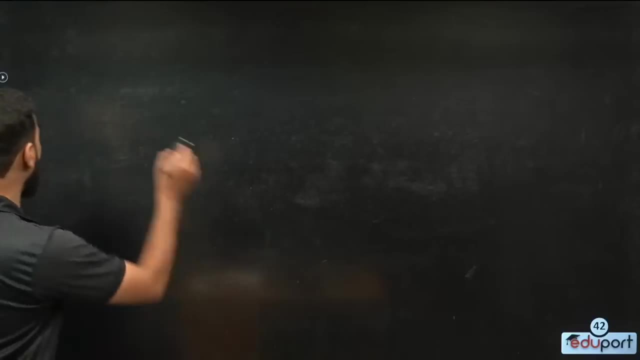 Be careful, hereous grew many. they came back乡. good, Excellent, Excellent. Look, children, how to name the cycle compounds, the cyclic compounds, What? All right, let's see we will do double bond, like the. 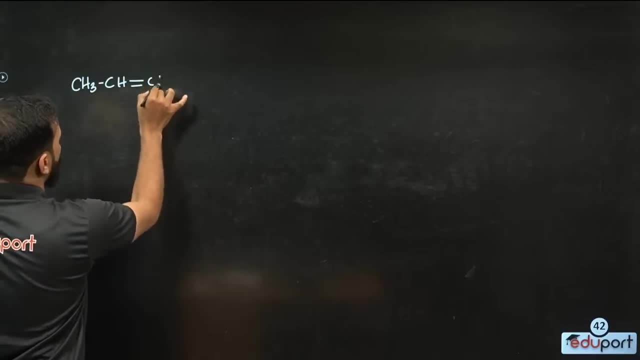 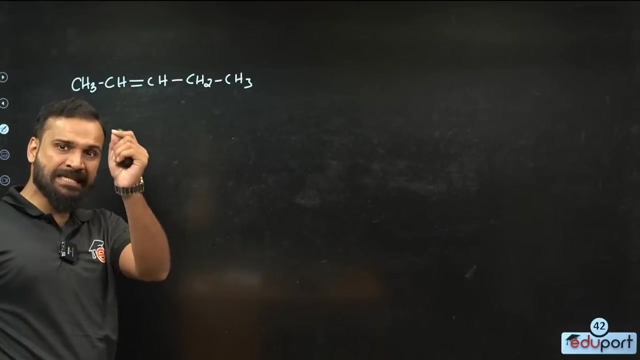 c h three c h double bond, ethical single bond. C epi two, c h three-erea. Here you. You have to pay special attention to one thing: There is a double bond here. right, That double bond should be numbered in the form of the least number. 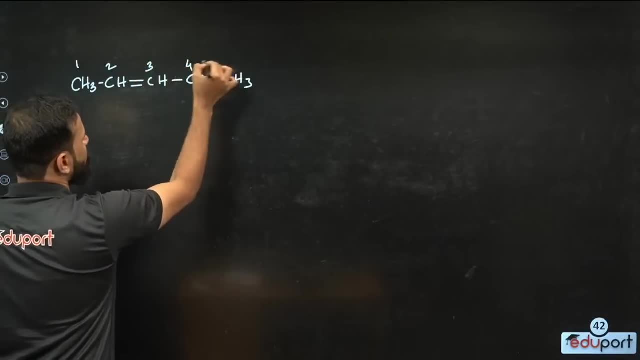 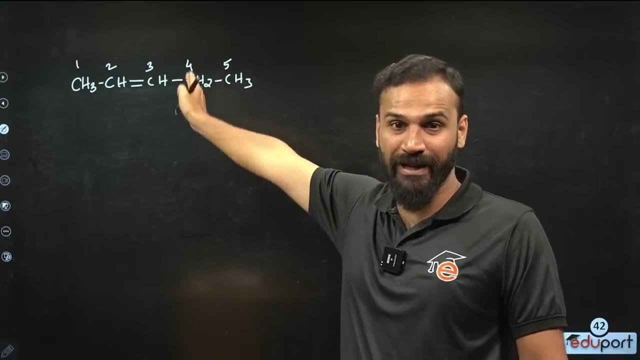 There is no doubt: 1,, 2,, 3,, 4, 5.. When you do this, the least number is obtained there, The least number is obtained in the double bond. So, dear children, you have to pay attention to one thing. 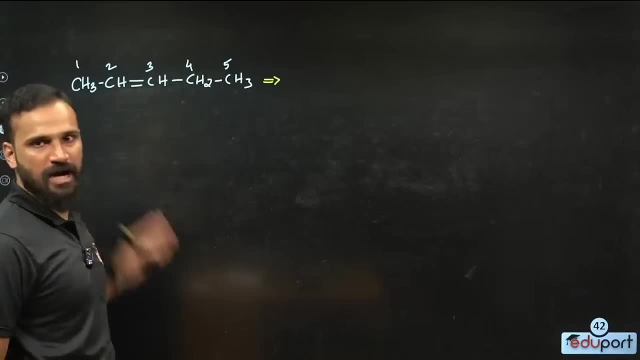 In the longest chain. what is it In the longest chain? 5 is carbon. So we understood that the root word is pend. There is no doubt. Now, in the second position, there is a double bond, So put a hyphen and write 2.. 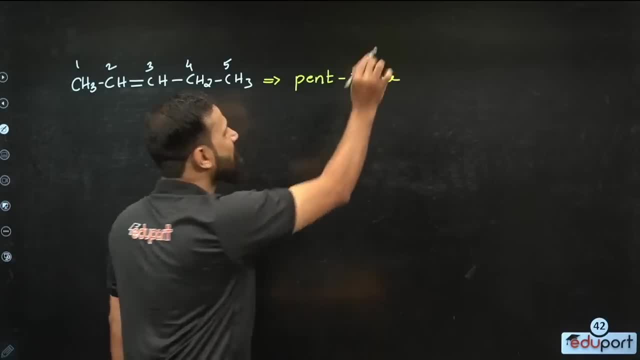 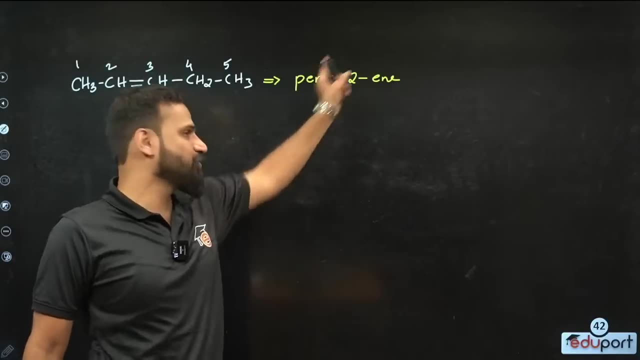 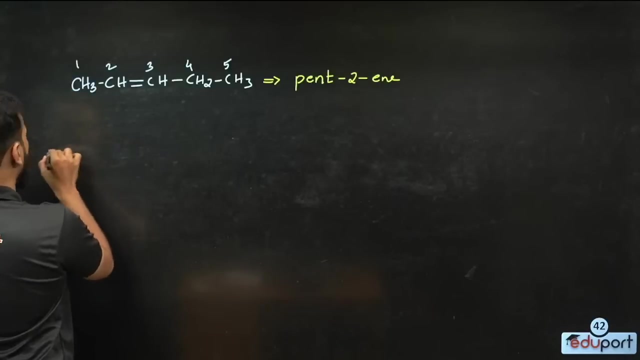 Put another hyphen and write ene, ene. So what is the name pend2e? What is the name pend2e? Look at the name Now. look at the next question. Look at the next question. dear children, 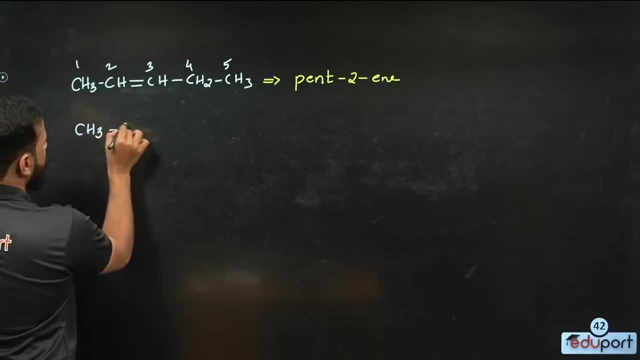 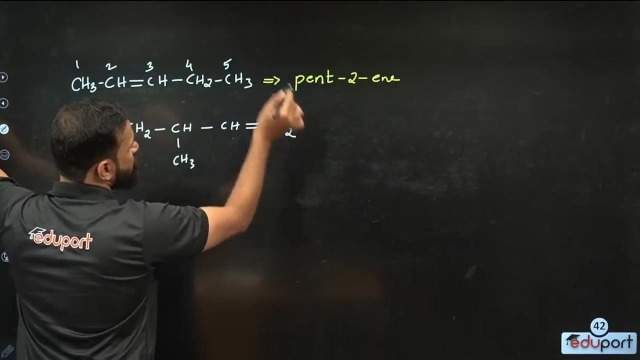 What is it? ch3, ch2, ch3, ch2, ch3, ch3, ch2, ch2.. Think that this is how it is given. This is how it is given How to give the name of this. 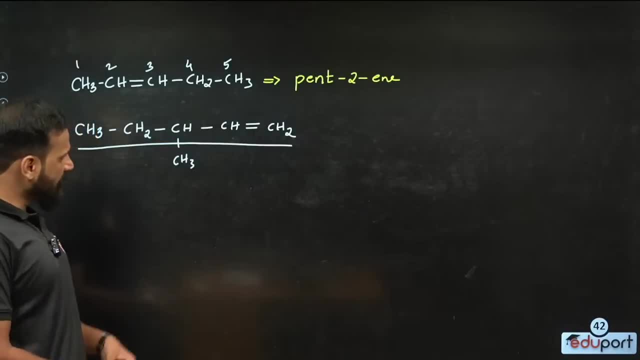 What is the longest chain? This is the longest chain. No matter how you number, you will get the position of 5 and 3.. Isn't it? There was a person who had to look before looking at it? Double bond If you want to get the number. 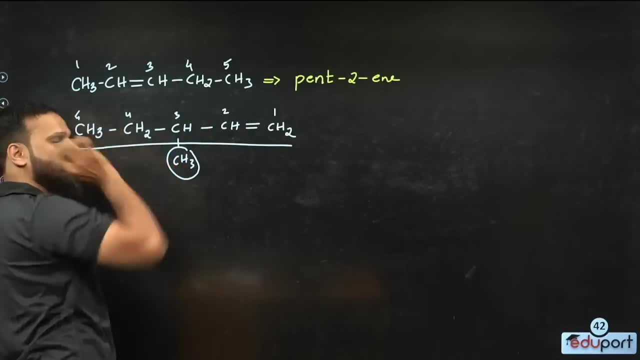 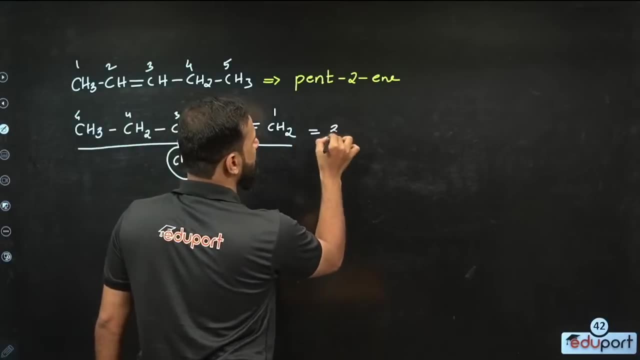 you have to start from here: 1,, 2,, 3,, 4,, 5.. You have to start like that, So the longest chain is 5, carbon. Before that, 3 is methyl, So you have to write 3-methyl. 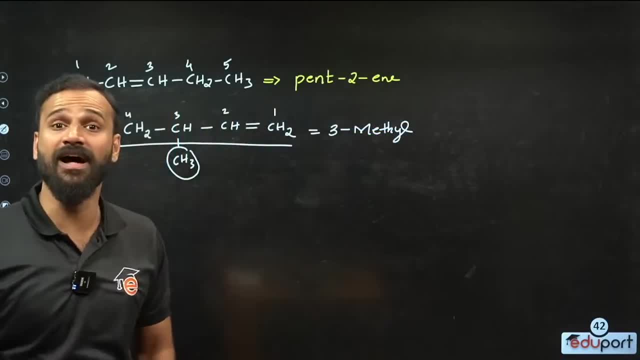 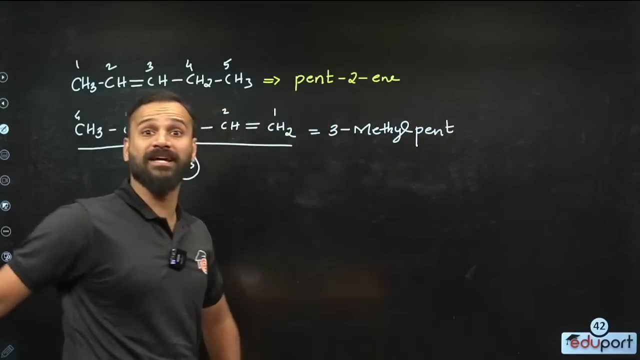 What do you have to write, children, 3-methyl? What do you have to write 3-methyl? Ok 1 carbon, So pende, So 3-methyl-pende, 3-methyl-pende. 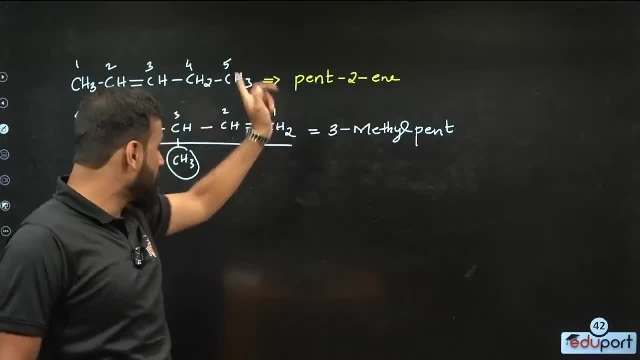 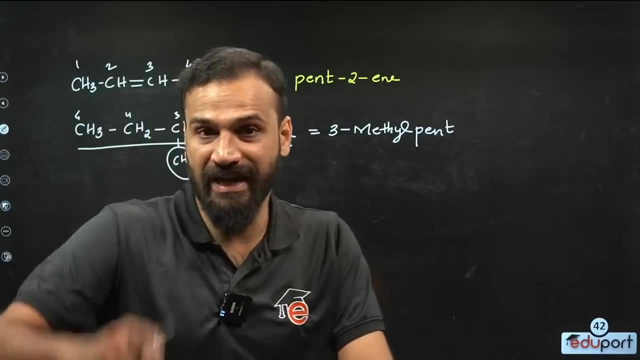 Is it pende? Is everything single bond or not? There is double bond, there is ene. Where is it? In the first carbon chain? So if it is in the first carbon chain 1-e, What children? 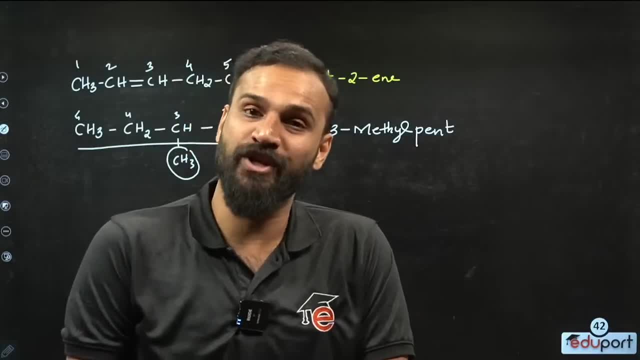 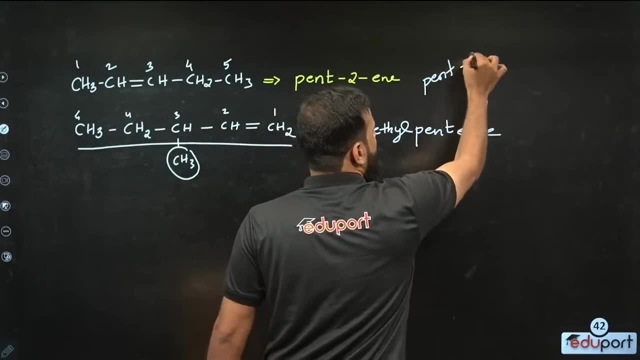 If it is in the first carbon, it is 1-e, But because it is 1, that number should not be mentioned, Just write pende. Actually we have to write pende-1-e, But because it is 1,. 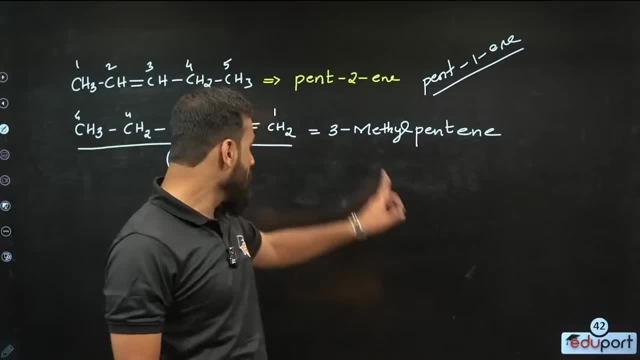 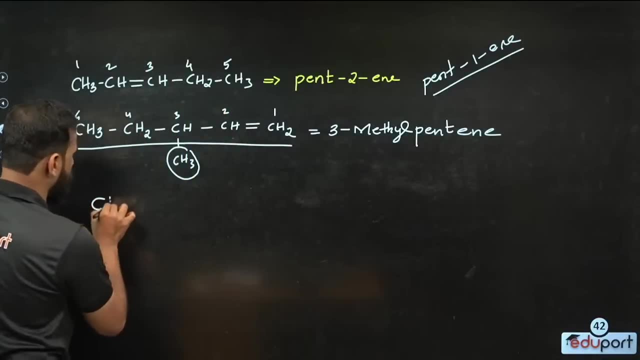 there is no need to represent it, So just write pende. So the name is 3-methyl-pende, 3-methyl-pende. Now, children, look at another question. Another question: CH3CH- single bond. 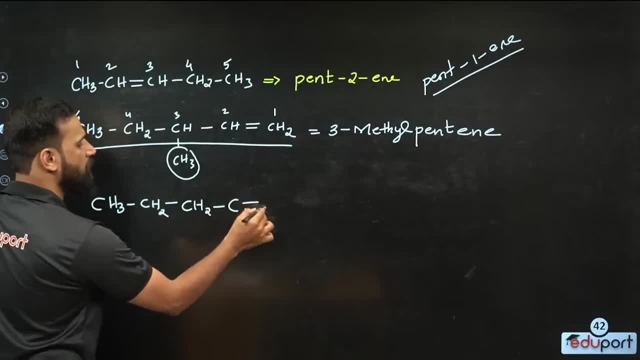 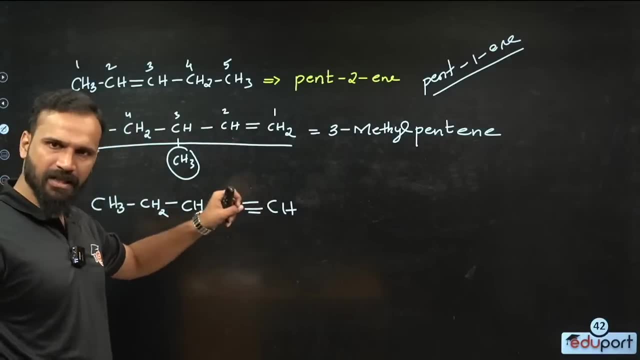 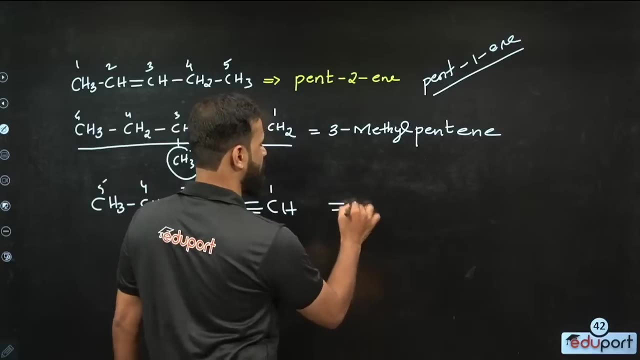 single bond. what is it? CH3CH? This is given. This is double, isn't it? This is triple. So triple bond is in this carbon, isn't it? If he wants to get the least number, he has to get the number from here. 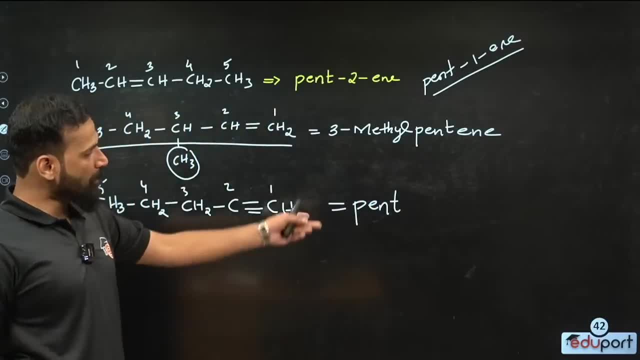 1,, 2,, 3,, 4, 5.. So what children? The name is pende In the first position, triple bond is ene, So pende-1-ine, isn't it. 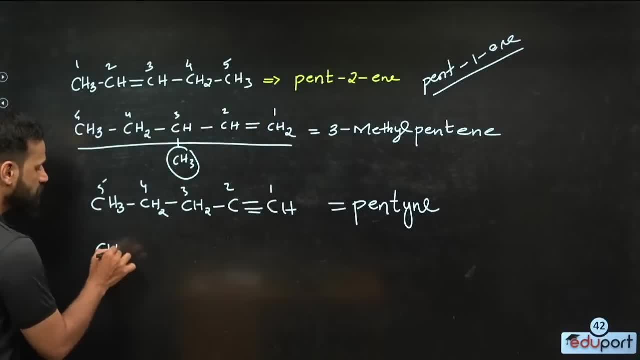 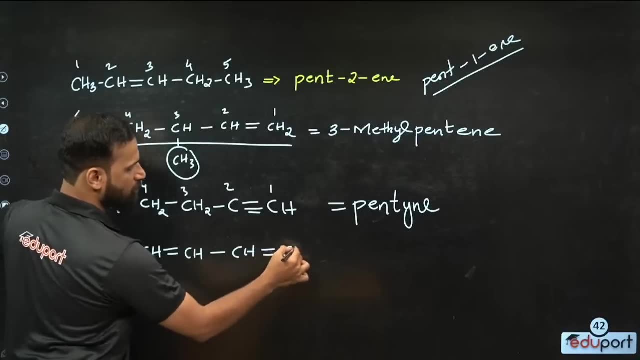 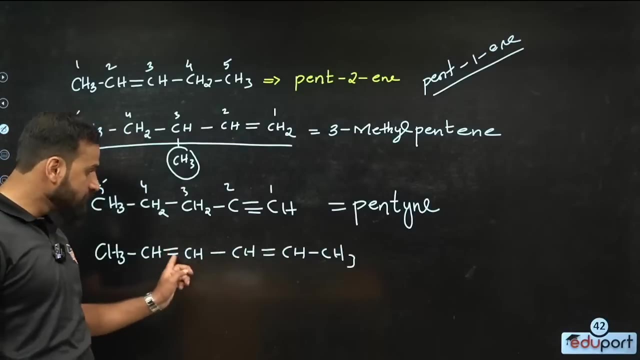 There is no need to show 1.. So pende-ine CH3CH- double bond- CH-single bond- CH-double bond- CH-single bond CH-3.. Assume that such a compound has come. Such a compound has come, There are two double bonds here. 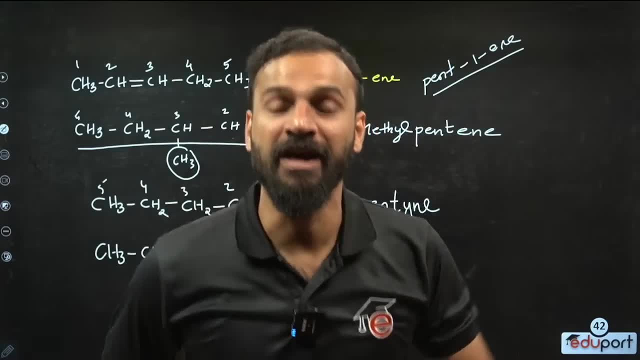 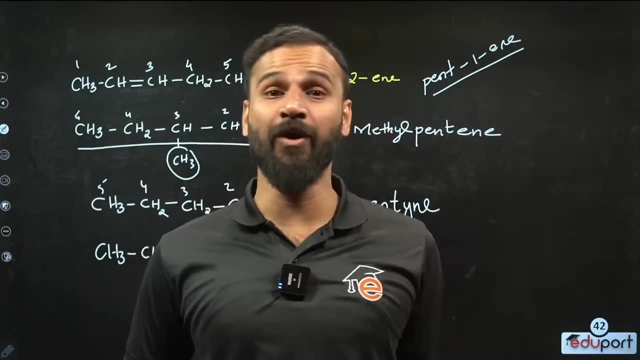 If two double bonds come, it is di-ine. If three double bonds come, it is tri-ine. If four come, it is tetra-, tetra-, tetra-ine. It is said like that: If two triple bonds come, it is di-ine. 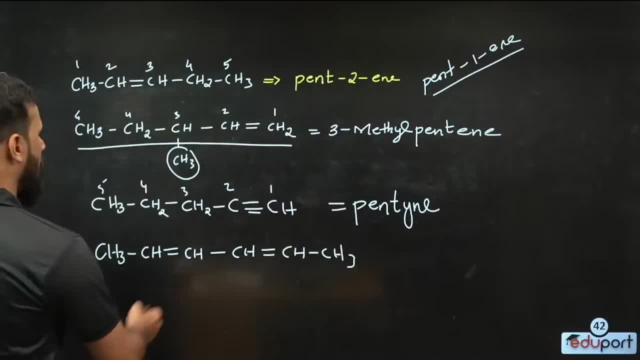 It is tri-ine. It is said like that. So look, the longest chain is 1, 2,, 3,, 4,, 5, 6.. There are double bonds in both of them and four. There are double bonds in both of them and four. 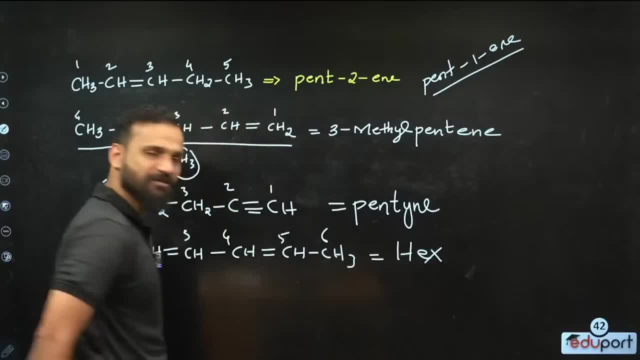 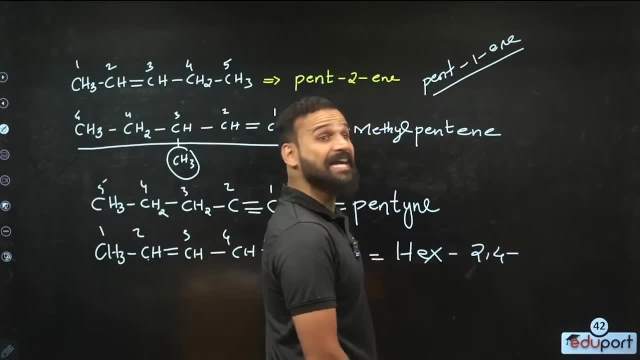 Since the longest chain is R, we can call it HEX, HEX. There are double bonds in both of them and four, So 2, 4.. What DI? There are two double bonds, right, DI-INE. So what is the name? HEX? 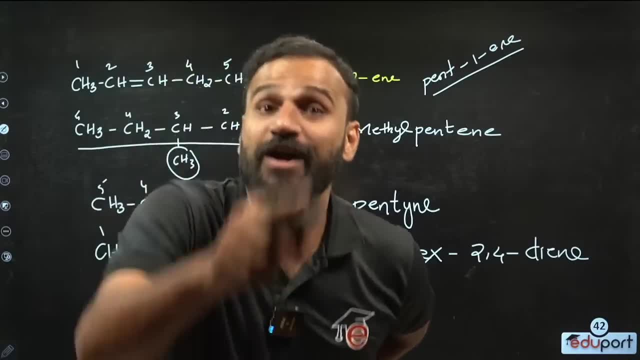 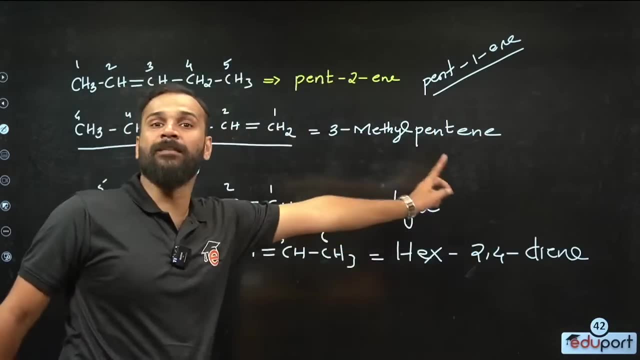 2, 4, DI-INE. HEX 2, 4, DI-INE. This is very, very important. What is it children? HEX 2, 4, DI-INE. HEX 2, 4, DI-INE. 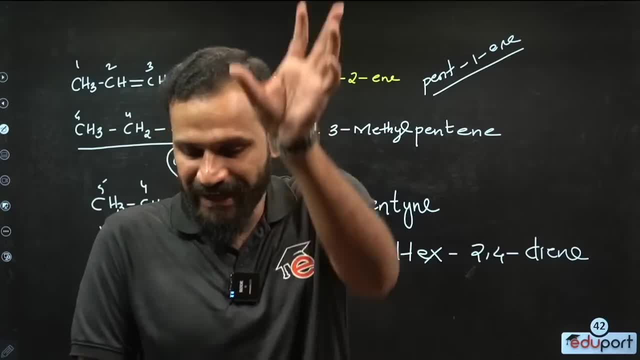 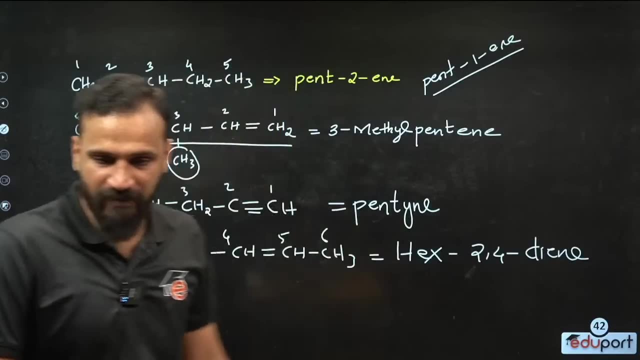 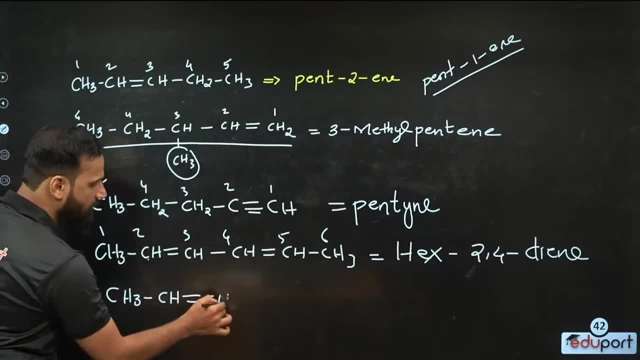 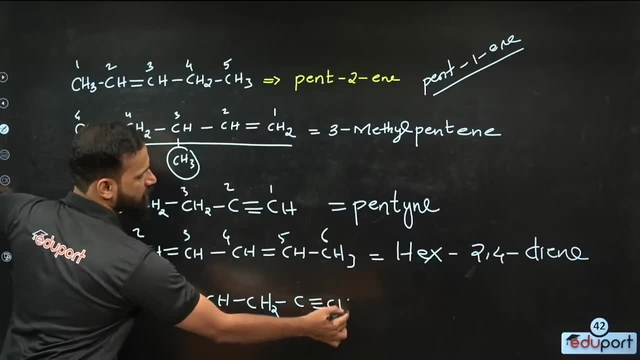 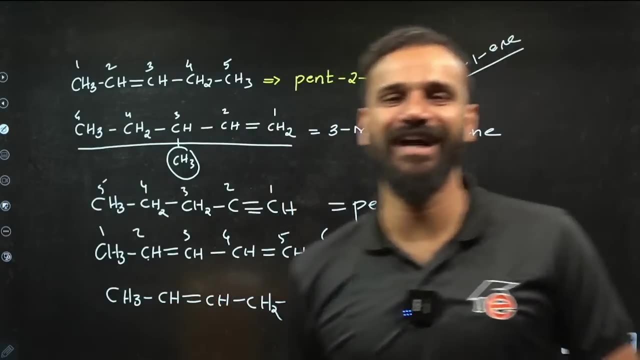 CH3, CH3.. CH double bond, CH single bond. CH2 single bond, C triple bond, CH. Think of giving such a compound. Think of giving such a compound. Do you know a good question about such a compound? Here there is a double and 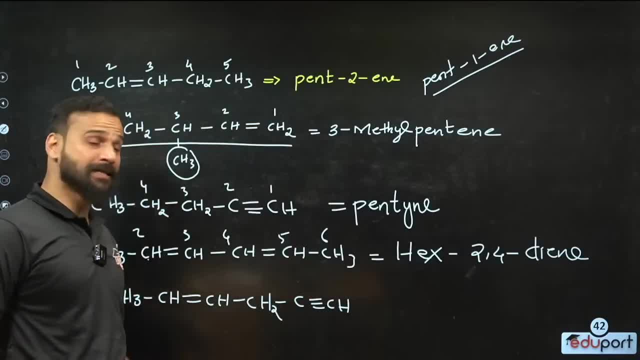 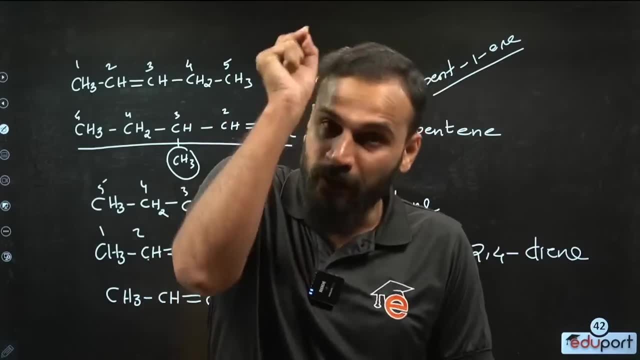 a triple. There is a double in one compound and a triple. When that happens, what do we do, children, When there is a double and a triple in one compound? what do we do When there is a double and a triple in one compound? what do we do? 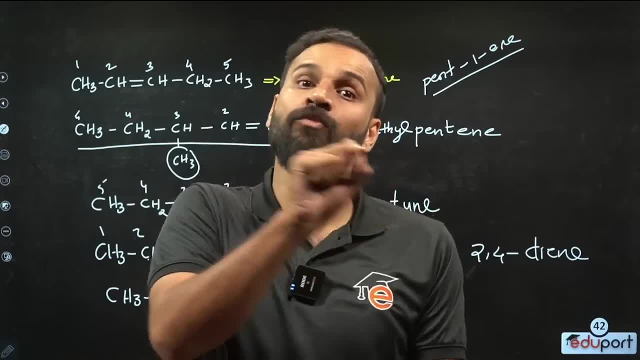 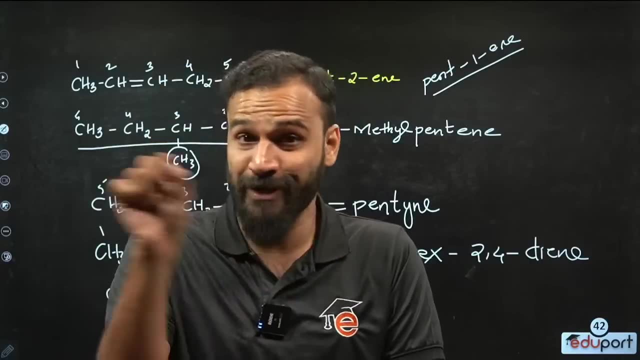 Double bond should be numbered in the form of the least number Because when you look at the priority order, there is a double bond priority than the triple bond. You have to pay attention to the number. So look if you make a number from there to here. 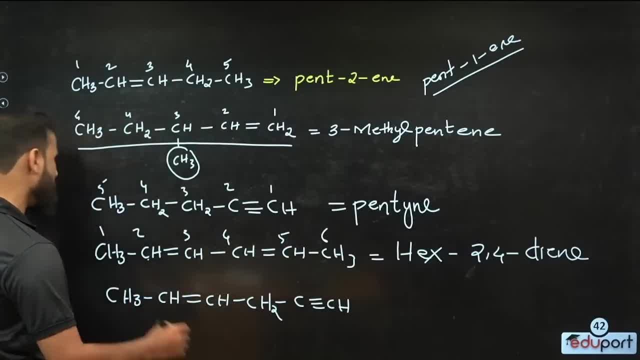 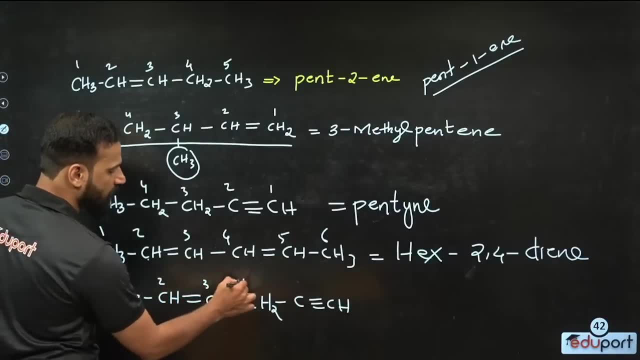 you will get a triple bond least. If you make a number from here to there, you will get a double bond least. So when you make a number, you have to get a double bond least, because the priority is double and that's how it goes. 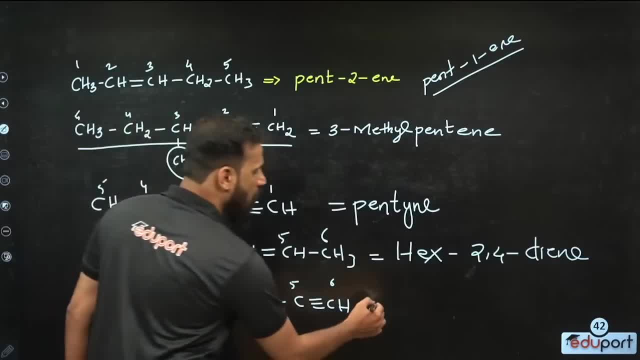 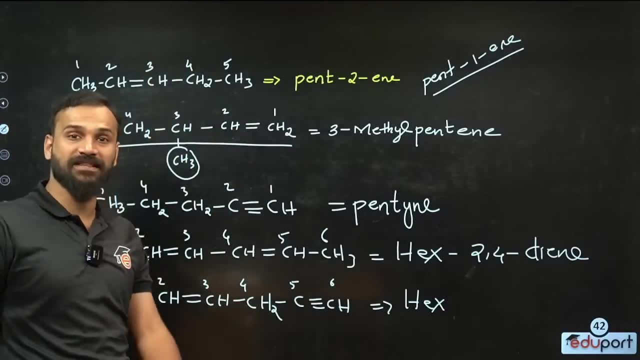 1, 2, 3, 4,, 5, 6. it goes like this, Since the longest cable is R-carbon 1 hex, But the name should be finalised by the triple bond itself. So what is this? 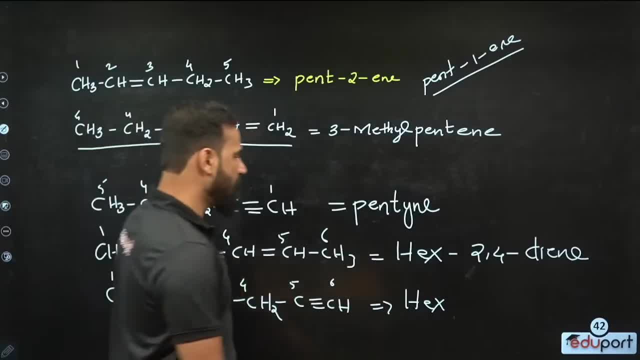 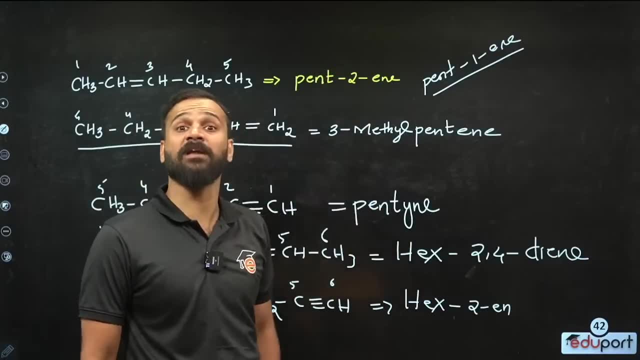 The second position of the hex has a double and in 5 there is a triple, So hex 2e. Usually e is not e-n, It is e-n and the name does not end. It is not the end of the name. 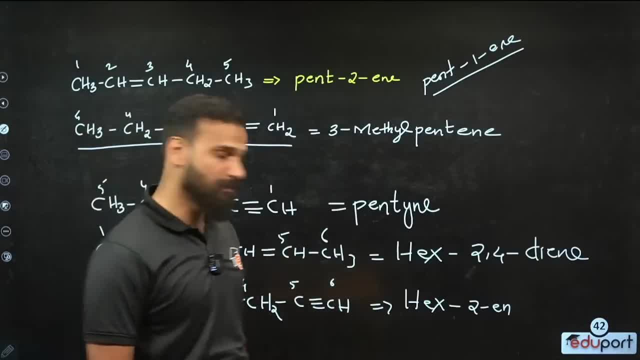 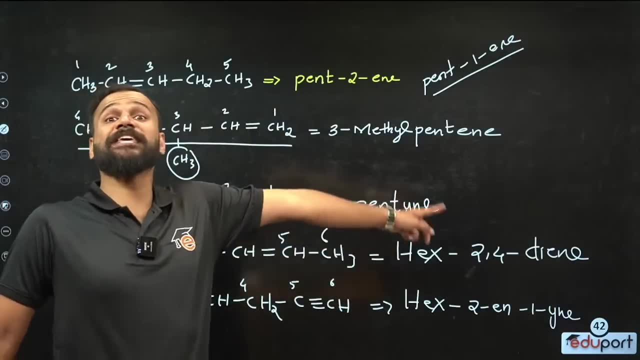 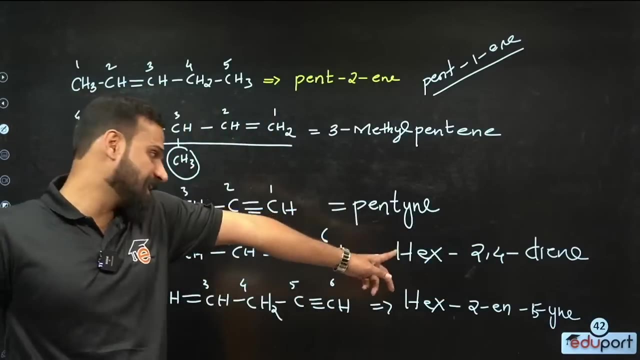 In the first position: triple bond, So one, nine, Let's say one nine, So hex, two in- sorry, not one, not five. there is a triple bond, So five, nine, Hex, two in five, nine. There are five triples, So five. 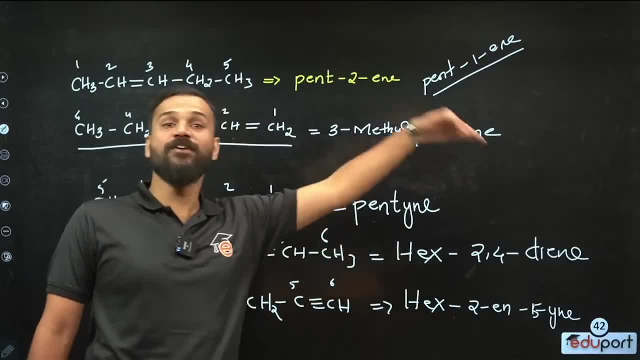 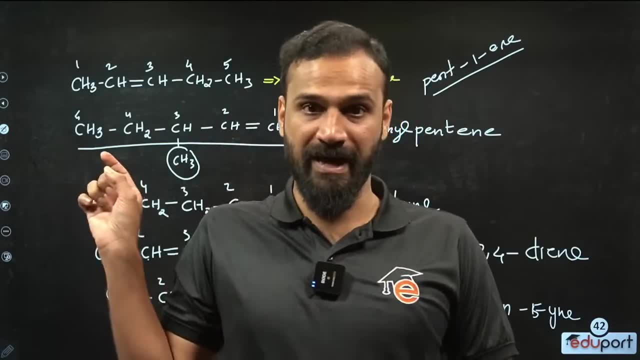 nine is not one. nine Hex, two in five, nine Give that name. So if there is a double and a triple, do the number in the form that the double gets the least number. Then you have to make the name end with the YN. 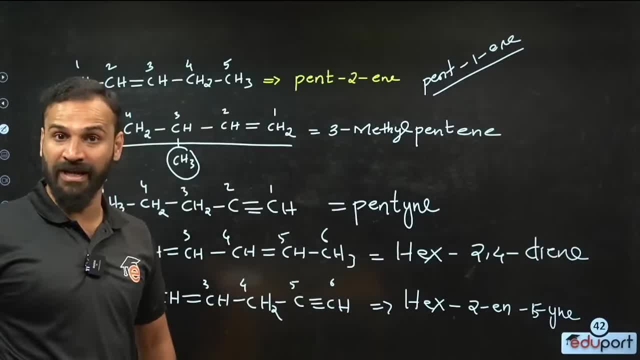 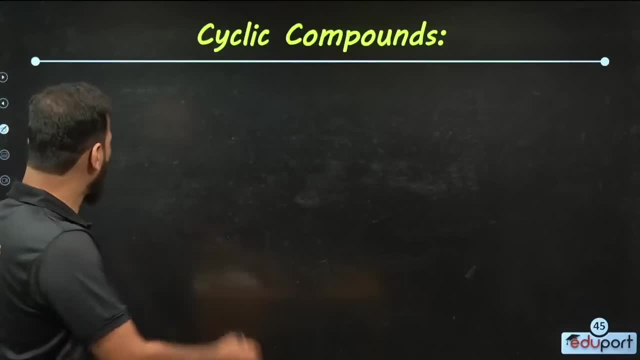 So that's how it comes. So all this should be known to the children. The questions can come in this form: Previous times asked what Naming? asked: How do you name your children when you come to cyclic? Look Look at this. Who is this? Who is this? This is a cyclic. You know, when you see it, If it is cyclic, it will say cyclo Cyclo. How many corners are there? Three, So three carbon. Then the name was given as prop Prop, All single bond Then added, So its name is cyclo propane. 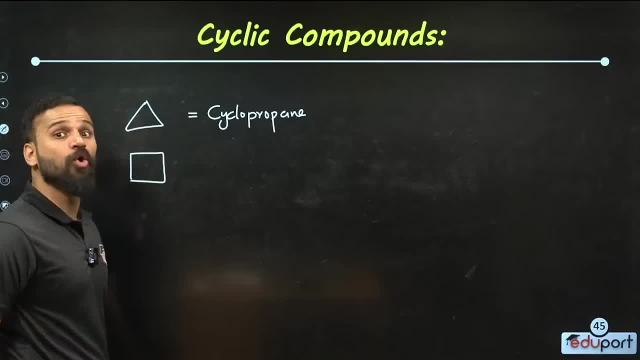 So you say: what is the name of this? Cyclo butane? So you say: what is the name of this? Cyclo pentane? So the name of this? you say it is called cyclohexane, right, Everyone? 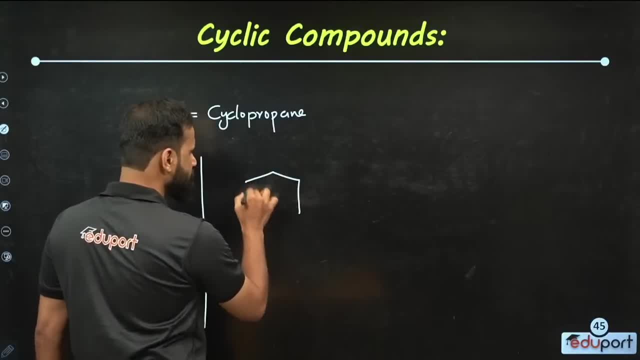 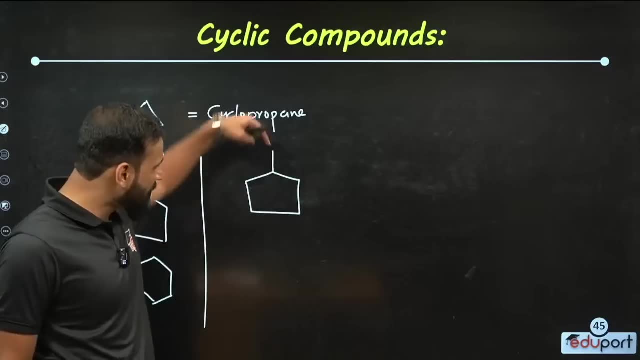 can say it. That's it, Let me ask. look at the children. Who is this? Who is this? This is cyclo pentane. One of its carbons is given like this, That is, there is methyl here. right, Methyl is good, right. 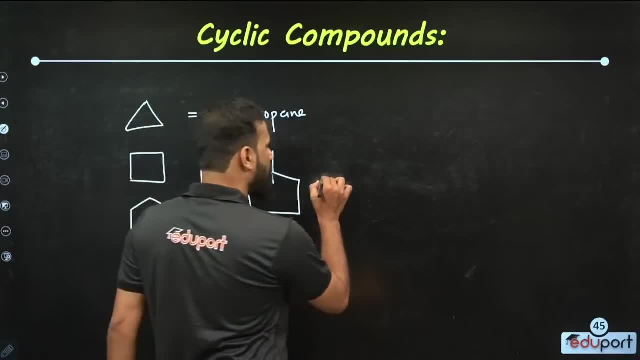 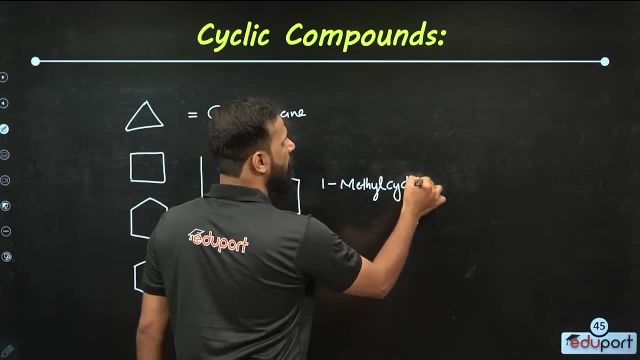 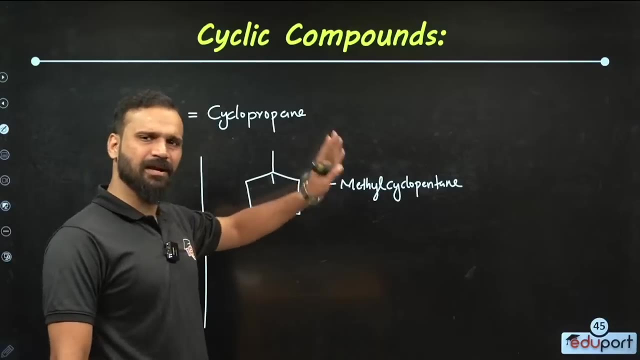 So there is no need to say that it is the first carbon, right? So one methyl, one methyl cyclo, one methyl cyclo ah, pentane, cyclo pentane, Or you can say methyl cyclo pentane, Isn't it? If there is only one methyl, there is no need to say that it is the first. 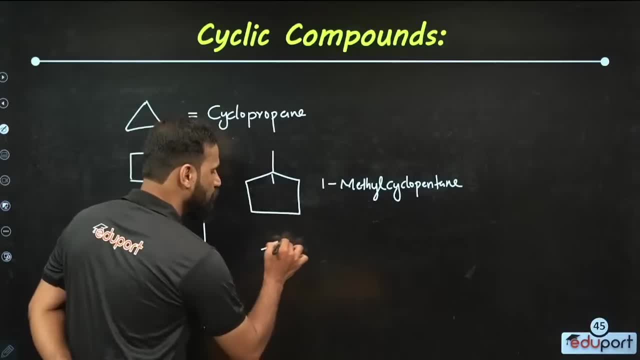 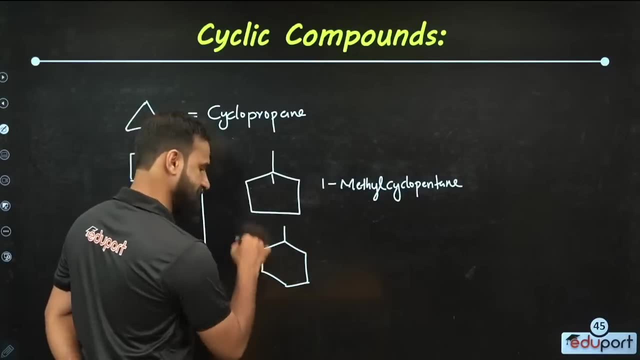 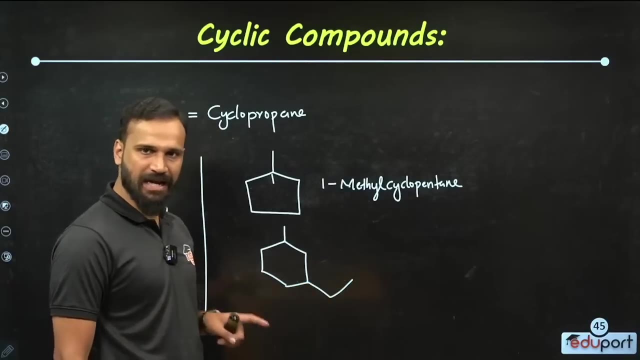 position: Look at this, children, Look, Look, Who is this. Who is this? Who is this? This is a cyclohexane. This is a methyl here. Who is this here? Here is a methyl Here. there Va. there are two carbons, right, So look, here is methyl, here is. 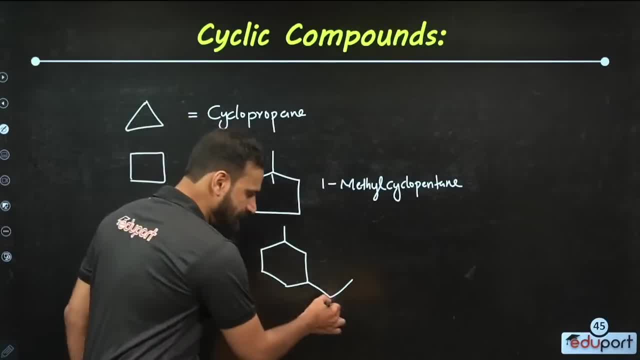 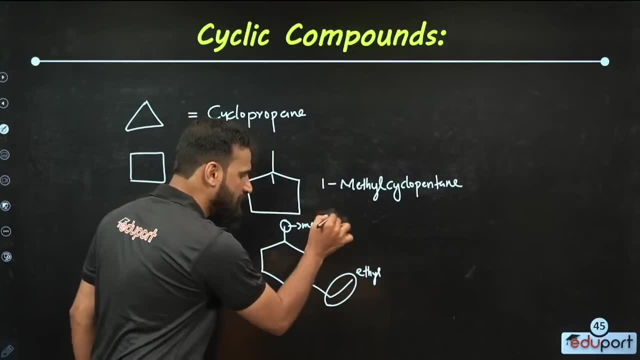 methyl right. The first in the alphabetic code is Ethyl. This is the Ethyl. Who are these Ethyls? Okay, who is here? Here is methyl. The first in the Image Icon is Ethyl right. Then I have to say Eожал trip diminish. 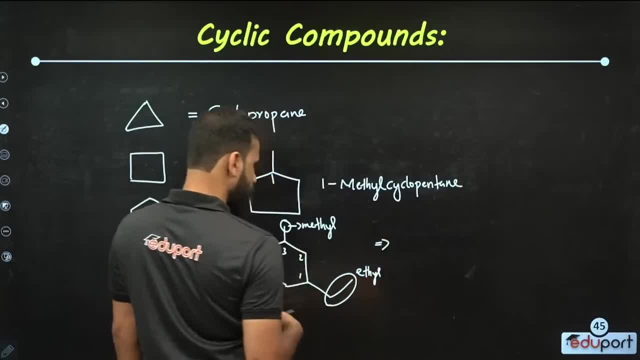 one, two, three. So what is it? Uh, in the first position, Ithail, in three of the methyl, only one, two, three. then what? The first position is Ethyl and thee in three is Methyl. So one Eotyli is Methyl. 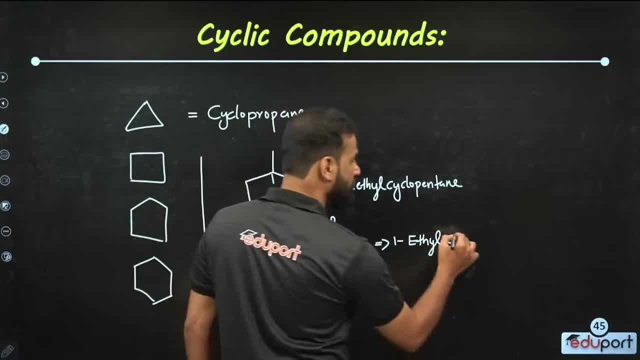 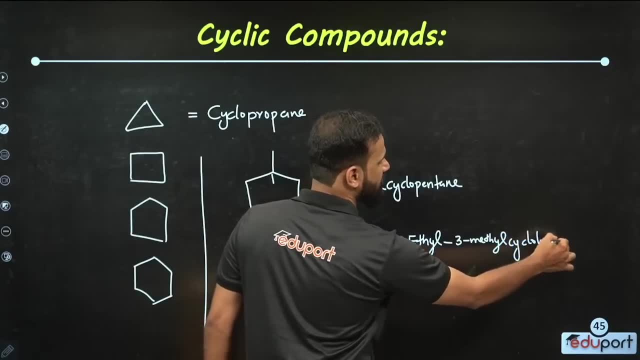 Thail. Then you guys, then you guys: three, three is Methyl, Methyl. Then you guys: longest chain: Cyclohexane. What are you guys? Cyclohexane? Give the name like this, So you should know the name of Cyclic. 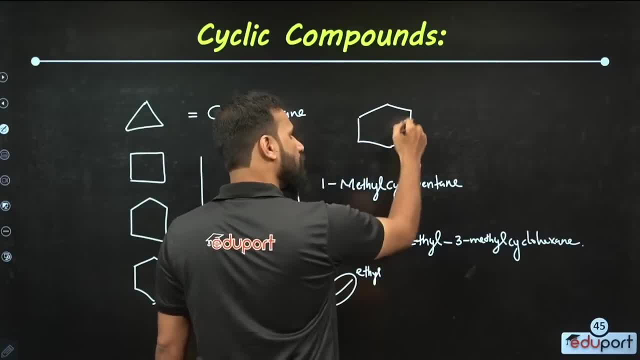 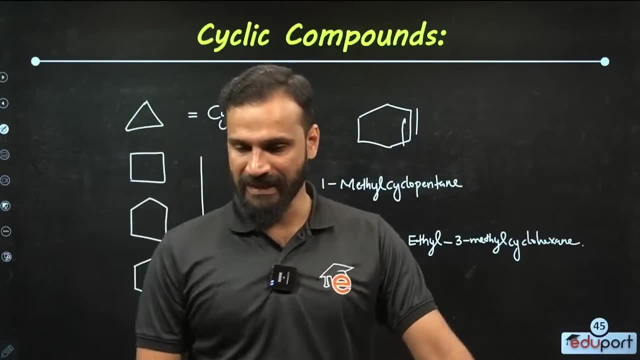 Then look, who is this? Who is this? Cyclohexane- If a double bond comes, Cyclohexane. If it is tripled, Cyclohexane Will give all this. We all know all this. What can we do as a cyclic Can name: 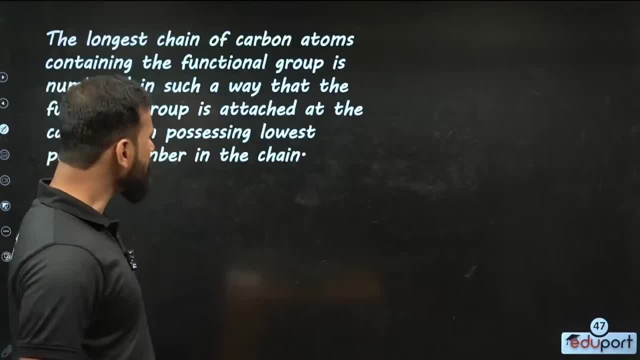 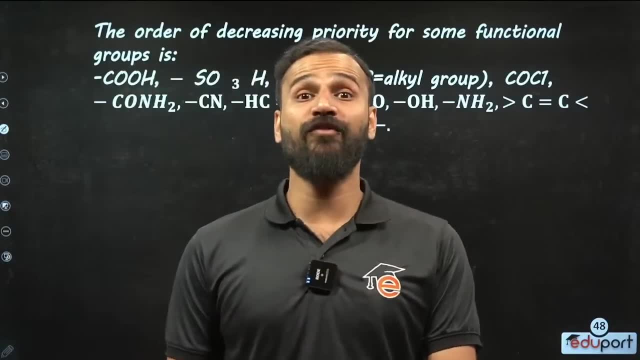 Must have connected. Move on, guys Functional. How will we name the group when it comes, When the function group comes for the first time? We must know First we must know the priority list of the functional group. We need to know: Look most priority. 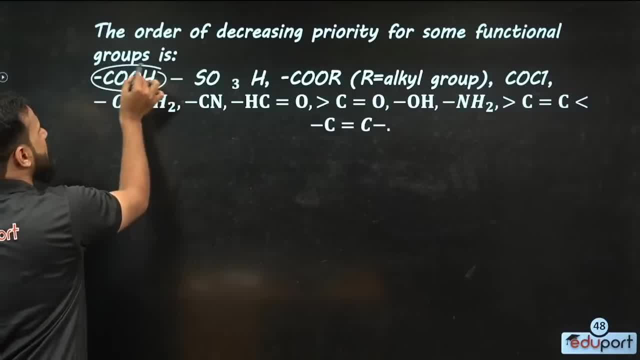 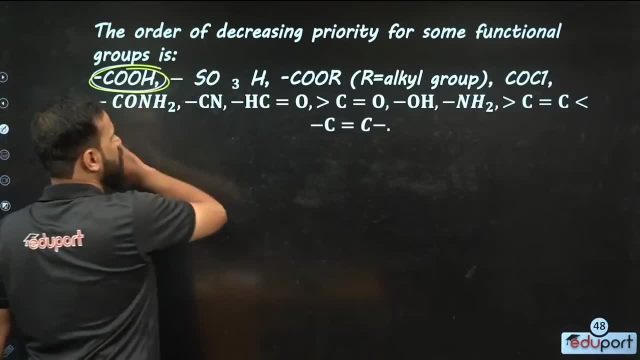 Acid. This is the most important This list. If there are those who do not know this order Can write it. it It can be learned. Look acid. Then that is sulfonic acid. Then this is acid. How much explicitly it can be written? Then it is sulfonic acid. 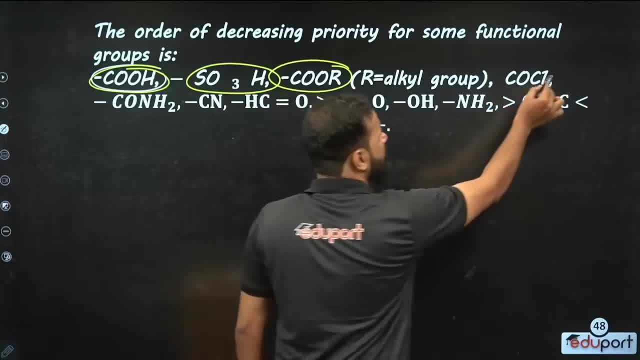 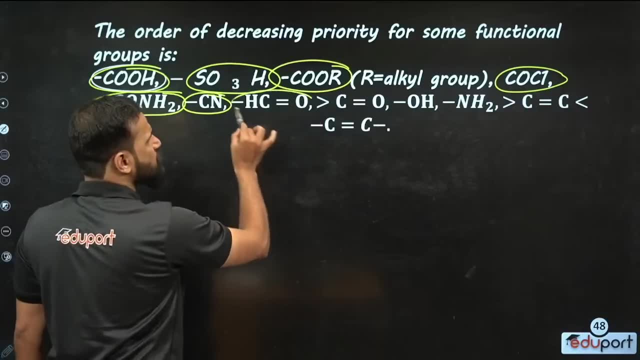 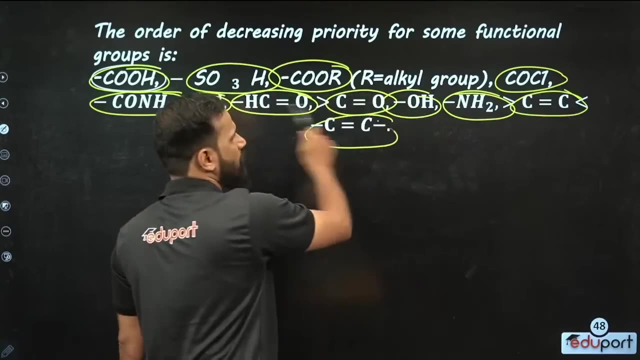 What is it? It is ester, After that it is acid chloride, After this it is acid amide, Then it is cyano group, Then CHO, is aldehyde, Then ketone, Then alcohol, Then amine amino group, Then double bond and triple bond. 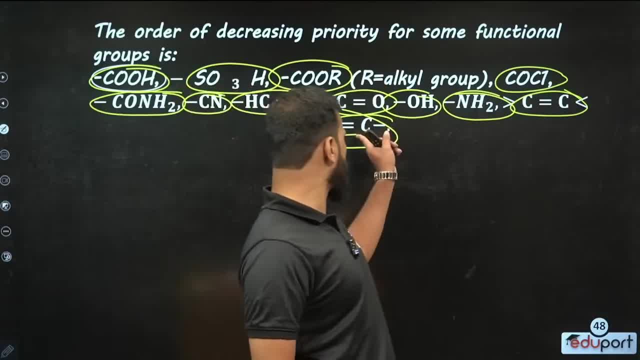 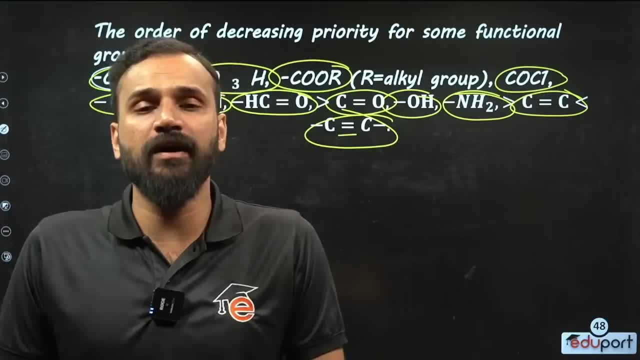 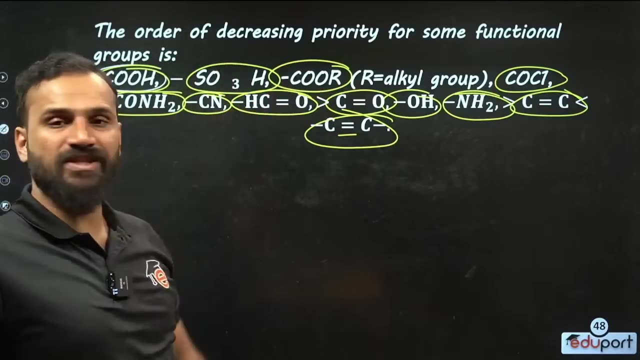 Ok, This is the triple bond, So the priority is more than the triple bond, double bond. So you can definitely learn this order, Because when the name comes to one or more functional groups, who should get the preference? today We look at the basis of this order. 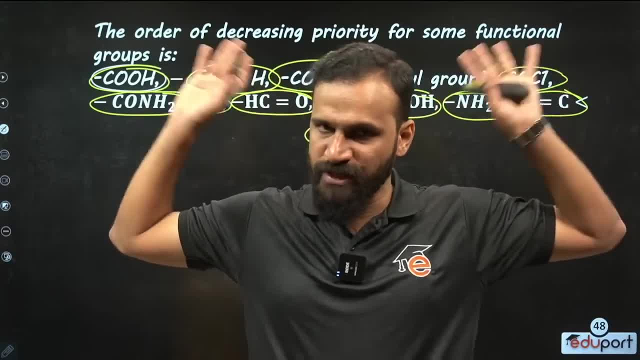 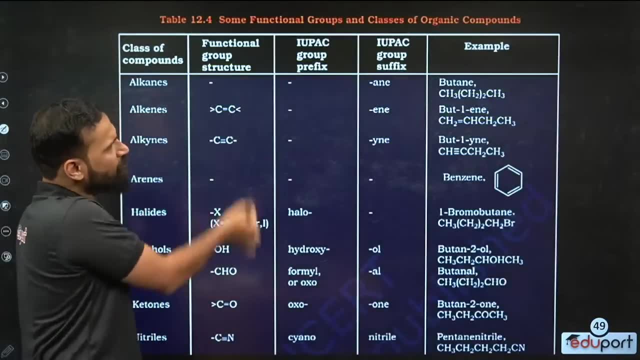 So those who do not know this do not have a doubt that it is written. Only if it is written, the compounds in the functional group can be named. Now we have to know the children. Each functional group has a prefix and a suffix. 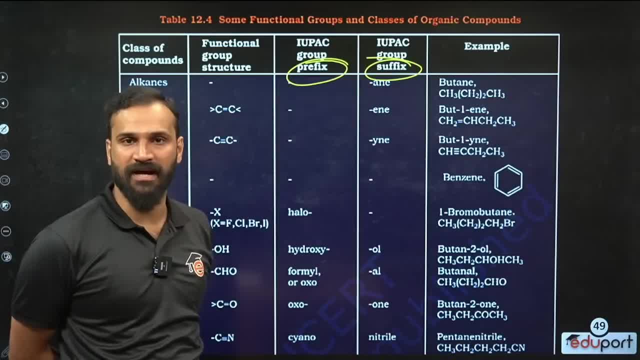 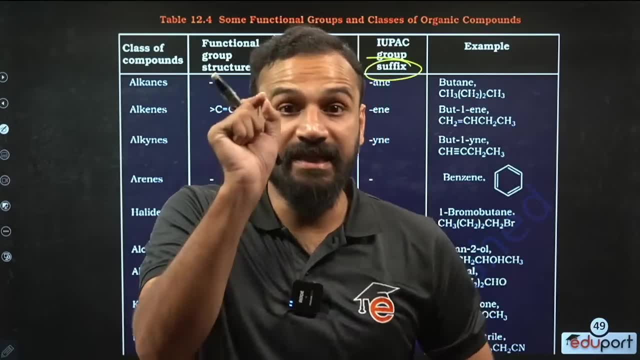 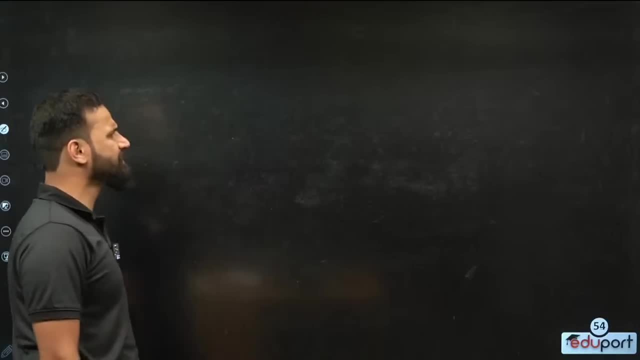 We need to have a clear idea about it. What is the prefix of each functional group, The suffix of each functional group? What is it? What we should know clearly is an important thing: here We have given each perfect and suffix, etc. The prefix and suffix are very important Look. 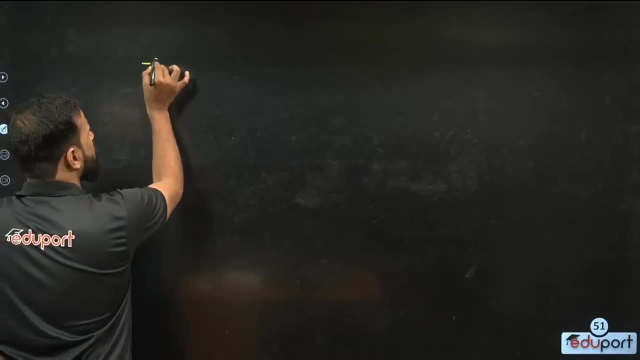 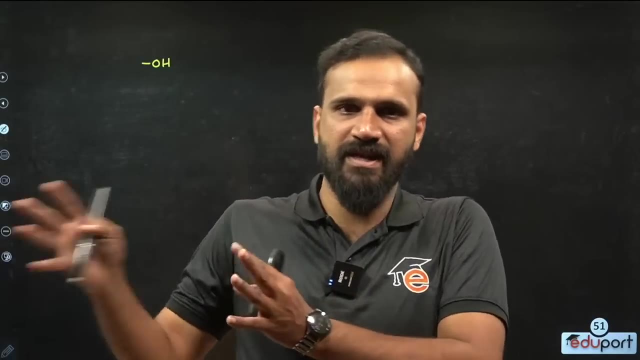 Of course the function we usually use for that is OH, Alcohol. Alcohol is a suffix that comes at the end Is suffix First is the prefix. Who is the first? we don't know the root of meth ethyl and propyl. The root of meth ethyl propyl is: 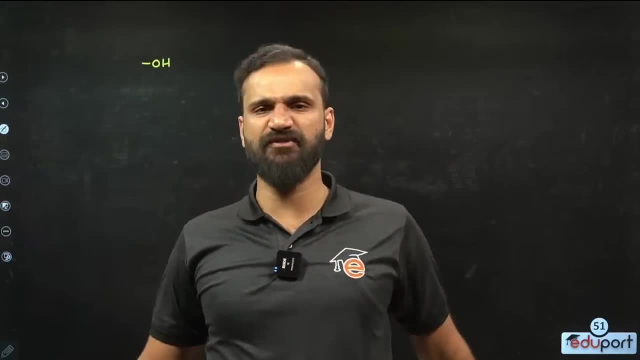 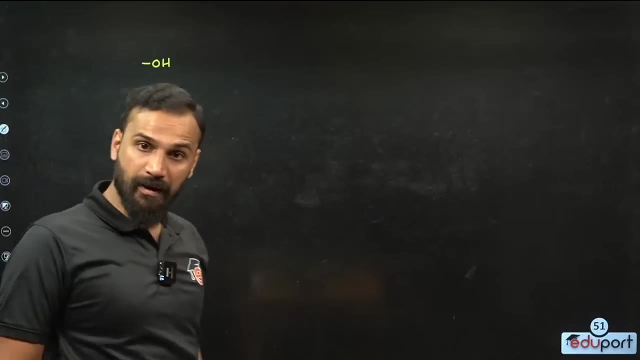 root word right. The suffix comes at the end of the root word. The prefix comes before the starting of it. So when does OH become a prefix? When does it become a prefix If there is a person with a priority over OH in that compound? 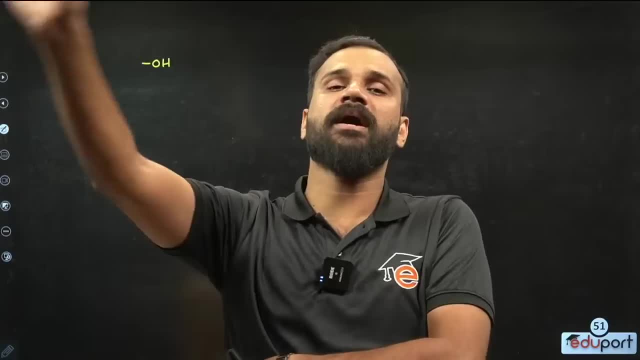 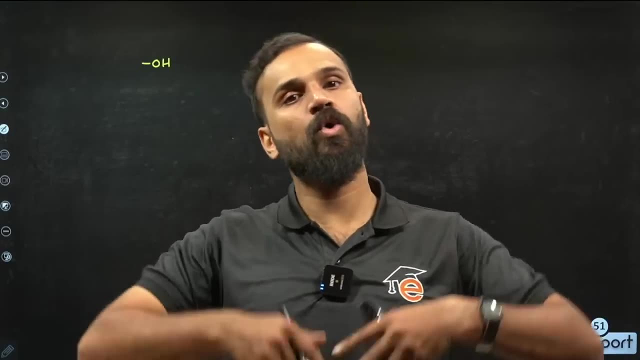 the suffix will be the person with more priority, The rest will become a prefix. Okay, Now there is only OH in an organic compound. So what is OH? OH is a suffix. In an organic compound there is OH, COOH and ACID. 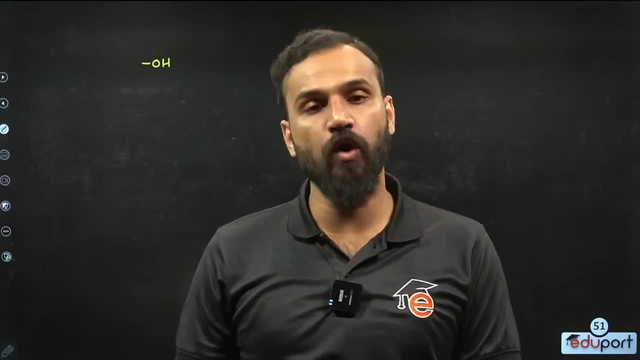 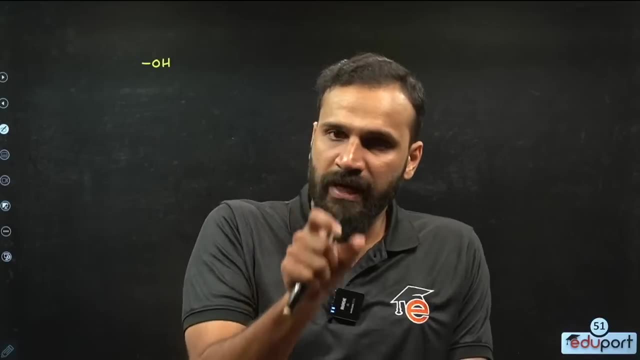 So we know right: The one with more priority over OH is COOH and ACID, So the suffix is ACID. So what is OH? It is automatically a prefix. So what is the prefix and suffix of a functional group? 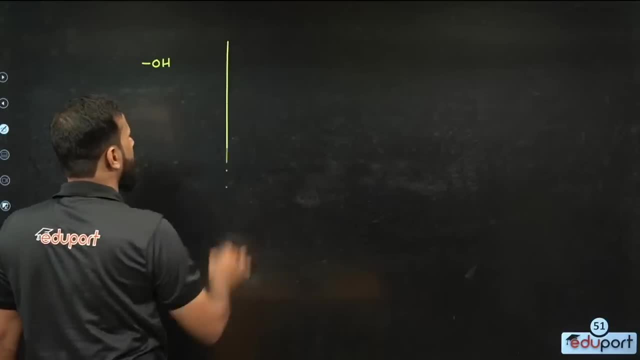 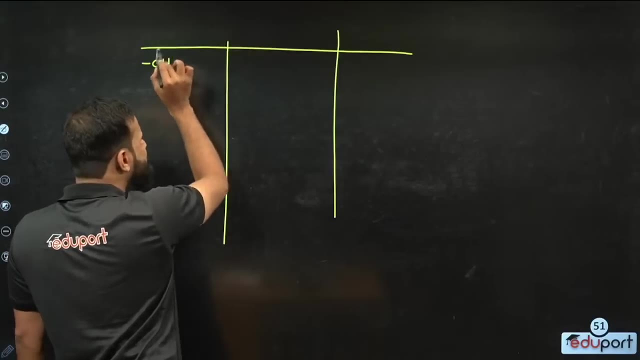 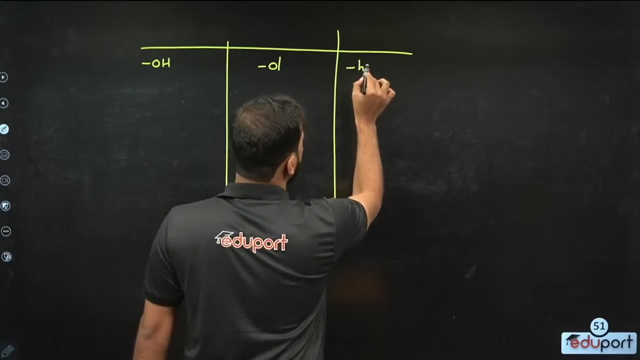 We need to learn this first. Look, I will give you an example. Look, Our functional group is OH. When OH becomes a suffix, we say OH. When OH becomes a suffix, we say HYDROXY When OH becomes a prefix. 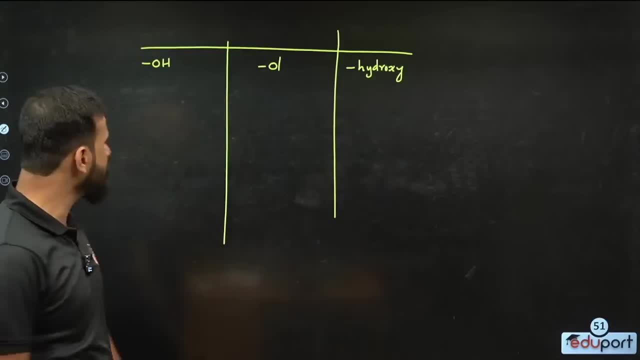 we say HYDROXY. What do we say? We say HYDROXY. We should know this. Our other functional group is ALDIHYDE. When OH becomes a suffix, we say AL METHANAL. 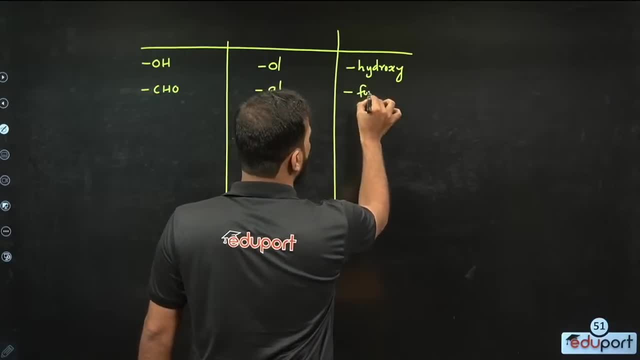 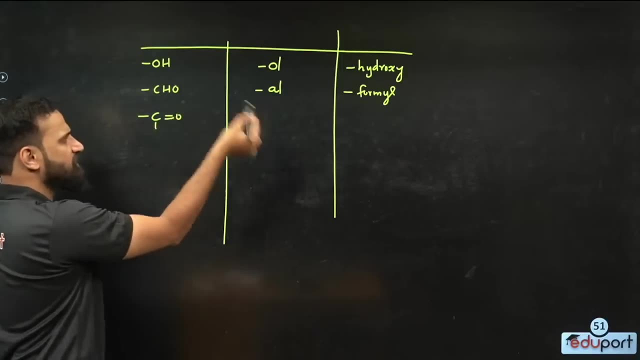 ETHANAL PROPANAL. When OH becomes a prefix, we say FORMYL. What do we say FORMYL? Now? the one we always use is KETONE. When KETONE becomes a suffix, we say: 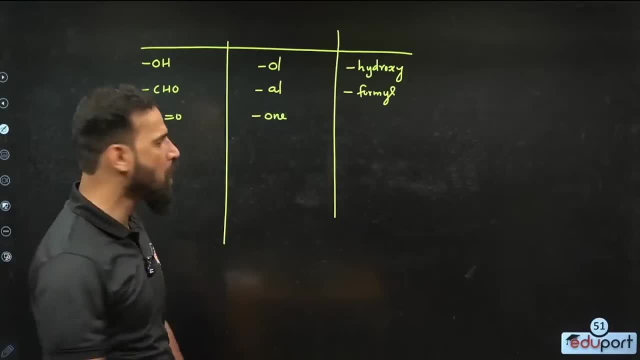 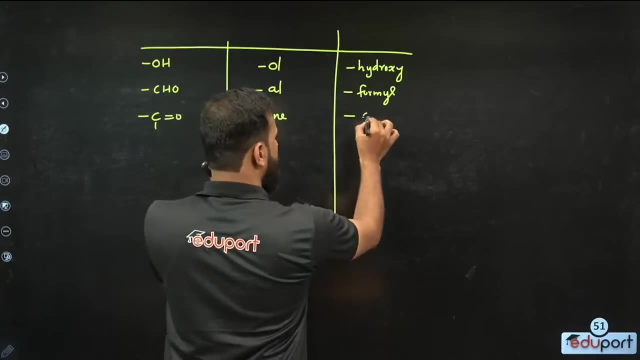 ON PROPANONE, BUTANONE, HEXANONE. When OH becomes a suffix, we say OXO. What do we say OXO Now? the other material we use is ACID CARBOXYLIC ACID. When OH becomes a suffix, we say OECACID. What do we say OECACID? When OH becomes a suffix? we say CARBOXY. What do we say, CARBOXY, When OH becomes a suffix? 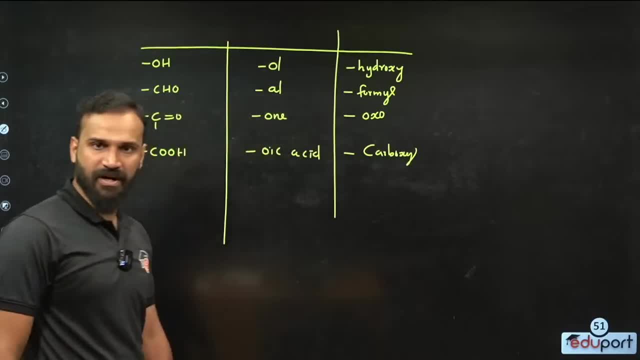 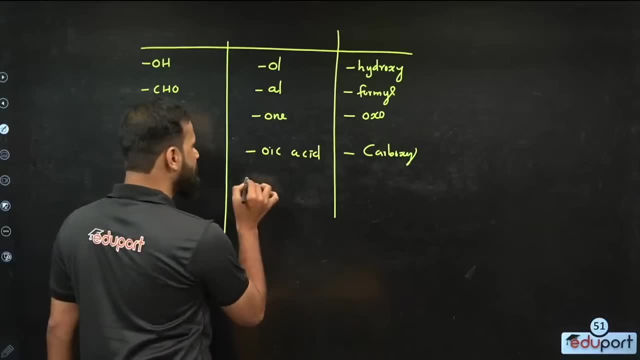 we say CARBOXY. What do we say CARBOXY Now? the one we usually use is NH2.. NH2. AMINE. It is an amino group. When OH becomes a suffix, we say AMINE. 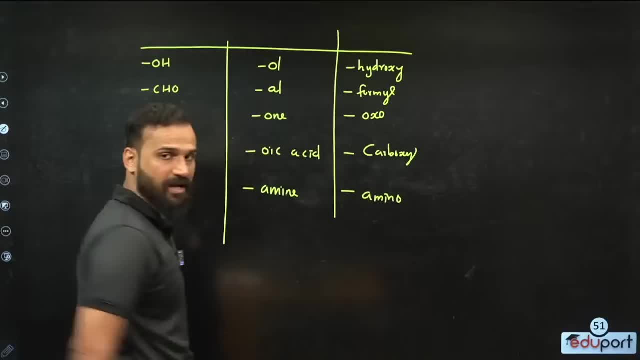 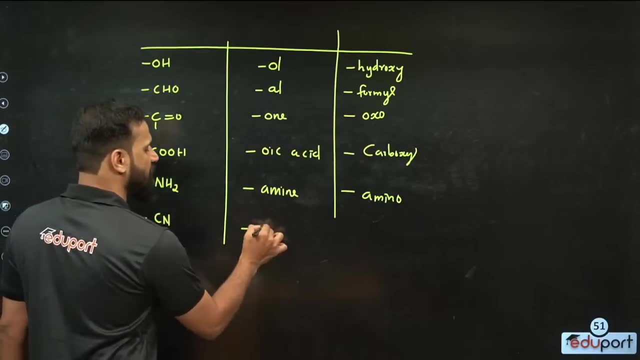 When OH becomes a suffix, we say AMINO. What do we say AMINO? Now, the one we know is what CN? When CN becomes a suffix, we say NITRILE, NITRILE. 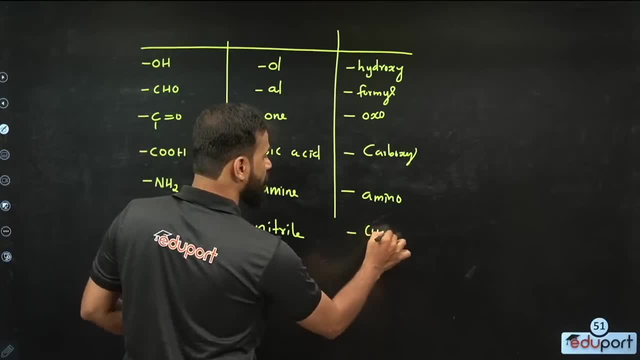 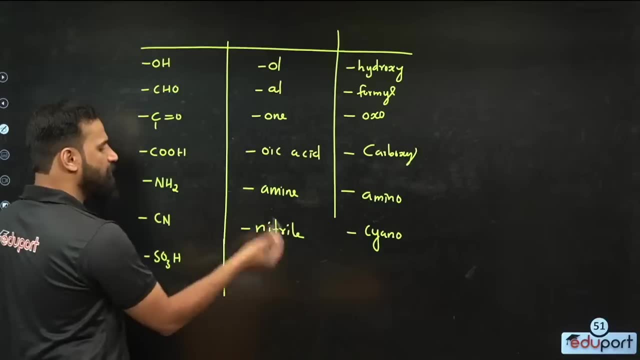 Similarly, when OH becomes a suffix, we say CYANO. What do we say? CYANO, Okay. Similarly, SO the sulfonic acid, SO3H, we always say sulfonic acid. What do we say? We always say: 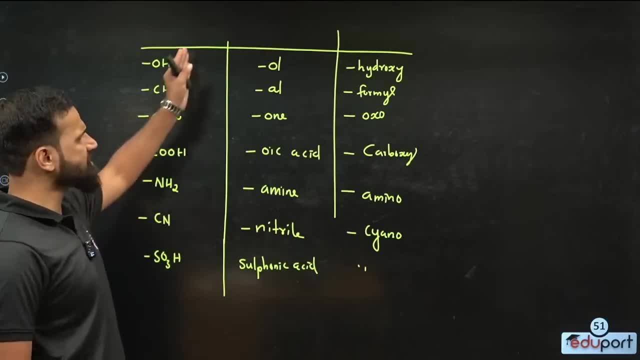 sulfonic acid: See. So these are the ones we usually use as functional groups, Then HALOGEN as well as NITRO GROUP. their characteristics: we always use them as well as METHOXY GROUP. 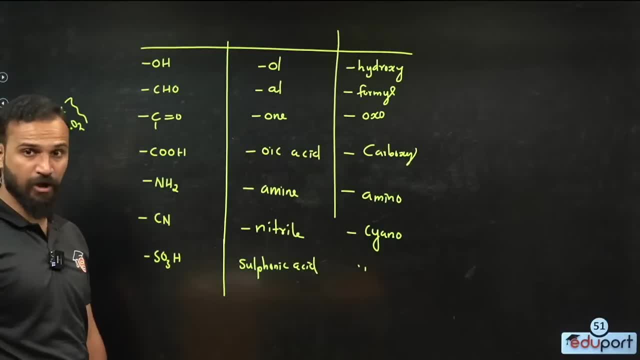 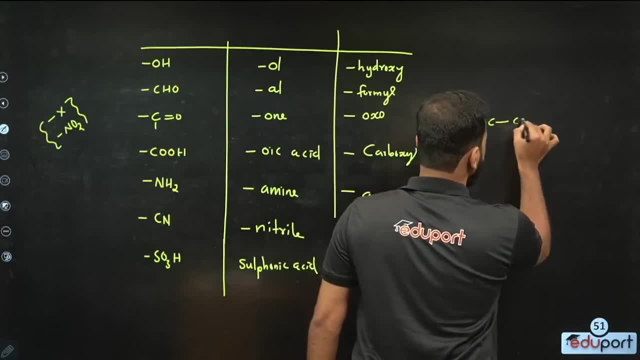 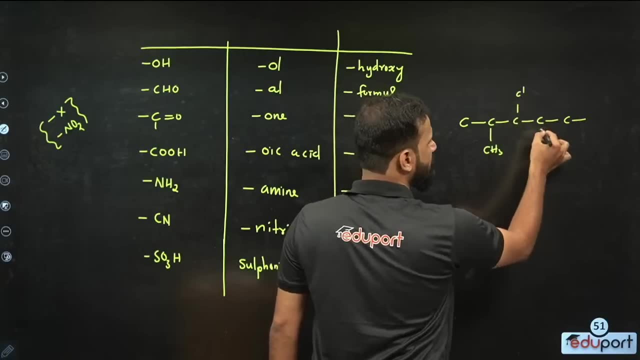 and, as a suffix, If there is an alcohol, we should know what its prefix is. Now look, there is a carbon chain. There is a carbon chain In that chain. there is a CH3 GROUP. there is a CL. 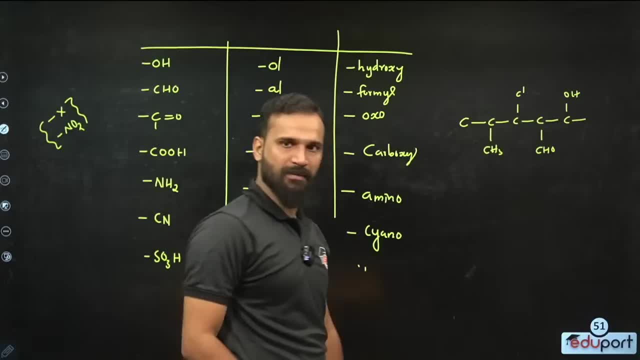 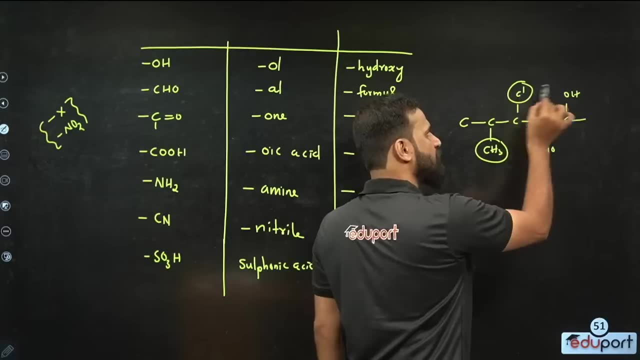 there is a CHO, there is an OH. Imagine there is a HALOGEN. We are explaining to understand, So we know. this is a branch, This is a- how can I say- a FUNCTIONAL GROUP. This is a FUNCTIONAL GROUP. 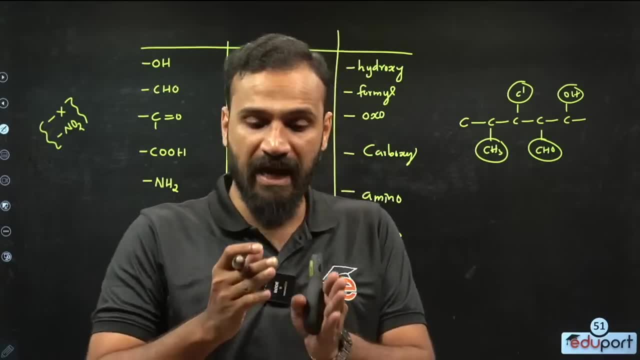 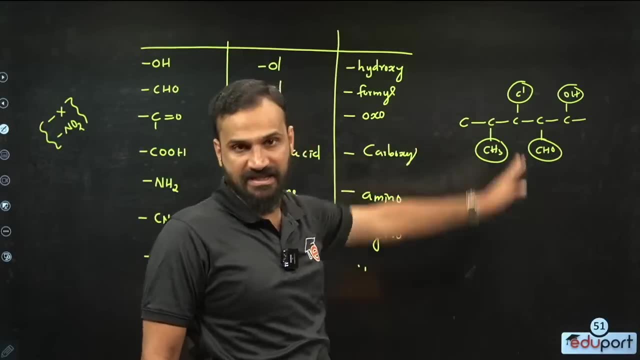 that is a FUNCTIONAL GROUP. who is the suffix in this? The suffix means that the name does not end with the suffix. If you ask who is the suffix, it is the suffix whose priority is more. So you have to look at the priority order earlier. You know, you know. 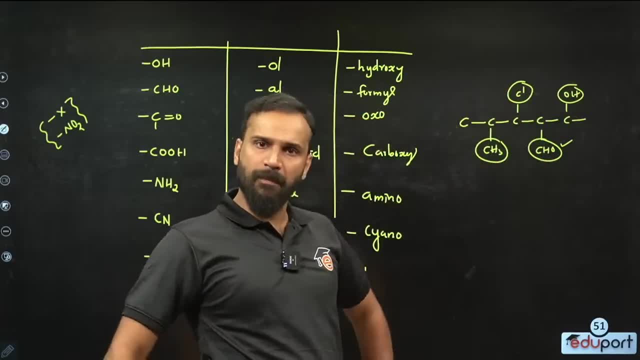 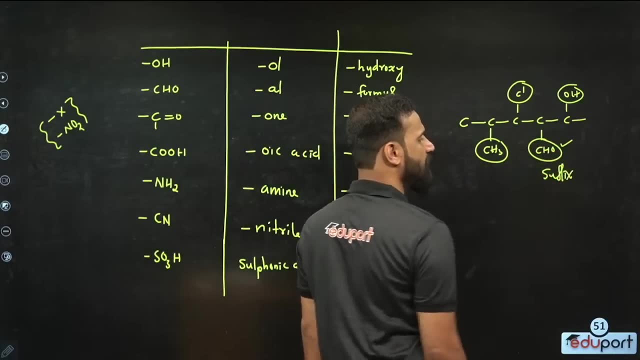 aldehyde has more preference than alcohol and halogen. We said that halogen is always used as a prefix. So what did this person change there? What did he change? Changed to suffix, So automatically. what did he change? Changed to prefix, What did he? 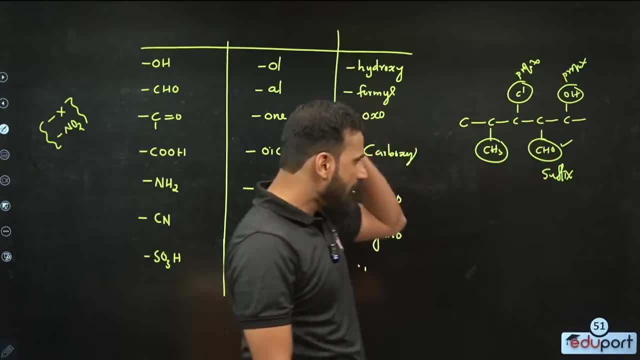 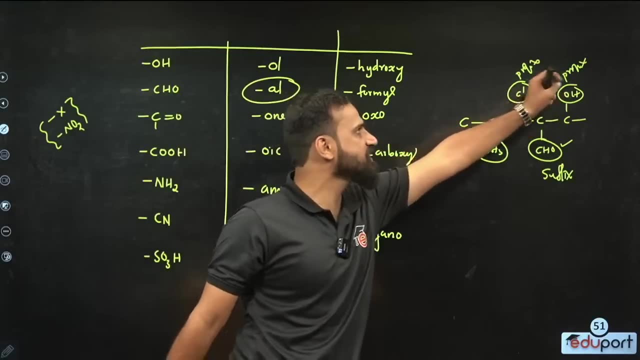 change, Changed to prefix. All this has changed to prefix. So we know that if aldehyde is a suffix, the suffix of aldehyde is said to be a. So OH is a prefix, So we use it in all. Hydroxyl is used for it, Isn't it? 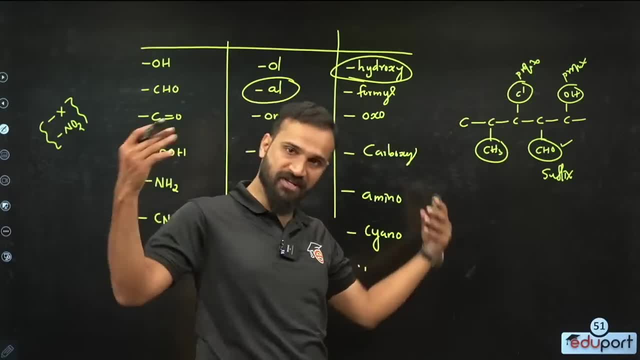 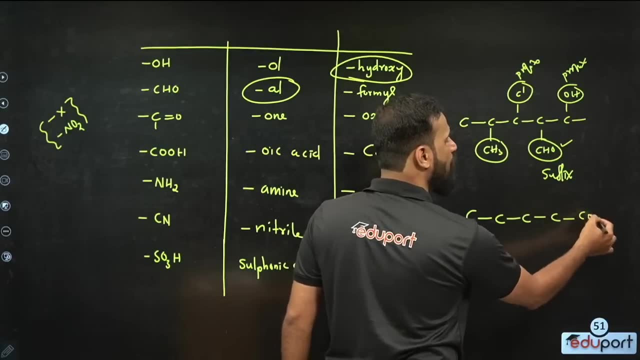 Halogen is used as a prefix. It is always used as a prefix. Now, when we look at a carbon chain, when we look at a carbon chain, there is only a COOH there, Only that, Only that. So he is the suffix, Isn't it? Now, 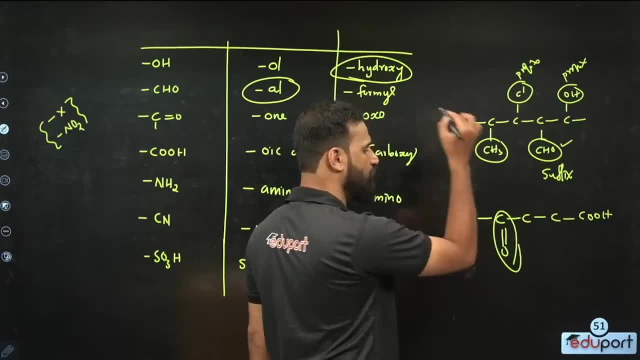 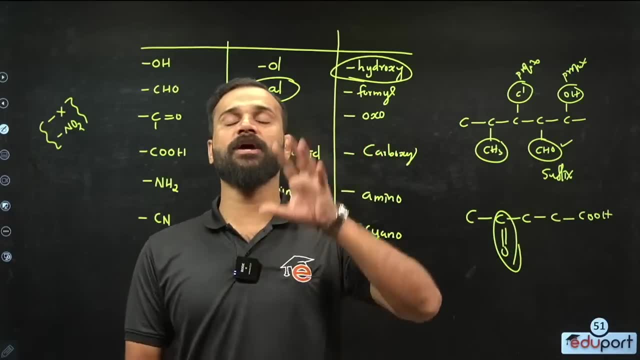 along with that, what to say? a COO, a ketone group, is coming. So then his suffix is because he has no preference than ketone, because he adds acid. So if you don't have the priority list or that order in your 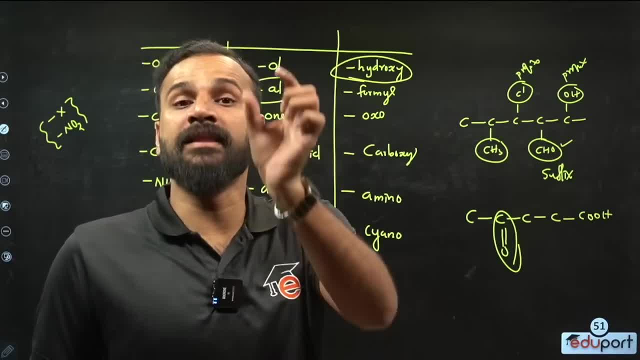 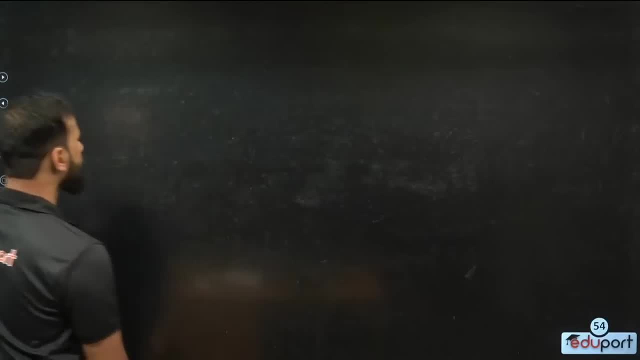 hands, or if you haven't studied it, you can't name it properly. There is a problem, So the children have to pay attention to it. well, Now, look, children, Let's do one or two and see. See C. 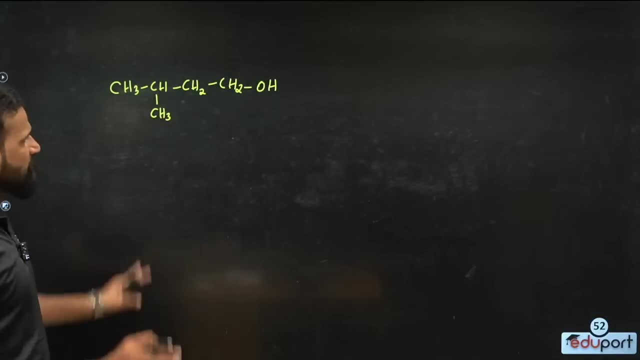 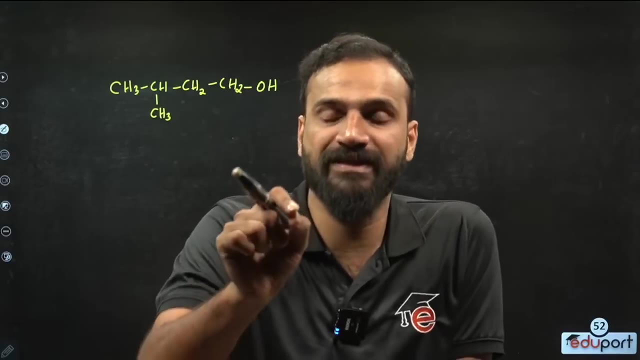 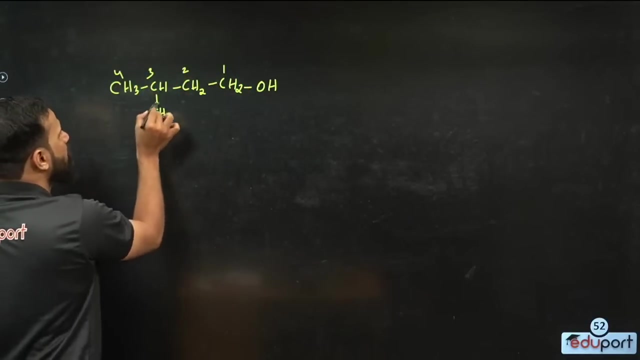 This is what I call it. So here is a functional group. Who O to? It is necessary to do the number in a way that gives the least number in that functional global. That's the rule: One, two, three, four, So one out of three, the other is six. you. 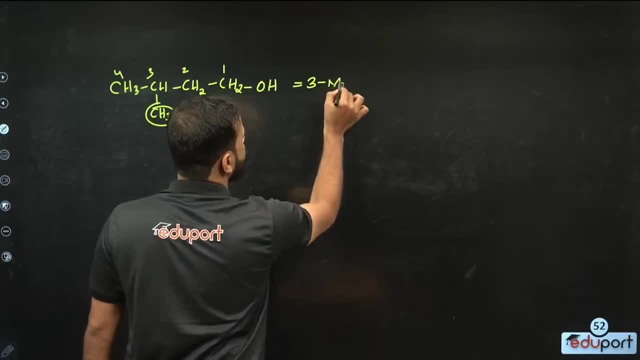 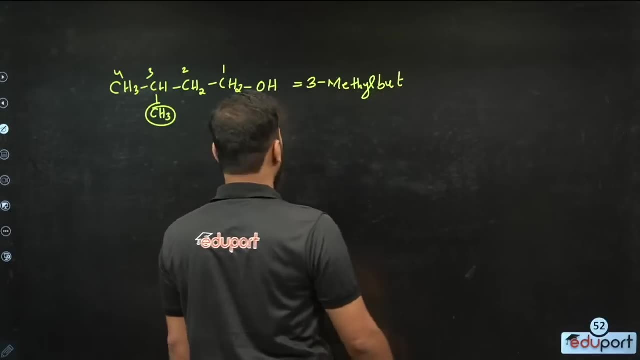 There is a methyl in three. Who is in three? A methyl, Who is in the longest? Four carbons, So butane. What to say in the first position? OH, So butane. Since it is a single bond, butane is given, AN is given. 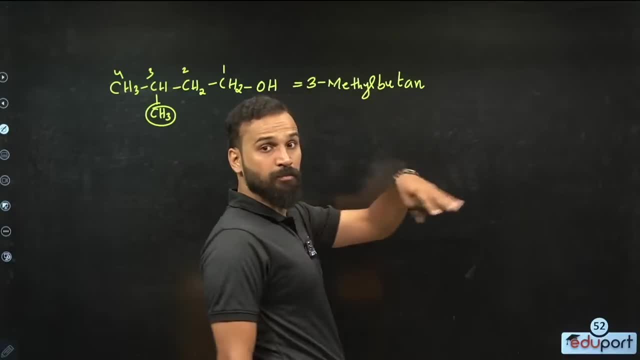 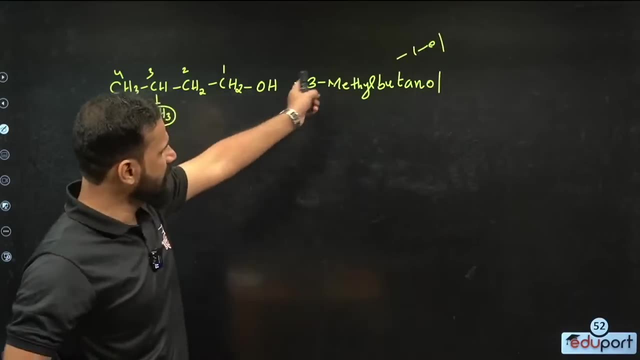 E minus ethanol is added. So because it is in the first position, Butane one, all is to be said. One is not to be specifically mentioned. So butanol is enough. So three methyl butanol, That is his UPSC name. The order of preference here is not to be looked at. 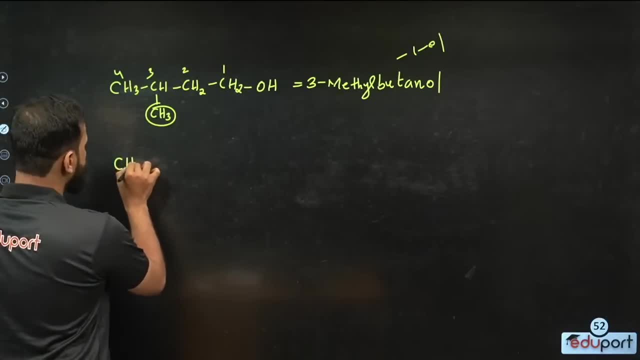 Because there is only one function loop. Now look at the other children: CH3COCH2CH3.. OK, There is a function loop here. CO means ketone. Who is ketone If he gets the least number one, two, three, four? 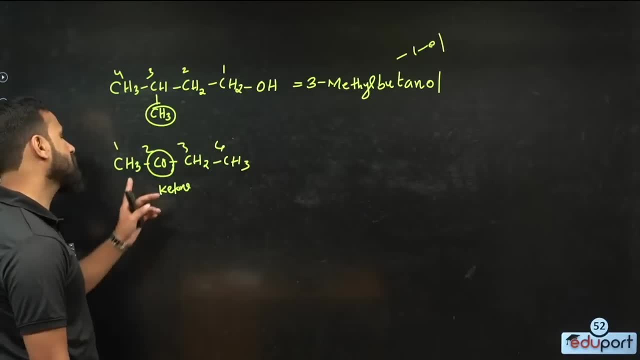 You have to do this number right, So you have to understand. The suffix of ketone is on. So what is it? It is written as bute. OK, OK, bute. Since everything is single bond, we can make it butane. 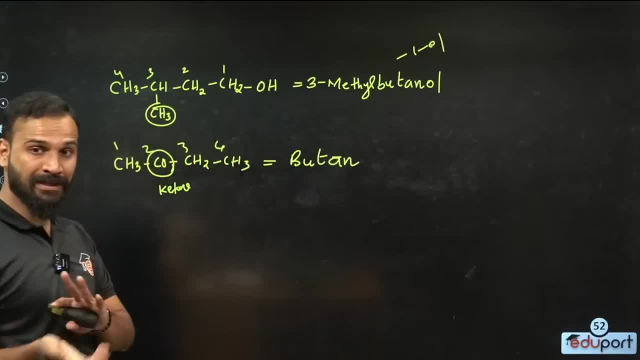 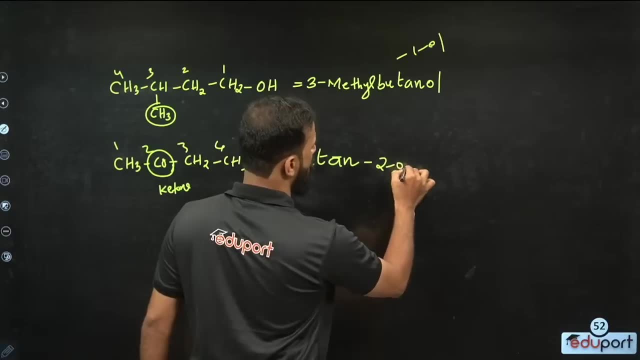 Made it butane. Butane is E minus from butane. Then what is the suffix of this ON? Where is the ON In both? So butane two on. So what is his name? Butane two on. That's why the prefix and suffix are to be studied. 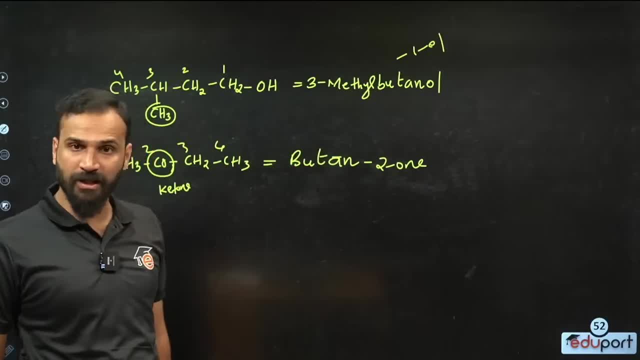 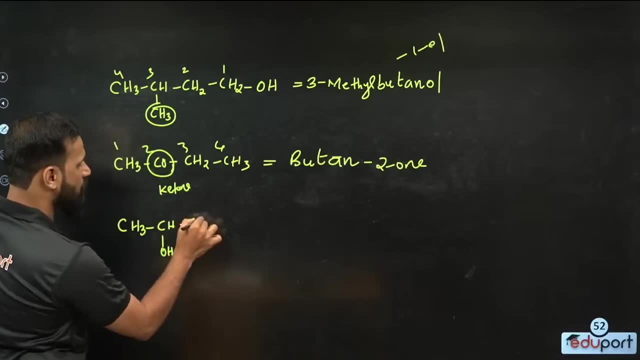 When ketone comes, it is used as a suffix. It is said to be used as ON. OK, Now look at the other children. CH3CHOHCHCLCH2COOH. It will come like this: You have to tell the name of this. 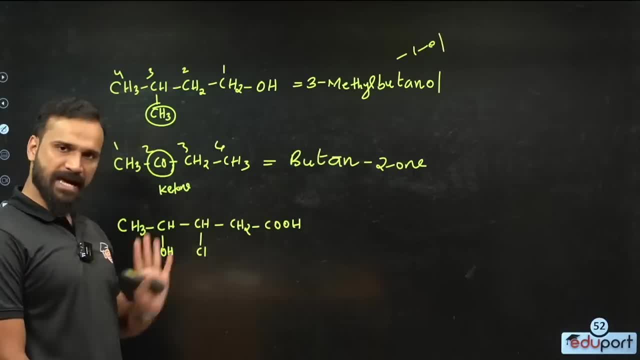 Who is the most priority person in this? It is acid. That person should get the least number. You should have given it once, because it has carbon Right. Then it is on the end. So you should have given it once, One, two, three, four, five. 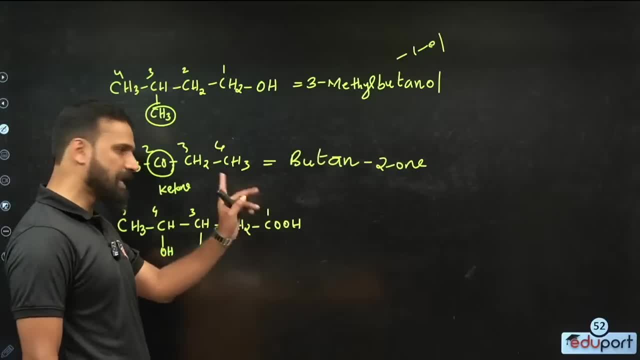 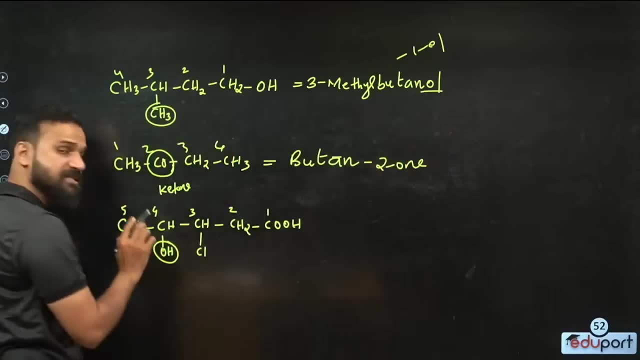 So he is the person with the most priority. He is the suffix. This is the suffix. The rest has become the prefix. So look, If this OH is the suffix, it is all Here. it is not the suffix, it is the prefix. 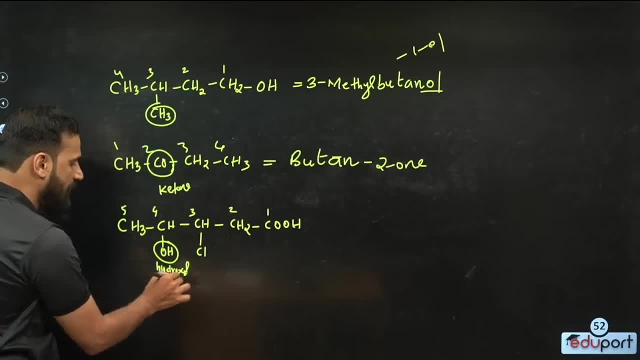 If it is the prefix, it is hydroxy. right, What do you say? Hydroxy? So what? H is the first letter. This is chloro. Chloro means C is the first letter, Right? So is it C or H? 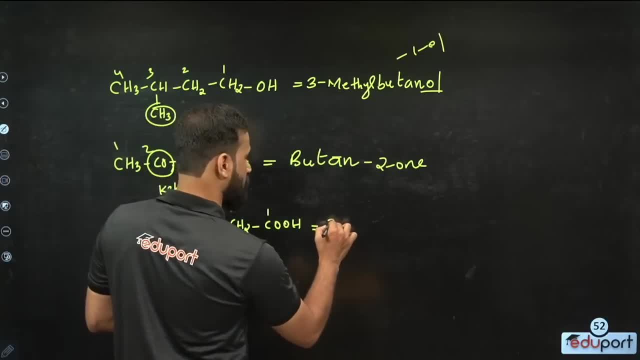 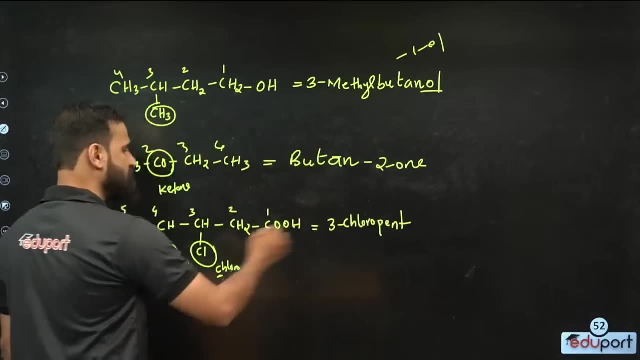 In alphabetical code it is first C, So his name is trichloro. Our name is trichloro. Longest cell has five carbonates, so it is pent. All are single bonds, so it is pentane. The first position is Oic acid. 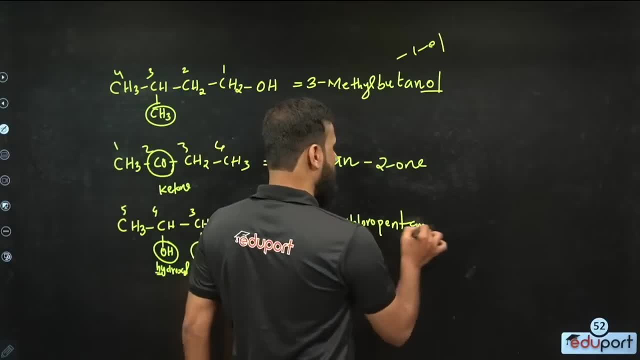 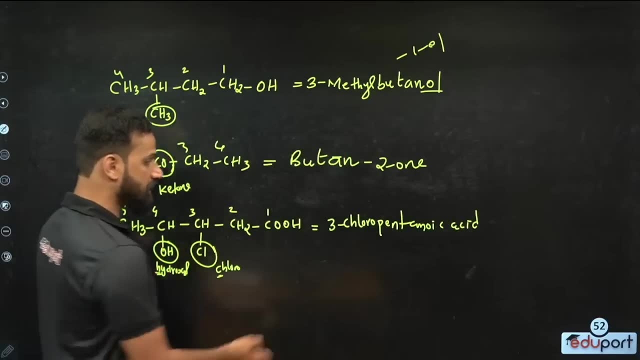 So pentane is one Oic acid. One should not be mentioned. So pentanoic acid is enough. So trichloro, Sorry, sorry. We have not mentioned hydroxy. After trichloro we have to say 4-hydroxy. 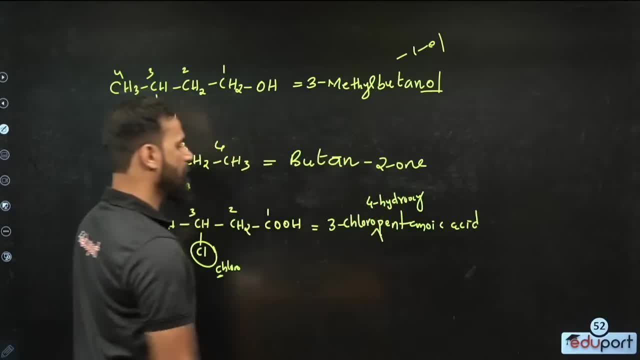 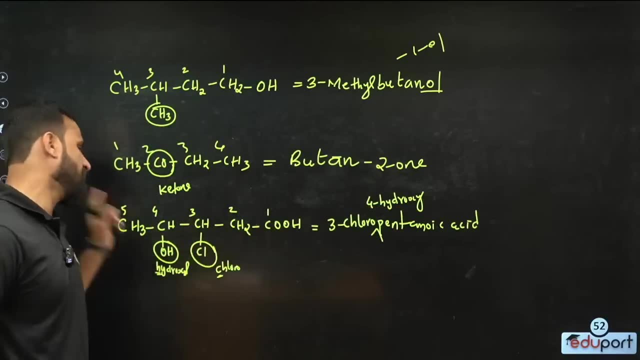 4-hydroxy. So trichloro 4-hydroxy pentanoic acid. What is it? Trichloro 4-hydroxy pentanoic acid- Ok, children. Trichloro 4-hydroxy pentanoic acid. 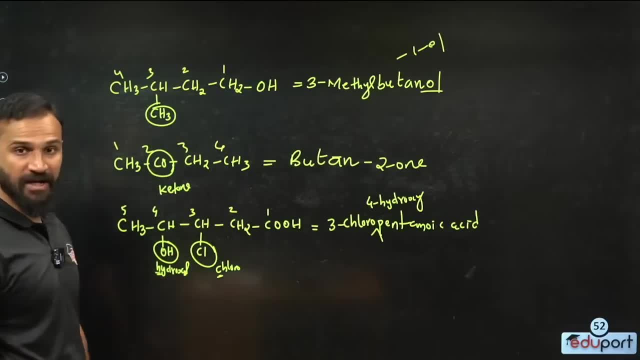 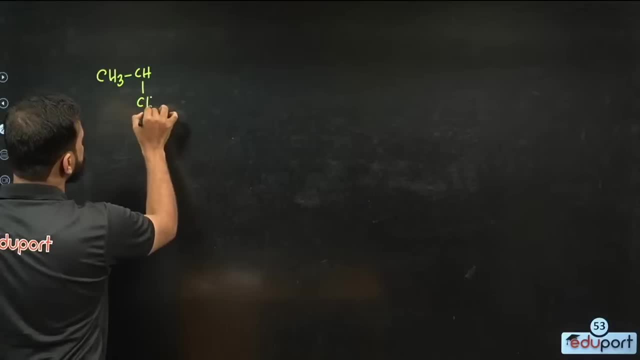 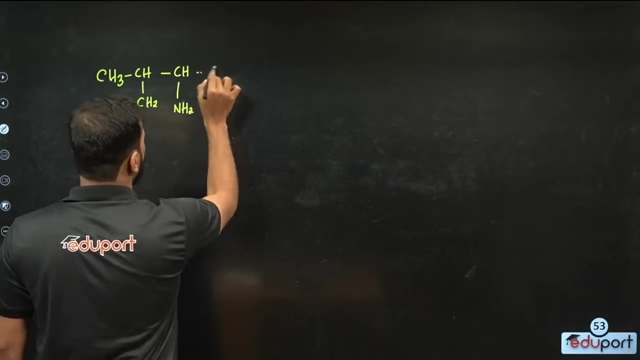 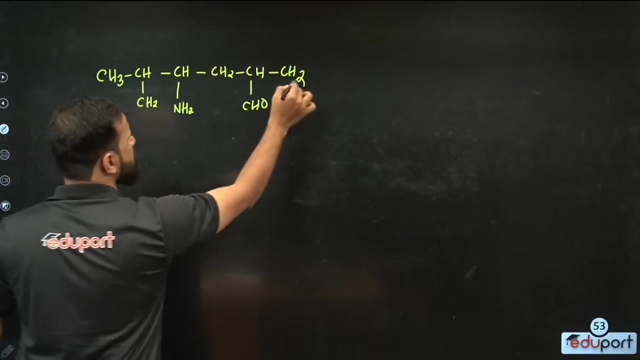 What is the prefix of this OH Hydroxy? That is what we have to learn Now. look at another compound, children. Look at CH3CH, NH2,, NH2.. CH2,, CH CHO, CH2.. Sorry, CH3.. 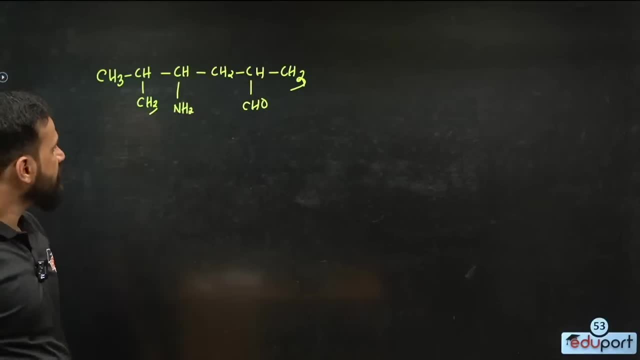 Here also, it is CH3.. What is the name of this? There is an aldehyde which has the most priority. Aminoglutamide compound is an aldehyde's priority. One should be given to it Because it has to be made in the longest style. 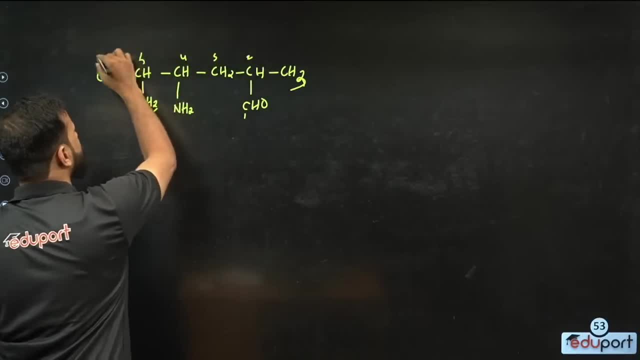 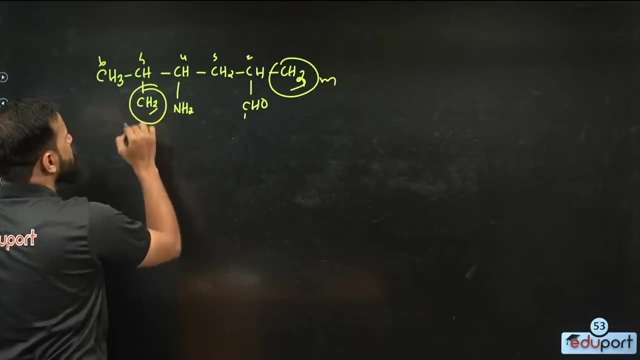 after starting from 2.. 1,, 2,, 3,, 4,, 5,, 6.. Ok, While looking at it, there is a methyl in 2.. There is a methyl in 5.. Aminoglutamide compound in 4.. 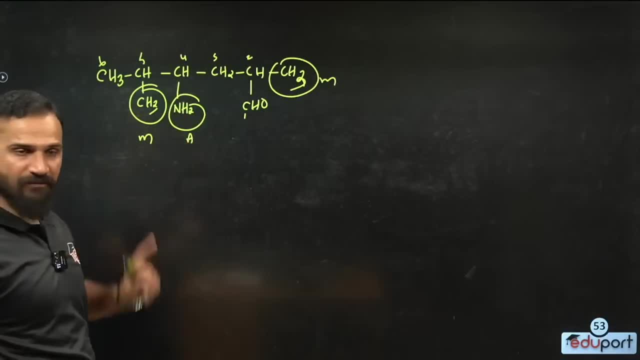 There is an amino group in 4. Alphabetic code is A only, So it is written as 4-amino. 4-amino Longest gel is carbonate, So it is Hex Because it is a single bond. 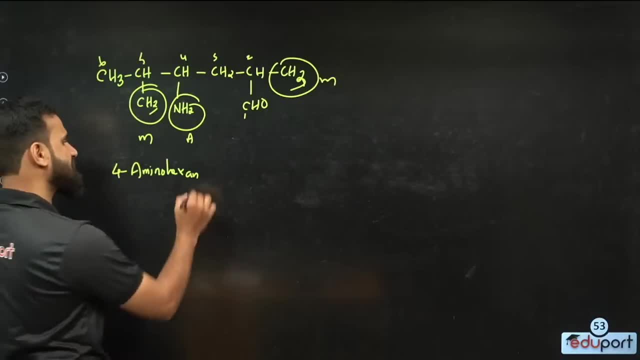 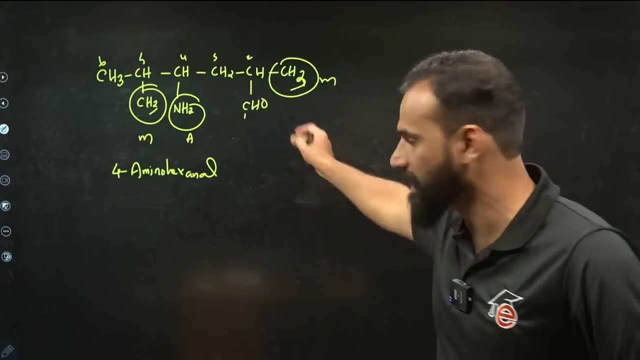 it is Hexene. The first one is Al, So Hex-en-al- Actually Hexene-1-al should be given Because it is the first carbon. we can simply say that it is Hexene-al, So that is how its name is. 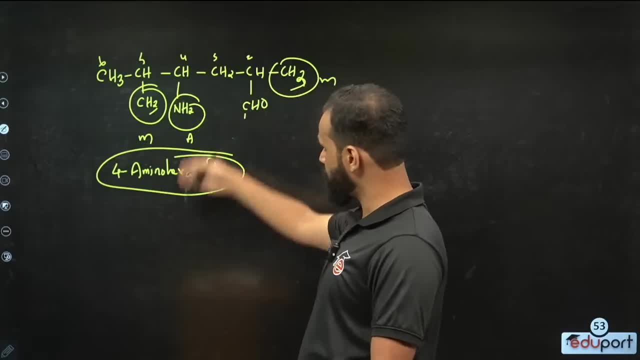 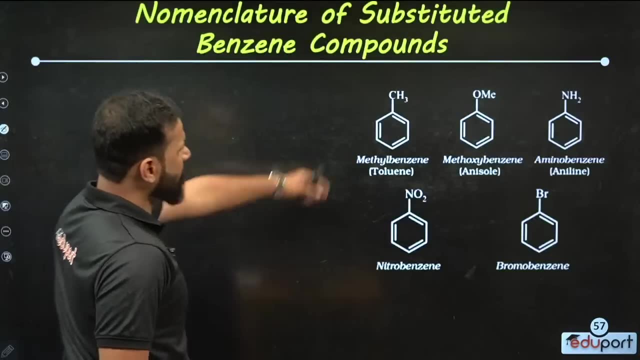 Children. please notice, It is very important. It is very important. So this is the name. We are going to the previous question. There are a lot of names there Before that. these are the derivatives of benzene. If CH3 comes on top of this benzene, it is called methyl benzene or TULU. 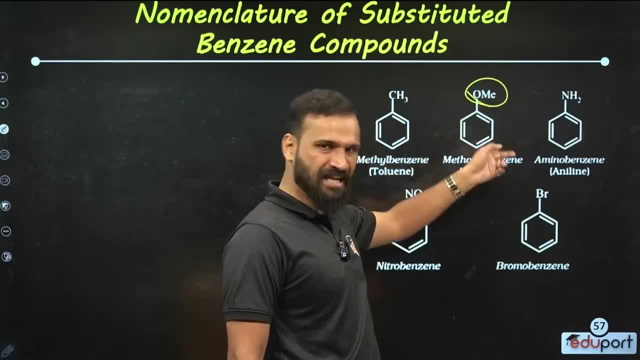 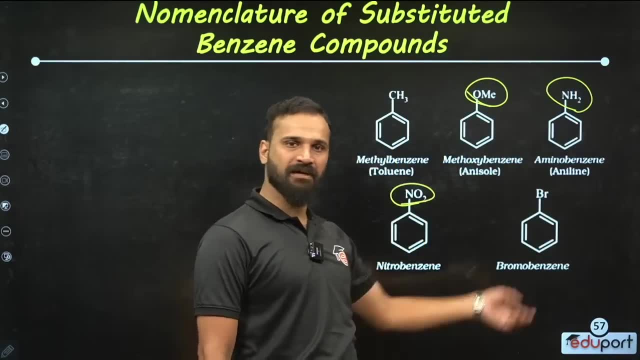 If COCH3 comes, it is called anisole or methoxy benzene. If NH2 comes, it is called aniline or amino benzene. If NO2 comes, it is called nitro benzene. If halogen comes, it is called halobenzene or bromine or bromobenzene. 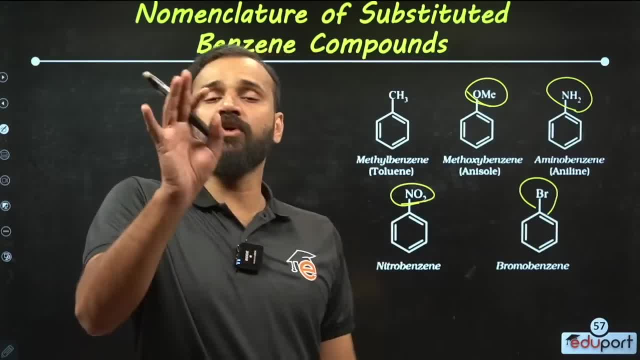 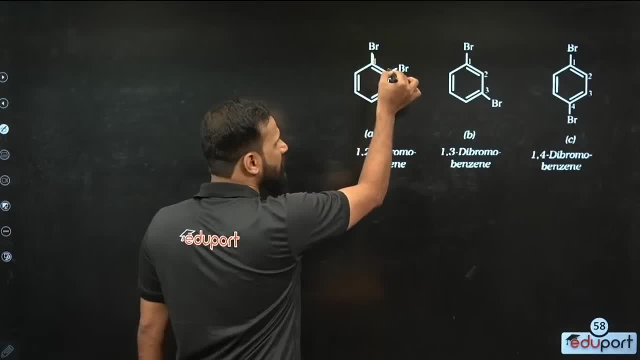 If chlorine comes, it is called chlorobenzene. These are the names. We need to have a basic idea about it. Look, there is one thing to note when naming them. If bromine comes in the first or second position, it is called 1,2-dibromobenzene. 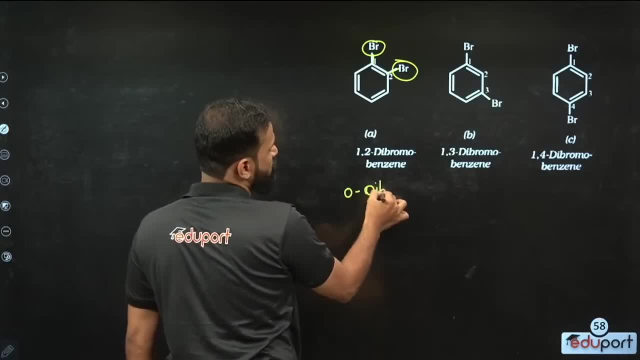 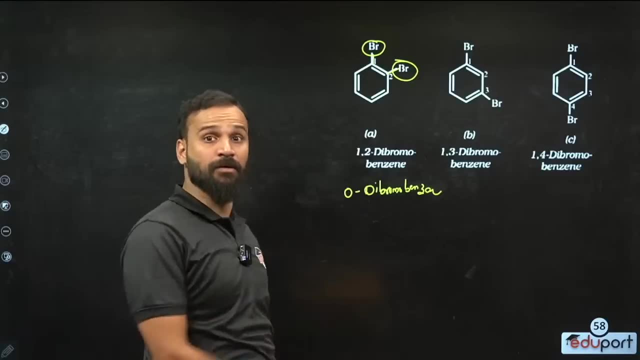 Or it can be called orthodibromobenzene. If it is 1 or 3,, it can be called 1,3 or metadibromobenzene. If it is 1 or 4,, it can be called 1,4-dibromobenzene. 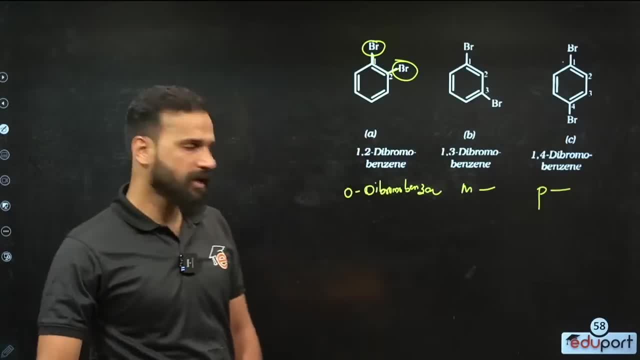 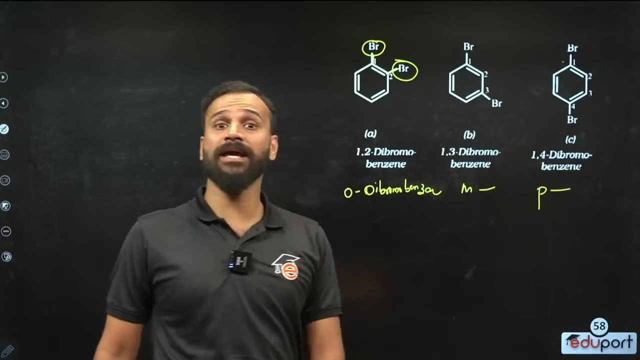 Or it can be called paradibromobenzene, Ortho, meta, para. If it is 1,2,, it is called ortho, If it is 1,3, it is called meta. If it is 1,4,, it is called para. 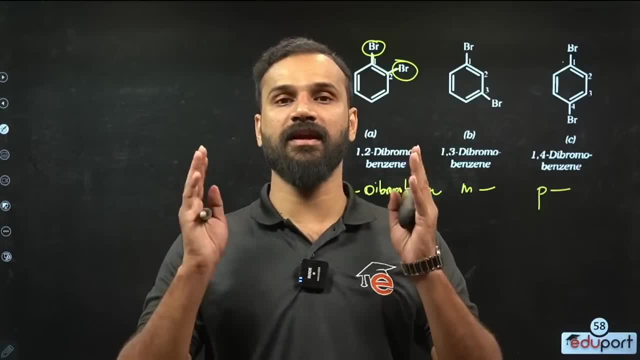 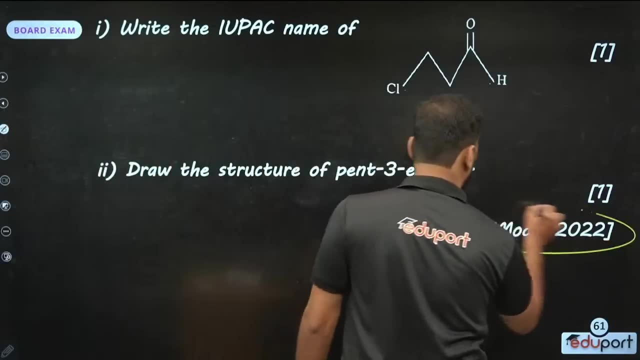 This is how the order comes. We need to pay special attention to it, Is that okay? Yes, Now look at the name: 2022 model. Now, children, you need to pay attention to this From what I have said so far. 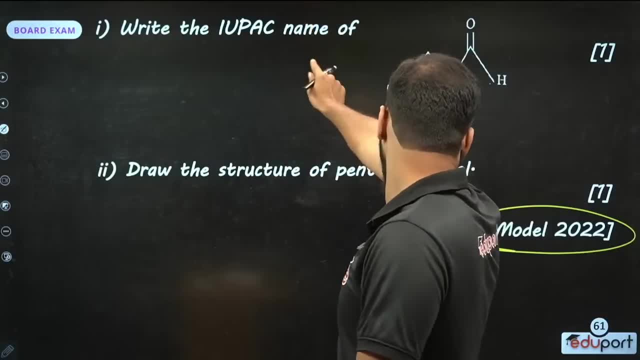 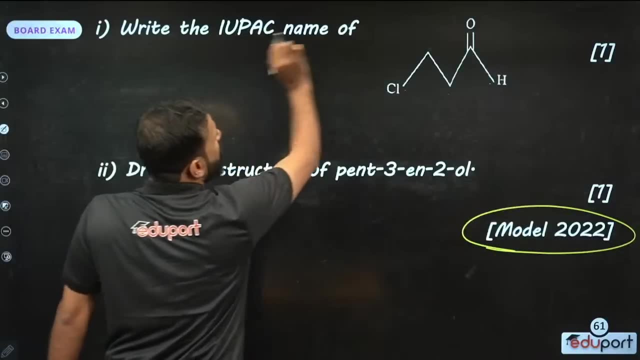 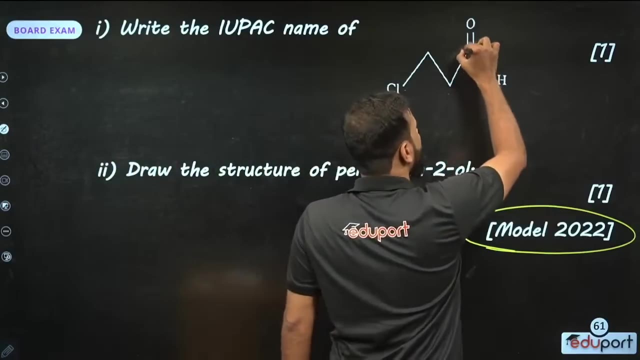 you need to use the things you have understood. you need to name the following compounds: It is very important You name it, You study it. Write the UPSC name. What is the UPSC name? Bond line representation. Do you know the problem here, children? 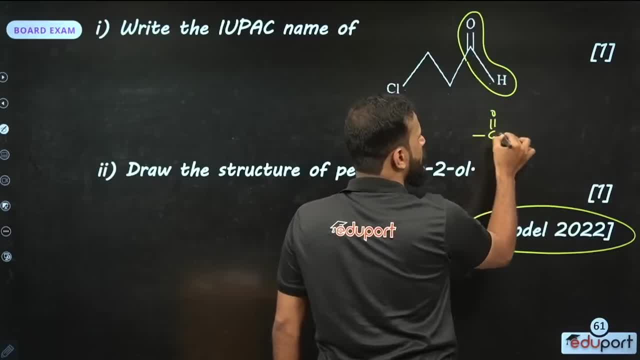 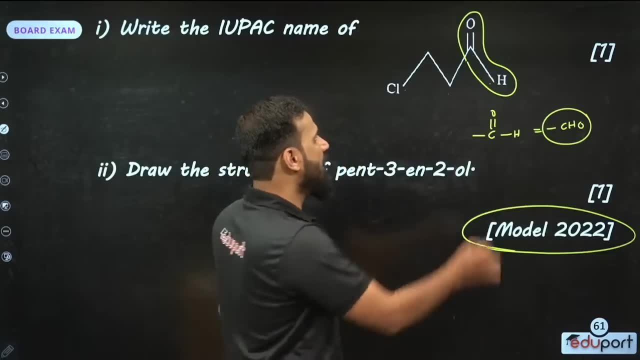 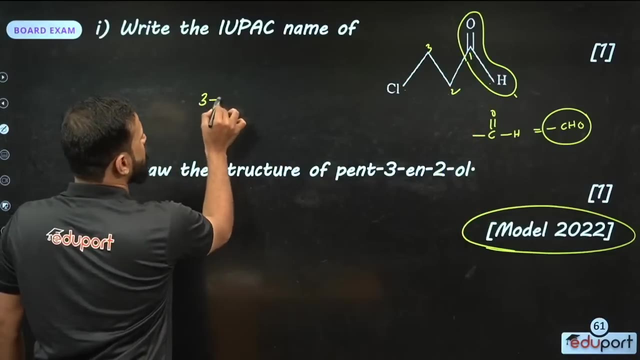 Do you know who this is? This is CHO. If we say C double bond, OHO, this is what we call CHO, Or it is aldehyde, Aldehyde. You need to understand that. One, two, three. In the third position there is chlorine. 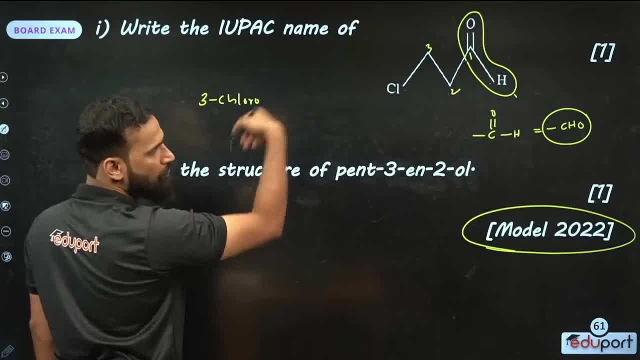 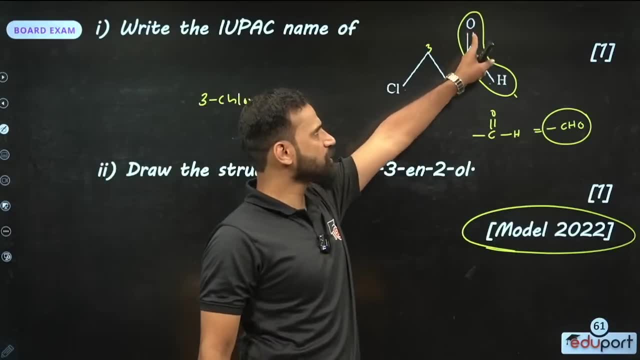 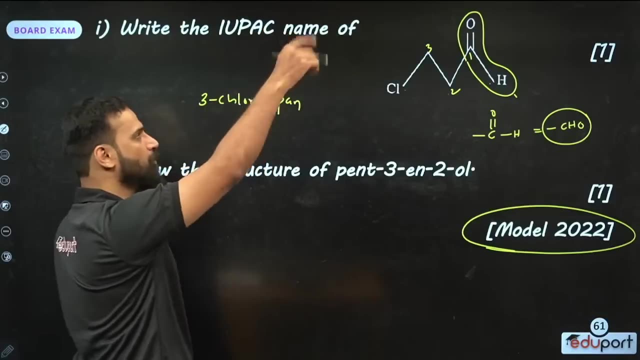 So three chloro, Three chloro, Three carbons, Prop, Prop, All are single bond Propen. Single bond means this is functional group CHO, It is CHO in its entirety. There is no double bond other than that. 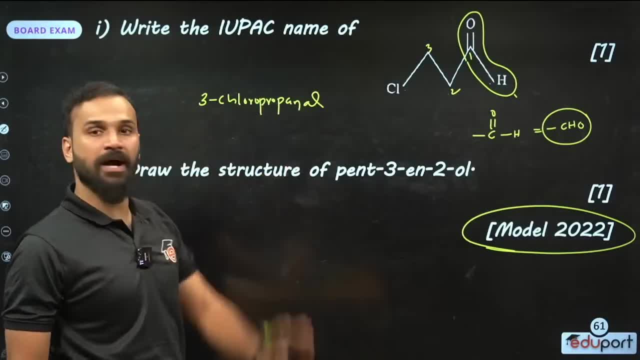 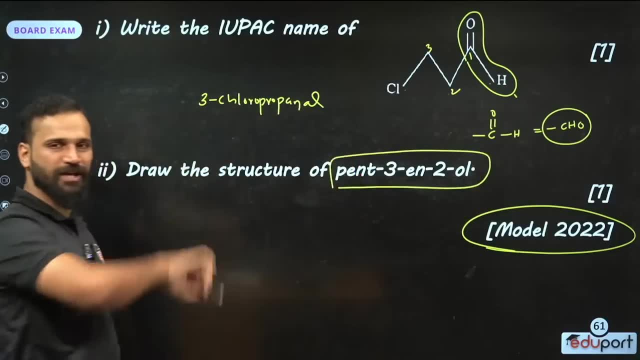 So propen. In the first position it is aldehyde, Propen 1 or propenol. What is the structure of propen 3 into all? We can ask this question again. We can ask to structure the name So propen children. 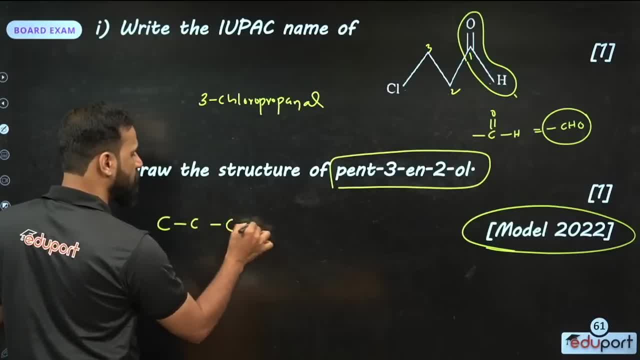 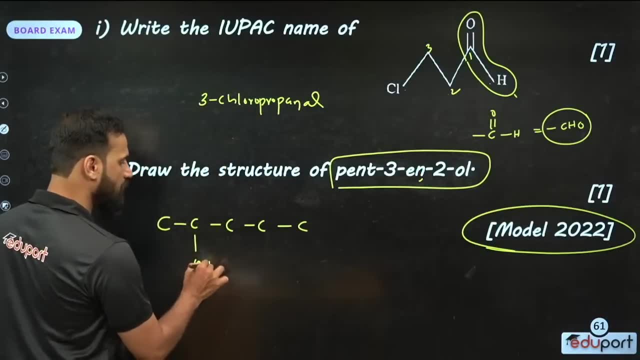 If you hear propen you can draw five carbon atoms: Three, four, five. In the third position there is CHO. In the second position there is OHO. So in the second position give OHO. In the third position, give double bond. 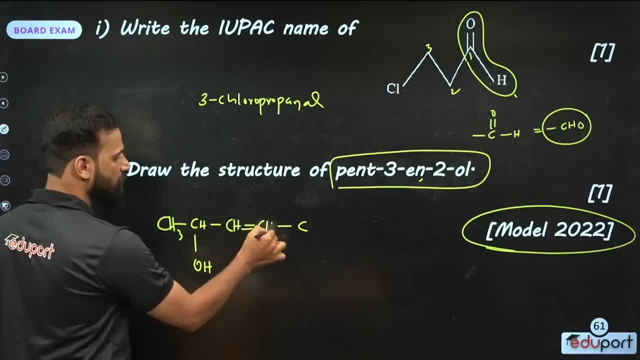 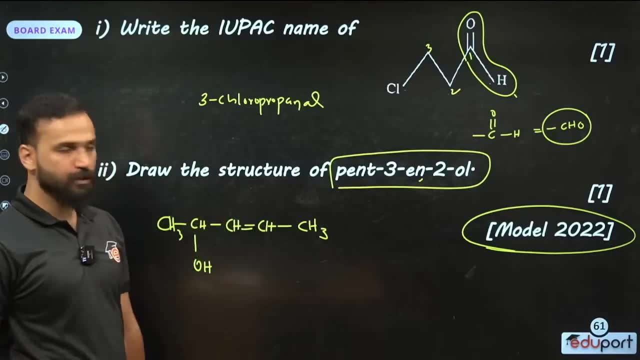 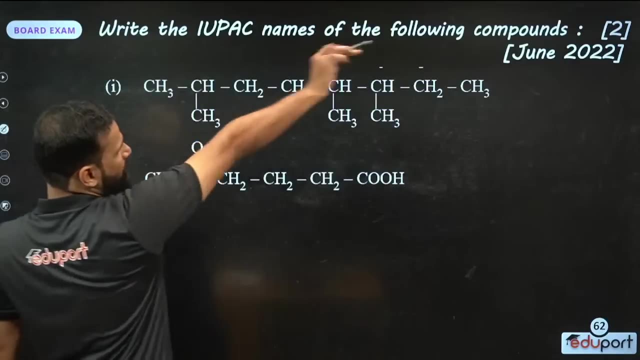 Now fill it with hydrogen. Here you need three hydrogen. Here one is enough. So this is what is: PEN2, PEN3 into all OK Structure with the UPSC name. We can ask this question again. Now write the UPSC name. 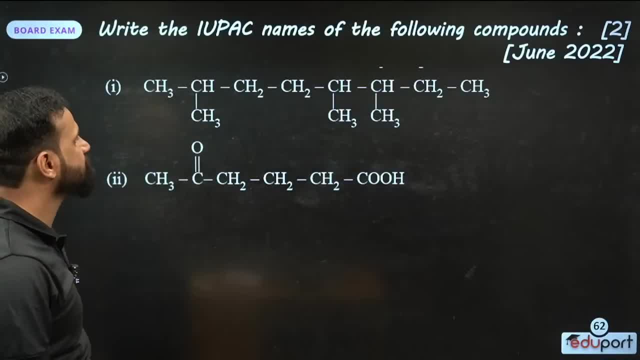 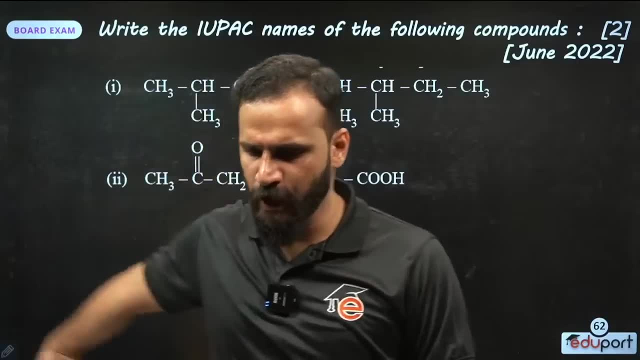 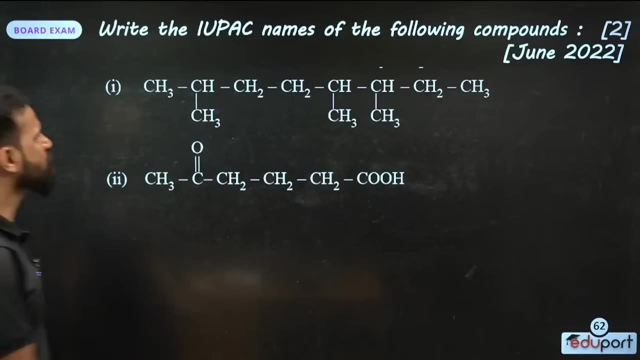 Children, you tell me How to write the name of UPSC. How to write the name of UPSC: Three branch and three methyl. Have you commented yourself: Three branch and three methyl, Three methyl. No doubt, There is no doubt. From there, children, do the number One, two. 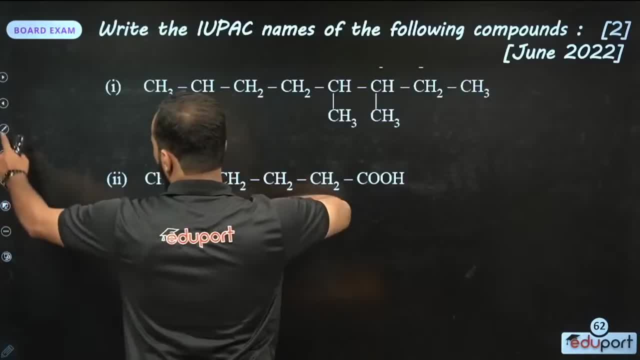 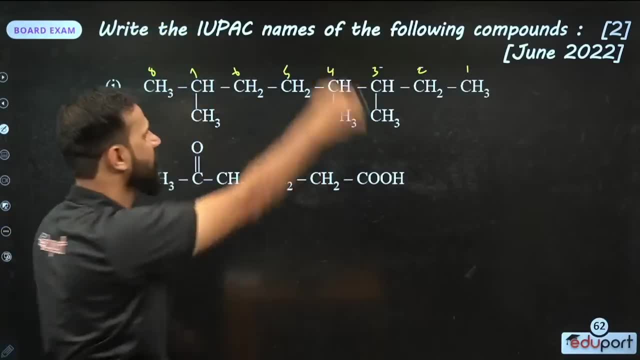 If you have a doubt, you have to try to number it. children, If you have a doubt, you have to try to number it. One, two, three, four, five, six, seven, eight. Is it okay? Yes, 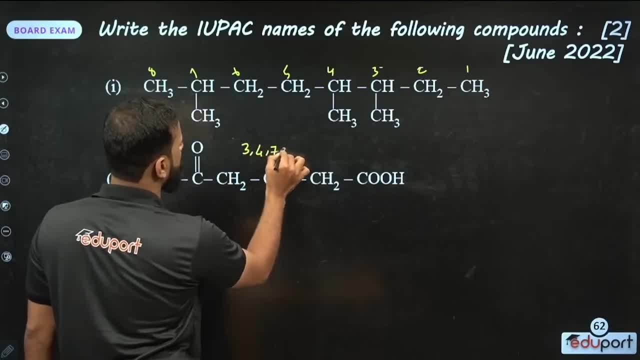 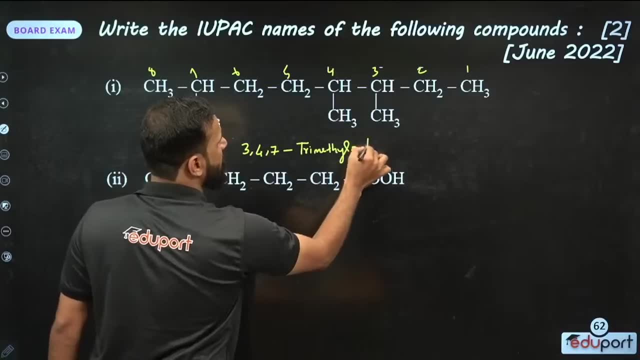 Methyl is present in three, four and seven, So tri-methyl can be said Tri-methyl, Longest cell. eight carbonate is oct. Everything is single bond, so any. So three, four, seven tri-methyl octane is the. 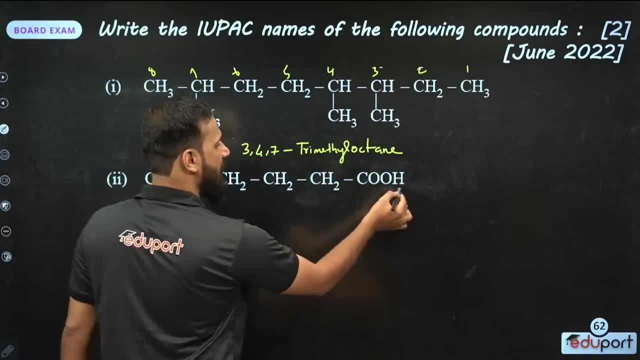 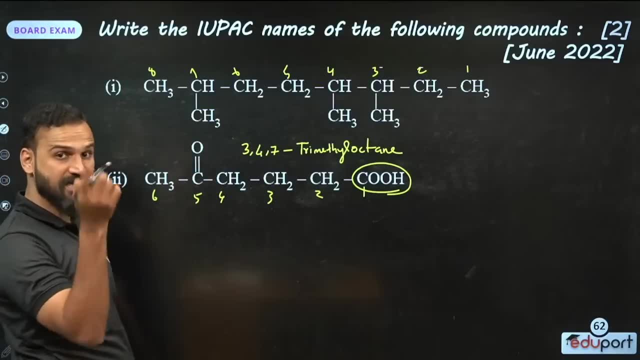 UPSC name, Now children. this is very important. Acid is the priority, So one, two, three, four, five, six. There is a ketone in five, but it is a suffix, not a prefix. Its prefix is oxone, So five: oxohexanoic acid. 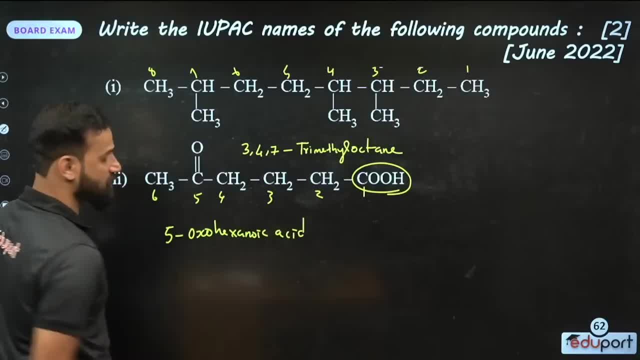 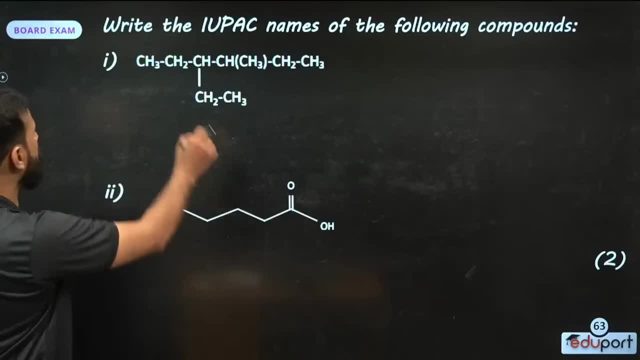 Hexanoic acid. Hexen, hexen. one oic acid Then one is not to be said, so it is hexanoic. We say it is very important. Now look, Write the UPSC name of the following compounds. Let's name this UPSC. 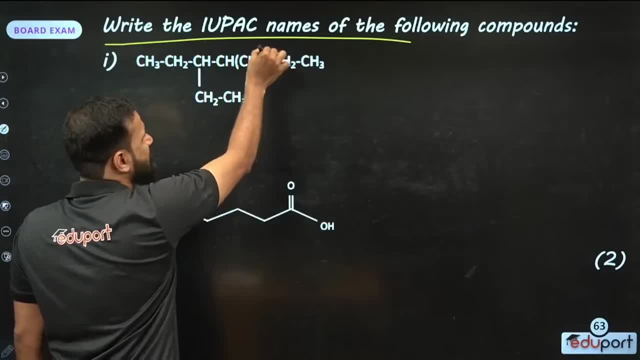 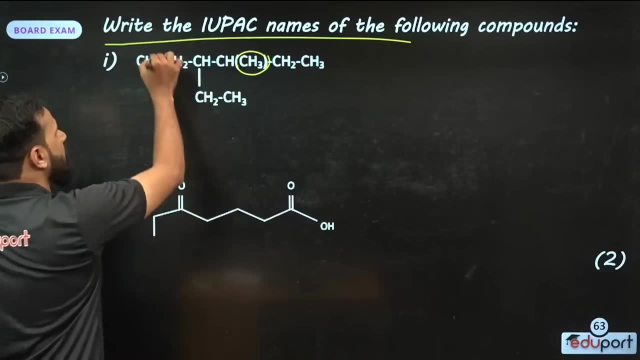 Look here after a CH. you can see CH3 in a bracket. Do you know what that is? That is the branch of CH CH3.. When it comes like that, we put it in brackets like that. So how to number it? One, two, three, four, five, six. 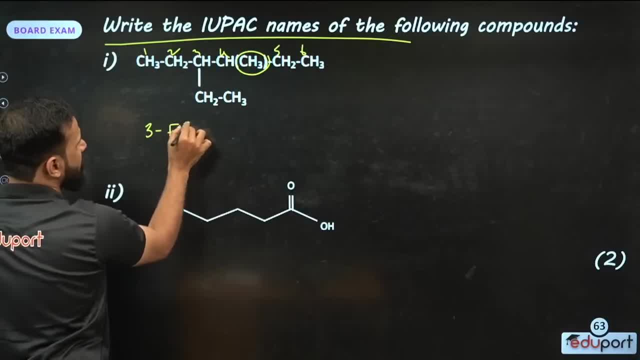 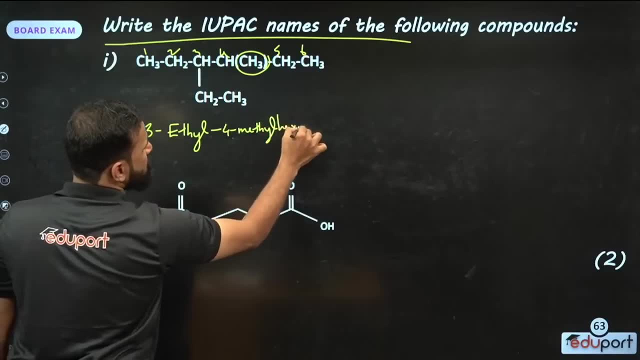 Ethyl in three. So there is three ethyl Four methyl Four methyl Two, The longest one is six. So hexane comes there. So three ethyl four methyl hexane. You have to see if you get it anyway. 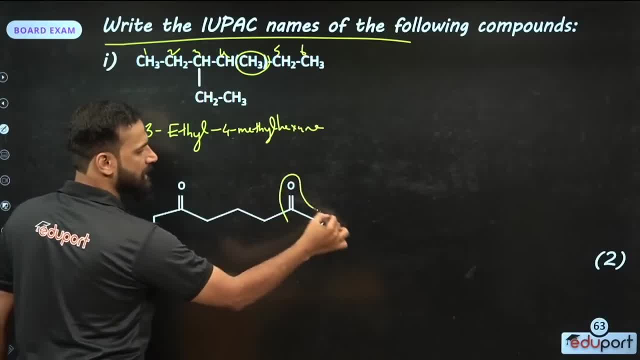 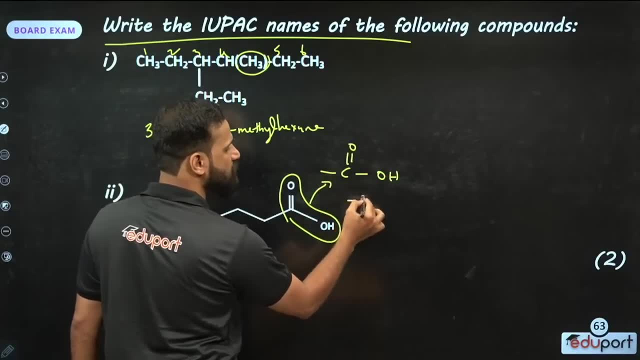 These are the questions asked in the exam. Now look, a person is not seen here. C double. Look, that is very important. C double bond. OOH, That's it. Who is this? This is what we call COOH. 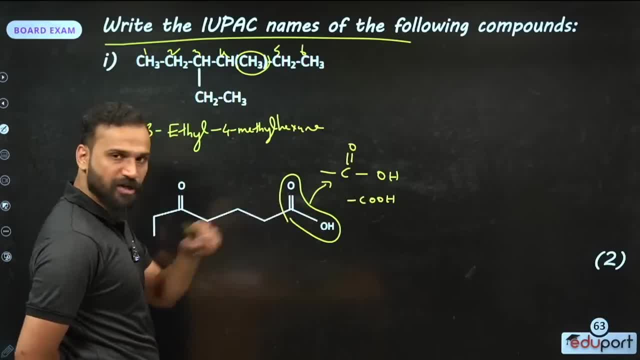 So how do you ask to confuse? Sometimes you think there is an OH in the ketone here, Not like that. This is COOH, That is COOH, It is a group. So you just need to give the number 1 there. 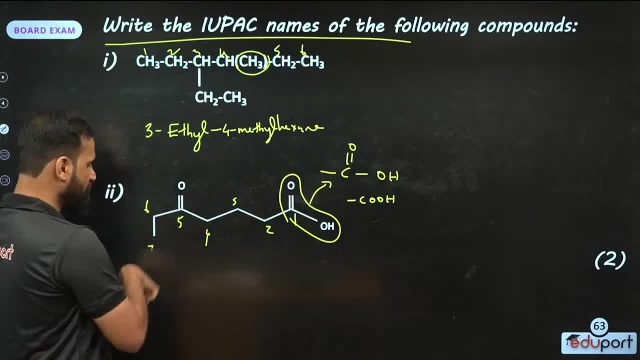 Here is 2, here is 3, here is 4, here is 5, here is 6,, here is 7.. 5 is ketone, So 5 oxo In the longest chain, 7 carbons, So hept. 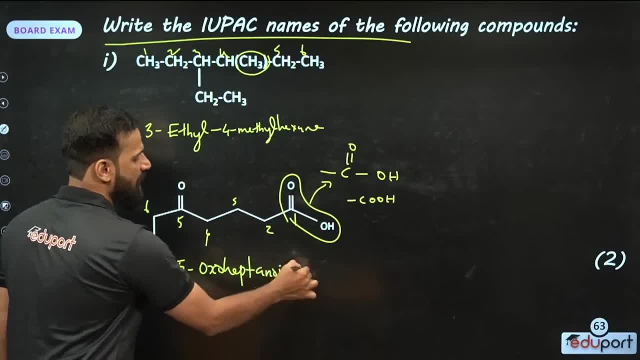 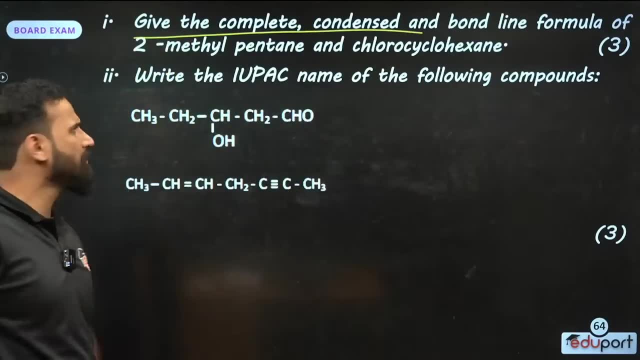 In the first carbon lowic acid. So heptanoic acid, Heptanoic acid. Now look, give the complete condensed. That is what we have to say. Write the UPSC name of the flowing. What is the UPSC name of this? 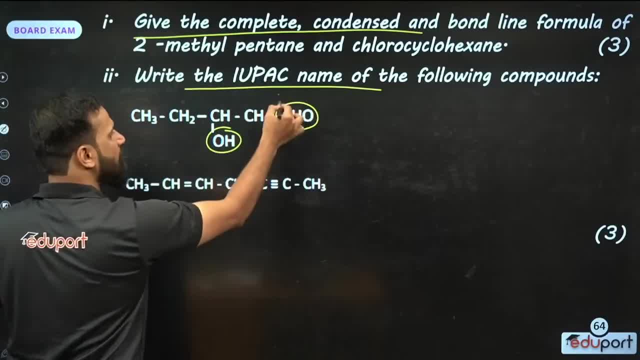 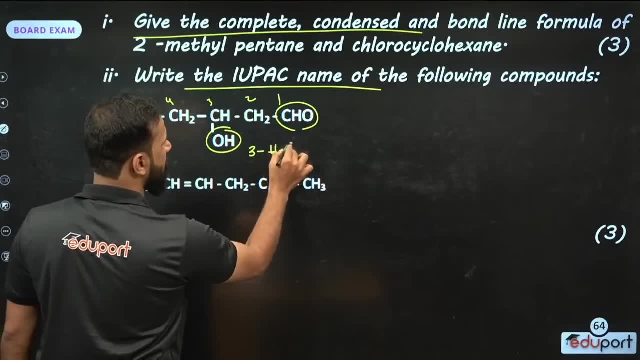 There is aldehyde, there is alcohol. The priority is more for aldehyde. So 1,, 2,, 3,, 4, 5.. Isn't it? So 3 is alcohol, So 3 is hydroxy. What is 3? Hydroxy? 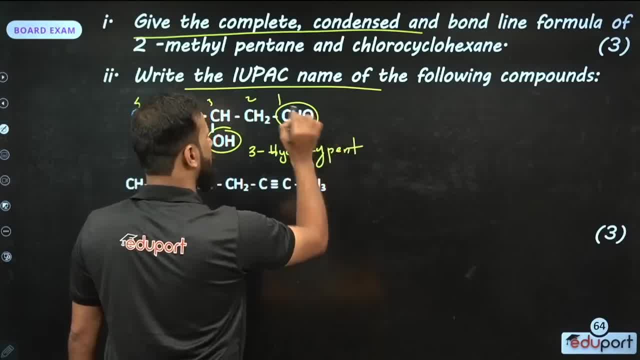 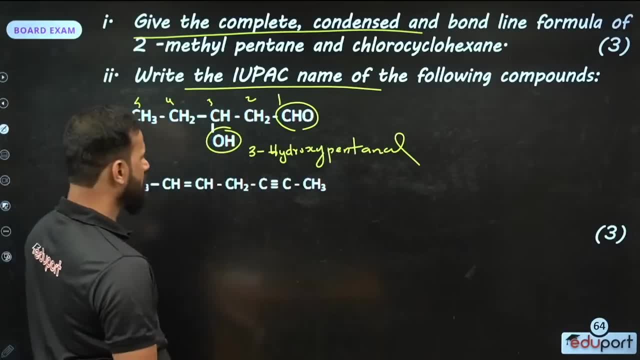 In the longest chain: 5 carbons, So hept In the first position, OOH, So heptanol, Heptanol. Now look at the children. What is here? There is a triple bond here. There is a double bond here. 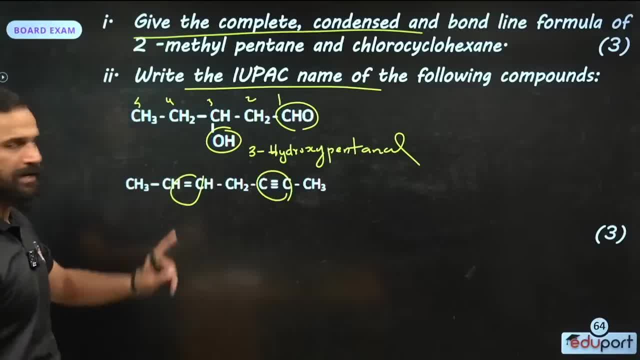 As we said earlier, there is a triple and a double. So what to do? As the double bond gets the least number, do the number 1, 2,, 3,, 4,, 5, 6, 7.. 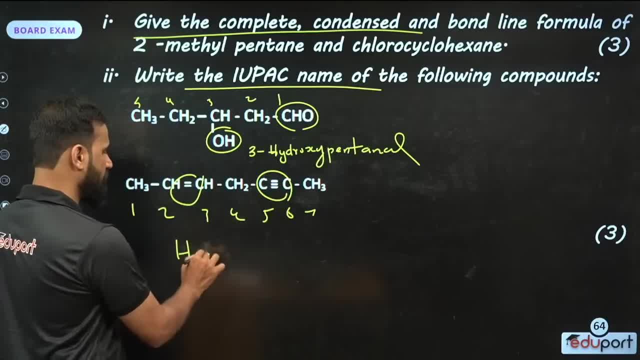 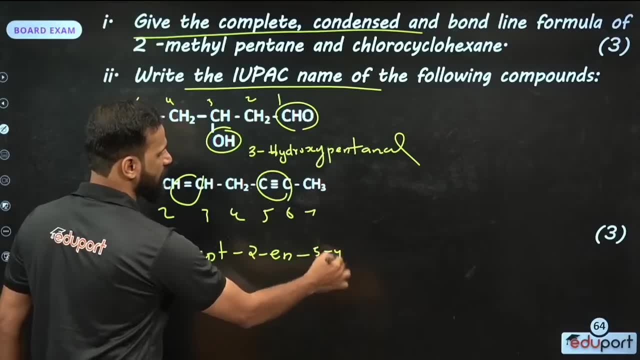 So what will it be? Hept will come, Hept, Isn't it? Double bond in the second position. So hept 2 in Triple bond in the fifth position. So 5 in will come. This is the UPSC name. 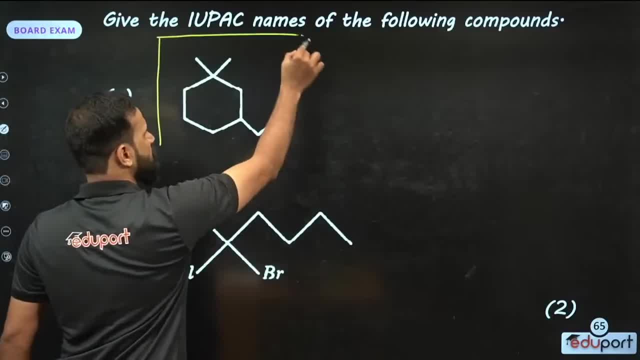 Isn't it? Now look children. This is something you have to pay attention to. Don't pay attention to this. This is a question asked many times in the exam. The speciality of this question is: what is here? Here is a methyl. 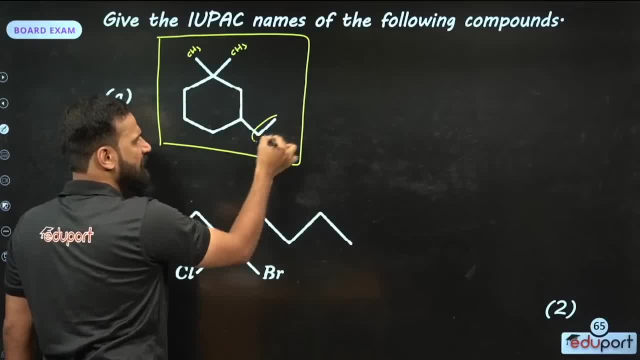 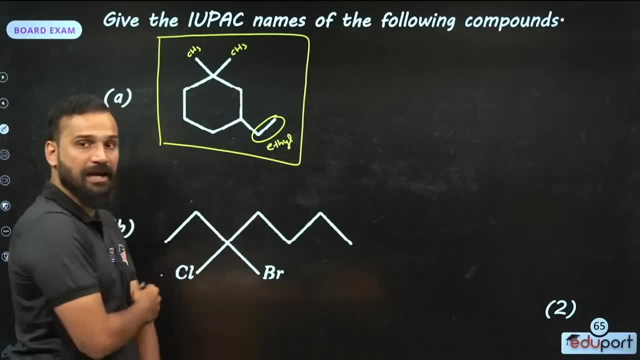 CH3 is there. Here is also a methyl: CH3.. This is an ethyl. You know this. So, looking at the alphabetic order, we have to write ethyl first, Isn't it? But what is the problem When naming cyclic compounds? 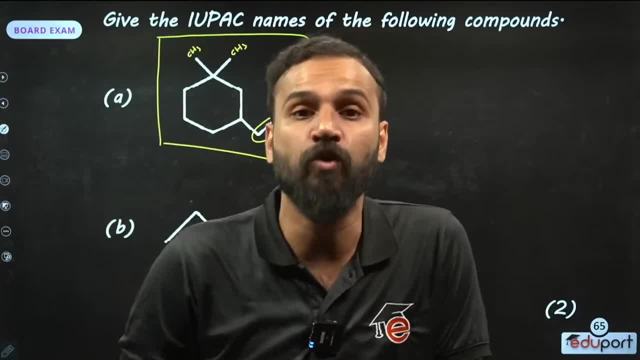 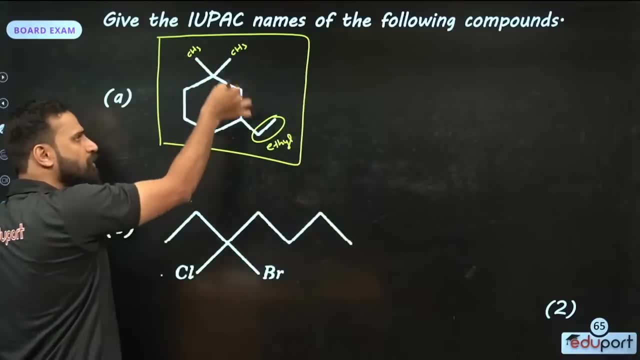 where is it? The number of branches is more. When doing the number of that carbon atom, there is priority, That is, whether it is from here to there. whether it is from there to there, if you ask, looking at the alphabetic order. 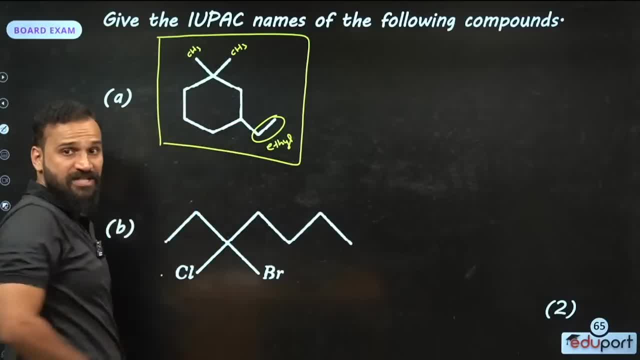 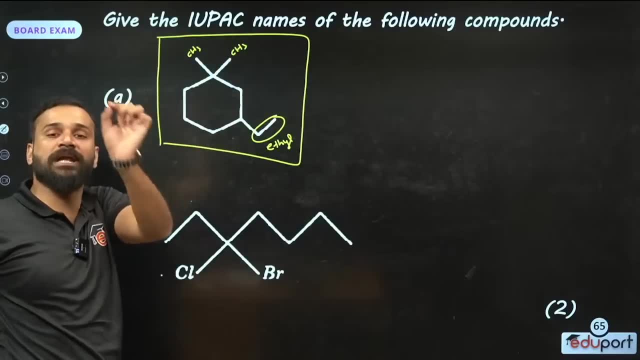 when E comes, here is MO, So you have to do it from here to there. But what is the problem? This carbon has two branches and this carbon has one branch. So which carbon is more than the number of branches When we name the cyclic structure? 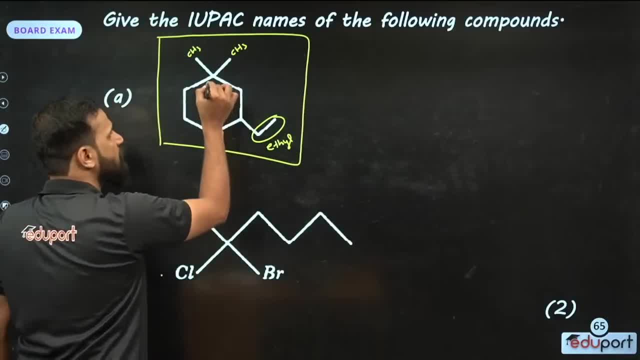 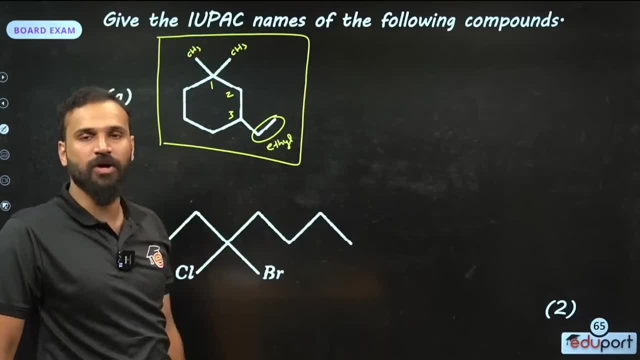 it has priority, That is, it should be done from here to below. One, two, three. Okay, So the carbon with more branches is numbered in the form of the least number, But when naming, the alphabetic order should be followed. 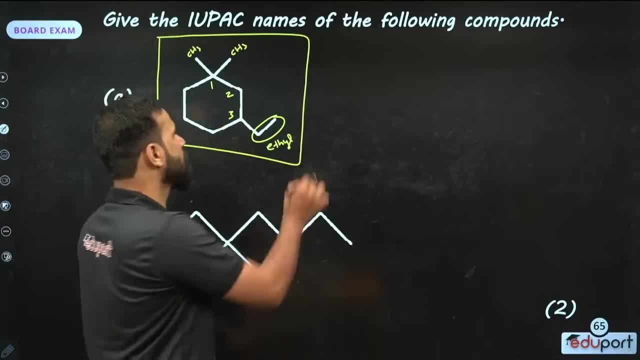 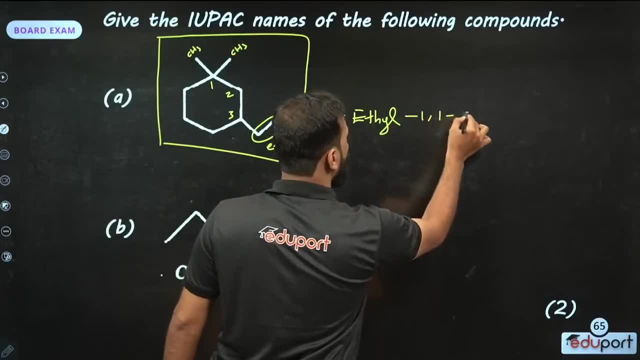 That is ethyl, should be said first. Where is ethyl In three? So three ethyl, One ethyl, three ethyl. Then what is it? There are two ethyls in one, So one comma, one dimethyl. 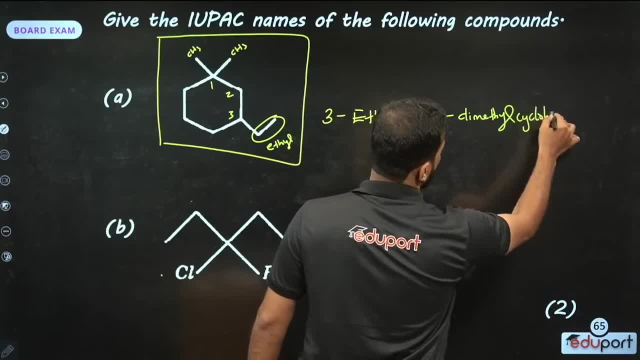 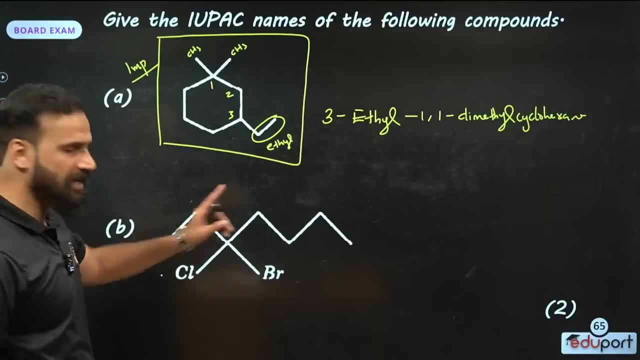 The longest chain is cyclohexane, So the area called cyclohexane is very important. This should be studied as important. This is the question asked many times. Now come to this, guys. This is also a repeated question In the third carbon. 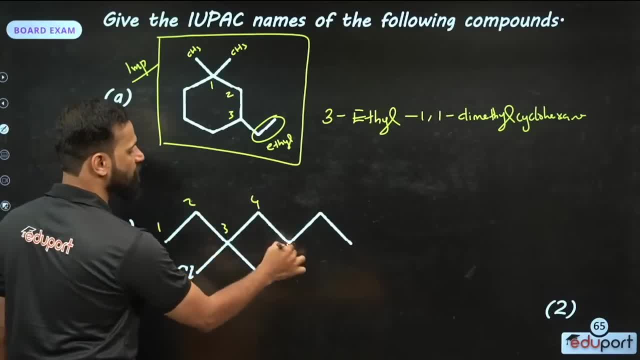 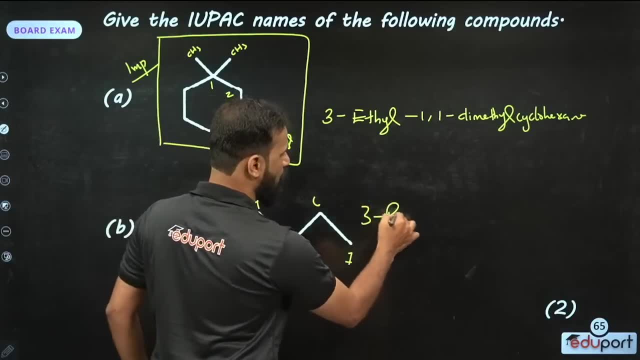 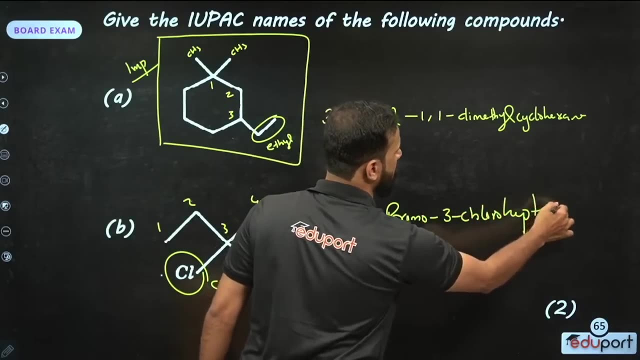 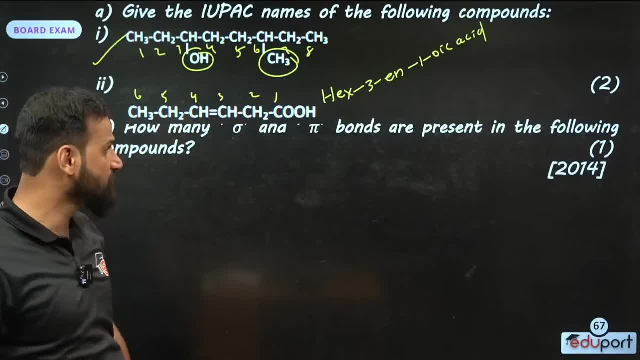 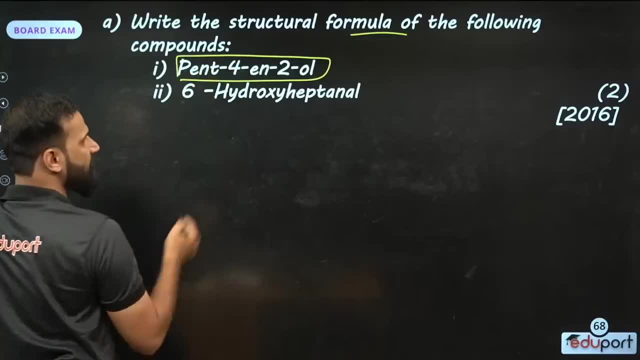 57,, 58,, 3-enoic acid. that's enough. Okay, now what do we have? Write the structural formula of the following: Pent-4-in-2-ol. As I said earlier, we did this right: Pent-4-in-2-ol. 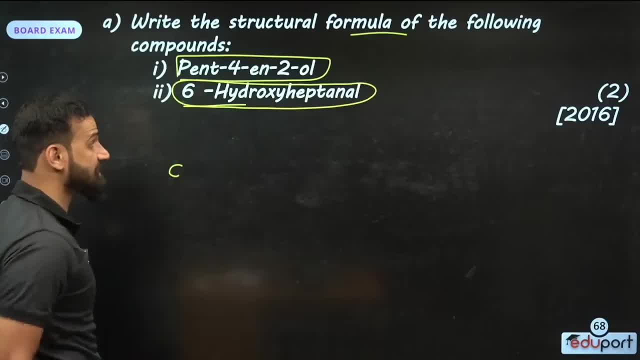 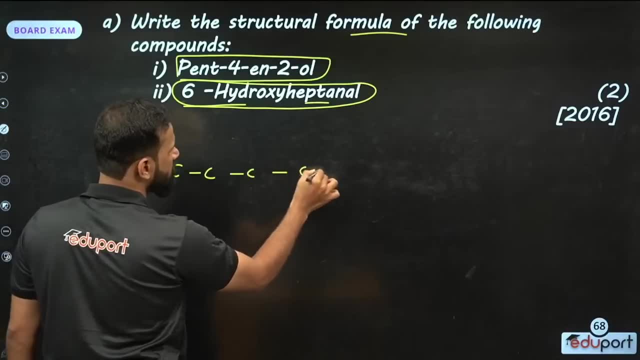 Now look 6-hydroxy-pentanol. 6-hydroxy-pentanol. So, since it is pent, 5 carbons. So 1, 2,, 3, 4, 5. Okay. 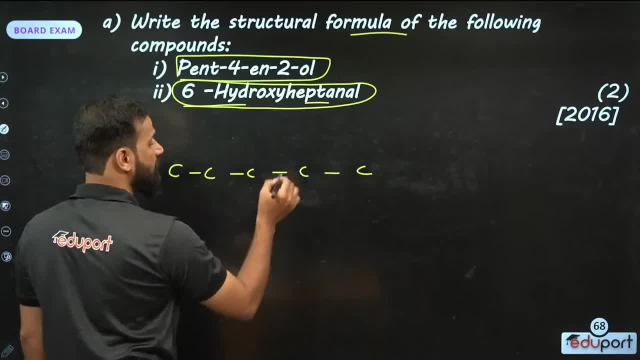 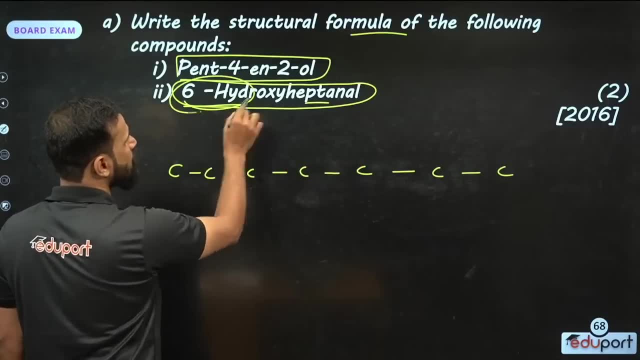 6-hydroxy: sorry, hept is here. So when we say hept, we need a 1,, 2,, 3,, 4,, 5, 6, 7.. 6-hydroxy-heptanol: Okay, heptanol. 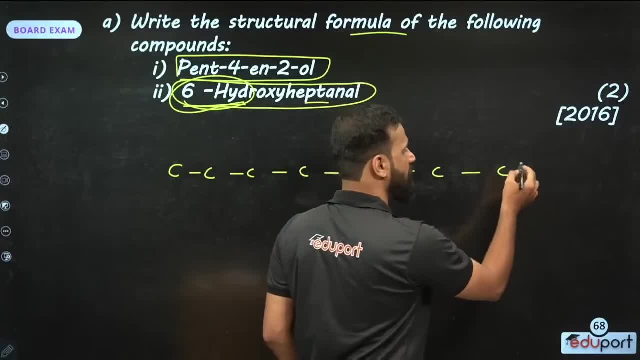 Heptanol is aldehyde, Where is aldehyde 1.. That's why I didn't mention the number. So if we take aldehyde 1,, 2,, 3,, 4,, 5,, 6. Here OH-1.. So hydroxy-i. 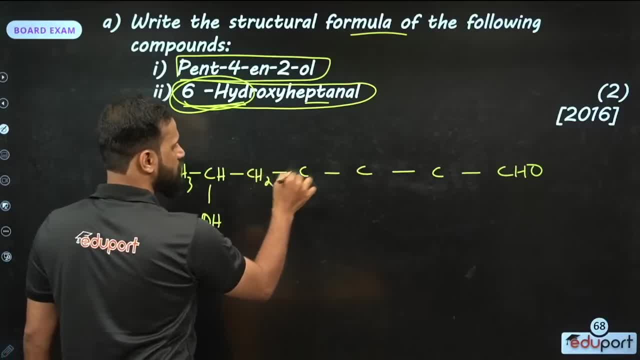 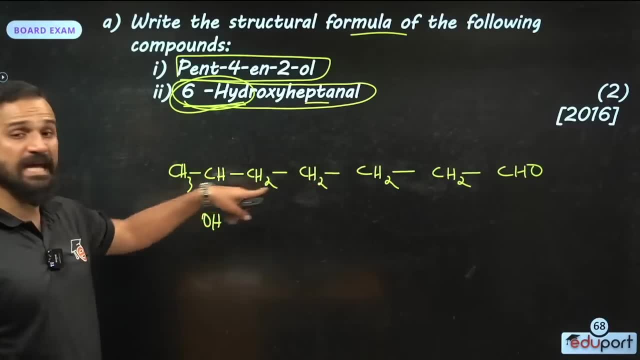 Now fill this: CH-3, CH, CH-2, CH-2, CH-2, CH-2, CH-1.. This is 6-hydroxy-heptanol. Yes, write the structure of the following compound. 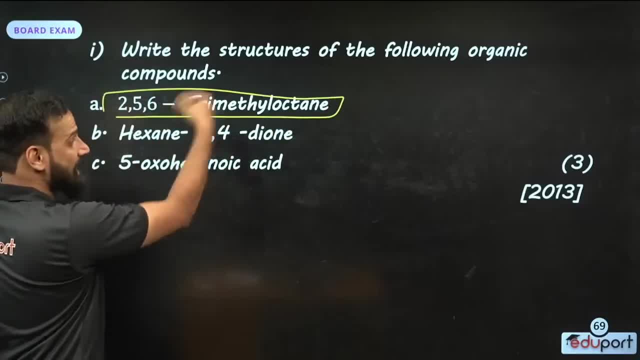 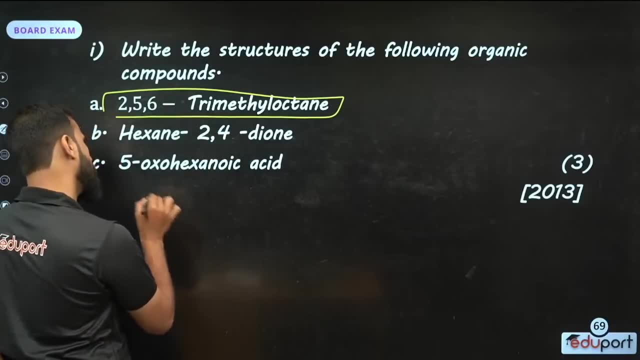 2, 5, 6,. what is it? Trimethyl-octane, Trimethyl-octane, Trimethyl-octane. What is octane, kids? 8 carbons, 1,, 2,, 3,, 4,, 5,. 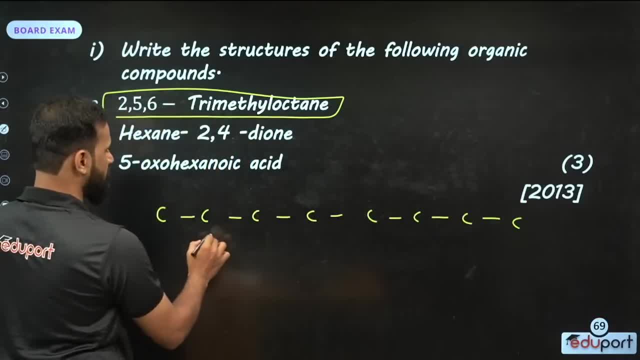 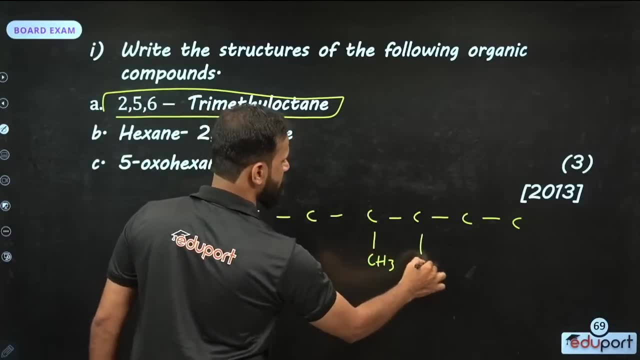 6,, 7, 8.. Okay, 2,, 5,, 6 are methane, So here is CH-3.. 5,, 2,, 3,, 4, 5.. Then where is 6?? Here is CH-3.. So the rest. 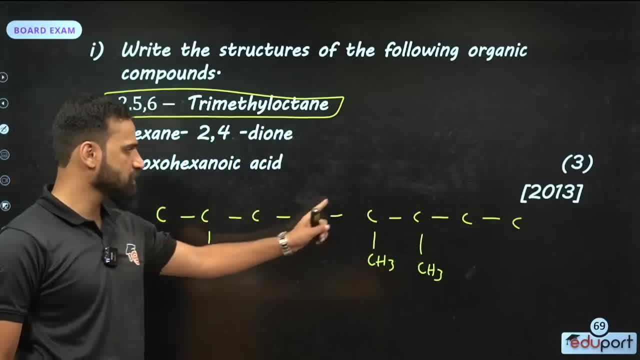 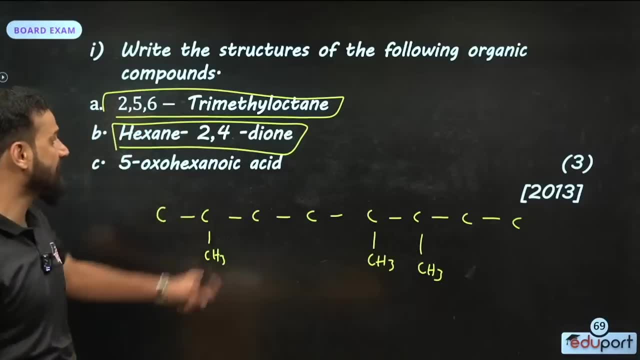 we can fill it with hydrogen, CH-3, CH, CH-2, CH-2, CH-2, CH-2, CH-3, CH-3 will come right, Nothing. Hexane-2, 4-dione Dione. 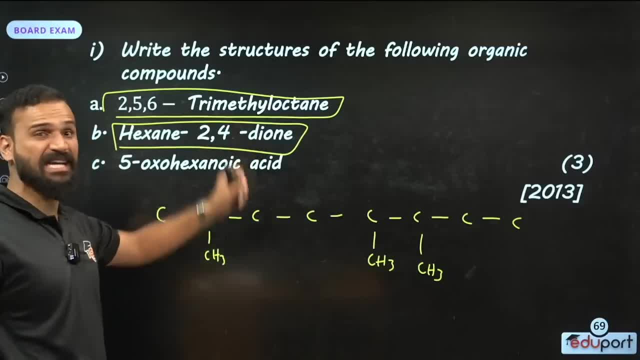 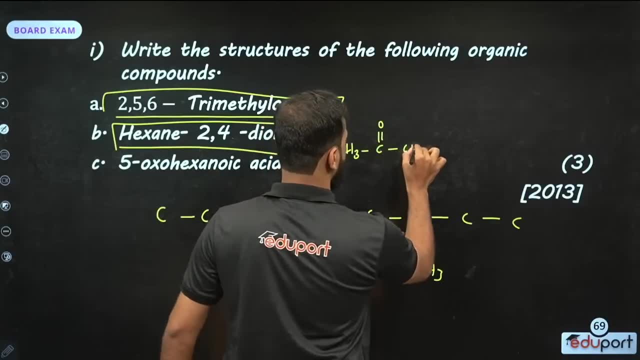 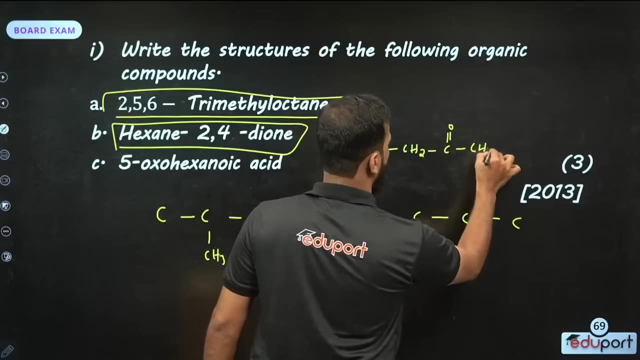 So hexane-2, 4-dione Dione means there are two ketones, So there are ketones in two. Then where is it? 4.. CH-2, C double bond O CH right 1,, 2,, 3,, 4,, 5,, 6.. 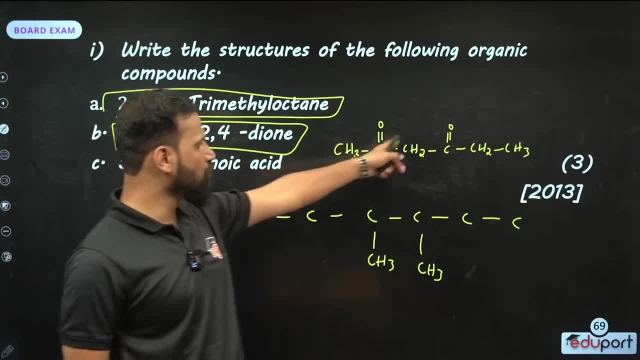 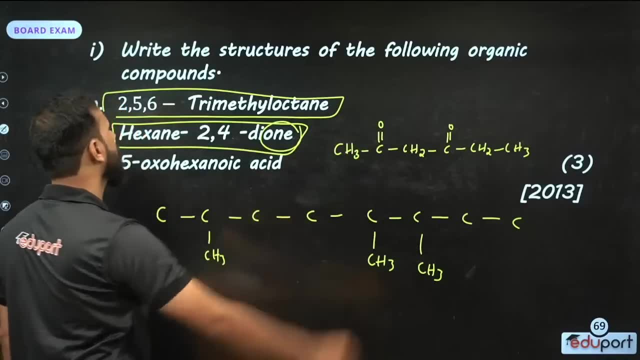 Children. this is hexane-2,4-dione 4.. CH-2, 4-dione Dione means it's a ketone. Dione means two ketones. There are 4 in 2 ketones. 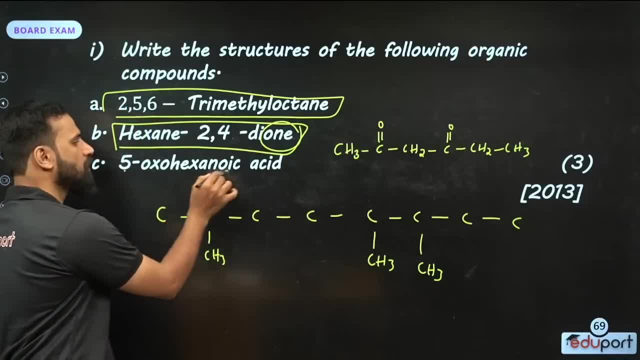 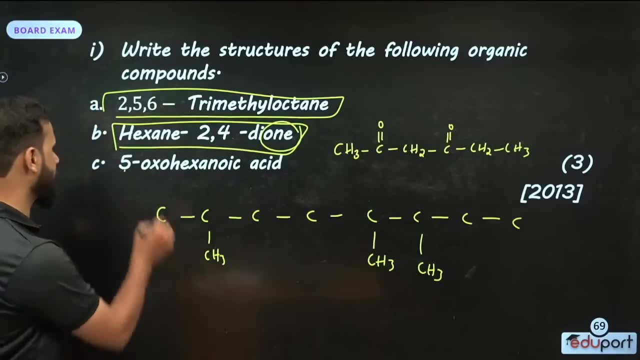 5-oxo-hexanoic acid That is. the fifth position is ketone and the first is acid. Total carbon is where 6 carbon. That is 5-oxo-hexanoic acid. We can show it later. 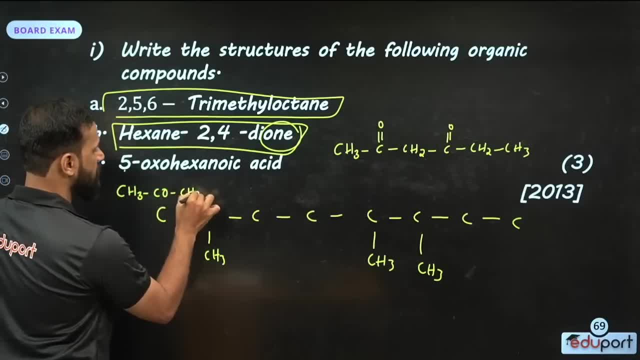 5 oxo, CH3, CO, CH2, CH2, CH2, COOH. okay, 1,, 2,, 3, 4, 5, 6.. In the 5th position, ketone is 5 oxo 6, carbon is hexane. 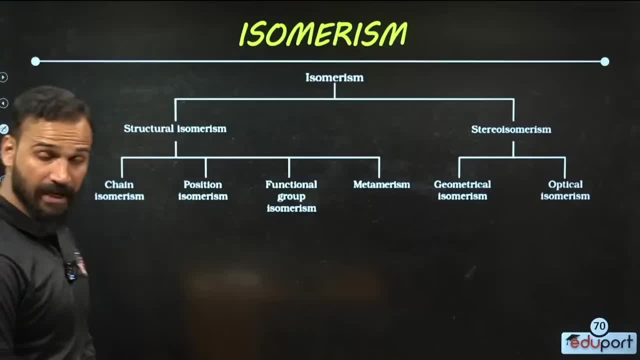 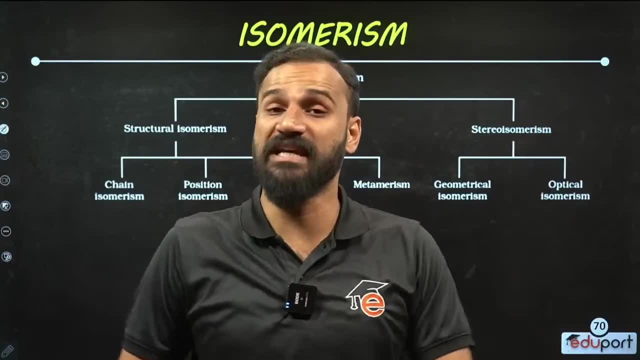 in the 1st position, oic acid is COOH. okay, simple, Okay, this is how we give the name. So we have given the name of all the compounds. We have done the maximum number of previous year questions. 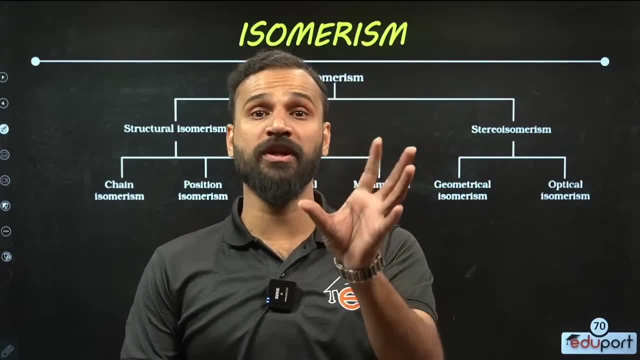 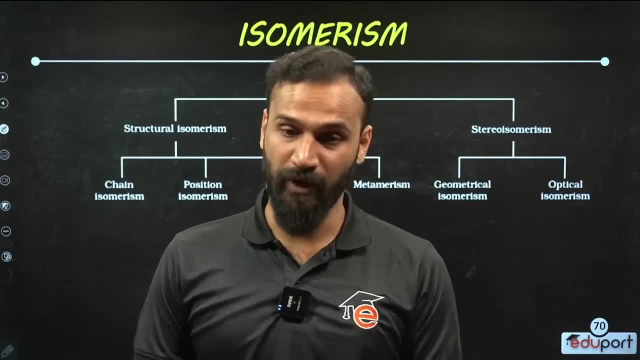 So this is how we give the name of the organic compounds. What do the students have to do? very clearly, They have to study, they have to remember. it is very important. So if you get an idea about naming, comment it quickly. 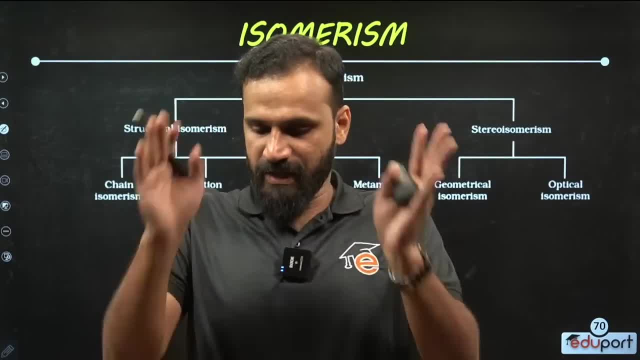 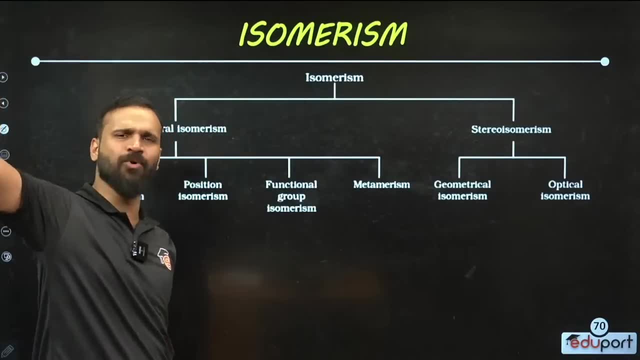 If you get an idea about how to give the name of organic compounds, comment it quickly. comment it quickly. Now we are going to study isomerase. You know, there is the same molecular formula but there is a different structural formula. 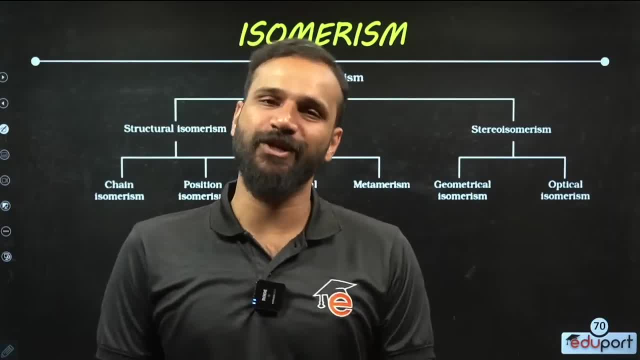 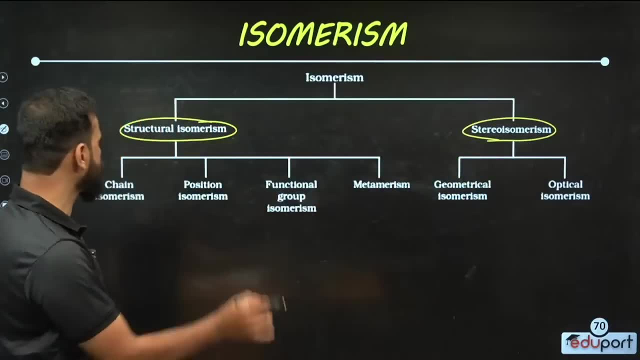 It is called isomers. What is that phenomenon? It is isomerism. There are two types of it: Structural isomerism and stereo isomerism. In this chapter we are focusing on structural isomerism. Structural isomerism mainly has four types. 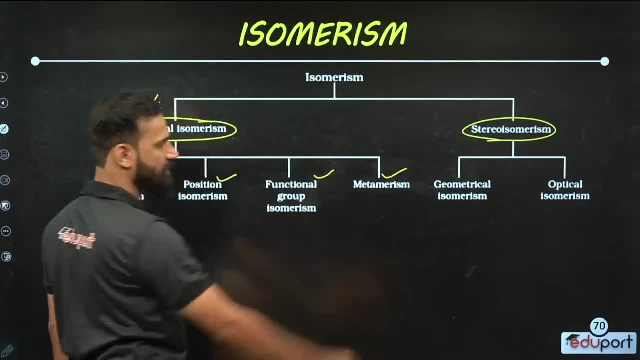 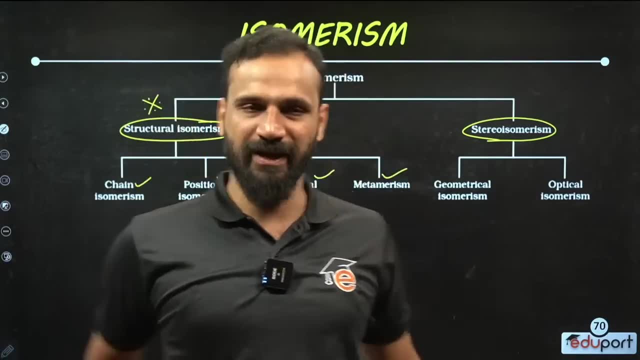 One is chain, two is position, three is function and then metamerism. What are we going to do with these four? What are we going to do with these four? We are going to study them properly. Pay attention. Look. first is chain isomerism. 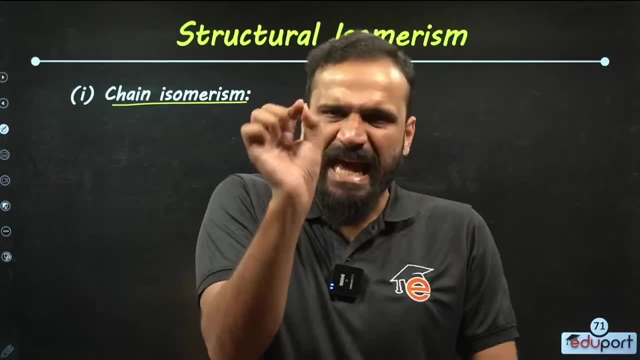 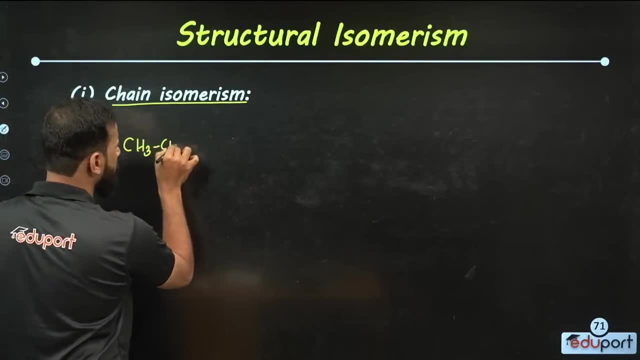 It is in that name. Chain isomerism means that there is a difference in the chain, but the molecular formula is the same. Look, look, look, look children. CH3, CH2, CH2, CH3.. Okay, right. 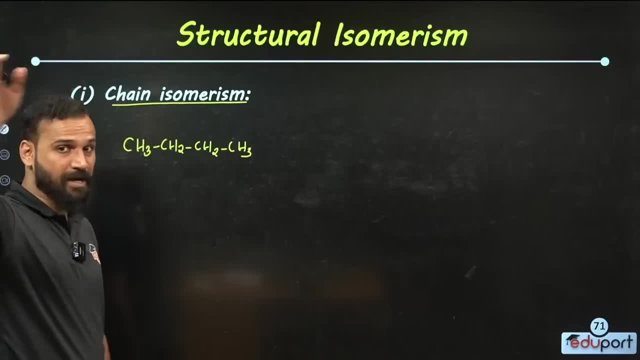 We will take a little more time, children. I will quickly finish the rest of the topic. No one should leave Because you can sit for a while in the main chapter, Or else I would have finished it quickly. We are going to spend the time by asking the maximum number of questions. 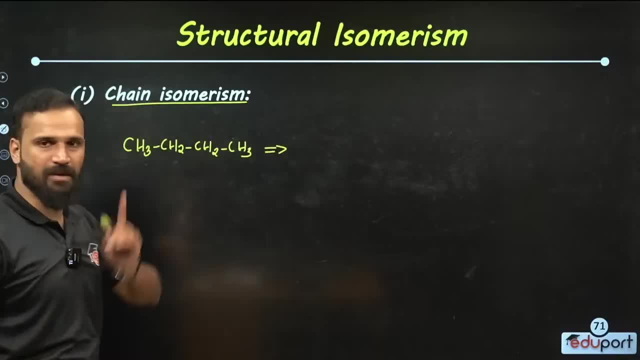 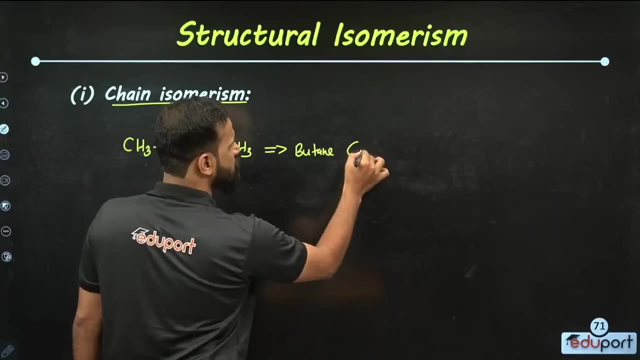 Yes, There is a reason for doing so. That's why, Look, Look, there is carbon, Four carbons, Isn't it butane? Yes, His name is butane. There is nothing to say. His formula is C4H10.. 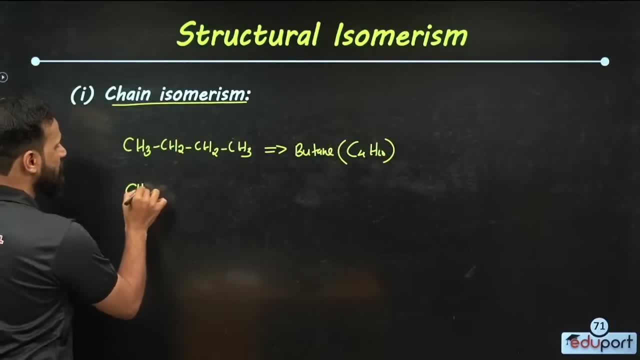 There is nothing to say Now look, CH3, CH2, CH3, CH3.. What is his name? You will say Two methyl, Isn't it? two methyl propane, children, Two methyl propane. What is the name? 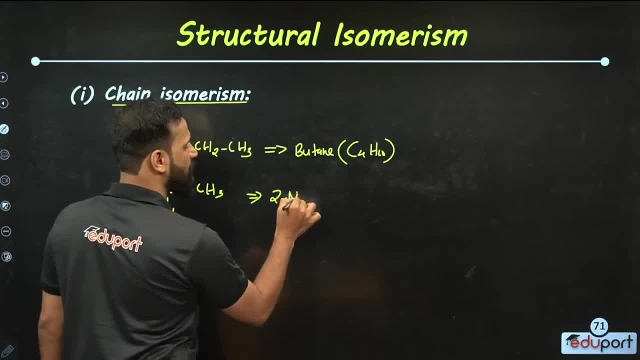 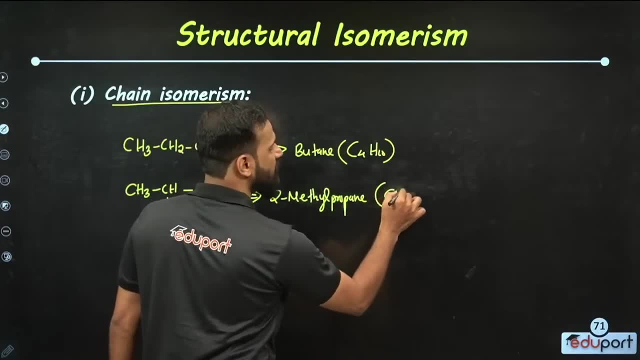 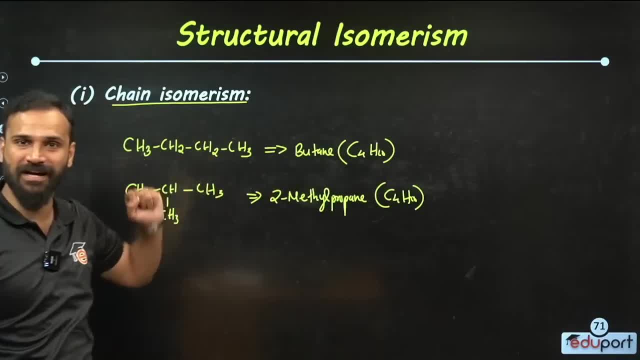 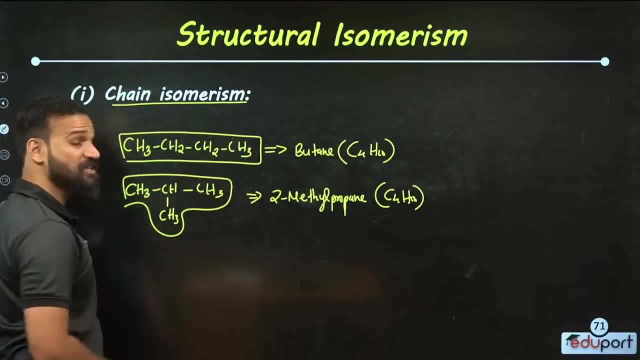 C4H10.. So it is the same molecular formula, But the chain is different. How is that? This is a straight chain. This is a branched chain, Isn't it? So the chain is different, The molecular formula is the same. 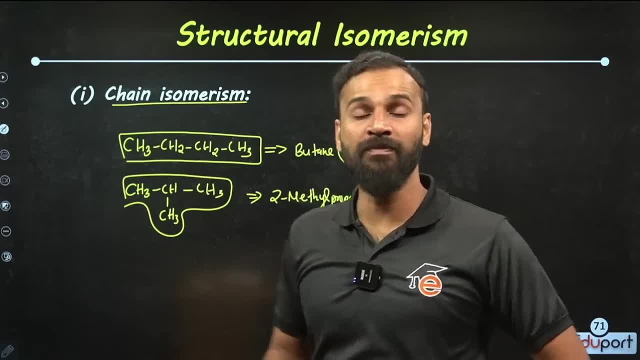 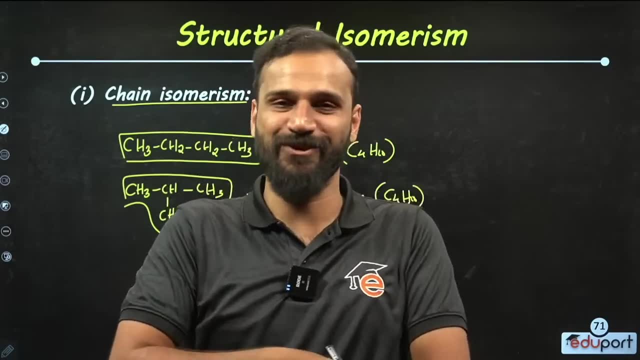 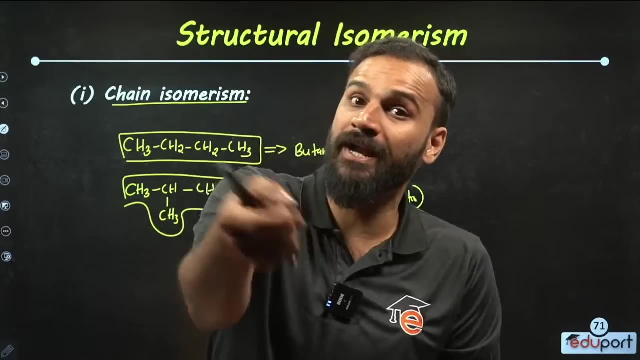 If so, this butane and two methyl propane can be called chain isomers. What is it called children Chain isomers phenomenon is chain isomerism. It is the same molecular formula but it is a different structural formula That molecules, isomers are that phenomenon, isomerism? 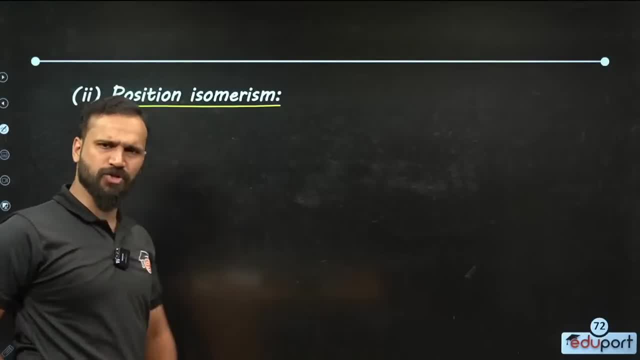 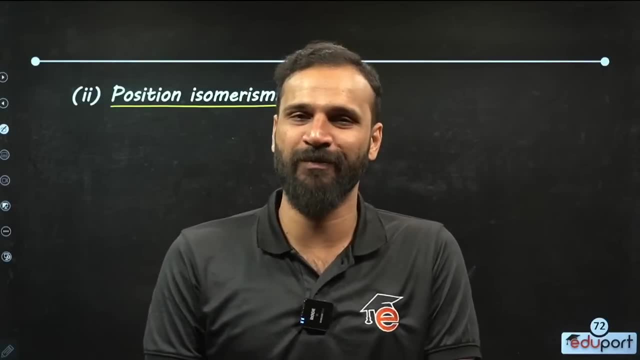 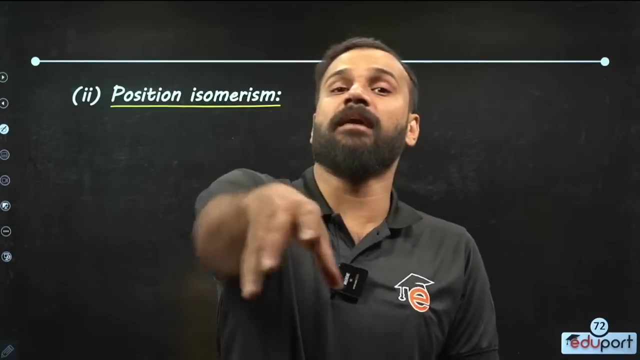 What is the second one? Position isomerism- What position? The position of functional entities is different, But it will be the same molecular formula. What is the position of functional entities? It can be the functional group. inside it, It can be the double bond inside it, It can be the. 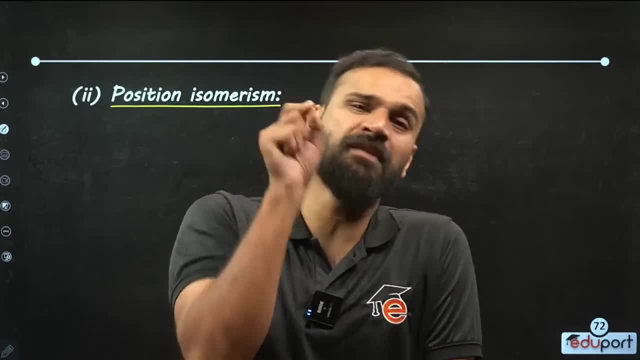 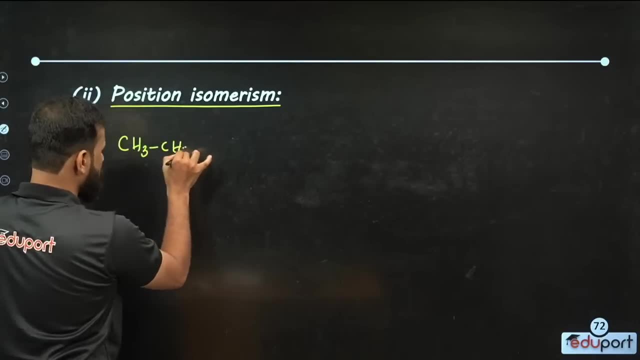 triple bond inside it. The position of such people changes, But the same molecular formula. Look at the children. let me give you an example. Look: CH three, CH two, CH two, OH. Next, Look at the child: CH three, CH, OH, CH three. What is his name? 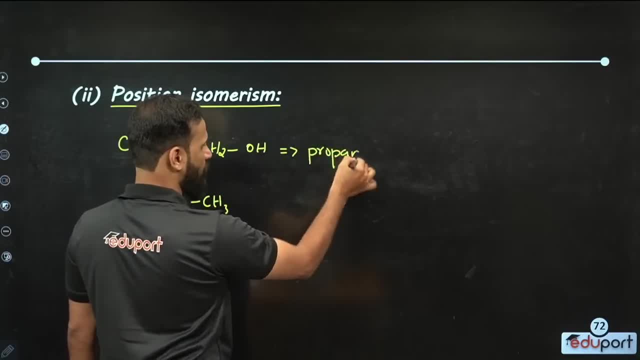 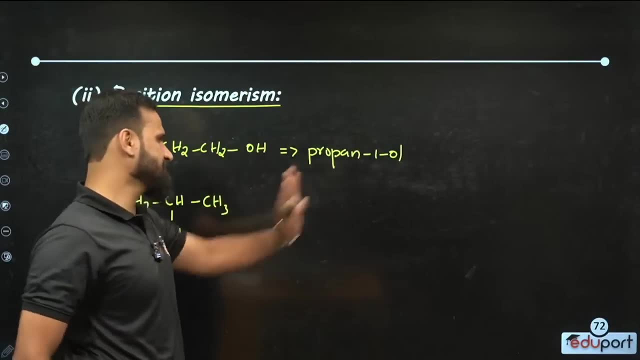 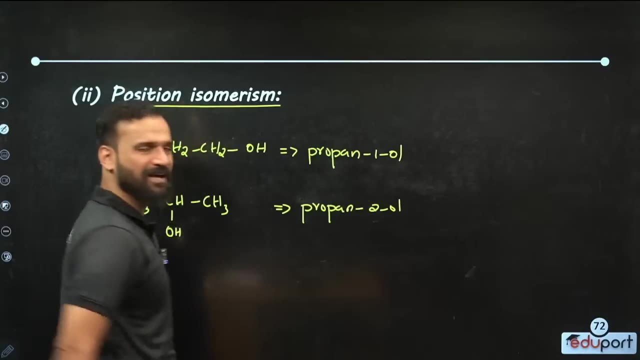 His name is propanol. Propanol. To understand propanol- We know that there is no mention, because it is one To understand What is his name? children, Propan to all. What is it? Propan to all, So what is the difference? Nothing. 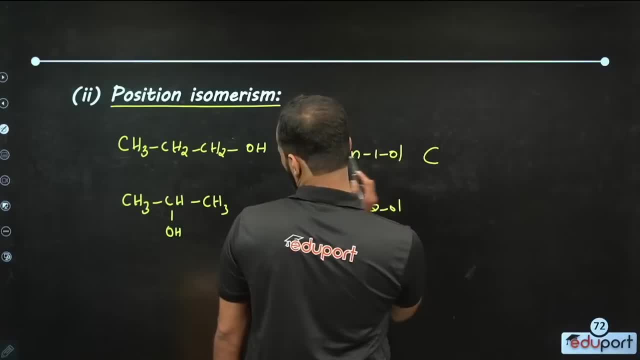 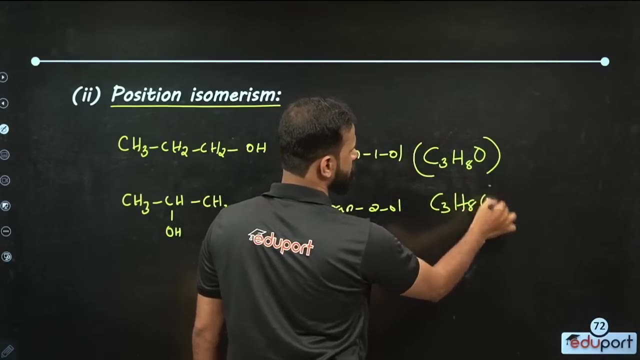 The same molecular formula. What is the prop in the molecular formula? Because it is propane: C three, C three, is not it, children? C three, H, eight O. This is coming: C three, H, eight O. Yes, It is very, very super important. It's very. He opened The. 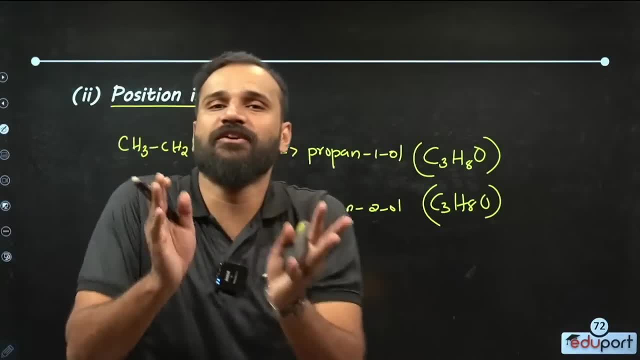 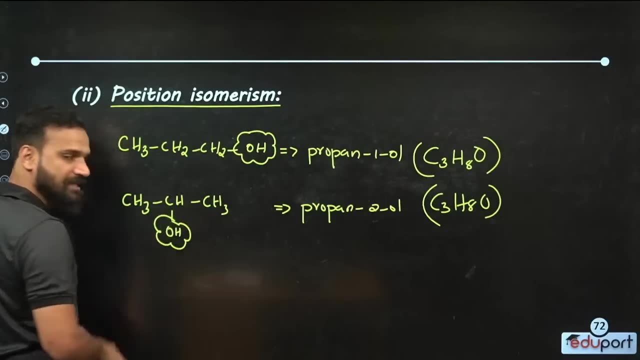 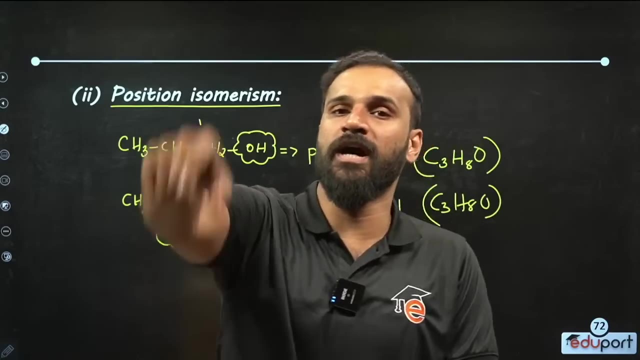 molecular formula of the two people is the same. So why is there a difference here? The reason for that difference is the position of the functional group here became different. Here is the first component function group. there are two here, Whether it is such a group, the double bond or the triple bond. the position: 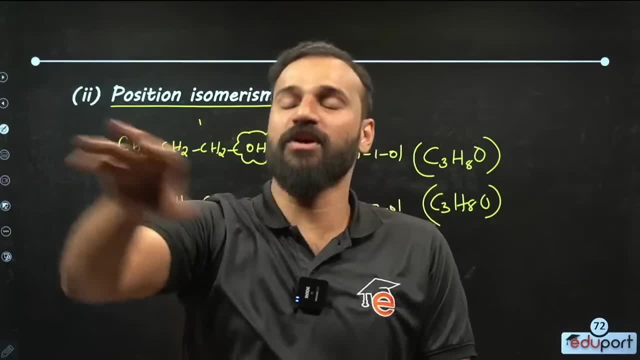 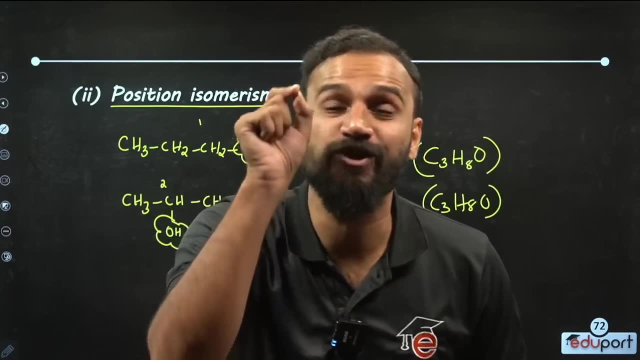 of such people is only different, But if there is no defect in the molecular formula, things will be good and bad because it is the same. let they are position isomers. What is that phenomenon? Remember that it is position isomerism. 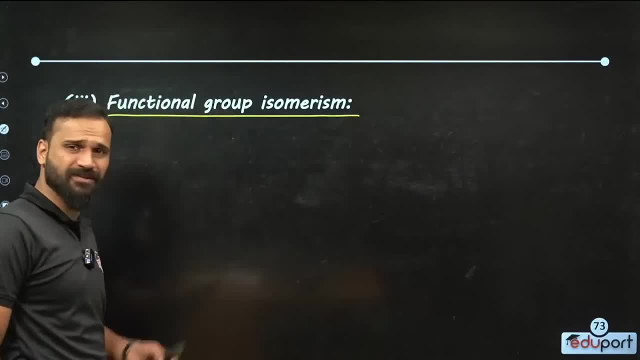 Now children, functional, iso, functional group, isomerism. What to say? It's in the name, Same molecular formula, But the functional group is different. Look, children, Look, you, look. CH3CH2CH2OH. Who is this? 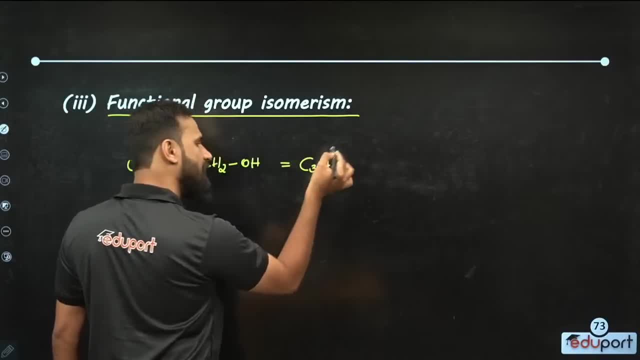 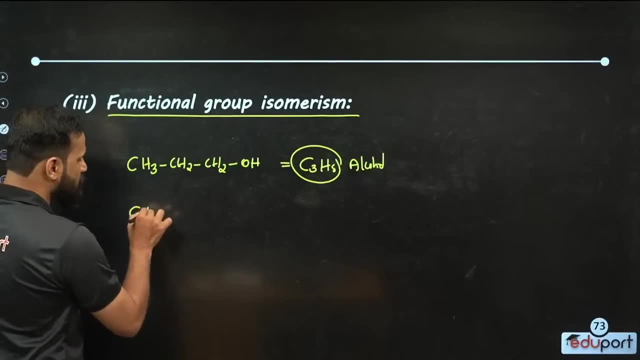 children. As I said earlier, the C3H8 is the one. The functional group in this is OHL, isn't it OHL, isn't it? Isn't this alcohol children? Yes, Now I'm here. Be careful. CH3OCH2CH3.. If you take In this in this. 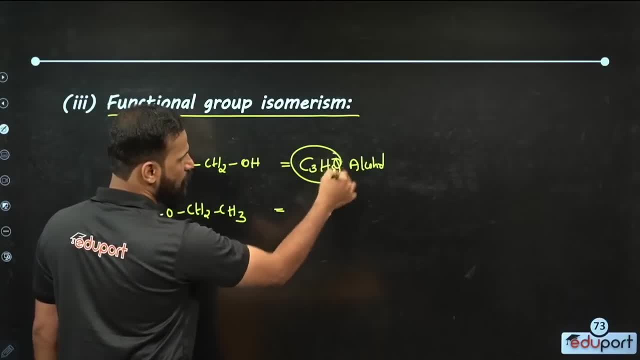 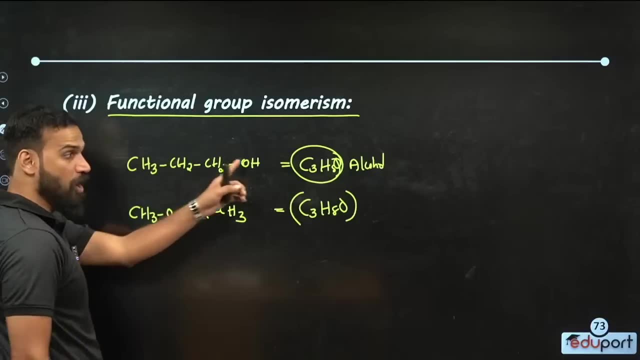 The molecular formula is also sorry. here is C3H8O. The formula in this is also C3H8O, But this, When the molecule group comes on both sides of the oxy, is it? Is it alcohol? Not, This is an ether. 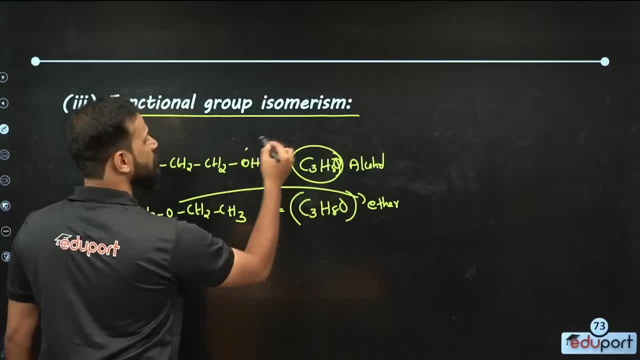 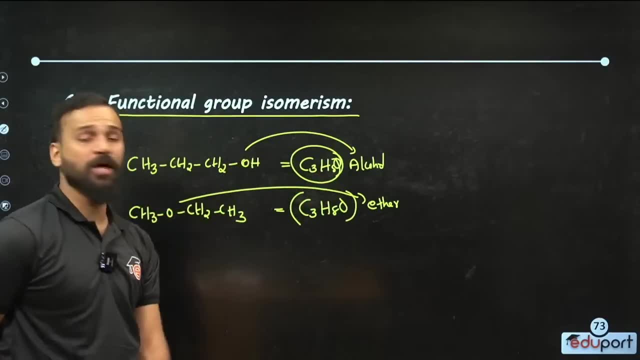 This is an ether. This is an ether. This is an. It's alcohol. So children be careful. In the same, It is in the molecular formula. What is it In the same? It is in the molecular formula, But the functional group. 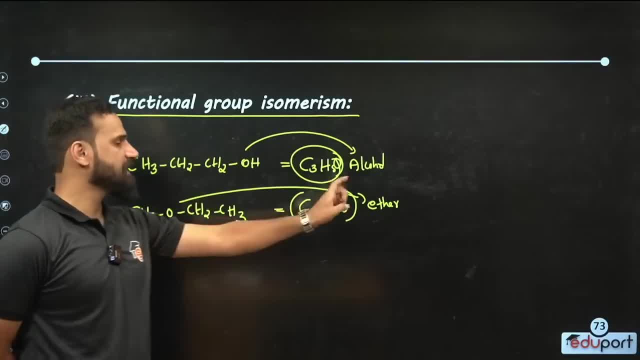 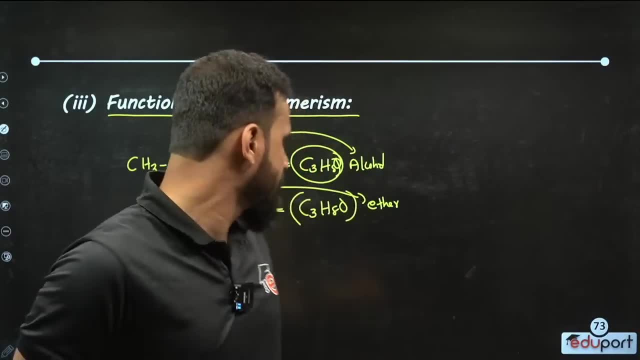 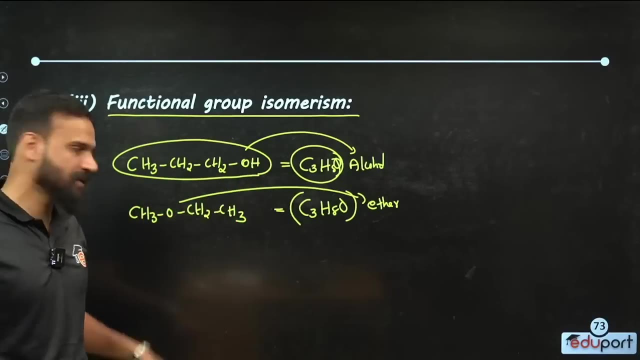 Difference: Here is alcohol, Here is ether. If so, what can we call these molecules? Functional isomers? You know, His name is propanol, His name is methoxy ethane, Methoxy ethane. So propanol and methoxy ethane. 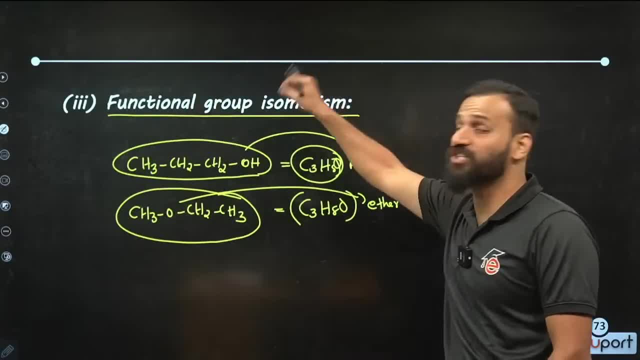 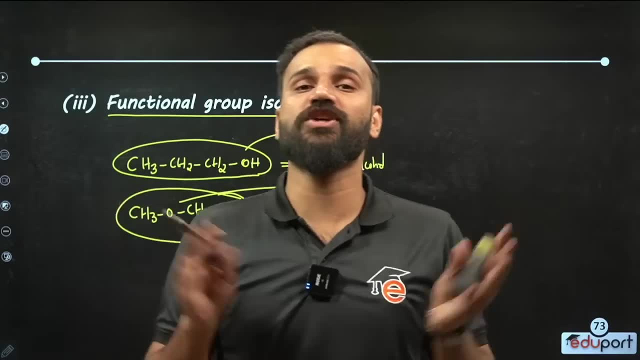 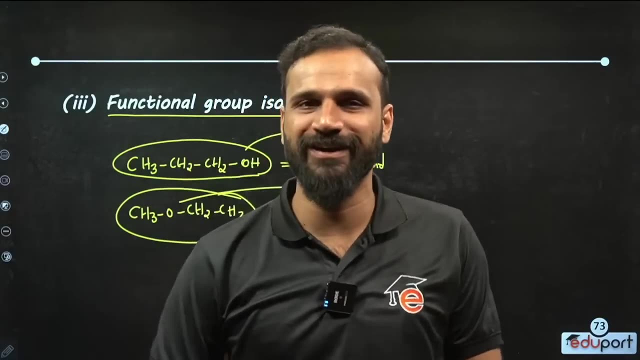 What? What is it? That's the functional compounds Example, Because it is in the same molecule of formula, But Functional group is two places. What is it? Is it different? is that that Children cooked very careful? A very important thing is: This is all Okay. children, Yes. now 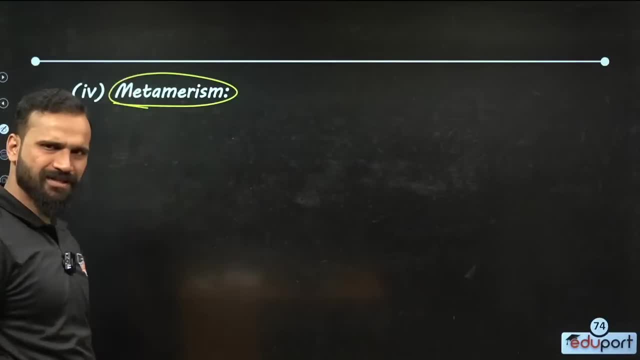 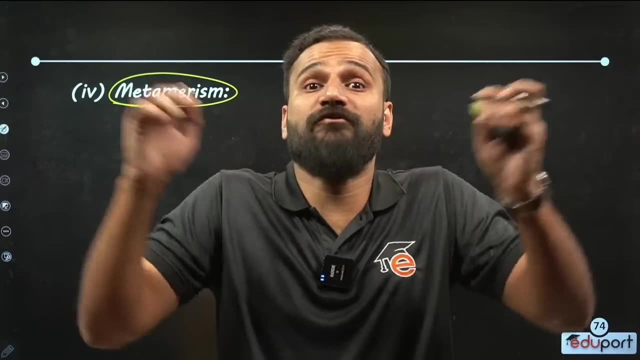 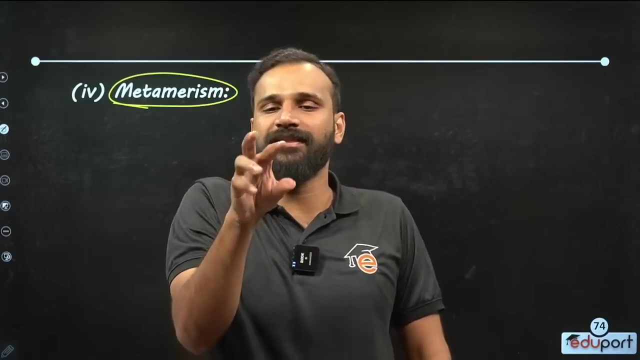 finally met 각 metamerism. Metamerism or who is metamors? Same molecules in molecular form. What is it? Same Metamors are molecules in molecular form But Alkyl group on both sides of the functional group inside that molecule. 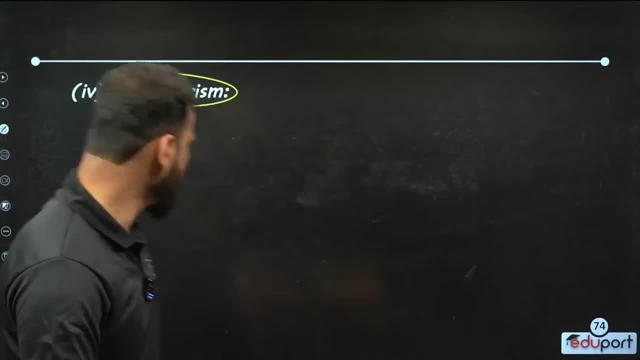 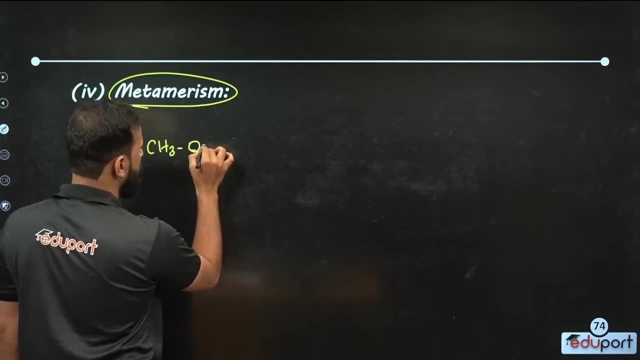 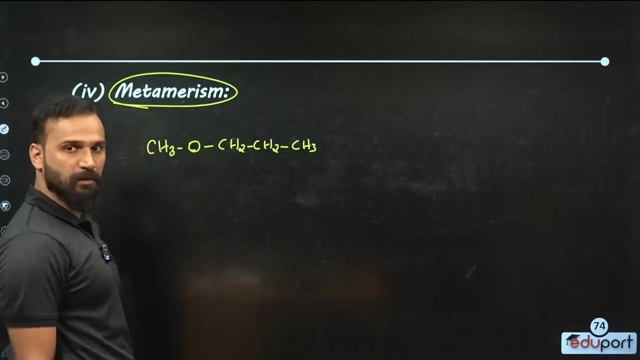 will be different. That is the specialty of metamors, For example, children, if you look at it. if you look at it: CH3CH3OCH2CH2CH3.. Okay, his name is methoxypropane. Next. 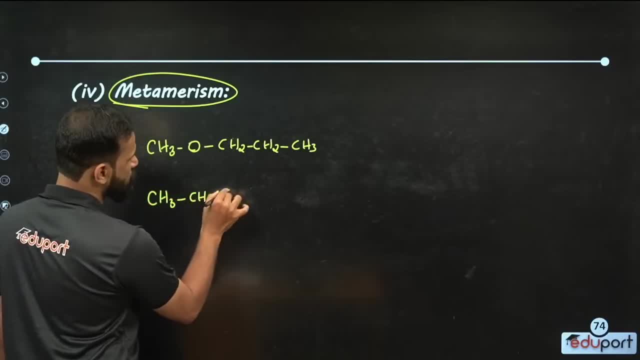 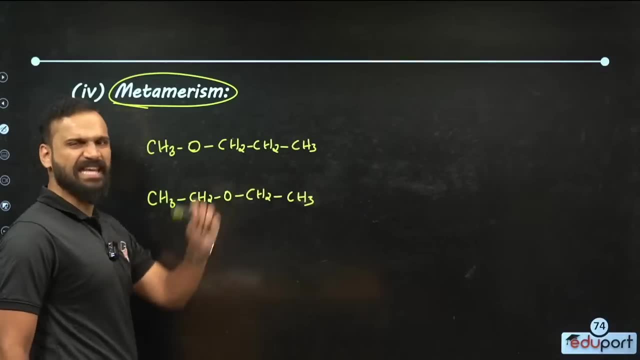 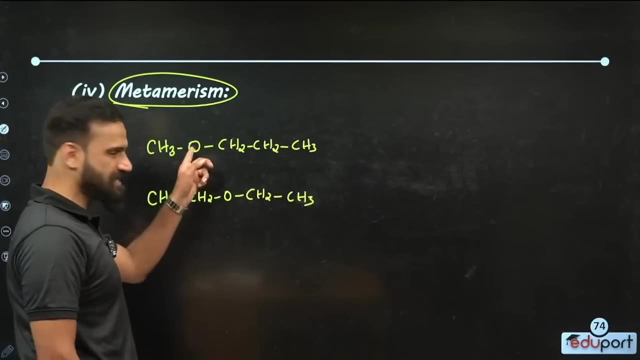 person if you look at it: CH3CH2OCH2CH3.. What is it, children? His name is ethoxyethane. So what is the thing? What is the thing? You have to understand it. There is a functional group here. This oxygen is the. 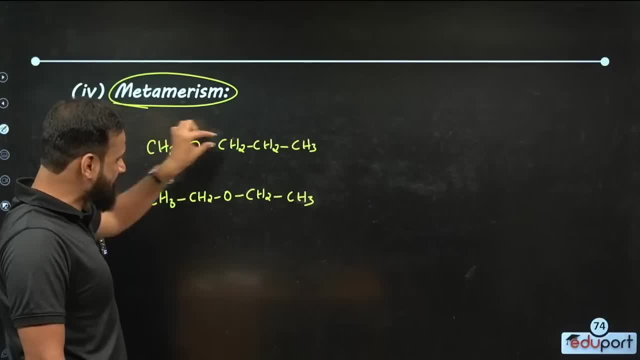 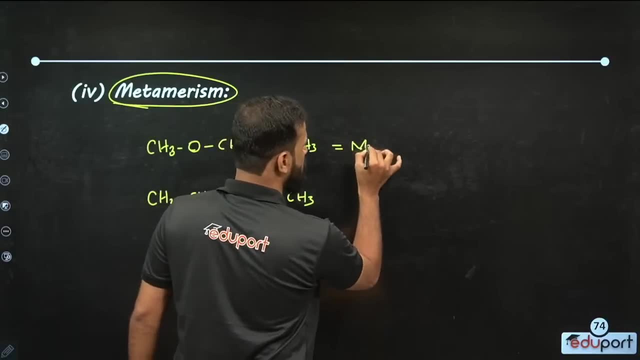 functional group. The alkyl group on both sides of that functional group is different, But there is no difference in the molecular formula. We are methoxypropane First, methoxypropane right, Isn't it? methoxypropane children? 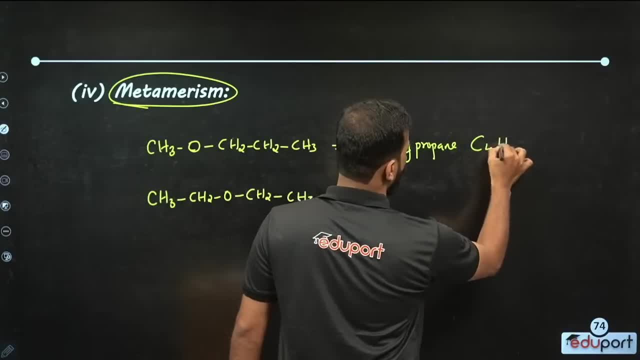 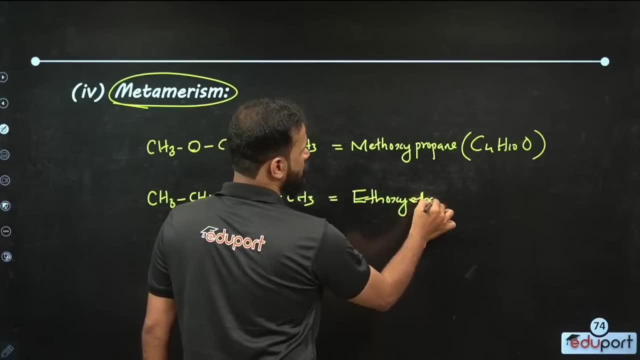 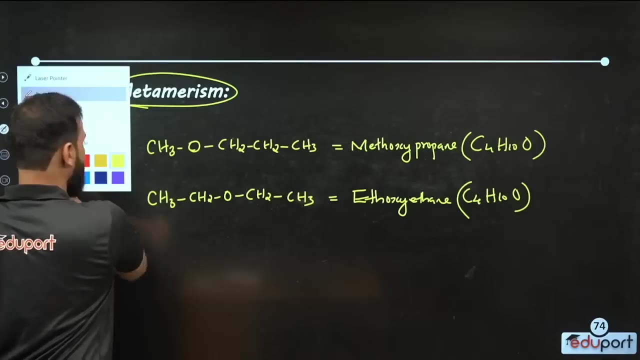 What is the formula of methoxypropane C4H10O? The second one is ethoxyethane. right, It is ethoxyethane, Ethoxyethane, C4H10O. Then what is the difference? Alkyltube on both. 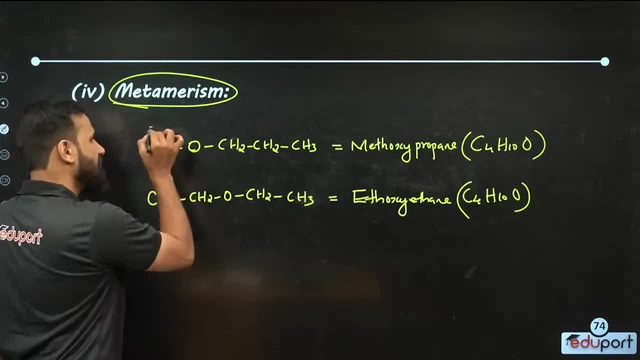 sides of this functional group is different. Here is one l, so it is a methyl. how, what do you say? alkyltube with a carbon? It has two carbons left of this alkyltube, So the one on the left is different. Now go to the right: Three carbons. 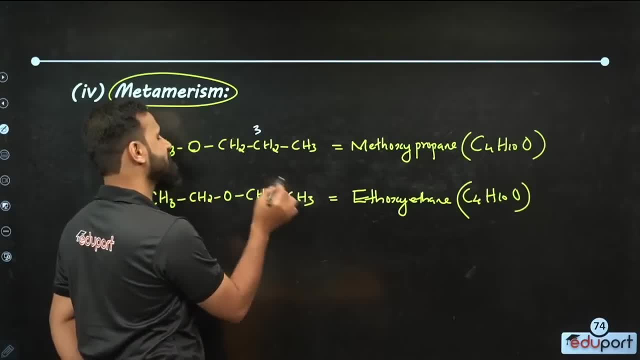 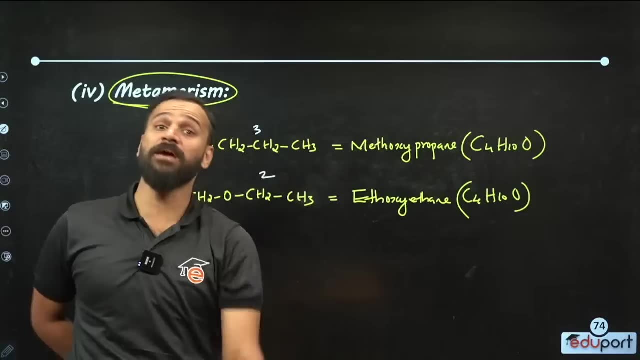 are in the right side of this alkyltube. Two carbons are in the right side of this alkyltube. Then is the molecular formula of both same or not? it is very same, But what is the difference? Alkyl group on both sides of the functional group. 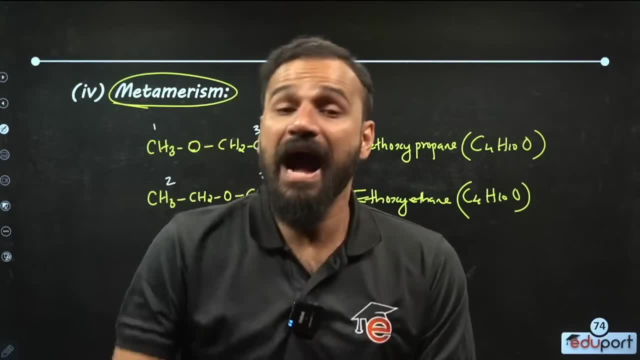 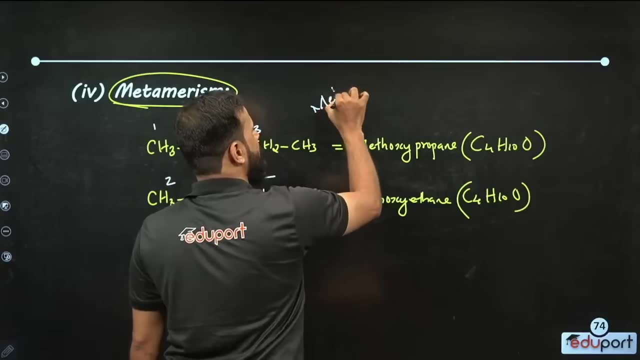 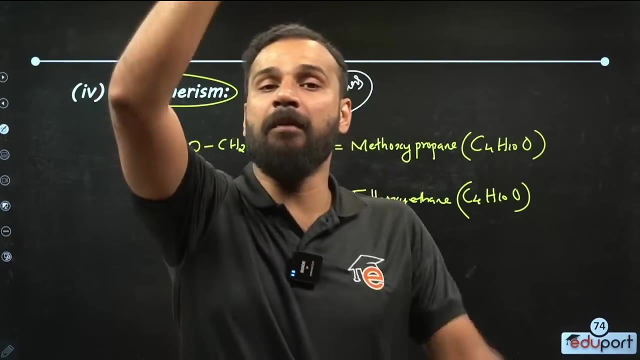 in it is different. If so, the name we call them is metamors. What is the name they call? What is the name they call Metamors? What is the name of that phenomenon That is called metamorism? Those molecules are metamors. 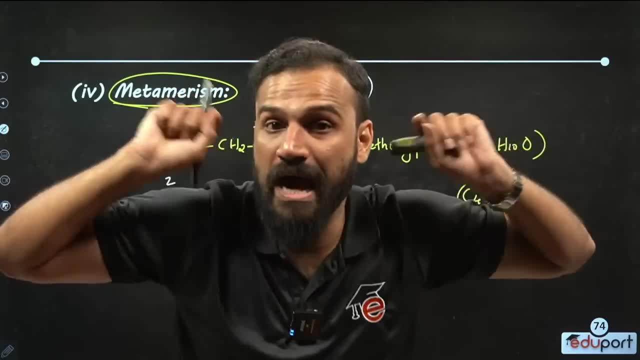 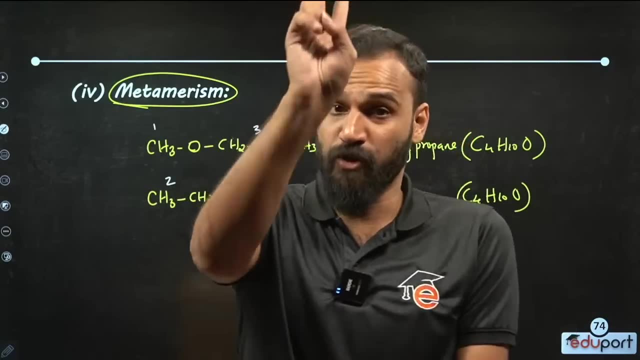 The name we call that phenomenon is metamorism. What is it called Metamorism? So children, chain isomerism should be learned, position isomerism should be learned. functional isomerism should be learned, metamorism should be learned. 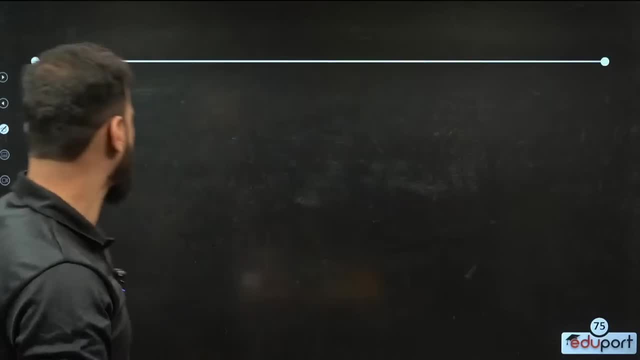 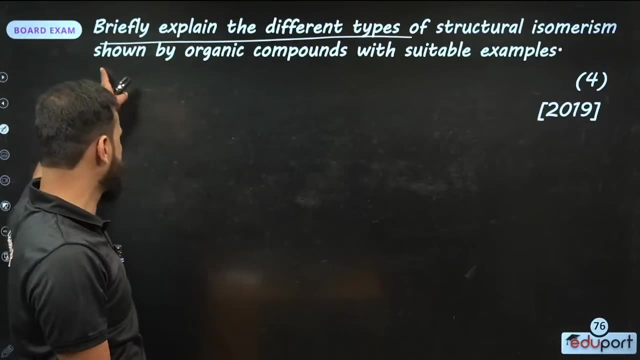 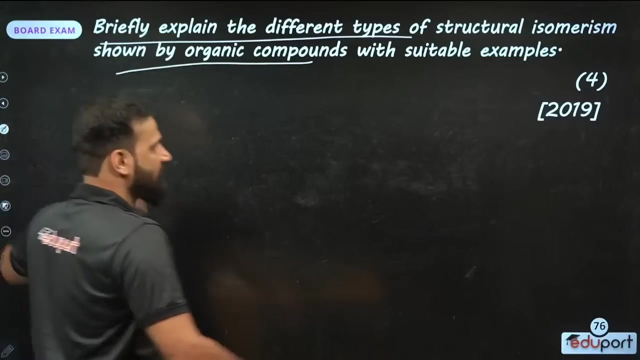 Each one needs an example. Each one needs an example. Look you look. briefly explain different type of structural isomerism shown by organic compound with the suitable example. two thousand and thirteen. You have to understand why you have to give four marks here. 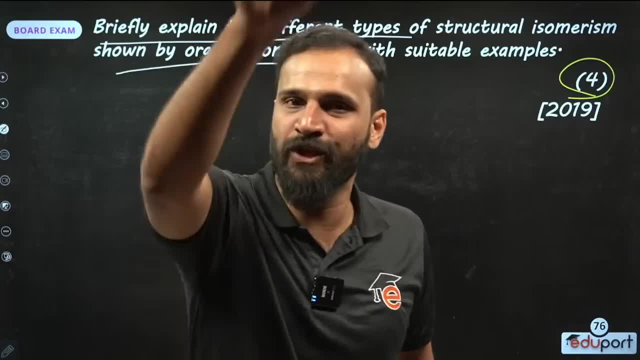 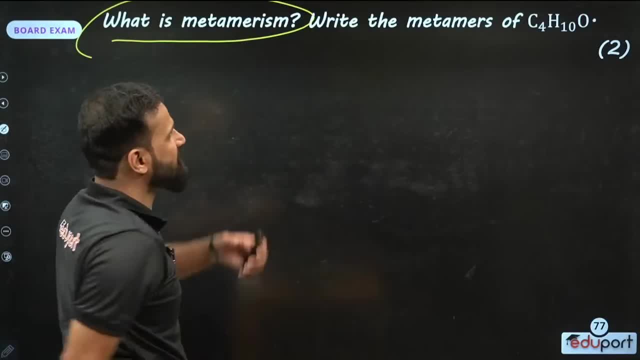 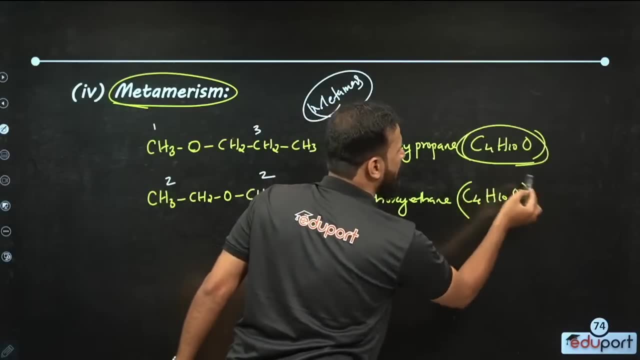 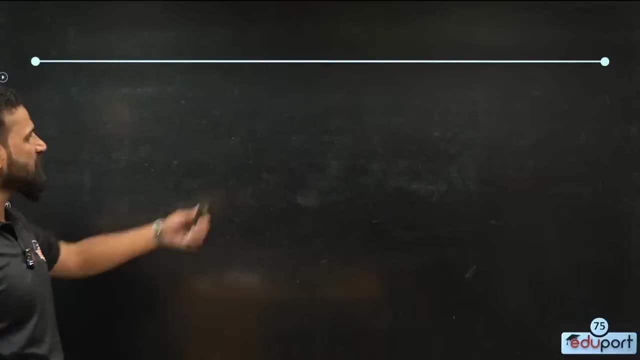 what is isomerism? Write the metamors of C4H10O. I have not written it because I have already written C4H10O, or the metamors that show it are methoxypropane and ethoxyethane, Isn't it? We have already done it, Already done it. 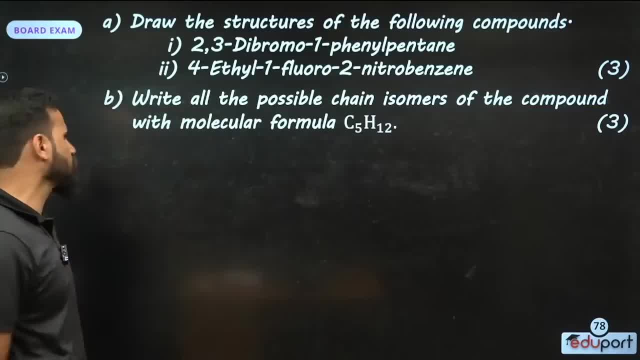 Now draw the structural formula. We don't have to say it, we have already said it. Now write all the possible chain isomers of the compound with the molecular formula ah- C5H12.. All possible chain isomers of these C5- H12 molecules. 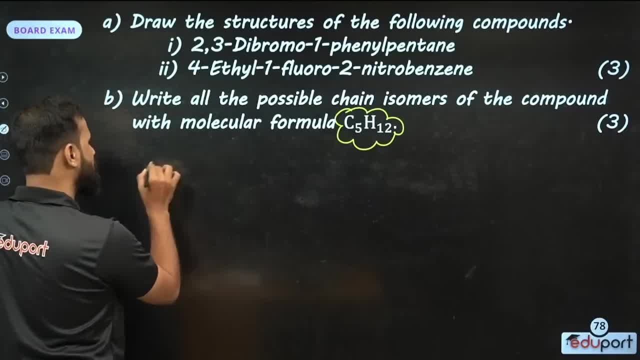 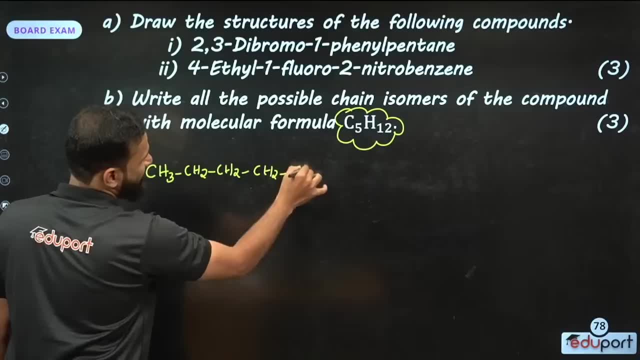 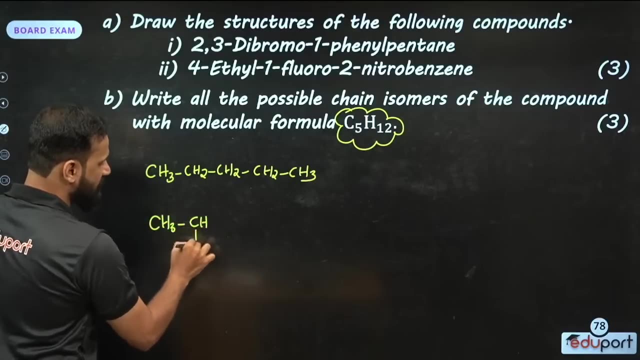 chain isomers. So if we say C5H10, first, we can do straight chain: CH3, CH2, CH2, CH2, CH3.. Right, This is C5H12.. Now look guys: CH3, CH, CH3, CH2, CH3. 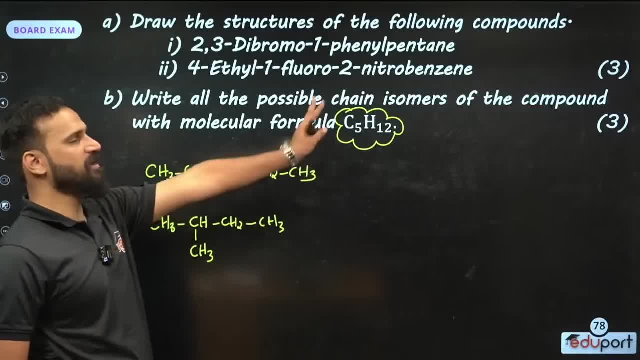 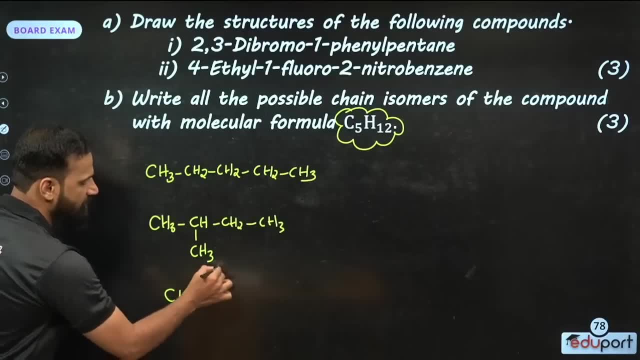 Ok, So if it comes like this, this is also C5H12.. If this is normal pentane, this is 2-methyl butane. Now one more is possible. How is that? We can give CH3 here, CH3 here. 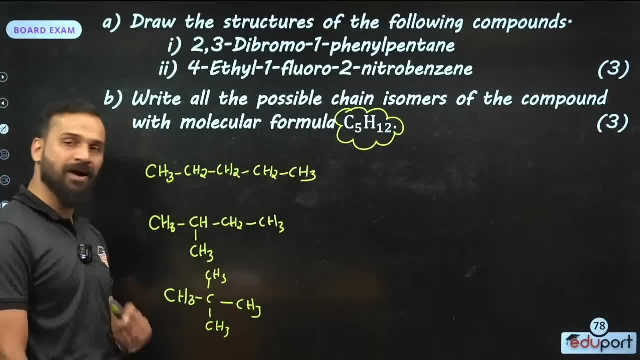 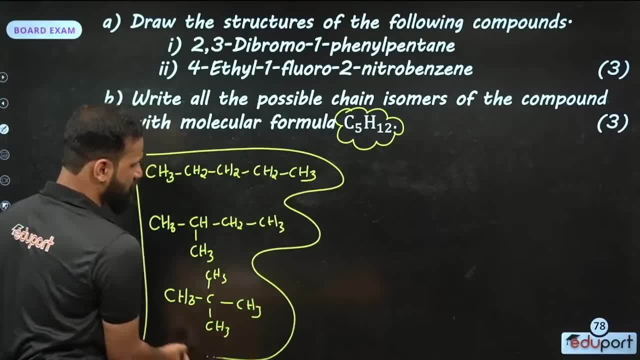 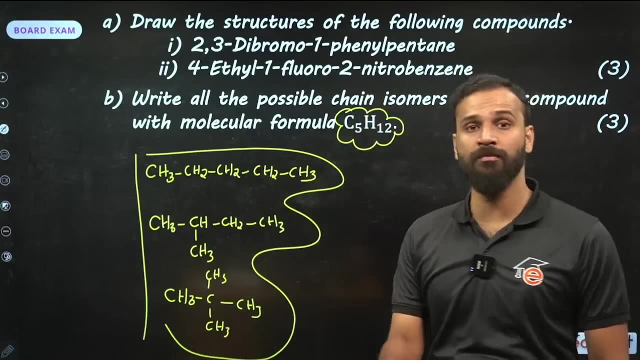 CH3 here. What is this? This is also C5H12, but the name is 2,2-dimethylpropane. What are these three? These are the possible chain isomers of C5H12, kids. So isomer chain isomers are in the same molecular form. 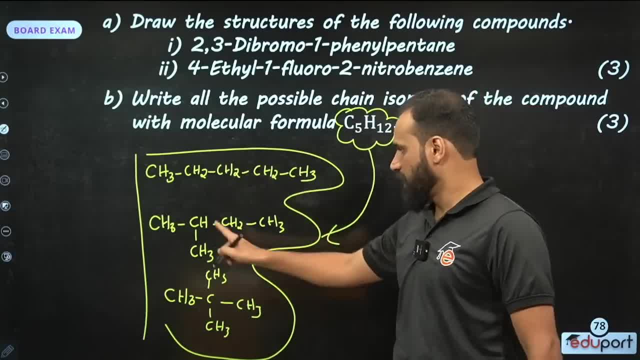 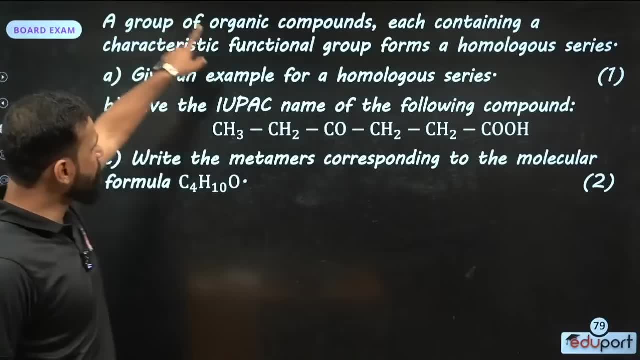 but there is a difference in the chain. This is a straight chain. This is one branch chain. This is a chain of two branches. Understand Now. look guys. A group of organic compounds each contains a characteristic functional group, form a homologous series. Give an example. 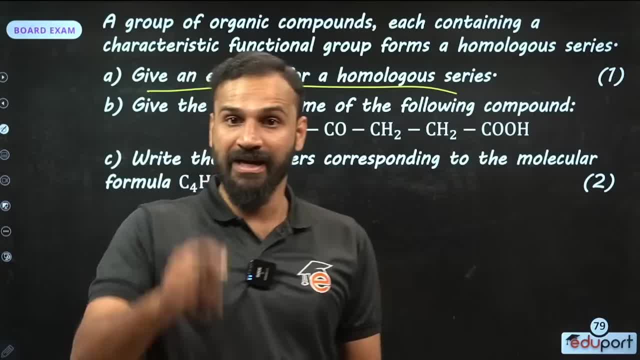 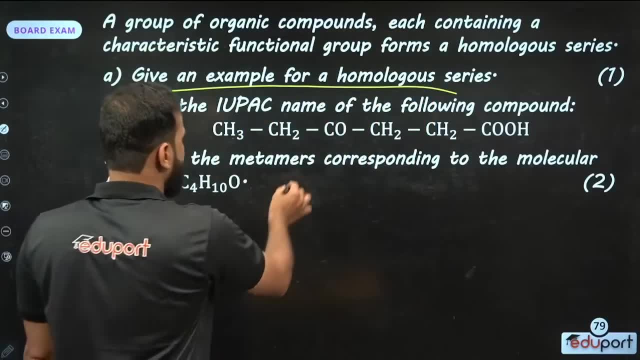 of homologous series. Earlier we had written right CH3, CH2OH, then CH2AD, CH2AD. If it comes like this, it is a homologous series. Now, guys, the IUPAC name of this we just said. 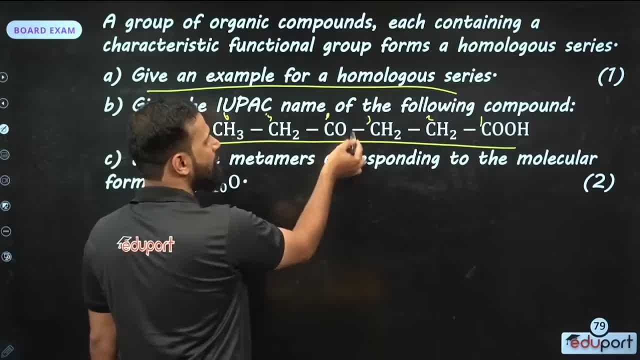 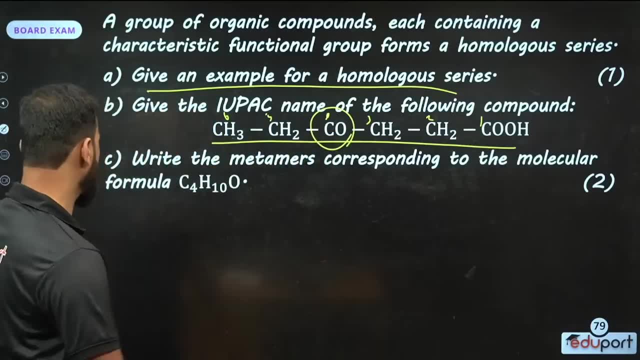 earlier: 1,, 2,, 3,, 4,, 5,, 6.. So what is it? This is the homologous series. So what is it? 4-oxohexanoic acid. 4-oxohexanoic acid. Write the metamors corresponding. 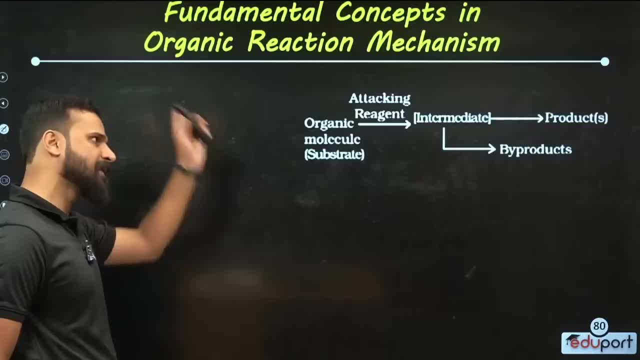 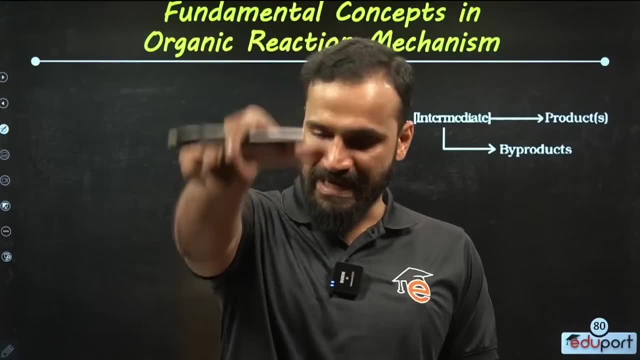 to the molecular formula C4H10O. The metamors of this is what we had written earlier. Okay, So, guys, if we say isomerism, what is it? Four structural isomers are what? Chain position, functional and metamors. 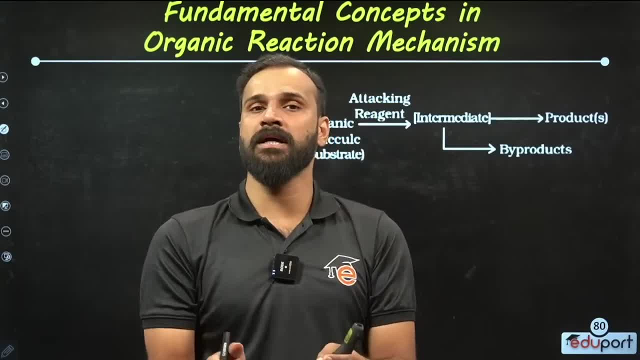 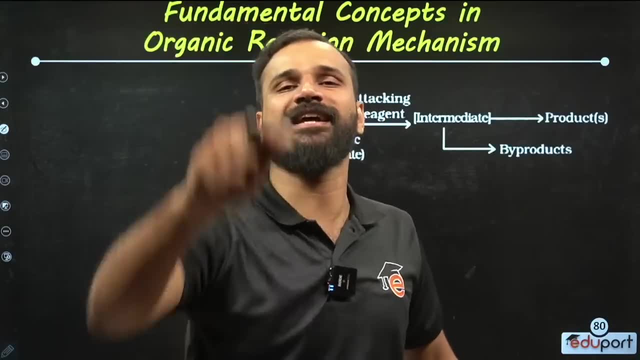 We studied with the example. What the exam asks is then: isomerism is what you learn from 10th grade. You have to study accurately with the example, Because that's what the exam asks. Now, guys, look we go to the reaction mechanism. What is a reaction? 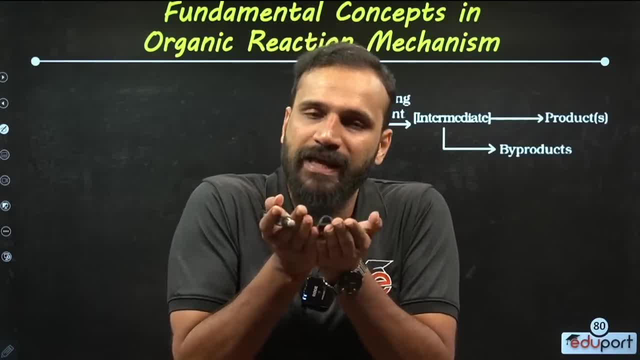 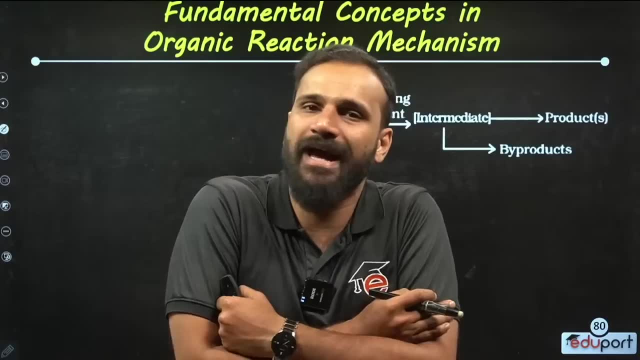 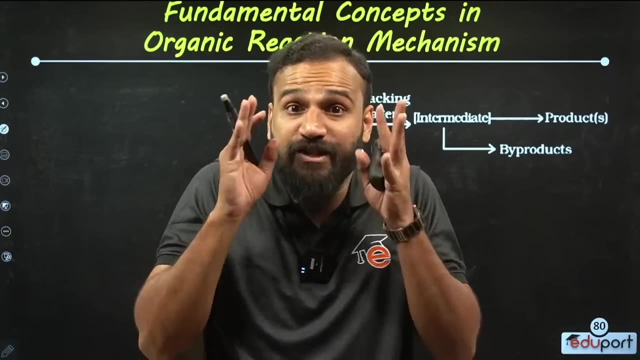 A reaction is basically a reactant molecule. It is called a substrate. I am a reactant molecule. I think it is a substrate. I won't react like this. If a reaction is going on, another reagent should come to me right. That day is called an attacking reagent. 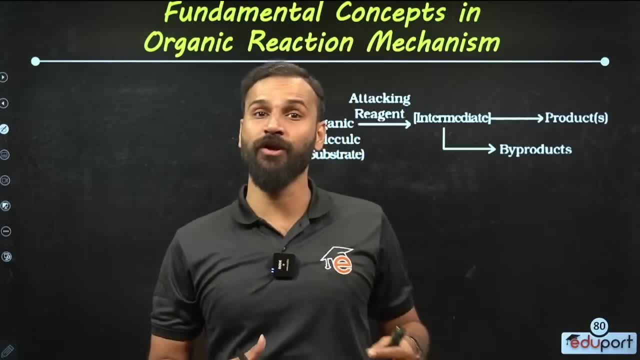 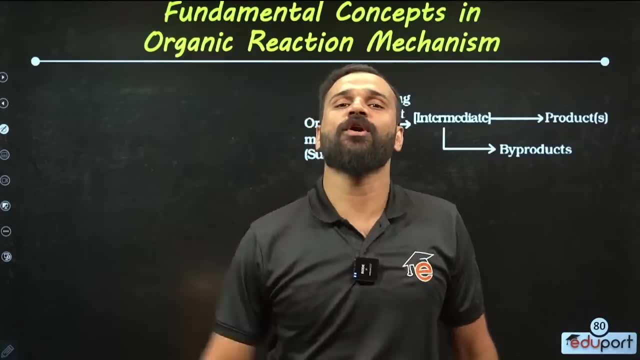 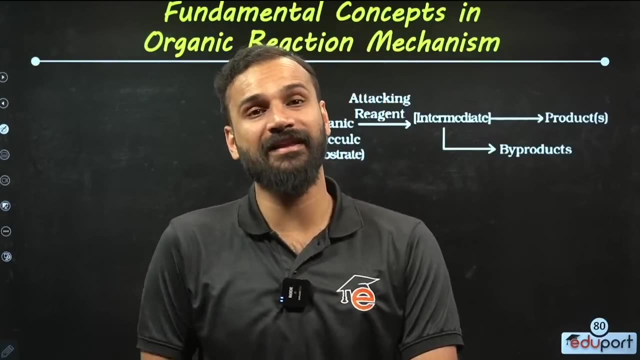 So a substrate molecule, that is a reactant molecule, reacts as an attacking reagent and turns into a product through an intermediate. It turns into a product through an intermediate. Okay right, Intermediate means the carbocation that is involved in it. 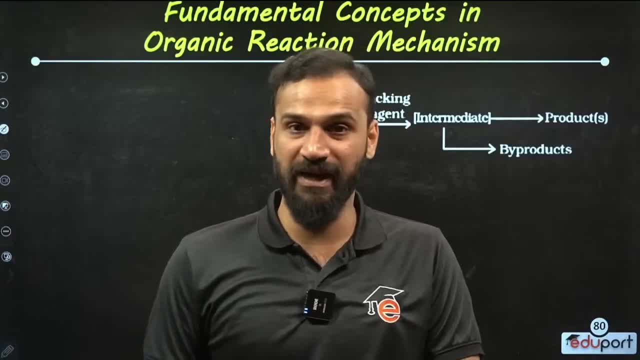 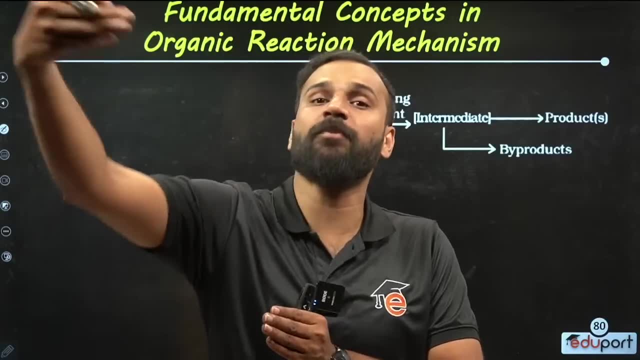 anion, carbanion, free radicals, etc. It is called an intermediate. So a substrate molecule reacts as an attacking reagent and turns into a product through an intermediate. That is called a reaction. Okay, right At times, what happens with a product? 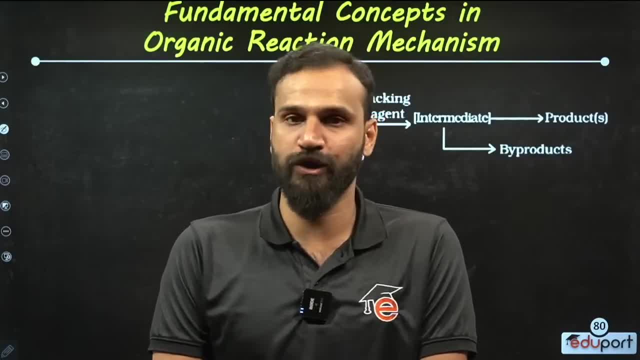 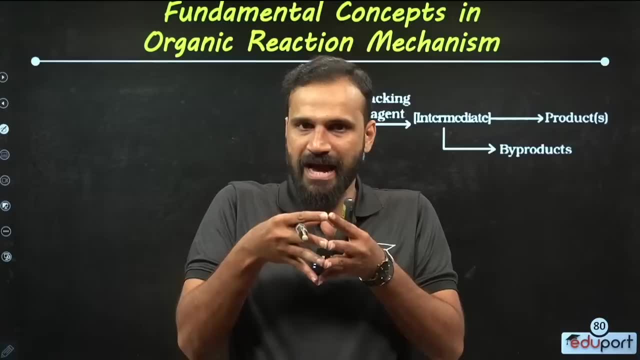 Keep in mind that there is a byproduct. Now, guys, look, we have just said right: A substrate molecule, An attacking reagent comes for it, They react, and there is a product through an intermediate. It may be byproduct, Isn't that what I said? 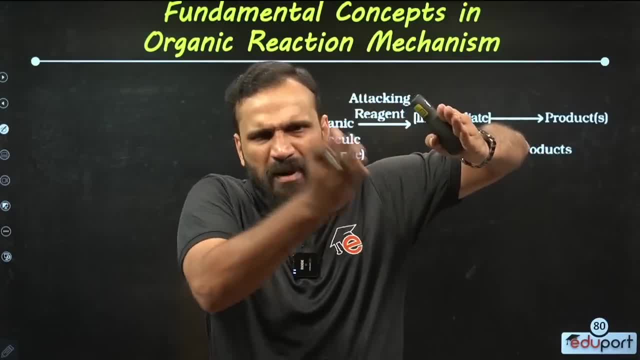 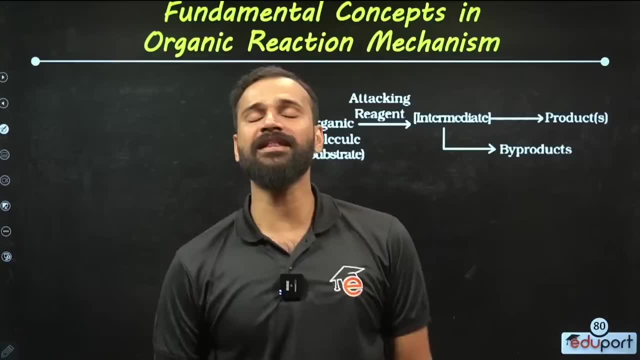 Each of these is a sequential, step-by-step reaction. This is called a mechanism. What is this called Mechanism? Now, guys, there is something you need to understand. What does it say In an organic reaction if it happens for the first time? 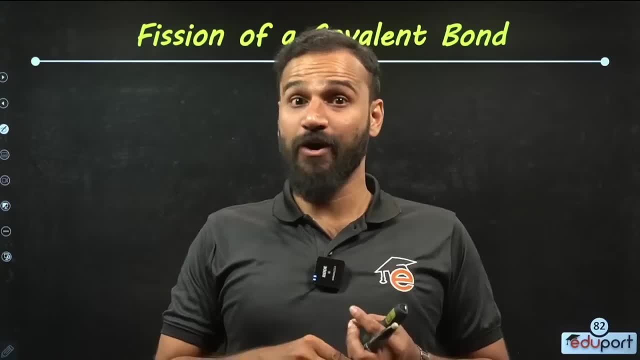 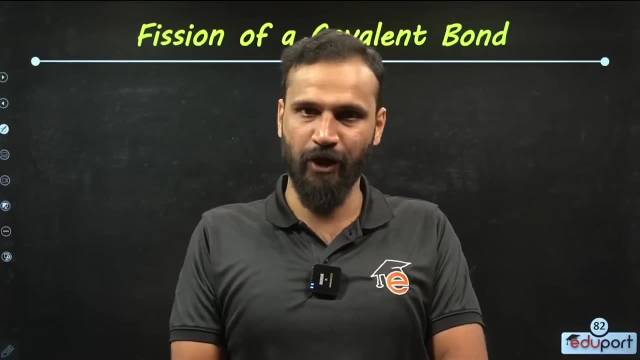 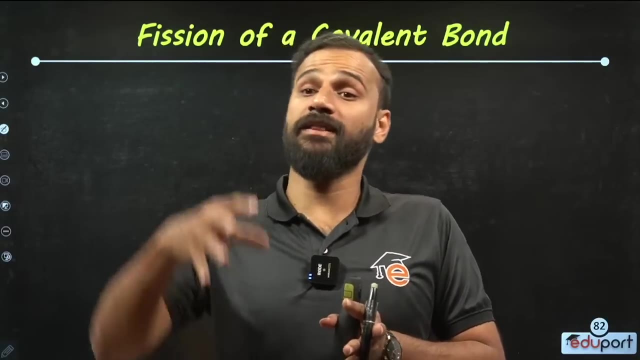 some bonds in the ground will break. If an organic reaction happens for the first time, some bonds in the ground will break, Okay right. And then some new bonds will make. Some bonds in the ground will break in reactants And then some new bonds will make as an attacking reagent. 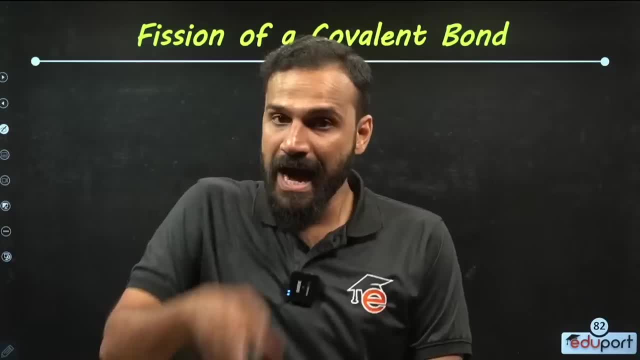 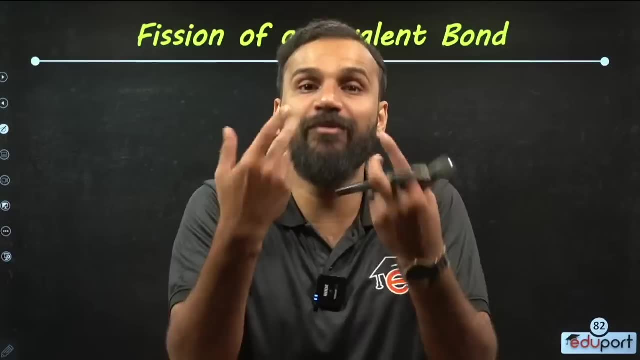 That is how reactants become a product, Or keep in mind that an organic reaction is happening. So what is the first step? The bonds in the ground should break covalent bonds. There are two methods to break such a covalent bond. 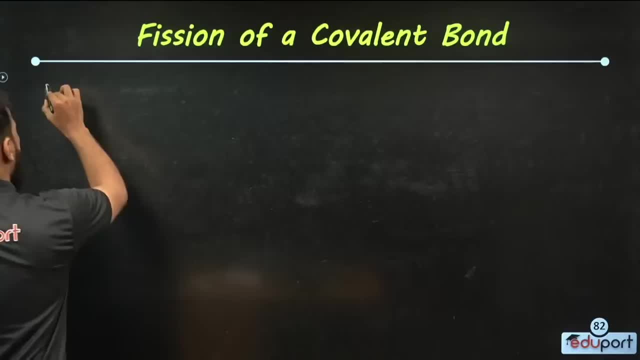 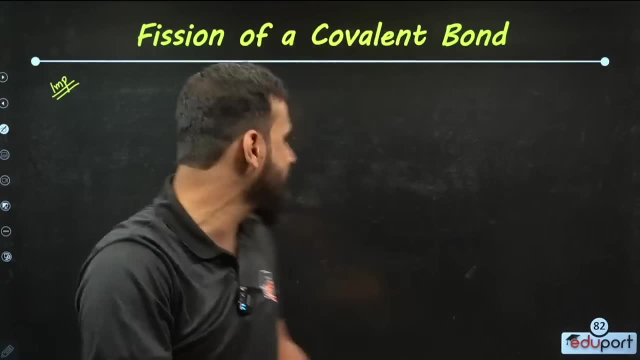 That is what the exam always asks. It is important for the children to mark and learn. It is important to mark and learn: Look: fission of a covalent bond. Look, fission of a covalent bond. If we say fission of a covalent bond, 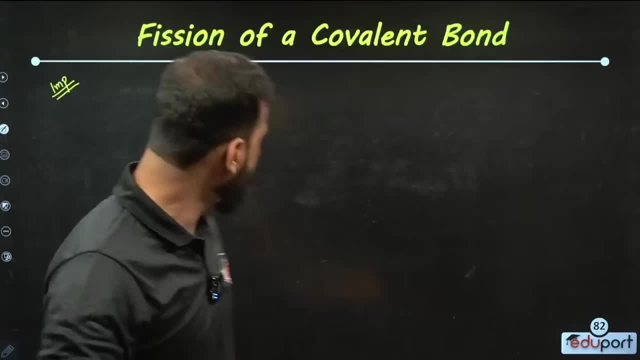 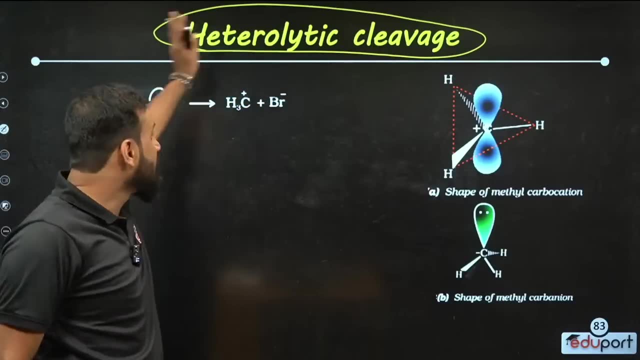 there are two methods to break a covalent bond. One of them is heterolytic breaking. Cleavage means breaking Heterolytic breaking. How do you know that, guys? How do you know that? It is very simple. 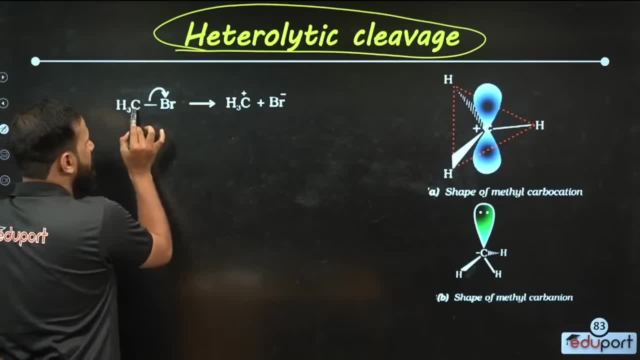 Look here: There is a bond between carbon and bromine, a covalent bond. It is breaking. How does it break? There are two electrons in it. A bond is two electrons. Those two electrons take bromine. If those two electrons take bromine, 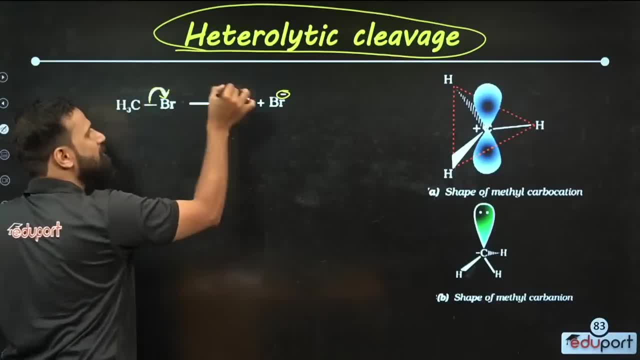 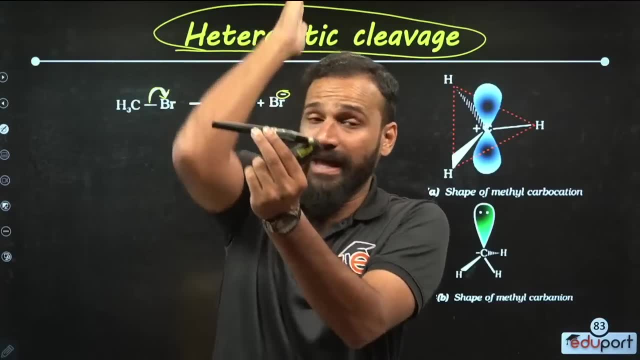 bromine will have a negative charge. The carbon bond here will have a positive charge. This is how it breaks. That is, there is a bond between two bonds. How does that bond break If one person takes two electrons when it breaks? 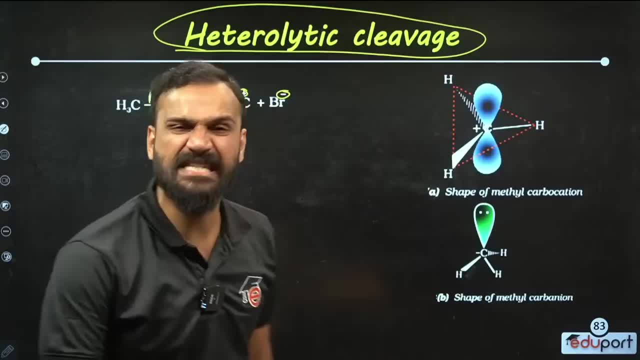 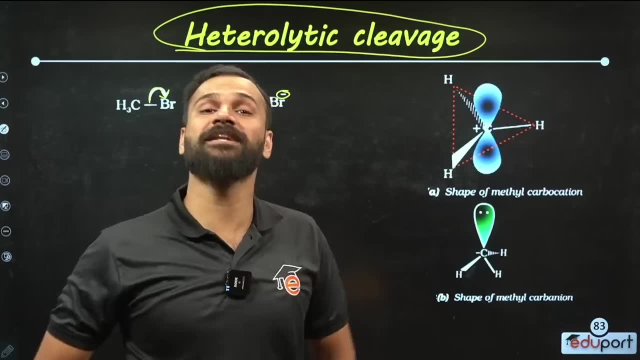 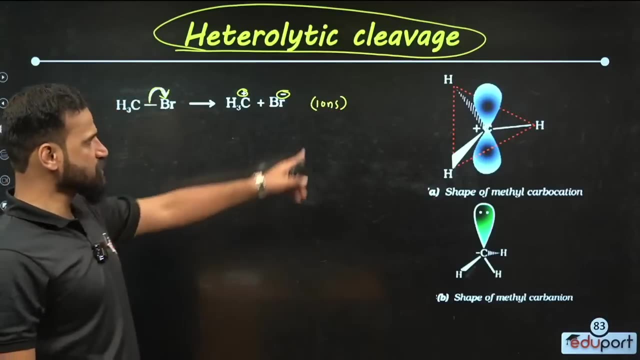 the breaking is called heterolysis, It is called heterolytic cleavage, It is called heterolytic fission. Do you understand What is the product of that? The product of that is always ions. Remember, The product of heterolysis is always ions. 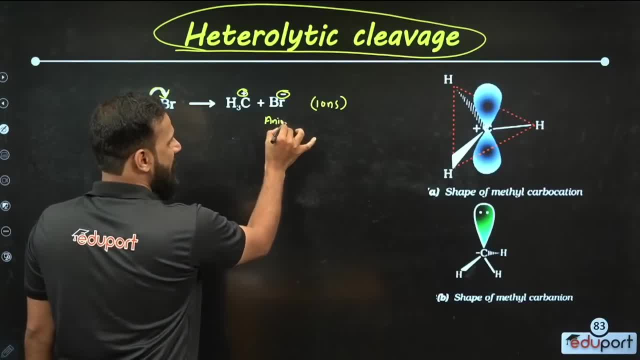 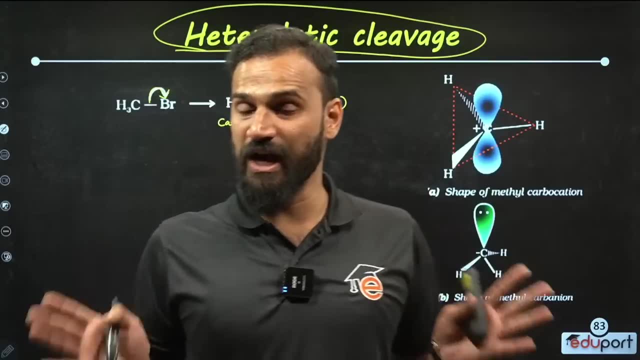 One ion. the ion with a negative charge will be anion. The ion with a positive charge will be cation. What is it? The ion with a positive charge is cation. The ion with a negative charge is anion. Now look at the kids. 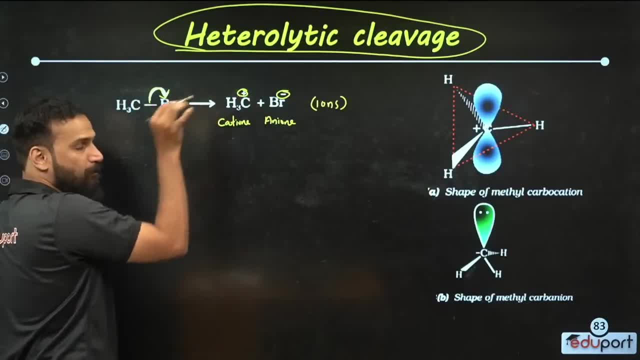 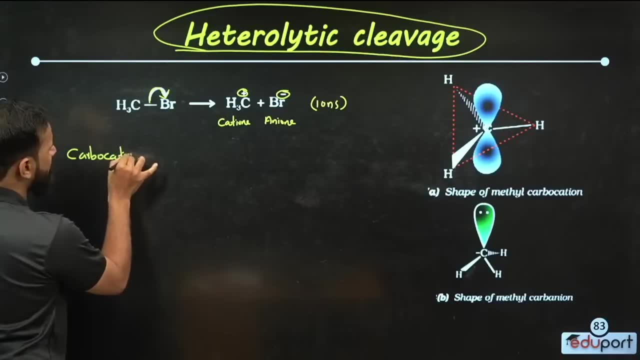 The one with a positive charge is carbon. I mean, if it is carbon, we will call him carbocation. What do you call it, kids, Carbocation? The main feature of carbocation is carbocation is unstable. What is carbocation, kids? 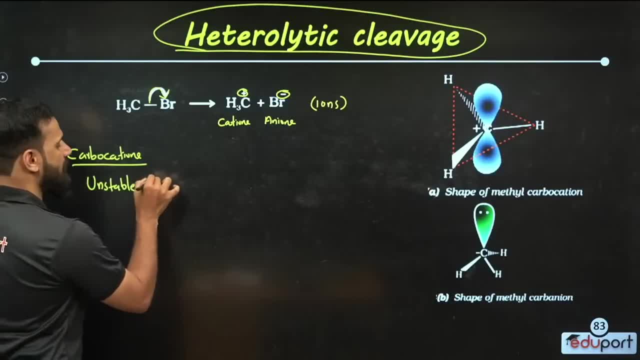 It is unstable. Likewise, carbocation is highly reactive. What is carbocation? It is highly reactive. What is carbocation? The form of carbocation is called trigonal planar. Look at the kids: It is trigonal planar. 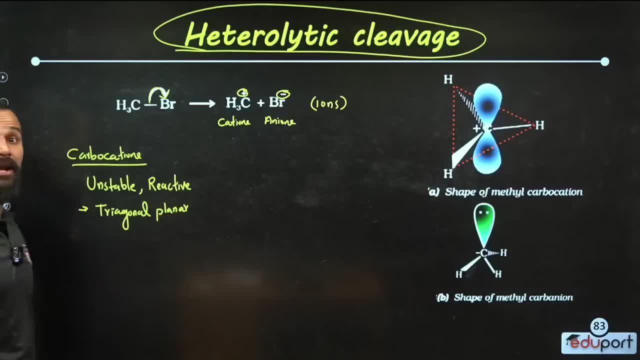 What is its shape? It is a trigonal planar shape. Its hybridisation is called sp2 hybridisation. Look at the kids. When heterolysis happens, the part with a positive charge is cation, the part with a negative charge is anion. 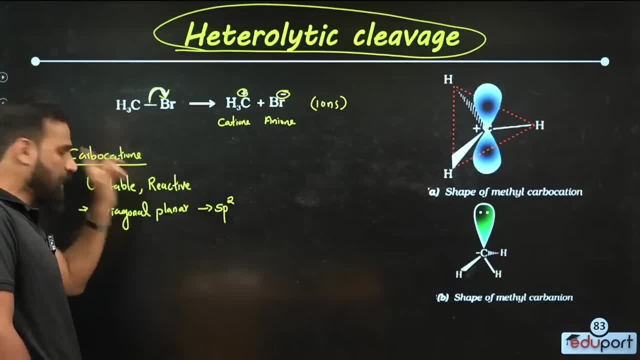 If the one with a positive charge is carbon, then he is a carbocation. That carbocation is unstable. He is highly reactive, That carbon triangular planar shaped SP two hybridization Lala. The most important thing is his order of stability. 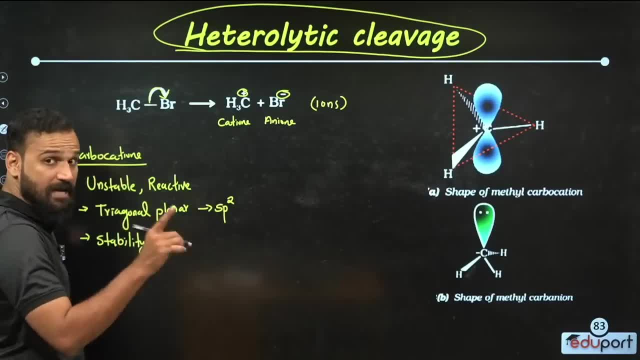 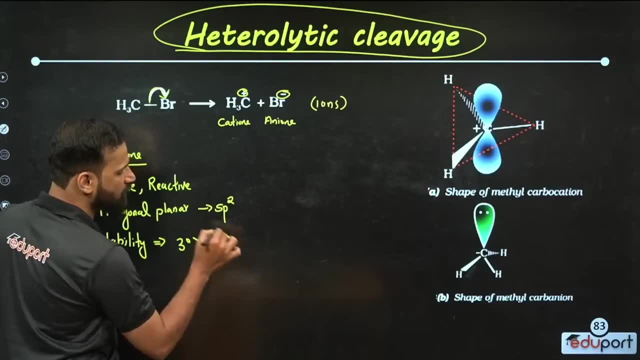 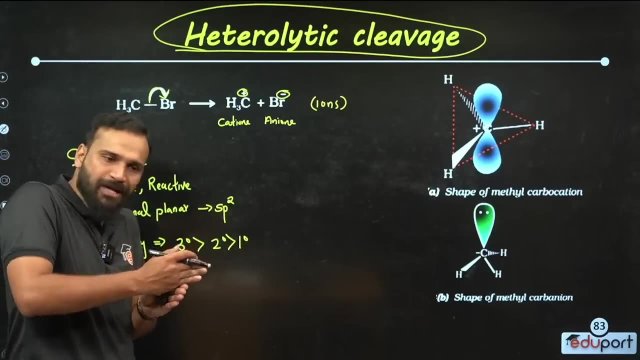 His order of stability. That stability, the stability of the carbocation, is the most stable, Then secondary carbocation, Then which carbocation? Primary carbocation, Methyl carbocation from primary carbocation and If there is a methyl carbocation, the value of the carbon. 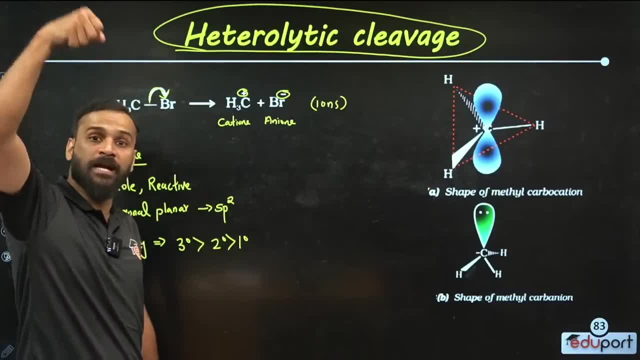 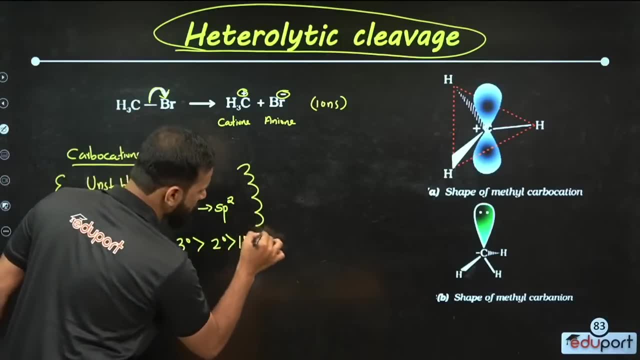 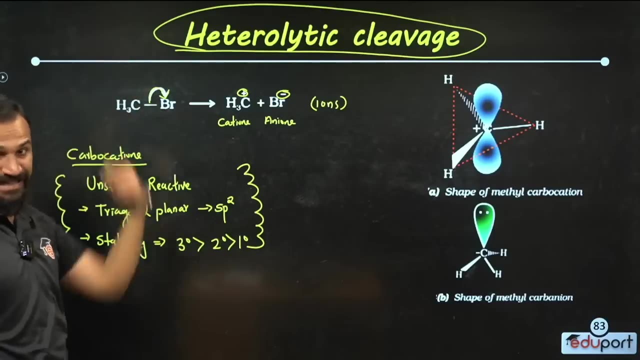 atom will be more stable. The value of the carbon atom will be less stable than the less methyl. Remember This, children- is related to carbocation. It is important to remember Now. look at the children. Now look at the name of the electron for this carbon atom. 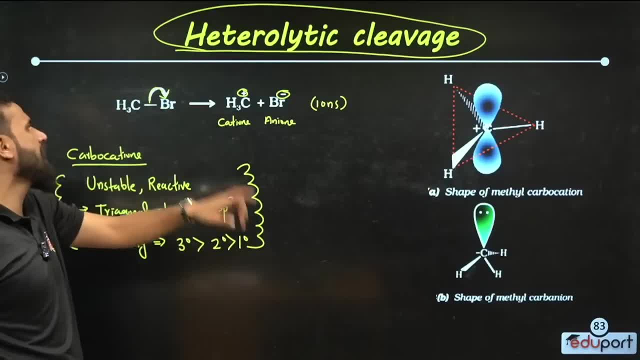 When do you get it? The electron is connected to the carbon atom and the carbon is less. If you have carbon, those two electrons and the carbon electron are taken. Then that carbon is negative and the other person will get positive Carbon. what do we get from carbon If you get negative? 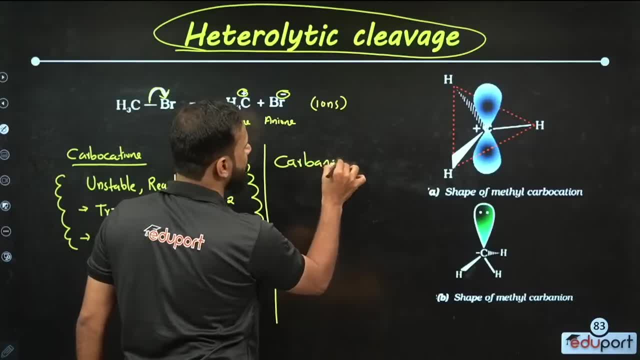 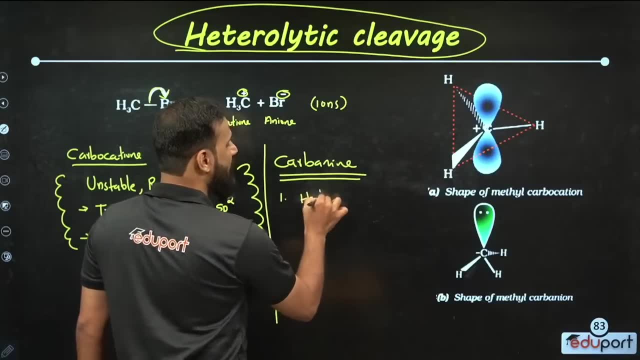 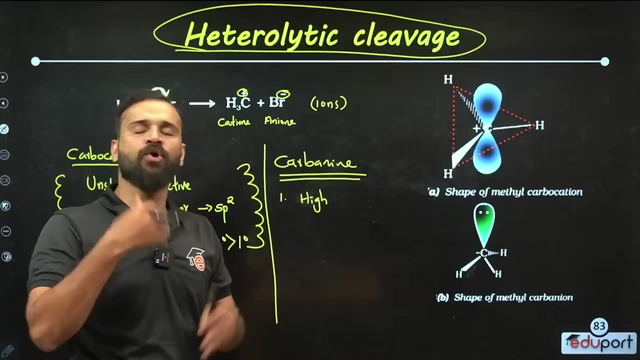 we call it carbanion. What do you call it Carbanion? Carbanion is also unstable, Highly reactive. It is unstable. It does not actually lose electrons- Electrons that are needed are getting, But still that charged anion is highly. 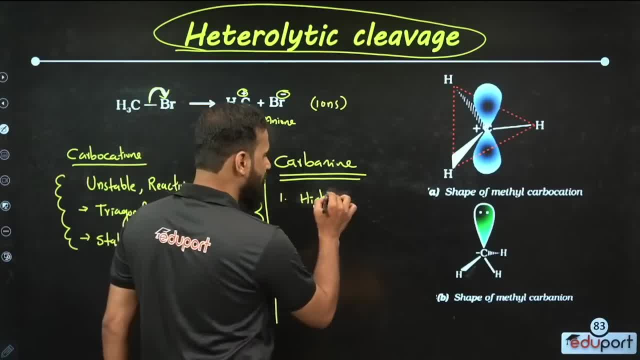 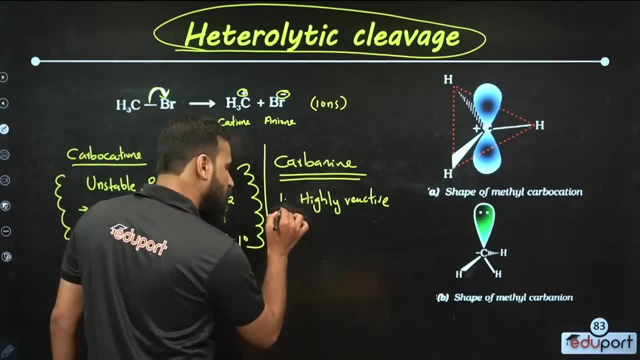 reactive itself. It is not highly stable. What is that highly? It is reactive itself. But we told here It is not the same. What he calls the shape is the tetrahedral. What children? the shape is a tetrahedral shape, The. 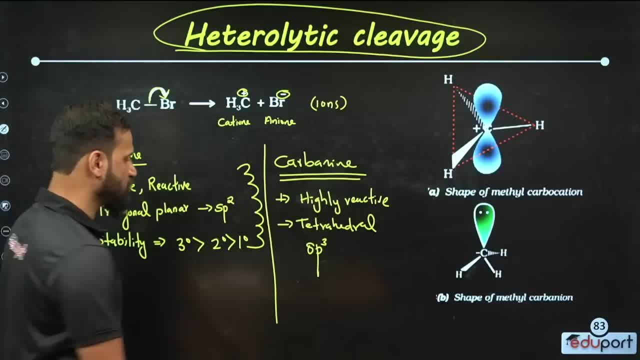 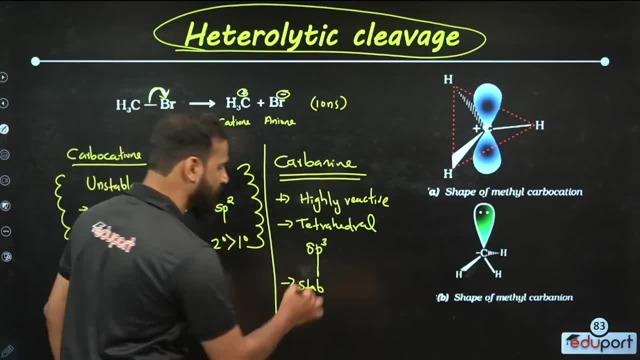 hybridization. is SP three hybridization Children that the stability order of it is studying Abah, carbocation and carbion are studied. Does it inquire for the exam? Stability question says that's the opposite of carbocation. the carbanion is very important. 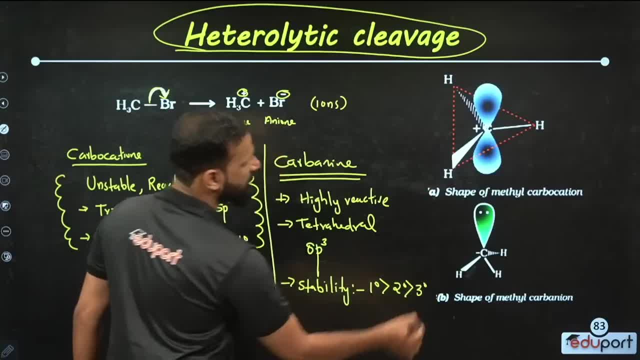 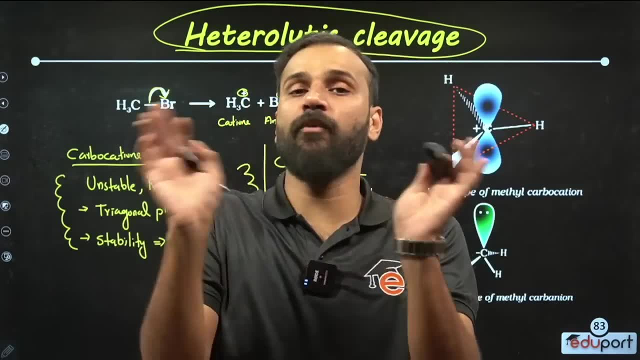 more stable, Then it is secondary. Then what is it? It is tertiary. So, guys, when a covalent bond is broken, it is not the same for both atoms. When two electrons are taken by one person, he will have a cation. 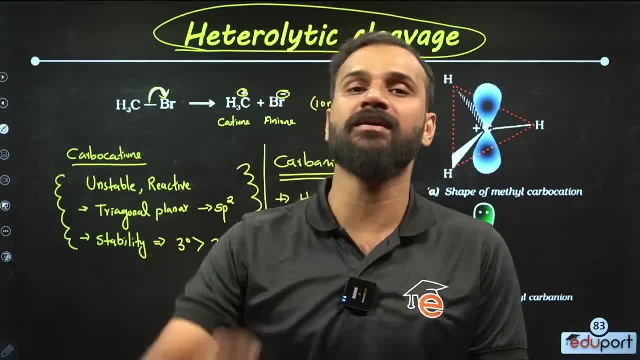 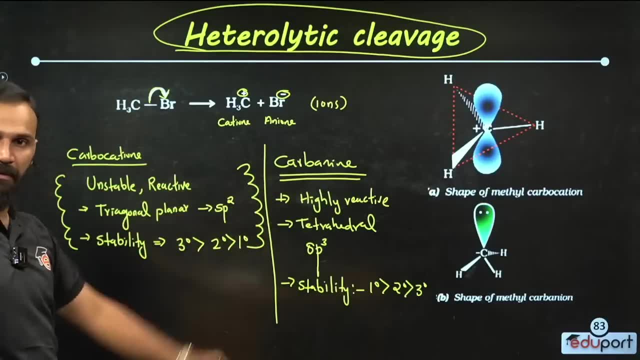 sorry, he will be anion, the other person will have a cation. This is how heterolysis is said to be broken. So when cation and anion are present, the properties of it are mentioned here: The properties of carbocation and carbation. 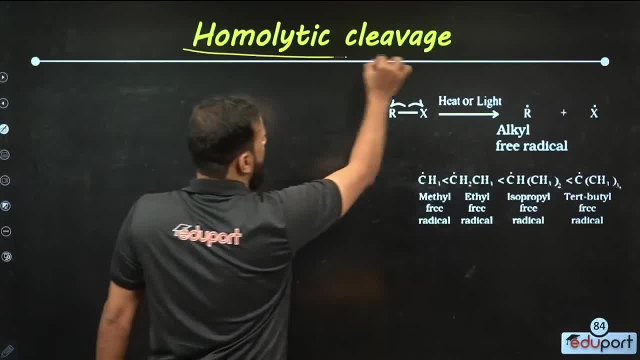 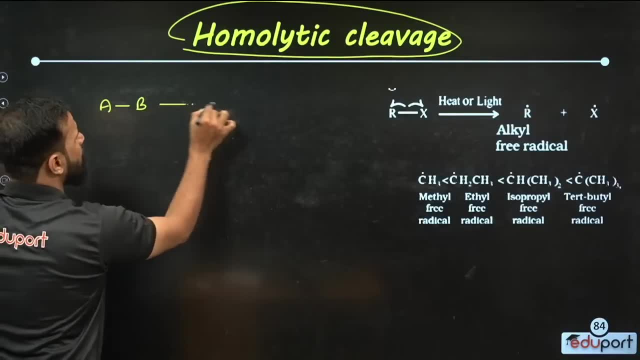 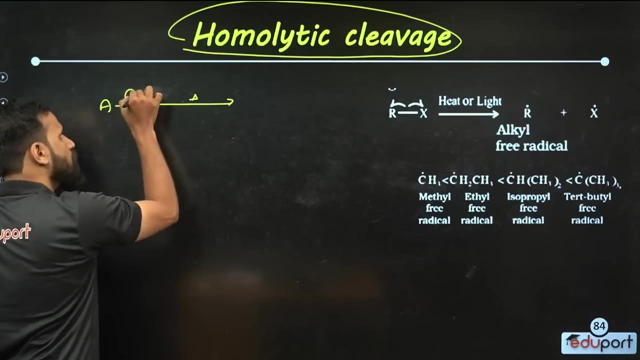 Learn that Now. look at the kids. Another possibility is homolysis. It is very simple. Look, let's say it simply. If we heat up the molecule called AB, we will think that homolysis is happening there. How do you know When this bond breaks? one electron is given to B. 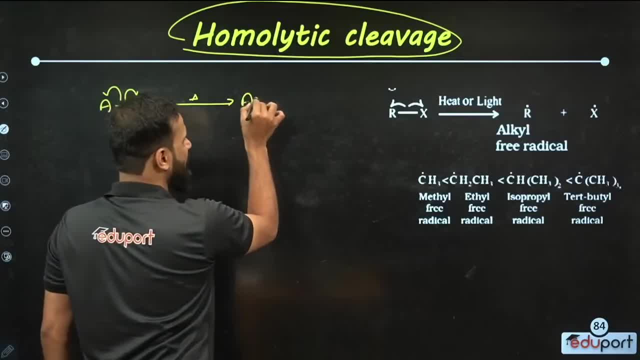 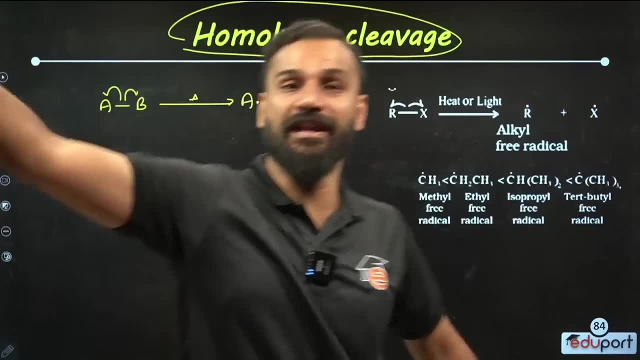 and one electron is given to A. So A has an electron in his hand, B has another electron in his hand. What kids? A has an electron in his hand, B has another electron in his hand. We call people with such an odelect or perchuss electron. 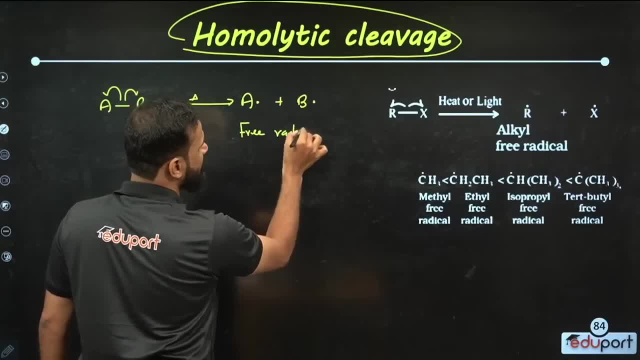 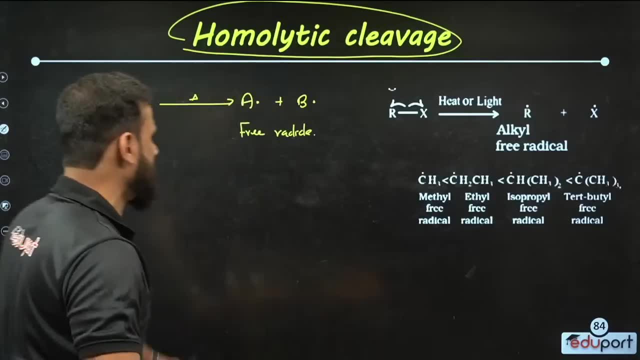 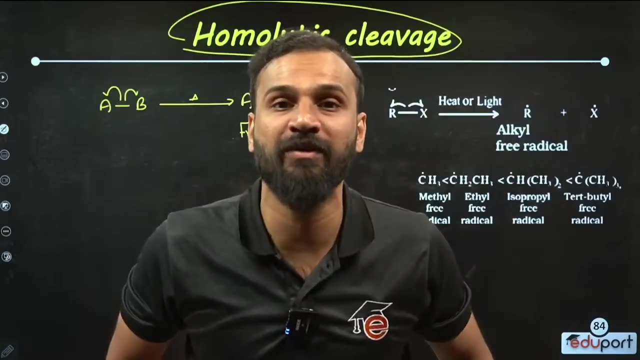 name free radical. What is it called? What is it called? What is an odelect or perchuss electron called free radical? What is it called free radical? So the product of homolysis is called the product of homolysis. the exam is asked for free radical Exams. 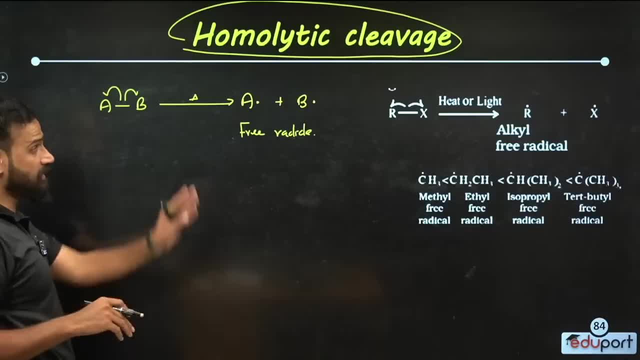 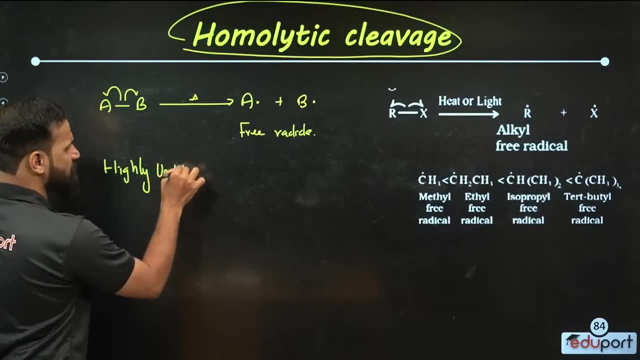 are asking Here, the kids are most often free radical from here. There is no doubt. What is it highly Highly? what is it Unstable? No doubt. What is it highly Reactive? No doubt The most important thing about it is its. 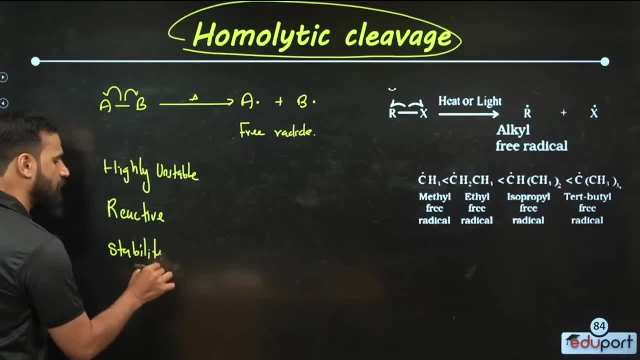 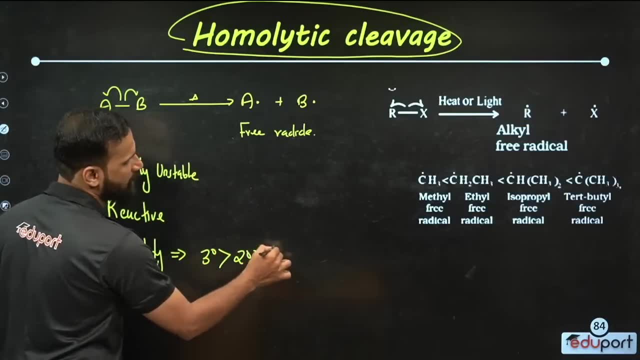 It is the order of stability. We are the order of stability. Who has the most stability? It is the same order for Carbocat: The most stability for tertiary, Then for secondary, Then who has the stability for primary? Here you can see: 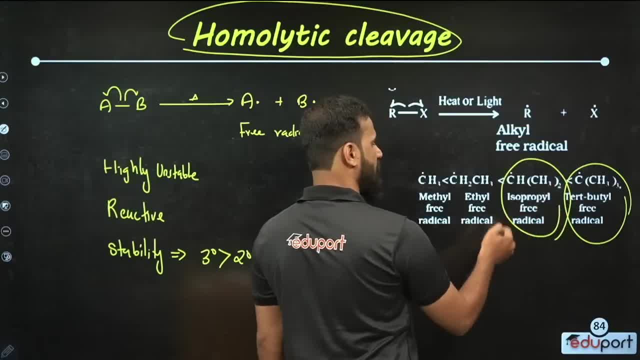 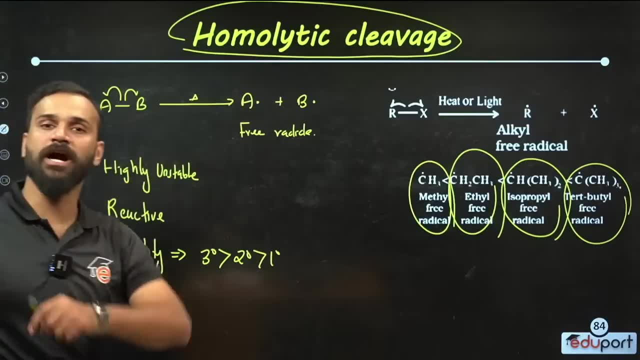 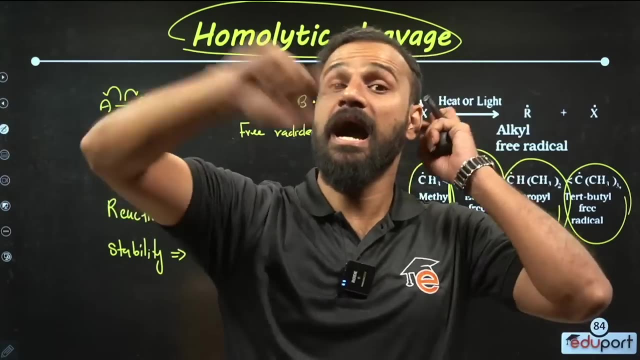 Tertiary is more stable for free radicals, Then for secondary, Then these two carbons are the primary, with another carbonyl, Very important Ask to arrange. So, children, you have to pay attention to what is it, What is the product of it. What is it, What is its product? 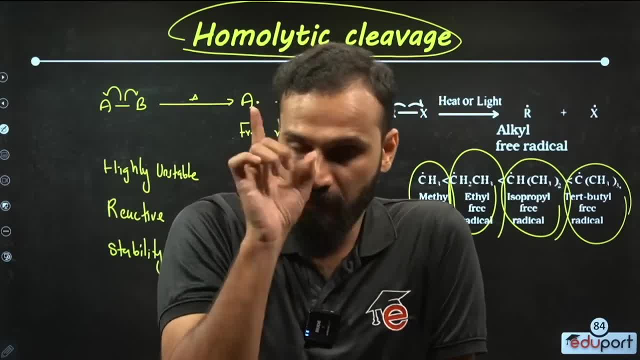 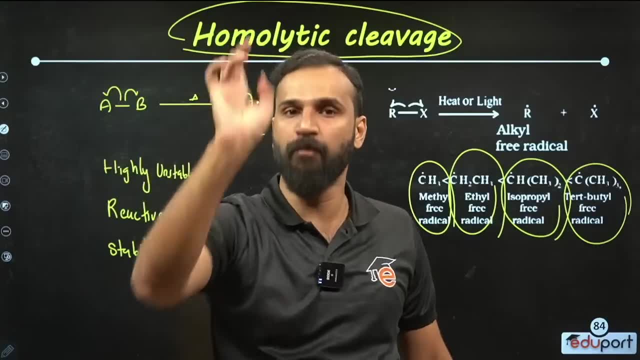 What is the stability order there? You can definitely learn, Because it is asked for the exam. It has been asked many times, So you should remember that you should not go to the exam without studying it, for one reason: Look, look, Two thousand and twenty-two. 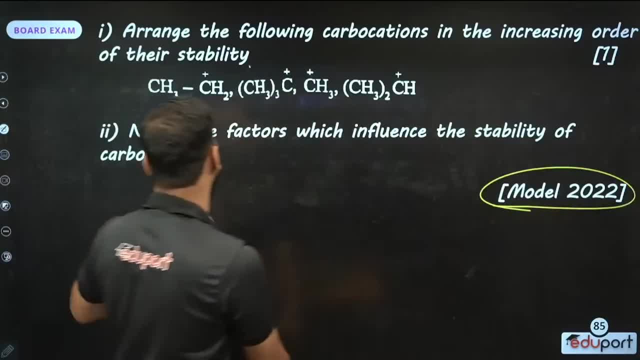 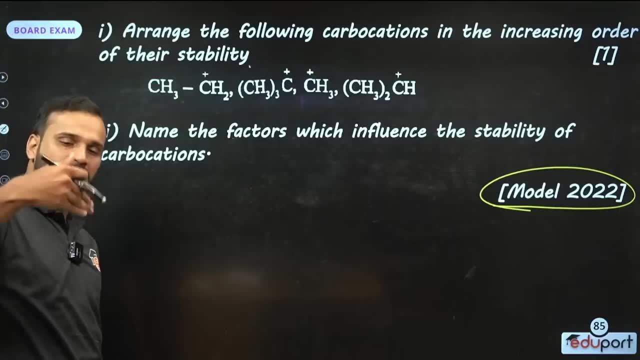 years. What did you ask for the model exam? What did you ask? Arrange the following carbocation in the increasing order of the stability. The order of carbocation is secondary to primary. There is stability for tertiary than that, So there is tertiary here. He is more stable. 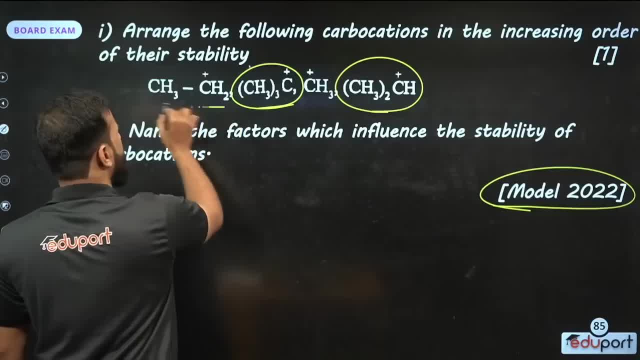 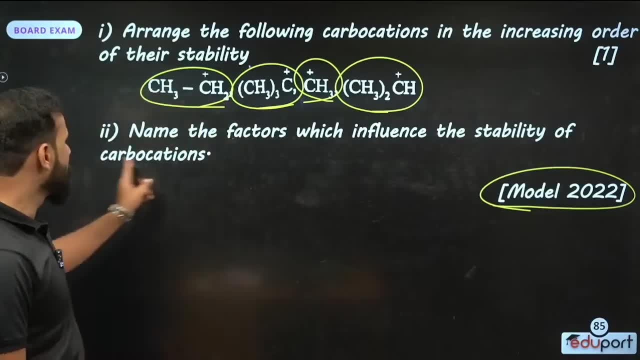 Then there is secondary. He is stable. Then what? Two carbonyl carbocation, Then one carbonyl carbocation. That's how the order comes. Name the factors which influence the stability of carbocation. The stability of carbocation. 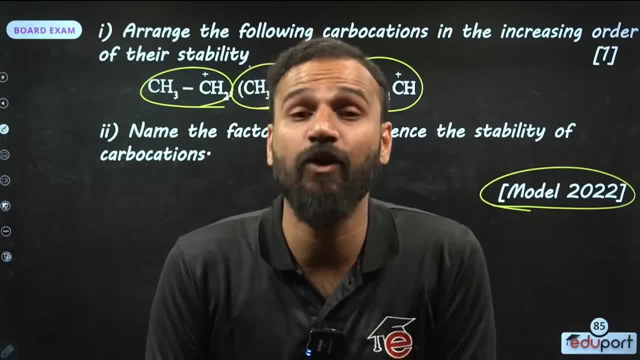 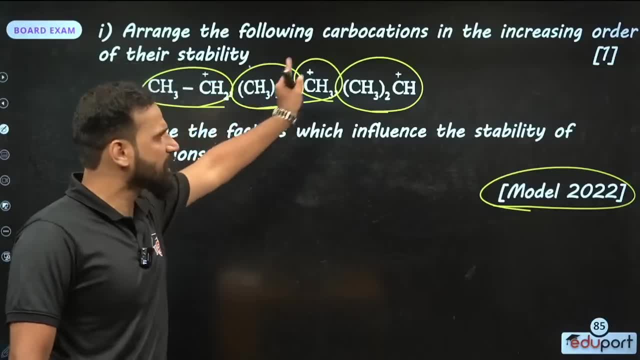 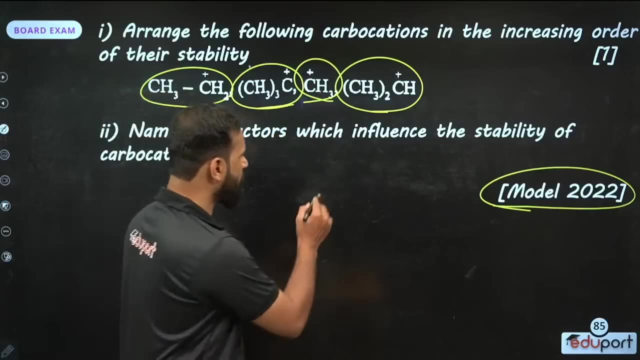 You've already said this. Then what do I say? which order is coming up? most is tertiary, then secondary is coming s aprox, then primary is appearing, primary, secondary and tertiary. To make you understand the difference, you can tell me It is the specialty of tertiary, which is believed to be the specialty. 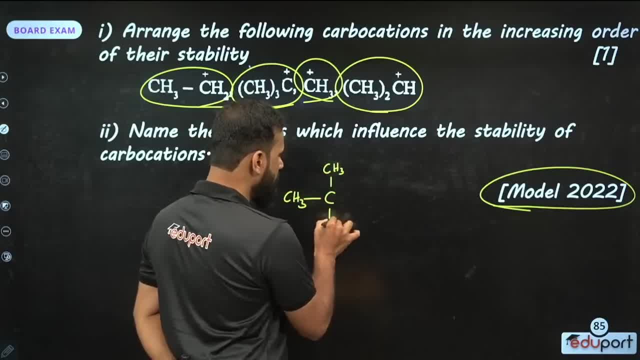 of tersary. There are three big groups around it. There are three big groups. This is not tertiary, So the Steric effect is very strong here. Sorghum in towards the very next is there. Keep your eyes on the khác and Apple 5.. Give such a feeling that desiring it may work more easily knowingly. 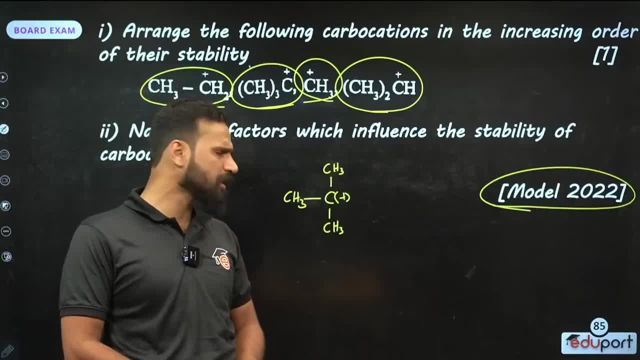 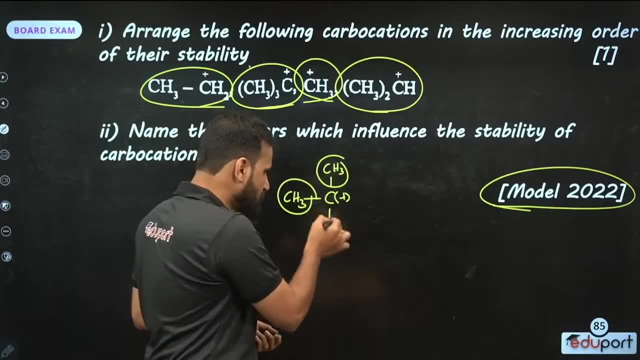 So there is no doubt that the steric effect is very high here. What is the steric effect? It is high. So here the size is high, the size is high. the size is high when the alkyl salt comes. 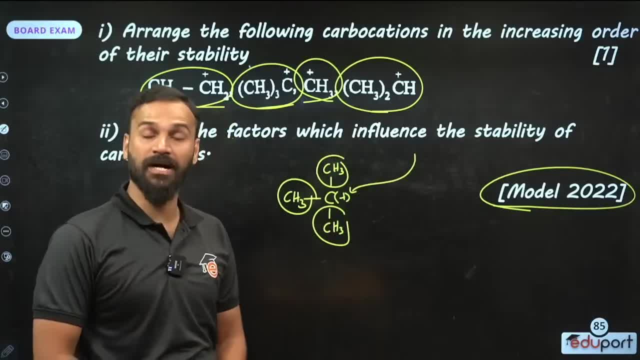 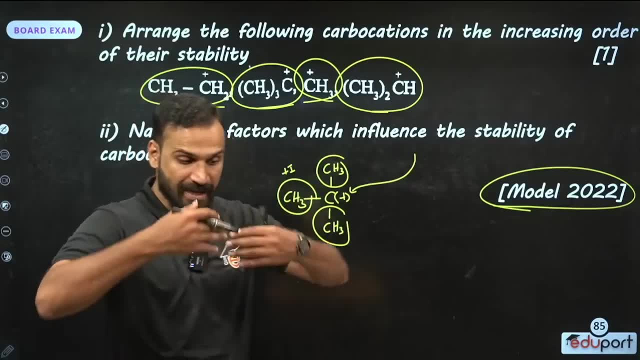 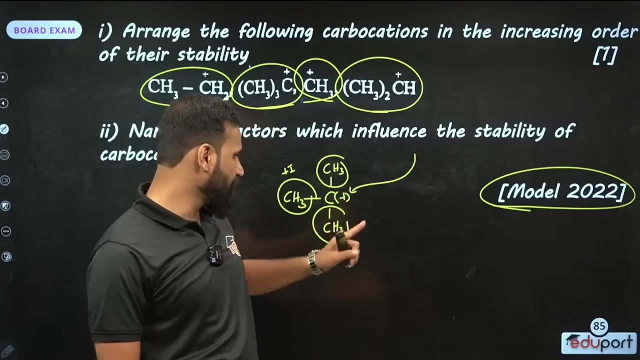 it is very difficult to attack another attacking reagent. This is very important. Another important thing is that this alkyl salt is a group that leaves the electron. that shows the effect as a plus. So if the electron flows there, the positive charge will decrease and the reactivity will decrease. 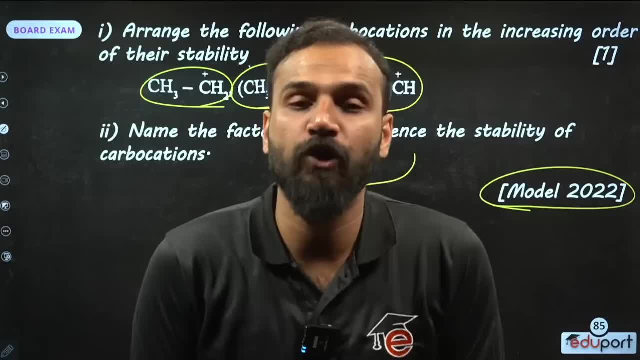 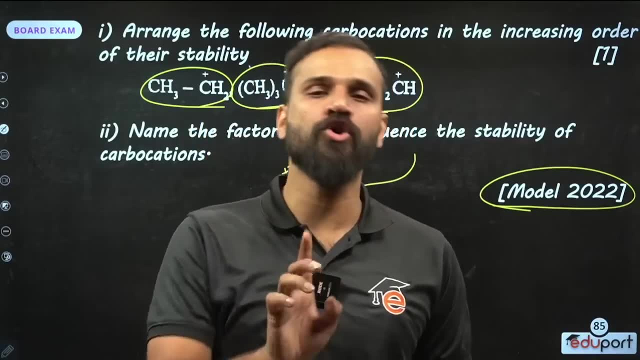 Now, in another sense, we can explain the stability of carbocation by using inductive effect and hyperconjugation effect. We are going to learn both: What is inductive effect and what is hyperconjugation effect? We are going to learn both. 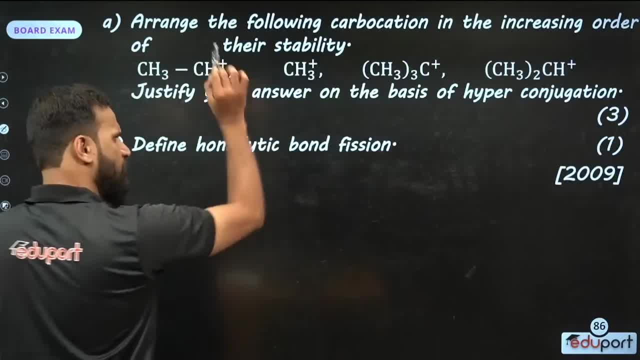 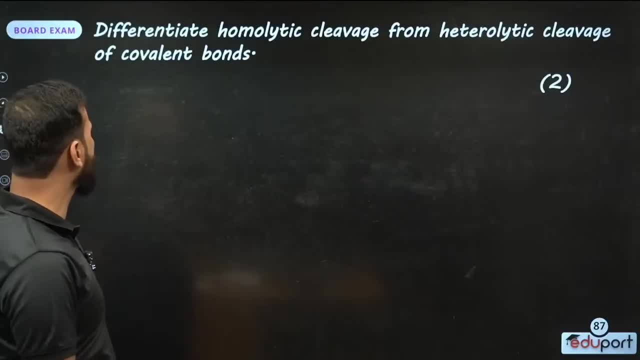 Both are important. You have to pay attention to that. Now, look, we are asking to arrange carbocation again. What is homolytic bone diffusion? I have already explained that Difference: differentiated homolytic cleavage from heterolytic cleavage. 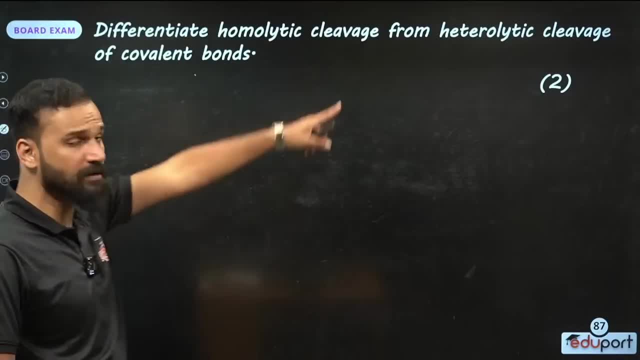 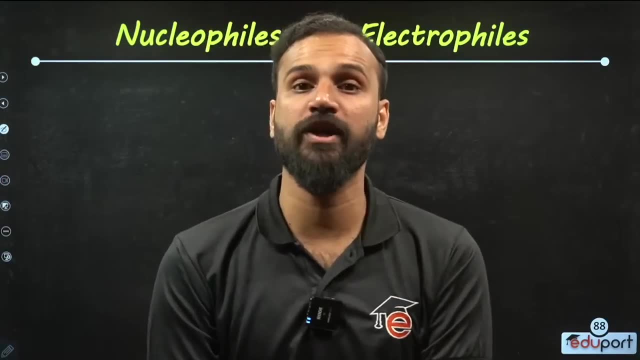 we are asking in the exam. Please pay attention to that. Please pay attention to that. It is a question of two words. You just have to give the correct answer Now: nucleophile and electrophile. Another question asked in the exam is: 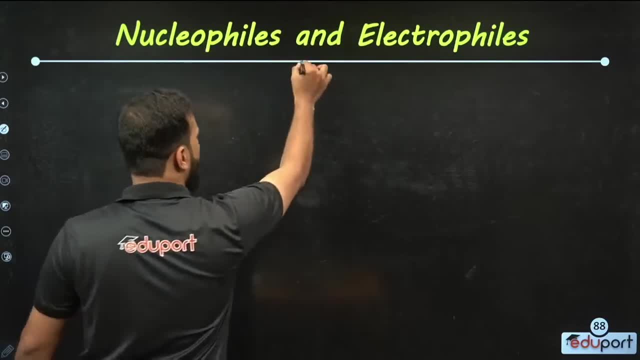 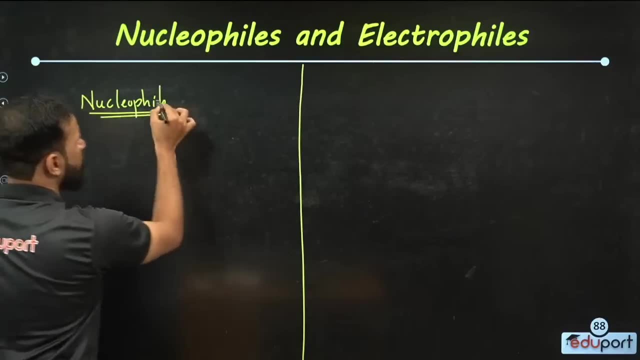 what is nucleophile and what is electrophile? We can say both. We can say both. Look, the first one is nucleophile. Who is the first one, guys, Nucleophile? Who is the second one? The second one is electrophile. 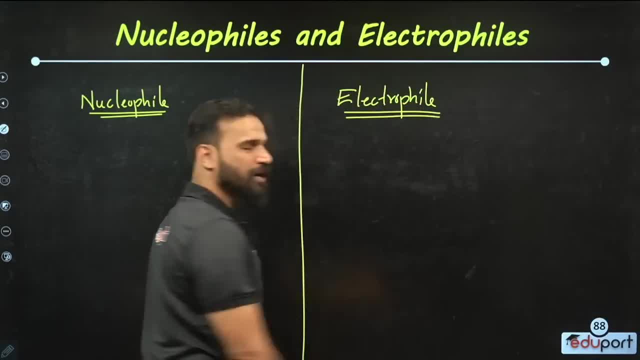 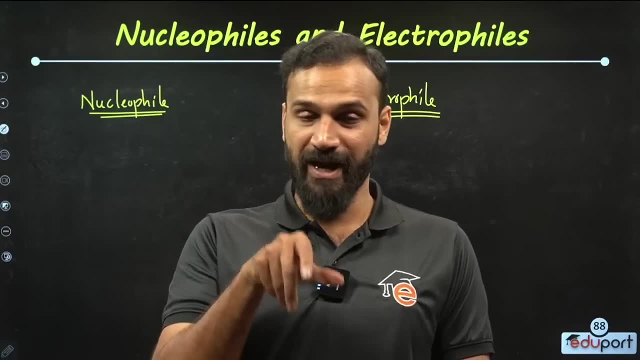 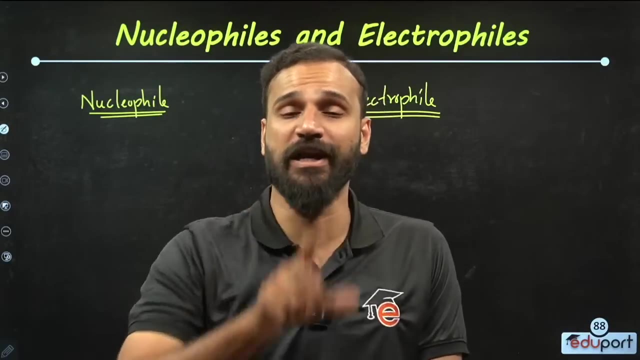 The second one is electrophile. If we say nucleophile, it is the species that attracts nucleus. The charge of nucleus is positive. It is the species that attracts nucleus, It is the nucleus loving species. that is called nucleophiles. So 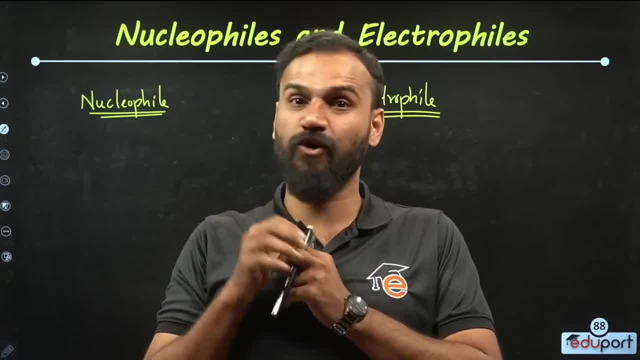 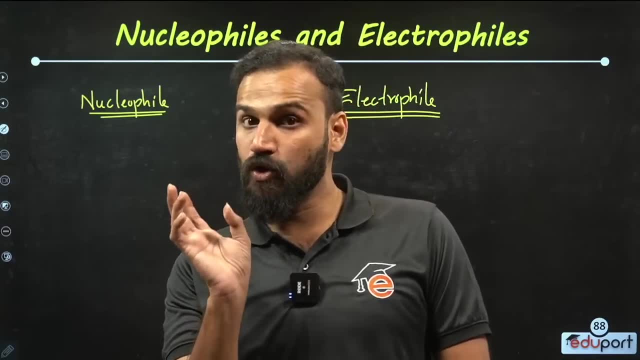 if we say that we love nucleus, we need electrons in his hand. We need negative charge, Otherwise we will die. So the specialty of nucleophiles is that they are electron bringing species. Nucleophile is the species that attracts electrons. 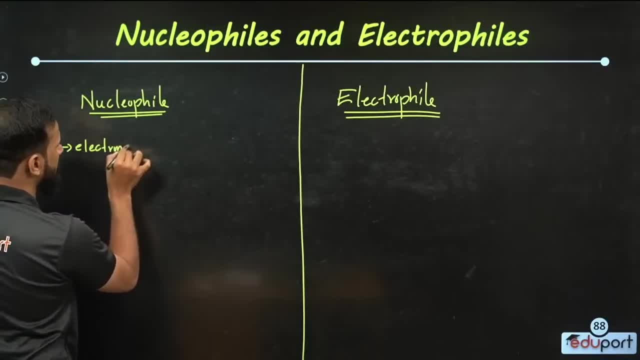 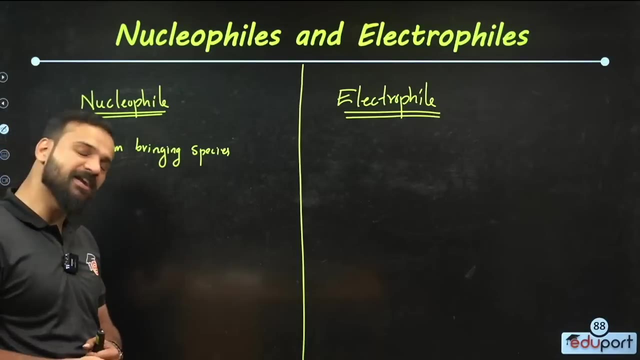 What is electron guys? They are electron bringing species. Electron bringing species. Electron bringing species is called nucleophile. Okay, right, Who is the one that attracts electrons? It is for two people, Electro. sorry, they can act as nucleophiles. 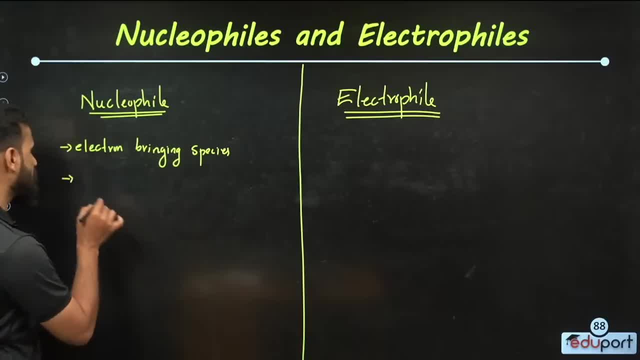 Do you know who they are? One ions with negative charge. They can act as nucleophiles. for OH- They can act as nucleophiles for Cl- Everyone with negative charge like this can act as nucleophiles because they can attract nucleus. 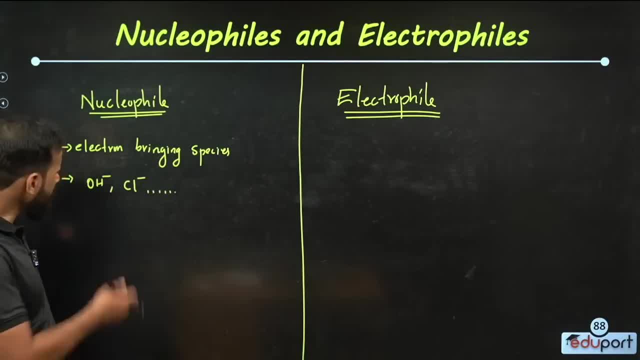 Who is the other one? Who is the other one? Who is the other one? guys, Can you tell Who can act as nucleophiles? It is for people with long pair. You know that in H2O there are two long pairs in oxygen. 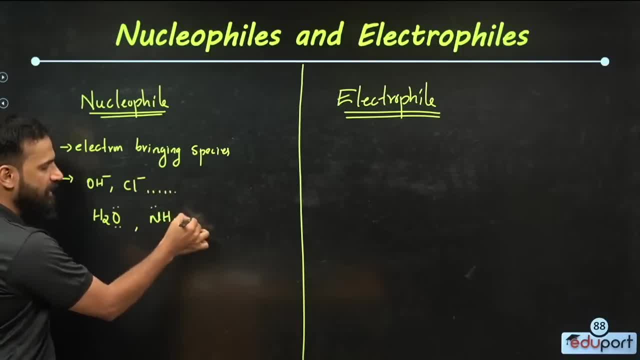 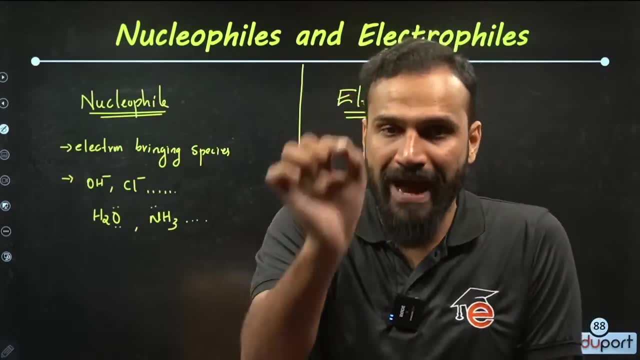 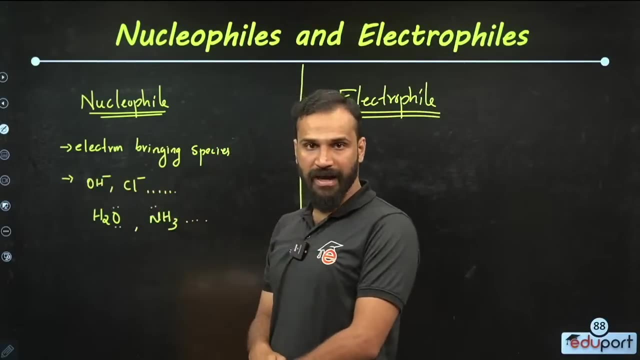 Ammonia. they have long pair. if they are neutral, Such people with long pair can act as nucleophiles. The smallest one is the species that attracts nucleus. It can be said that they are nucleophiles. It can be said that all those with negative charge can act as nucleophiles. 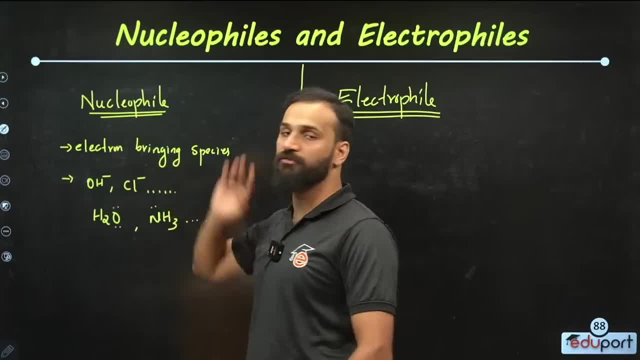 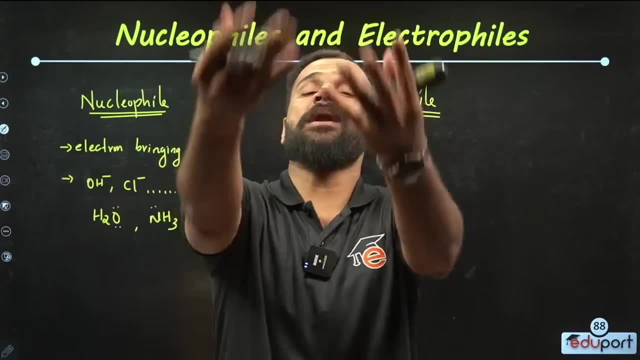 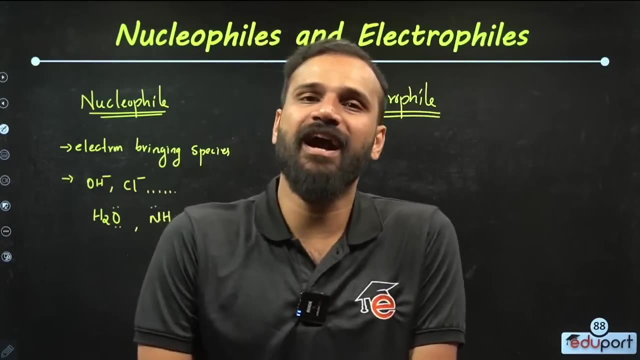 Neutral molecules with long pair electron can act as nucleophiles. Now look Who are electrophiles, Species that attracts electrons. Electrophiles are electron-loving species. So if electron-loving, if you feel the attraction of electrons, this person should be electron-deficient. 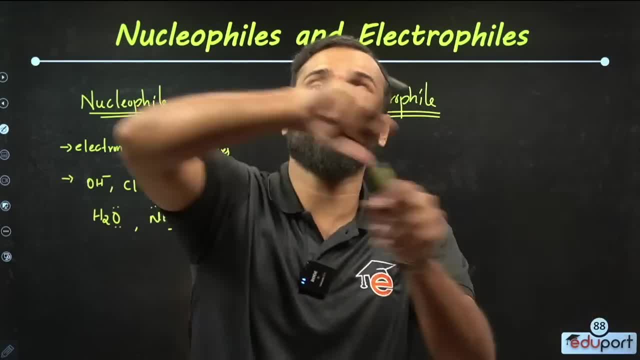 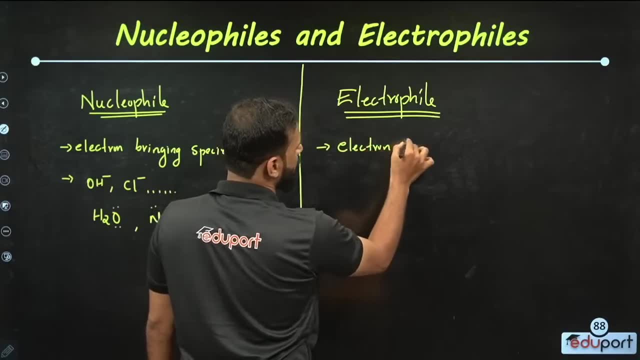 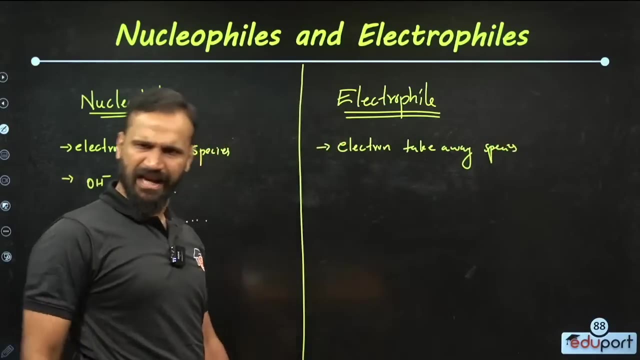 That means this person is not bringing electrons. He is taking the electrons inside. No, Not electron-bringing species. What is it? Electron, Electron, Take away. Take away Electron, take away species, Electrophiles, Or simply, if there is confusion. 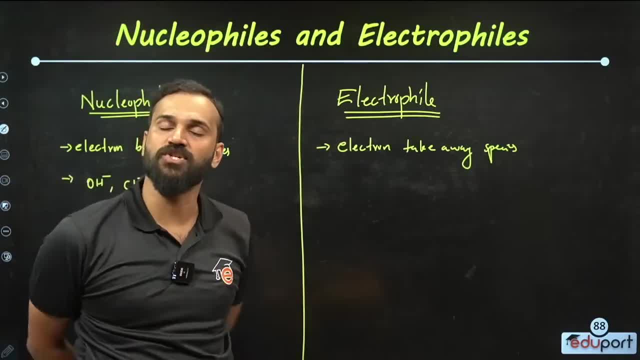 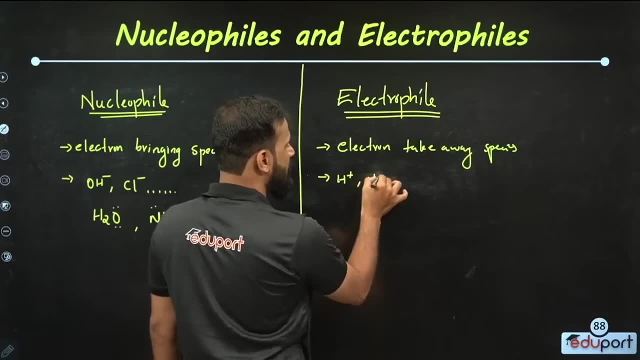 don't say anything. It is enough to say that it is a species that attracts electrons. Who can act as an electrophile? To act as an electrophile? all those with positive charge, all those with positive charge ions. how can they act? 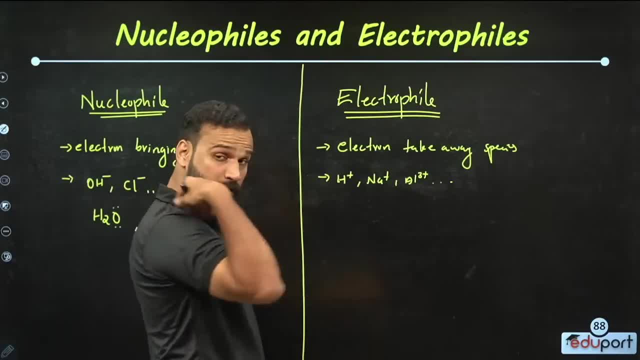 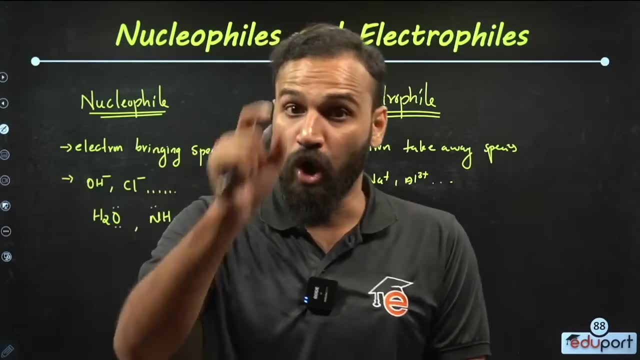 They can act as electrophiles. Now look, Can neutral people act? They can. How can neutral people act? They should be electron-deficient. In chemical bonding we learn the limitation of the octet rule. The first limitation of it is the incomplete octet right. 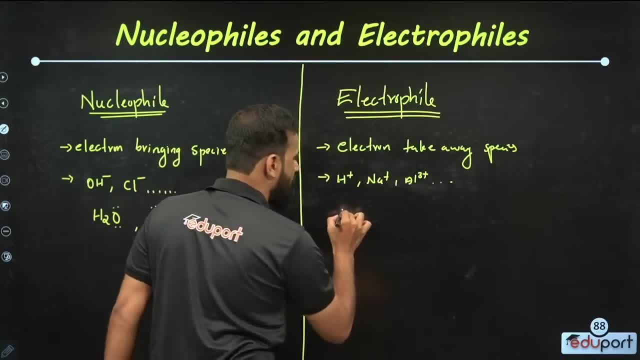 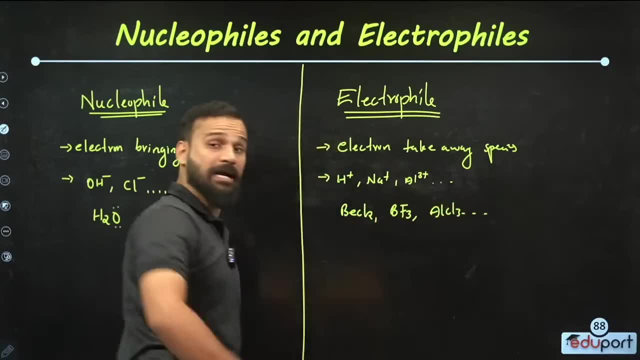 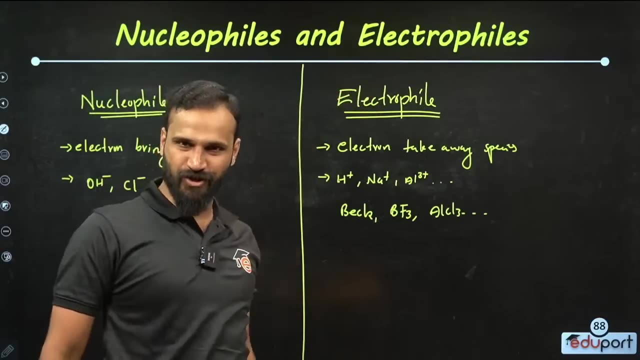 Species that do not have electrons, for example BeCl2,, for example BF3,, for example AlCl3,, for such electron-deficient neutral molecules that do not have electrons will attract electrons. So how can they act? 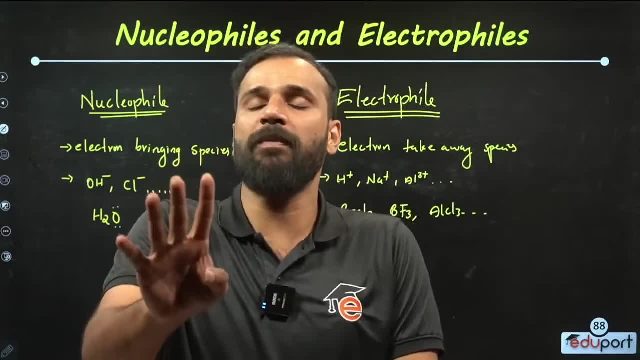 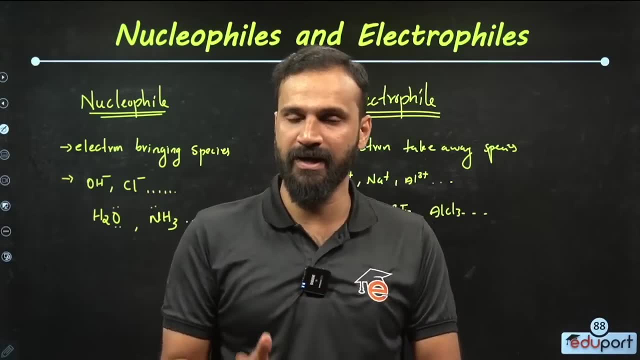 They can act as an electrophile. So, guys, the last four points I said are very important. Homolysis exam is asked. Heterolysis exam is asked. Their carbocation, carbionion, free radical stability order is to be studied. 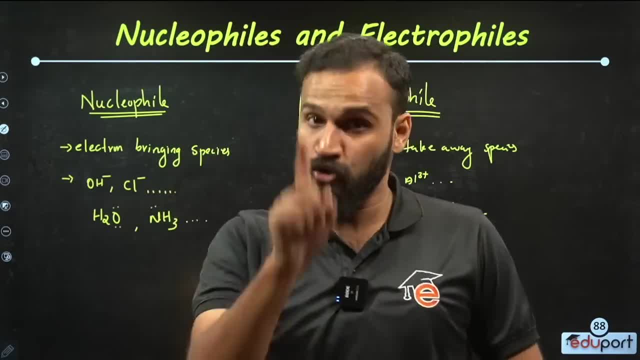 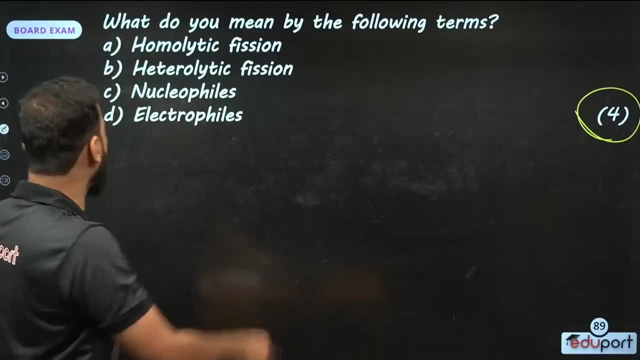 What is nucleophile and electrophile? What is the example It is asked? Write it down, guys. Ask about the four marks, Not just four. Ask about the four marks. What is homolytic fission, heterolytic fission? 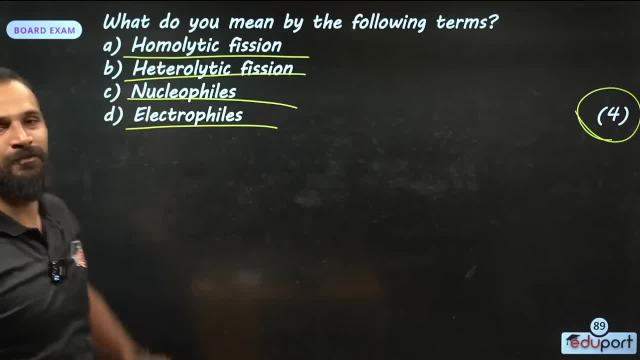 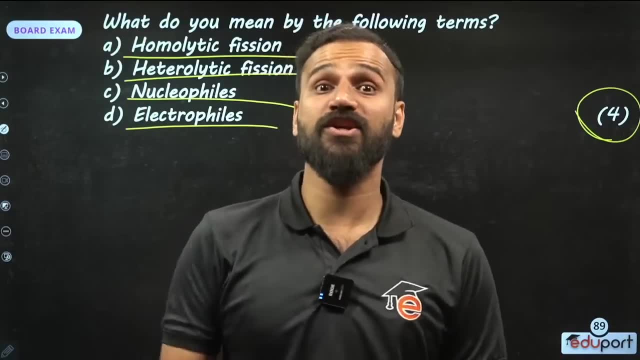 nucleophile, electrophile. What are these four? Next, please, What is this? You will have to answer the questions one by one, So write it down simply. But you can write if you know it. That is why it is said to be studied. 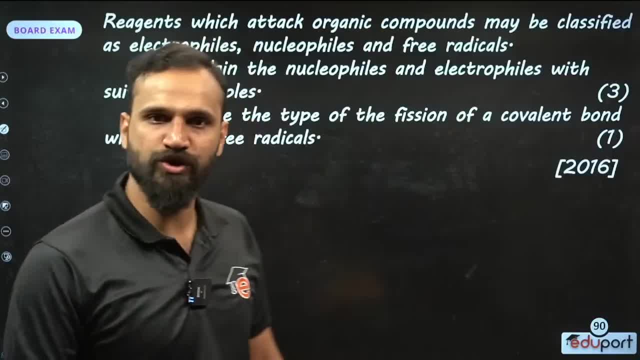 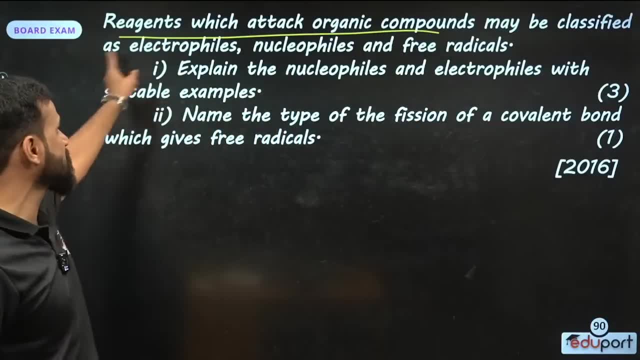 Don't go without learning. This is the question asked by the exam many times. Now, guys, the question in 2016,. Reagents which attack organic compounds may be classified as electrophiles, nucleophiles and free radicals. Explain the nucleophile. 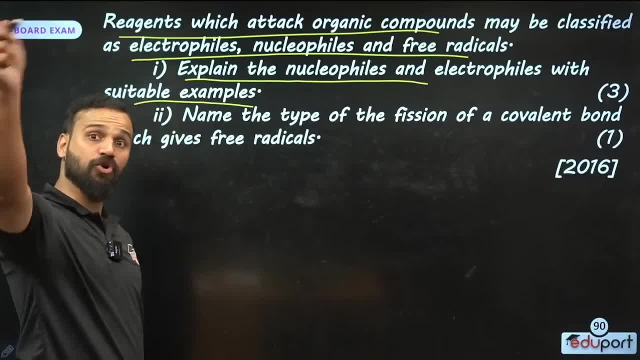 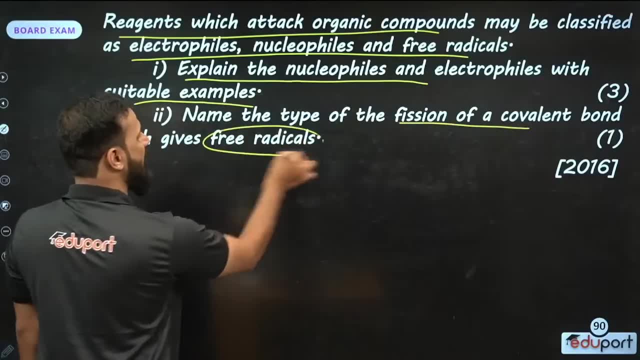 and electrophile with a suitable example. Electrophile and nucleophile should be explained. example to explain: Name the type of fission of a covalent bond which gives free radical, Which fission gives free radical, That is, homolysis or homolytic fission. 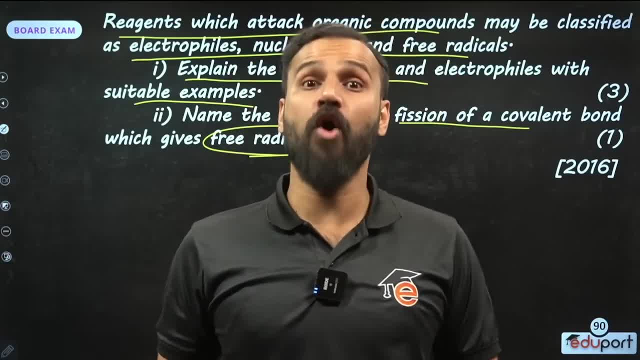 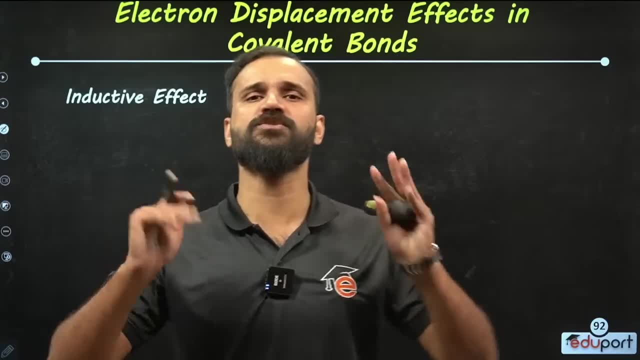 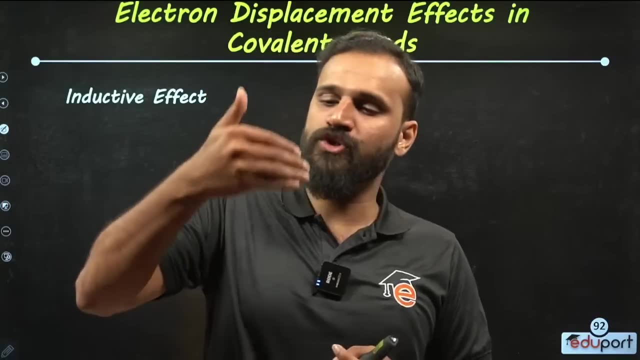 When homolytic fission takes place, free radical becomes the product there. Remember this. Now look at the electron movement. There is nothing there. Electron displacement effect. When a reaction takes place in an organic molecule, what happens? The displacement of electrons is taking place. 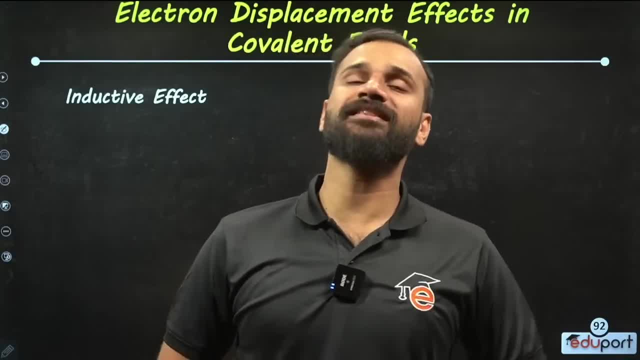 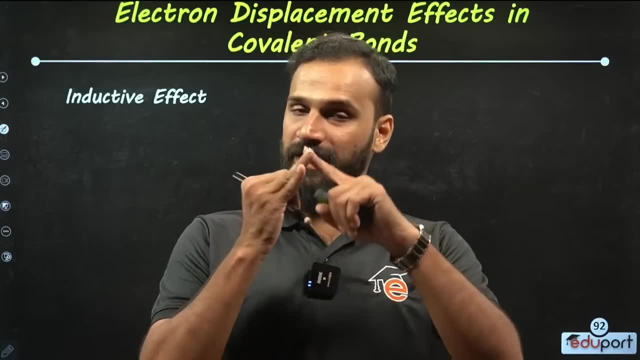 The movement of electrons is taking place. It takes place in four forms. That is called the electron displacement effect. One is the inductive effect. Two is the resonance effect. Three is the electromeric effect. Four is the hyperconjugation effect. 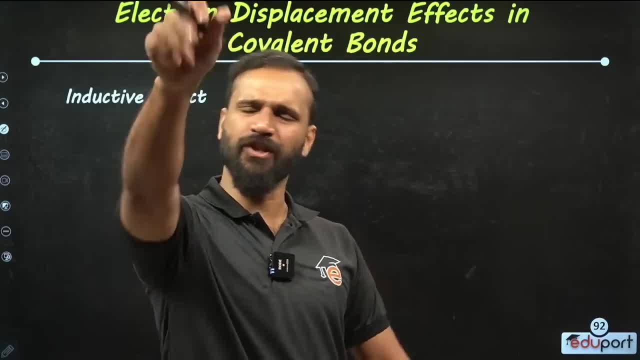 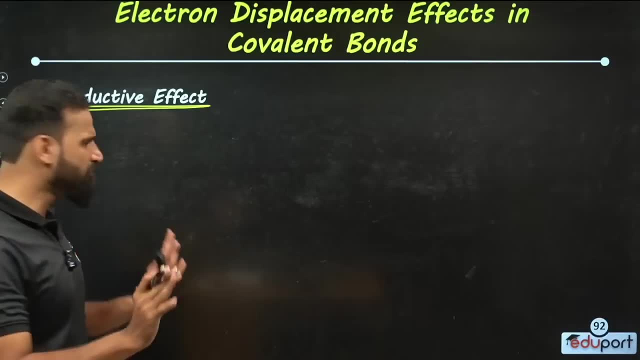 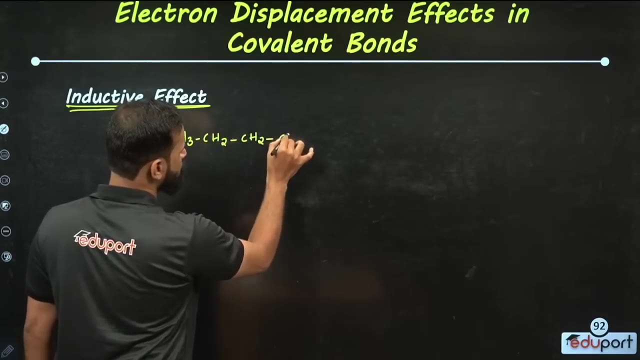 It's very simple, But you have to learn it by heart. you have to learn it by writing. Look at what the inductive effect is. What is inductive? I will explain it in a simple way. I will take a compound. Look: CH3CH2CH2CH2Cl. 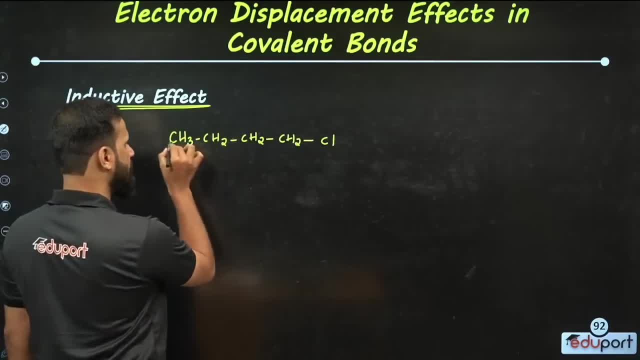 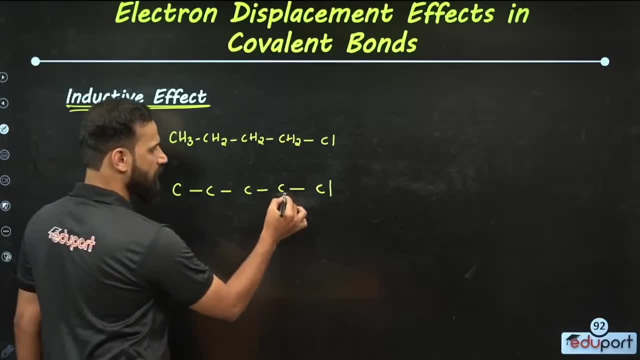 Okay, guys, To understand, I will take only carbon: One, two, three, four. Then there is chlorine. Okay, I am giving the number One, two, three, four. I am giving it to understand. Let me ask. 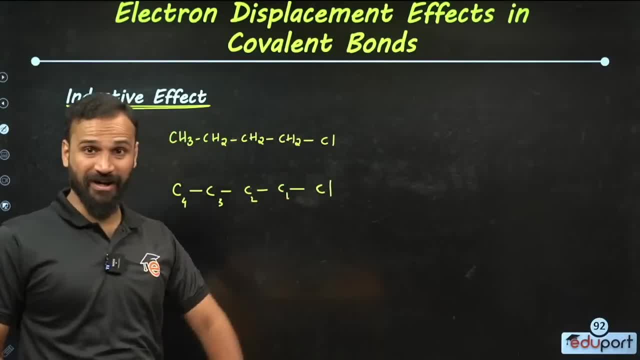 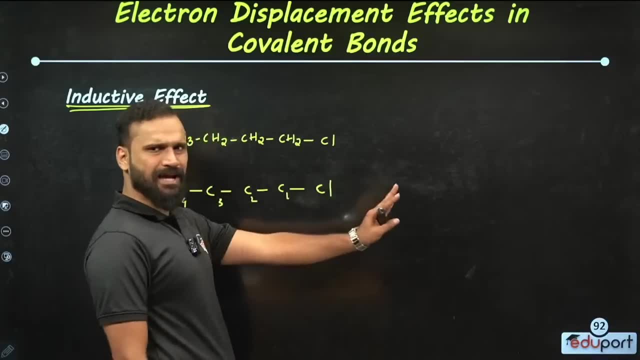 Between the carbon, called C1, and the chlorine. there is no electron. There is no electron. There is no electron, There is only a electron. Where does that one electron move? Is it near chlorine or C1?? There is no doubt. 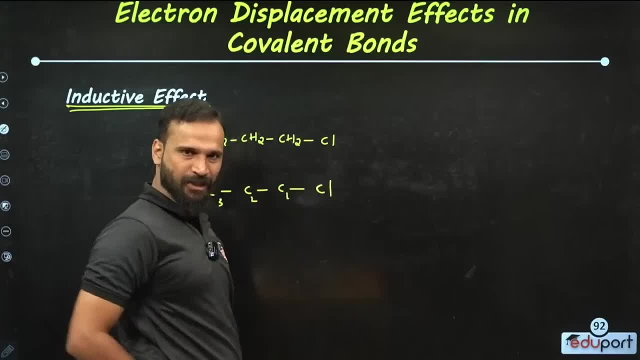 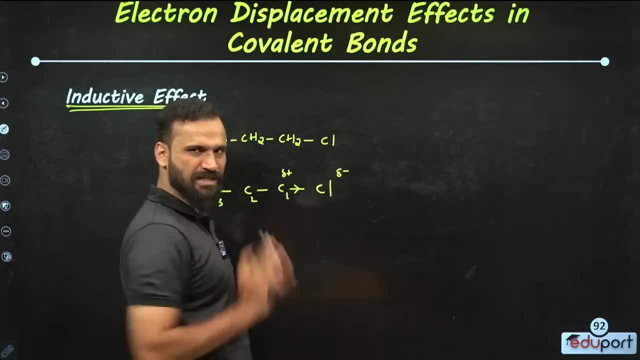 Is chlorine electronegative than carbon, Then it will stay there. So there is a partial negative here, There is a partial positive here, right? So through this sigma the electron is a little closer to chlorine. Let me see, If C1 and C2 are taken, who is more electronegative? 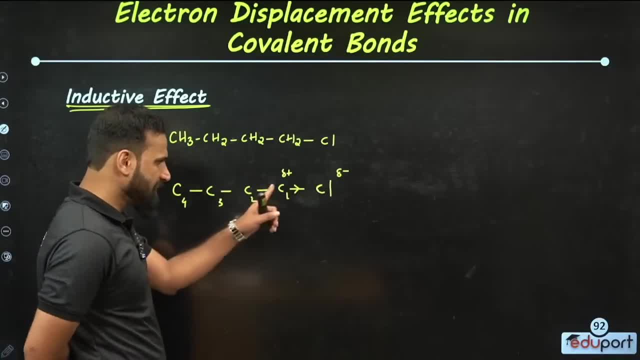 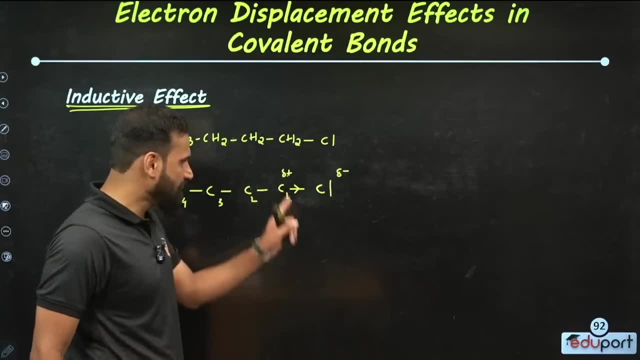 The electronegativity of both is the same, But there is a positive charge near C1, right? Yes, Yes, There is a positive charge near C1, right? I mean, there is a small positive charge, right? So the electron pair that has to stand in the middle here will stand close to C1. 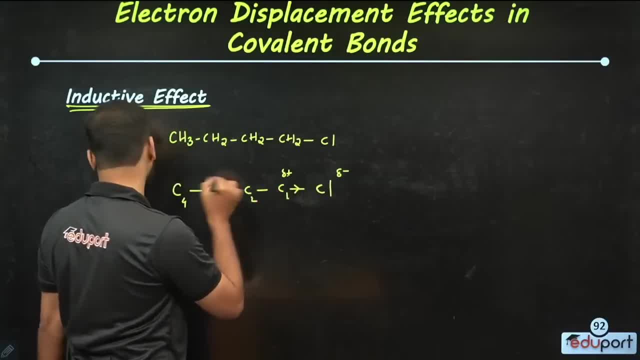 It will stand close to C1. So the electron pair moves from here to there. The electron pair moves from here to there through the sigma bond. So there is a loss here. Usually it is given by delta plus Here. delta plus is only given here. so delta will be given by delta plus. 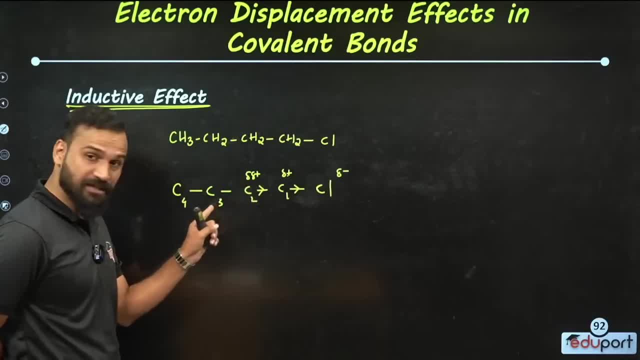 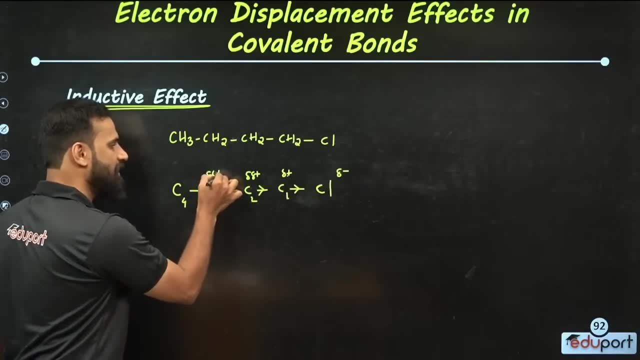 Now look, the same question is asked Between C2 and C3, where will this electron pair go? It goes to C2.. Why it cross? Because C2 and C3 have a positive charge there. Hence it is given by delta plus. 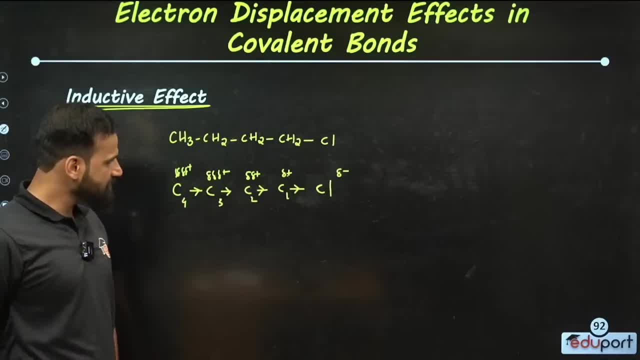 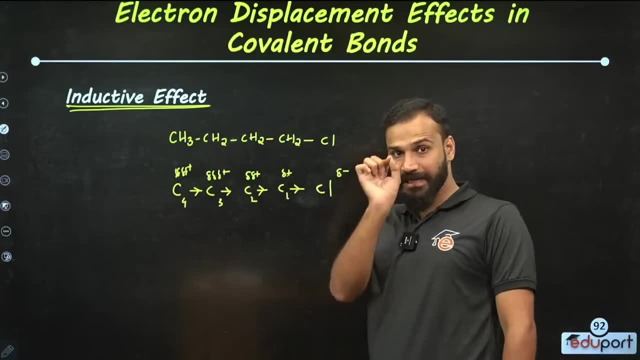 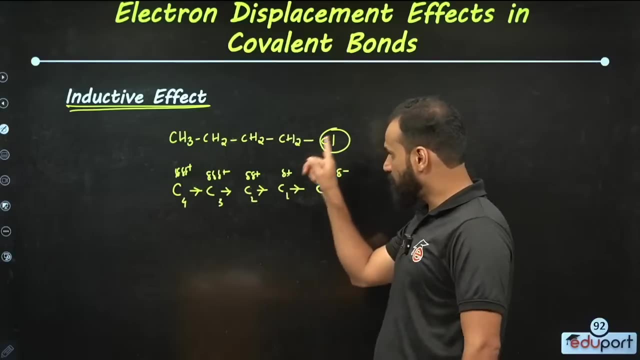 That's it right, It is the same here. But let me ask you what happened here. When a group with an electronegativity difference came to this organic compound, then what happened? The electrons flow through the sigma bond. The electrons don't get so much at a distance. 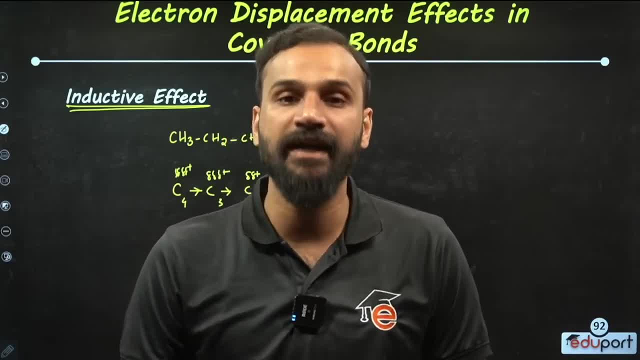 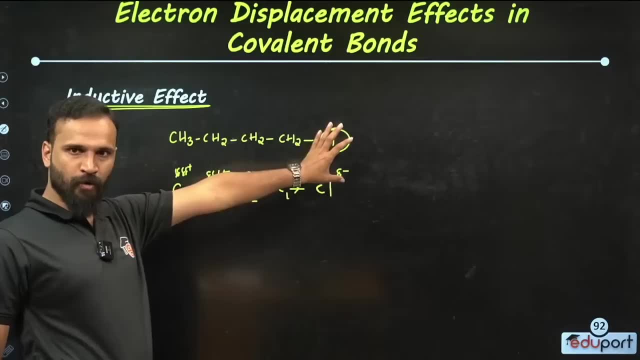 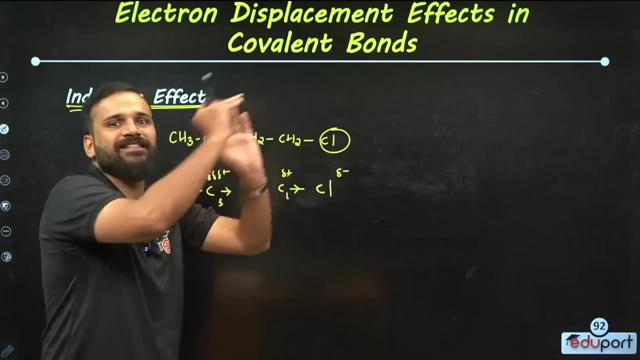 This phenomenon is called inductive effect. See how simple it is. There is nothing for those who think it is a big thing. When an atom with electronegativity difference comes inside an organic compound, it goes near that atom. sorry, I can't say that. 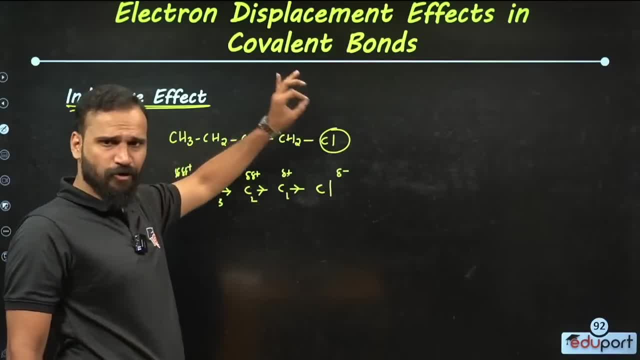 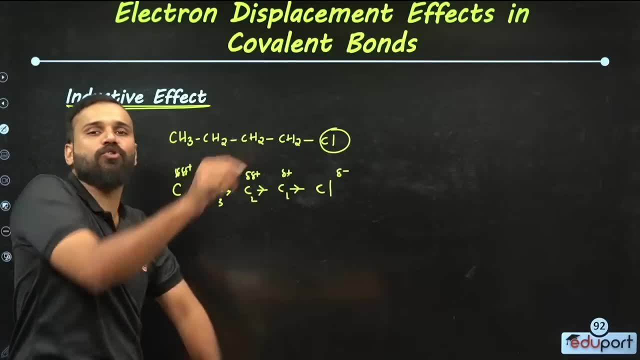 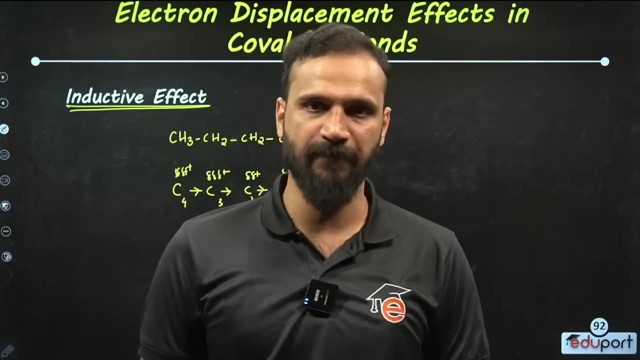 When an atom with electronegativity difference comes inside an organic compound, electrons move through the sigma bond inside that molecule. This is called inductive effect or I-effect. There are two types of inductive effect. One is positive inductive effect. 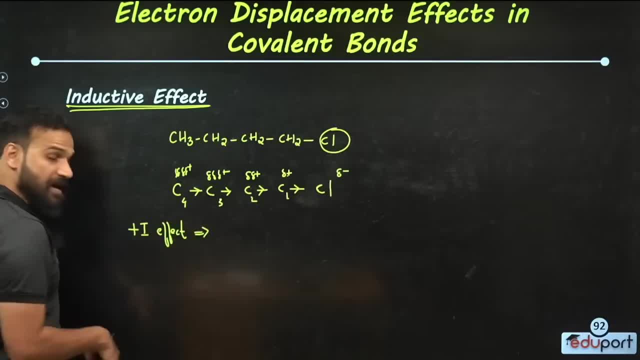 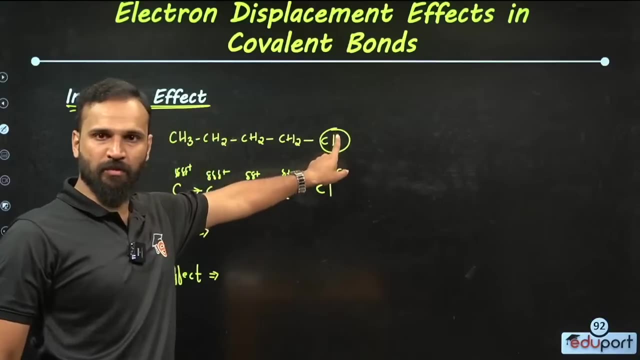 It is called plus I-effect. The second is negative inductive effect, It is called minus I-effect. What is inductive effect? There are two types. One is positive and the other is negative. Let me ask you something. When an atom with electronegativity difference, 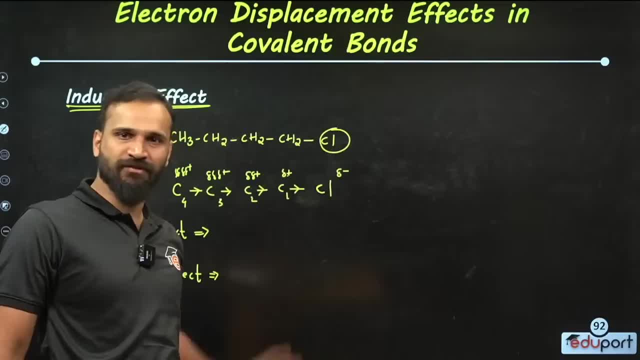 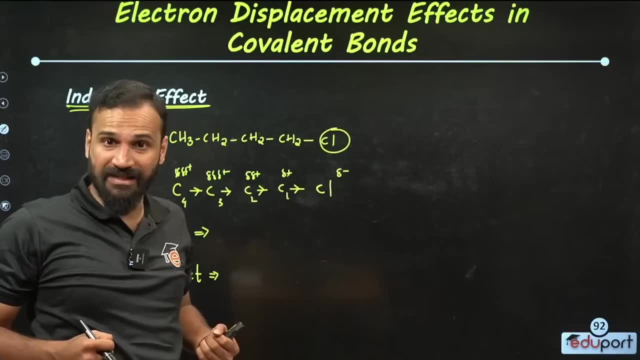 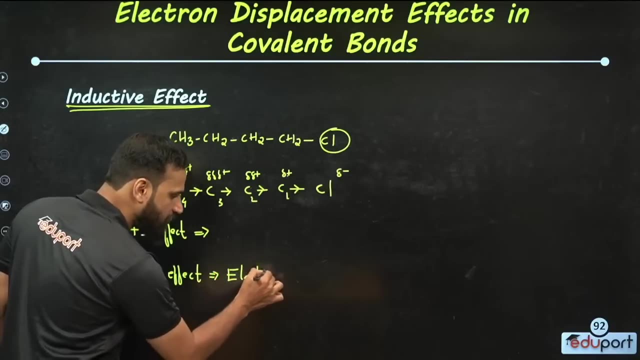 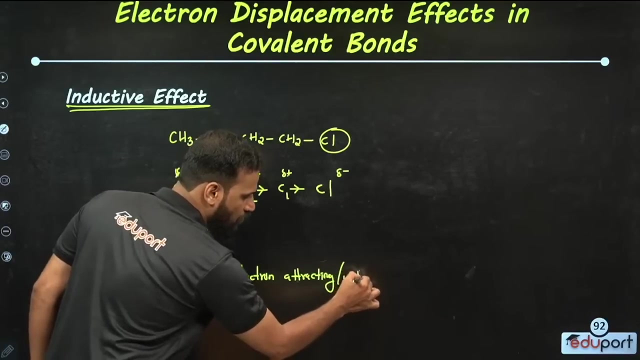 called chlorine comes inside an organic compound, what happens? The electron is attracted to it. The electron is attracted to it. That is called minus I-effect. What is the effect of this? It attracts electrons Or it withdraws. It withdraws electrons. 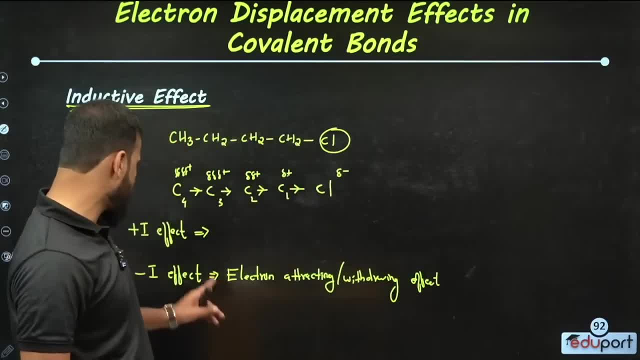 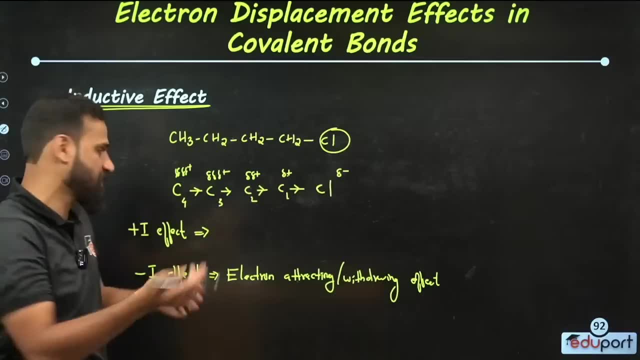 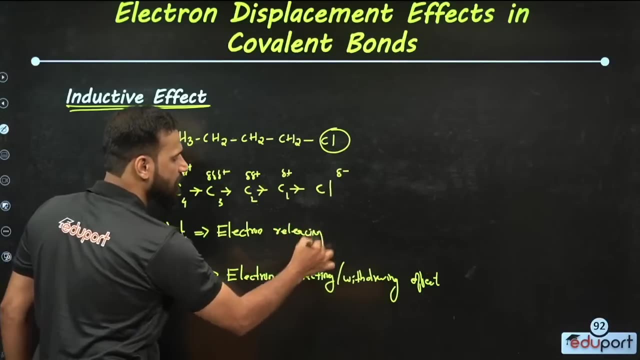 It attracts electrons Or it withdraws electrons. That is minus I-effect. What is plus I-effect? It brings electrons to the carbon chain. That is called electron releasing effect. What do we call it? Electron releasing effect? Electron releasing effect. 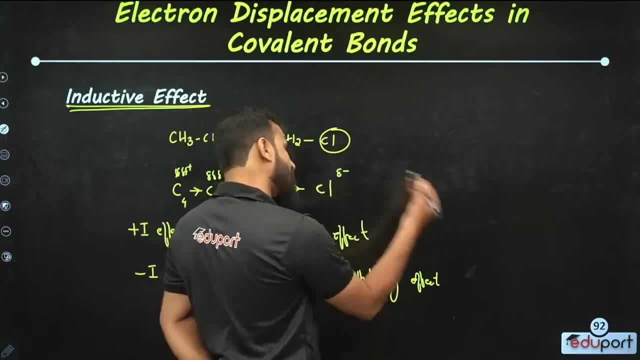 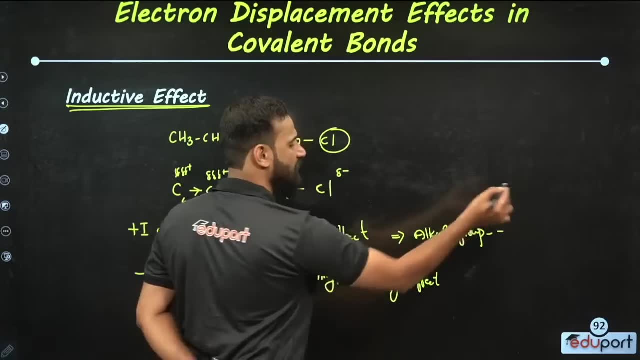 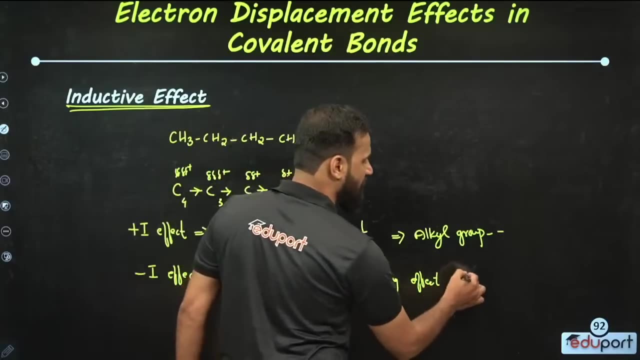 Or electron donating effect. Usually, usually, electron donating effect is shown by alkyl groups: Primary, secondary, tertiary and so on. Alkyl groups are given to electrons At the same time. minus I-effect is shown by halogen. 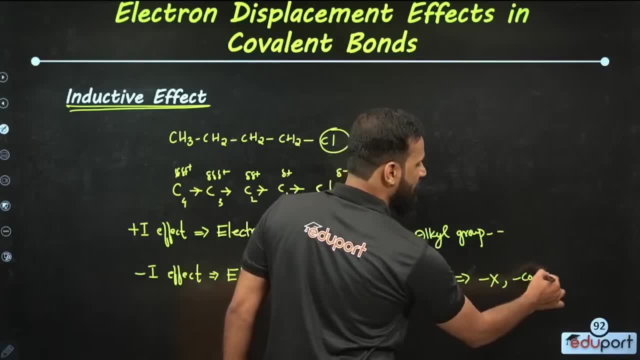 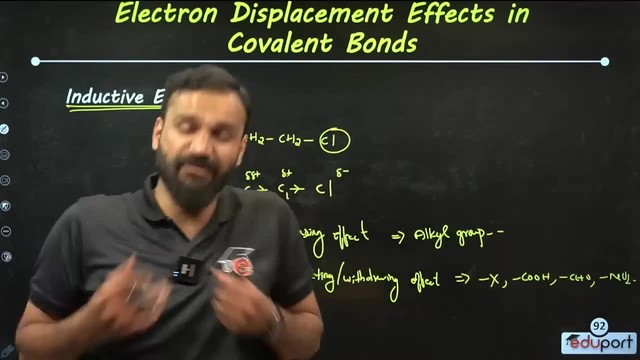 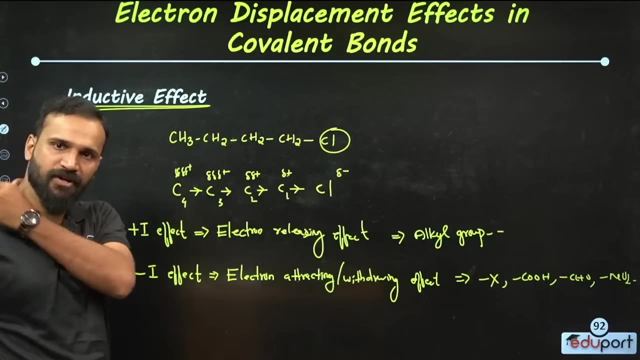 chlorine, bromine, iodine acid, aldehyde, ketone, NO2.. They are the ones that attract electrons. They are the ones that show minus I-effect Children, I am asking you what is inductive effect? Nothing. 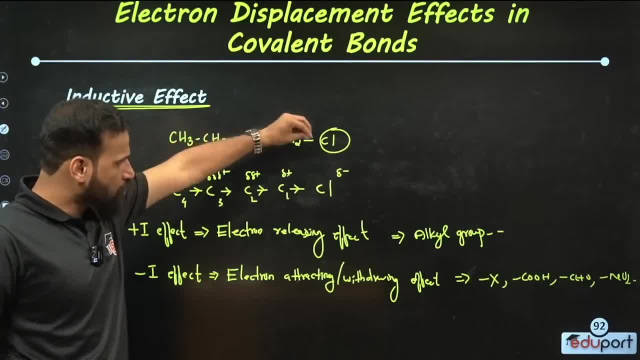 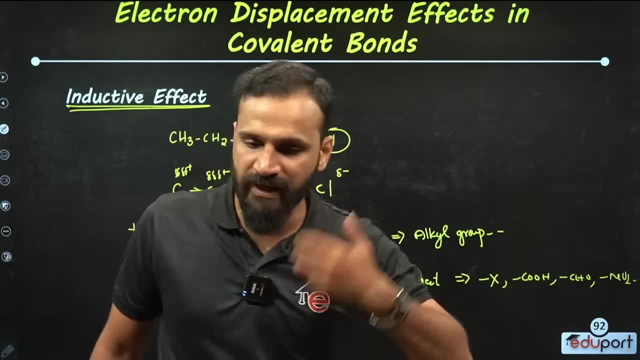 In an organic compound when there is a difference in electronegativity in that compound. through the sigma bond, electrons move. This phenomenon is called inductive effect. There are two types of it. One is the effect that attracts electrons. 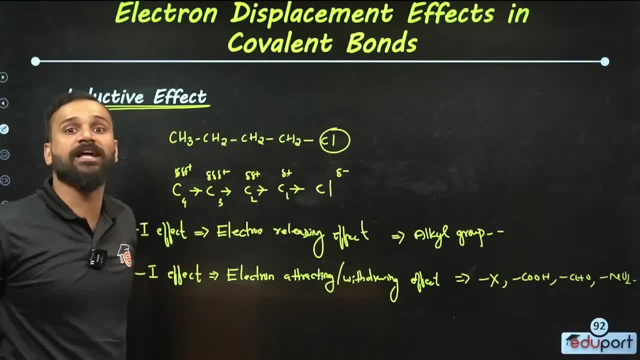 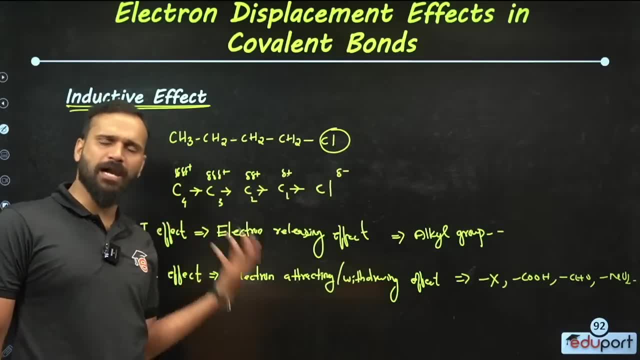 That is minus I-effect. The other is the effect that brings it there. That is positive inductive effect Plus I-effect. Usually plus I-effect is shown by alkyl groups, Then mainly halogen nitro groups as well as. 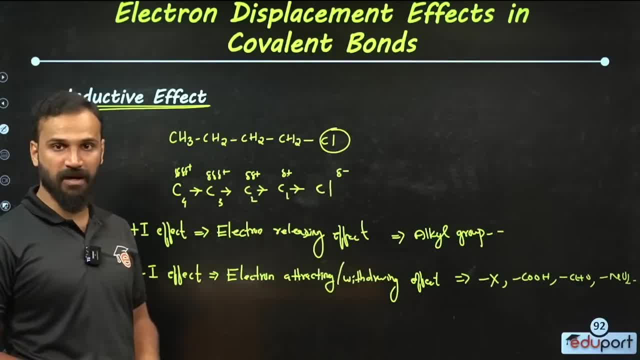 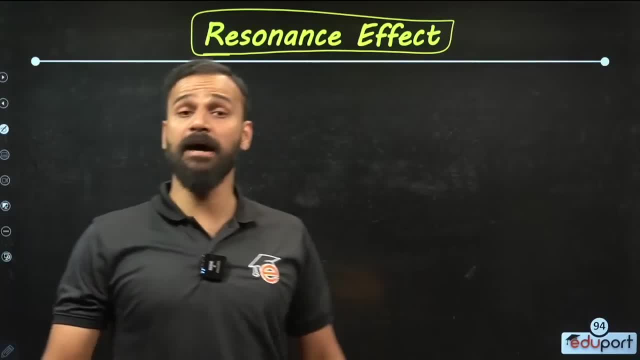 acids are shown as minus I-effects. That is the example. Keep that in mind. Now, children, look at the resonance effect. Resonance effect- What is it? It is the second electron displacement effect. I will show it through an example. 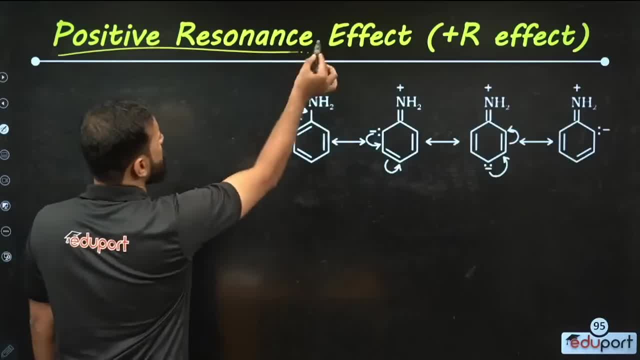 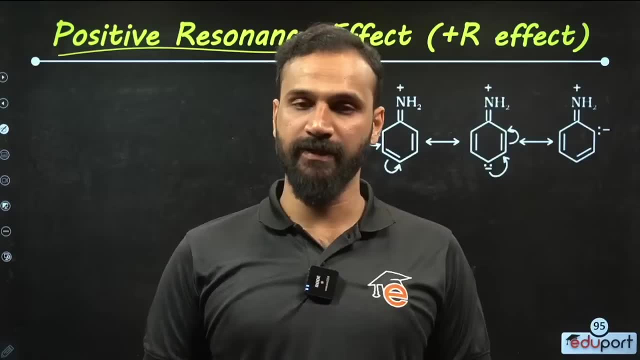 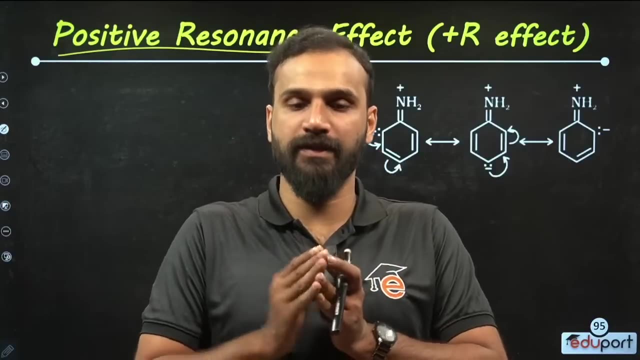 Look, children, There is a positive resonance effect, There is a negative resonance effect. It is simply said like this: In an organic compound there are two pi bonds, So pay attention carefully. In an organic compound, there are two pi bonds. 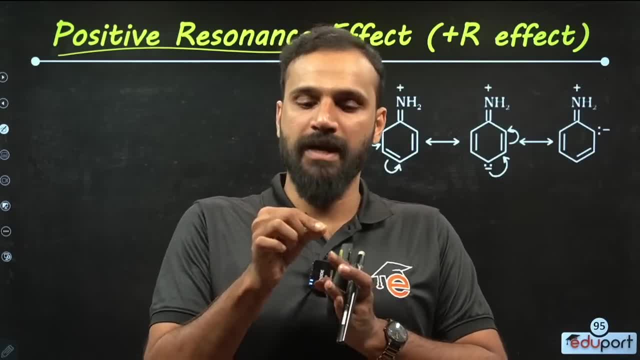 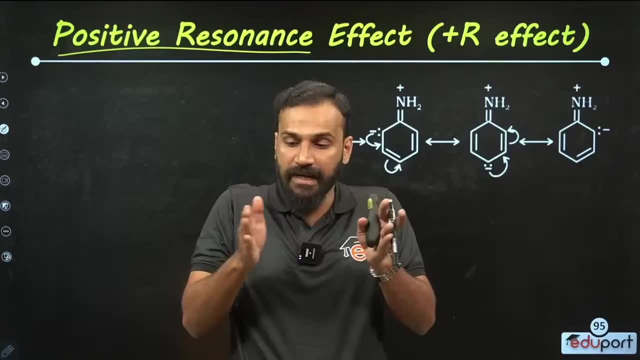 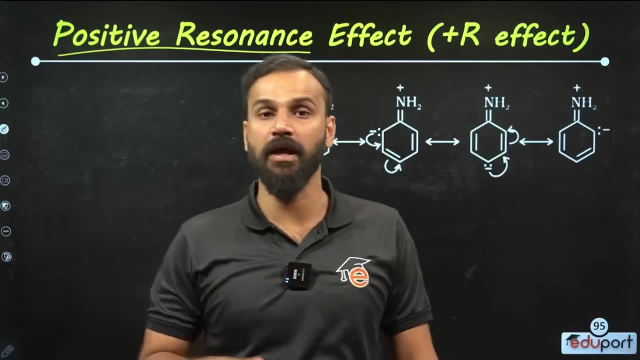 Or in one of the pi bonds there is a lone pair. Listen carefully: In an organic compound there are two pi bonds, One or two pi bonds, Or in one of the pi bonds there is a lone pair. When there is an interaction. 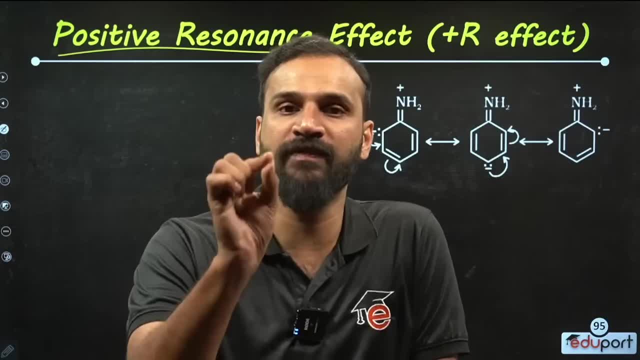 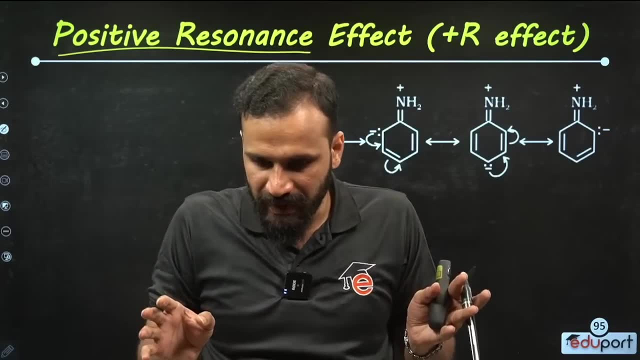 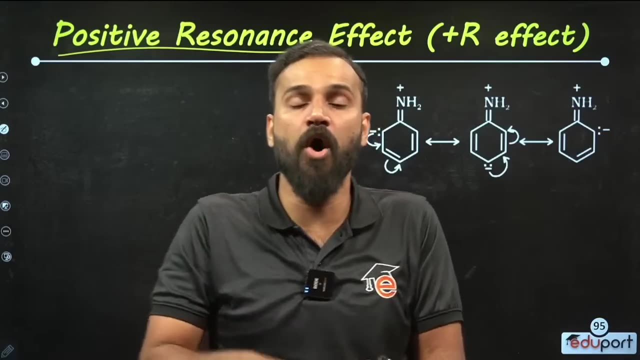 the phenomenon with polarity is called the resonance effect. Let me say one more thing. In an organic compound there are two pi bonds, Or when there is an interaction between a pi bond and a lone pair, the phenomenon with polarity is called the resonance effect. 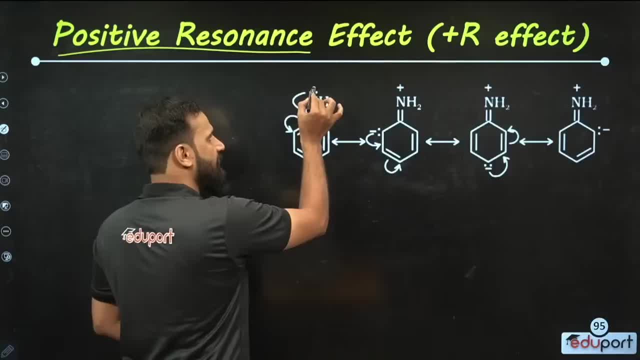 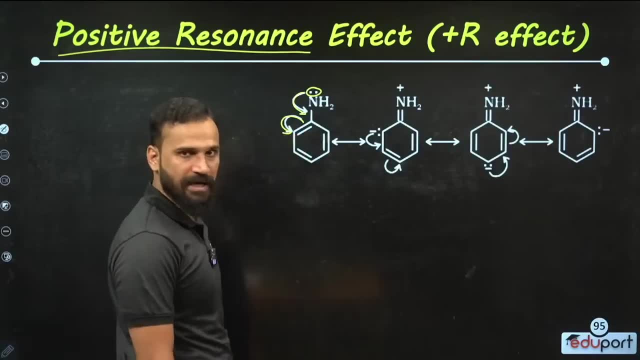 I will show you. Look here, Look here. When an electron pair in the hand of nitrogen comes down, a pi bond will shift here. When this lone pair comes here, a pi bond will shift here. What did we say? The interaction between a pi bond and a lone pair. 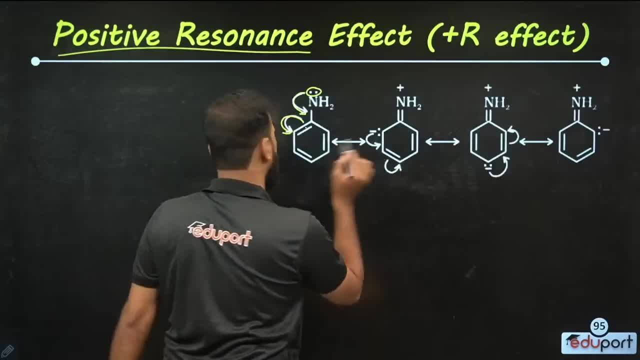 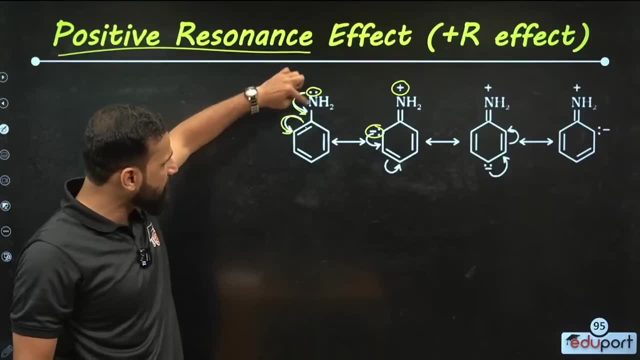 Ok, So you can see a plus here. Sorry, You can see a plus here, You can see a minus here, Isn't it? That is when there is an interaction between a pi bond and a lone pair. When there is an interaction, 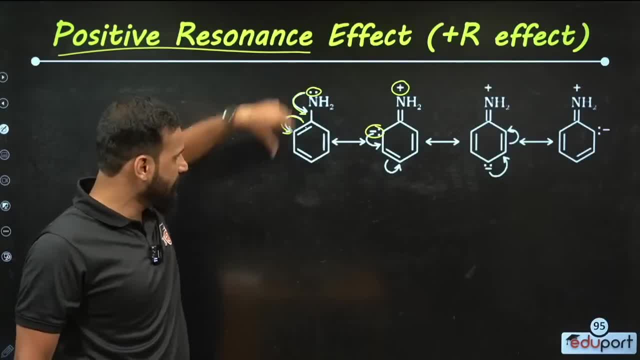 when the lone pair comes here, the pi bond will not go here. That is an interaction. When there is an interaction, there will be a plus and a minus. there, Polarity will be there. This phenomenon is a positive resonance effect. Now look. 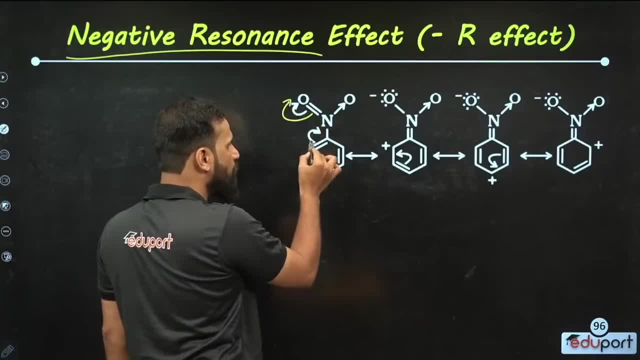 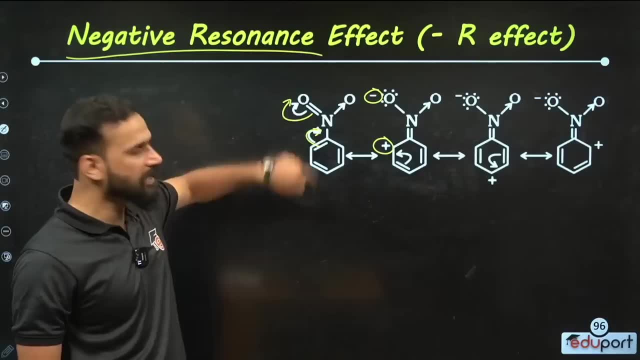 Here. when this pi bond goes here, this pi bond goes here. So look, Here there is a minus, Here there is a plus. What is this? This is the interaction between two pi bonds. So basically, when there is an interaction between two pi bonds, 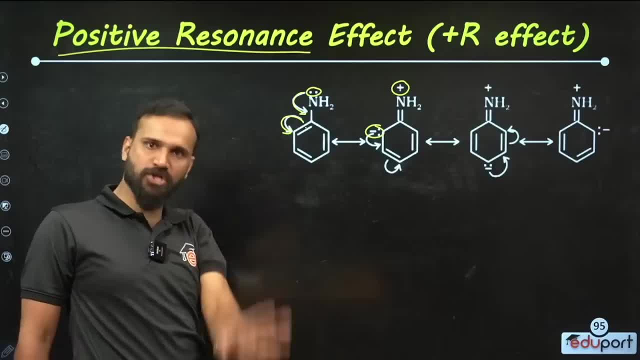 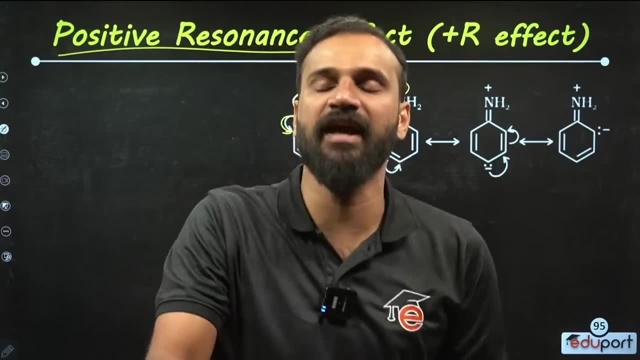 when there is an interaction between one pi bond and a lone pair, there will be a charge there, There will be a polarity there. Then the name we call that effect is the resonance effect. The name we call that effect is the resonance effect. 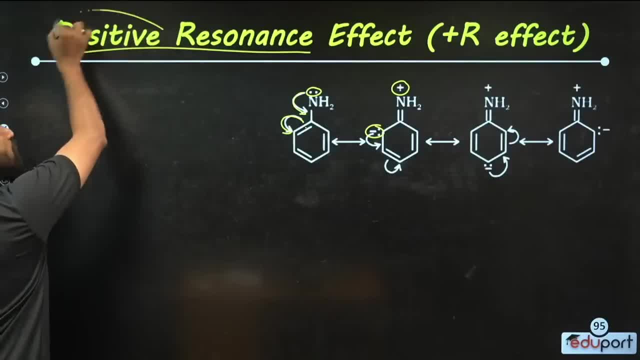 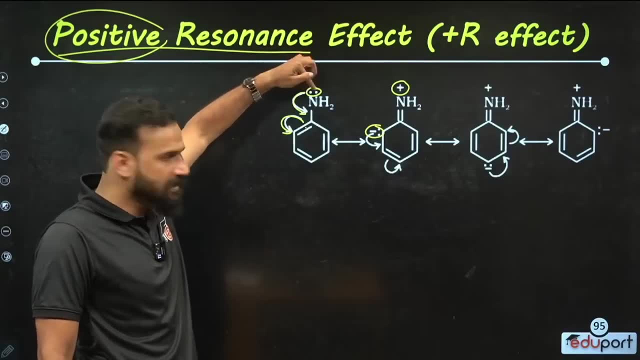 Look, There are two types of that resonance effect. One is positive and the other is negative. Do you know what the positive is? The positive is from the functional group to the benzene ring, or we can call it the delocalized system of the benzene ring. 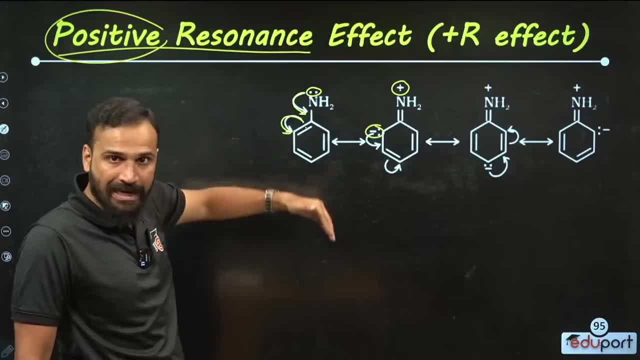 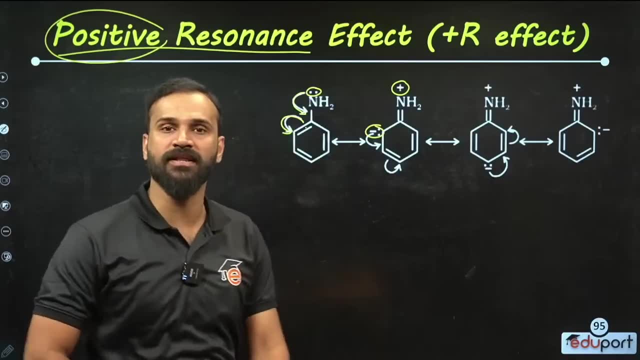 From the functional group to the benzene ring or to the delocalized system, the electron pair comes, That is, the electron pair comes down from there. If it is so, it is a positive resonance effect Now from the benzene ring. 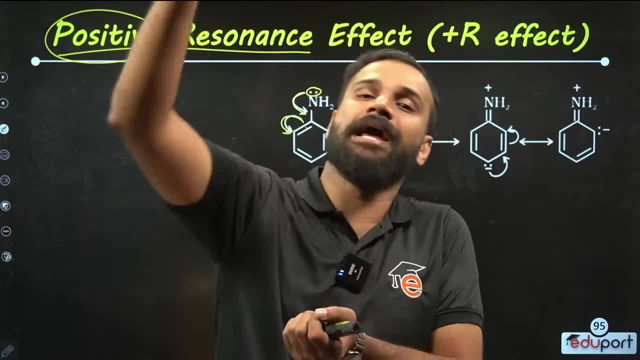 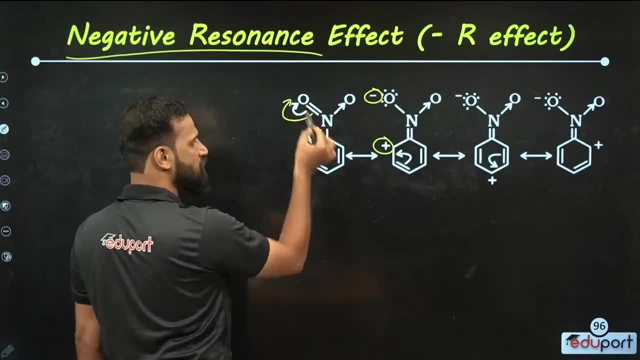 or from the delocalized system to the functional group. if the electron pair moves it is a negative inductive effect. You can see here When this pi bond goes here, the electron in the benzene goes up to the functional group. 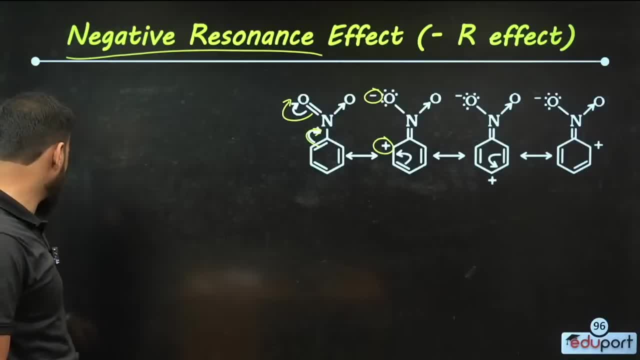 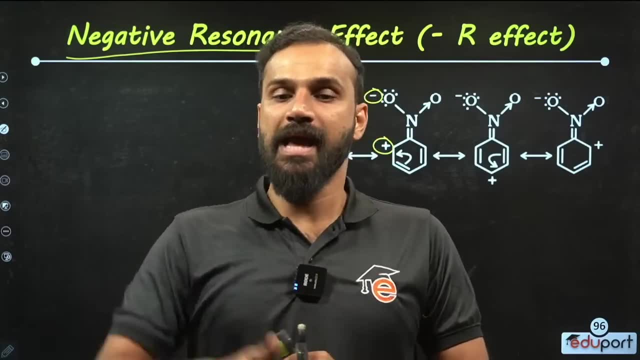 That is the negative resonance effect. What do you call it Negative? So I will say one more thing. Between the two pi bonds in one molecule, or when there is an interaction between one pi bond and the electron pair, the phenomenon with polarity in that molecule. 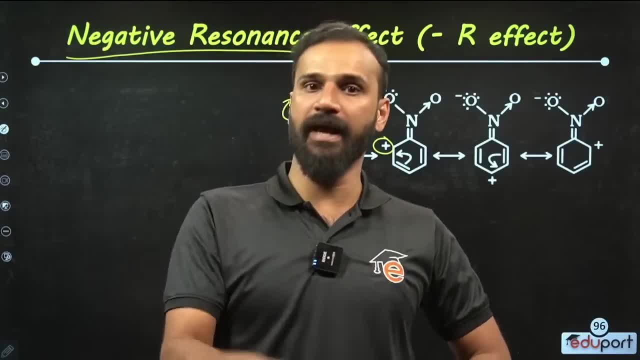 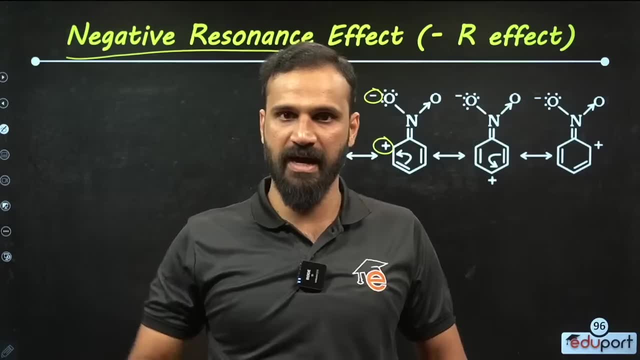 we call it the resonance effect. There are two types of that. If the electron pair goes down from the functional group to the benzene ring, that is a positive resonance effect. If the electron is displaced from the benzene ring to the top: 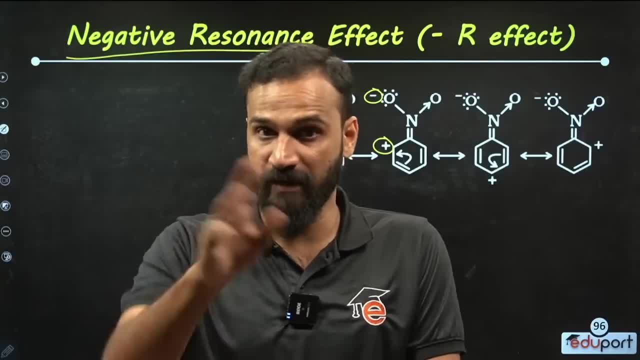 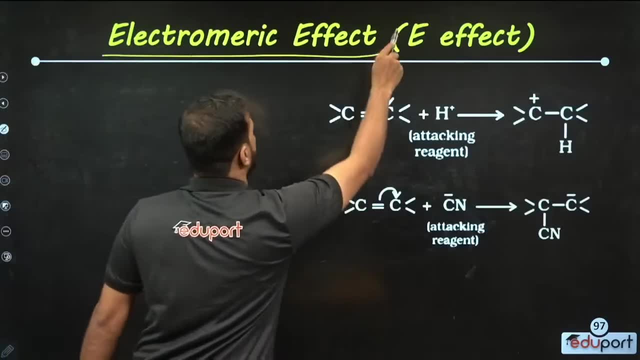 it is a negative resonance effect. Not an inductive effect, but a negative resonance effect. Please understand this. Now look at the third electron displacement effect. What does it mean? Electromeric effect- Which effect is it? Which effect is it? 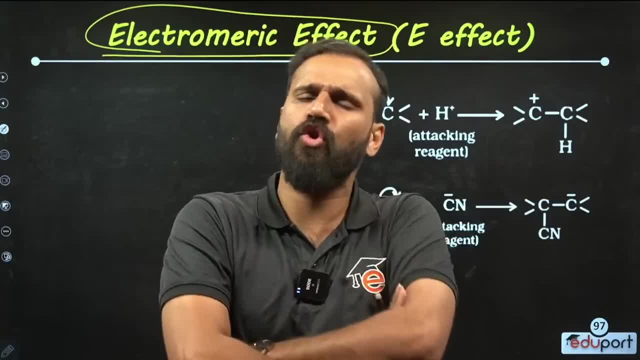 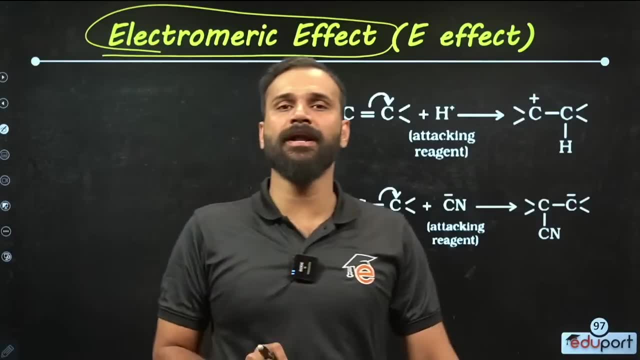 Electromeric effect. What is an electromeric effect? It is a very simple thing. What do you know guys? A double bonded or a triple bonded system, or generally a multi-bonded system, What do you call it? 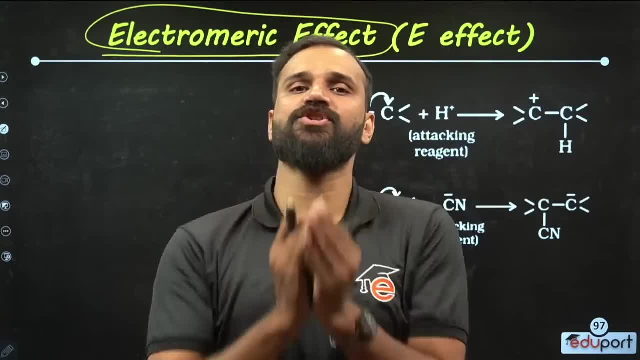 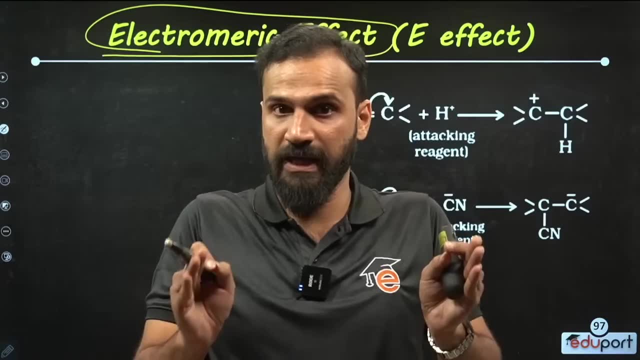 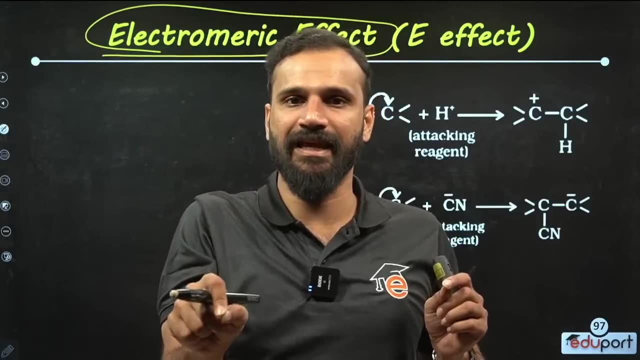 Multi-bonded system When an attacking reagent comes to such a system. when an attacking reagent comes to such a multi-bonded system, that is where we apply this: When an attacking reagent comes to such a multi-bonded system. 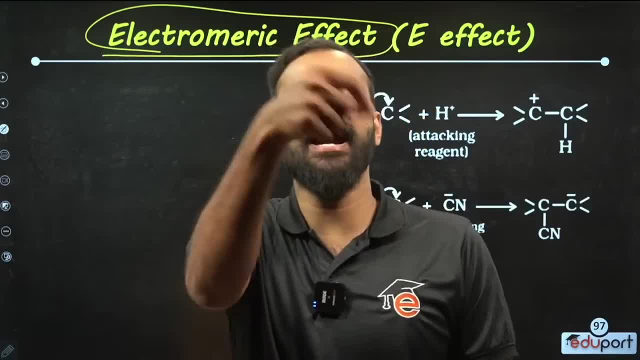 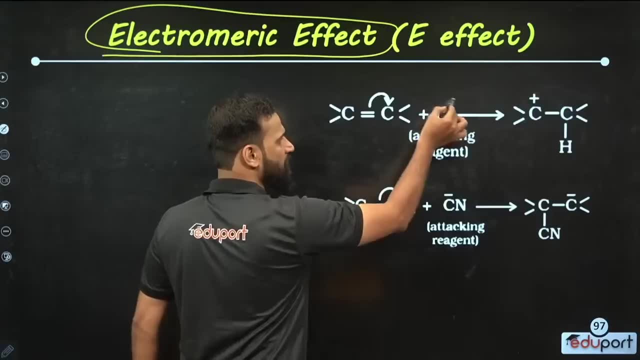 the pi bond. there is a phenomenon that shifts to any one axis. This is called the electromeric effect. You can see it here: When an attacking reagent called H plus comes here, this pi bond shifts with it. That is the electromeric effect. 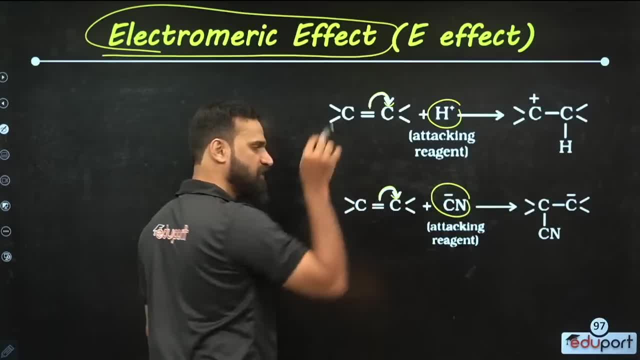 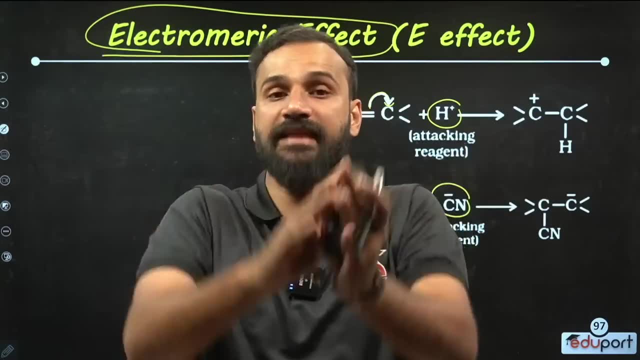 When an attacking reagent called CN comes here, this pi bond shifts with it. When an attacking reagent comes here, if the pi bond there shifts to any one axis, that process is called the electromeric effect. Now, guys, there are two types of that. 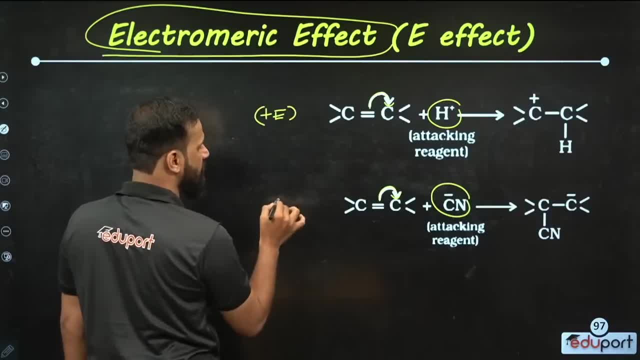 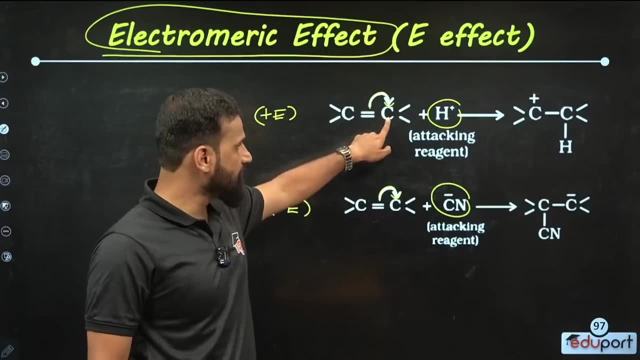 One is positive electromeric effect and the other is negative electromeric effect. What is the positive electromeric effect? Where does this pi-bond shift? It is near this carbon, doesn't it? If the attacking reagent is bonding to the same carbon. 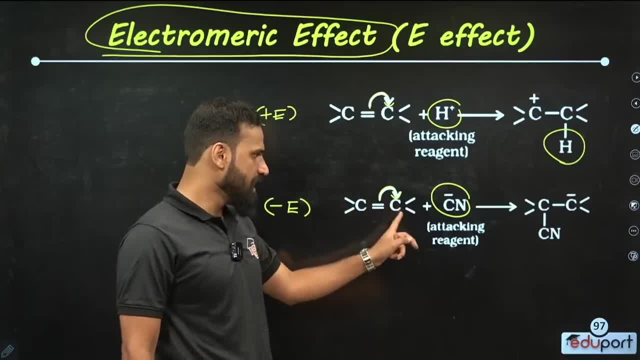 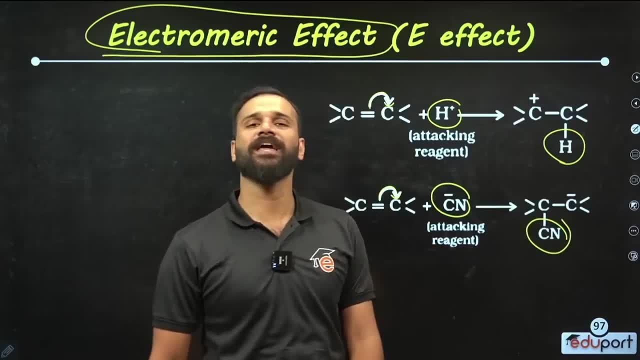 that is the positive electromeric effect. Where does this pi bond shift? It is shifted here But is attacking reagent bonded there Non-stop. It is bonded to the nearby carbon, So negative electromeric effect. Where does the pi bond shift? 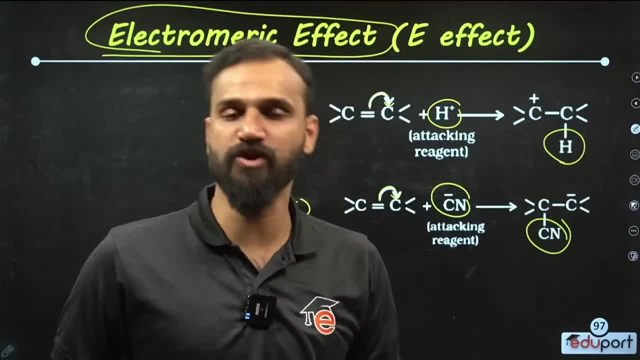 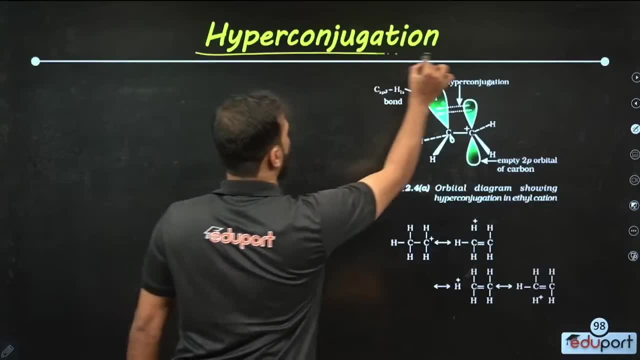 If the attacking reagent is bonded to the same carbon, it is positive. Otherwise, if it happens again, it is a negative electro-american reaction. Now look at the hyper-conjugation effect. Hyper-conjugation effect is a CH-sigma bond. 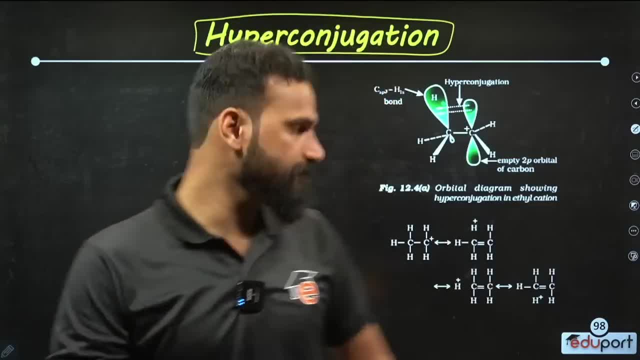 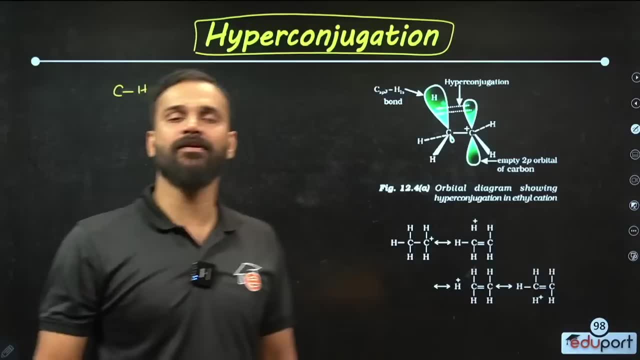 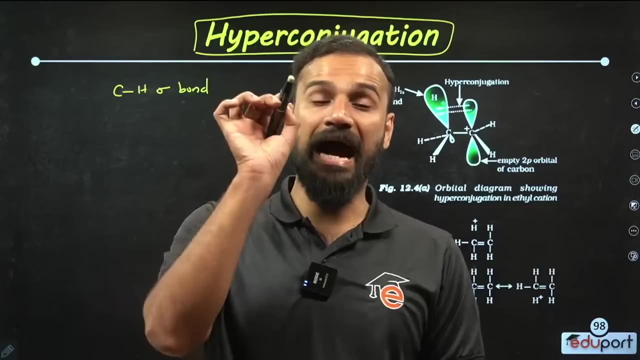 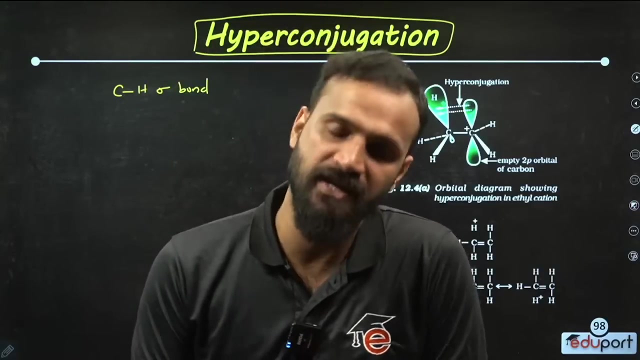 inside an organic compound. CH-sigma bond interacts with anyone. It is the carbon atom near the unsaturated carbon atom or the carbon atom in the unshaded P orbit. Either way, the partial conjugation layer is the effect. Let's call it the hyper-conjugation effect. 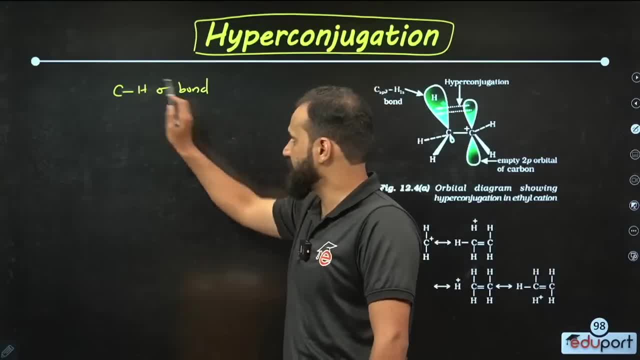 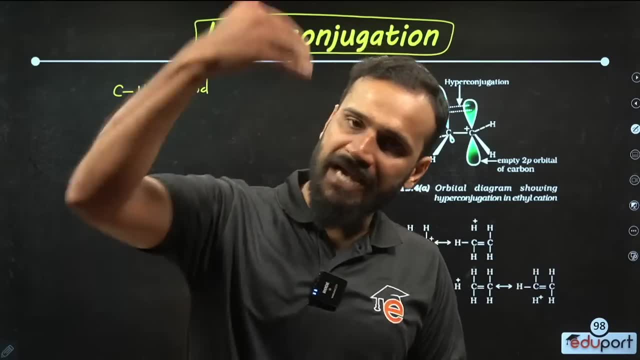 There is a CH-sigma bond inside an organic compound. The unsaturated carbon atom, near it, the carbon atom with 00000, or the carbon atom in the unshaded P orbit. it is the unsaturated carbon atom. conjugation layer effect is called. 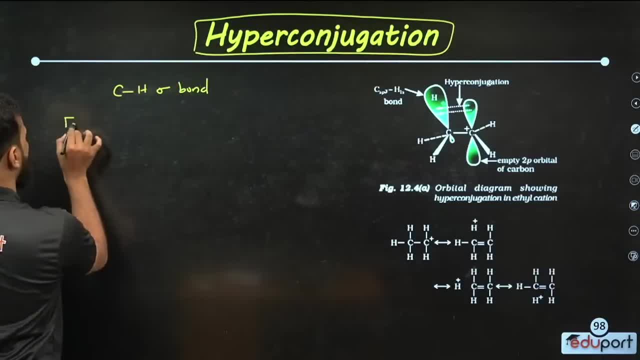 hyperconjugation effect. The most typical example of this is ethyl cation. We can say ethyl carbocation or ethyl cation. It is actually like this: Ethyl cation, We can take ethyl cation. Now see what else you can take: CH. 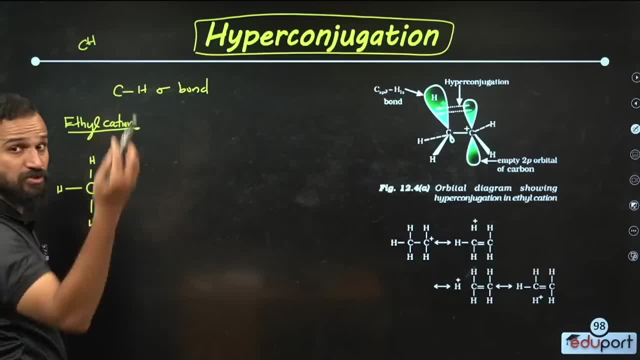 double bonded system, unsaturated system, or you can take ethyl cation. How do you take ethyl cation CH2O+? This is ethyl cation. If you want to represent this as a bond, you can do that. If there is a problem. 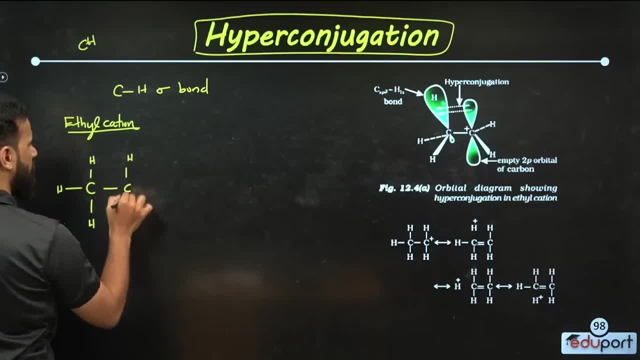 in giving H2, you can represent it as a bond. You can give an H here and an H there. This is an unshaded pure orbital carbonate. It has 3 CH sigma bonds around it. Those 3 CH sigma bonds shift towards it. That is the partial conjugation layer effect. 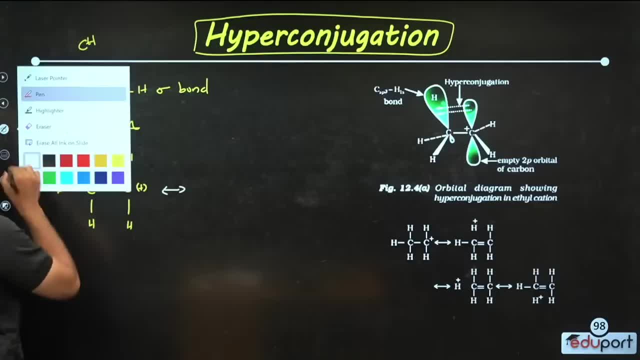 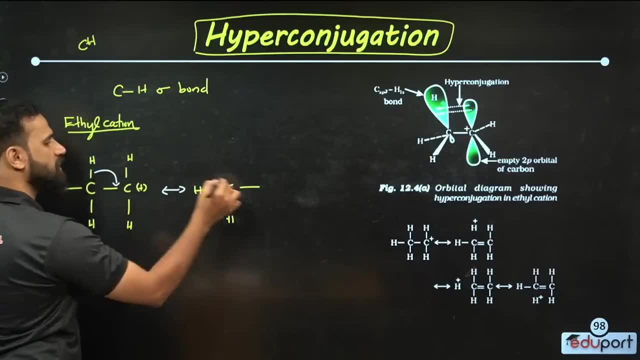 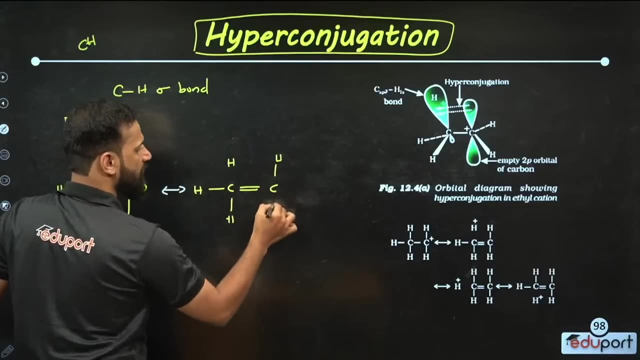 That is what we are trying to say. So we will get the next resonance structure, This H, carbon H. There is no change in that. When this bond shifts towards it, this single bond will become a double bond. The bond shifts and the hydrogen is there itself. 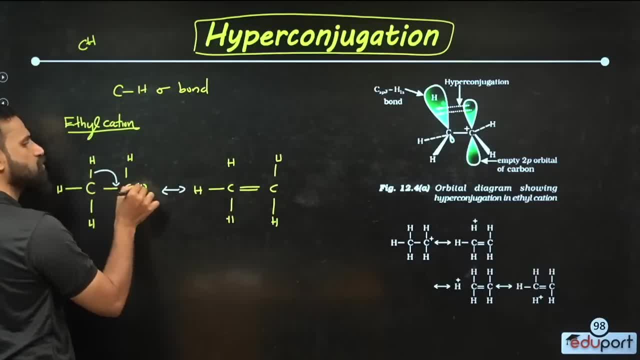 Now there are 2 H's with this carbon. Since there are 4 bonds with this carbon, he does not have to give a plus. That plus will automatically go to him because the bond is lost there. He can move towards it. That is the next resonance structure. 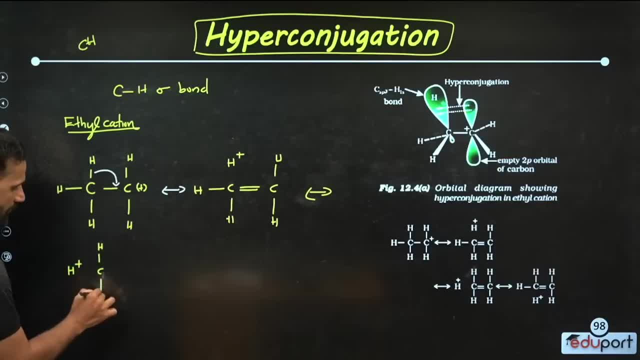 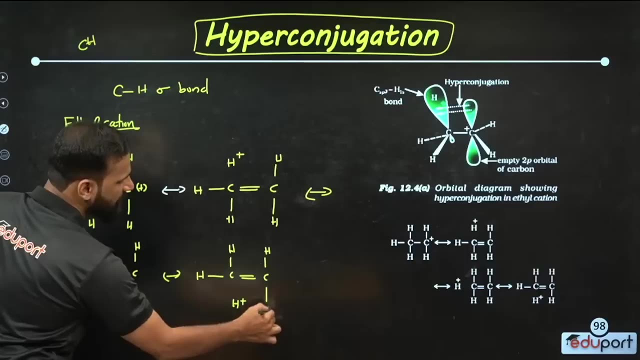 If he moves towards it, that H will get a plus, That H will get a plus and this single bond will become a double bond. If he shifts towards this H, he will get a positive. There will be no bond there. So you have to understand that this effect. 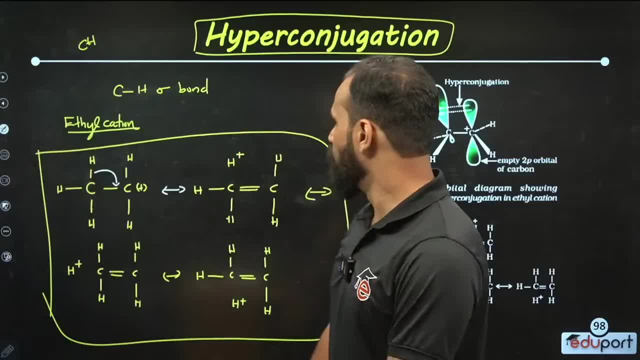 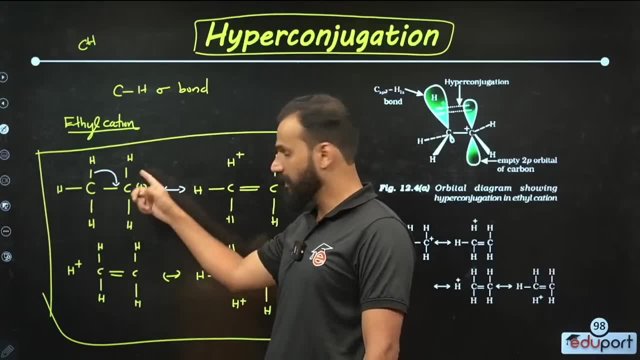 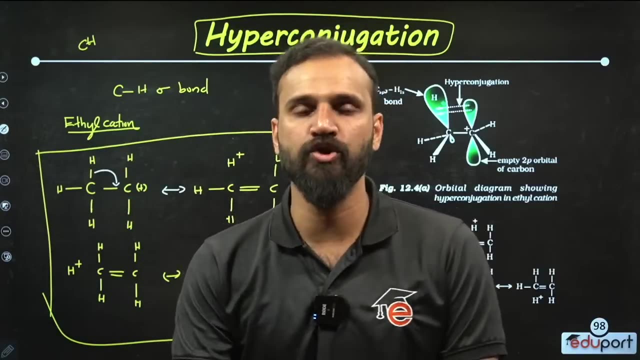 is called the hyper conjugation effect. In other words, a CHs bond inside an organic compound with the unsaturated carbon nearby or with the carbon atom in the unshaded p-orbit is called the partial conjugation layer effect. This is the hyper conjugation effect. 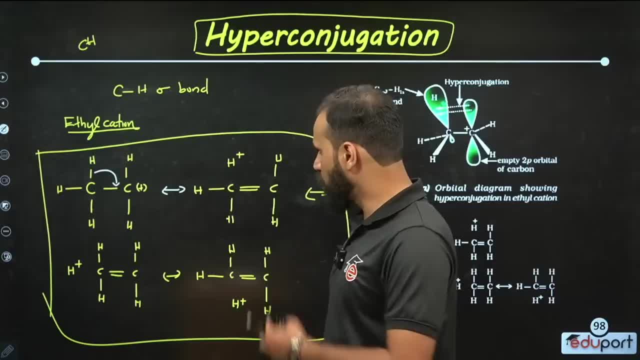 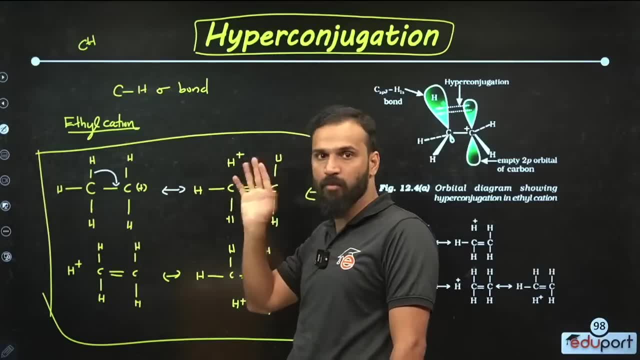 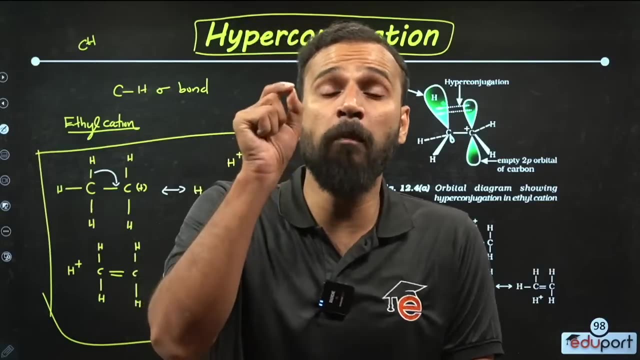 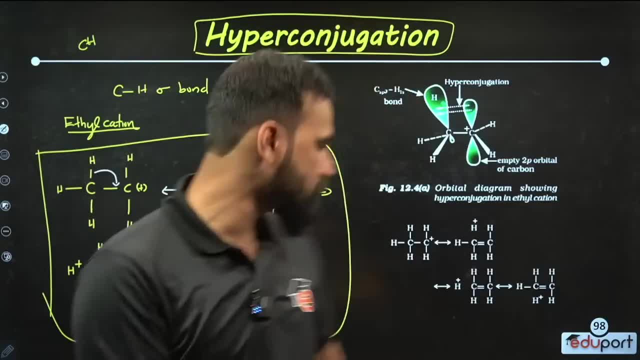 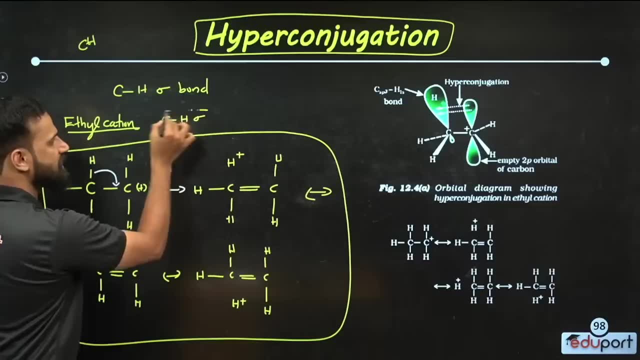 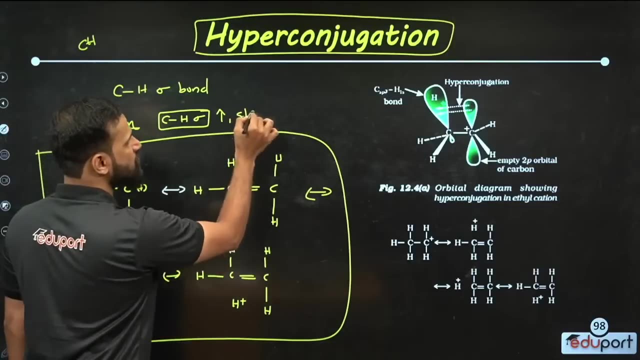 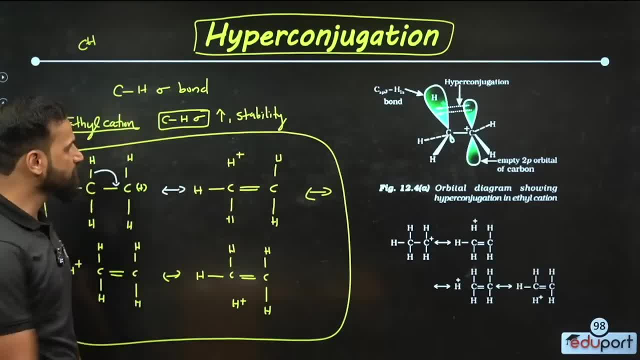 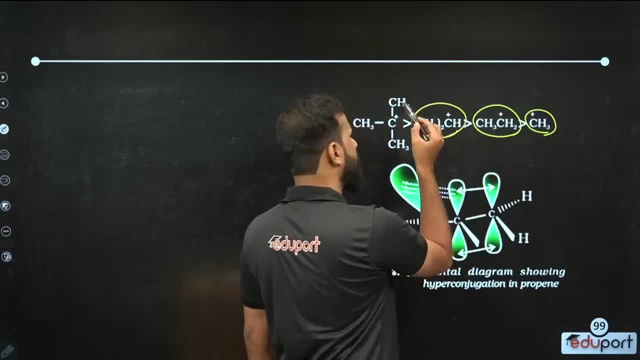 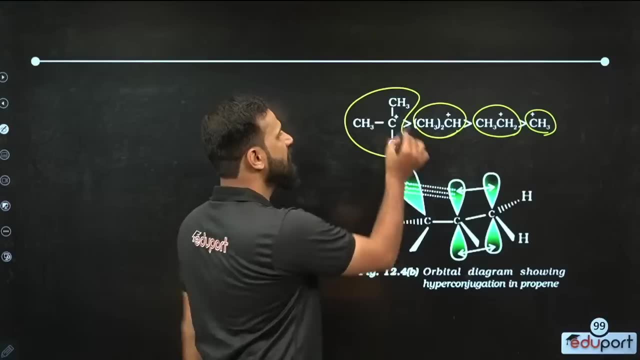 And the stability of the molecule will increase. The stability will increase. So, if we look at it, the methyl cation and the secondary cation and the tertiary cation are tertiary right. Stability is the most important thing, Because here there are 9 CHs bond. 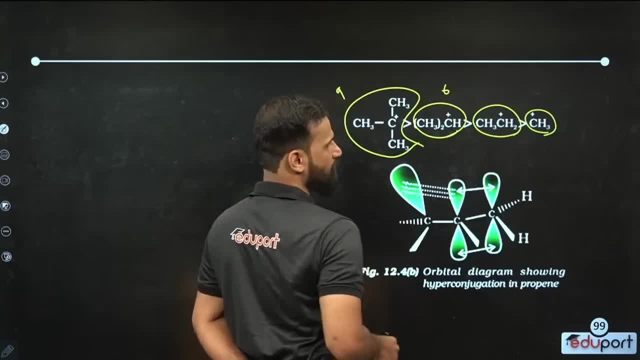 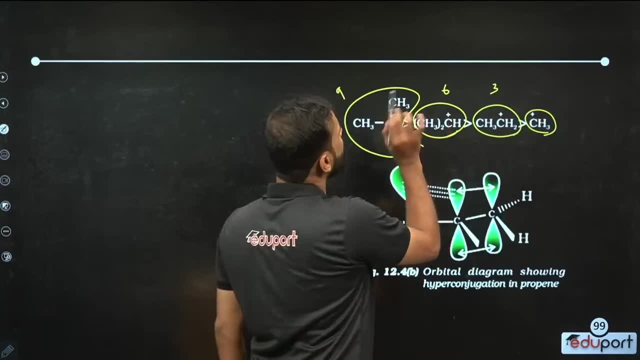 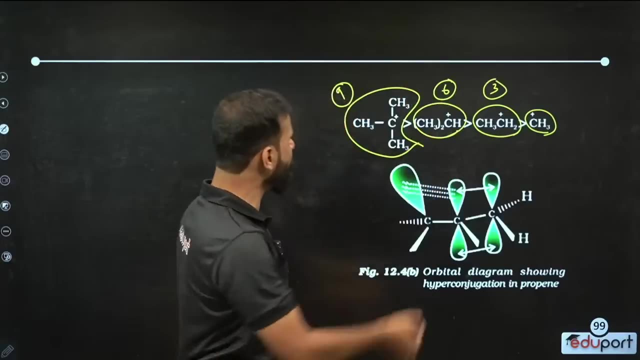 How many CHs bond are there here? Here there are 6 CHs bond. Here there are 3 CHs bond. So you have to understand that if there are 9 CHs there will be 9 resonance. Here there are 6 resonance. There are only 3 here. 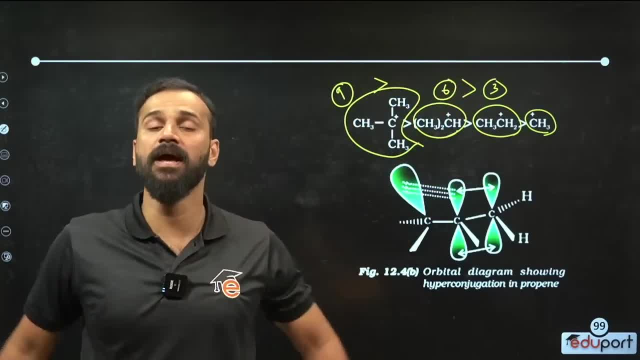 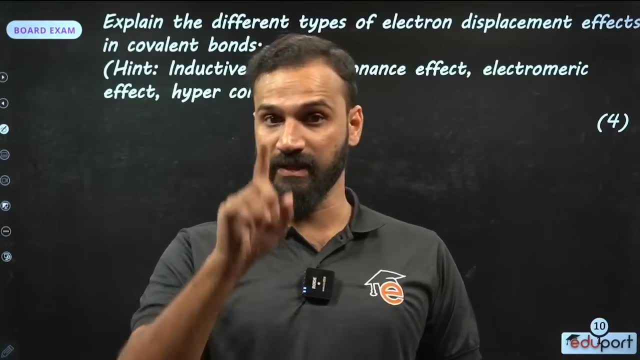 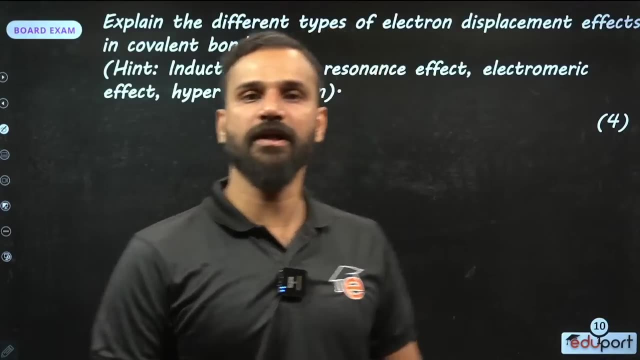 So you have to understand that there is a stability in the tertiary or secondary or primary. So you have to understand that there is a stability in the tertiary or secondary or primary. You have to learn about the electron displacement effect. You have to learn inductive effect resonance. 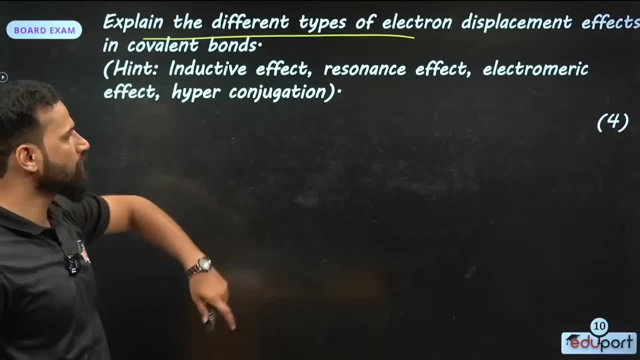 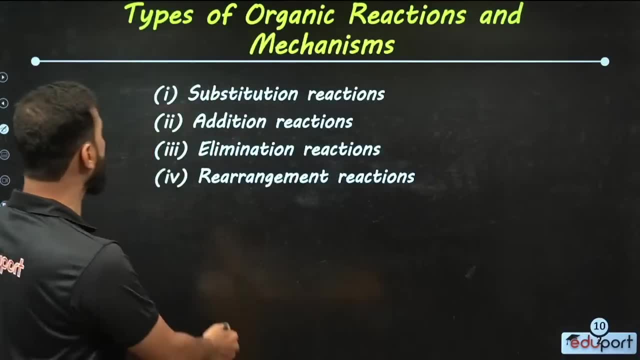 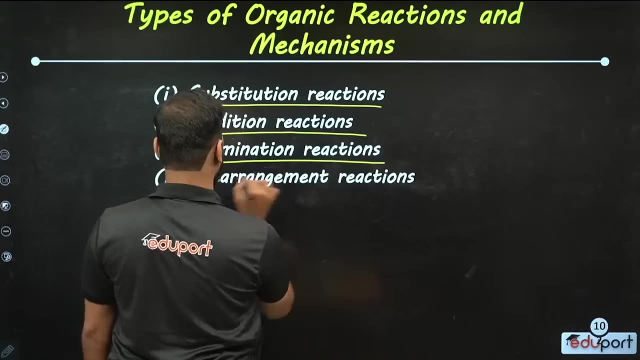 and electro-americ and hyper conjugation. Explain the different types of electron displacement effect in covalent bond should be done Now look, children. there are four types of reactions. What are they? One is substitution, addition, elimination, rearrangement reaction. What is? 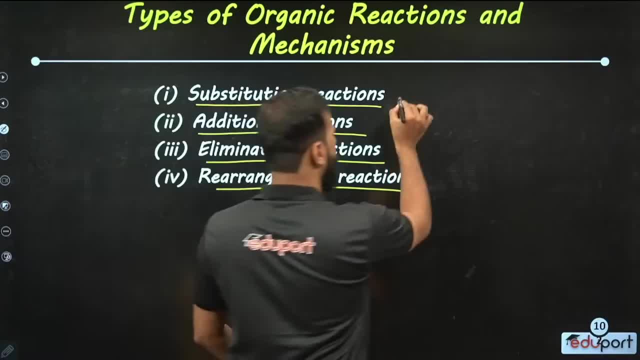 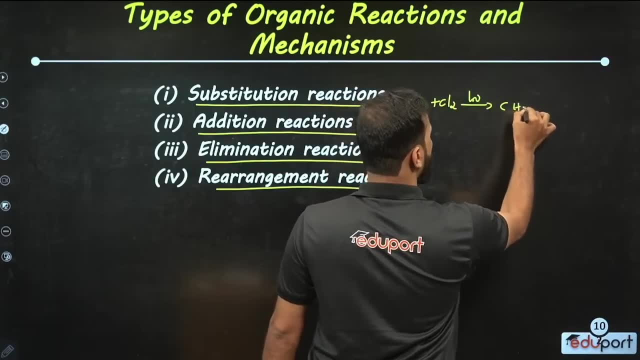 substitution reaction. You know one person goes and another person comes. For example, we add chlorine to CH4 in the presence of light, Then a hydrogen goes and chlorine comes, Then CH3Cl plus HCl will come. That is an example of substitution. What is the addition reaction? 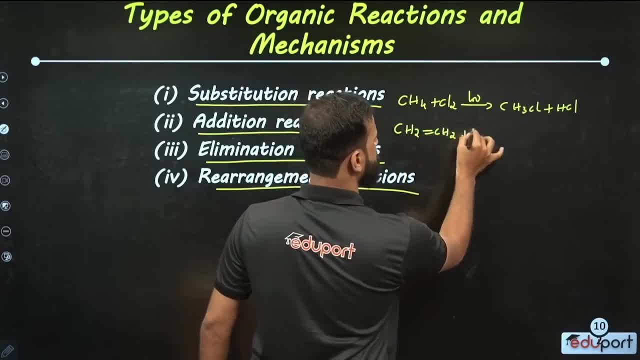 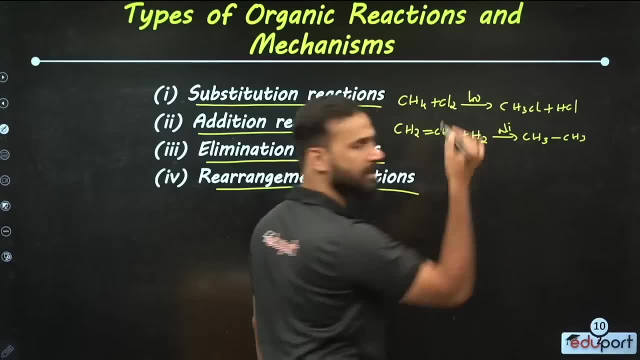 We add something to a reagent- For example, I added H2 to ethylene- What do we get if we add it to nickel presence, CH3- single bond, CH3 is not obtained, So this H2 was added. What is elimination? 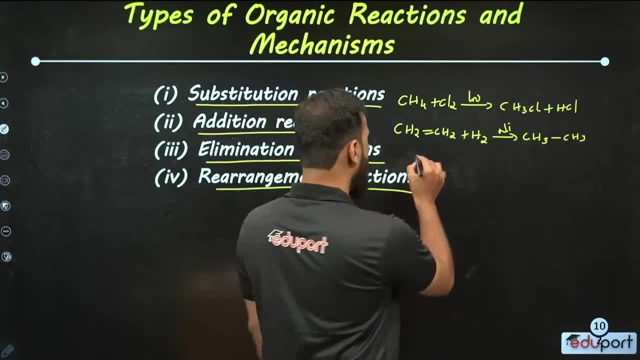 Someone will eliminate it. Someone will eliminate it. For example, what do we do to CH3CH2OH In the presence of concentrated sulfuric acid? If the concentration is treated in the presence of sulfuric acid, then the concentration of sulfuric acid is reduced. 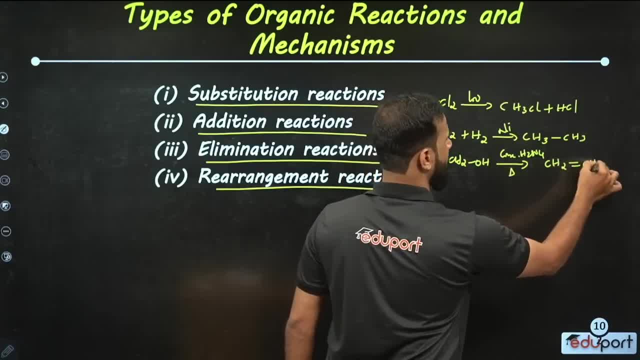 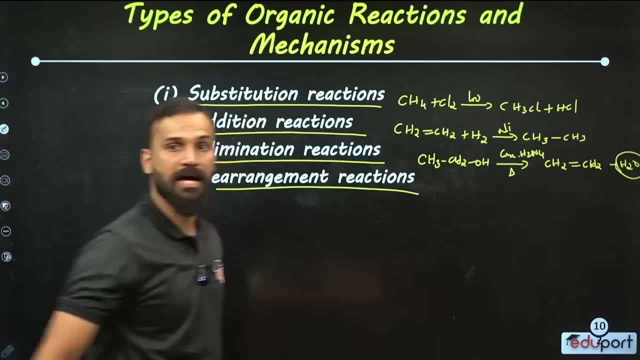 If heated, the water is eliminated there, and then what will happen? children? The water will be eliminated and then only ethylene will be there. So the water is eliminated here and gone. What is that? an example Example of elimination reaction. Then one person goes and another person comes. 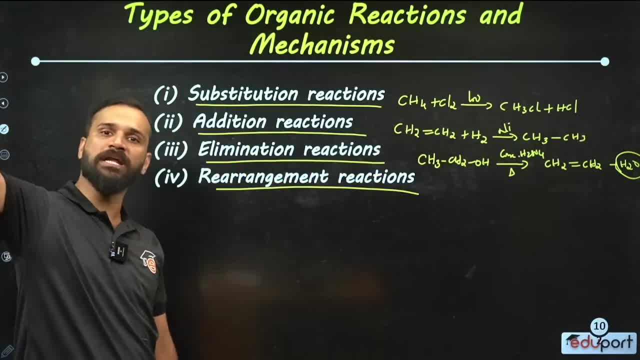 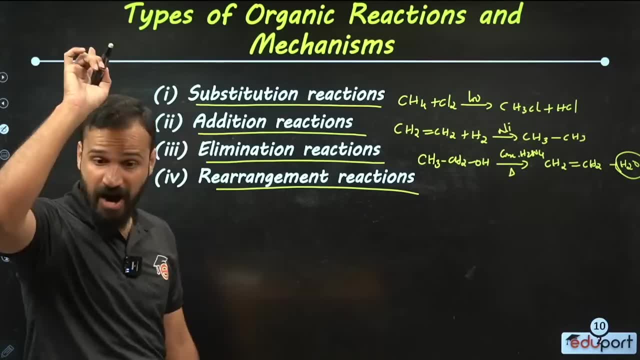 When you say addition, when you add, Elimination means someone eliminated. What is the rearrangement? No one in that room is coming or going. Rearrange what you have. In the first part of this chapter we said the reaction of Frederick Wallen. 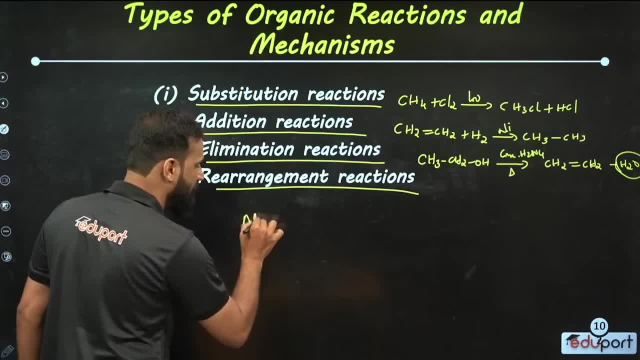 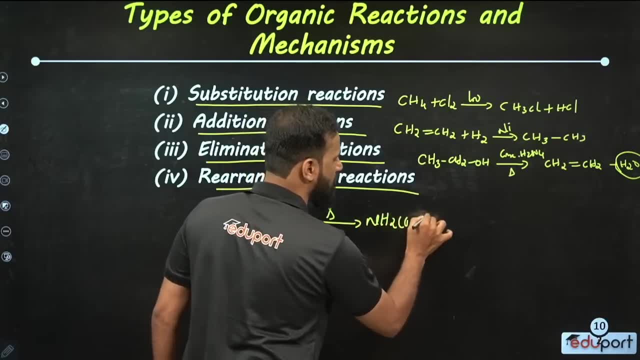 That is an example of it. What is the example of that? MH4C and Ammonium Cinate heat at the time of NH2C or NH2. right, No one goes, no one comes, but the one who is there. Ammonium cyanide uriate turns into a a. 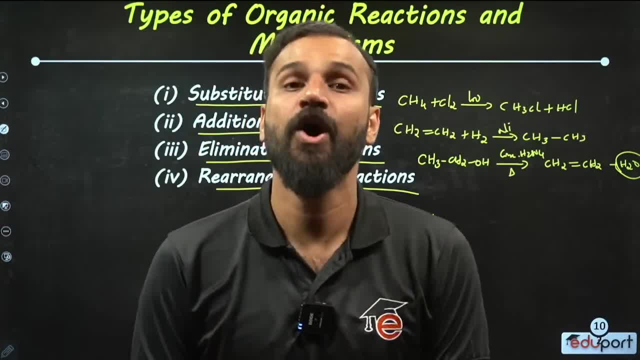 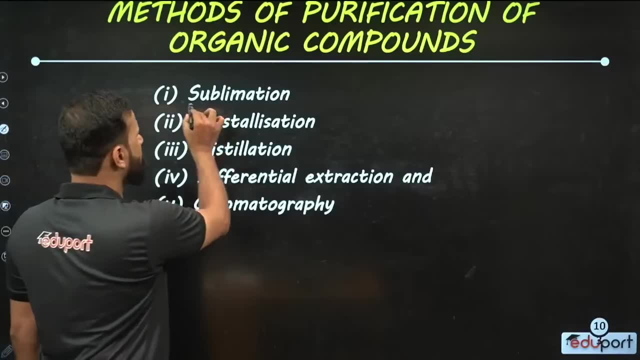 rearrangement reaction example. Please remember that thing. Okay, right, friends, Now we can quickly complete the purification. What is it? Sublimation, crystallization, distillation and the distribution of the having for the ammonium cyanide reaction reaction. 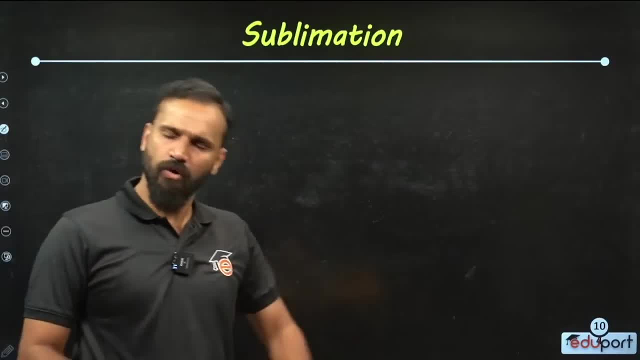 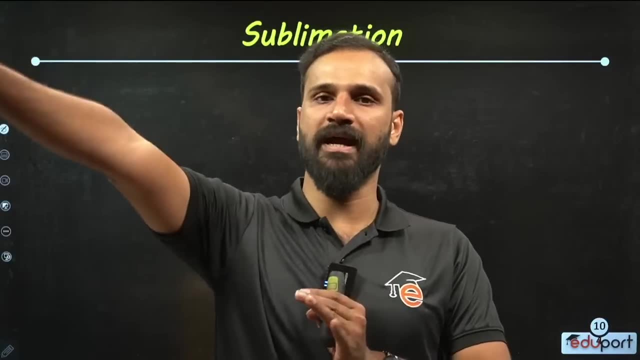 differential extraction and chromatography. What is sublimation? I am not saying anything. You have an organic compound in your hand. It has impurity. Impurity is sublimable. Sublimable means it becomes gas directly. Organic compound is not sublimable. 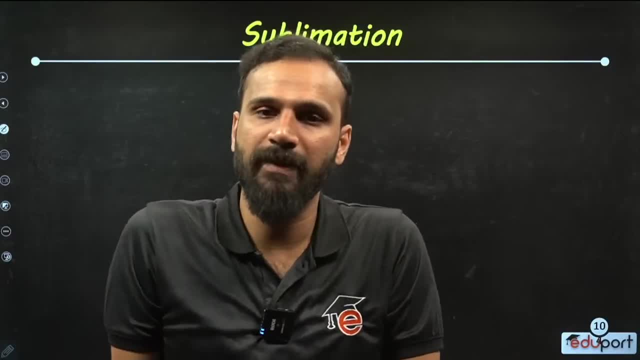 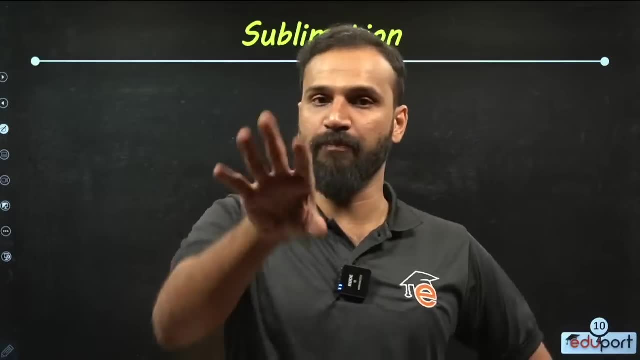 Either organic compound is sublimable or impurity is not sublimable. If one person is sublimable and the other person is not sublimable, you can purify it with the method called sublimation When you purify it. 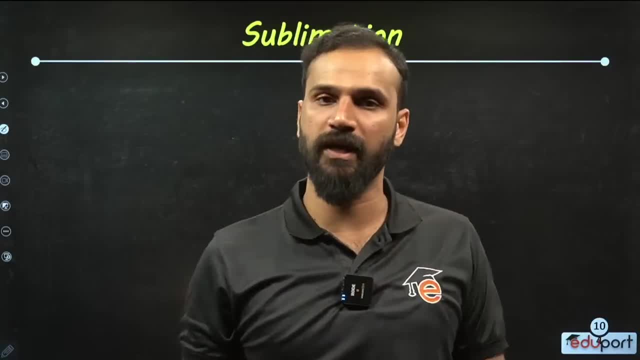 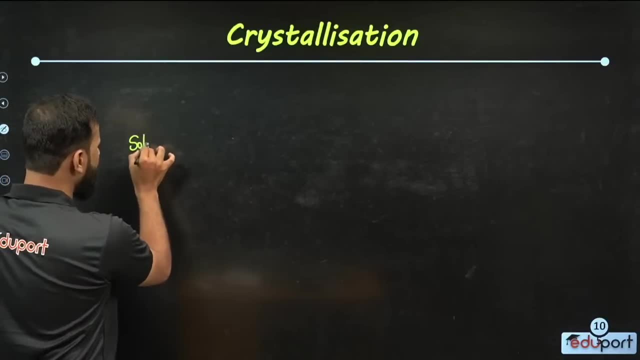 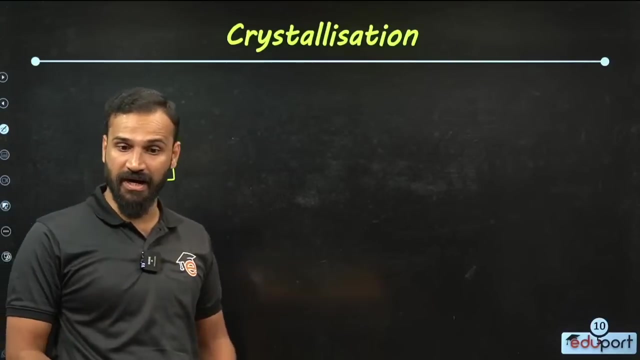 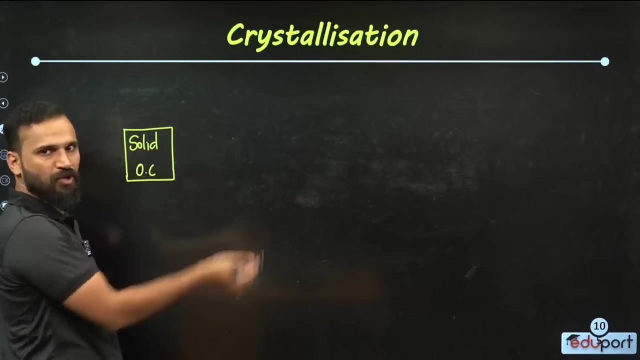 the sublimable compound becomes gas and the sublimable compound remains. That is called sublimation. What is crystallization? Usually a solid organic compound. to purify a solid organic compound we use crystallization. We have organic compound and impurity. 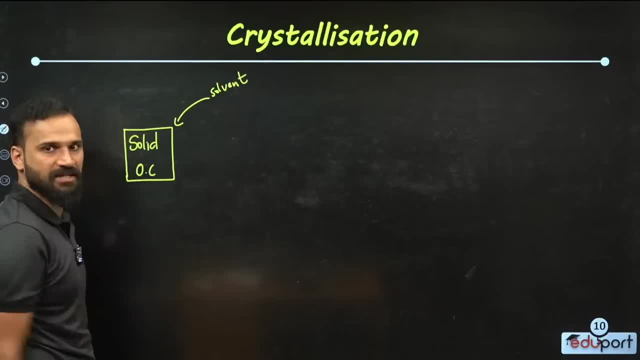 We add a suitable solvent to it. The peculiarity of that solvent is: only the organic compound in it should be dissolved. in it Impurity should not be dissolved. So if the solvent is added and heated, well, only the organic compound dissolves. 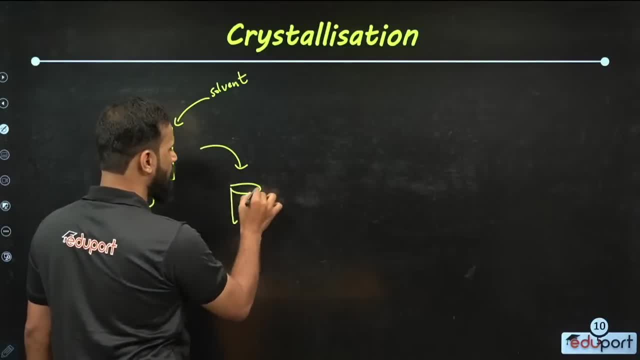 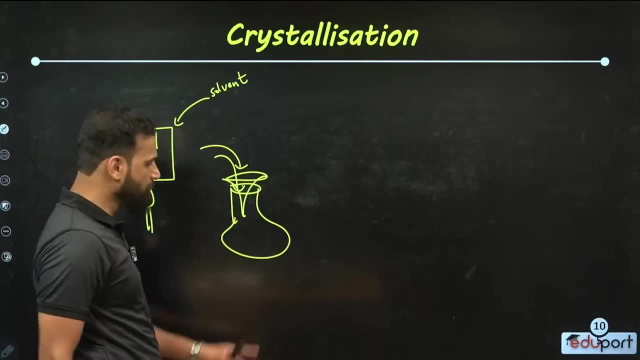 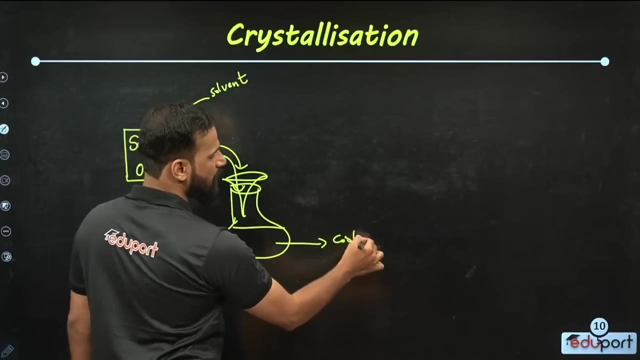 and impurity does not dissolve, Then filter it with a conical flask and filter it with a funnel. When filtered, impurity will remain here. The organic compound dissolved in the solvent will be here. If this is collected and cooled, we will get the organic compound. 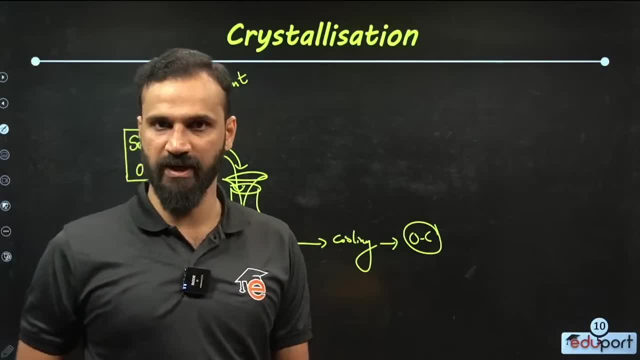 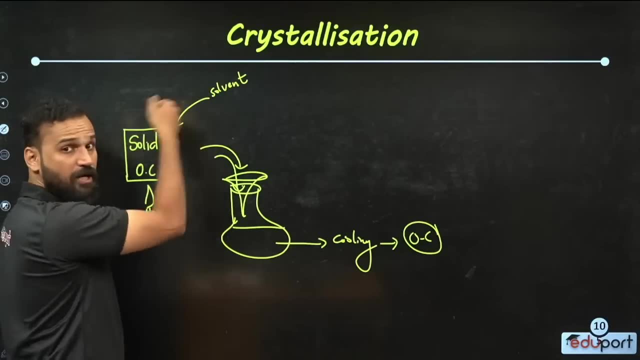 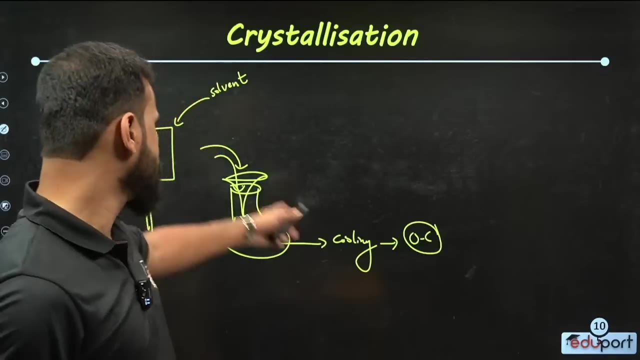 as a crystal. This is called crystallization. So crystallization means first of all the organic compound should be dissolved in the solvent. If added, it should be heated and dissolved. Then filter it. If the organic compound is cooled, we will get the organic compound. 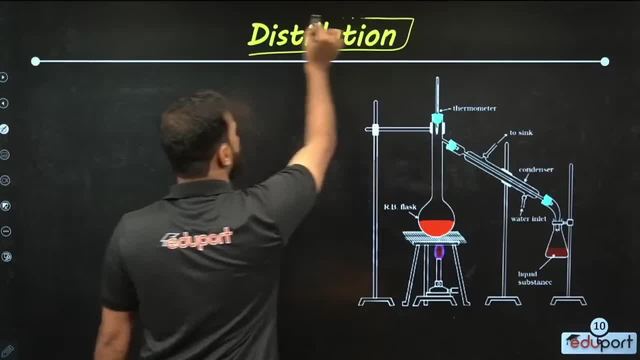 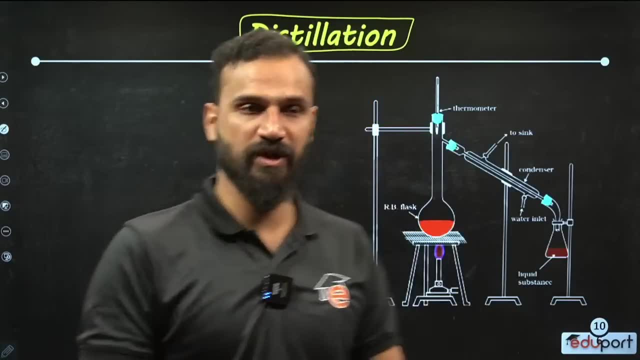 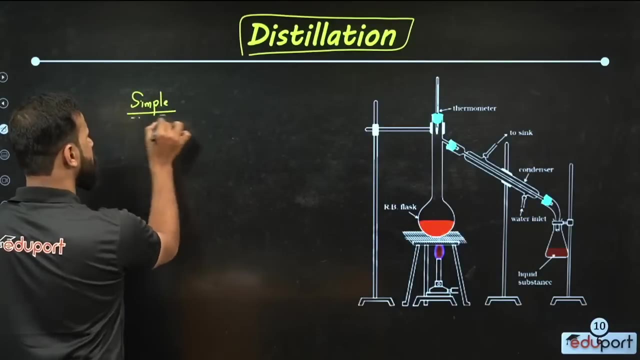 This is called crystallization. Next is distillation. There is simple distillation, fractional distillation, distillation under reduced pressure and steam distillation. What is simple distillation? When we think about when to do simple distillation, there is a big difference. 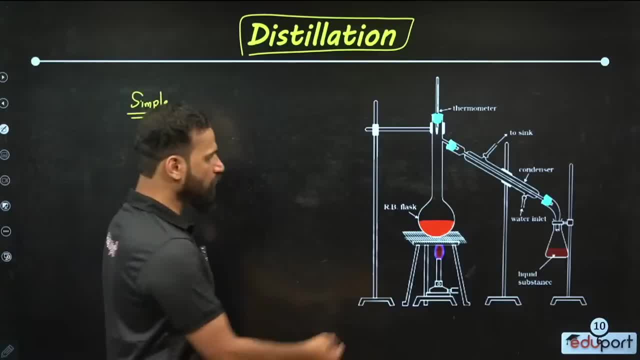 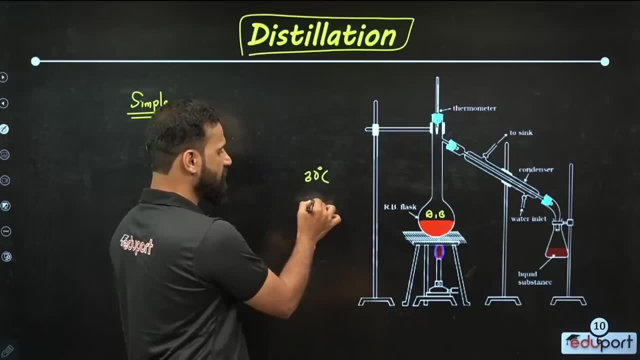 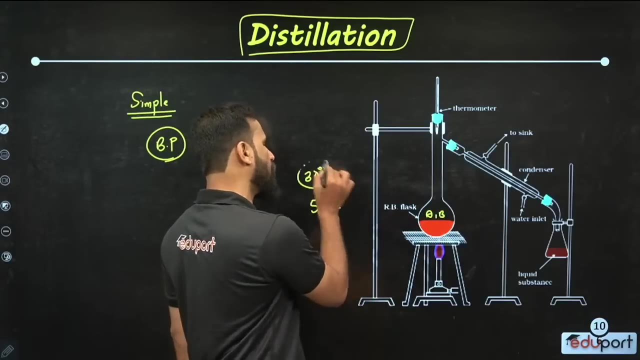 in the boiling point of the components. There is a component called A and a component called B. The boiling point of A is 30°C and that of B is 55°C. If there is a big boiling point difference between the two, what can we do? 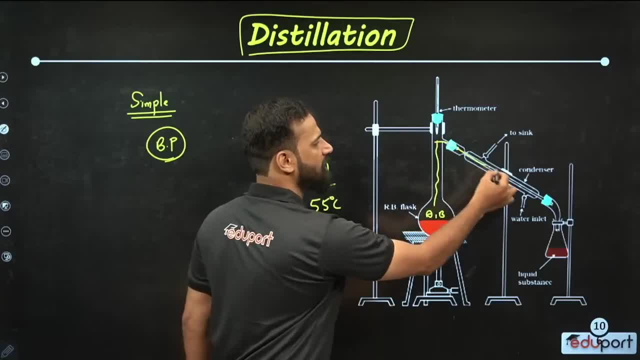 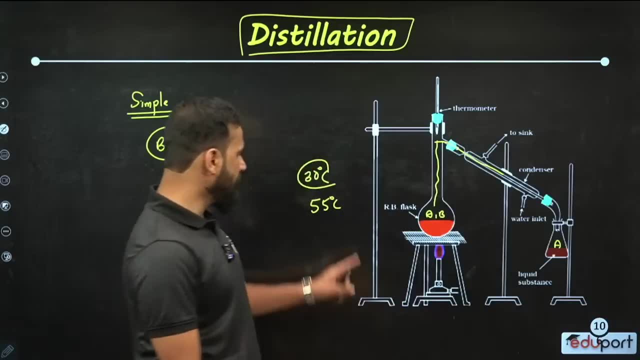 If the small boiling point is applied here, it will go deeper, It will condense in the condenser and we can collect it. So if the boiling point of A is less, we will get A there. If the boiling point of A is less, 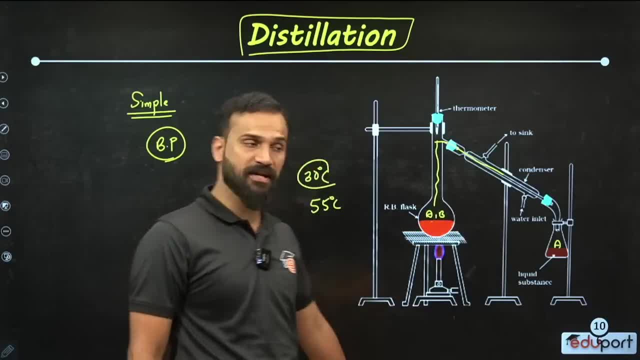 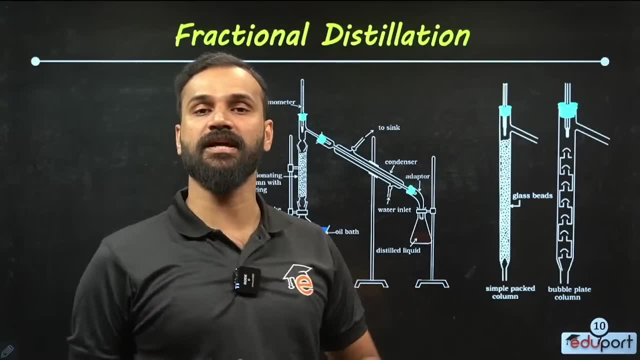 we will not get A there, So who will be in the RB flask? B will be there. This is how simple distillation is separated. Next is fractional distillation. The specialty of fractional distillation is that if there is no big difference, 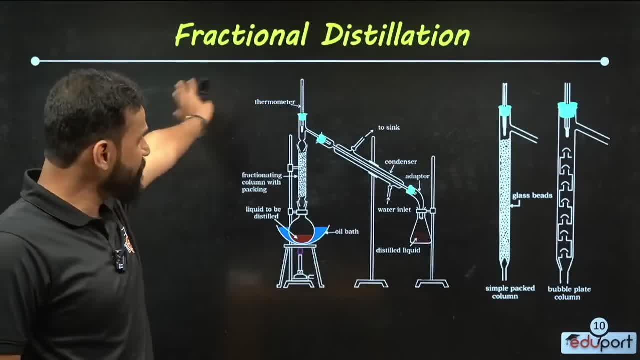 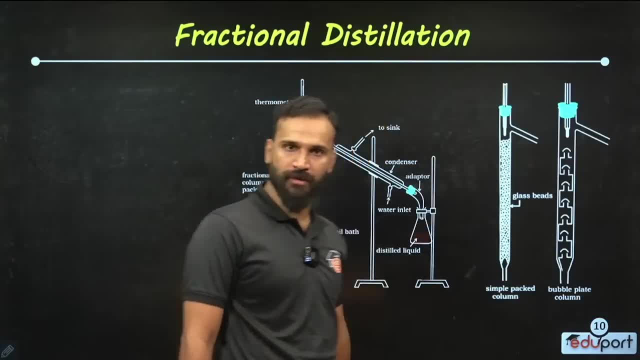 in the boiling point of the components. it is called fractional distillation. To do fractional distillation, we take the fractionating column. You can see it here. It is called the fractionating column. We use that to do distillation- Fractional distillation. 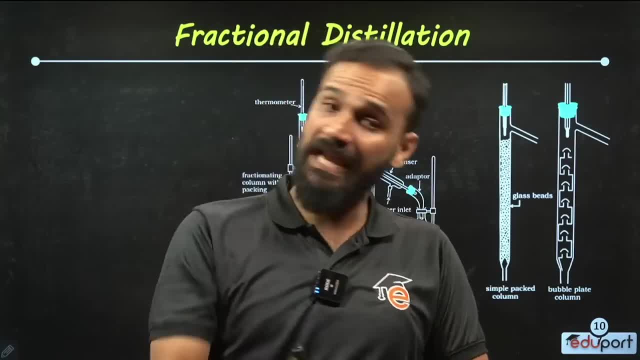 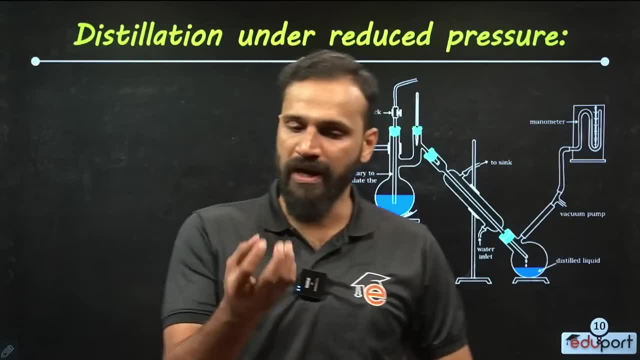 When fractional distillation is done. if there is no big difference in the boiling point of the components, it is called fractional distillation. Next is distillation under reduced pressure. We know that when we apply boiling point, if that component is boiled. 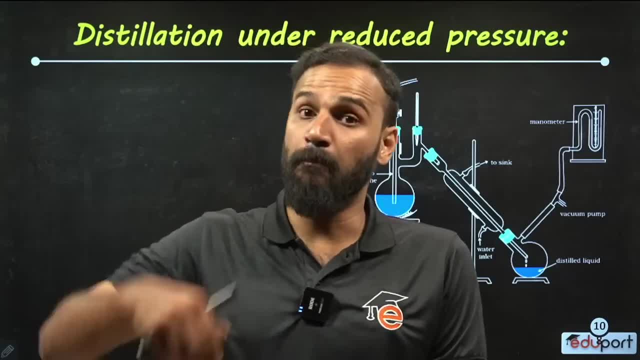 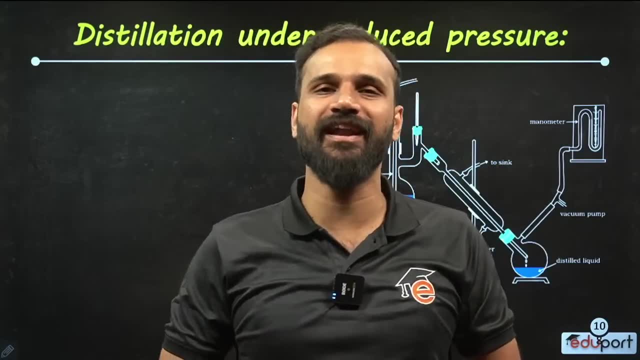 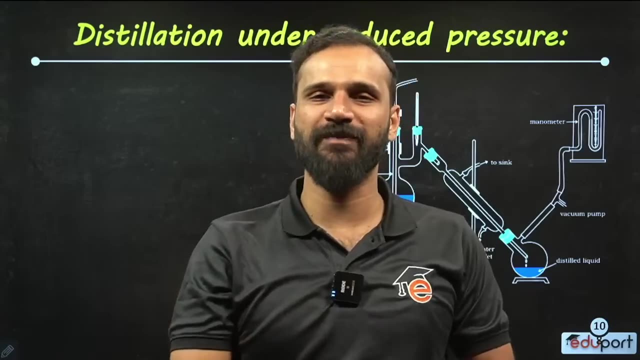 it will not turn into vapour. But some components decompose before boiling. If there are people who decompose before boiling, what will we do Before decomposing? we will reduce the boiling point and boil it. What is boiling point? It boils when the vapour pressure. 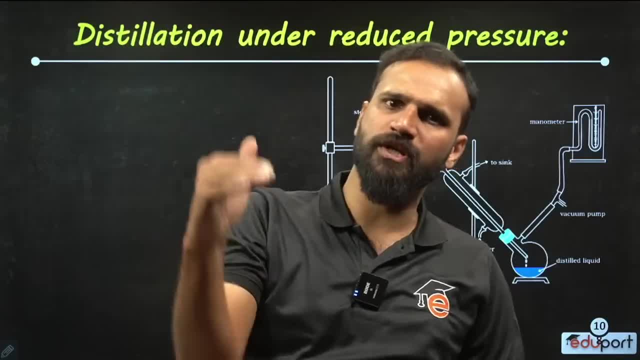 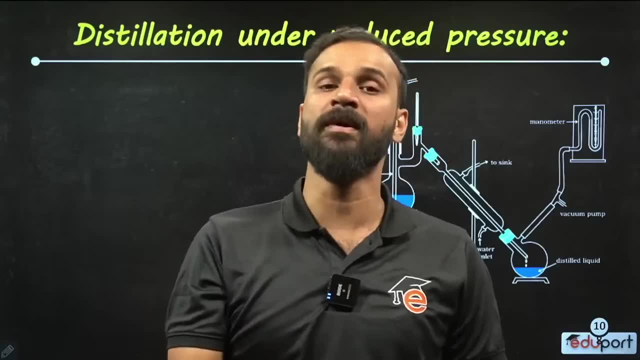 and atmospheric pressure are equal. If external pressure is reduced, the boiling point will be reduced To boil before decomposing. the boiling point will be reduced If the pressure is reduced. the boiling point will be reduced If external pressure is reduced. 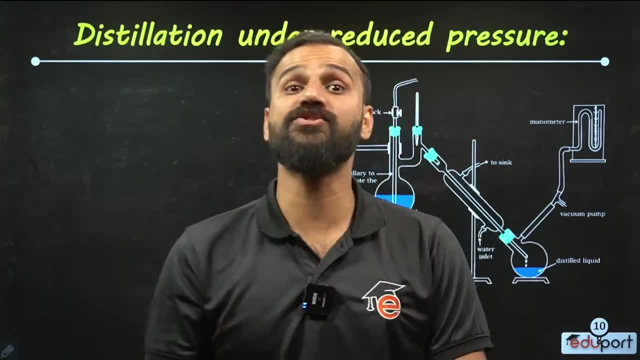 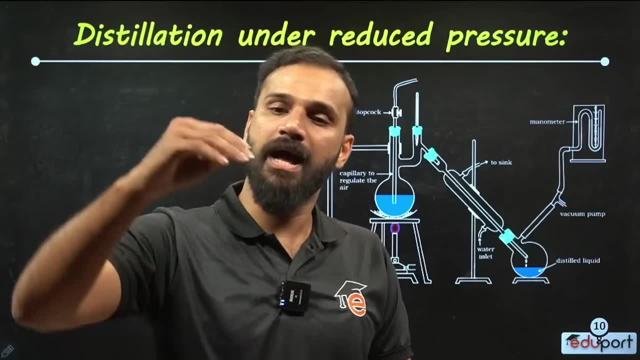 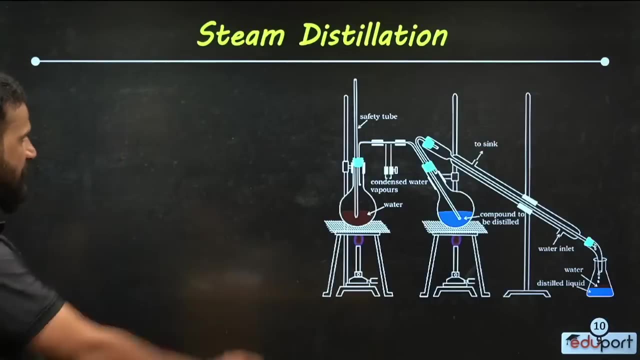 the boiling point will be reduced. Distillation is done under reduced pressure. Distillation under reduced pressure? Who do we mean by distillation under reduced pressure? It is the compounds that decompose before boiling, like glycerol. Remember this. Next is steam distillation. 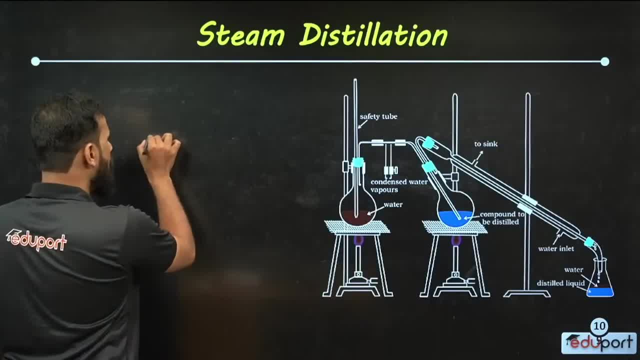 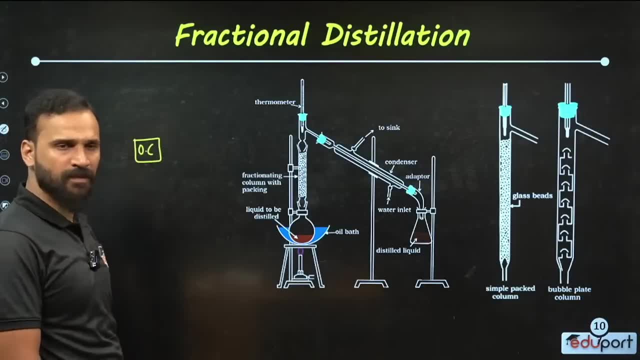 If we do steam distillation, there are two conditions. One is the organic compound. Who is the organic compound? Who is the organic compound? What should it be? It should be immiscible in water. It should not be dissolved in water. 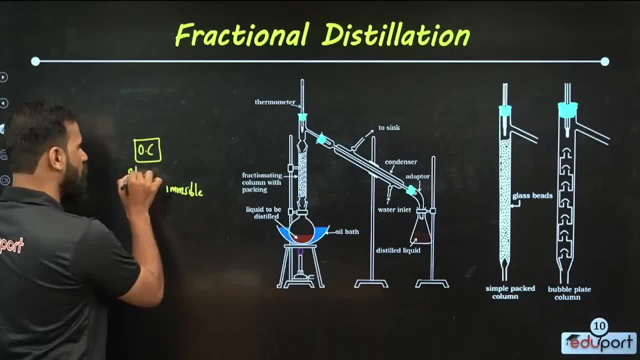 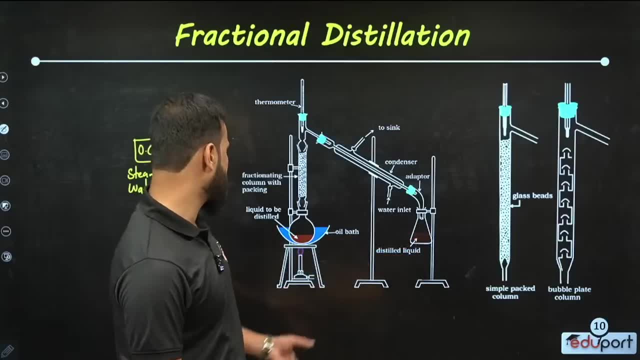 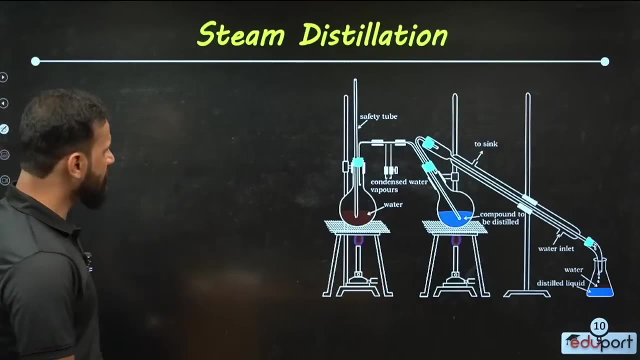 It should be immiscible. Moreover, the organic compound should be steam volatile. What should it be? It should be steam volatile. So to our organic compound. sorry, this is fractional distillation. steam distillation means that our organic compound 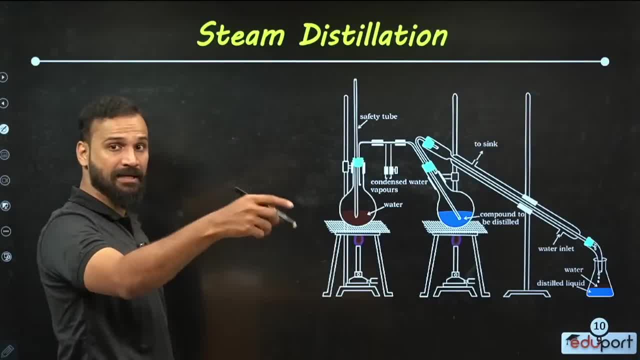 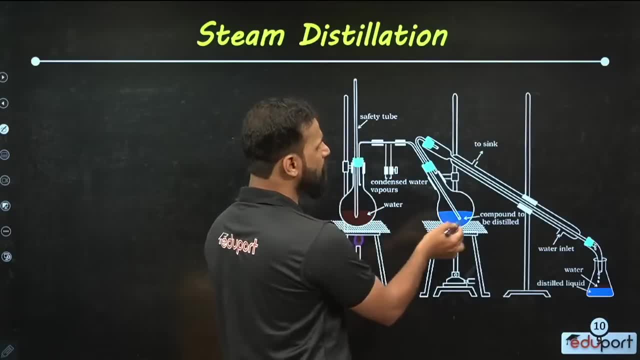 should be steam volatile. What are the other two? It should not be dissolved in water. So where is our organic compound? To that organic compound we pass steam. When steam is passed, only the organic compound vaporizes. Steam is already in vapor state. 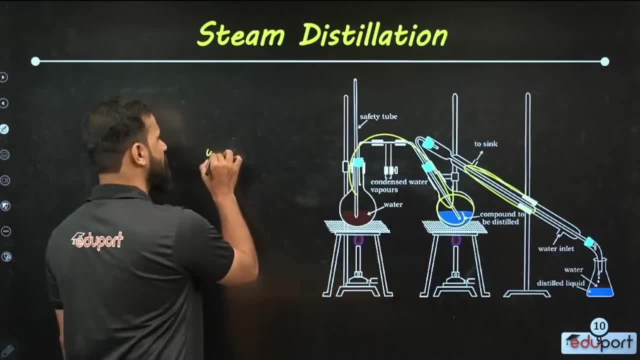 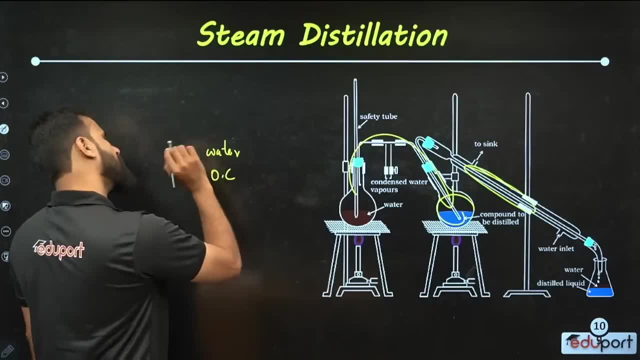 So who condenses in the condenser? If steam is condensed, it becomes water. Similarly, if organic compound is condensed, it will be in liquid state. But what is special here is that it is not dissolved. it is immiscible. 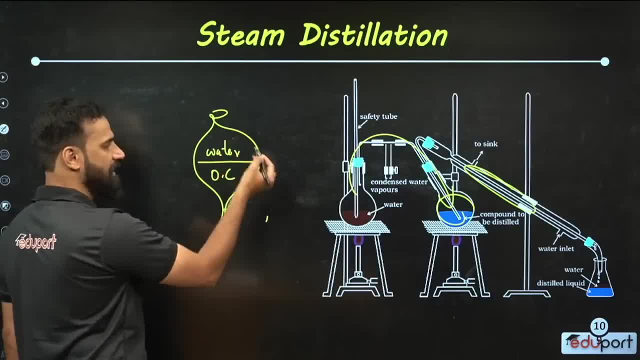 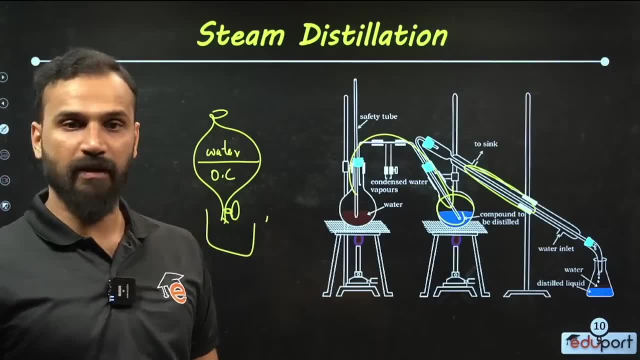 So we can separate using separating funnel. If we use separating funnel, they will be in two layers because they are not dissolved, So we can separate using separating funnel. This is steam distillation. You have to remember all these conditions. What are the conditions? 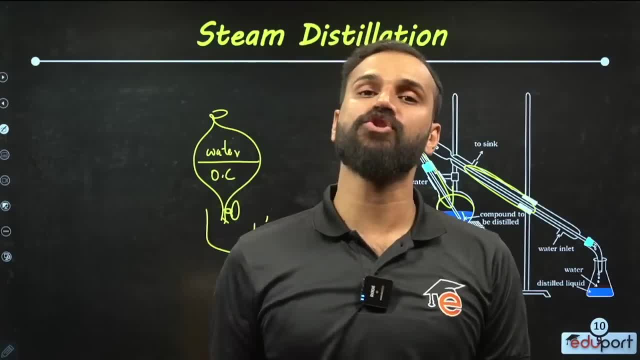 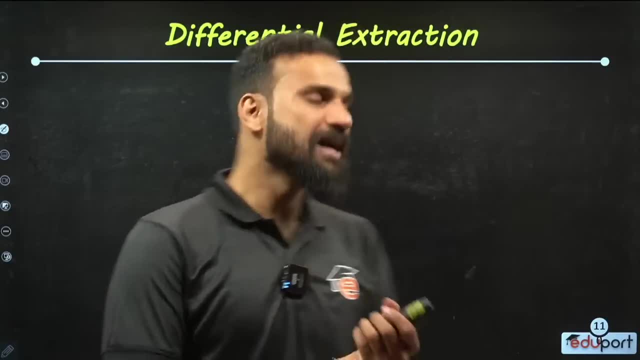 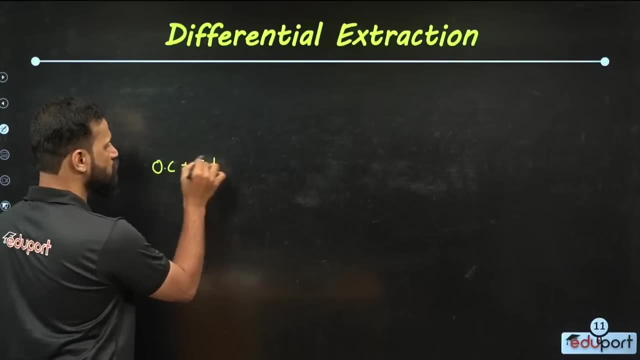 Organic compound should be steam volatile. Also, it should not be dissolved in water. Now, what is differential extraction? What is differential extraction? Differential extraction means there is a condition here. also, Do you know what it is? Our organic compound is used in solution state. 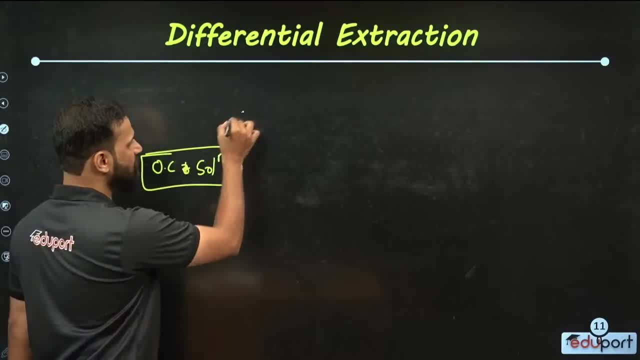 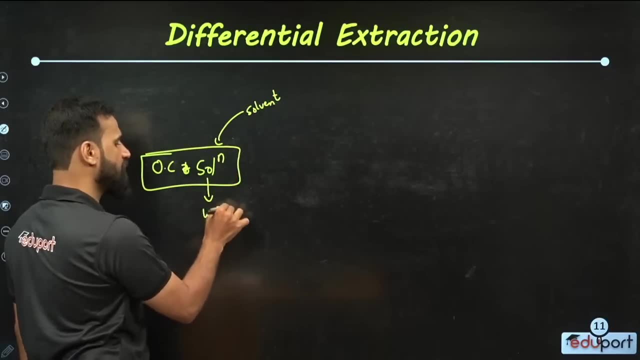 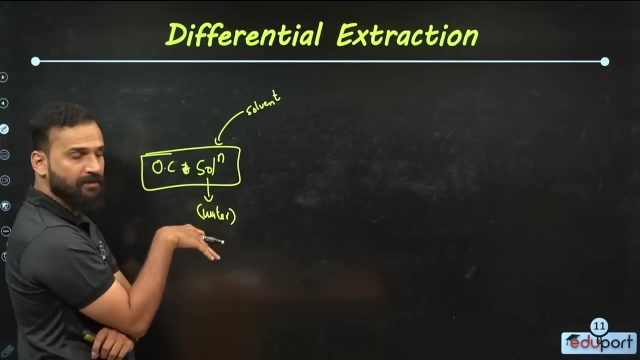 For that we have to add a solvent. For that we have to add a solvent. The solution already here has water in it. Solvent is water, So we are adding another solvent. The solvent we are adding is the organic solution. 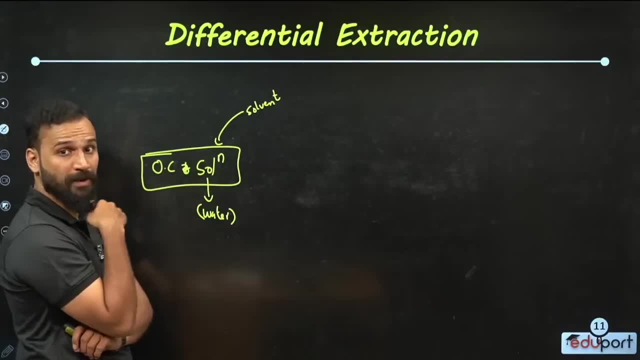 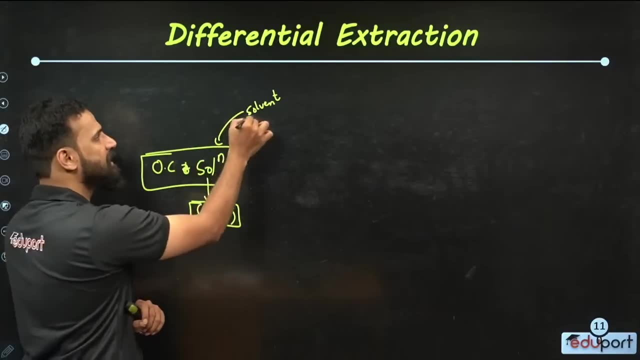 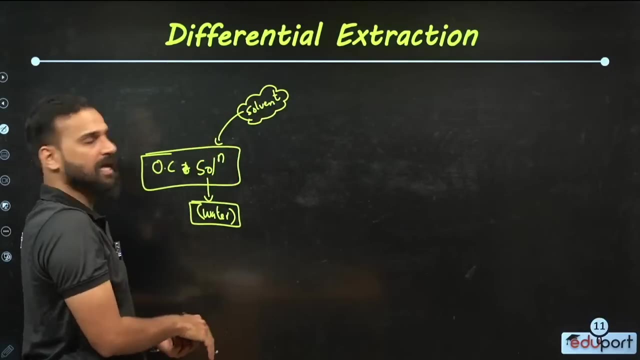 in the solvent. So the organic compound should be more soluble, That is, it is already dissolved in water. The solvent we are adding should be dissolved in the solvent. So it is already dissolved in water. But when the solvent comes, 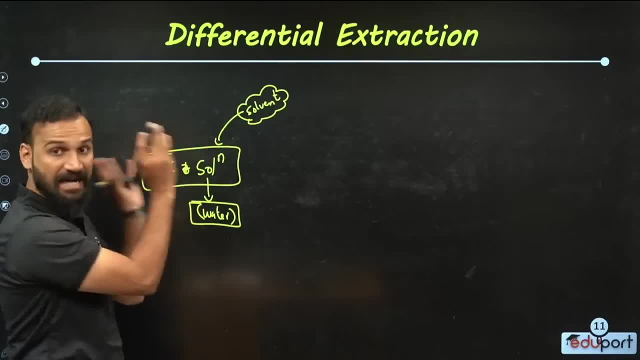 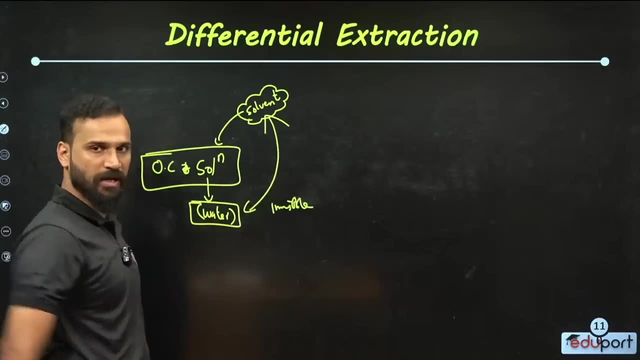 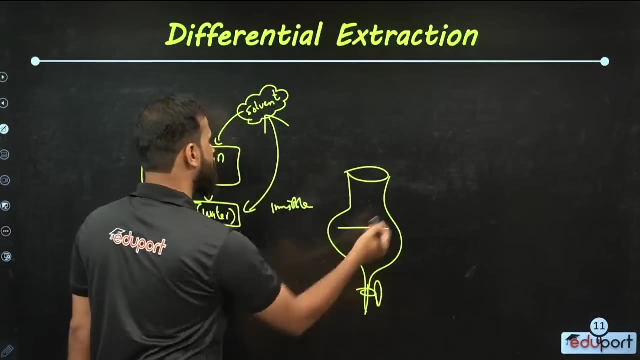 the organic compound should be more soluble. That is the condition here. Along with that, this solvent and this water should be immiscible. We can use separate and funnel. So what happens? One layer contains water. In the next layer we have 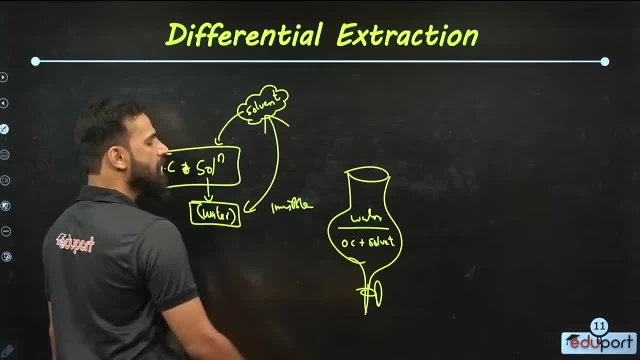 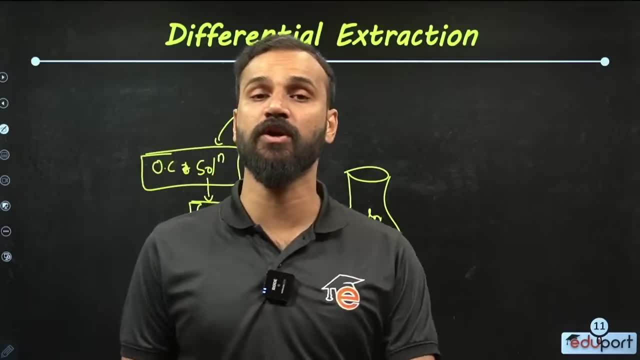 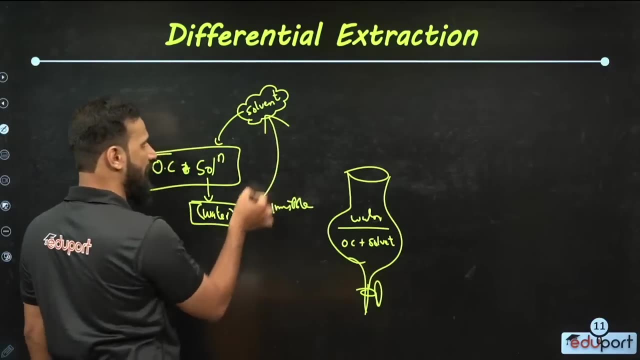 organic compound plus the solvent we have added. So we can separate the organic compound from water. But when we separate there will be solvent For that. we can separate it with any distillation method. This is called differential extraction. So the water and the 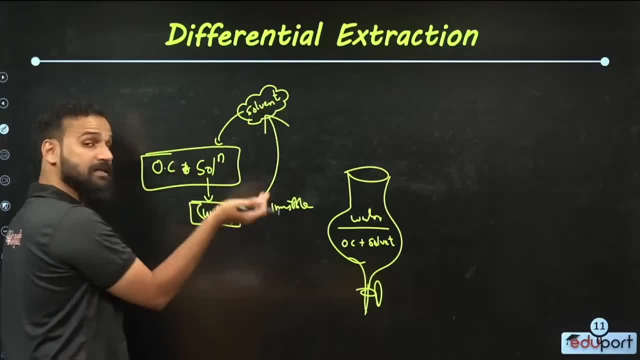 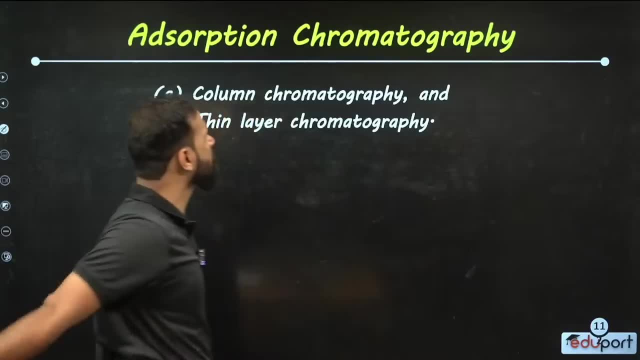 new solvent that we have added should be immiscible. That solvent should be dissolved in the water. That is the condition. Now look at chromatography. There are two types of chromatography. One is column chromatography. Sorry, it is adsorption chromatography. 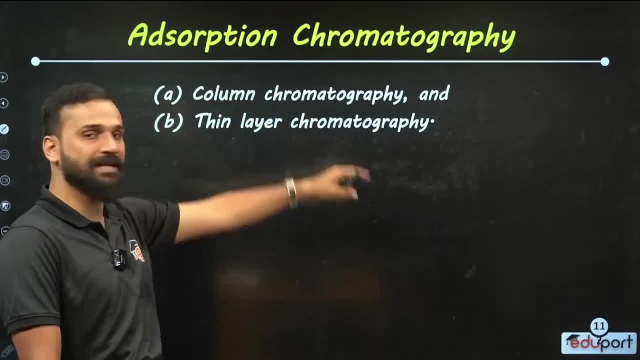 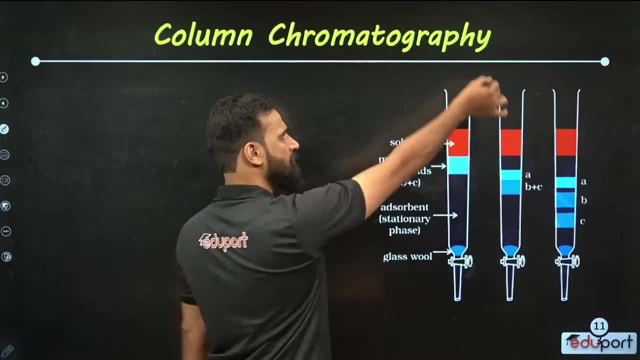 Two are partition chromatography. There are two types of adsorption chromatography. One is column chromatography and the other is thin layer chromatography. What is column chromatography? There is nothing. First, we take this column, We add silica gel to it. 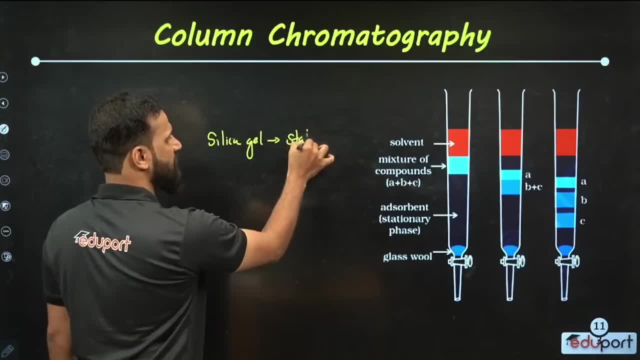 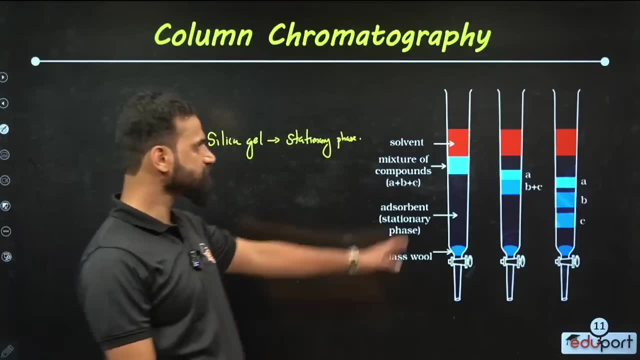 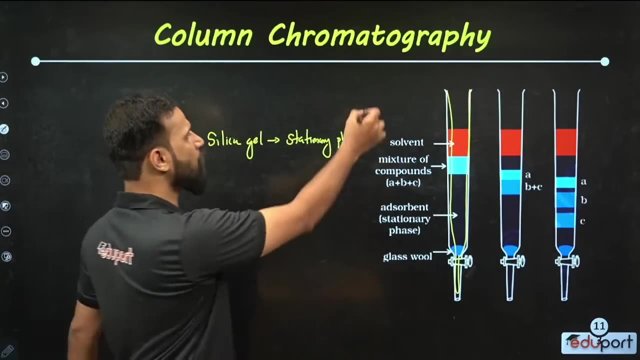 Silica gel acts as a stationary phase. What is it? It acts as a stationary phase. It acts as a stationary phase. It is placed on the side of the column. It is placed on the side of the column When we add organic compound to it. 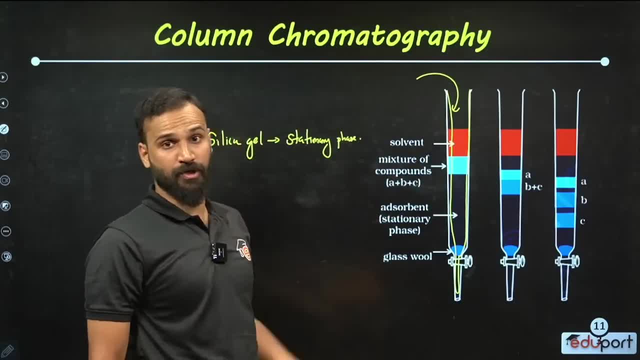 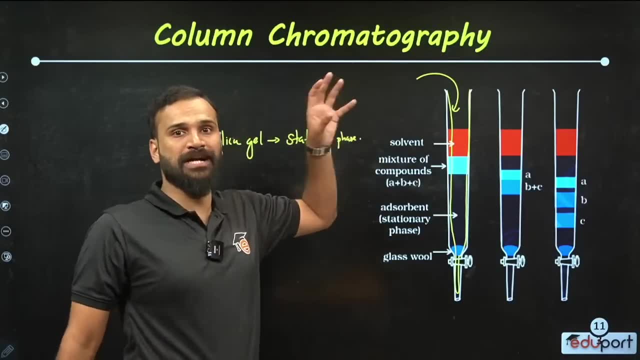 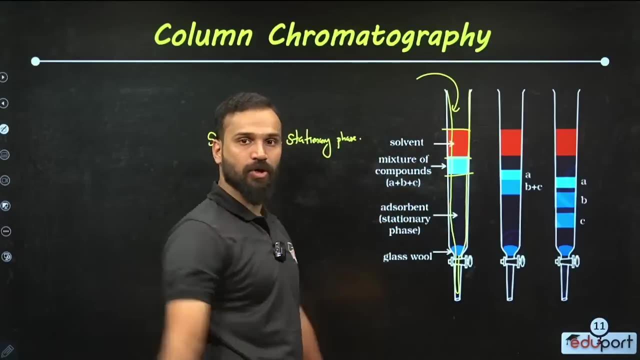 when we add organic compound to it. the organic compound has impurity. The adsorption capacity of organic compound and impurity will be different. The one with the highest adsorption capacity will absorb it first. The one with the lowest adsorption capacity will absorb it later. 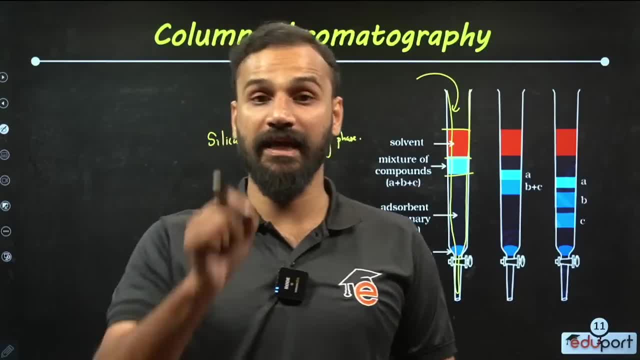 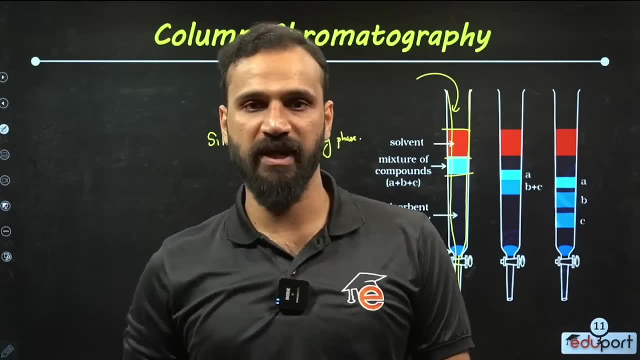 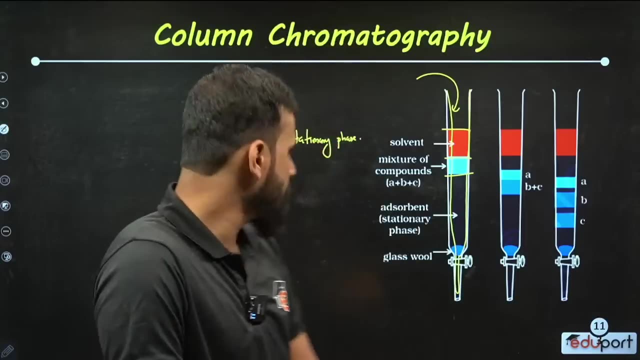 Organic compounds will be placed in different layers in the column. From there, whichever component you want, you can pour the solvent that dissolves only that and separate it. The solvent that is poured is in liquid state. We call it a mobile phase. 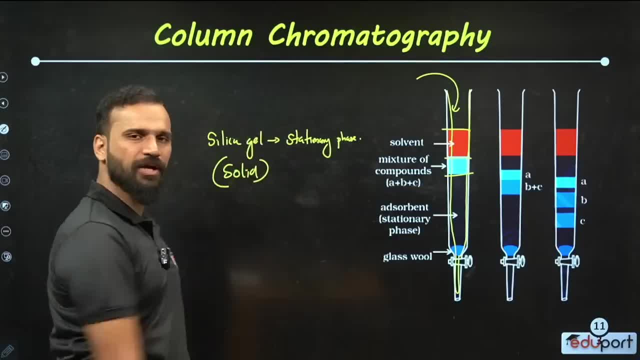 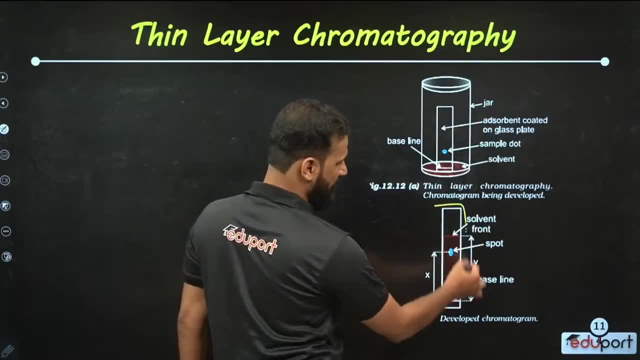 It is usually solid. In the mobile phase it is usually liquid. That is how we separate it. Now, what is the Thiller chromatography? This is a plate of Thiller chromatography. After dipping it in silica gel, we can spot the organic compound. 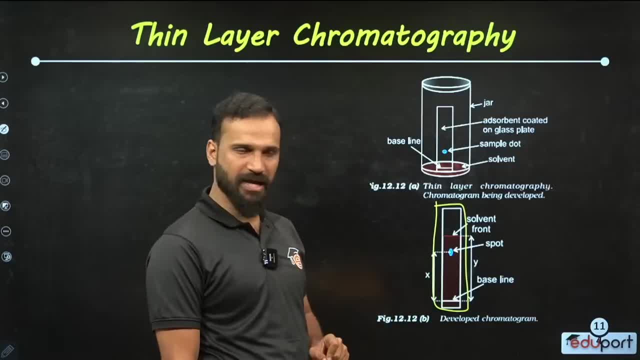 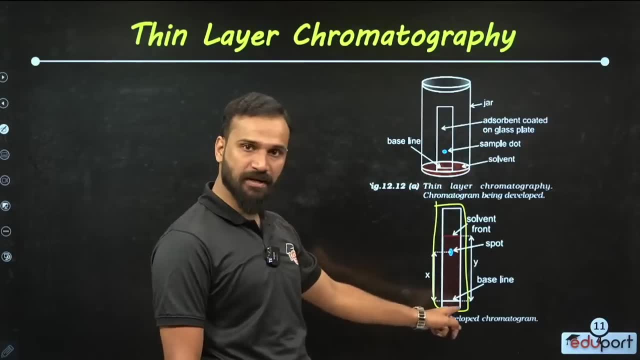 containing impurity in it. Then we move it to a container. There is a solvent in that container. That solvent acts as a mobile phase. The silica gel coated in this plate acts as a stationary When the plate is dipped in the solvent. 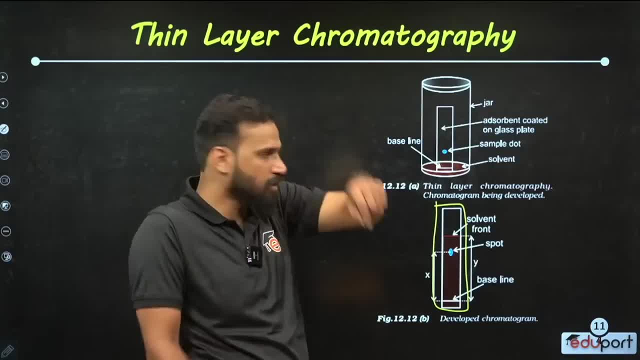 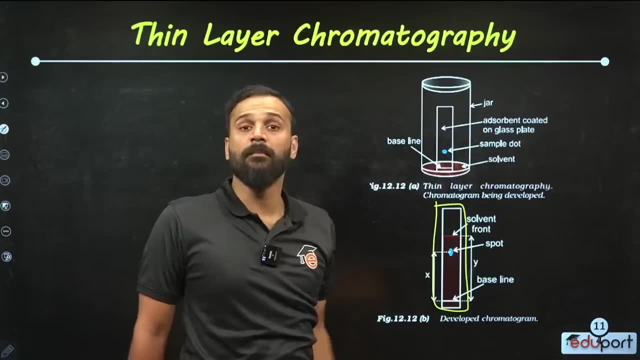 the paper is dipped in the water and the water comes in. like this, The solvent comes on top of it. As the solvent comes on top of it, the organic compound and impurity will come. But since the adsorption capacity of both people is different, 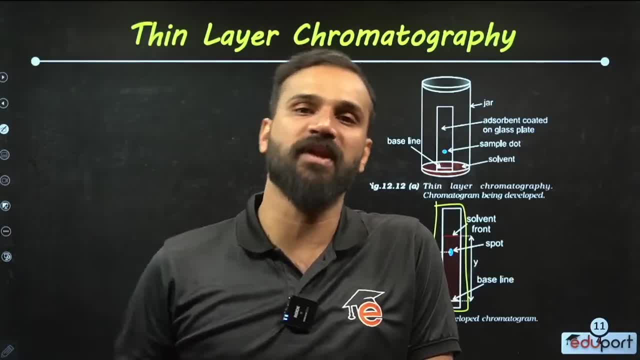 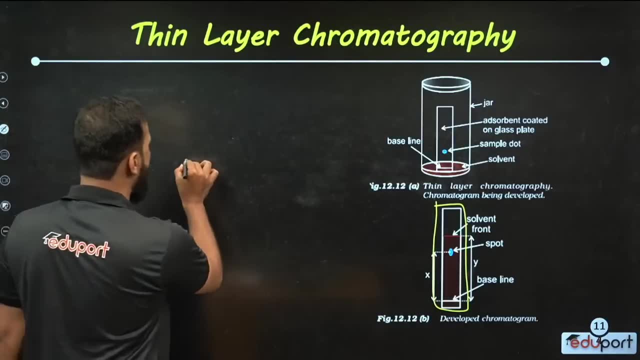 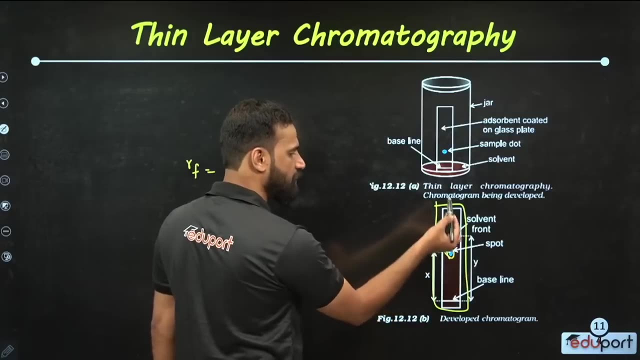 both come at a different level. That is how we can separate the components. This method is called Thiller chromatography. In Thiller chromatography we see the Rf value. the retention factor, That is, the organic compound, is here. 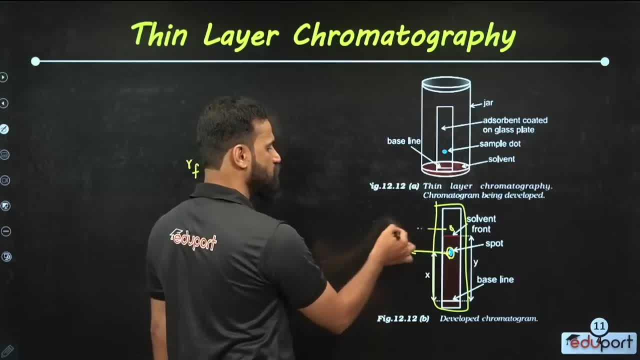 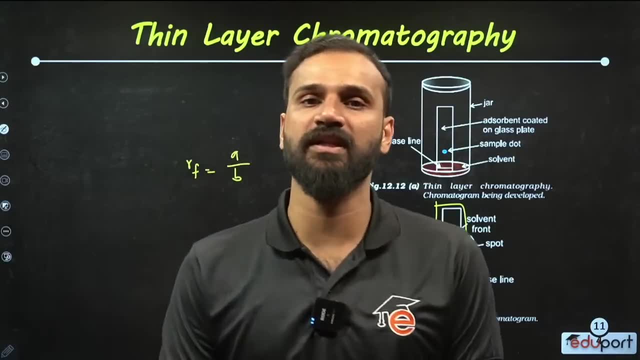 the solvent is here. If the distance travelled by the organic component is A and the distance travelled by the solvent is B, A by B becomes the retention factor. Some people ask what the retention factor is: Distance travelled by the component divided by distance travelled by the solvent. 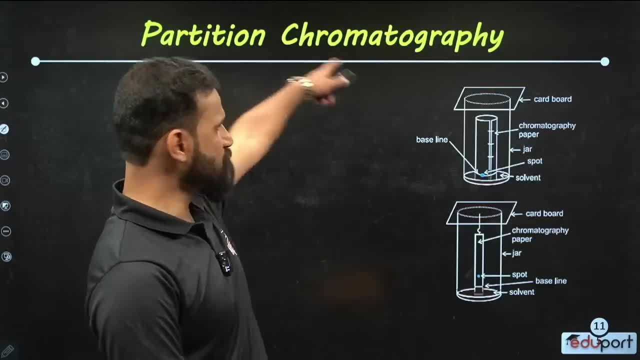 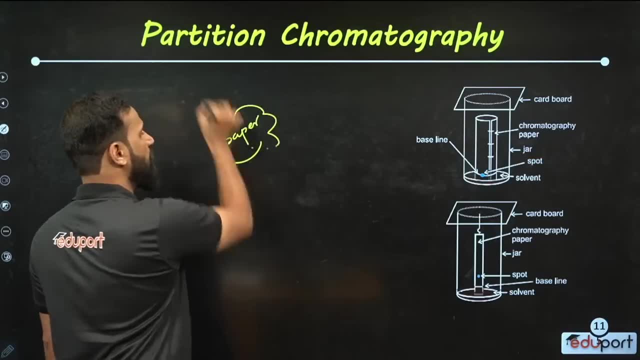 is the Rf value or the retention factor. The typical example of partition chromatography is paper chromatography. What is paper chromatography? The speciality of paper chromatography is that it is similar to Thiller chromatography, But the stationary phase is also liquid. 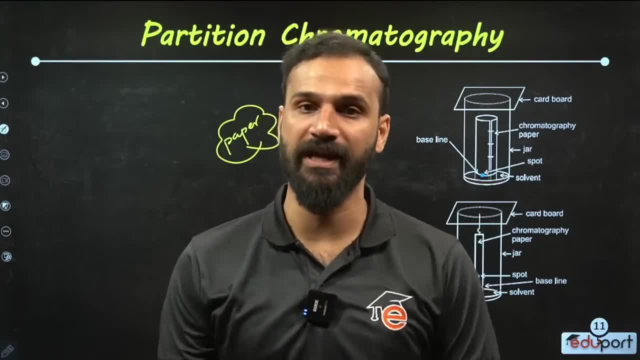 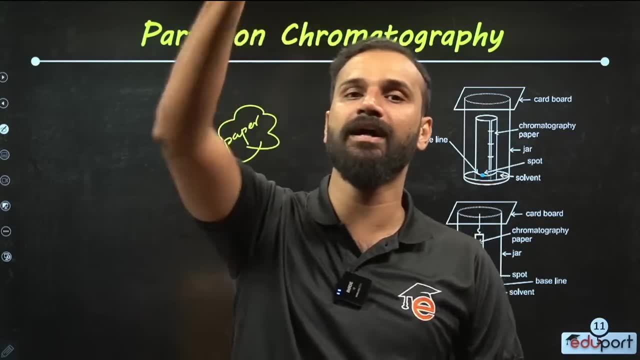 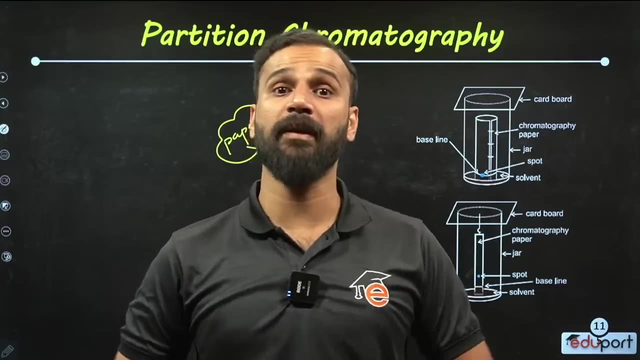 Similarly, the mobile phase is also liquid. It is done using a special type of paper. There are cavities in that paper. In those cavities the organic compounds are partitioned. Through that we can separate the organic compounds. That is called what Paper chromatography. 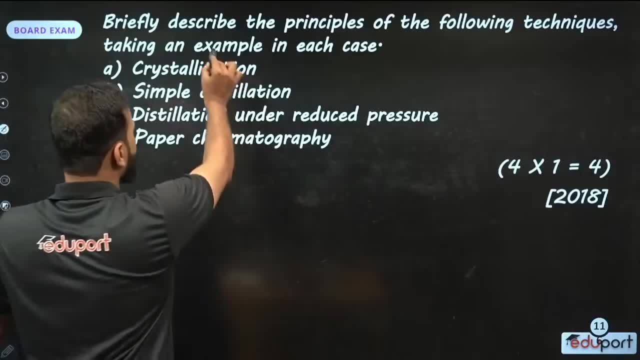 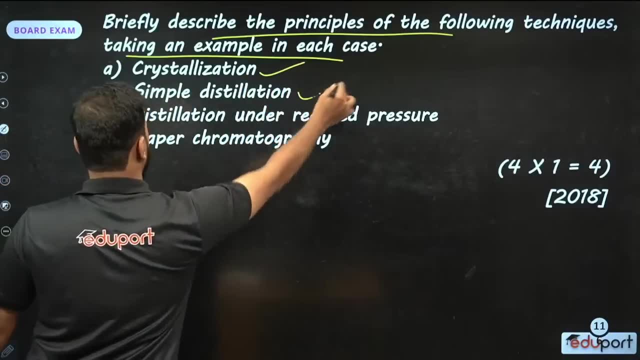 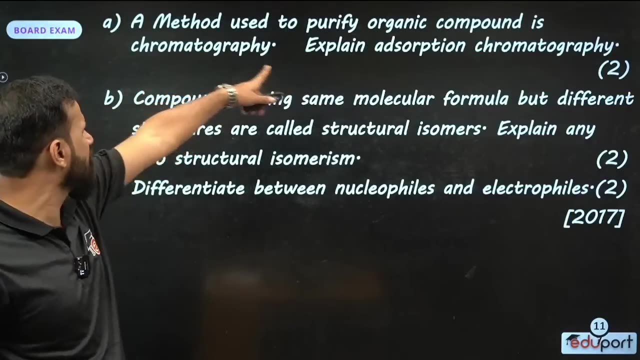 Just know this. Now look at the children. Briefly describe the principles of the following techniques, taking an example in each case: Crystallization, simple distillation, distillation under reduced pressure, paper chromatography- Just know all these- The method to purify organic compounds. 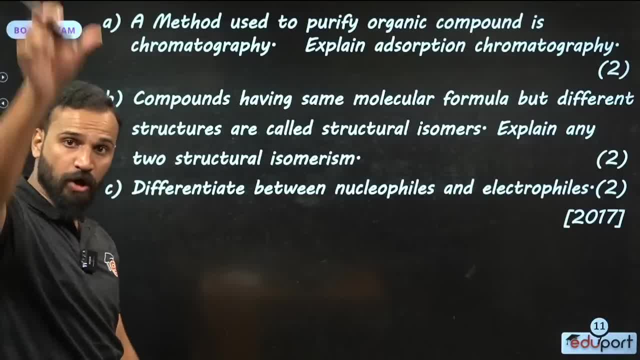 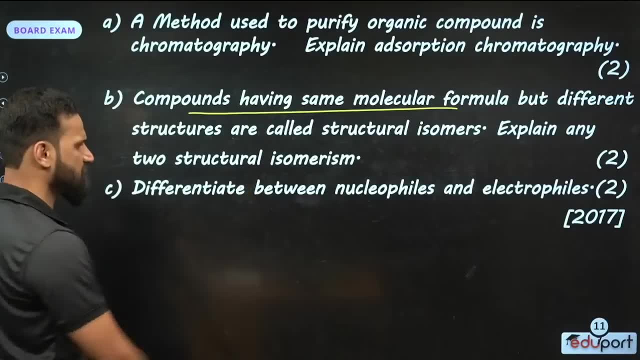 is chromatography? Explain adsorption chromatography. In adsorption chromatography, column chromatography is explained. Similarly Thiller chromatography is explained. Compounds having same molecular formula but difference in isomer is known. Difference between nucleophile and electrophile is known. 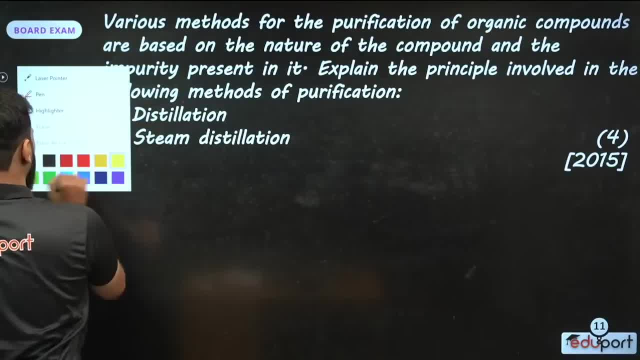 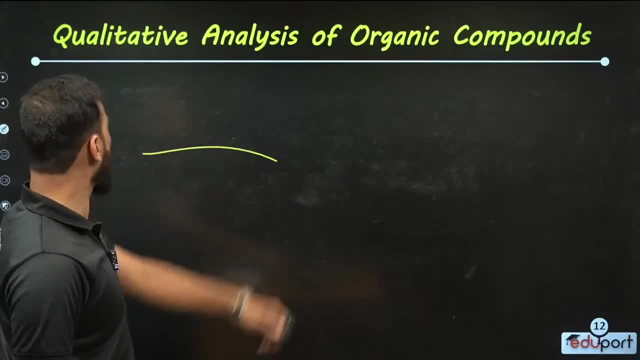 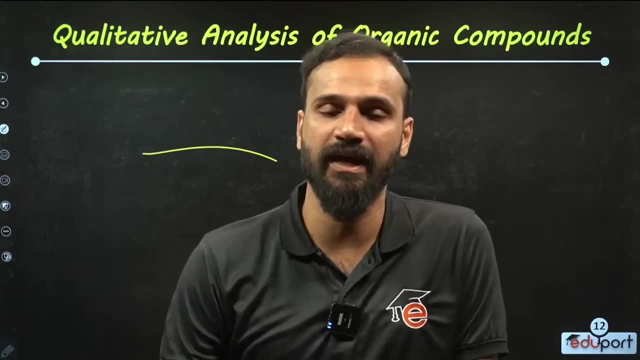 Okay, Distillation and steam distillation is known. Now, what is? what is resonance effect? What we have discussed earlier? Now qualitative analysis, The method to find the elements in an organic compound. Is there carbon in it? Is there hydrogen in it? 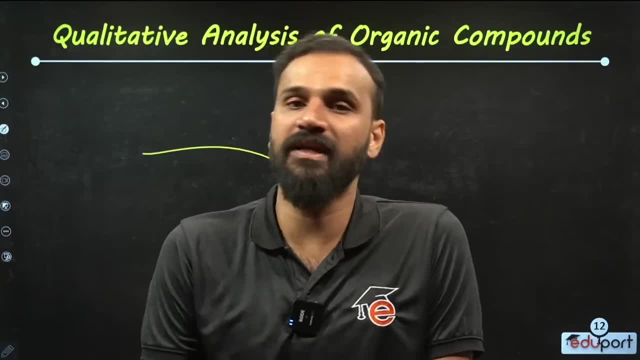 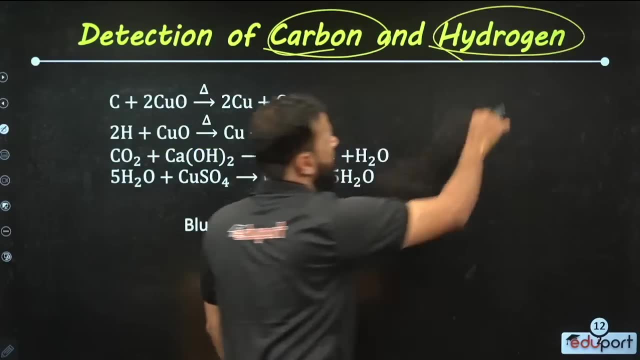 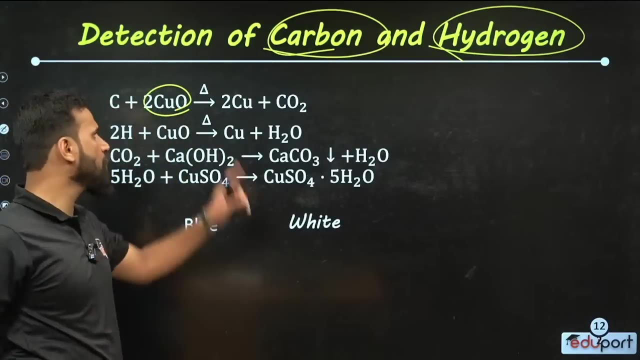 Is there nitrogen in it? This method is called qualitative analysis. In that qualitative analysis, detection of carbon and hydrogen is very important. Nothing else In the organic compound given to you, COO- copper oxide, is heated. When copper oxide is heated, 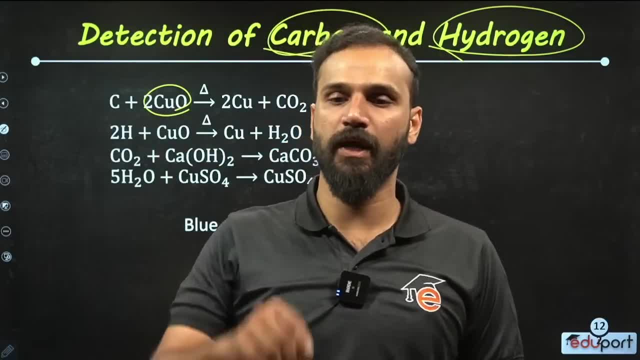 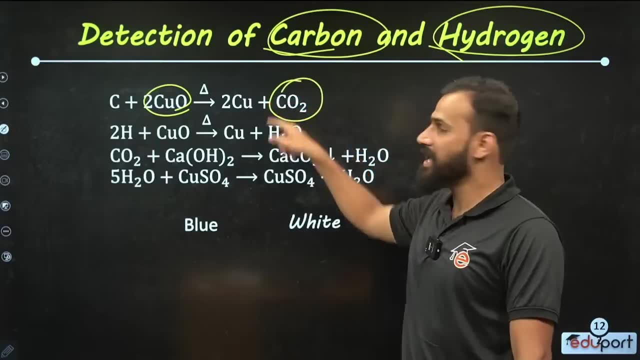 if there is carbon in it, it will turn into carbon dioxide. If there is hydrogen in it, it will turn into water. To know if there is carbon dioxide in it, add some lime water or calcium hydroxide to it. When you add hydroxide, 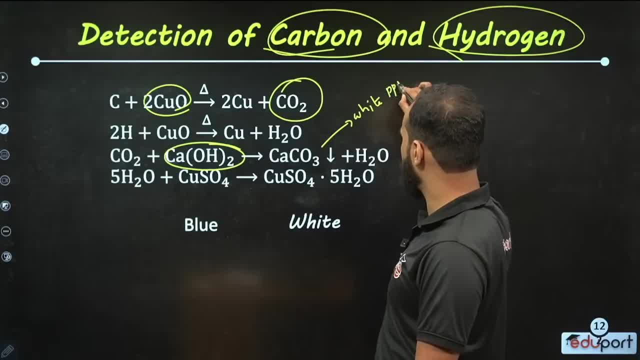 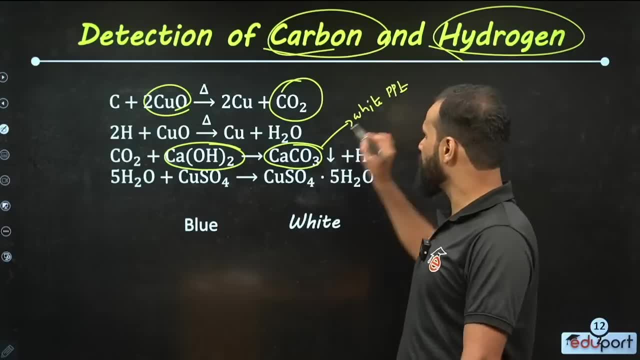 see if you get white precipitate. To get white precipitate, calcium hydroxide is combined with carbon dioxide and turns into calcium carbonate. If you get white precipitate, you can say that there is carbon in it. Now do you know if there is carbon in it? 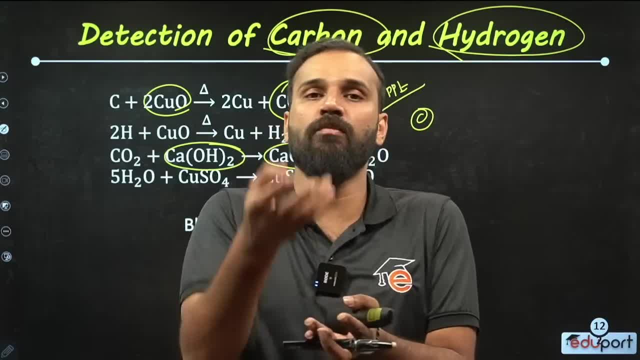 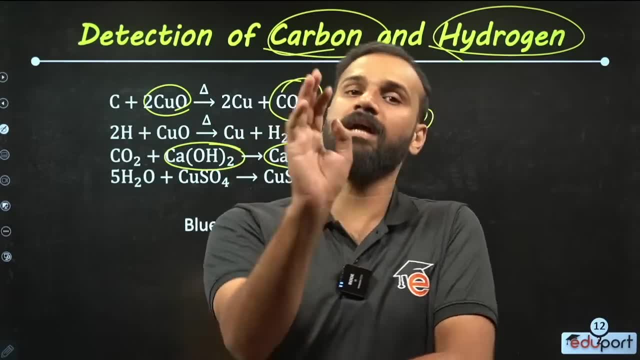 When COO oxide is heated in the given organic compound, it will turn into carbon dioxide. To confirm, if you get white precipitate when lime water is added to it, you can say that there is carbon in it. Now, if there is hydrogen? 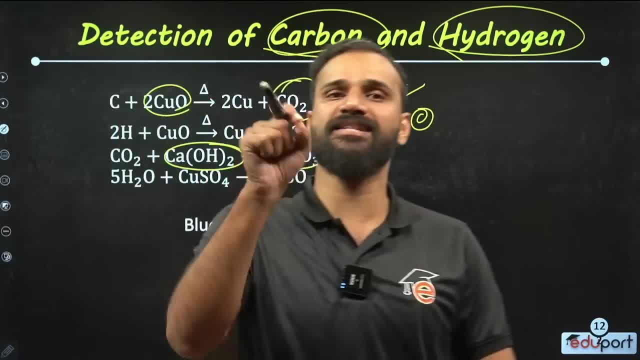 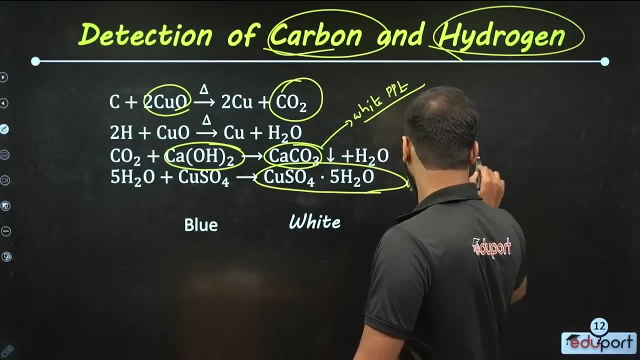 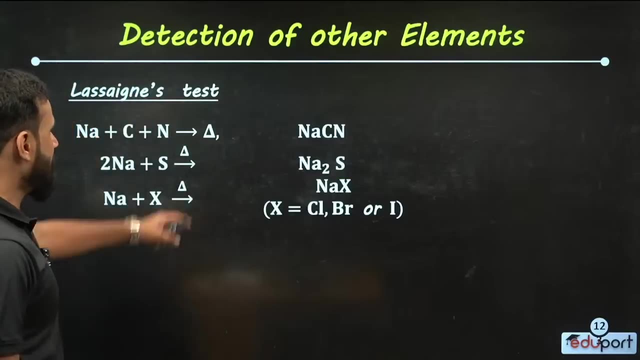 it will turn into water. Add anhydrous copper sulphate to that water. When copper sulphate is added, if you get blue colour, you can say that there is hydrogen in it. This is how we understand carbon and hydrogen. Now to find. 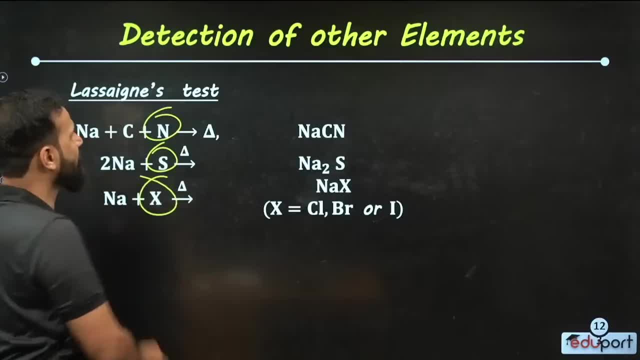 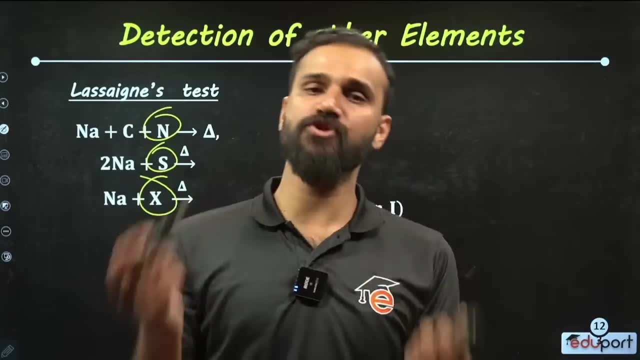 nitrogen and sulphur and halogen. we will do a lecithin test. To do a lecithin test, we need to make a sodium fusion extract. How to make a sodium fusion extract: Take a fusion tube and add organic compound and sodium metal. 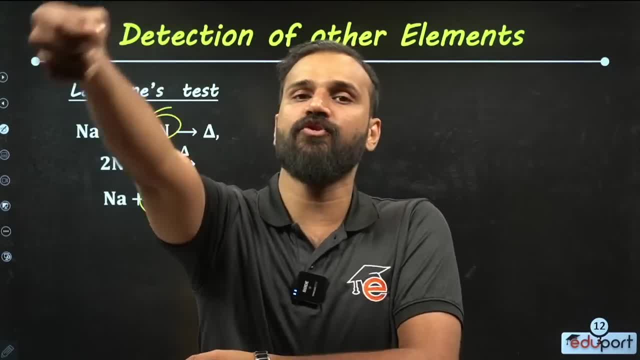 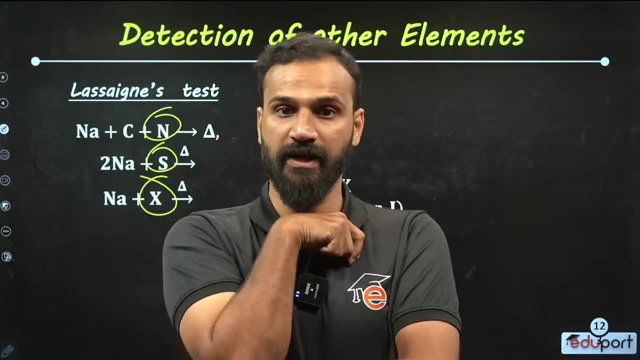 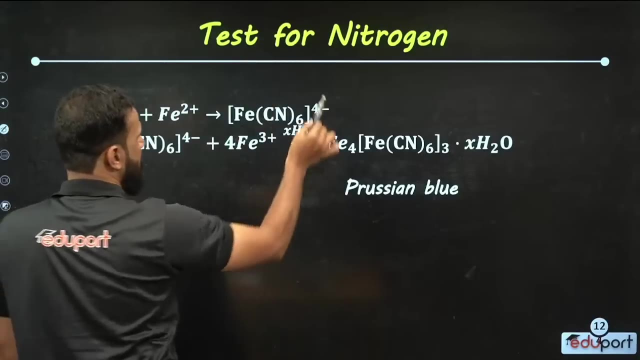 to it and heat it well. Add the heated substance to distilled water and filter it. That filter is called sodium fusion extract. By taking that sodium fusion extract we are doing lecithin test. How to do hydrogen test? Take a little from: 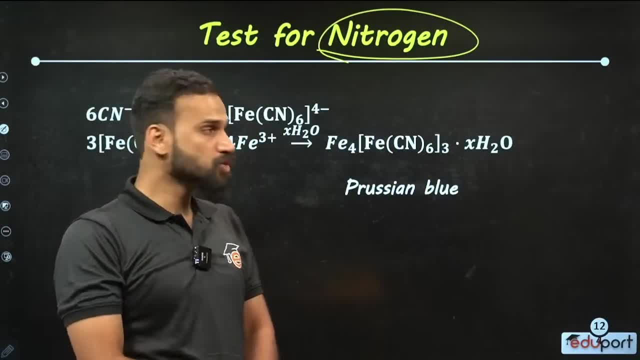 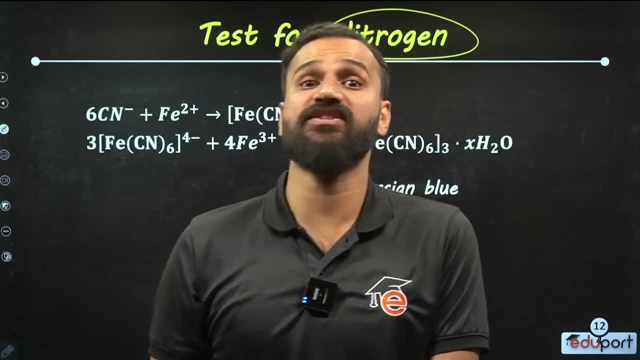 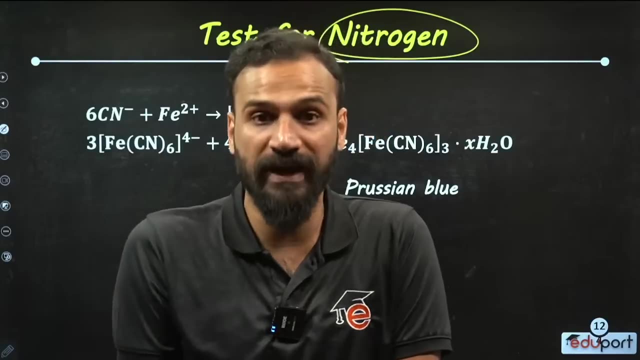 the sodium fusion extract we have made. Take a little from sodium fusion extract. Take a little from sodium fusion extract and add freshly prepared ferrous sulphate to it. After boiling the freshly prepared ferrous sulphate when few drops of concentrated sulphuric acid is added. 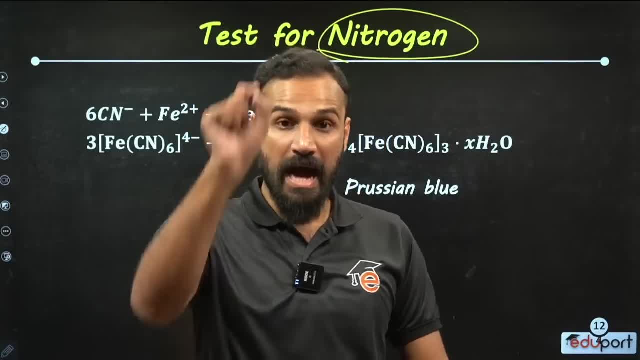 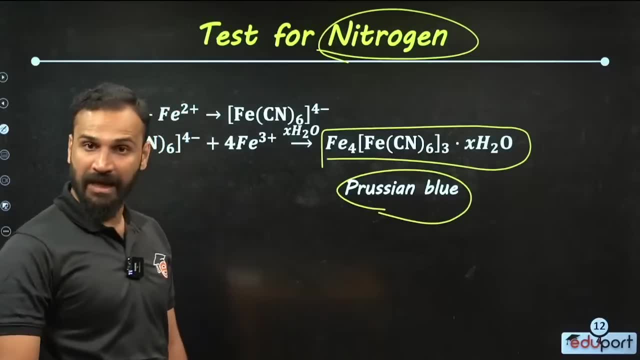 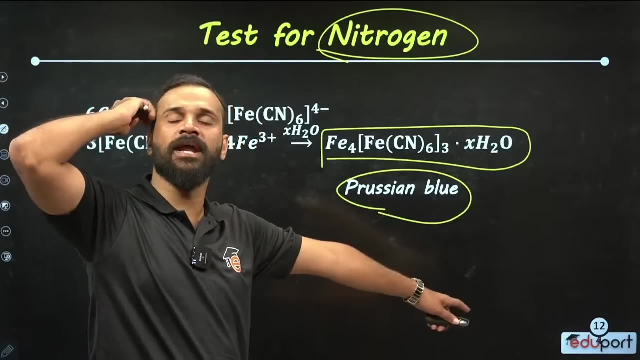 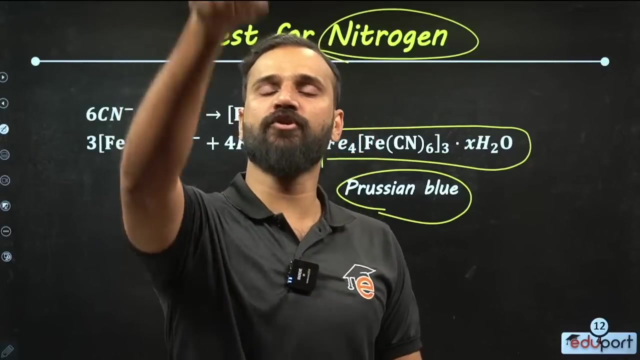 if you get any blue colour or green colour, it indicates the presence of nitrogen. We call that blue colour, Prussian blue. We call that blue colour nitrogen. This is the presence of nitrogen. Take a little sodium fusion extract and add freshly prepared ferrous sulphate to it. 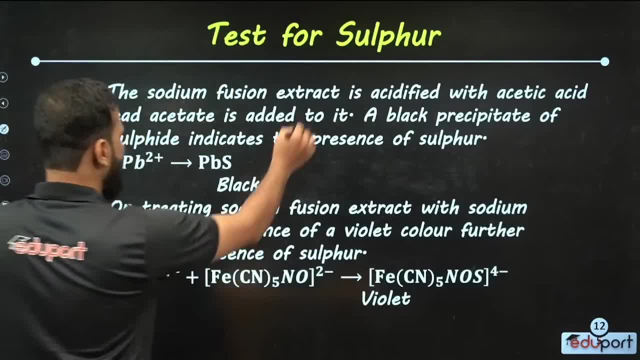 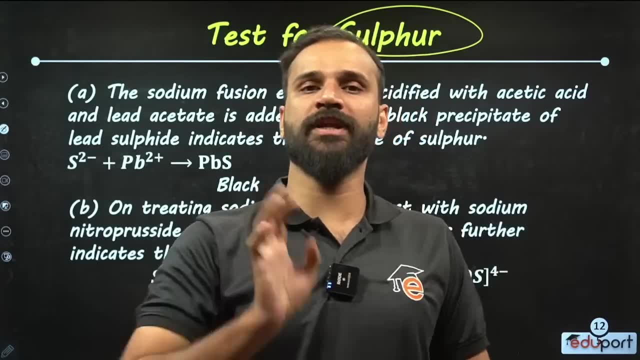 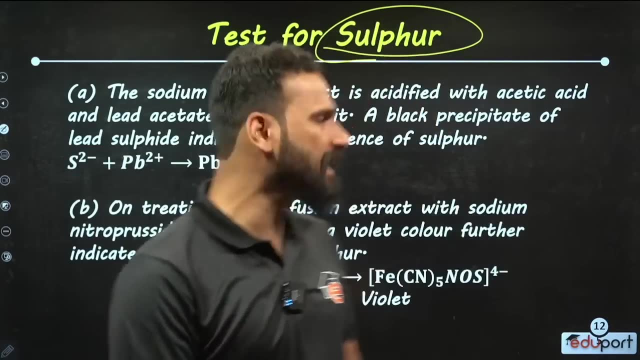 When few drops of sulphuric acid is added, you get the presence of nitrogen. Now, how do we identify the presence of sulphur? acidify it. When you do that, you should get black color. What is it? Acetic acid and lead acetate. 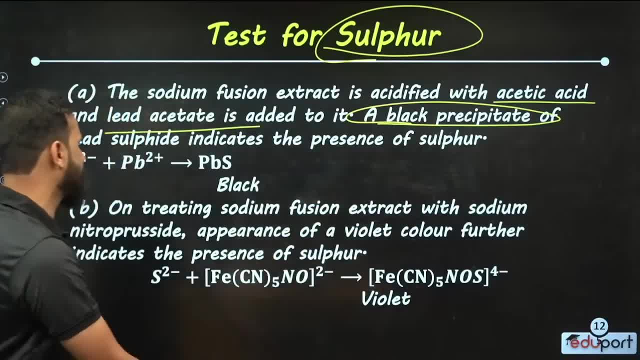 when added. if you get black precipitate, lead sulphide is black. If you get that black precipitate, you can say that it has sulphur. Otherwise, what do you have to do? Take sodium fusion extract and treat it as sodium nitroprusside. 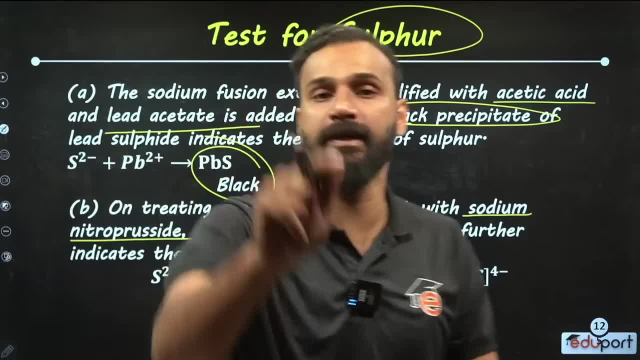 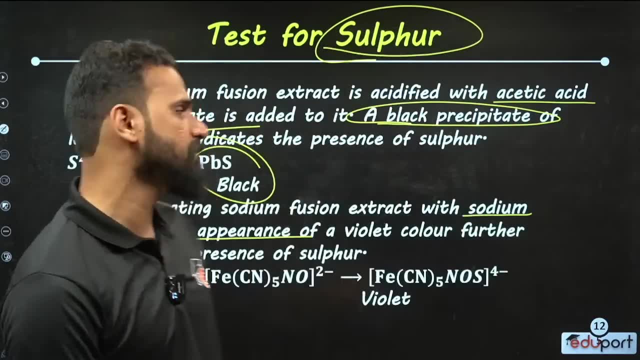 When treated as sodium nitroprusside. if you get violet color, it indicates sulphur. What is it? Sodium nitro pursuade? when treated as sodium nitroprusside. if you get violet color, it also indicates sulphur. How do you indicate halogen now? 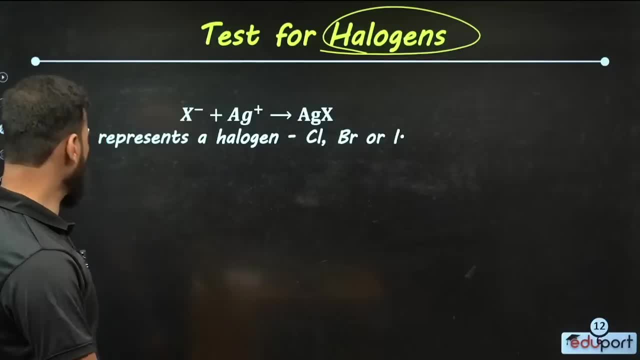 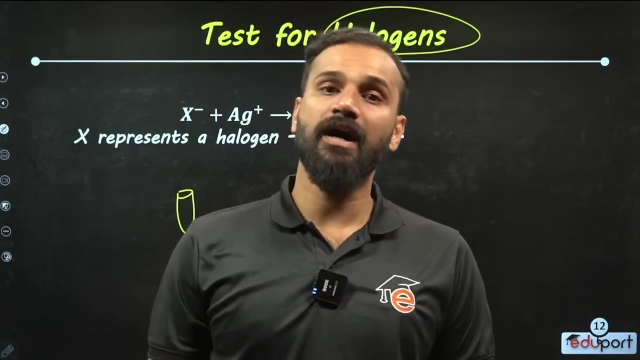 It is very, very important. It is very, very important. If you think about it. what do we have in our hands? Sodium fusion extract is there? Sodium fusion extract is there? What should we do in that sodium fusion extract? What to do? We can add nitric acid and acidify it. 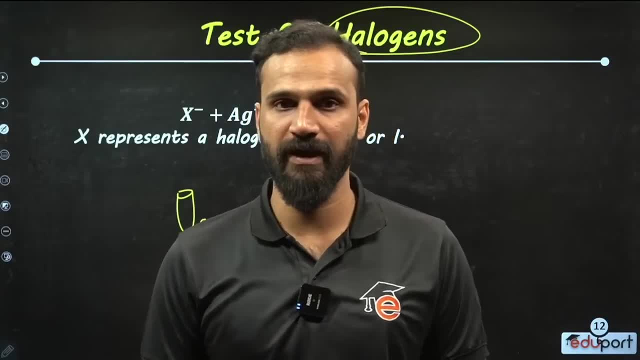 Then you can add some silver nitrate solution to it, And then you can add some silver nitrate solution to it, And then you can add some silver nitrate solution to it, And then, When we add it, we have to check the color we get. 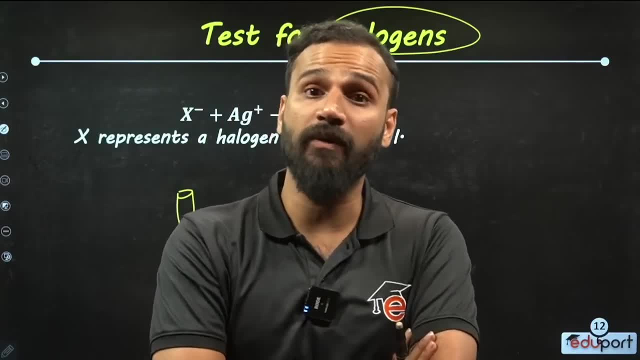 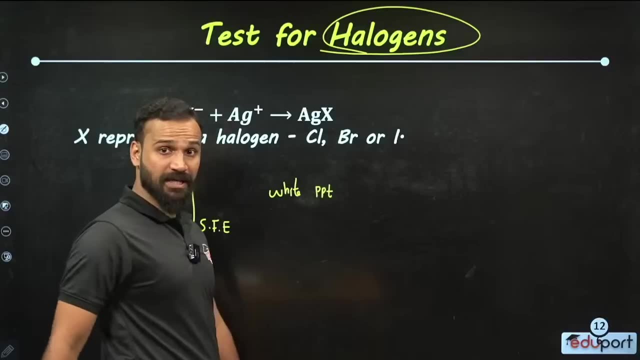 What color do we get there? Maybe we can get white precipitate there. What can we get? White precipitate, White precipitate. After adding nitric acid and acidification we can add silver nitrate. When silver nitrate is added, we can check. 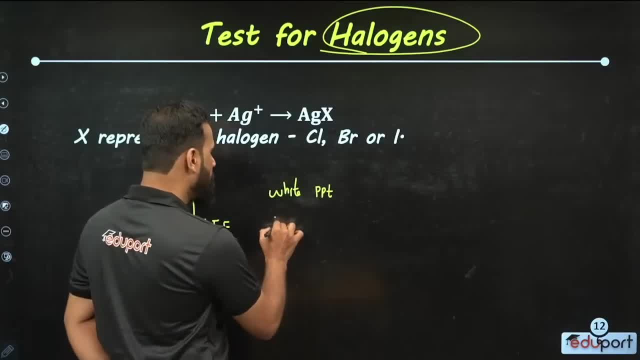 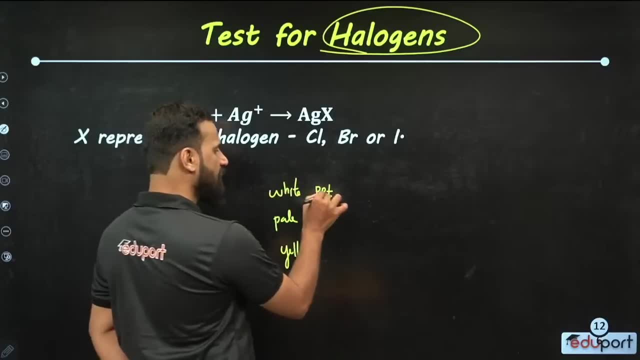 if we are getting white precipitate, Otherwise what can we get there? We can get pale yellow, Pale yellow color, We can get pale yellow. So you get white color. You add ammonium hydroxide to that white color, Then it dissolves. 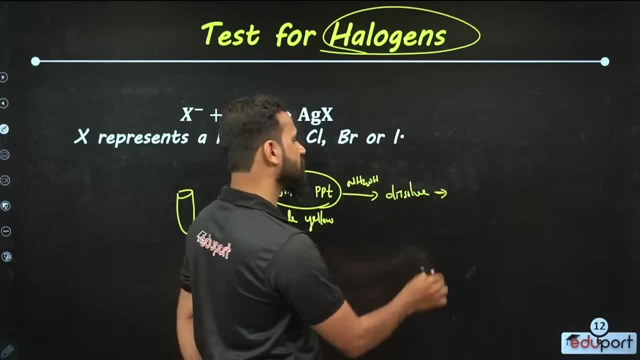 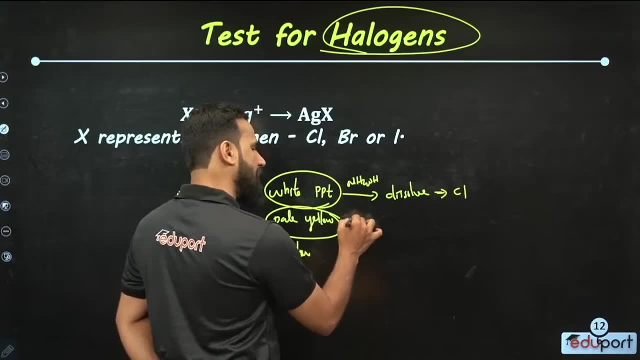 If it dissolves. don't wait even for a minute. What can you understand? You can understand that there is chlorine in it. Now you get pale yellow When ammonium hydroxide is added to it. it is partially soluble, Not completely soluble. 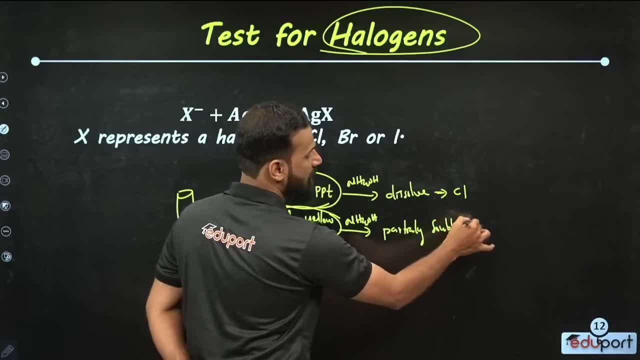 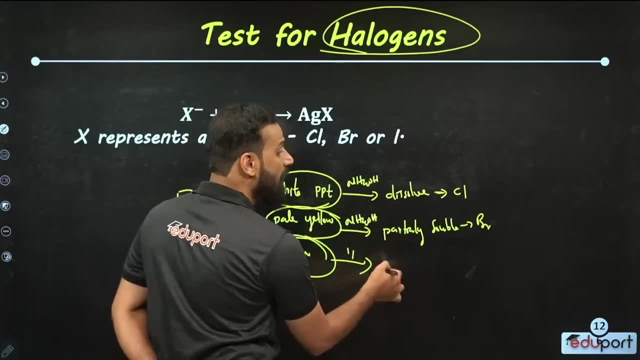 What is partially? If it is partially soluble, it indicates the presence of bromine. Now you are getting good yellow When ammonium hydroxide is added to it. if it is insoluble, what does it indicate? It indicates iodine. 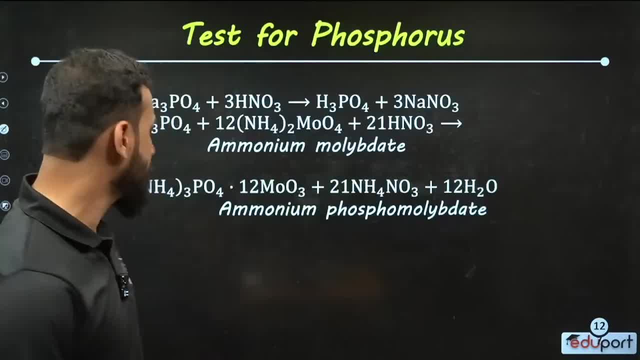 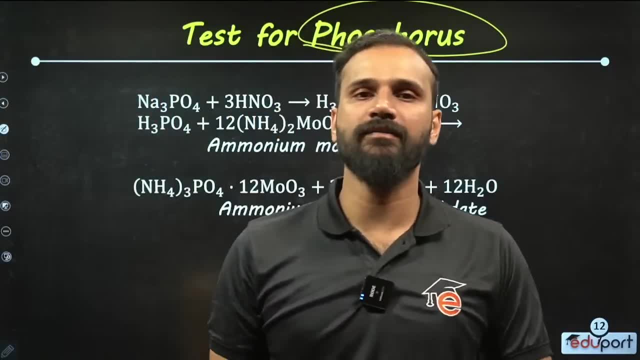 Chlorine, bromine, iodine should be learned. well Now, children. how can we identify phosphorus? There is nothing to identify phosphorus. What can we do? Add nitric acid. When we add nitric acid in the presence of hydrogen peroxide, 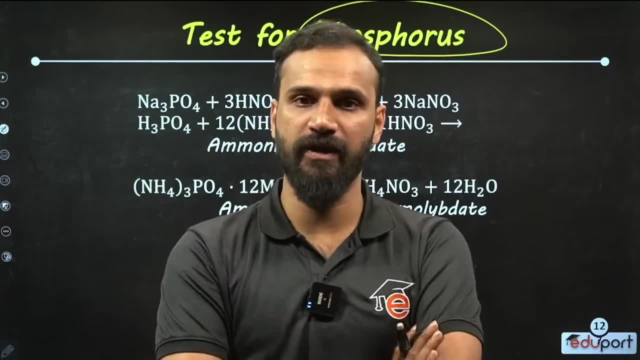 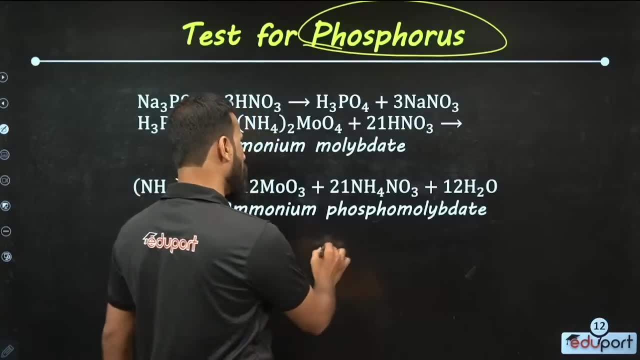 if there is phosphorus in it, it will turn into phosphate. We add ammonium molybdate to it. When we add ammonium molybdate, if we get good yellow precipitate, what do we get? If we get yellow precipitate, 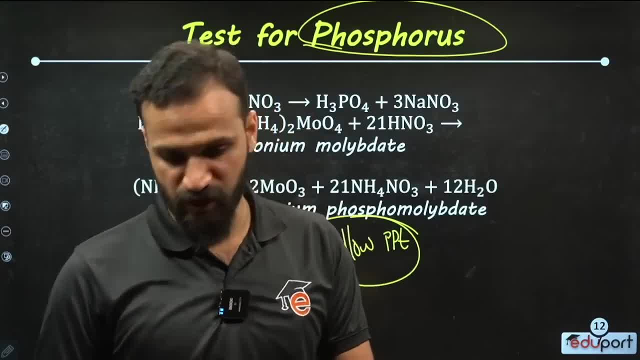 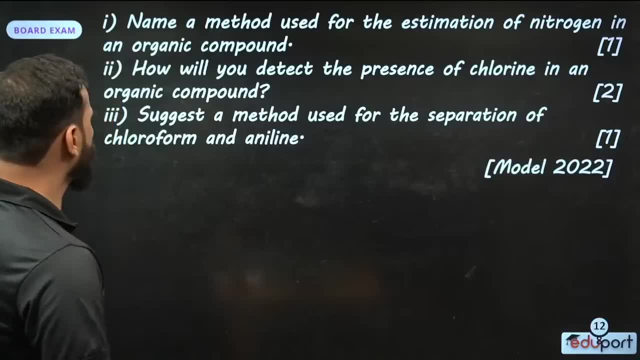 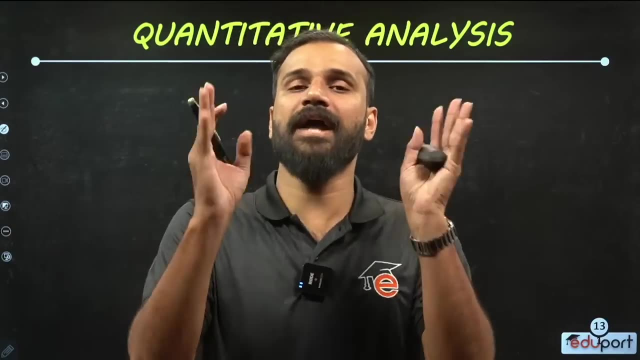 what does it indicate? It indicates phosphorus, So learn it. It is very important. Detection should be learned properly. Then look at the children. There is a question in that part, After that quantitative analysis. I am not saying it in detail. 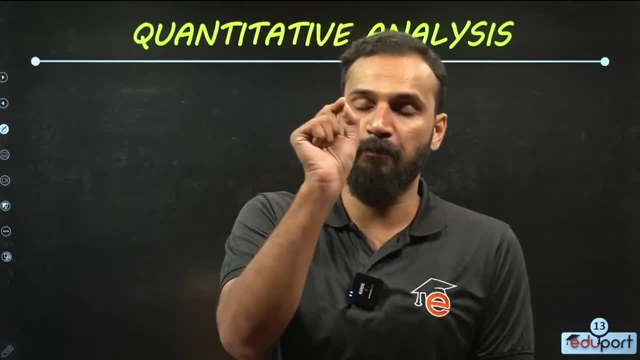 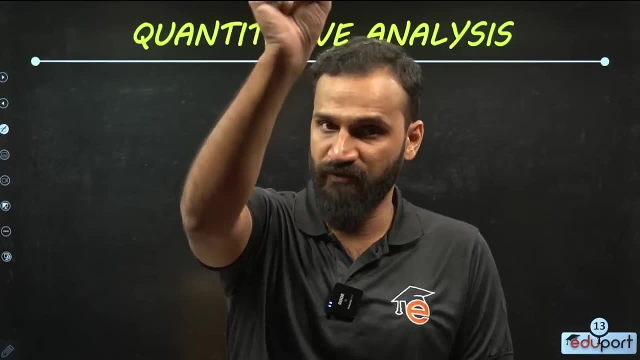 I have only one thing to tell you: To see the percentage of hydrogen in each method, to see the percentage of carbon, to see the percentage of nitrogen in Dumas and Zeldas methods. to see the percentage of halogen in Carrier's method. 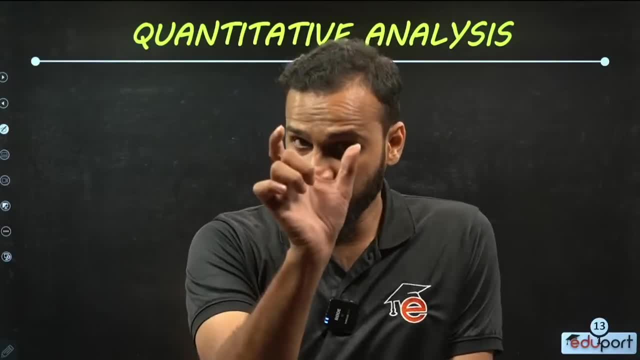 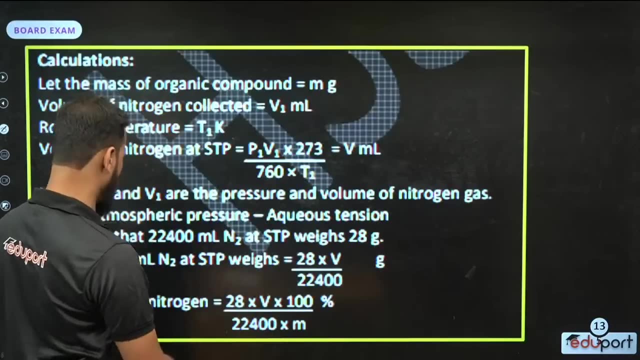 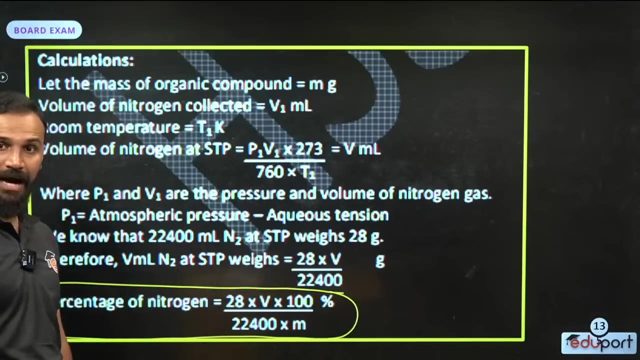 to see the percentage of oxygen, to see the percentage of phosphorus. there is an equation. The equation should be learned properly. Look at the equation to see the percentage of hydrogen. The equation is like this. Since the time is less, I will not explain it further. 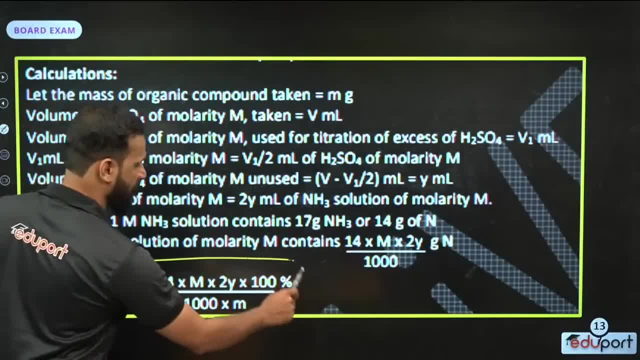 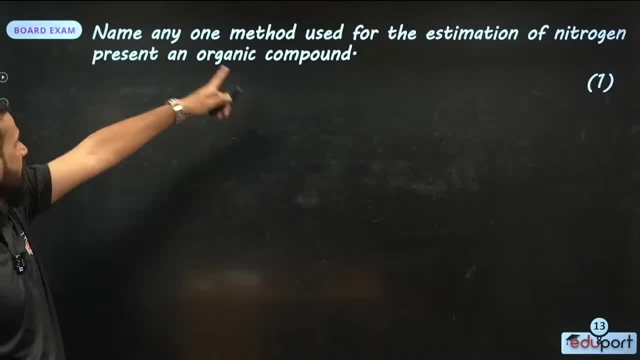 Write the equation. Learn the equation well. In the Zeldas method we also get the equation to see the percentage of hydrogen. We have to learn without seeing the equation. Then look at the children- Any method to see the percentage of hydrogen. 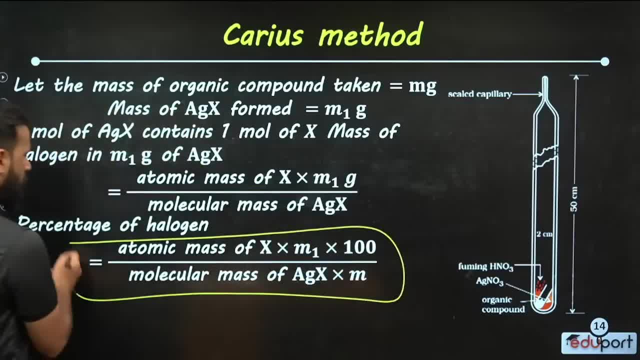 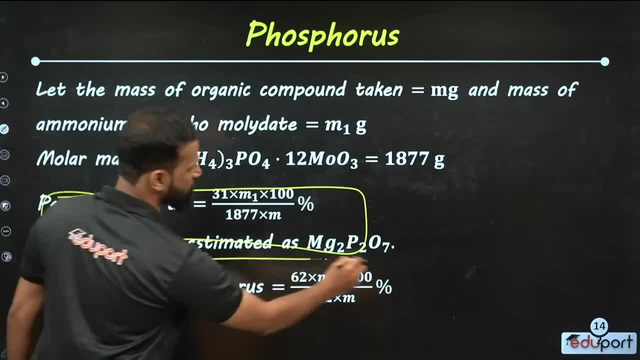 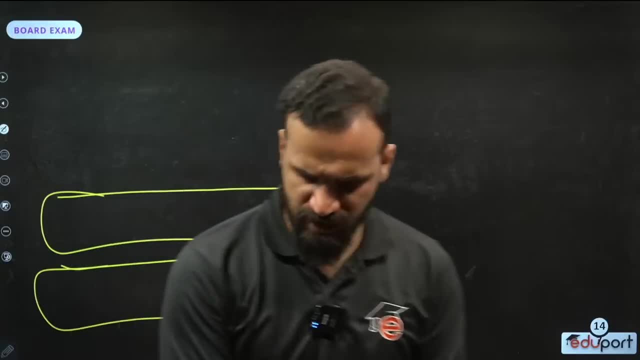 is asked: Dumas method, Zeldas method, look at it. Look at the equation to see the percentage of sulfur. Look at the equation to see the percentage of phosphorus. Look at the equation to see the percentage of oxygen. There are simple questions here. 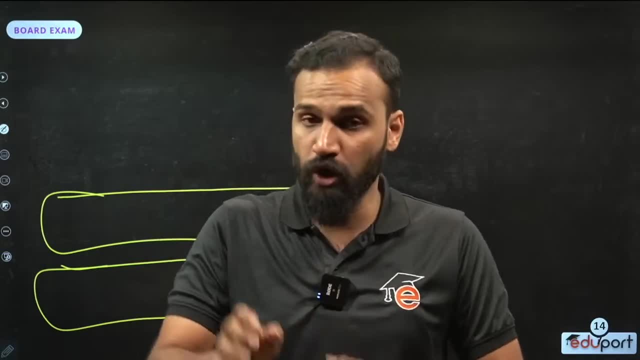 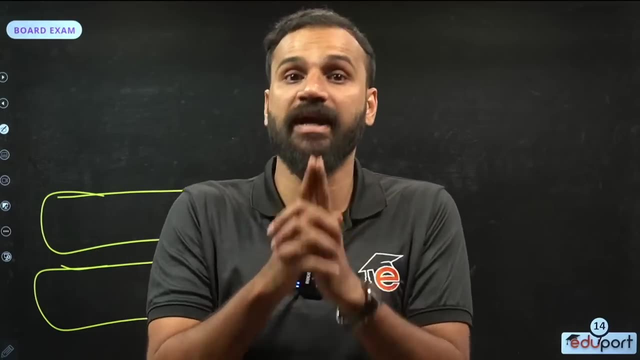 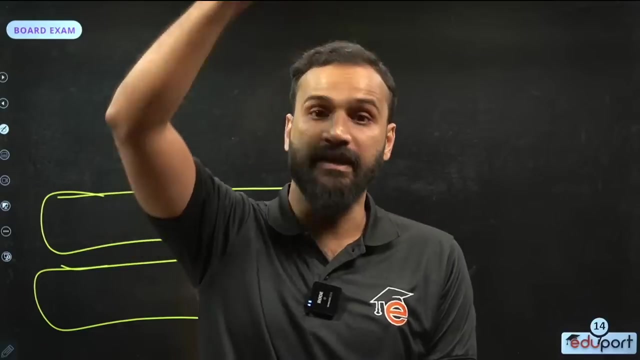 We have taken some time. What you have to do is to learn this chapter. well, We have gone a little faster in the last time, Since the time is over before the model exam. what is the organic chemistry coming again? We will come to you through our